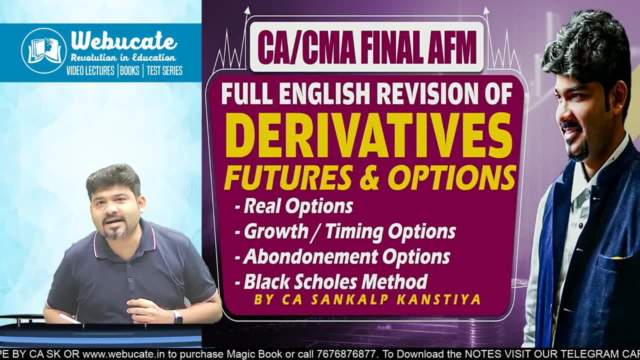 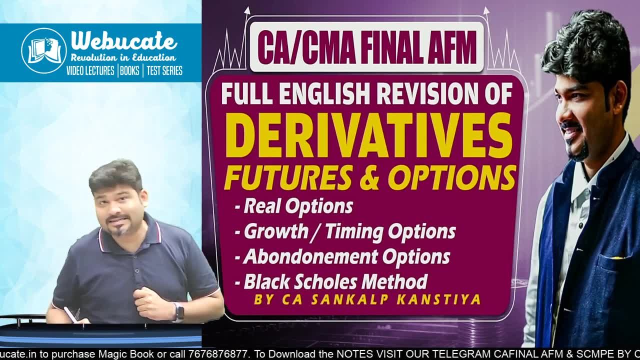 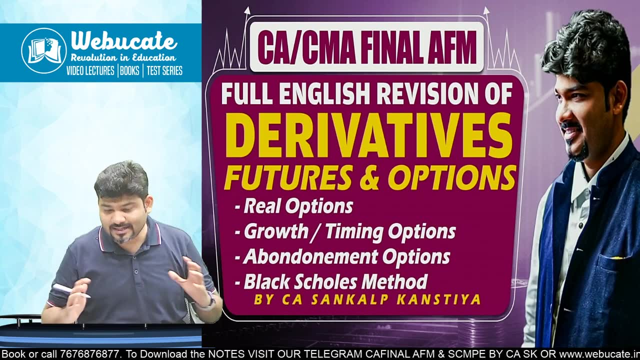 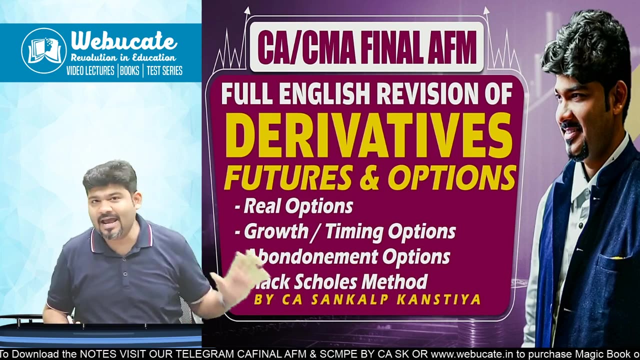 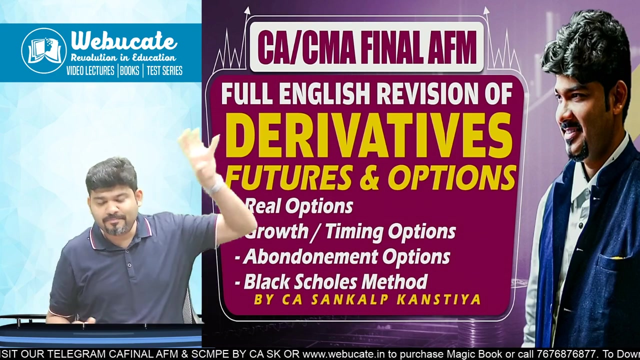 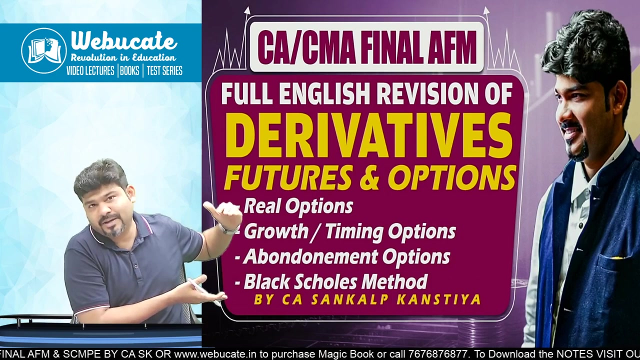 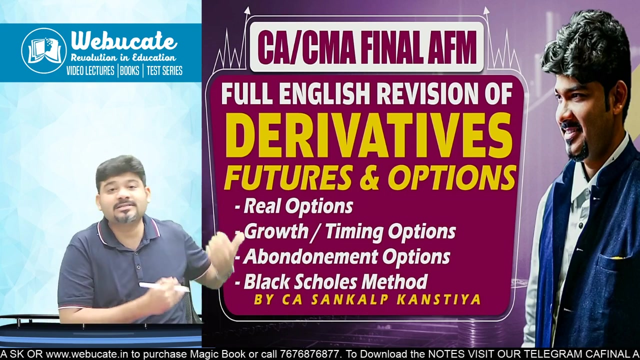 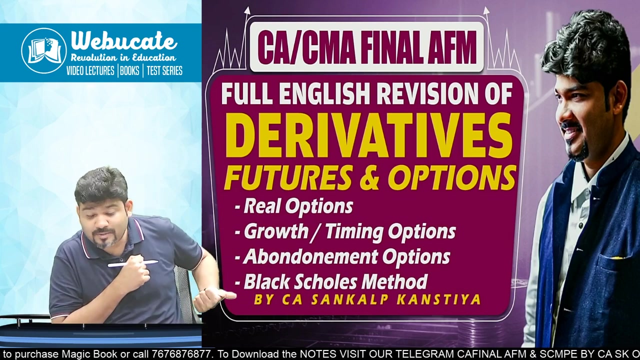 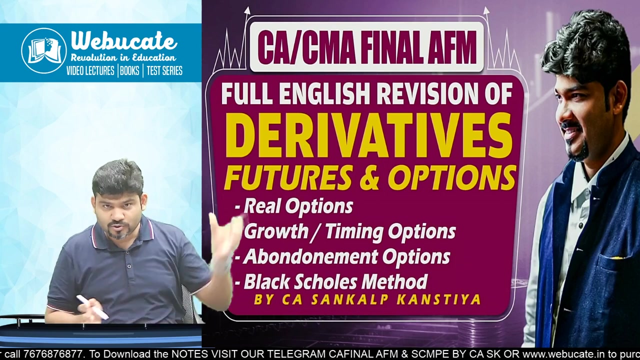 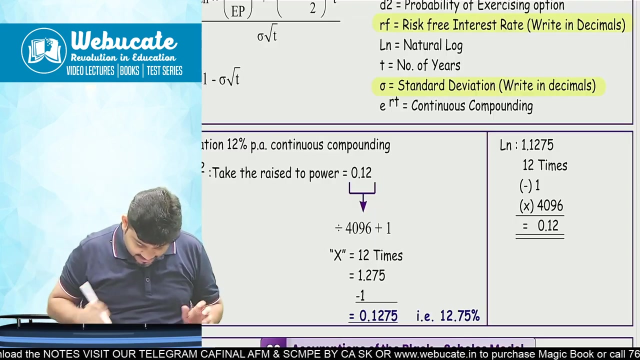 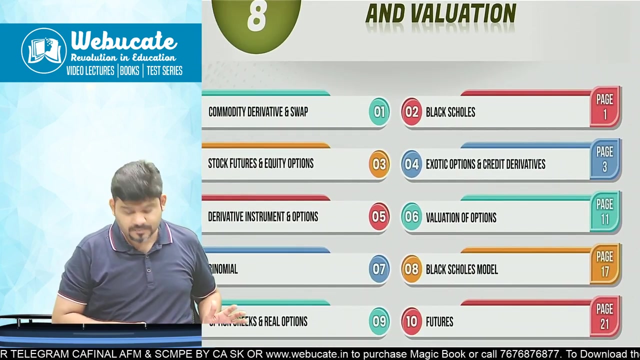 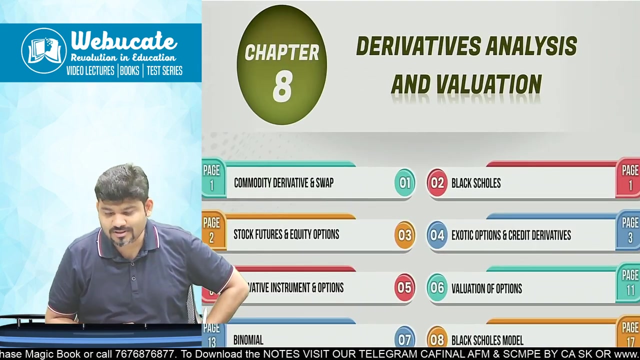 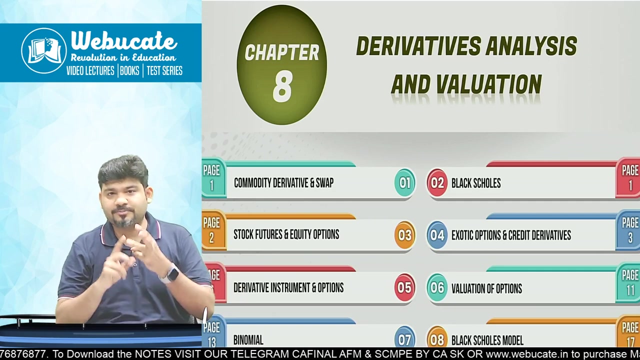 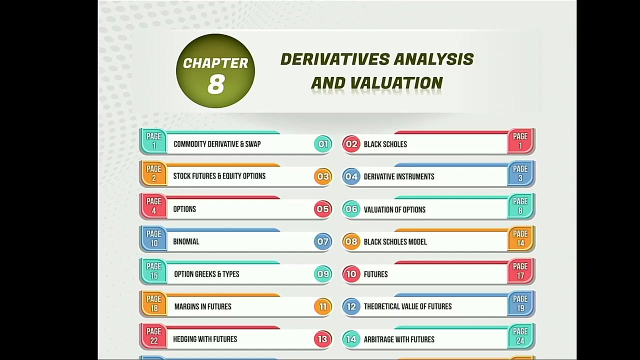 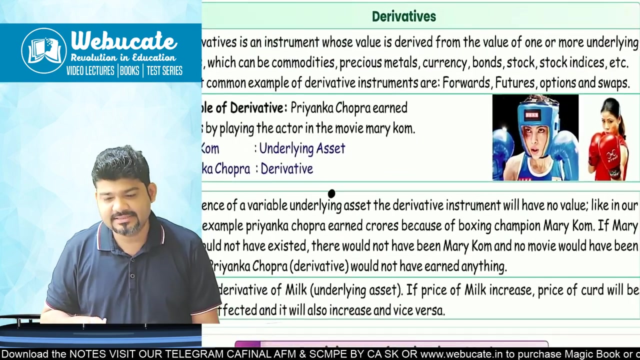 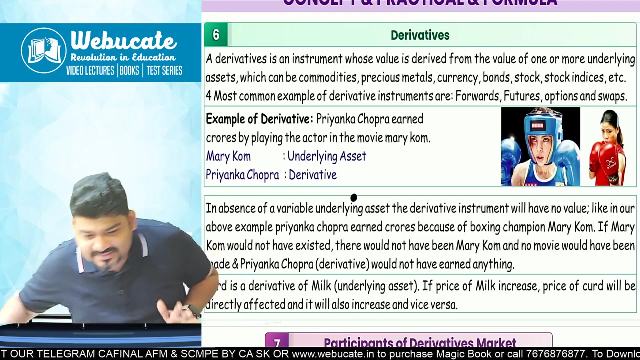 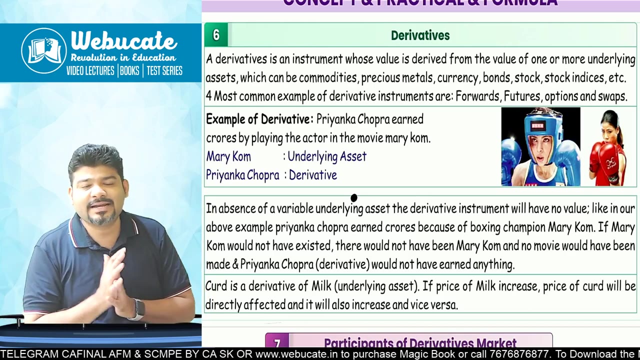 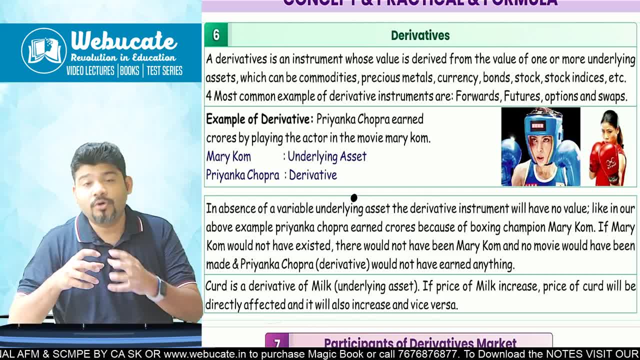 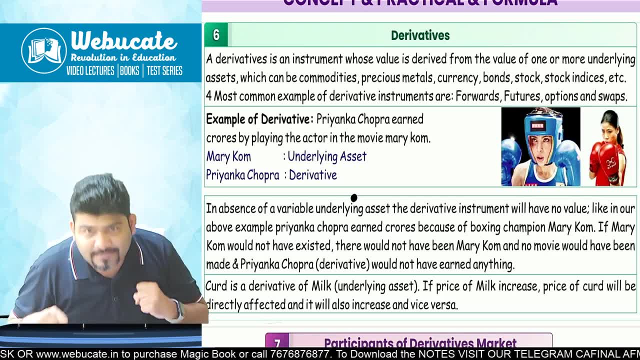 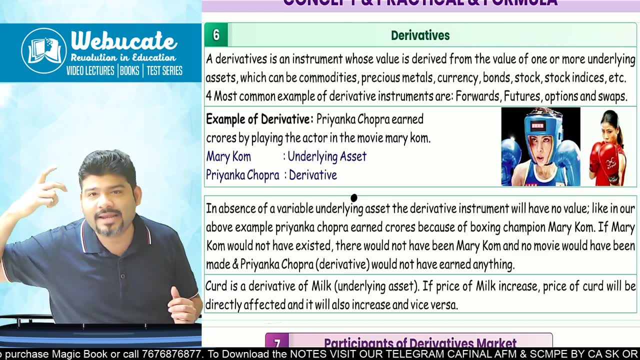 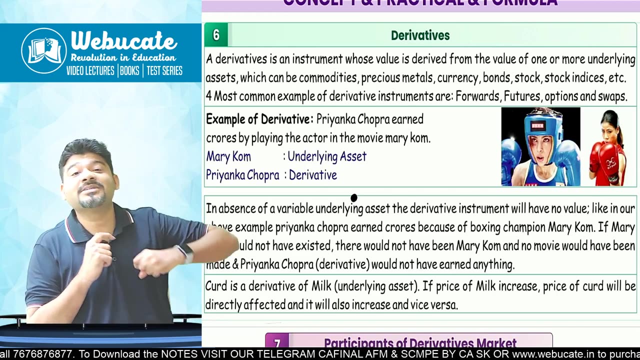 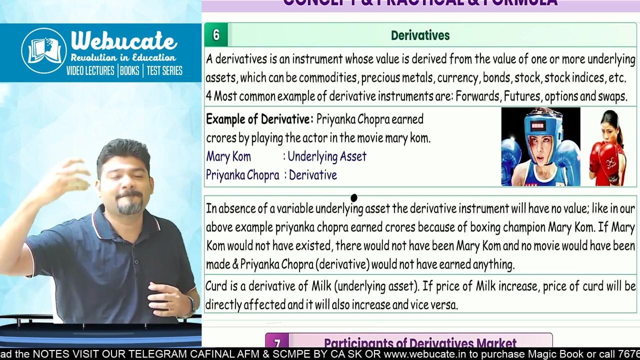 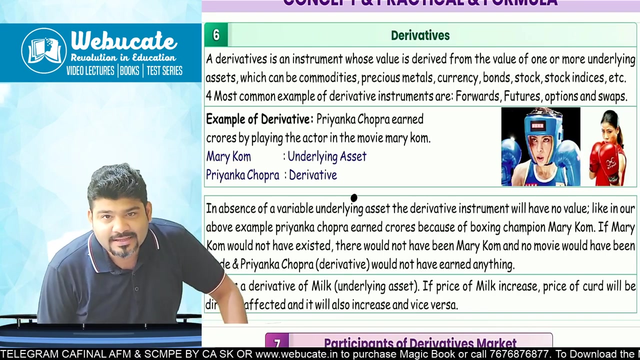 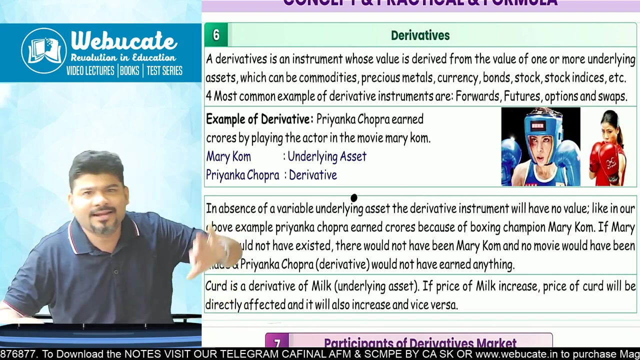 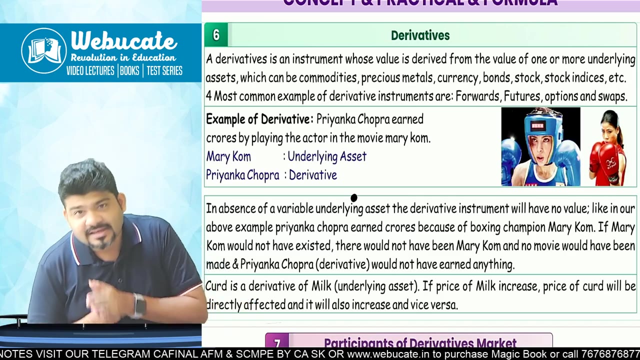 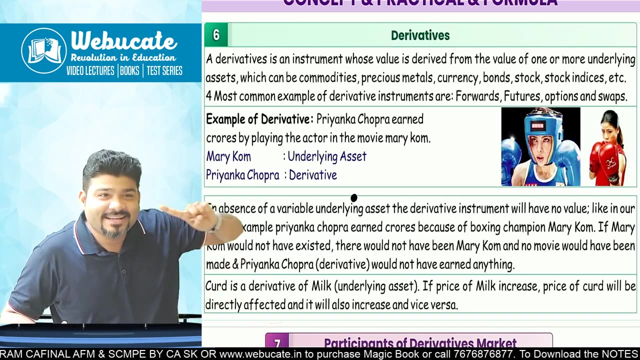 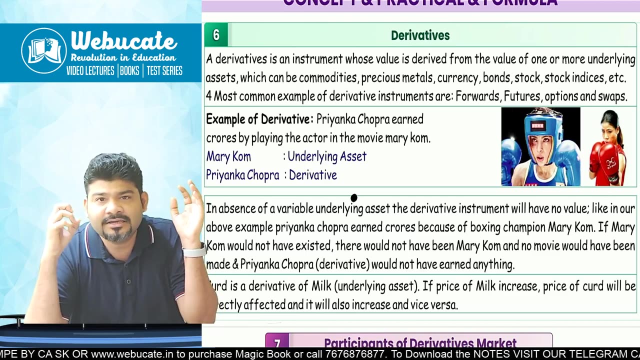 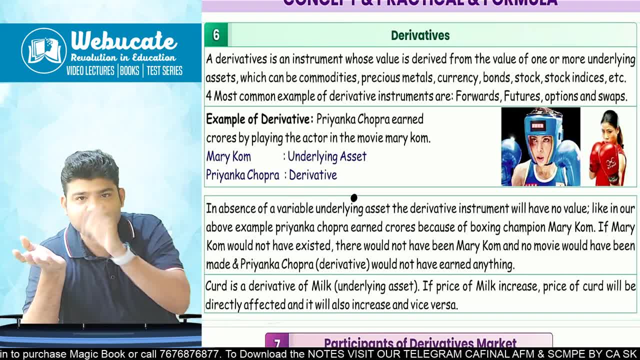 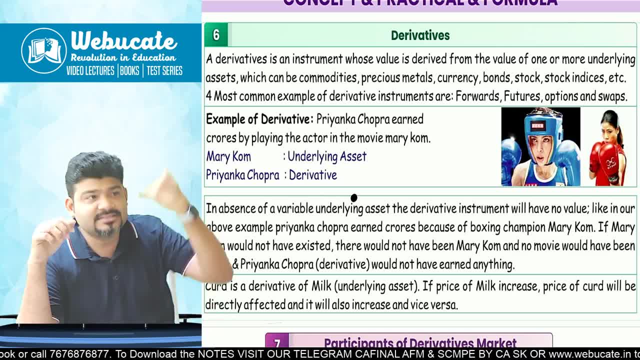 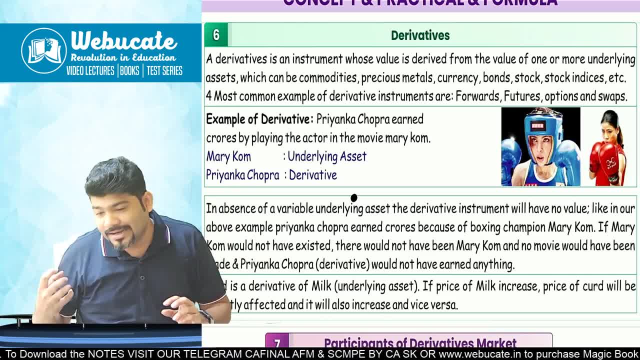 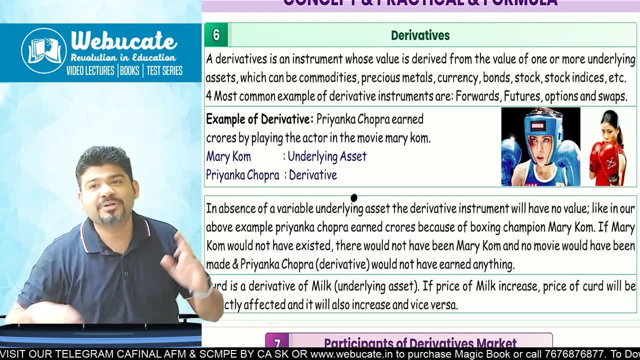 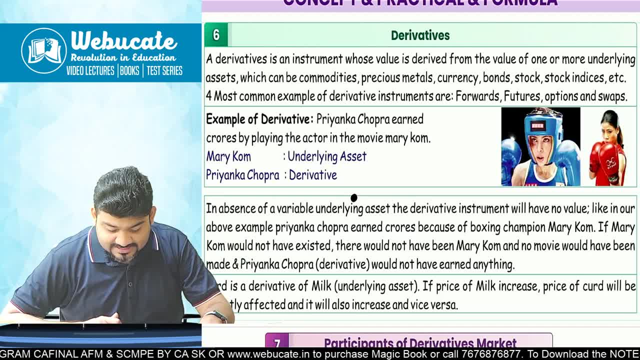 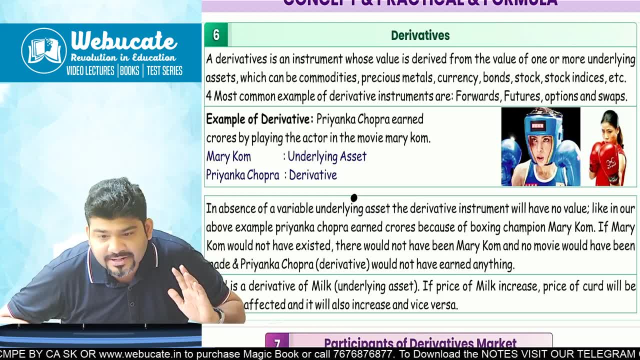 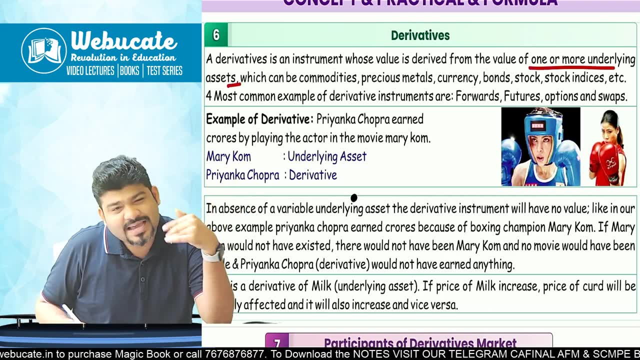 now of what is an underlying and what is a derivative, so that derivative is derived from the underlying and is also traded independently. let's see, a derivative is an instrument whose value is derived from the value of one or more underlying assets, which can be anything. so there 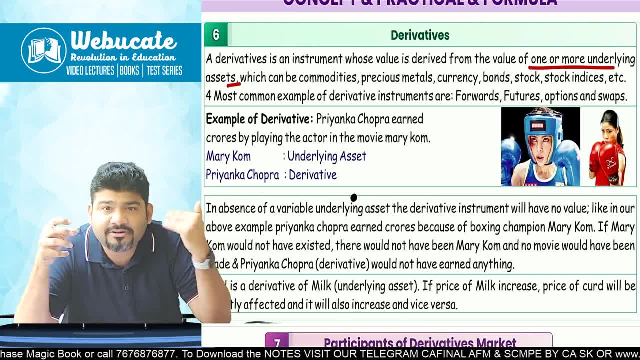 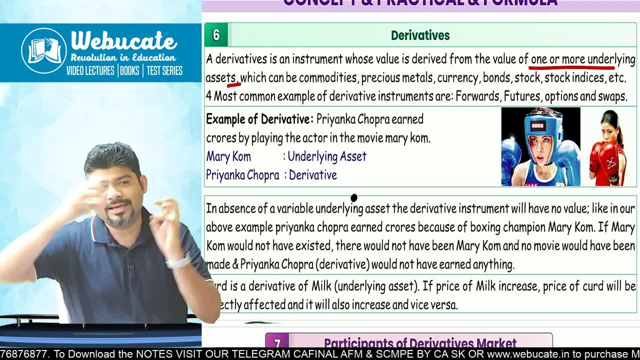 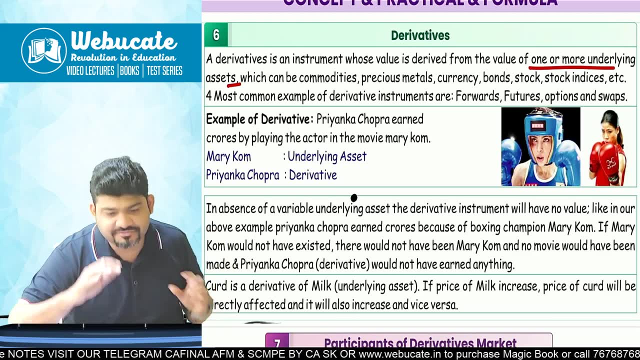 is a real gold and then there is a derivative of a gold. now there are various kinds of derivatives. what are they? that will will try and understand. but what exactly is the meaning of derivative? did you get it? yes, so there is an underlying asset, so please keep on confirming so there. 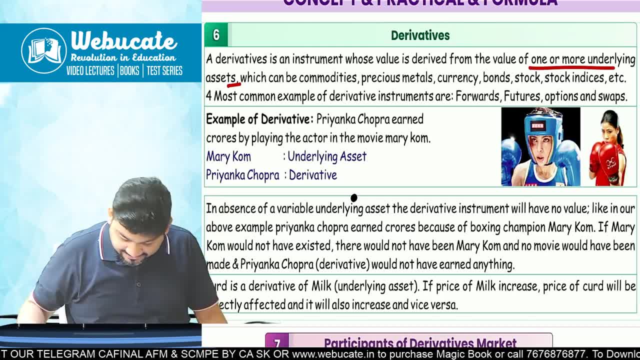 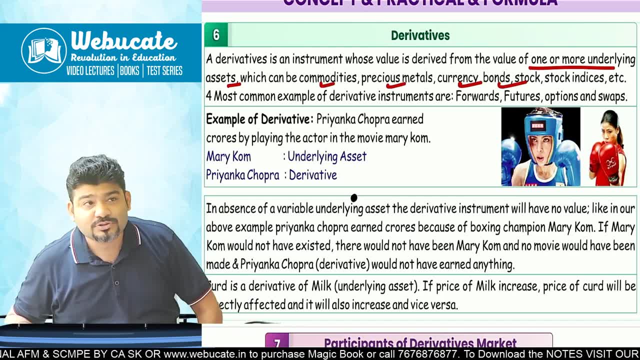 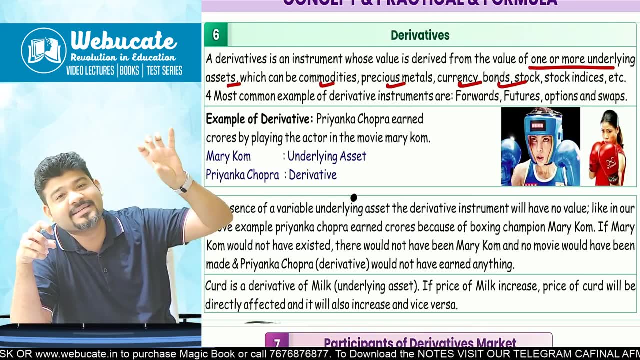 is an underlying asset and then there is a derivative who, which can be commodities, precious metals, currencies, bonds, stock, stock indices, etc. so what is stock index? so it is like a nifty. so nifty, nifty, nifty is the underlying asset and its stock index derivative is a nifty derivative right example. 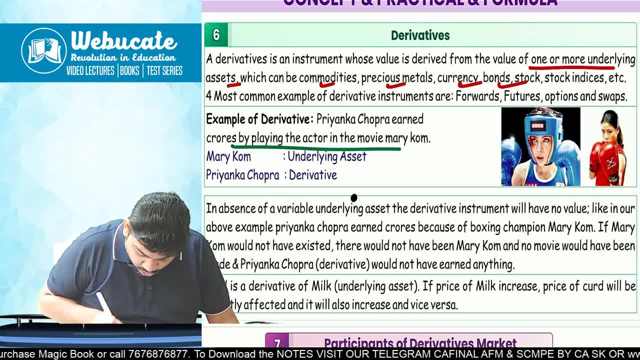 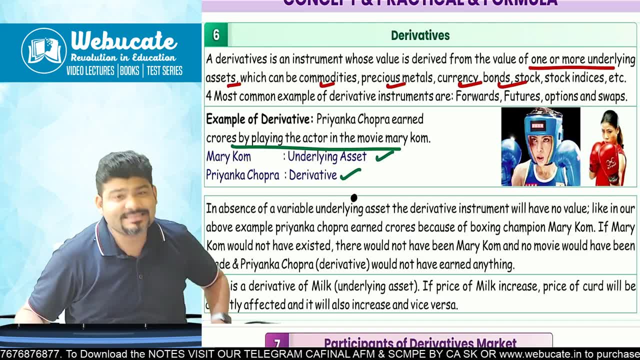 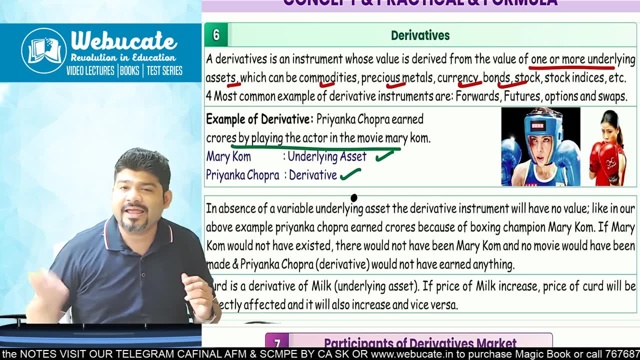 of derivative. as i told you, priyanka chopra earned crores by playing the actor in the movie maricom. maricom is the underlying asset, priyanka chopra is the derivative. can i say, without the underlying asset, the derivative will have no value whatsoever if maricom wouldn't have become so great and played. 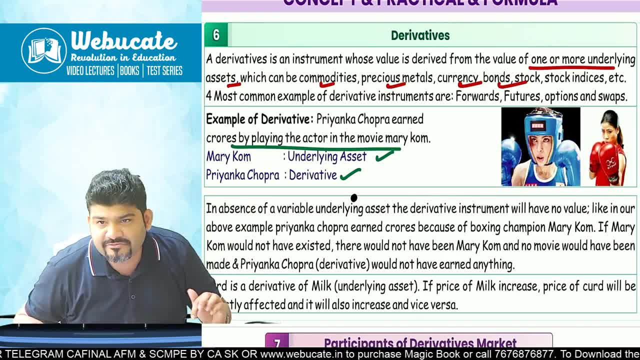 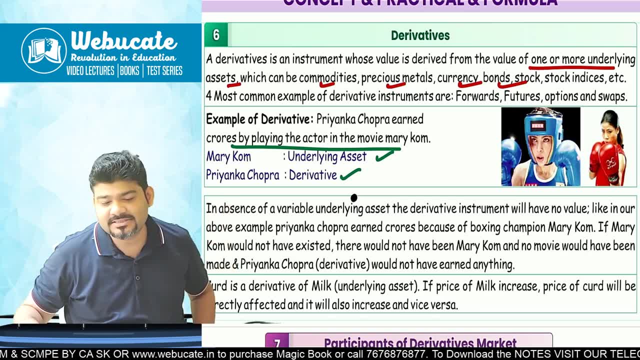 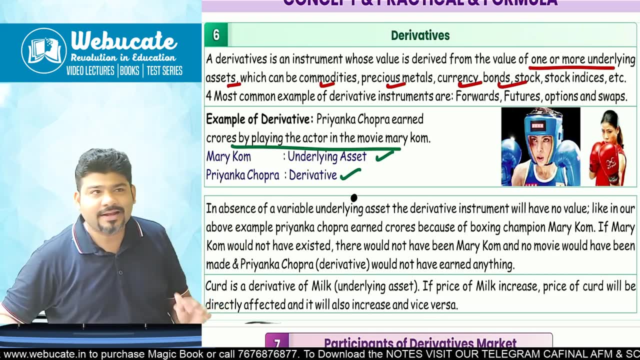 for india, priyanka chopra won medals, then do you think the movie would have been made? never can you make code directly without milk. never, right? so that's how it works. so derivative is always dependent on an underlying asset. say, for example, i will tell you that if virat kohli makes a century for rcb and rcb wins the ipl trophy. 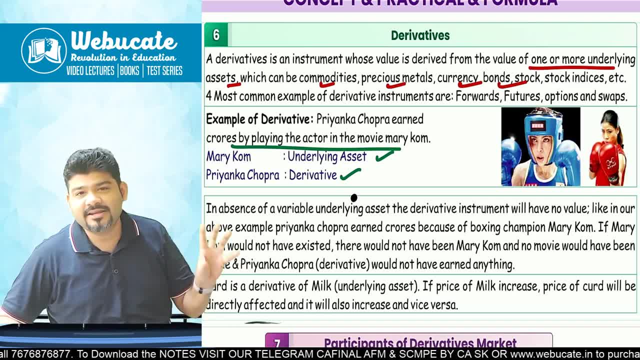 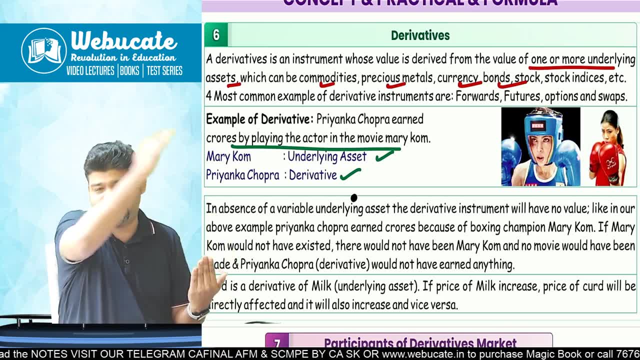 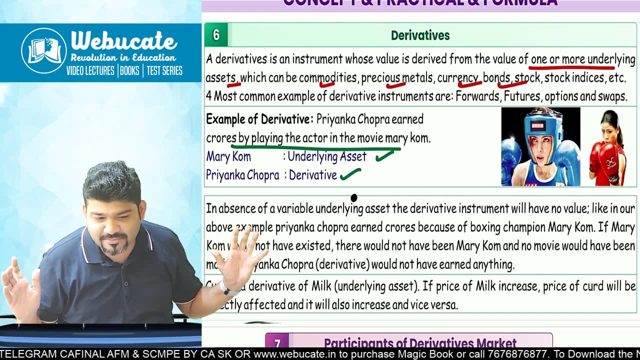 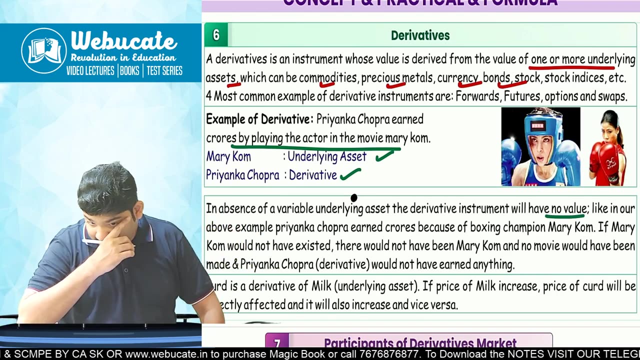 then i will give 100% discount on my lectures. so discount on my lecture is a derivative of the underlying asset: rcb winning the world cup. so that's what it is, everybody. yes, in absence of a variable underlying asset, the derivative instrument will have no value. like in our above example, priyanka chopra earned crores because of boxing champion maricom. if maricom would not have existed, there would not have been maricom. maricom and no movie would have been made and priyanka chopra derivative would not have earned anything. code is a derivative of milk. if price of milk increases, price of code will also be directly affected and increase and vice versa. and there is a direct connection because the derivative is based on the underlying asset. the change in the underlying asset will impact the derivative as well. right, and this change is based on the real market change of milk. prices of milk increase. what will happen is the derivative will change the levels of theρω. 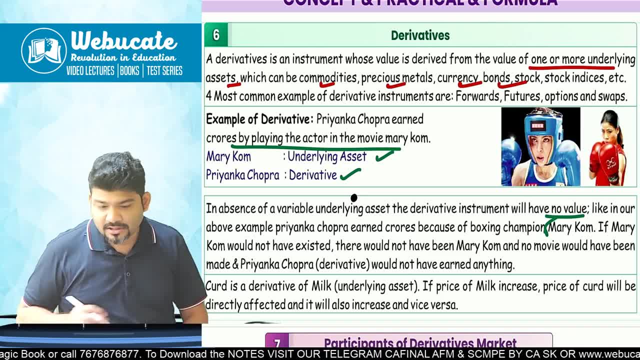 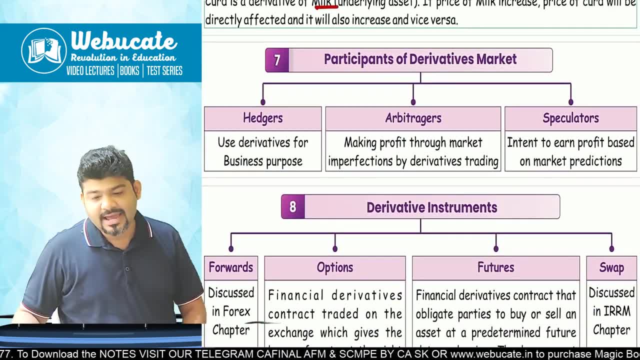 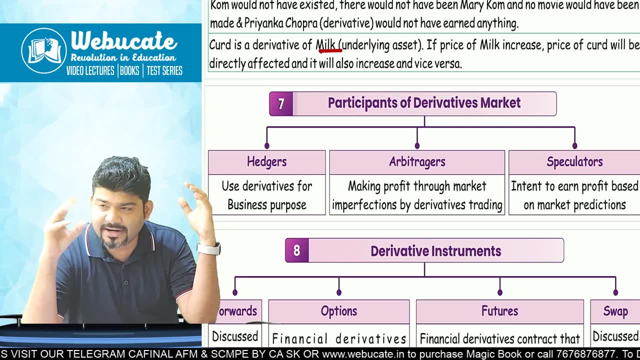 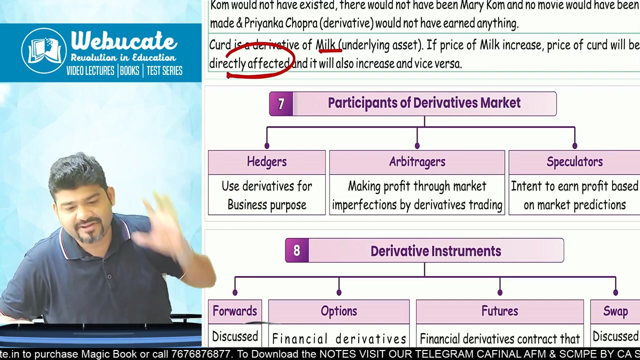 pure Loki 1: 97 rep. Octo. AC 1: 7 happen to the prices of curd. correct but obvious. the prices of curd will also increase, will have a direct. the derivative will be directly affected. okay, what are the participants in the derivatives market? so there are three kind of participants in the derivative market. one is called the hedger. 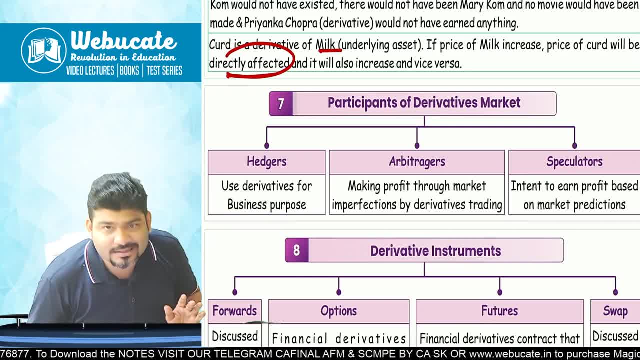 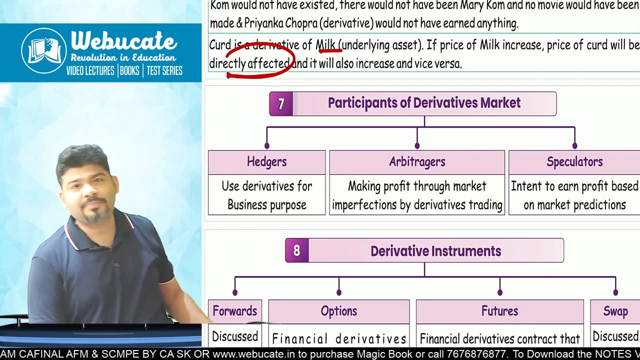 the other is called as the arbitrator. and then there are the speculators, the first one being the hedgers. now, who are the hedgers? these are the real businessmen right say, for example, i am a adani or i am ambani, i have sold goods worth rupees ten thousand crores, or worth dollar one. 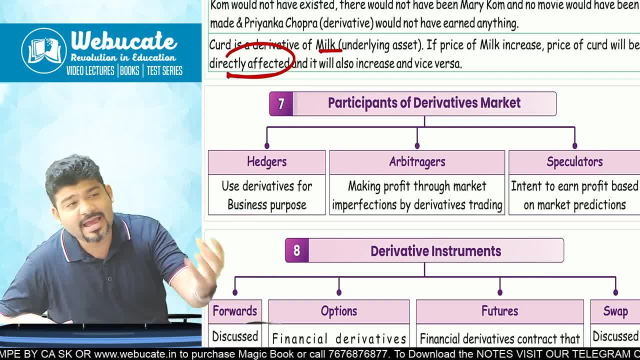 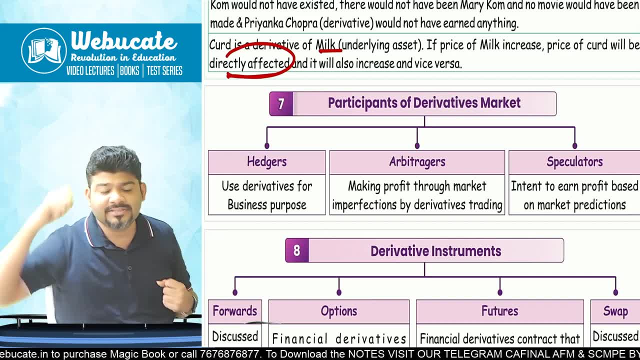 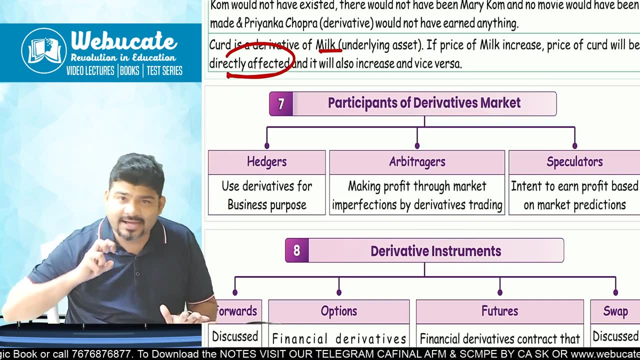 lakh. now, after three months, i am going to get a dollar one lakh. but i am afraid what if the prices of one dollar two rupees fluctuate? then i will want to cover myself in the derivatives market. so the underlying currency rate will be there. that is the underlying asset, but i can enter. 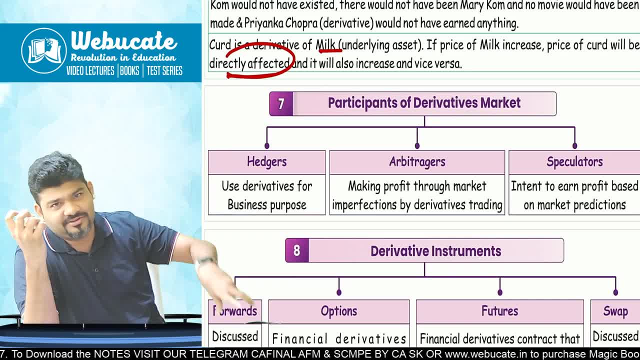 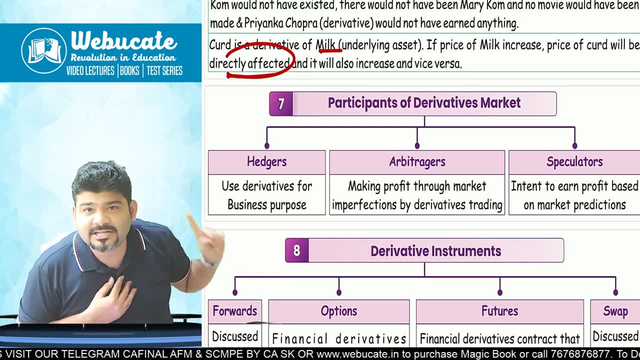 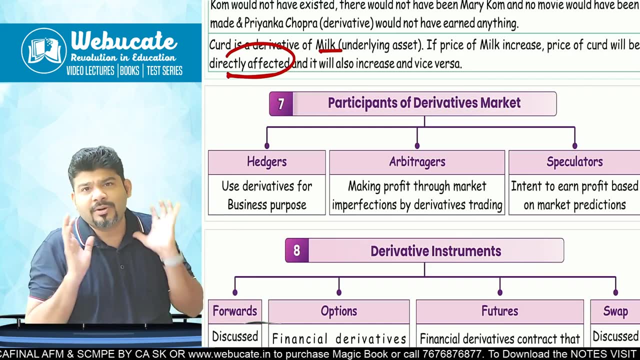 into a derivative and protect myself from the currency fluctuations. that is called as hedging. so i have used it for a business purpose. suppose i have to pay five lakh dollars after three months? now, if i have to pay five lakh dollars- today's rate is one dollar equal to 80- i have to pay. 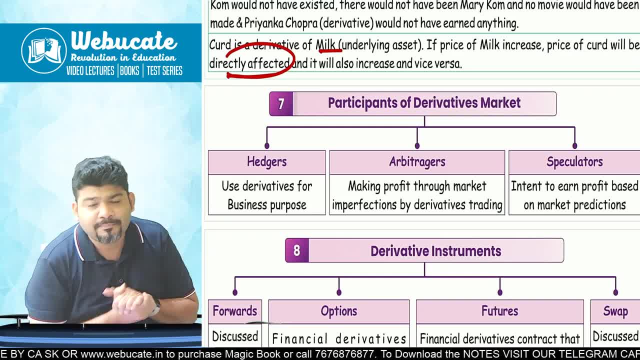 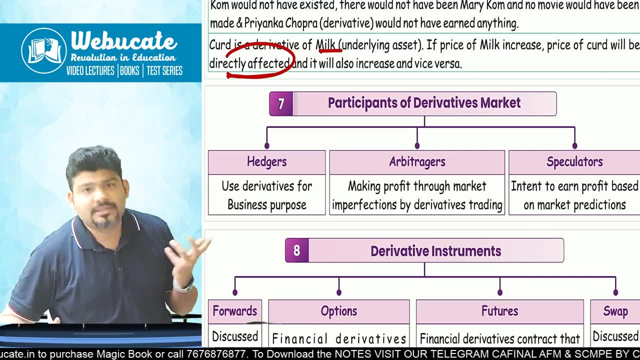 five lakh dollar. according to that it will be four crore rupees, but that rate is two is today. i have to pay after three months. what will happen to one dollar equal to 80? will it remain? the answer is no. what if it goes to one dollar equal to 90? then in that case it will. 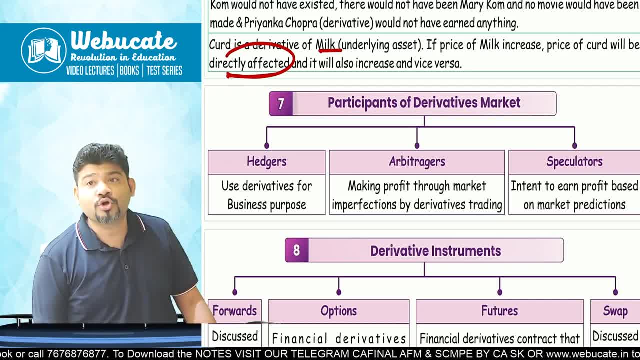 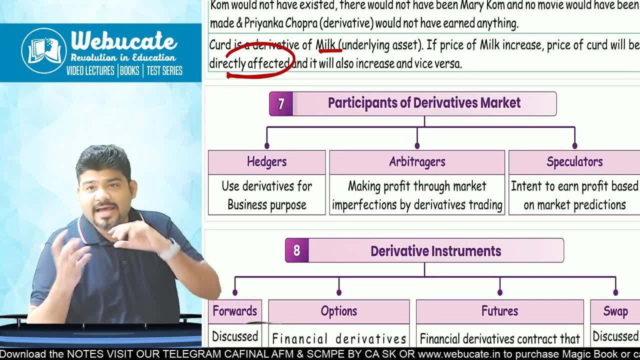 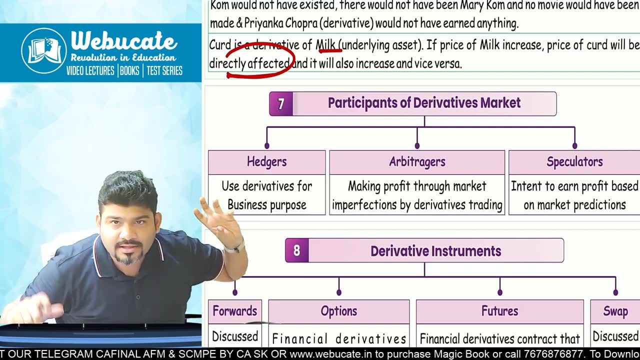 become four crore fifty lakh. oh boy, four crore fifty lakh, yes, instead of four crores, so that fifty lakh can be a loss to me. i want to hedge that i can go into the derivatives market. what is hedging? protecting myself from the risk of that currency fluctuation. so i will go in the 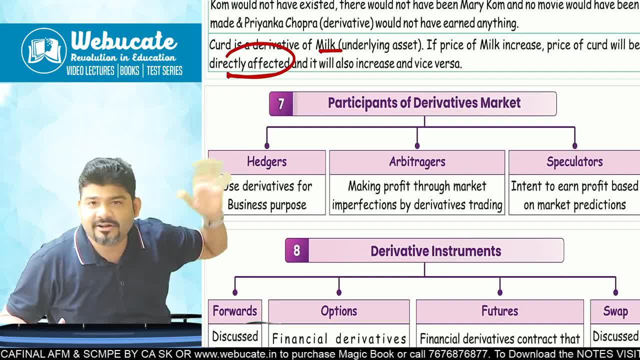 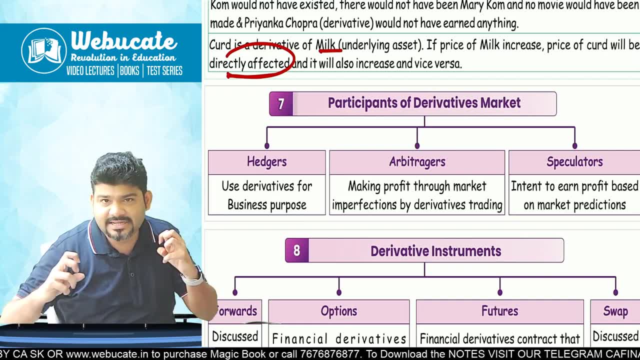 derivative market and i will go into the derivatives market and i will go into the derivatives market and i can ensure, kind of ensure myself- that basically is hedging. i am using it for my business purpose because there is a business deal and i want to correct you know. 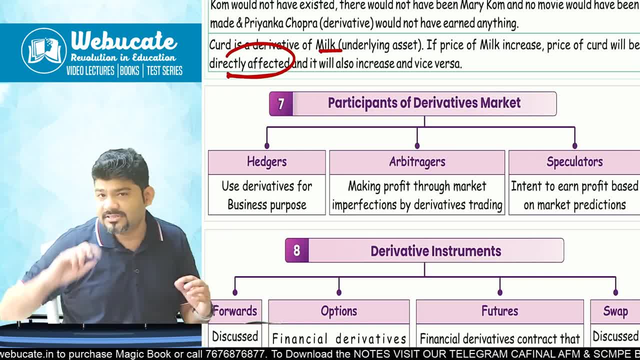 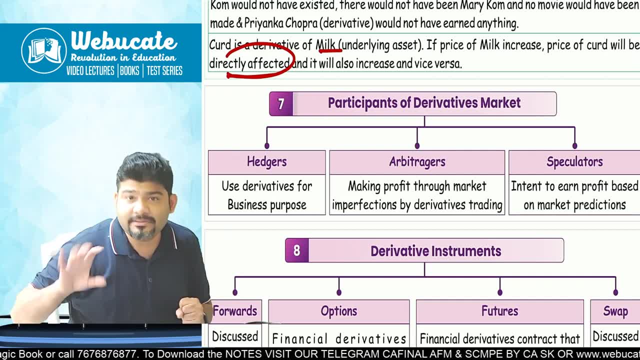 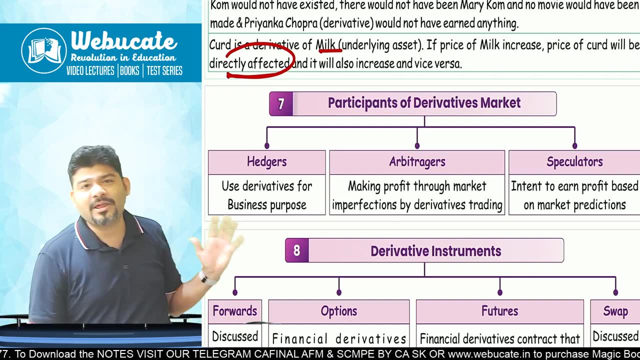 save myself from that dollar currency fluctuation. this is just an example of currency. it could be anything else. so if i am using the derivative market for protecting myself from a loss in my business, it is called as hedging right now, suppose people like you and me who have no business 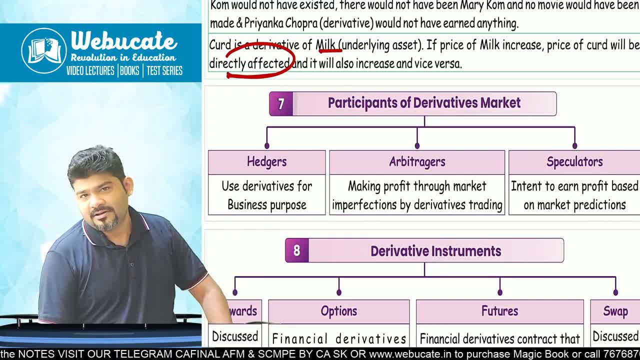 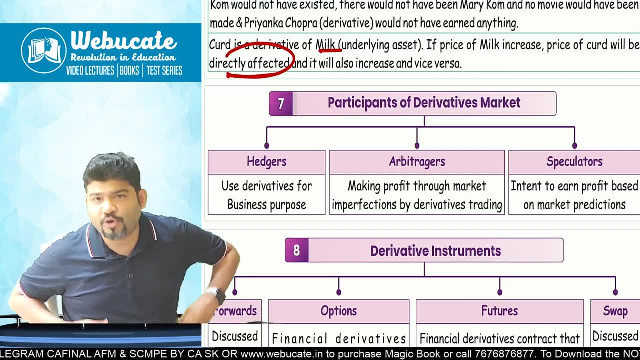 with me. i am using the derivative market for protecting myself from a loss in my business of currencies or any other business. we don't have a business of trading in shares or anything. we are just students studying. but i want to trade in shares and want to earn money from the derivatives. 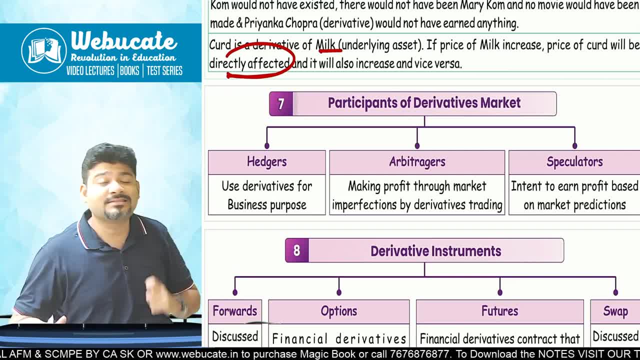 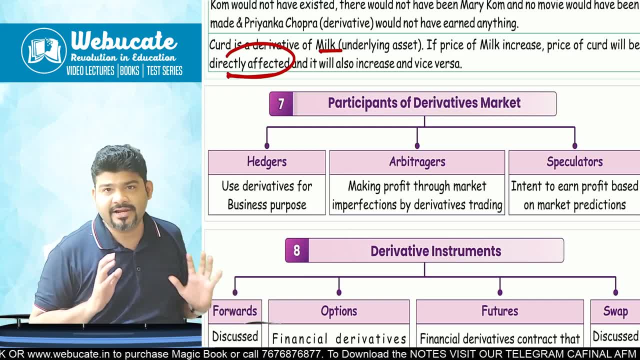 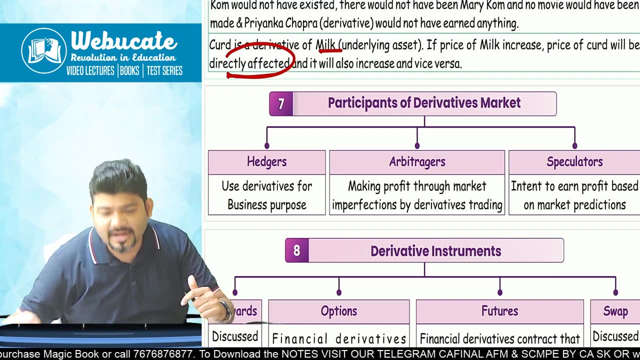 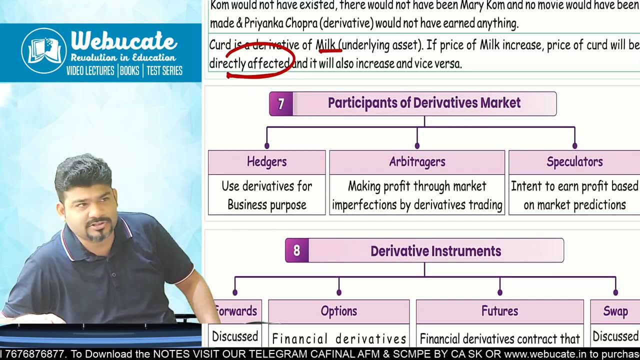 market. okay, then we will be called as the speculators. we will be called as the speculators. we want to earn money from the derivatives market without having any business interest whatsoever, and we are basically relying on our gut feeling. so that is called as a speculator. that okay. i feel that the market will increase because of this. this. 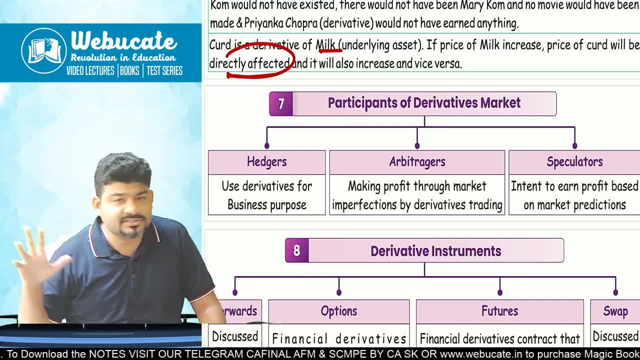 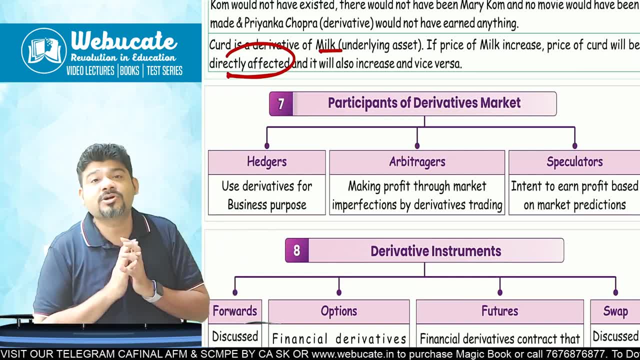 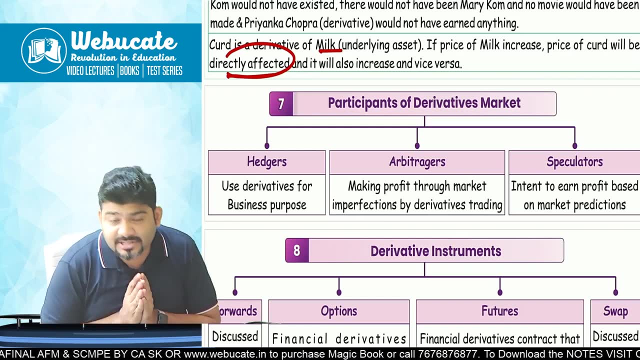 that, that i feel that the market will go down because of this, this, that that, and based on that, i take a position, a buy position or a sell position, as the case may be. that is called as speculation. got it guys done. and then there is arbitrager. who is a arbitrager? arbitrager is a person who 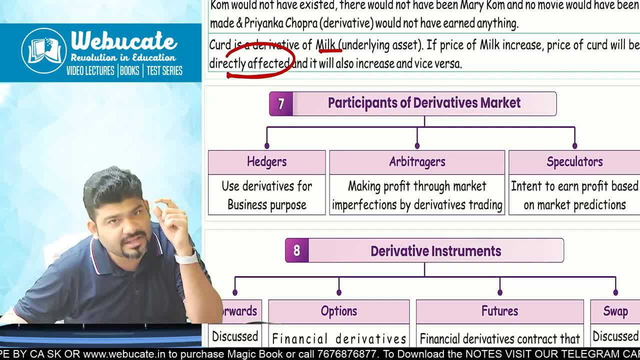 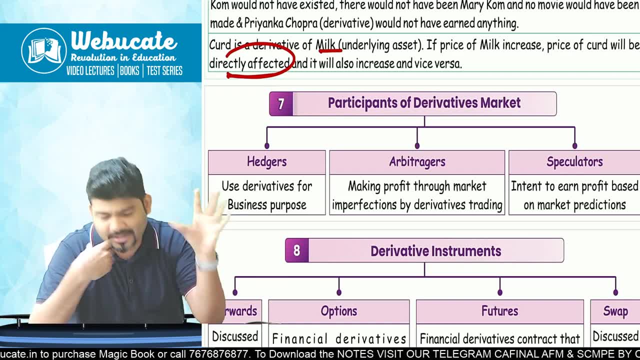 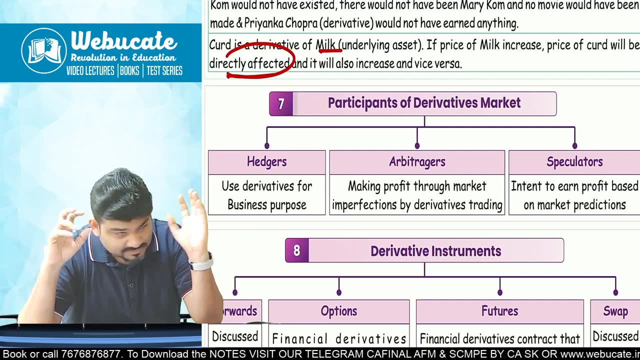 will make a risk-free profit. he knows that the derivatives market- in the derivatives market, the price of gold is, uh say, one dollar or 10 grams is equal to rupees 75 000 in one market. or let's take a simple example of equity share: equity share in the 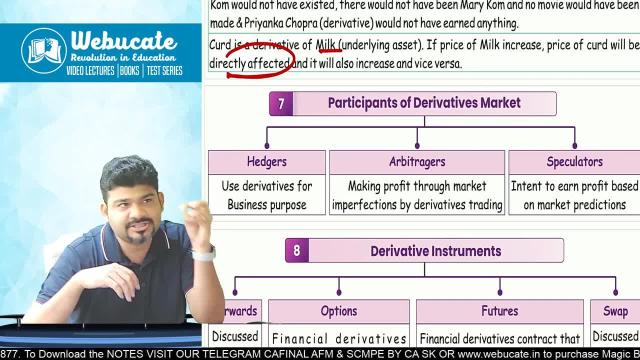 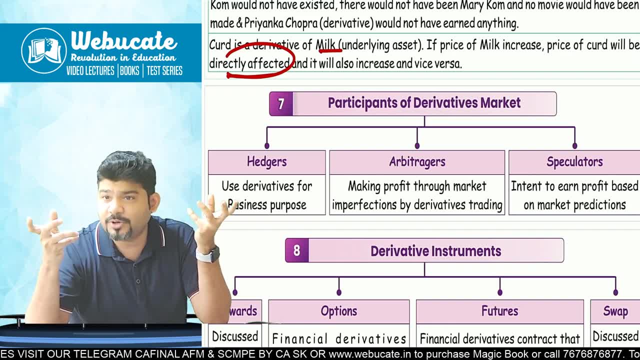 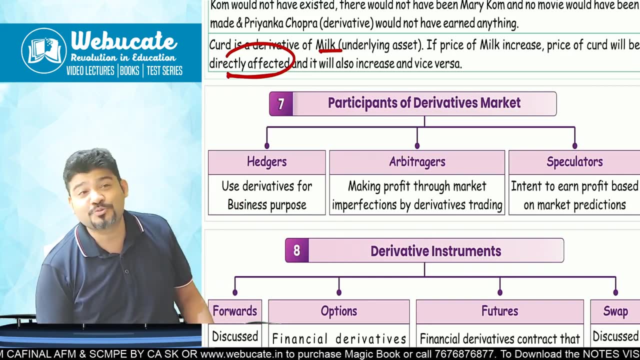 national stock exchanges. one uh equity share equal to rupees 2500 of reliance and in bombay stock exchange it is 2550. is that a possibility? yes, so what i will do? i will buy in nsc, i will sell in bsc. yes, that is also possible. so can i say i will make a risk-free profit of 50? that is what. 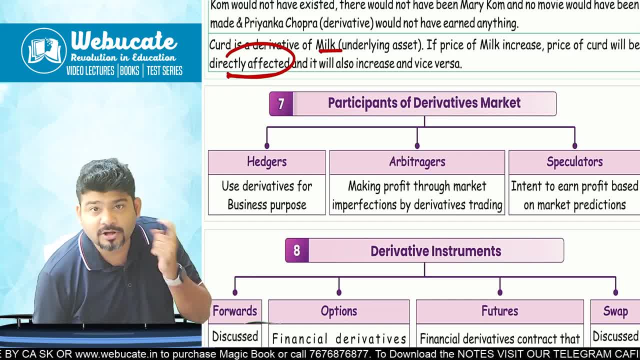 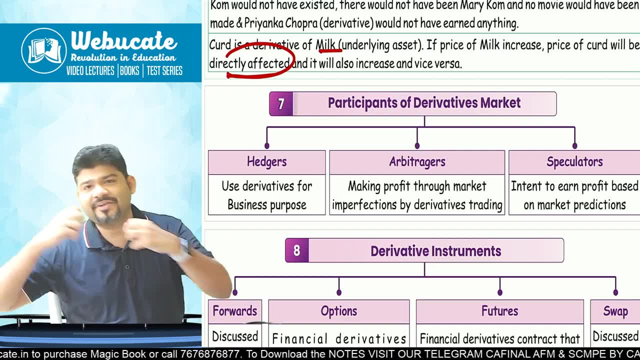 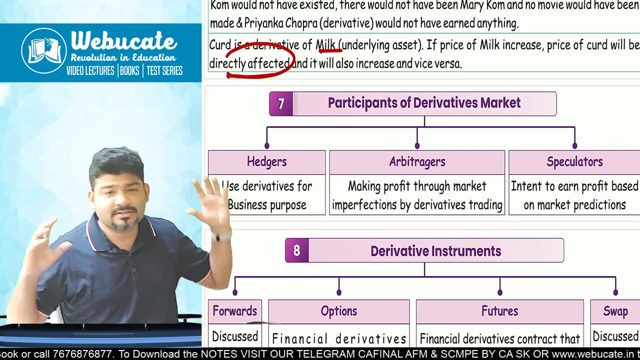 arbitrage does. utilizing the benefit because of market imperfections is called as arbitraging. so your derivative market, if it is imperfectly priced in two different markets, the same asset, you can use the benefit of arbitraging. so these are the three participants. it comes in the 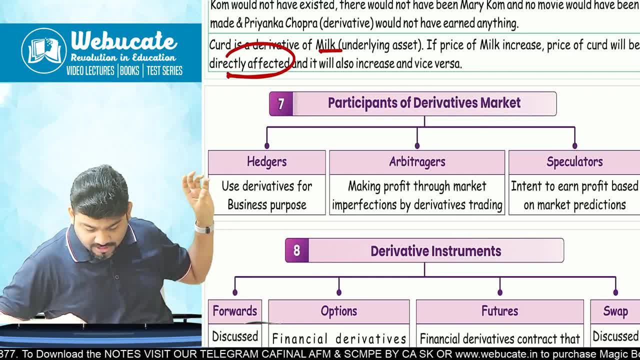 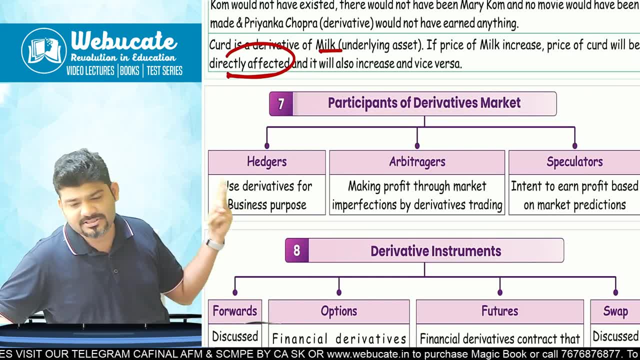 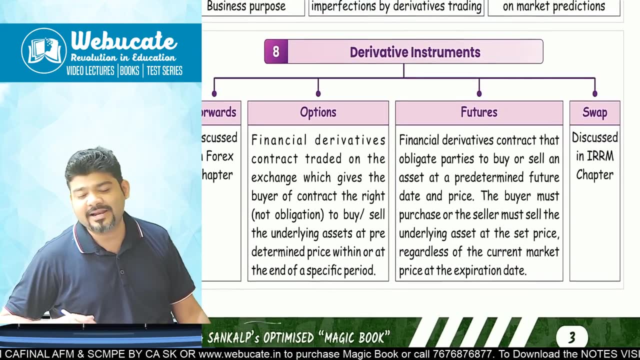 examination. that's the reason i explained you in detail. so who is a hedger? a hedger will use it for the business purpose. arbitrager will see a riskless profit opportunity and start. and speculator is a one who, just you know, speculates kind of and tries to earn profit out of his market predictions. 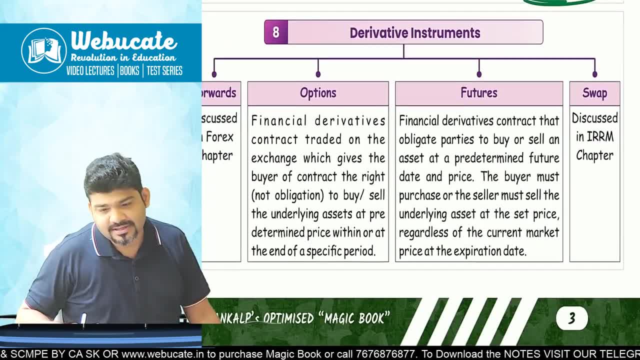 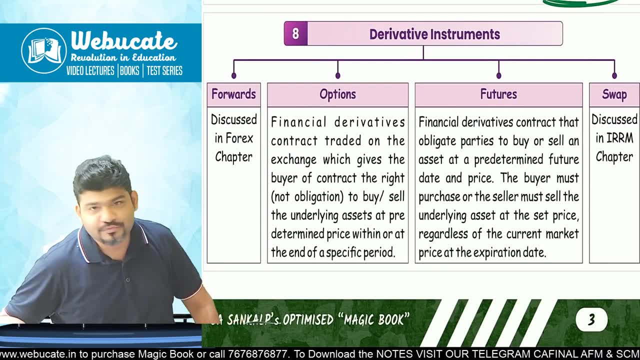 based on his market predictions. gotcha everybody. yes, sir. then we have the next thing, and that is called as derivative instrument. so now, sir, we are very excited because we want to be a speculator. some may say, sir, i want to use hedging for my father's business. 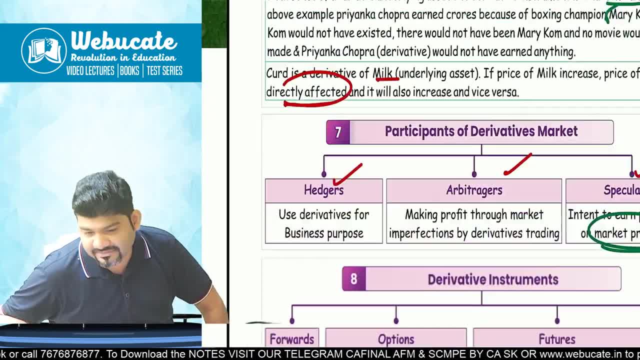 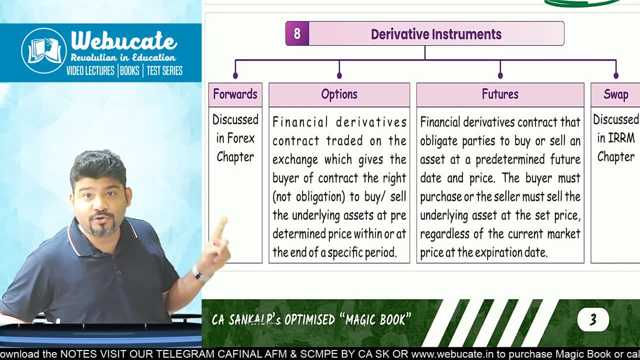 then there are arbitragers, so i want to use my derivatives market. so in this derivatives market, there are four instruments which we are mainly going to study. one of them is forwards. yes, forward is also kind of a derivative instrument and you are using it for hedging, but that is. 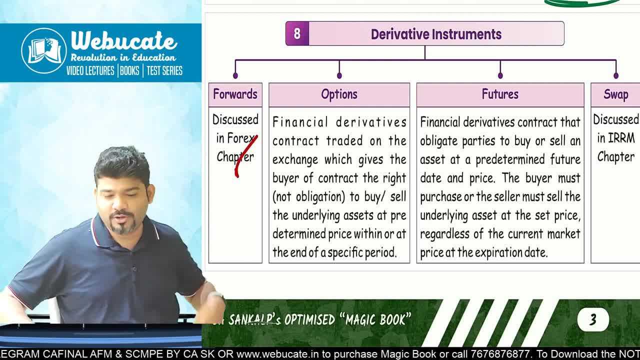 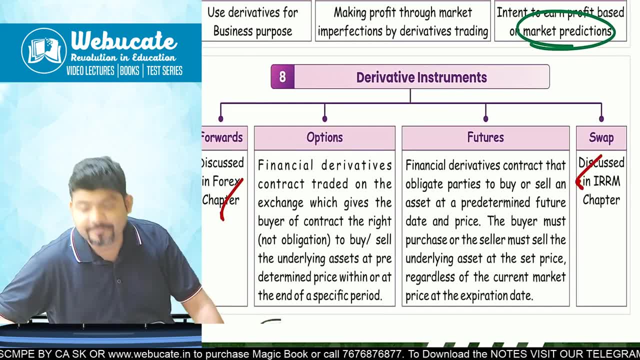 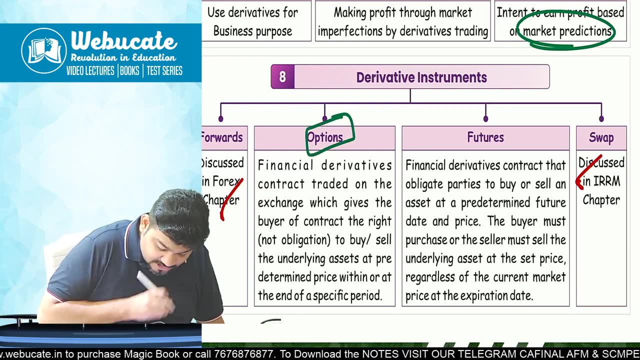 discussed in the forex chapter. you have to comment and tell me whether you want the revision for forex chapter. yes, sir. then comes the swap. can i say? the swap is discussed in irrm interest rate, risk management chapter. so now we are left with the two chapters options and futures. now we are left with two chapters. options, uh, two. 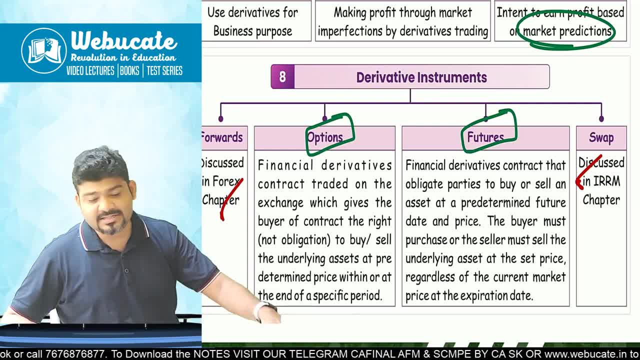 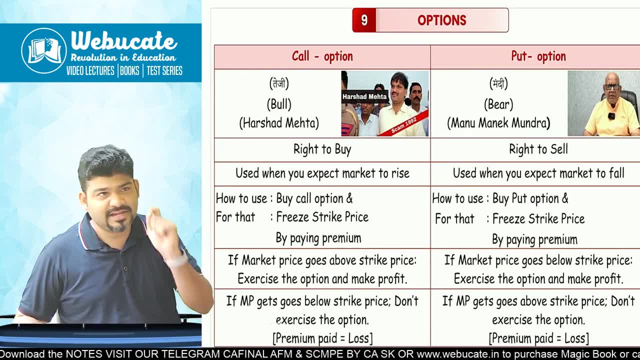 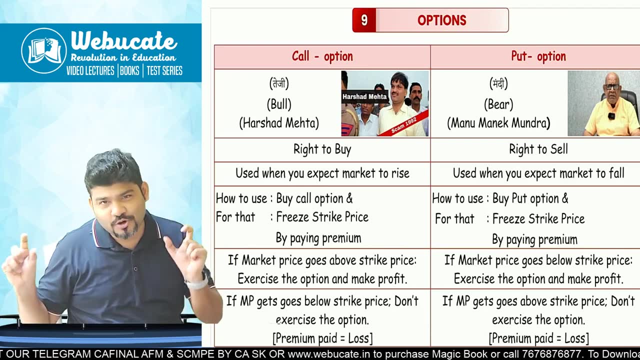 concepts: options and futures. so let's start with our first concept and that basically is called as the options market. so first derivative that we are going to study is options. second derivative that we are going to study is futures. for the remaining two options, there are separate chapters and that we will do when we pick. 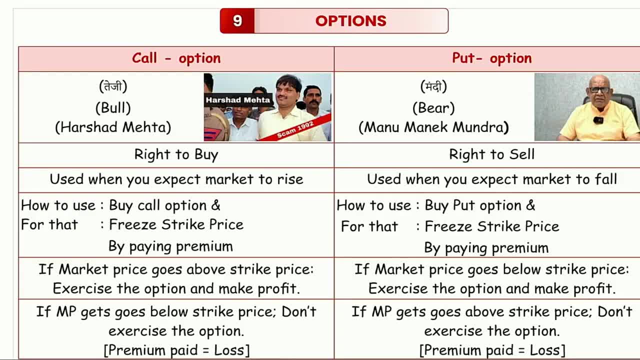 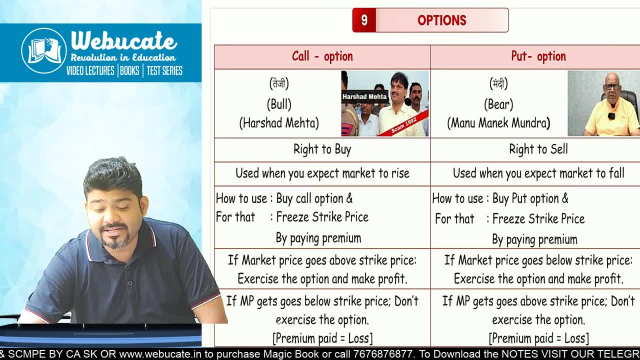 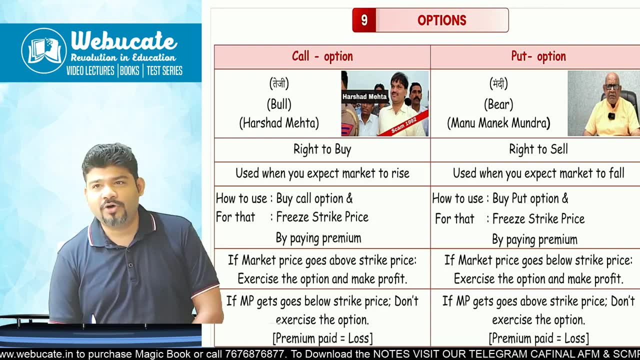 up those chapters? are we clear everybody? now we are going to start with options. options is the only derivative market which gives you a right to decide what you want to do. yes, you heard that right. you can decide the course of action based on your preference, if the things are going in your favor. 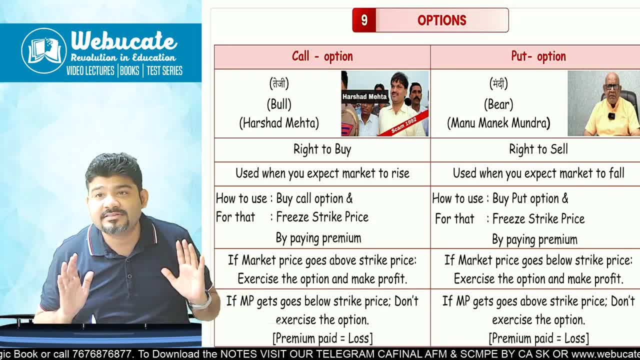 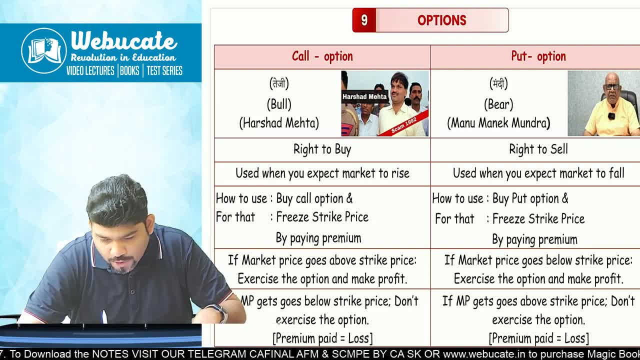 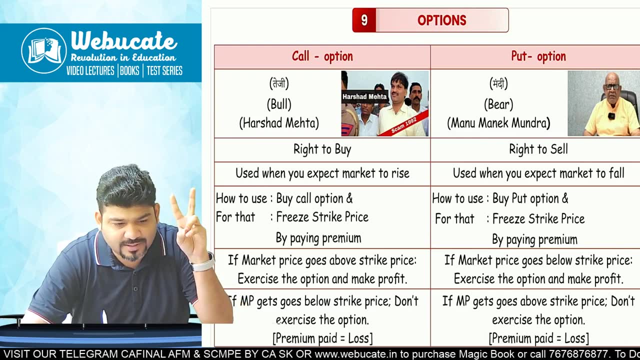 you will exercise the preference. if not, then you can also reject the preference and that basically is called as the options market. so let's try and understand. there are two kind of options market. one is called as the call option- right to buy- and the other is called as the put option, which is called as the 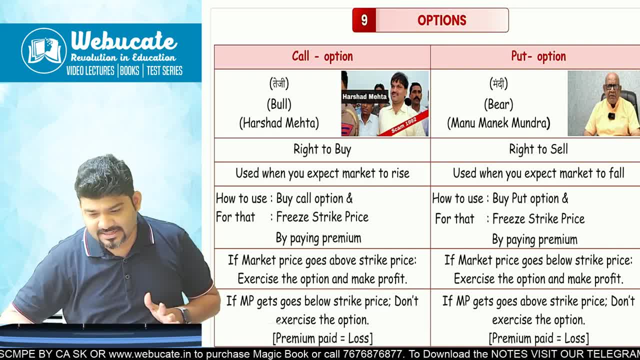 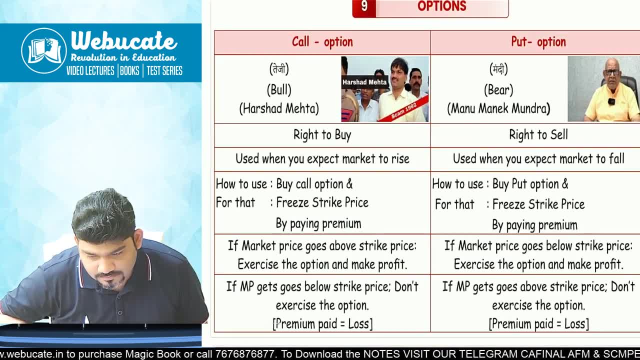 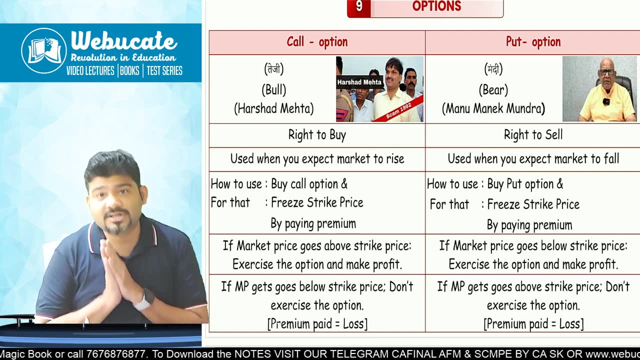 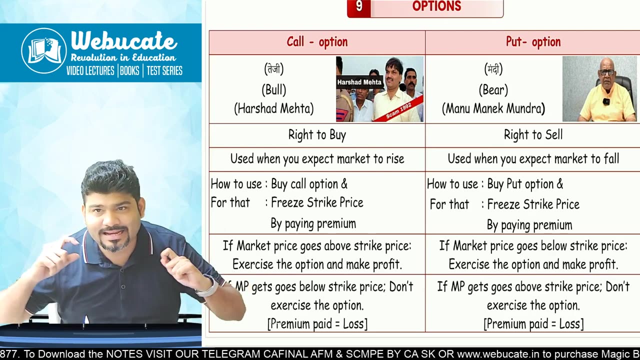 right to sell. now what exactly is the difference between both of them? let's start first. first is called as the call option. what is the call option? right to buy? right to buy means i can buy it at the price that i freeze. yes, you heard that right now. what does that mean? that the price that? 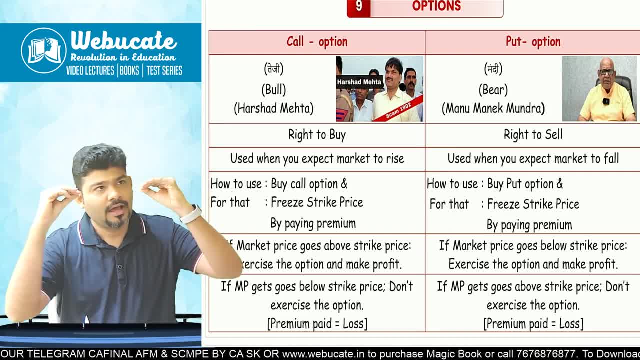 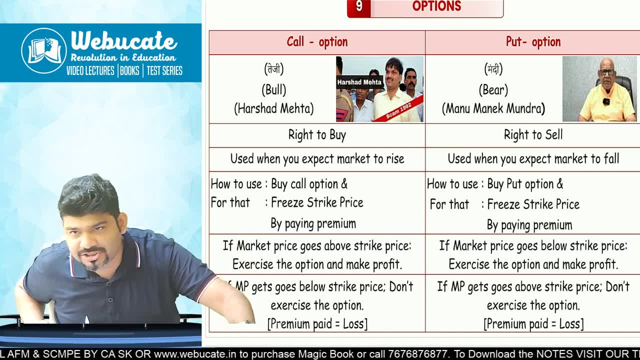 i freeze. so suppose, for example, i feel that one thousand is the price that i freeze, i can buy it at is its correct price. suppose 1000 is the correct price of a particular share. say, this is the share. i feel that 1000 rupees is the correct price of this share. so i will freeze this price for me. 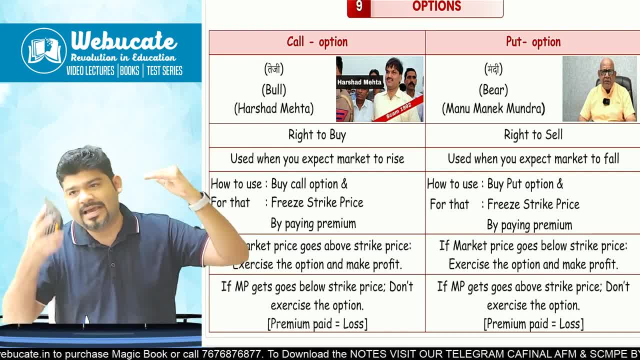 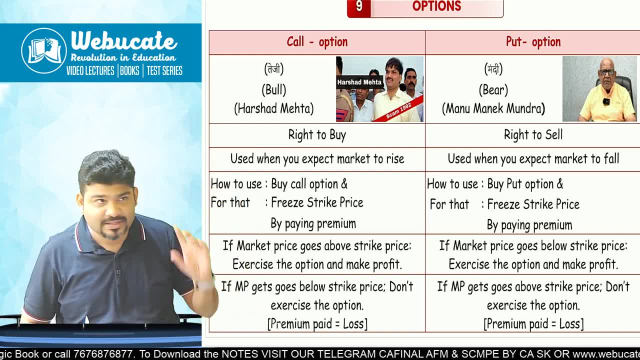 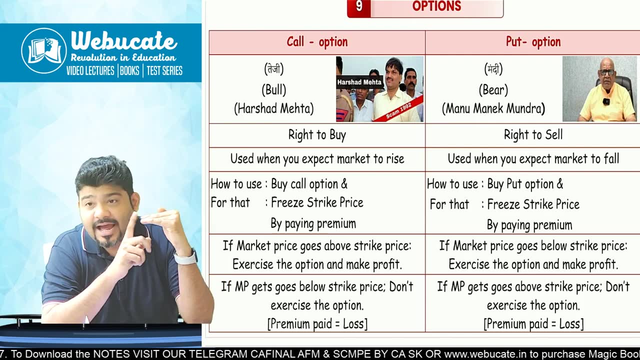 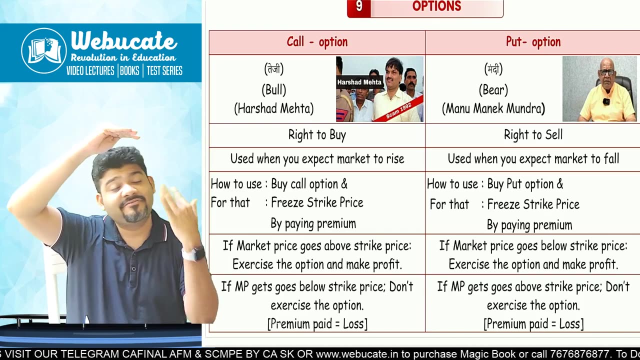 so 1000 rupees i have freezed for this calculator. now, if, in future, i feel that the market is going to go up, that is when i will freeze the price. now, pay attention: 1000 rupees is freezed by me. i feel that the market is going to go up and it does go up, then i have a right to buy because i 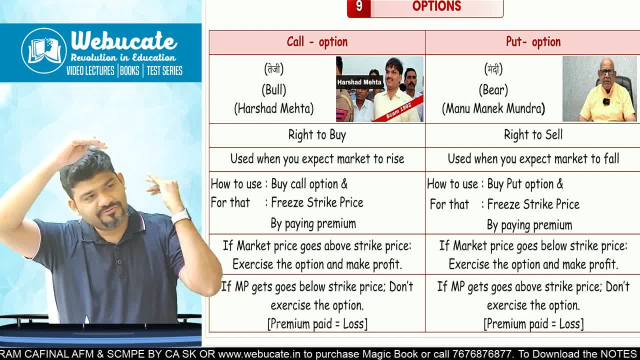 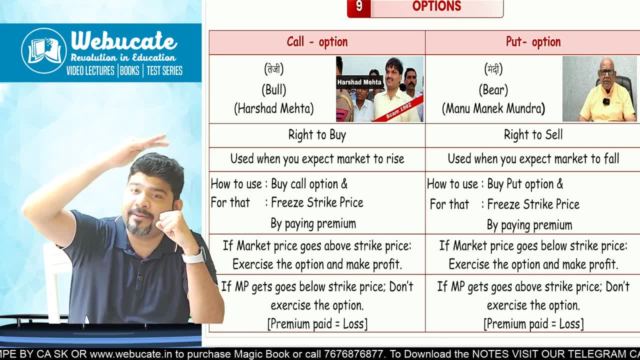 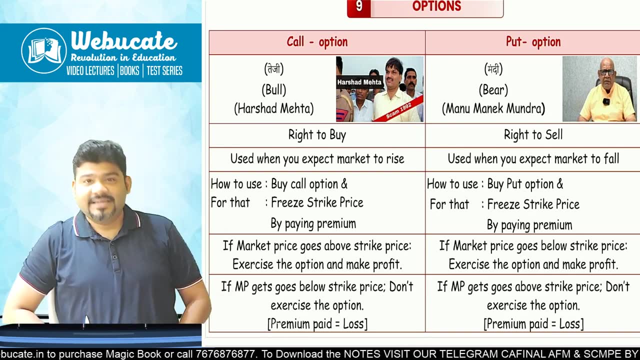 have taken the call option. so if i take the call option, i have freezed the 1000 rupees which gives me a right to buy. the market has gone up. the market essentially has gone up because that's what my expectation was. the difference will be my profit. yes, you are that right, the difference. 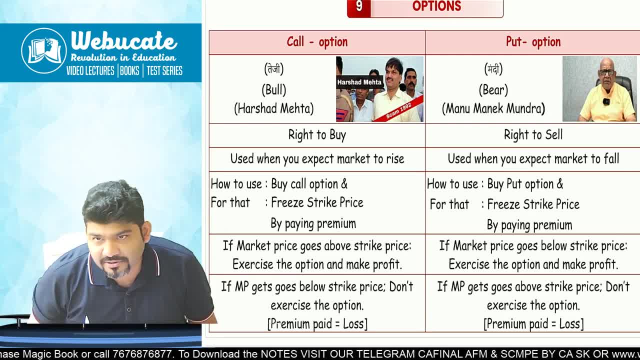 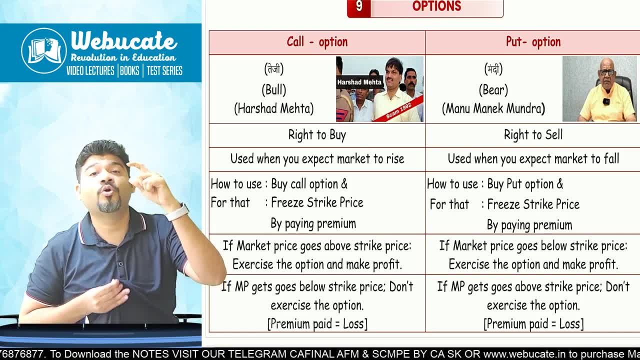 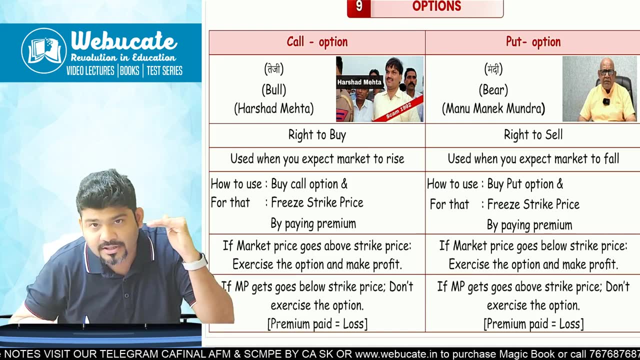 will be my profit. are you clear, everybody? and on the flip side, there is something called as a put option. if you are expecting the market to go down, then you will take the put option. what is a put option? it gives you a right to sell. so suppose, if the market is here and you have freezed your price, 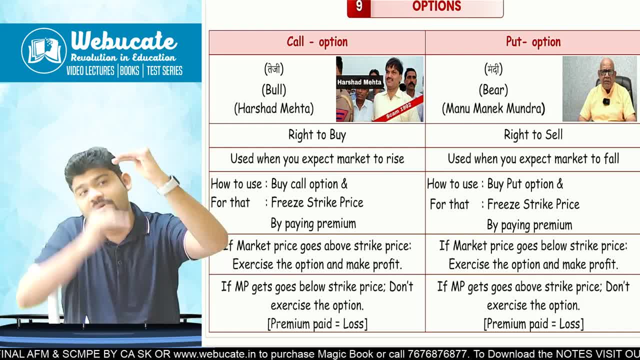 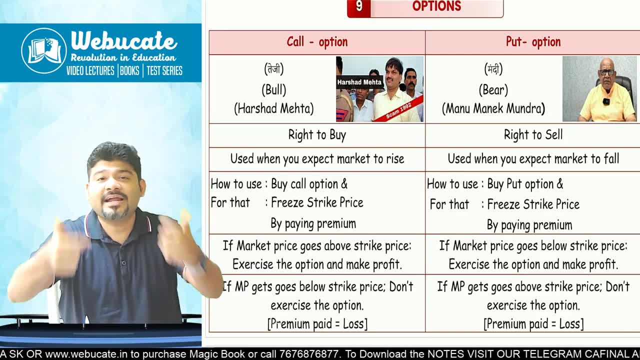 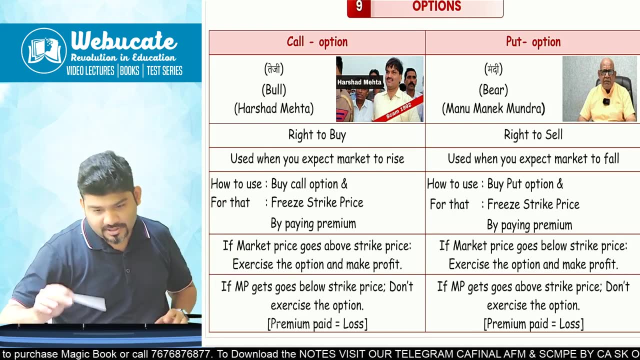 at 1000 and the market goes down, the difference will be your profit, sir. what if the market goes up, sir? how do you freeze the price, sir? what that freezing of the price is called? so many questions going in your head is now what i am going to answer. pay attention: call option is used when. 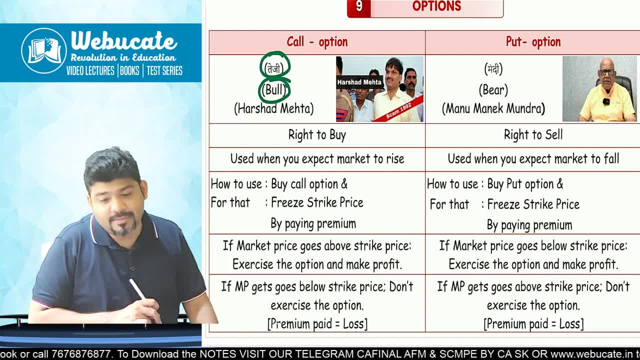 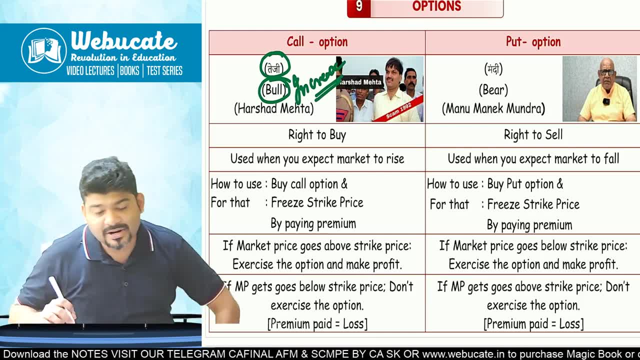 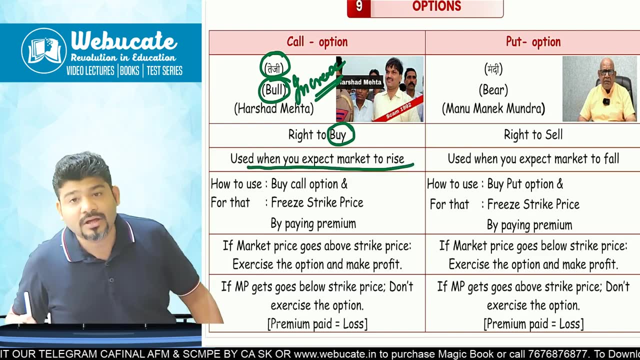 you are expecting teji, something called as a bull market, or when you expect the price to basically increase. you expect the price to increase. that is where you take the right to buy used when you expect the market to rise. so how do you freeze the price, sir? how do you freeze the price, sir? what that? 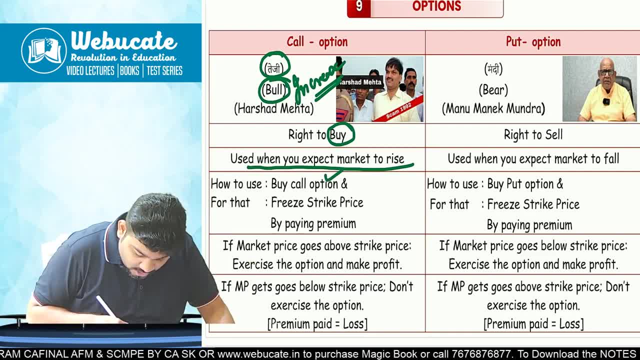 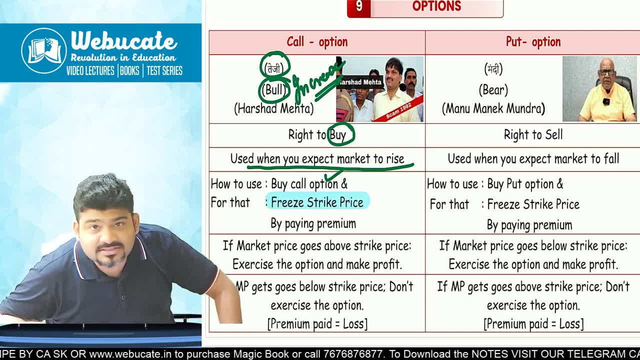 freezing of the price is called. so what that freezing of the price? and freeze the price is called. now what independent price is called? so again, a tier is a inside condition which says you have to take an option on your offer at that point. okay, so if this is a three point, 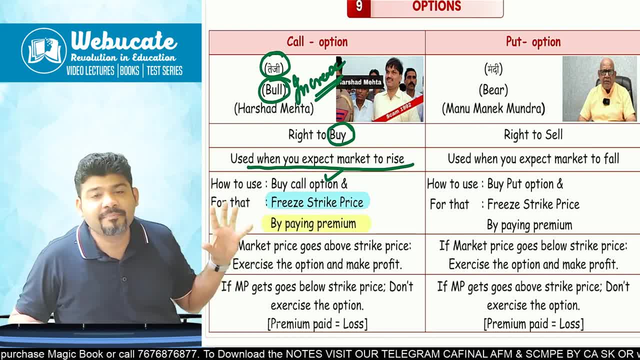 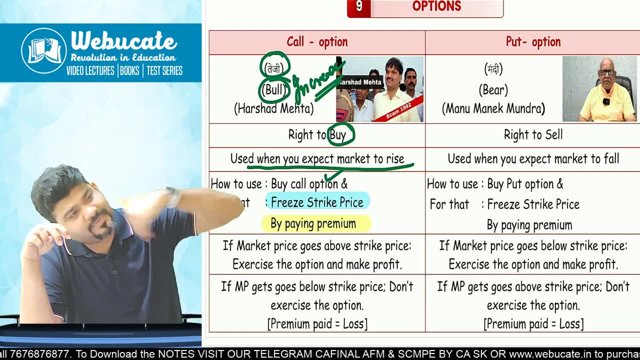 product, you will want to accept the cost, which is outside this company's bidding premises for your contract at all. it's going to be free. this bank is going to be free because the you are expecting the product to go down and then you would have to do that. so, for example, 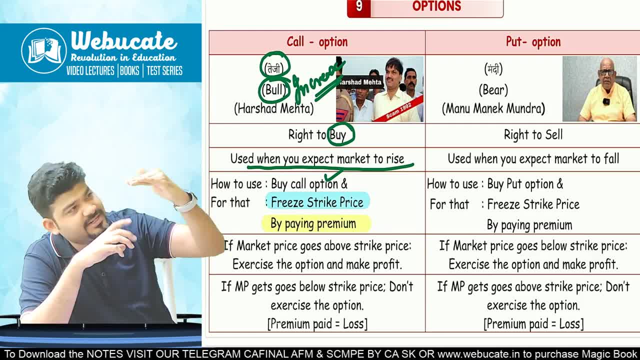 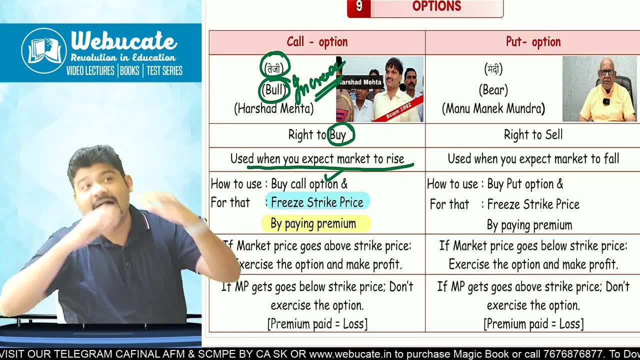 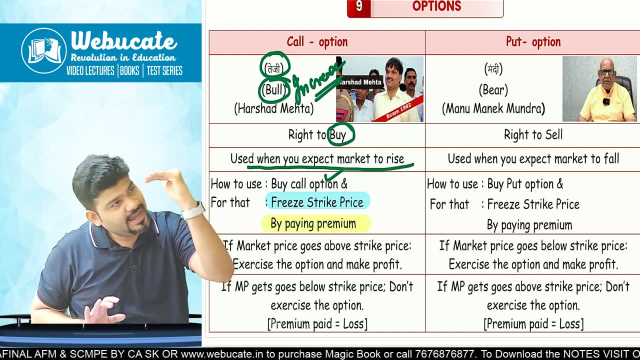 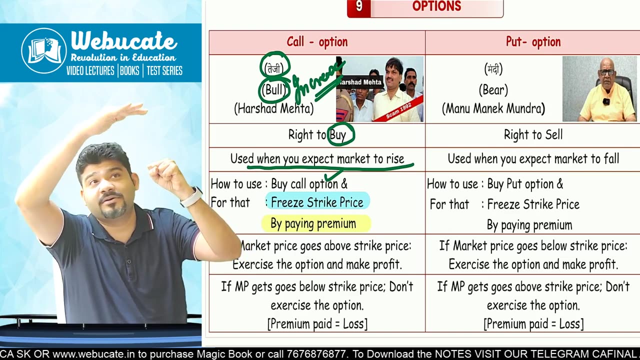 when you were any financial perspective that that is going to be free right now, the initial price that the bank will trade. as the price is going to be free, your partner price will be on the当ล, So I have freezed it at here. Beyond this point, the prices will increase. Now, if the price actually increase, I have a right to buy freezed at this point. For this I have paid a premium. Hello, for this I have paid a premium. I have a right to buy at this price. If the market increases, what I will do- I will buy it at this price, sell it at this price, because now the market has gone up, So 1000, 1200, 2200 rupees will become my profit. 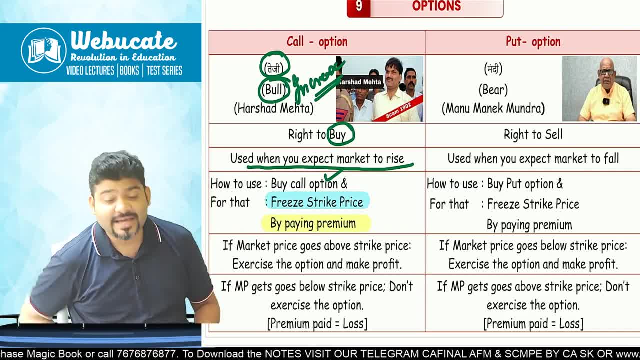 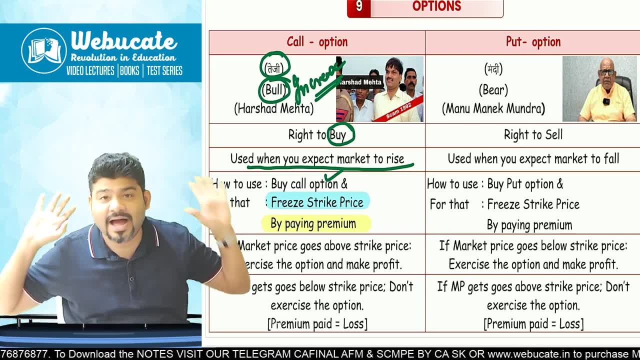 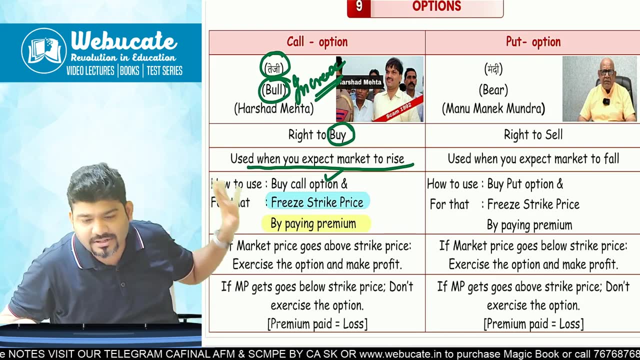 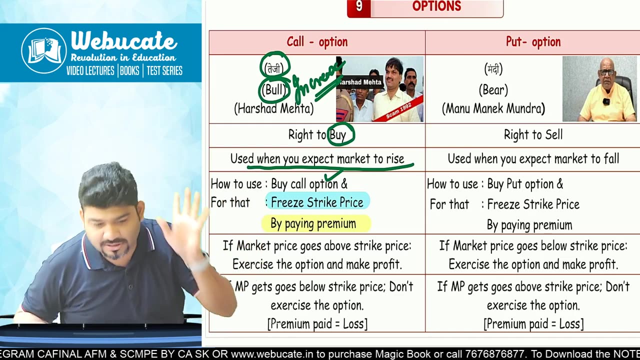 Sir. but what if the market goes down? then you will make a loss. The answer is no, I will not make a loss. Why? Because I have a right to buy. For that right I have paid a premium. Now, if the market goes down, I will not exercise the right and that premium that I have paid will become my loss, and that premium that I have paid will become my loss. Are you clear, everybody? 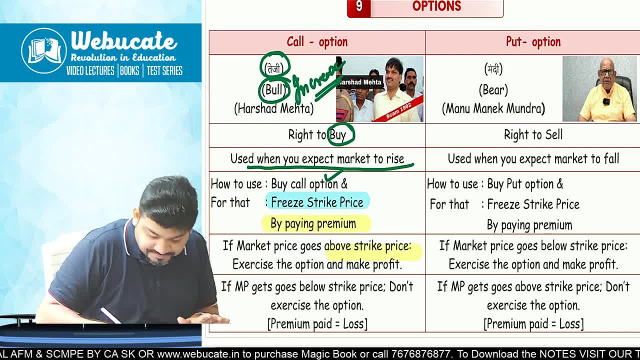 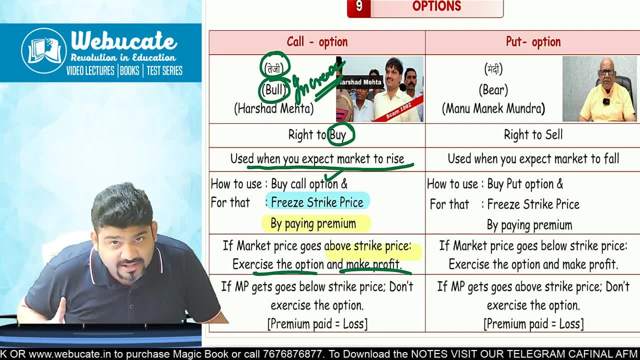 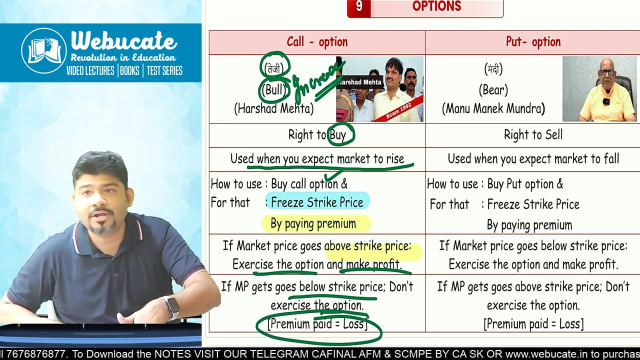 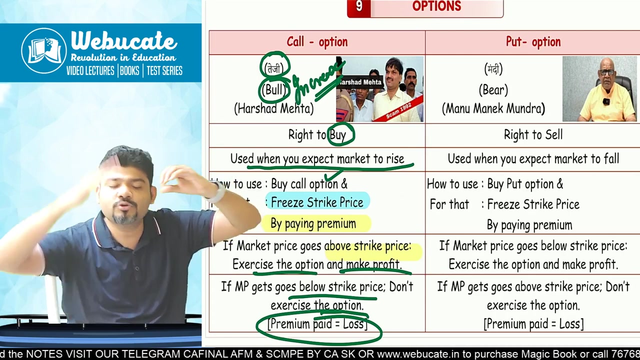 If the market goes above strike price, hello. if the market goes Above strike price, exercise the option and make profit. See, your fundamental should be very clear, because when I do advanced things, these things will matter a lot, right? So, if the market goes above strike price, exercise the option and make profit. If market goes down below the strike price, don't exercise the option and premium paid will become your loss, and exactly vice versa In case of put option. you want the market to go down or you are expecting the market to go down, So you freeze this, and that put option is called as right to buy. 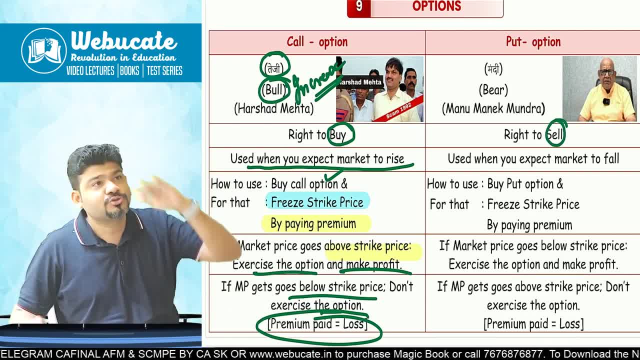 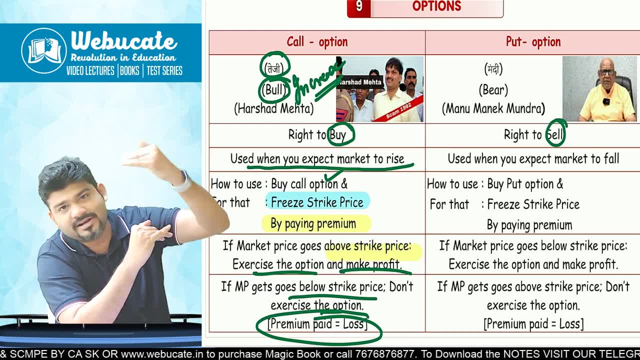 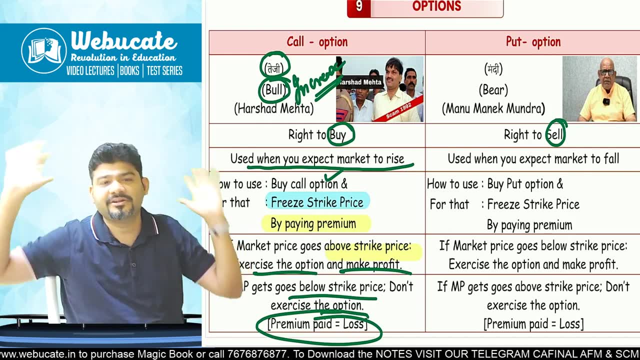 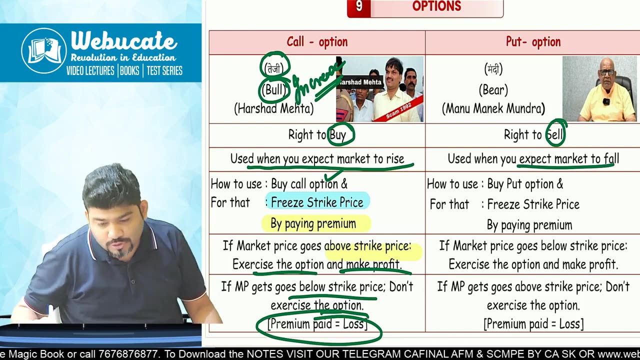 Right to sell. That option is called as right to sell, So you have freeze this. You have a right to sell. Market goes down, So right to sell. You will buy it again here. So you have a right to sell at 1000.. Market goes to 800. The difference 200 will become your profit. The difference 200 will become your profit, Got it guys? So used when you expect the market to fall. How to buy? put option Free strike price, pay the premium If the market goes below strike price, exercise the option and make profit. 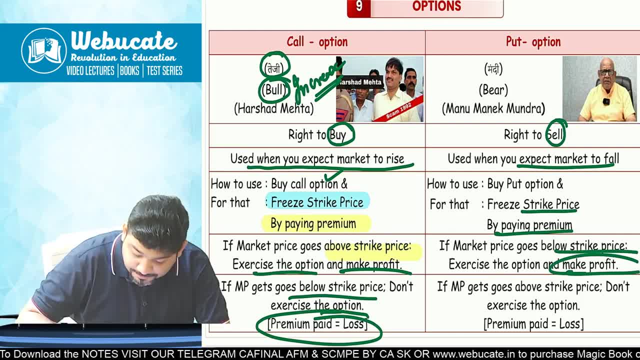 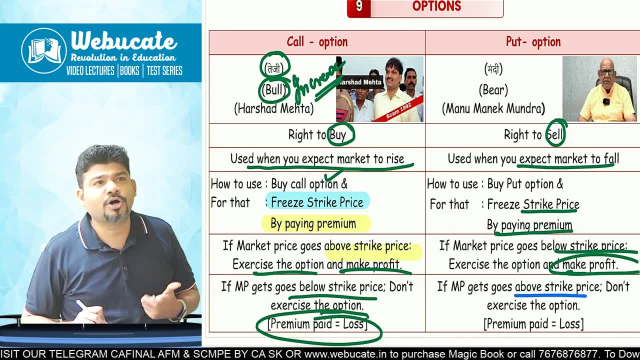 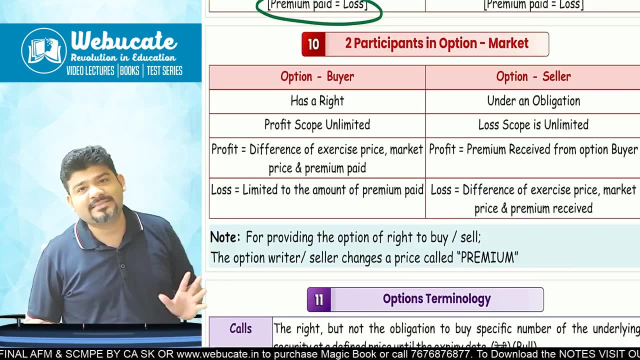 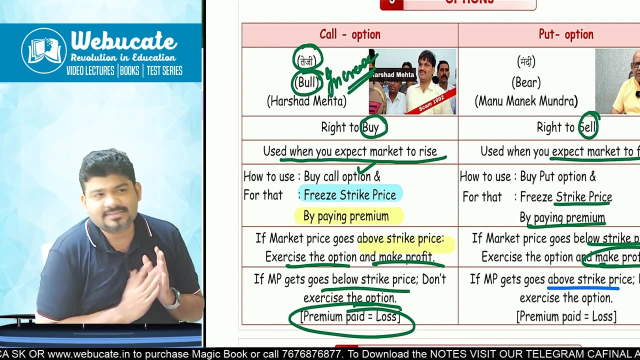 Exercise the option and make profit. Simple as that. But if the market goes up, goes above strike price, don't exercise the option. Whatever premium that you have paid will become your loss. Clear cut, Done, sir, Done. Next, two participants are there in the options market. Now see this: You are taking a right to buy. You will exercise it if you want, If the market goes against your expectations. See again, I'm telling you: if you are expecting the market to go down, you will exercise it. 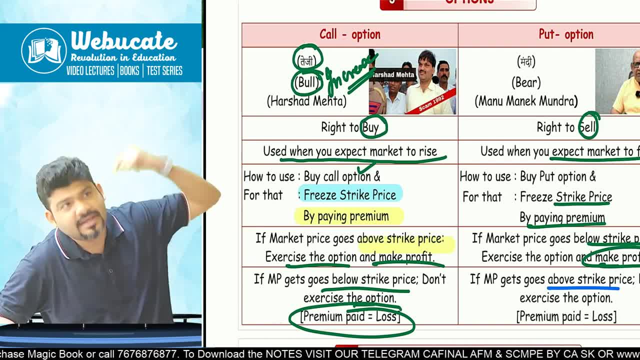 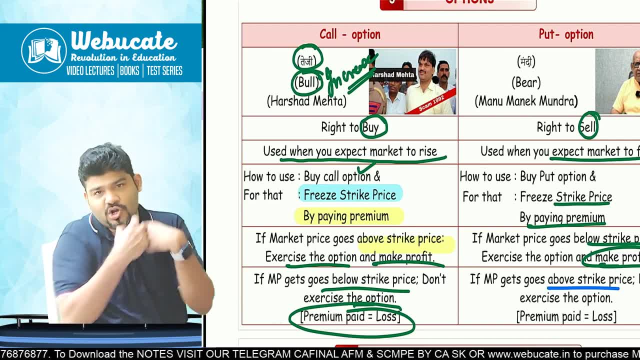 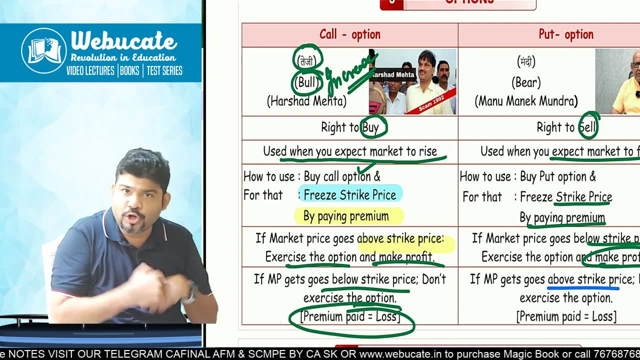 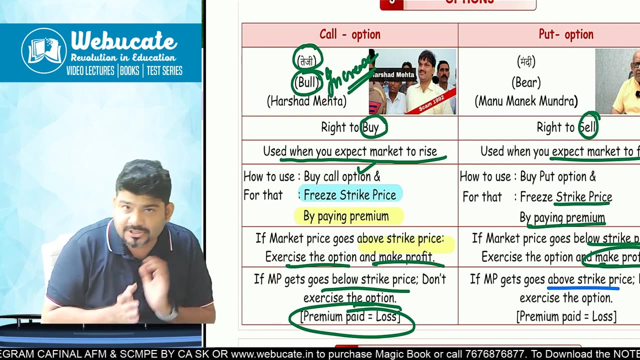 If the market goes up, take a call option, Exercise it. If the market actually goes up, that difference will be your profit and vice versa. But if you are buying that call option, somebody else is selling you that call option. So you are options buyer. You may buy a put option. Put option is right to sell, But you are buying that put option. Try and understand that. So you are buying a put option which gives you a right to sell. So one is buying put option and the other is buying a put option. 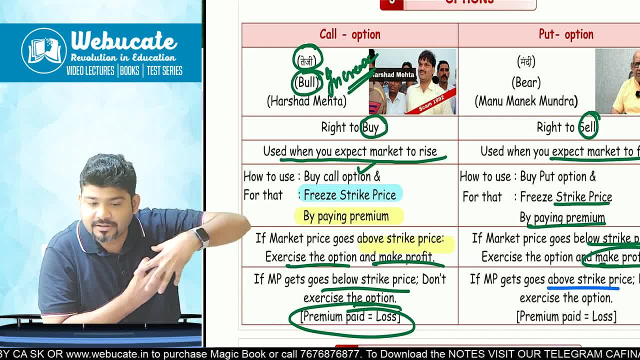 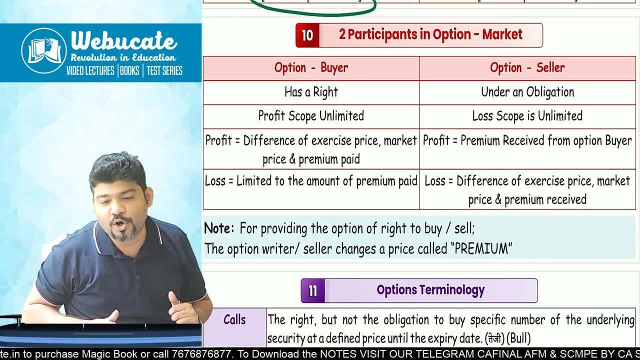 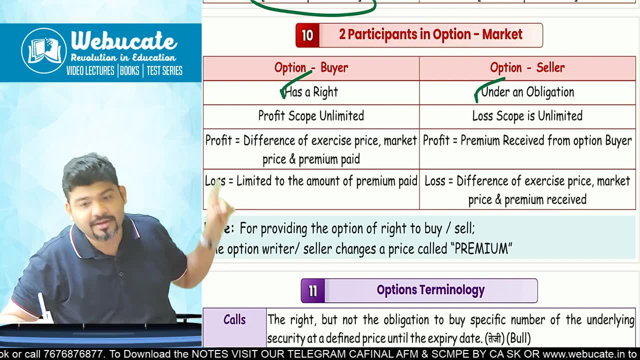 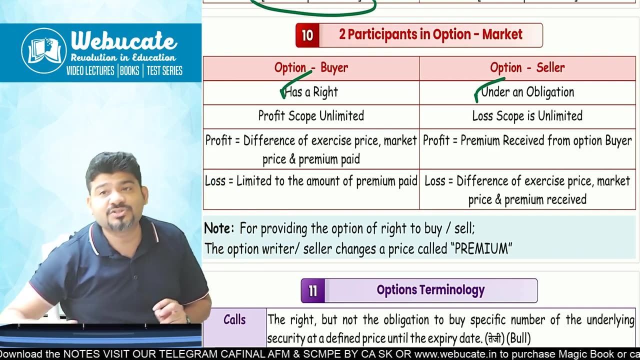 So one is buying, call option, So buying an option. And the second part is if you are buying, somebody else has to sell. That other person is called as the option seller. If you have a right, that other person has a obligation, If you have a right to buy, that other person has to sell. If you have a right to sell, that other person option has to buy, Got it guys? So that's what the other person is called as the option seller. 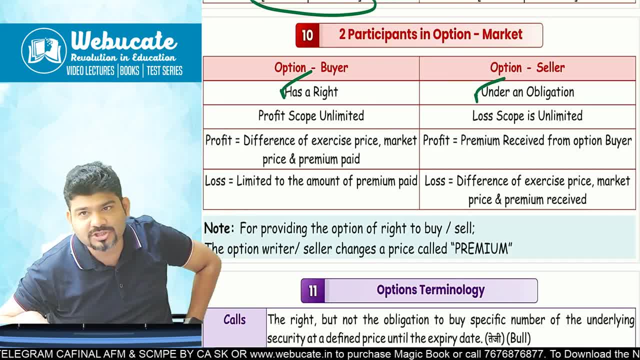 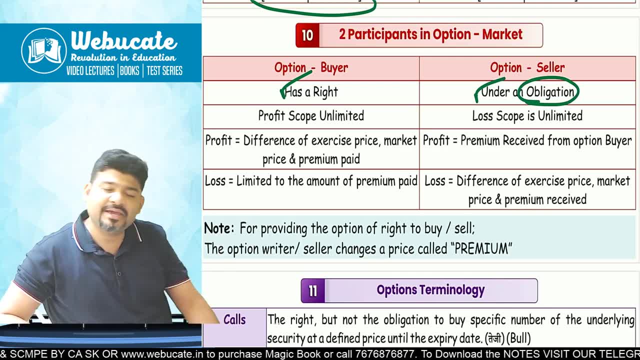 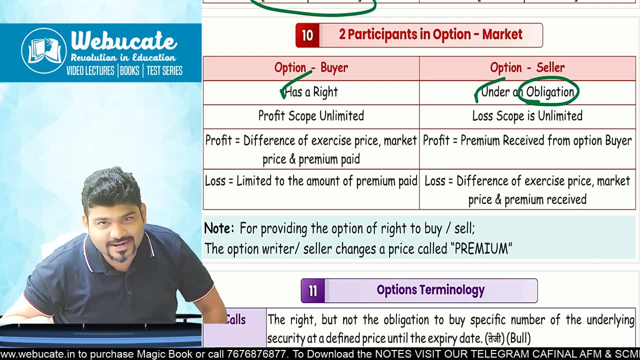 Now you will feel, sir, it is so harsh on that person. We have a right, but he is under an obligation- Yes, he is under an obligation. Still, he makes a good amount of profit. You don't have to feel pity on that person. As per SEBI stock market, in stock market, eight option sellers earn money and two option buyers sell money If you take a range of 10 traders. 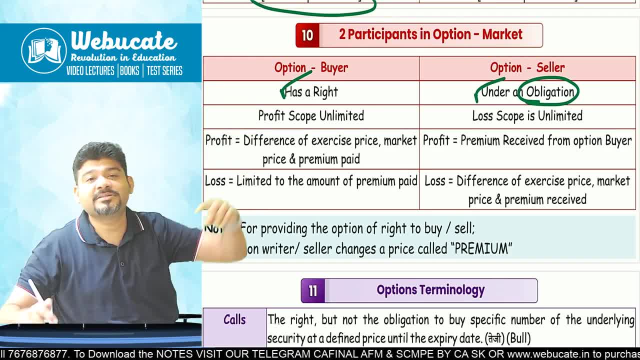 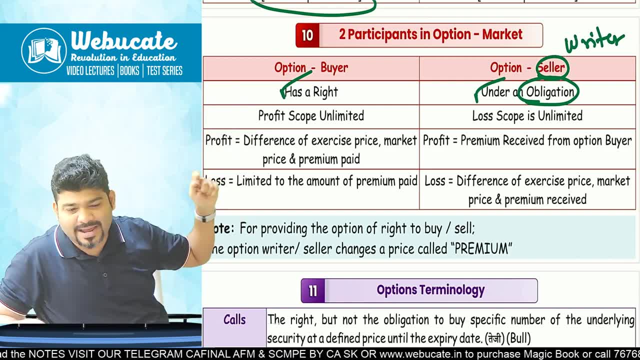 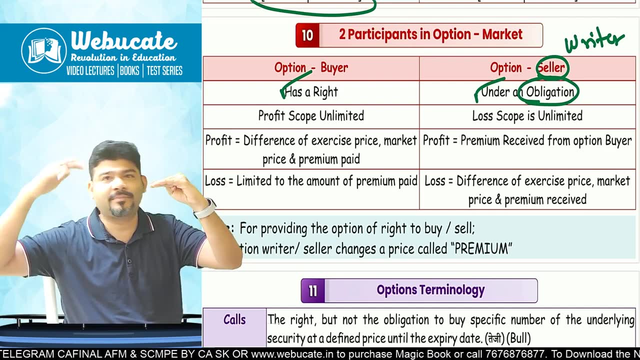 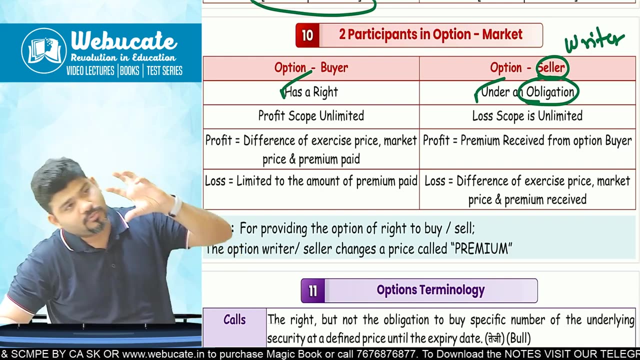 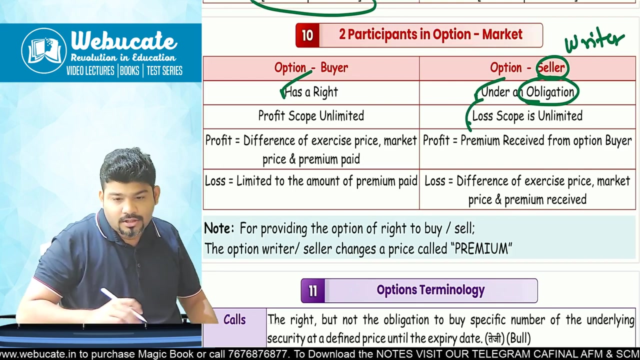 So we have a right That other person is under an obligation- Option is called as the option seller, also called as the option writer- that in case you are buying the option, your profit scope is unlimited because you have freezed the price Here. call option here. You want the market to go up. Market goes up, up, up, up, up, up out the world. So I the all difference will become your profit. But whatever is your profit will be- option sellers, option writers- loss. I hope you are clear with that as well. What is the profit that you are going to make? the difference between the two. 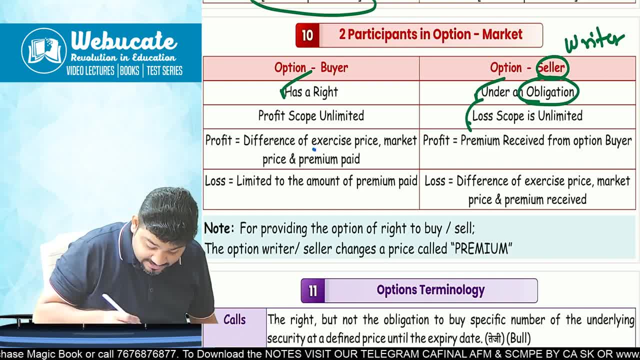 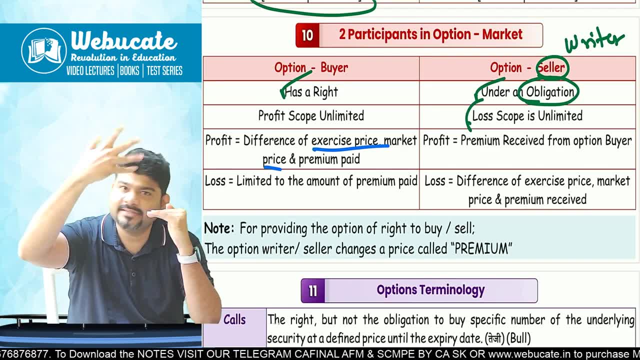 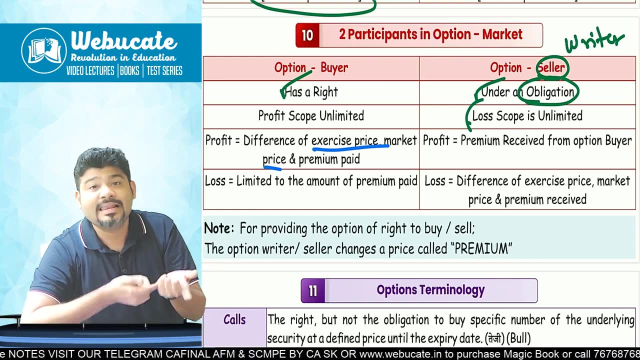 the exercise price and the market price. so that's what is written here: the difference of exercise price, market price and premium paid. so see: difference between the exercise price and the market price. in case you have a put option. difference between the exercise price and the market price difference is going to be your profit, less premium paid, because premium paid is like: 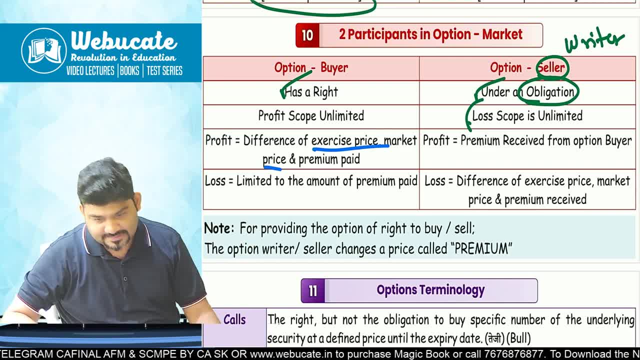 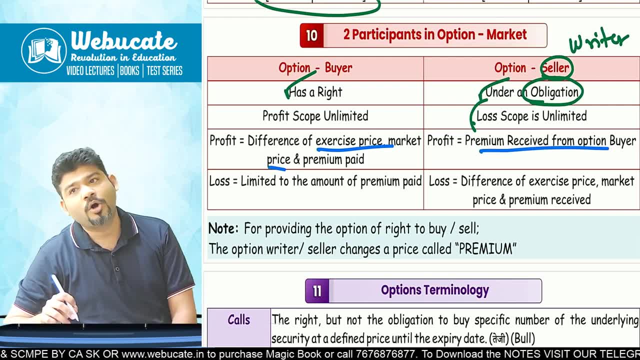 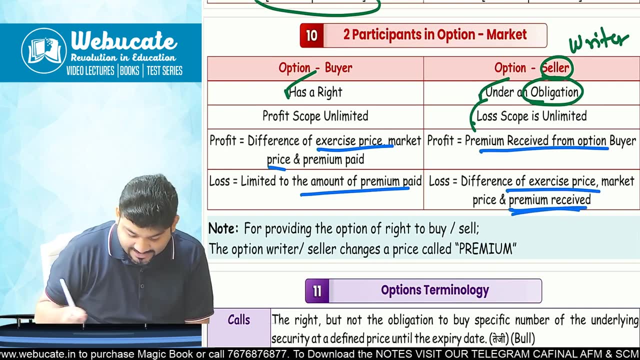 your cost, are you done everyone? yes, sir. and in case of option seller, profit is premium received from option buyer. loss is limited to the amount of premium paid. loss is equal to difference of exercise market. so see here, his profit is his loss. very true, and his profit is his loss. 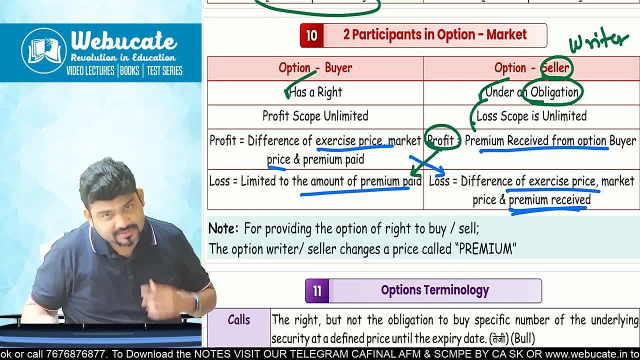 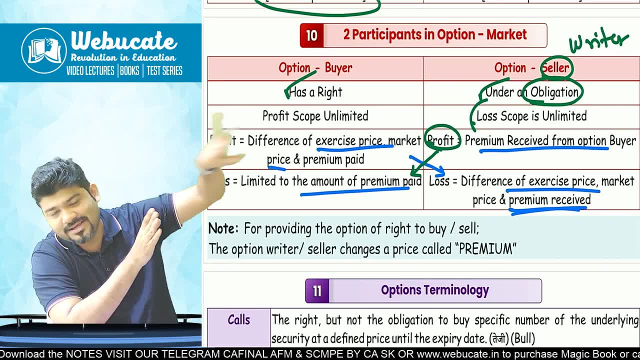 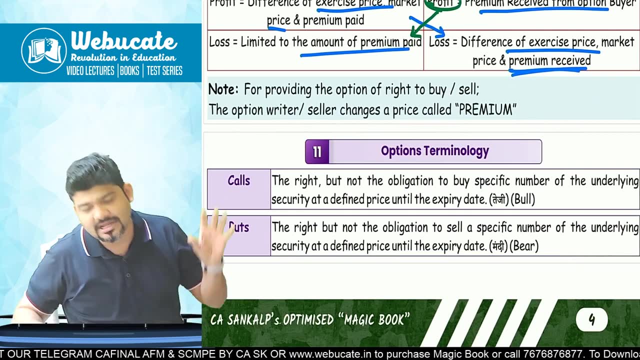 right. what is profit for him? that if that option buyer does not exercise the right, then whatever premium he has paid becomes that option buyer's loss, but that becomes option sellers profit- everybody. yes, sir, so that's how it works. now we will quickly see the options terminology. we know what is a call. 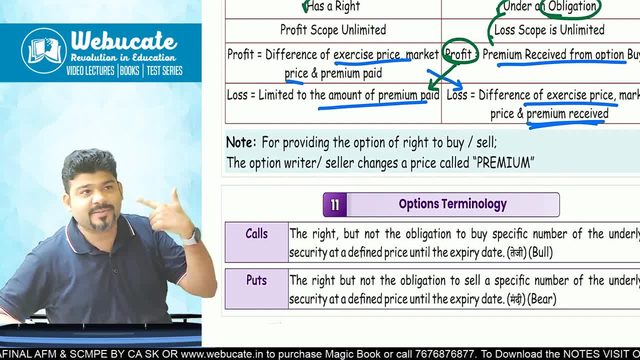 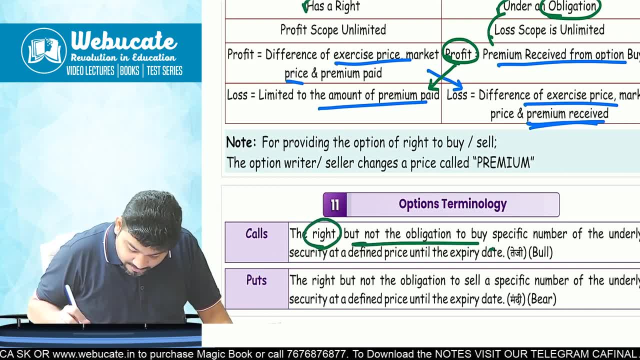 call is giving me a right option when i am expecting the market to go up, and i will exercise it only if it is in my favor. the right, but not the obligation, to buy specific number of underlying security at a defined price until the expiry date. so what is expiry date coming to it, right? 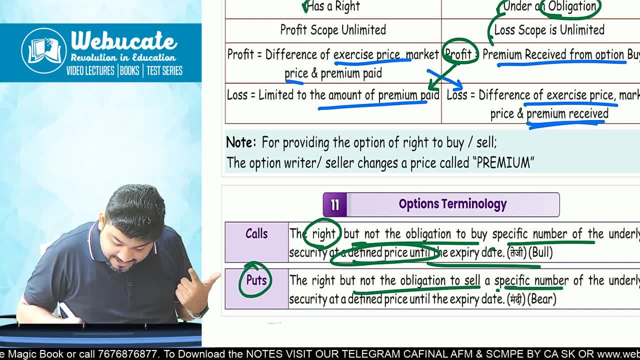 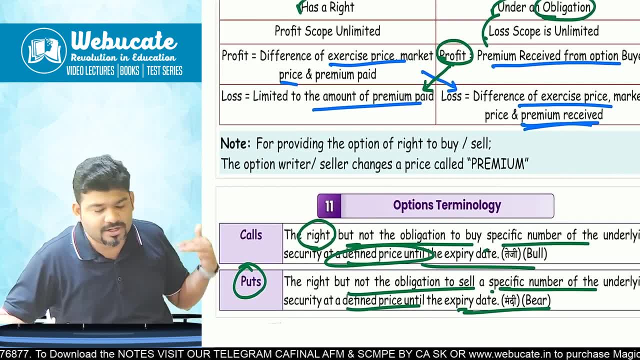 and then there is put the right, but not the obligation, to sell a specific number of underlying at a defined price until the expiry date. that is called the expiry date. so what is expiry date? call as a put. so when you are expecting the market to go down, take a put option. expecting the market: 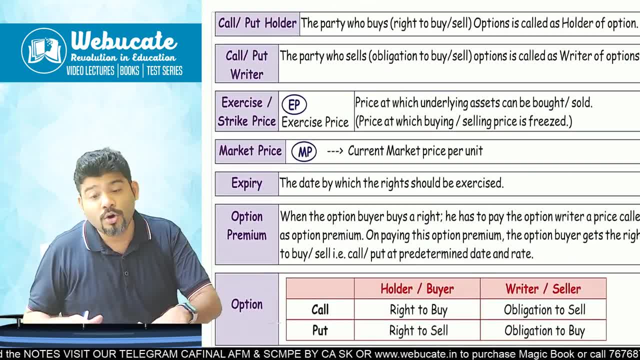 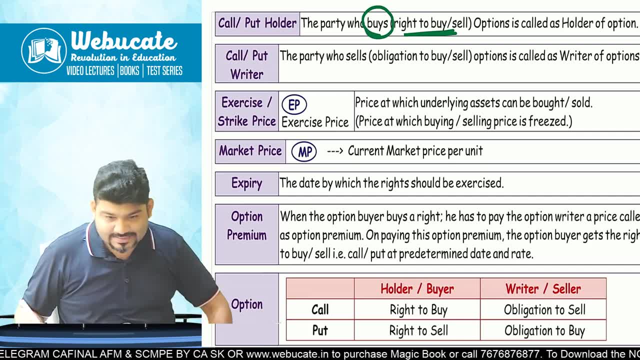 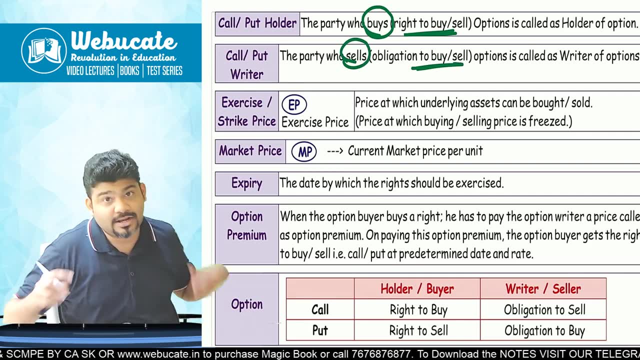 to take a call option, call put holder, which is the buyer, the person who buys the right to buy or sell is called as a holder, holder of option. and then there is a call put writer, the party who sells obligation to buy or sell obligation. so when will he have obligation to buy when somebody 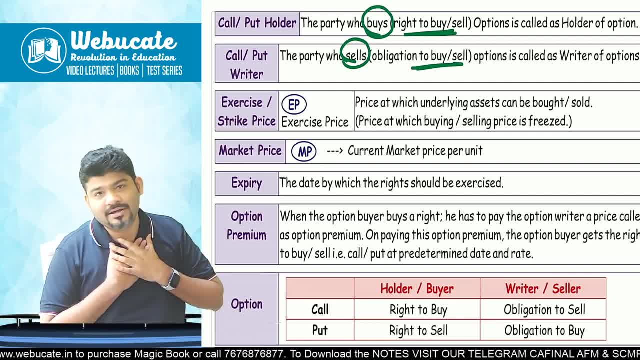 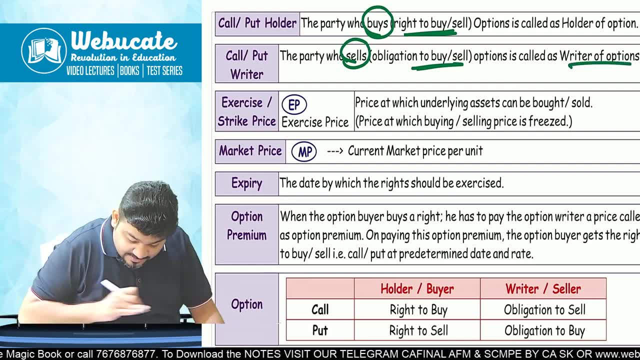 has taken a put option. so suppose, if i have taken a put option, i have a right to sell, the other will have obligation to buy got it and vice versa. it's called as a writer of option. exercise price is the price at which underlying this can be bought or sold, which is the freest price, market price. 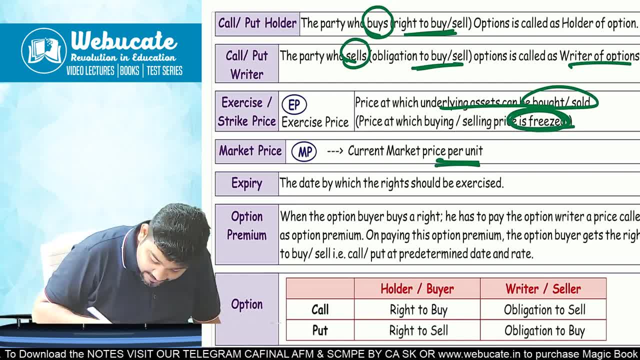 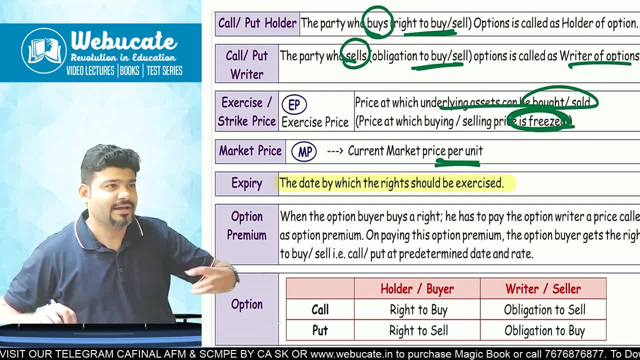 current market price, which is going on expiry, the date by which the right should be exercised. so you have paid a premium, not for lifetime, but for a particular period. that, okay, i am paying this for three months, within three months. whenever i want to exercise, i will exercise and i am paying. 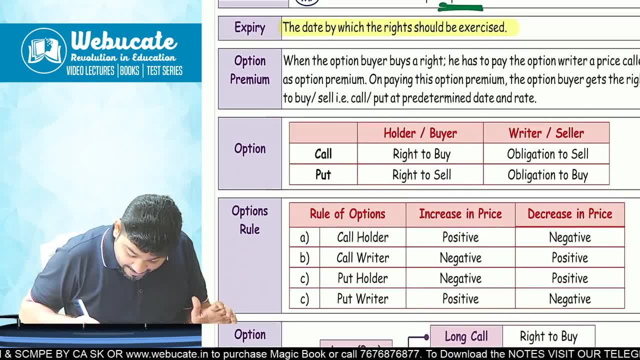 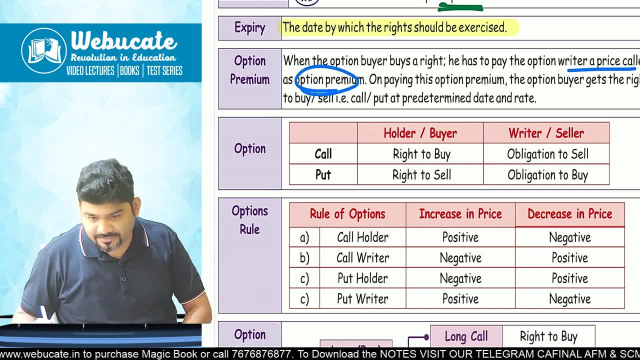 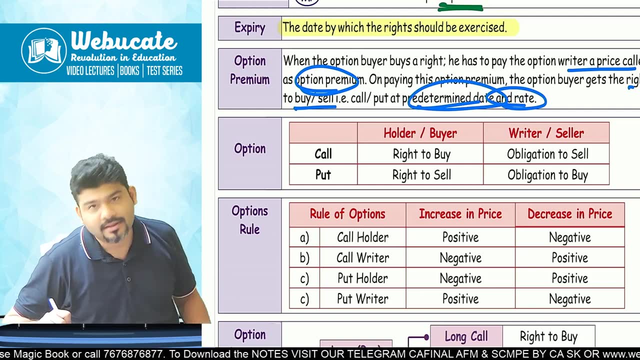 a premium for that. so when option buyer buys a right he has to pay the option writer a price called as option premium. on paying this option premium, the option buyer gets the right to buy or sell at a determined, pre-determined date and pre-determined rate. got it everybody? yes, sir. so option call put: right to buy, right to sell. 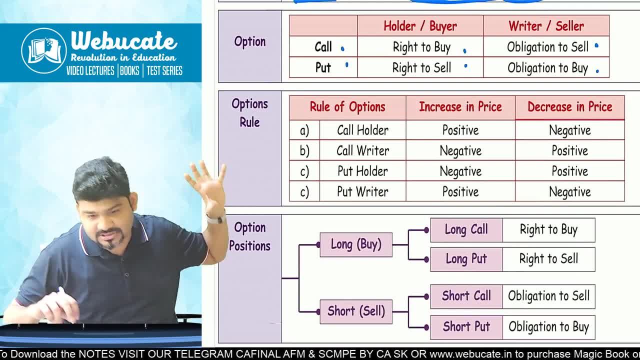 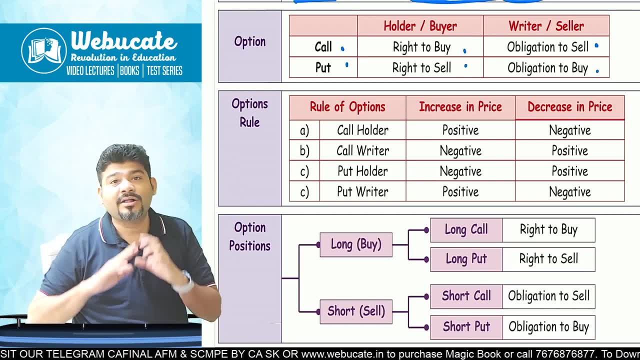 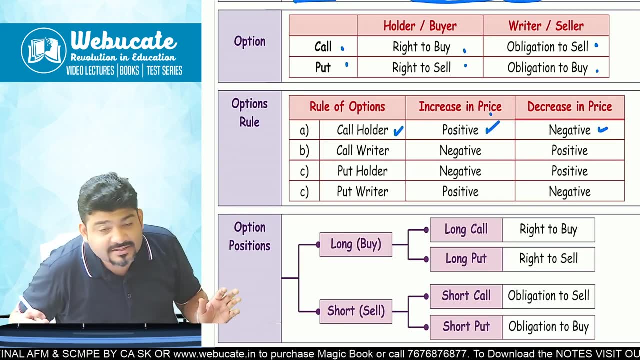 obligation to sell, obligation to buy, rule of options. now i hope we are all clear with this. so who is the call holder? the call buyer wants the market to rise. the call seller wants the market to go down. call writer: increase in call holder: increase in price positive, decrease in price negative. vice versa for a call writer: he wants the price to. 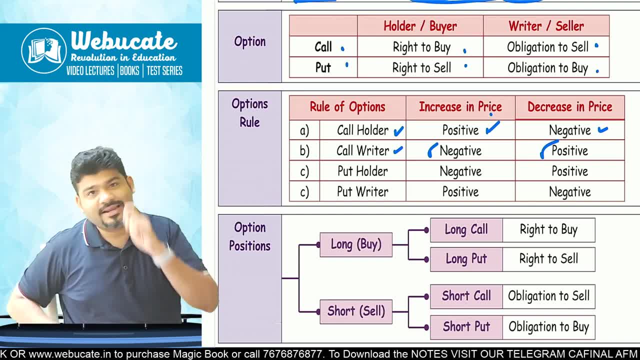 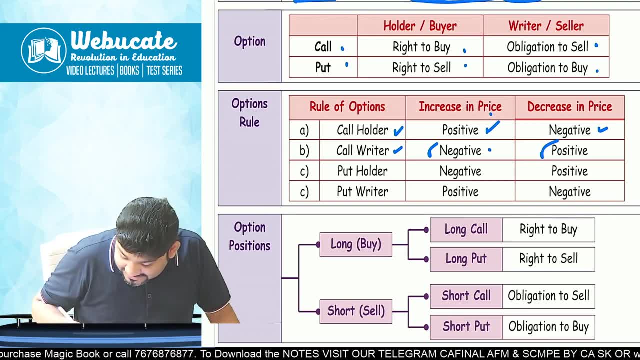 rise and he wants a decrease in price. so if there is a call writer, then he wants the price to go down. so if the price goes up, it is negative for him because that will be his loss, the other person's and vice versa. option positions. now this is very important. 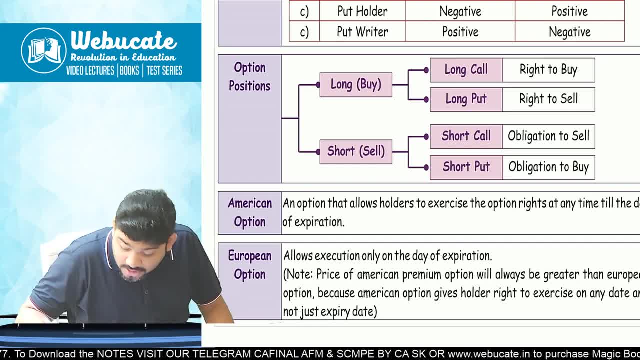 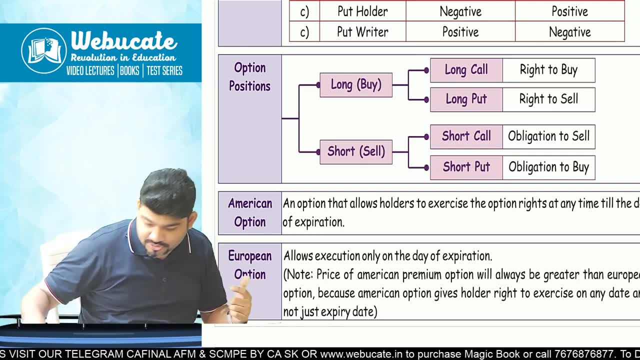 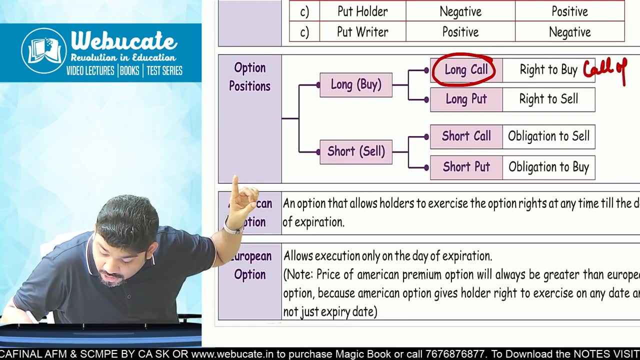 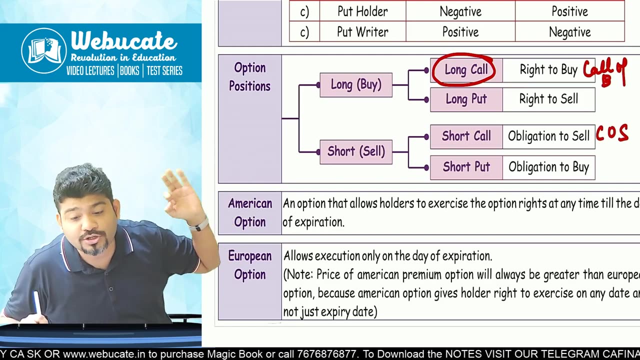 guys will be used ahead. long call means right to buy call. short call means i have sold call, so this is option. this is what option buyer does. this is what call option buyer does. call option buyer. what is a short call? call option seller is called as a short call: obligation to sell. you have a short call. 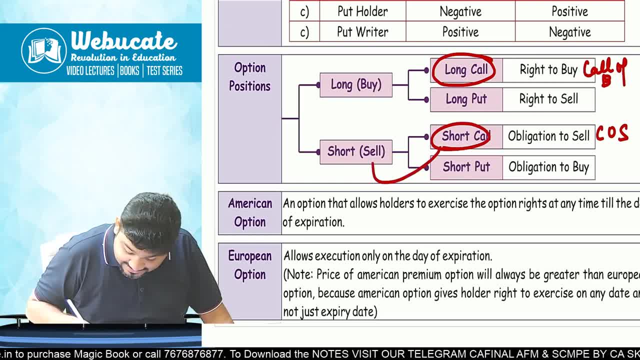 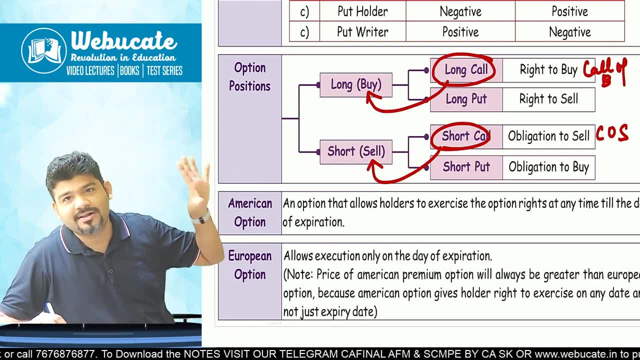 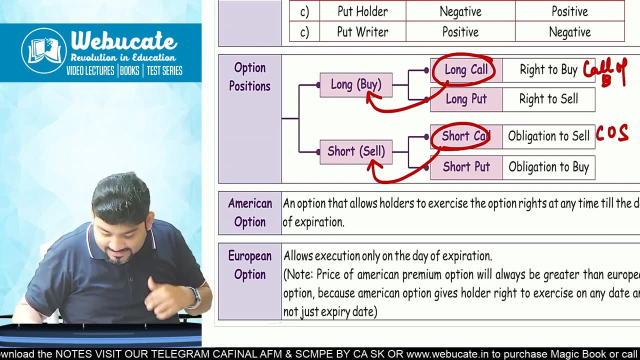 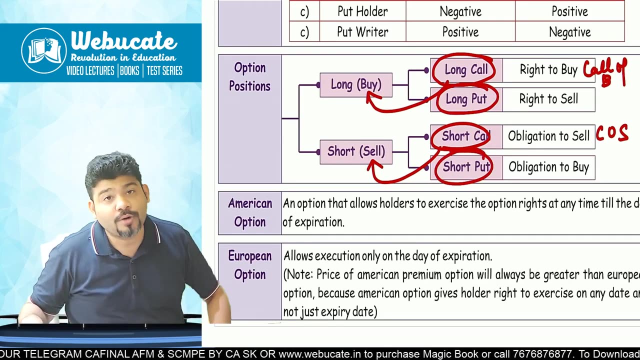 so short means sell, long means buy, got it. so sell call. long call means long right to buy a call right. and then there is long put- i have bought put, i am the put option buyer and short put put option seller got it guys. so this is the put option seller and put option buyer. so i have 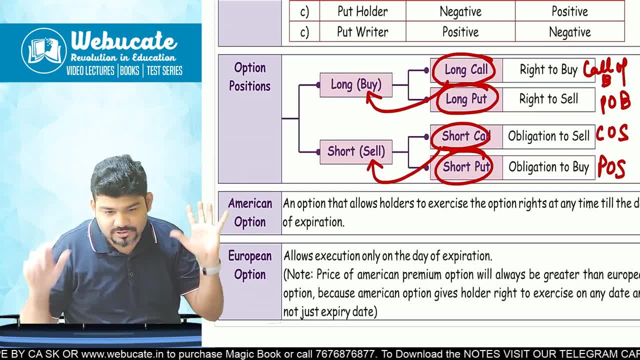 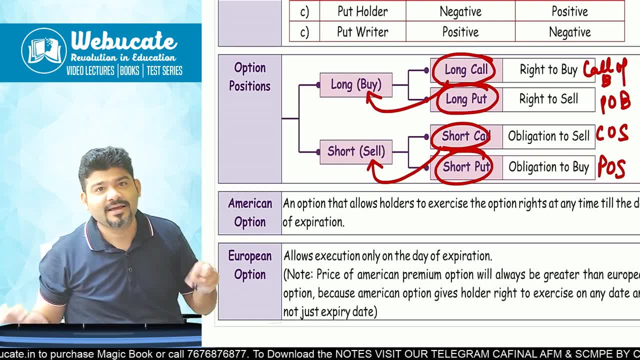 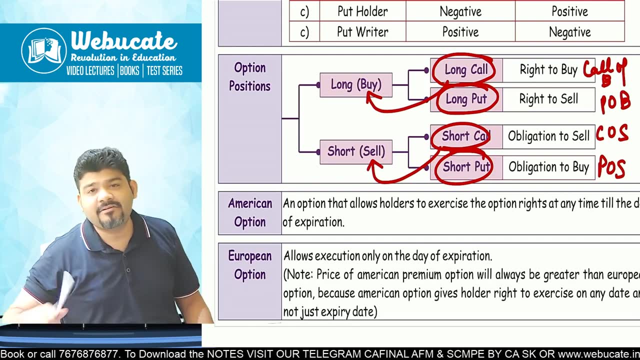 buying a put option giving me a right to sell. don't confuse, but that's what it is. and if i am buying the other person is selling, so short put he has done to me. i am buying the put option long put. i have bought the put giving me a right to sell. done. then we have american option and european option. 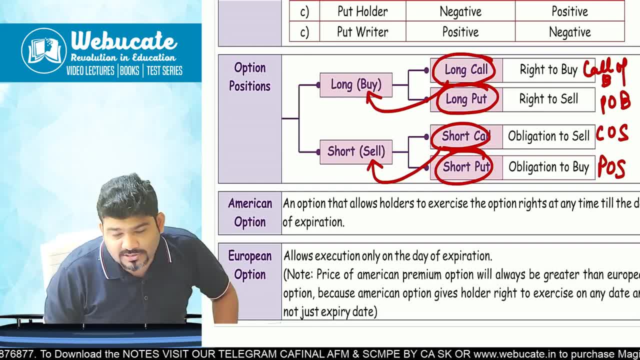 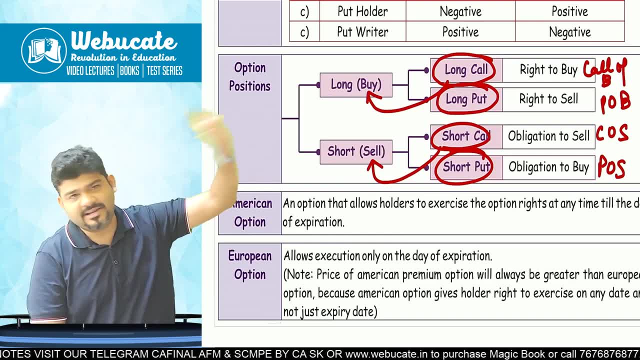 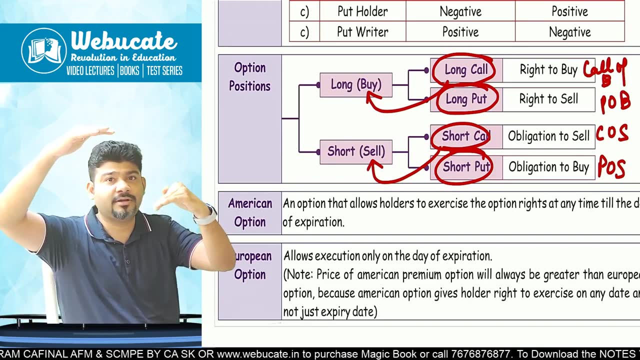 nowadays, everywhere the american option works. what is it? it means that, till the date of expiry, i can exercise my right whenever i want to. in three months, whenever i want, i can exercise the right to sell, right, sir? if you thought that the market will rise, you took the call option, but the market didn't. 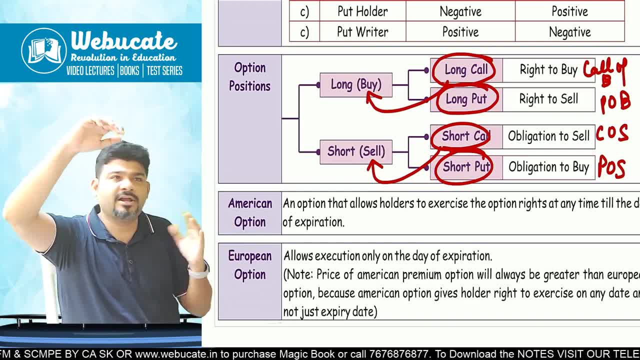 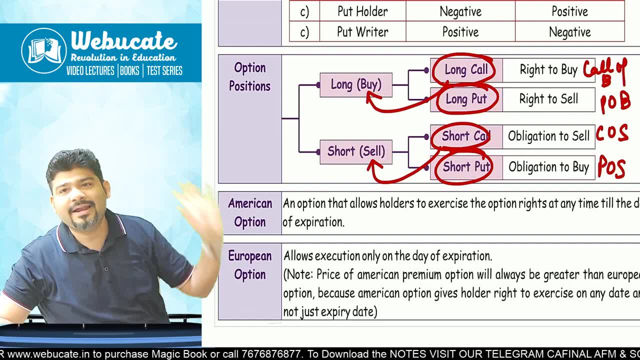 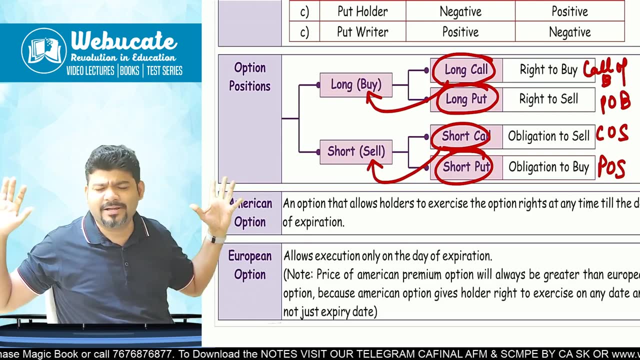 rise at all. it always went down and down and down for three months. then what will happen on the expiry? it will automatically be converted and i will have to bear the loss of the premium because it's a right. so i will not exercise the right at all till three months. i will not exercise the right. 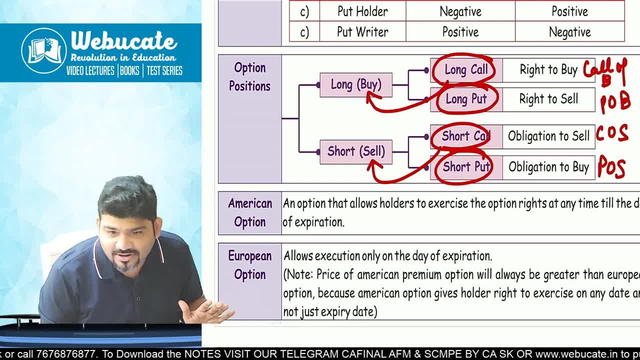 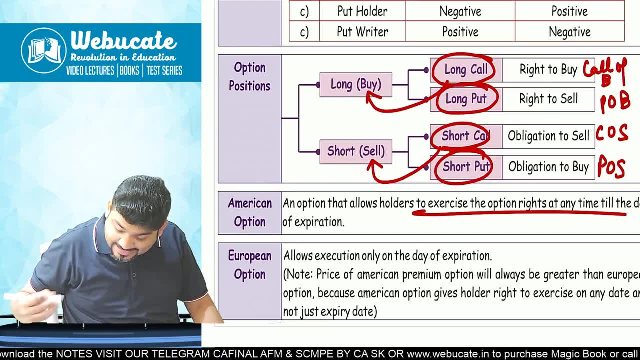 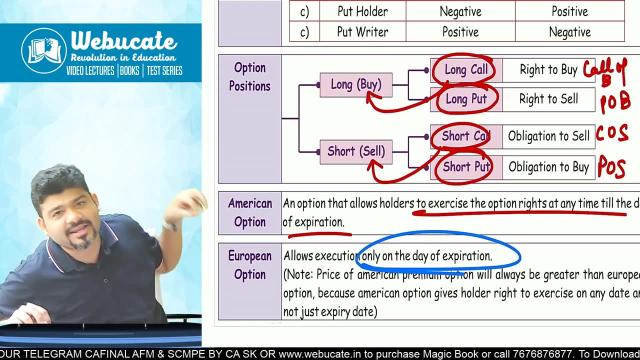 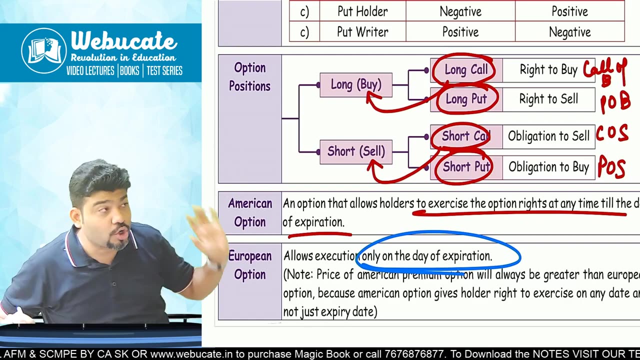 so whatever is the premium becomes, my loss got it. so american option till the expiry, any time you can exercise. so allows the holders to exercise the option right at any time till the date of expiration. but what is the european option? only on the day of expiration. yes, so american option any time you can exercise, but european option only on the day. 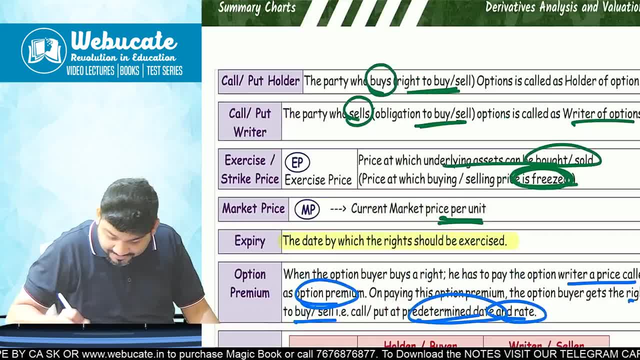 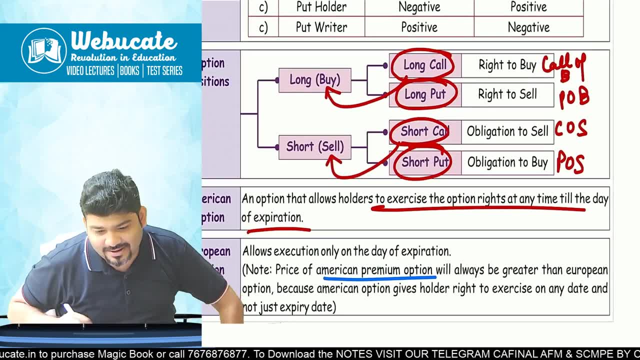 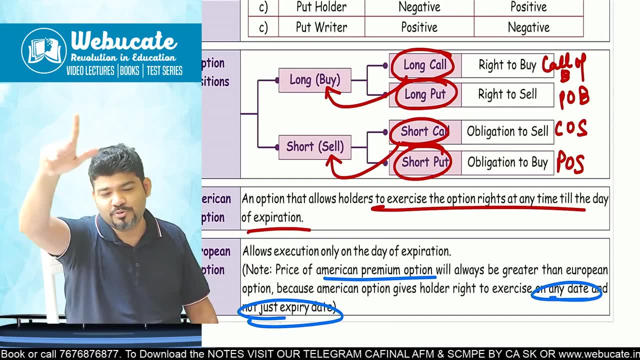 of expiration. so price on american premium will always be higher. so that's a fair point. see, a price of american premium will always be higher than the european because american option gives the holder to write exercise on any date and not just expiry date. any date you can exercise everybody. yes, sir, till here. any doubts anyone? 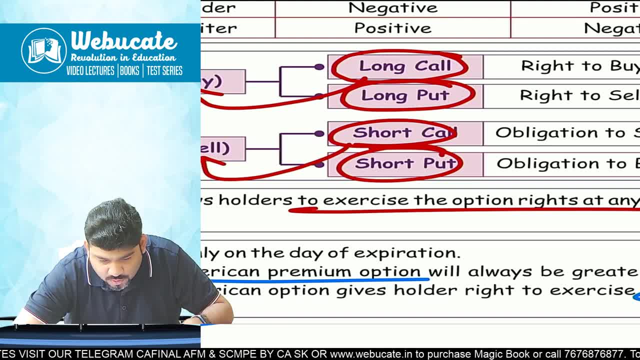 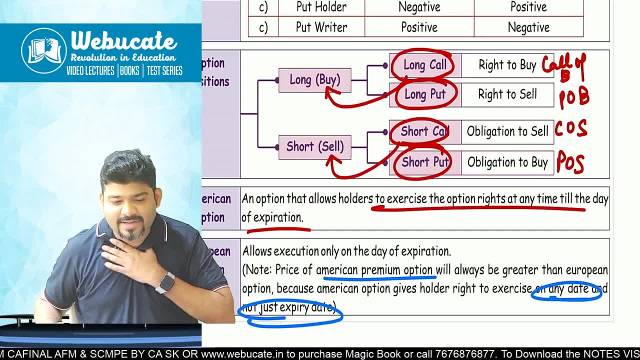 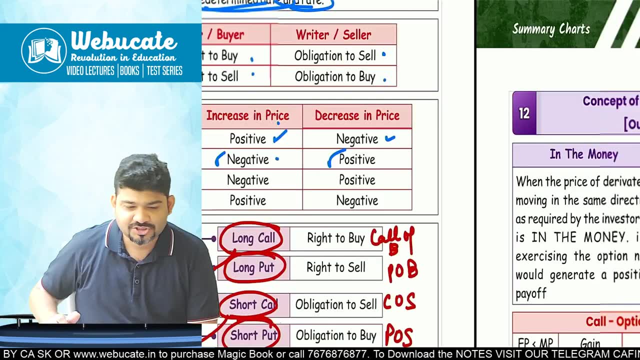 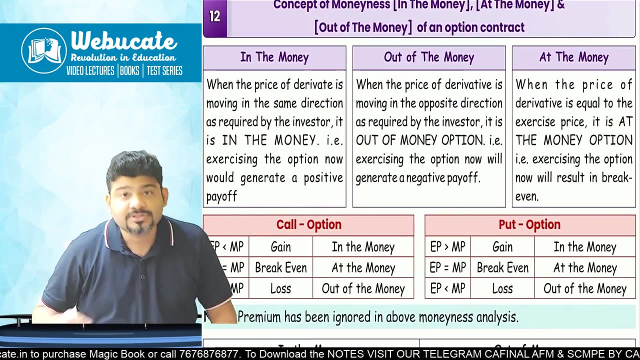 yes, so rightly said by money that, uh, open ended is like american option: exercise it whenever you and the other is the close ended. okay, now we move on to the next concept, and that is called as in the money out of the money and at the money option. okay, so what is in the money if the market is going as per your expectations? 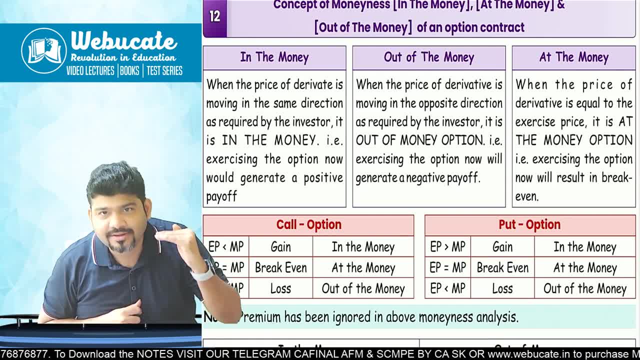 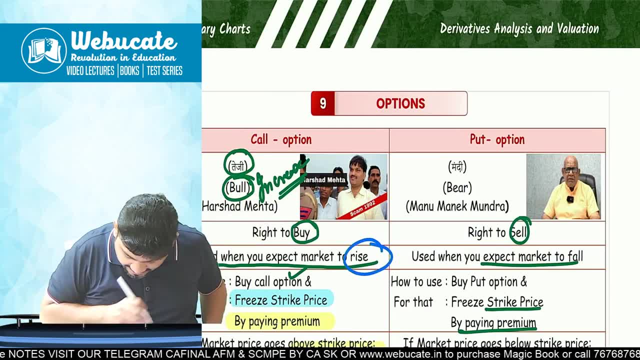 meaning you have taken a call option. what is your expectation? that the market should go up again? i'm telling you guys, be clear. with this call option, you expect the market to rise. put option: you mark- expect the market to fall. so if the market is going as per your expectation, you expect the market to. 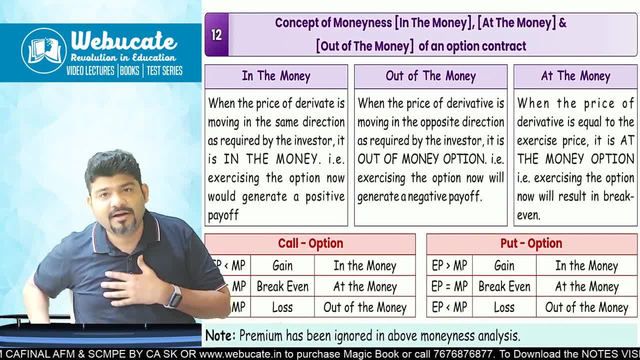 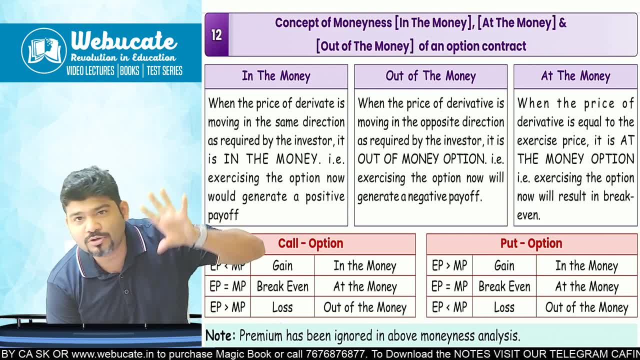 rise put option. you expect the market to fall. so if the market is going as per your expectation, it means that the market is in the money, and if the market is not going as per your expectation, the market is out of the money. okay, if it is actually as per what you are expecting, then it is at the 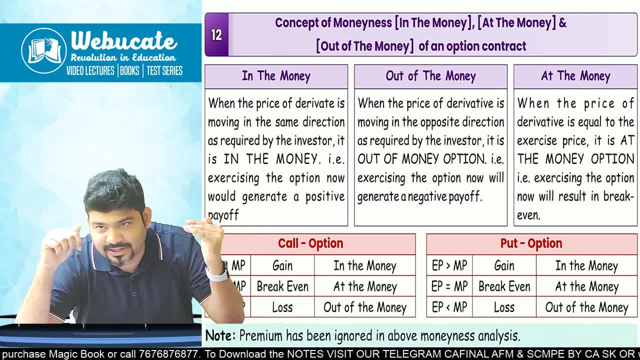 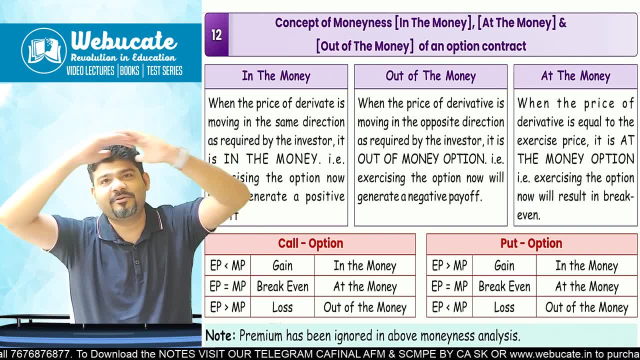 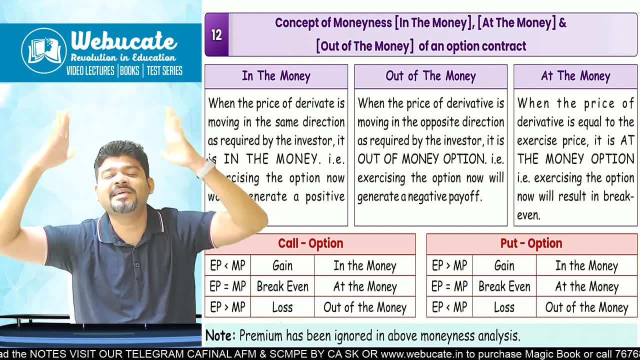 money, as in suppose you have freezed at 1000, you have paid 20 rupees as premium, so you want the market to go till 1020 at least. so it will become at the money: thousand rupees, twenty rupees, you above. so 20 rupees profit, premium paid, 20 rupees. zero is at the money. if it goes beyond that in the 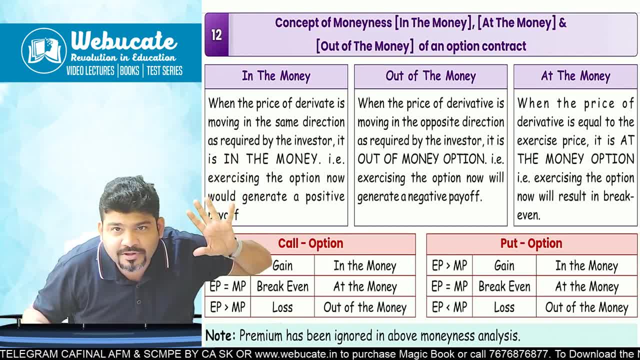 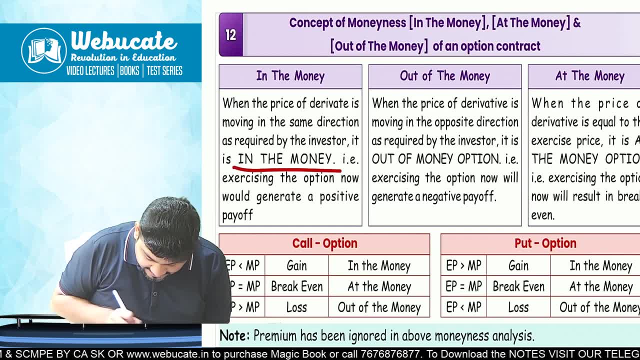 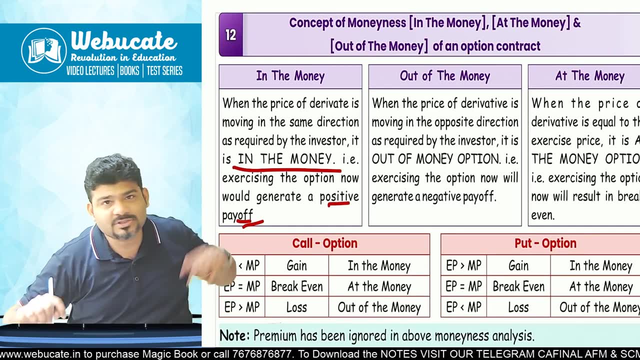 money. if it goes below that, it is out of the money got it. when the price of a derivative is moving in the same direction as required by the investor, it is in the money that is. exercising the option would generate a positive payoff. so in case of call option, you want the market to go up. 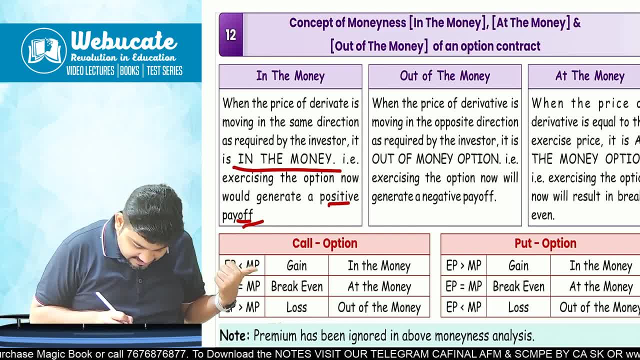 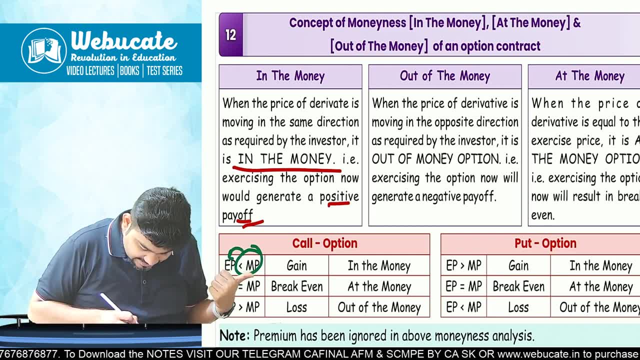 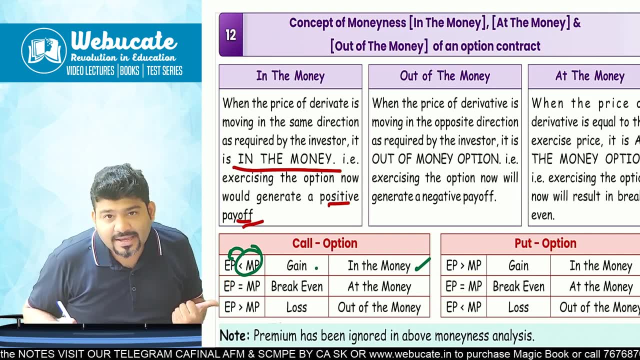 right. so exercise price is less than the market price. meaning exercise, meaning market price. meaning market price is greater. meaning market price is greater than the exercise price. it is a gain. it is in the money equal break even at the money. some size rise is greater than market. 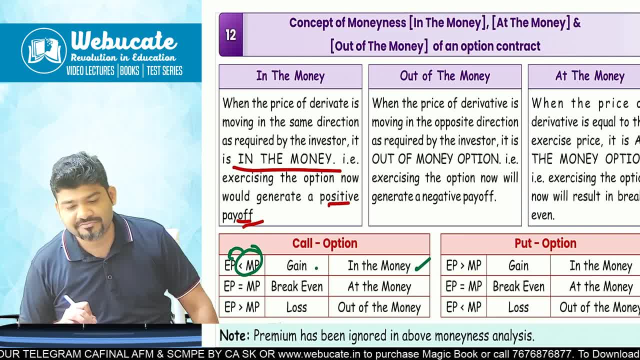 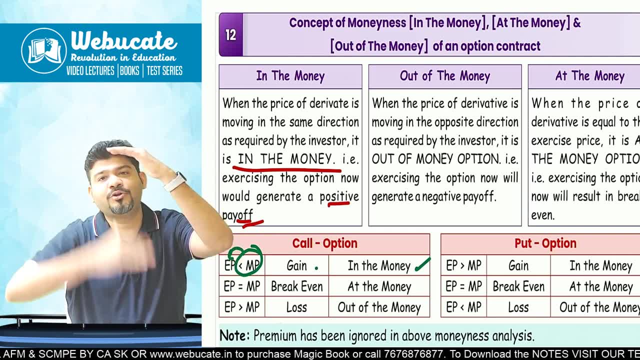 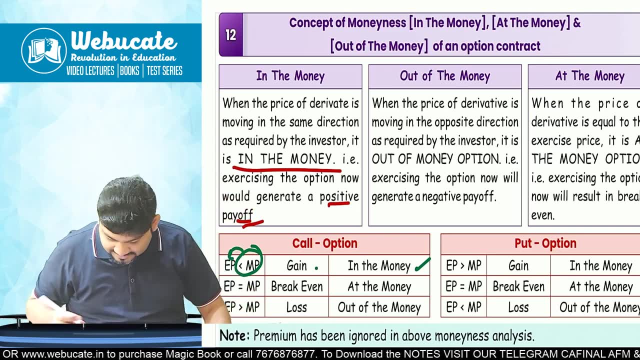 price, Oh, it is a loss and that will be out of the money. and in case of put option, vice versa. you expect the market to go down and it goes down, so you want the market price to be low than the expected price. so here you want the market price to be low, so exercise price high. 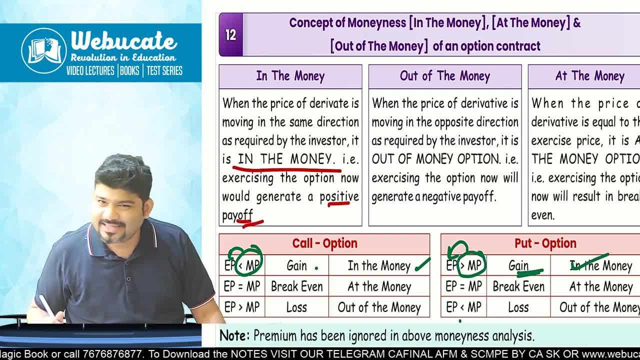 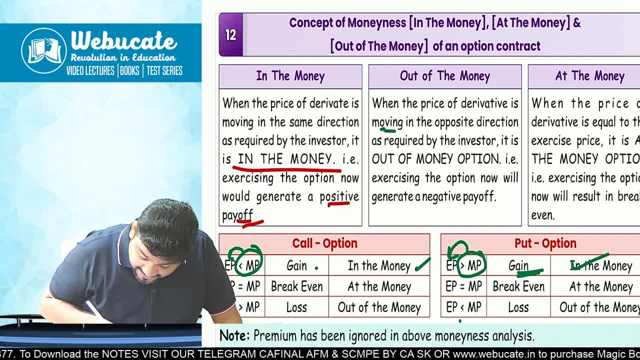 market price, low gain in the money. then at the money and out of the money. are we clear everybody? yes, sir, so that is called as the moneyness. when the price of derivative is moving in opposite direction, as required by the investor, it is out of the money and the price of derivative is equal. 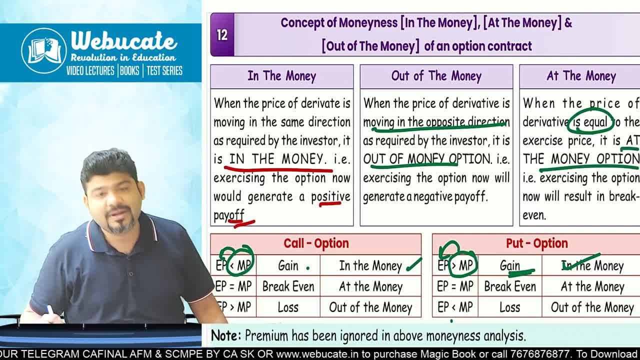 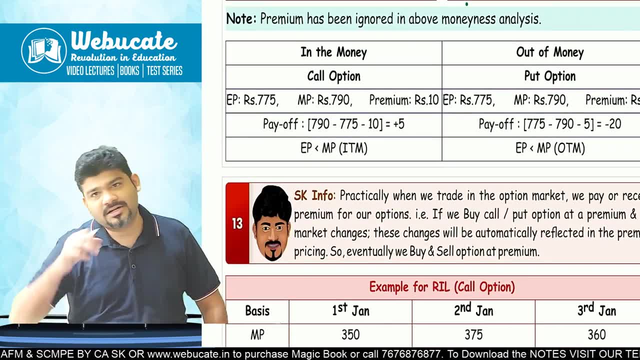 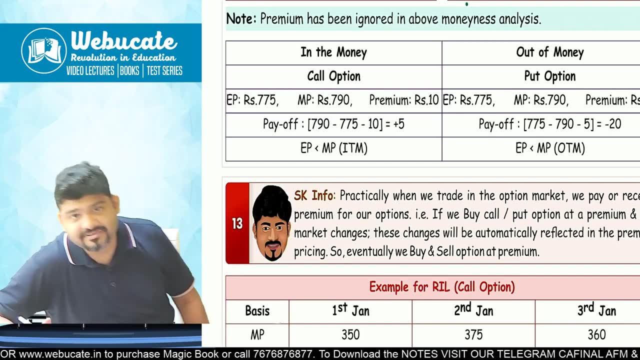 to the exercise. it is at the money option done, sir, no worries at all. so again, if you consider the premium, so that premium amount will be adjusted, which i had already told you in the example time. now i have taken a specific example for you in case of in the money option, for in the money for. 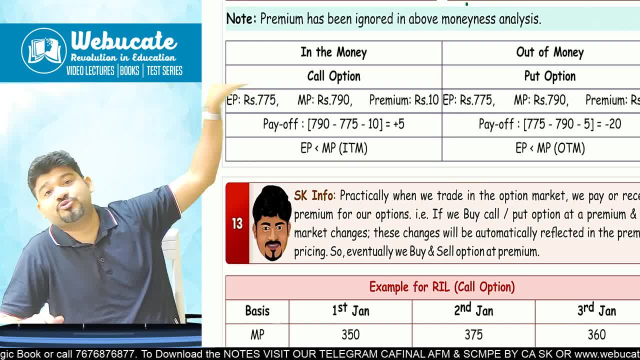 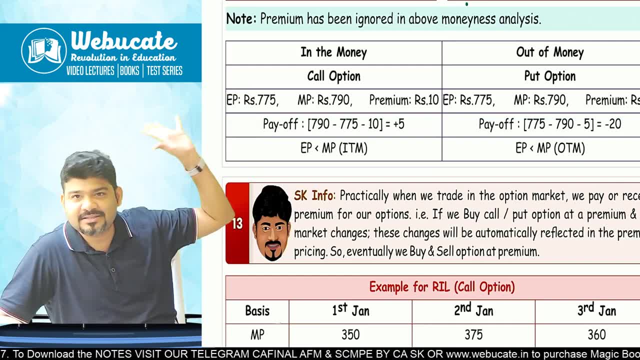 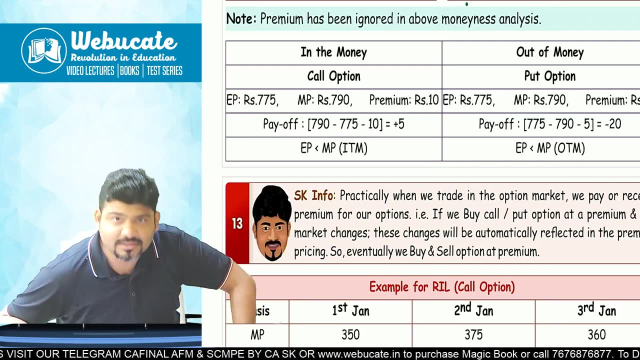 call option. suppose your exercise price, the price at which you have reached, is 775, market has gone to 1, 790. so can i say 15 rupees is the profit that you are making in the money premium paid, 10, 5 rupees is the payoff in the money. the moment, remember this. the moment. exercise price, sorry, the moment. 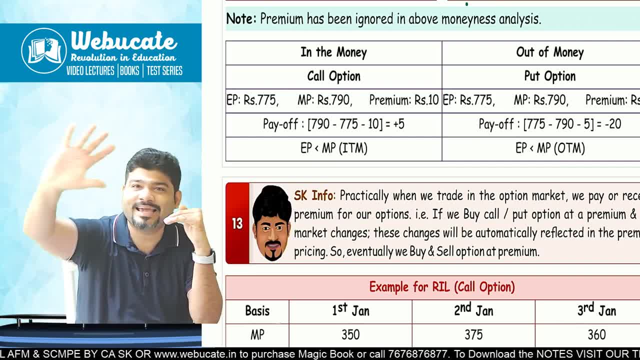 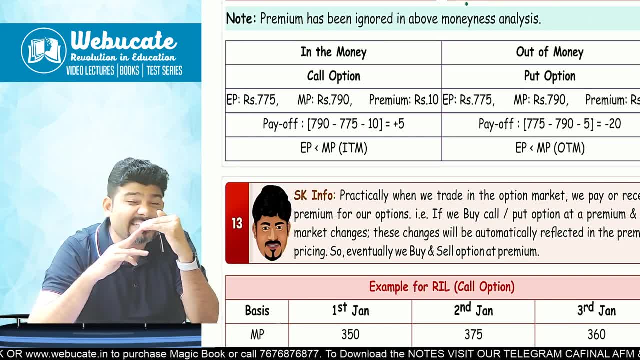 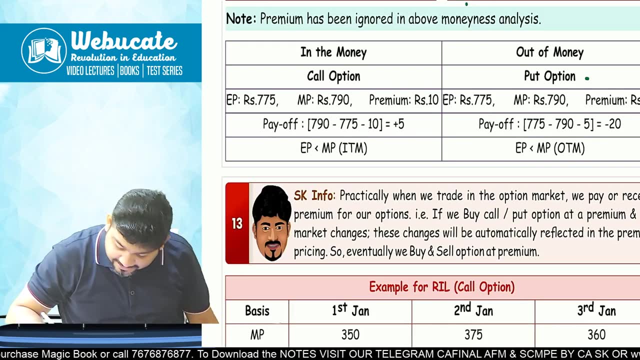 market price is more than the exercise price. in case of a call option, it is in the money, irrespective of premium and the moment market price is less than the exercise price in case case of put option, it is in the money and vice versa, out of the money put option. let's see. 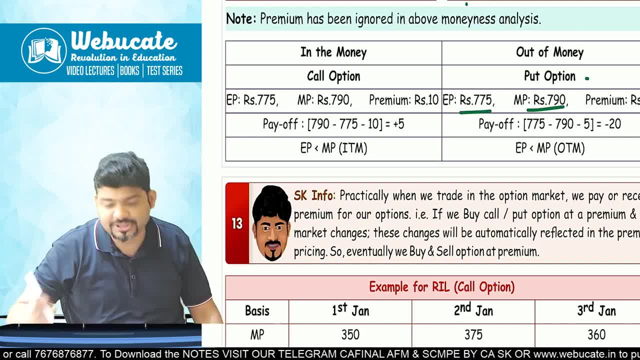 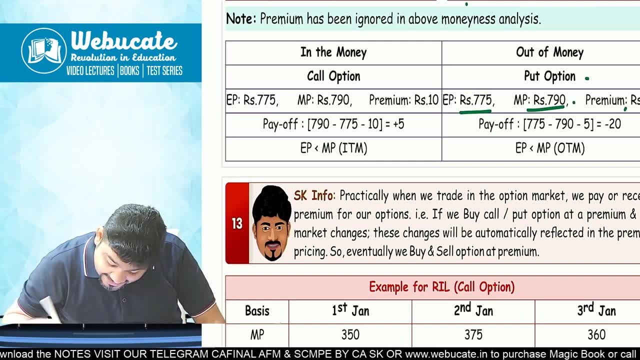 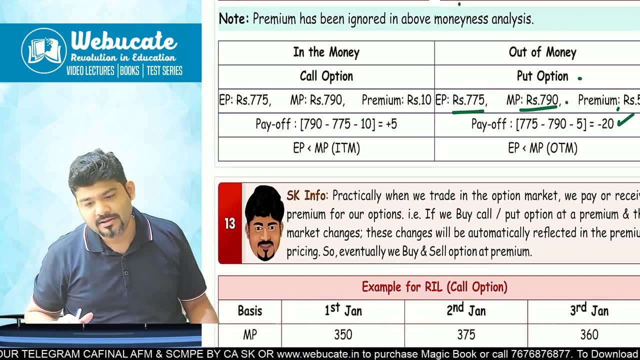 exercise price: 775. same position. market price 9, 790. so can i say payoff will become 775 minus 790 and the premium paid is a different thing. so overall 20 is the loss exercise price less than the market price out of the money exercise price. in case of call option: exercise price less than. 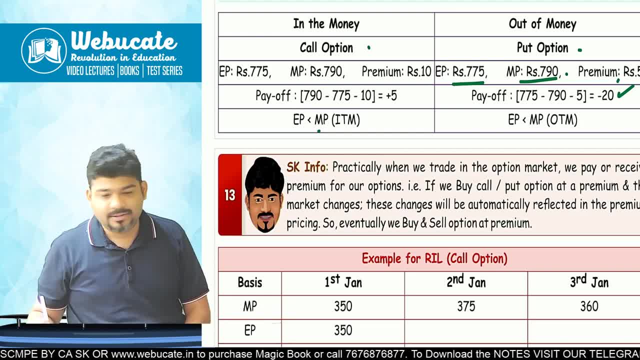 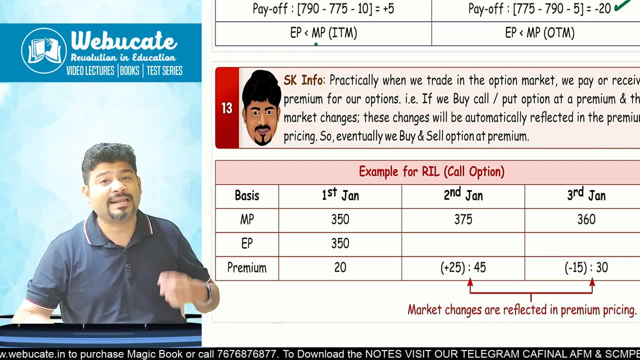 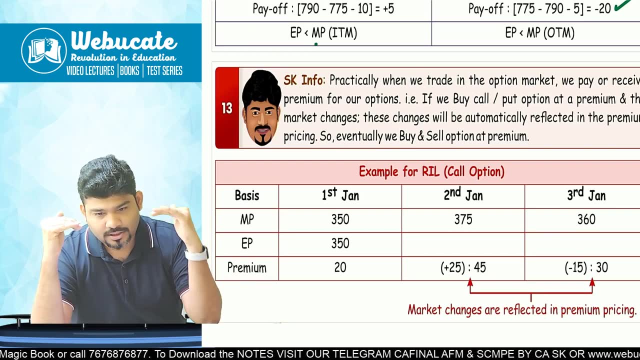 the market price in the money got it done. now some additional information that i want to give you practically. how does it happen? practically, what happens is you trade in the premium, as in suppose you take a call option, you pay a premium of 20 rupees. okay, you have taken, you have freeze the. 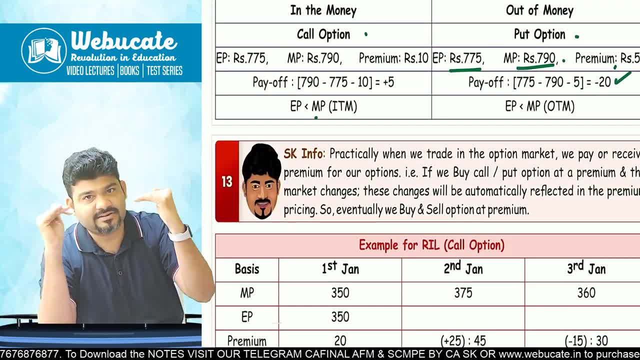 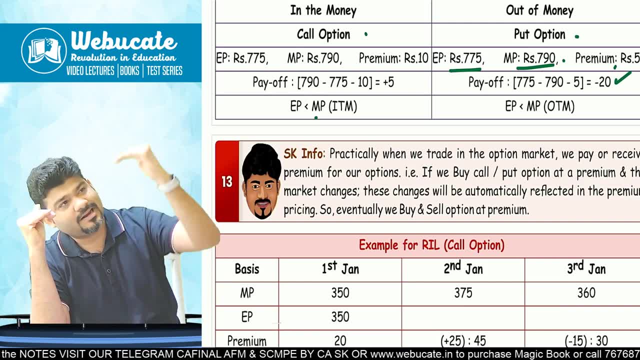 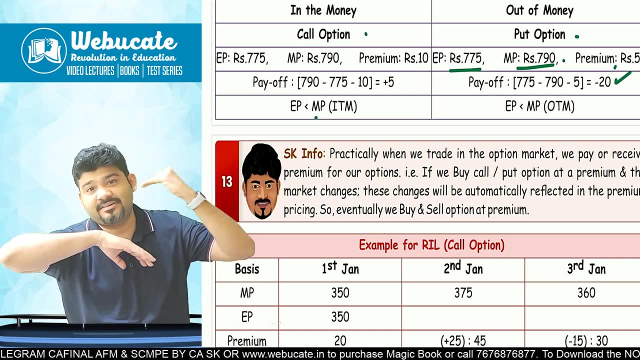 price at 775, as in our case, 775 rupees. you have taken, uh, 10 rupees premium. you have paid. okay, now, when the market goes up, It is the premium which will change. So you have bought the call option 775- freeze price by paying 10 rupees. 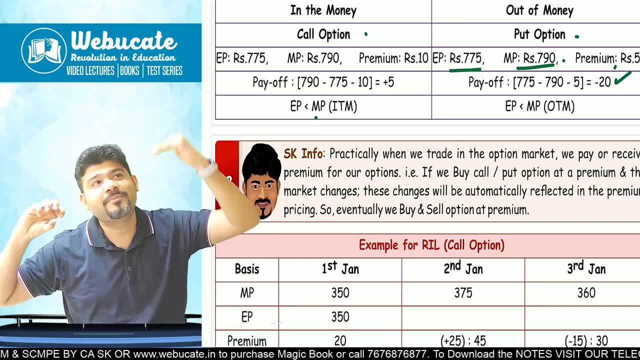 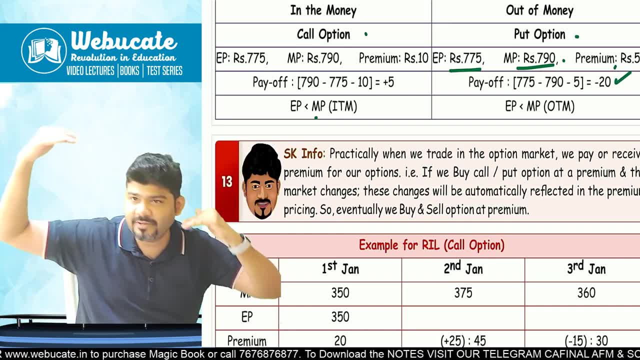 Now if the market goes up, hello, if the market goes up, then in that case this premium will also increase. because you have taken a call option. you want the market to go up, the premium will increase. Now suppose this premium goes from 10 to 18 rupees. you can sell this in the market at. 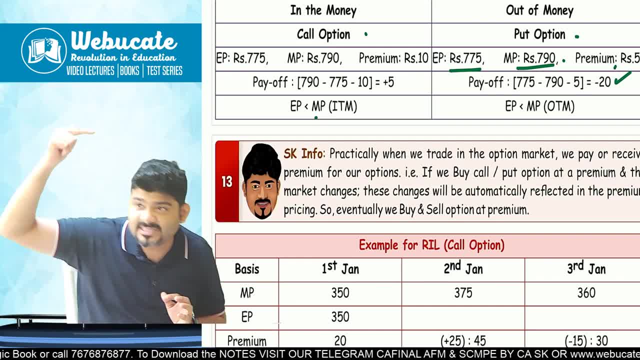 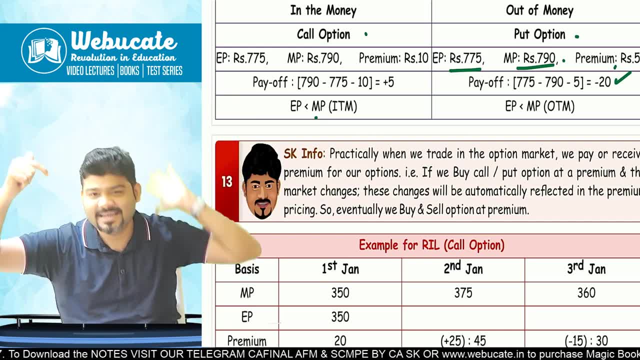 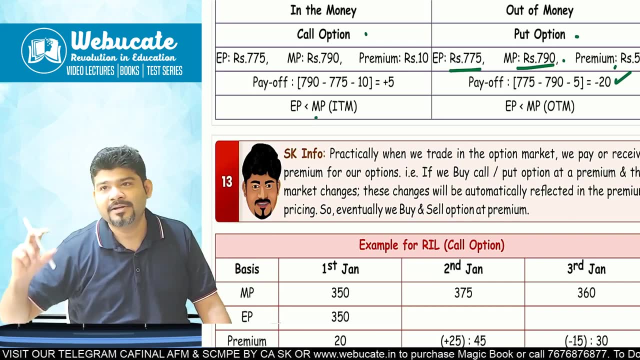 18,, 8 rupees will be your profit. But why did this premium increase? Because the call option market increased here, because the call option market price increased here, and vice versa, in case of put option got it. So the real trade is in the premium, but premium works on the real market price which, if you 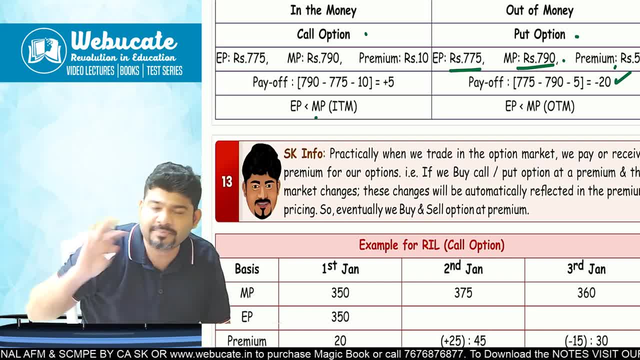 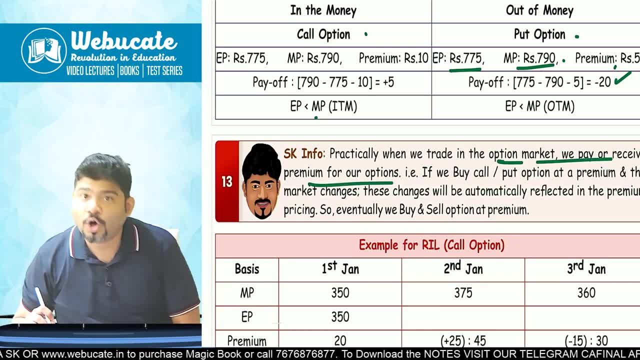 have taken a call. option goes up, premium goes up. you can sell the premium, earn the money. got it. So practically, when we trade in the option market we pay or receive the premium for our options. That is, if we buy or call, put option at a premium and the market changes, these changes. 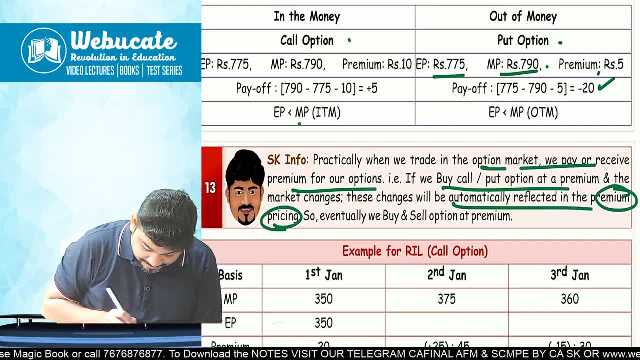 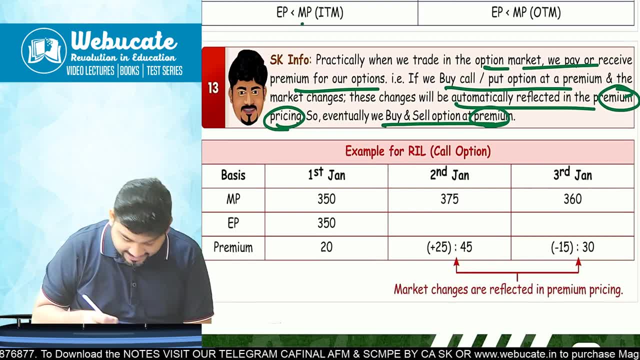 will automatically be reflected in the premium pricing. So eventually we buy and sell option at premium. got it, Got it, sir. Example: see here: market price was 350, exercise price was 350, we paid a premium of 20.. 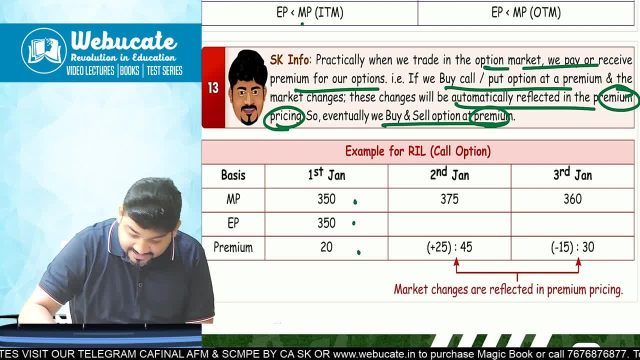 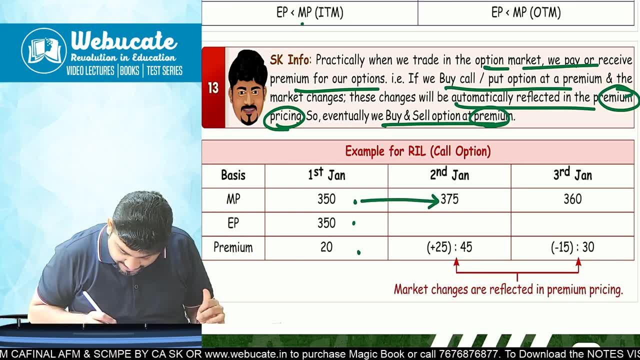 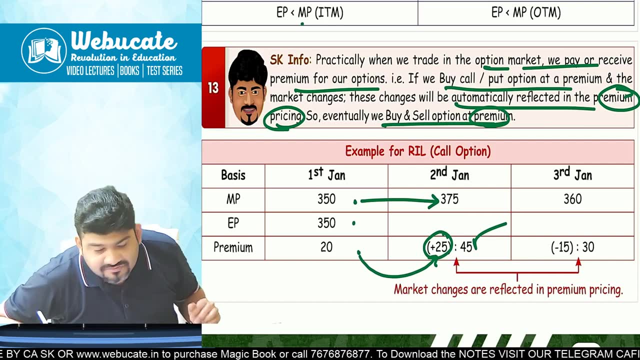 Now suppose if the market price goes to 375, got it. So can I say: 25 rupees increase in the market price, Automatically your premium will increase by 25 and the premium will be reflected at 45. Now you have earned 25 rupees. sell that premium. sell that premium. 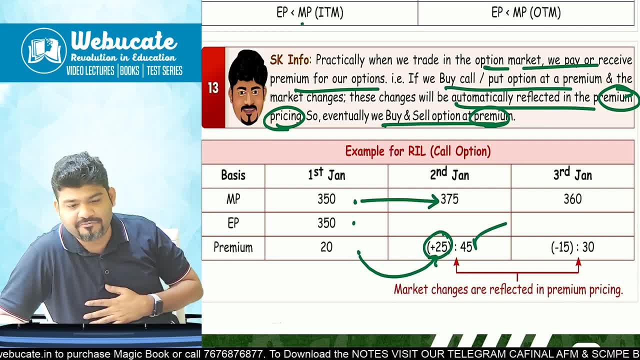 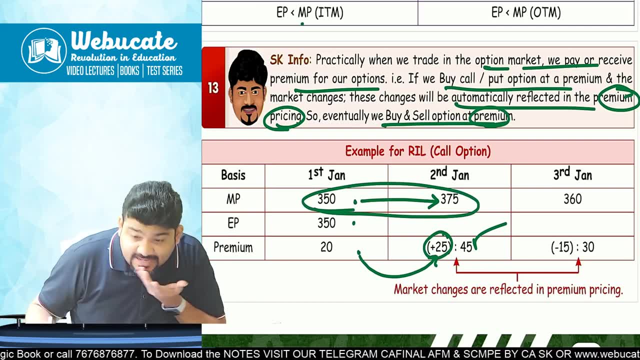 So you will get 45,. you had paid 20,. 25 rupees is your profit, which also happened on account of change in this market price and vice versa. It can also go down, yes, very much, from 375, it can also go to 360, so 15 rupees decrease. 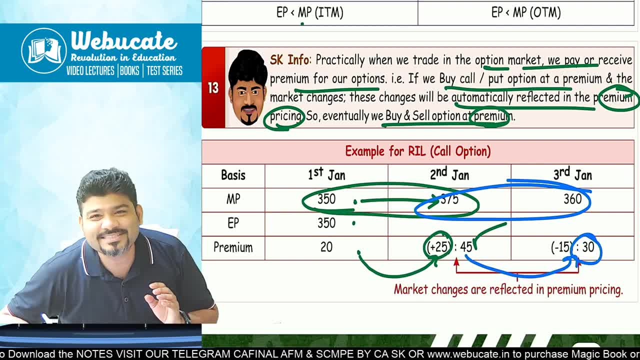 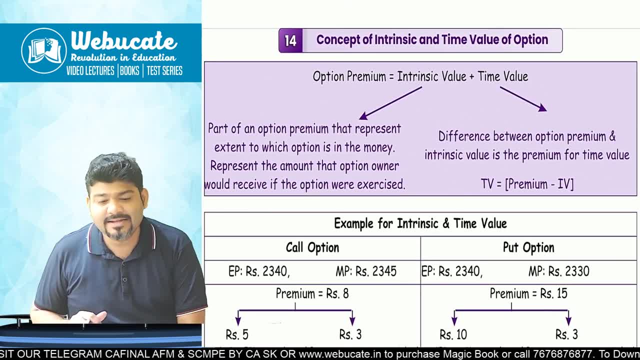 So from 45, now the premium will go to 30 rupees. got it. So that's how Practically the system works. Now we come to the next concept, that is intrinsic and the time value of money. What is this? 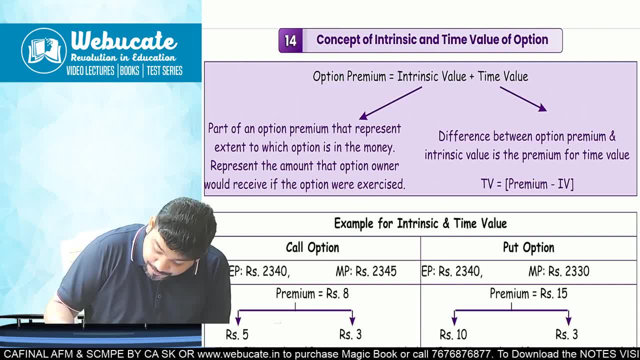 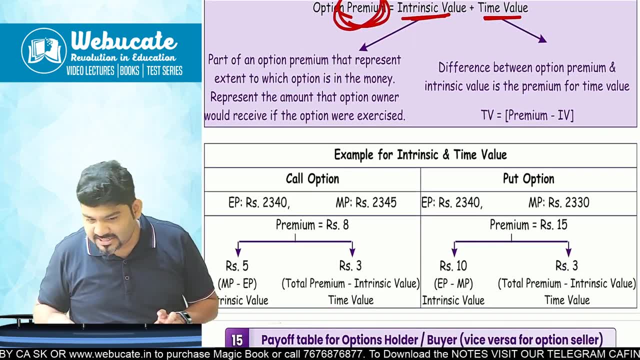 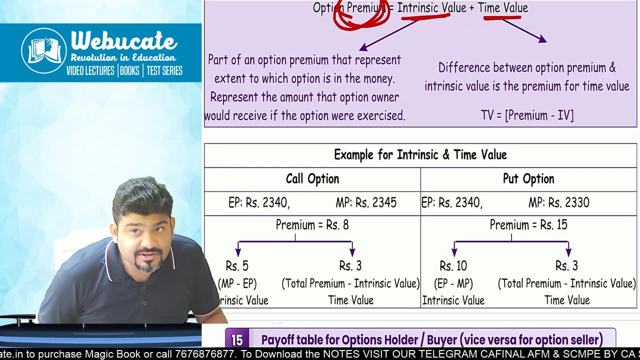 This is the option premium working. So the option premium has two components. One is called as the intrinsic value and the other is called as the time value. I'll explain you with an example. it will be very, very clear easily. Suppose the exercise price is 2340, market price is 2345. 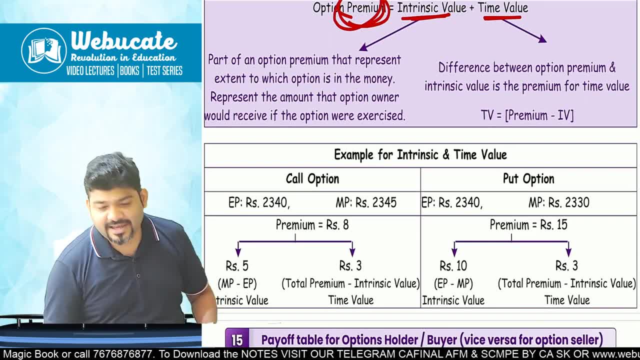 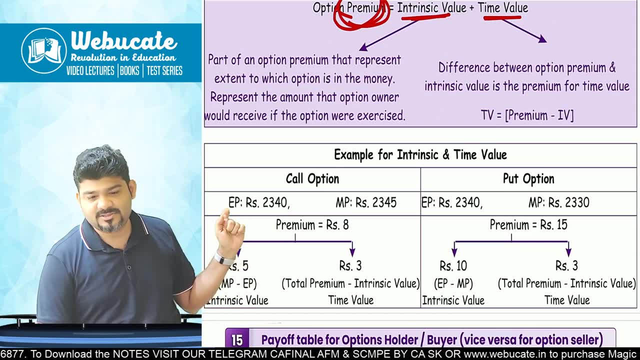 Now look here. Automatically we will gain. See here, See here, See here: This exercise price is 2340.. Pay attention, Hello, This exercise price is 2340.. Market price is 2345.. So you have you freeze this year. 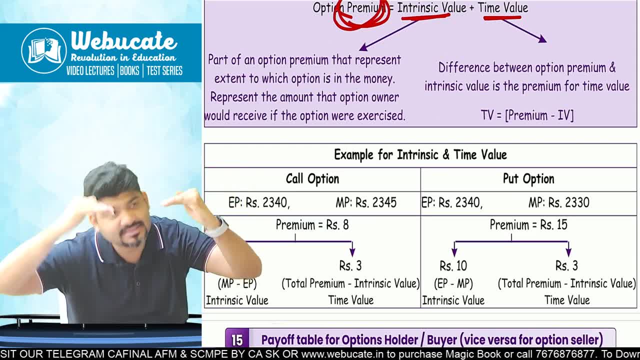 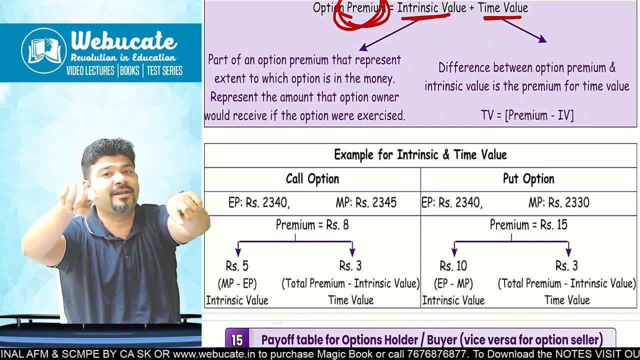 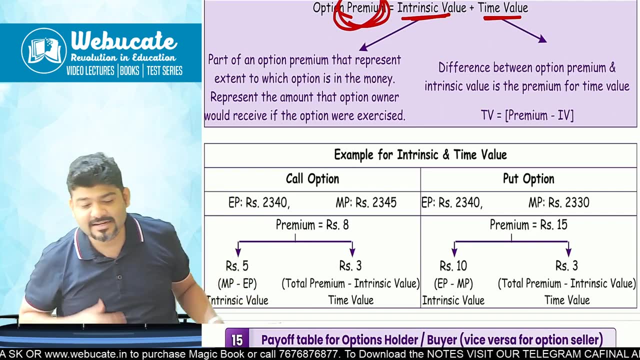 You have a right to buy. So buy at this, sell at 2345, automatically five rupees profit you will make. but that will never happen because that will be the minimum, That will be the minimum premium that you will have to pay And that, basically, is called as the 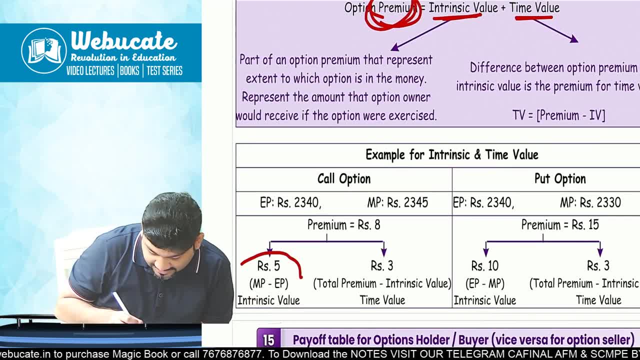 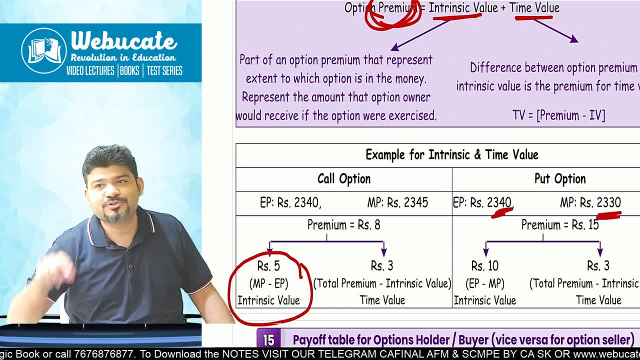 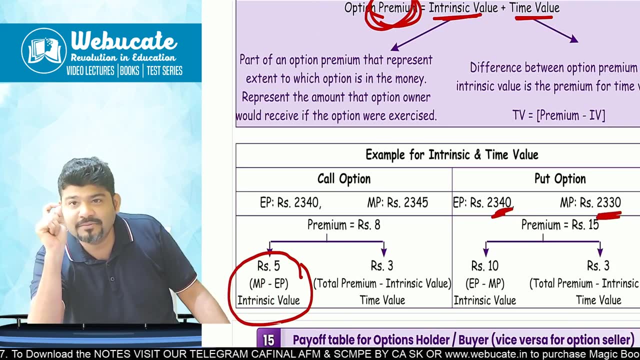 Intrinsic value. that basically is called as the intrinsic value. What it see? a put option: two, three, four, zero, and the market price is two, three, three, zero. So by default, 10 rupees. you are making a profit. Yeah, you will never be able to make that because that will become your premium. minimum intrinsic value of premium. 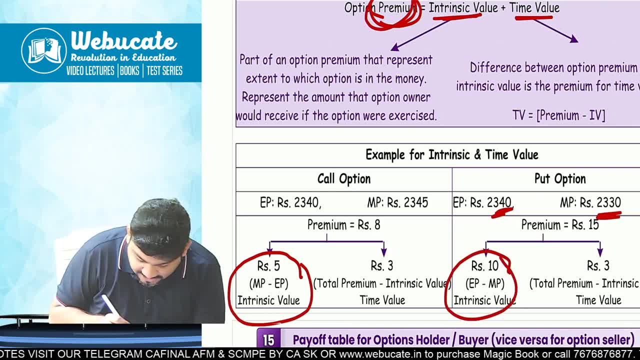 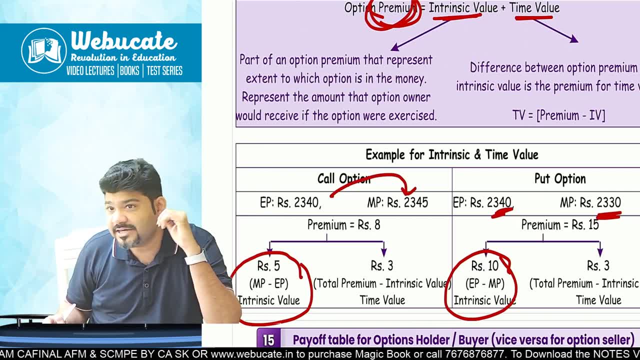 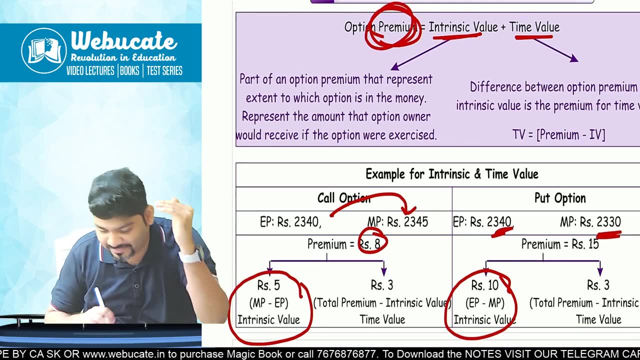 But suppose now you see that premium search all of 45 rupees. We understand about five rupees. We understand because two, three, four, zero, two, three, four, five or five rupees is the premium. But instead Of that suppose the premium is eight rupees, then so three rupees extra, three rupees extra that you are paying is called as the time value. 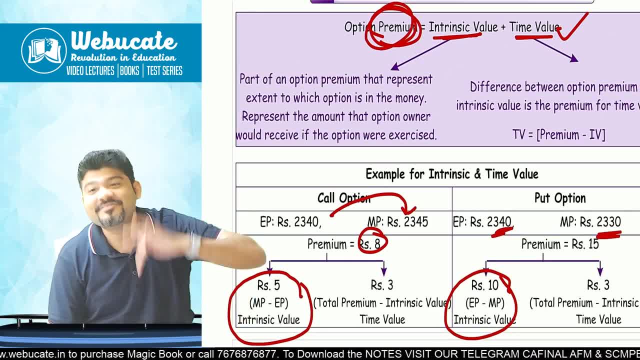 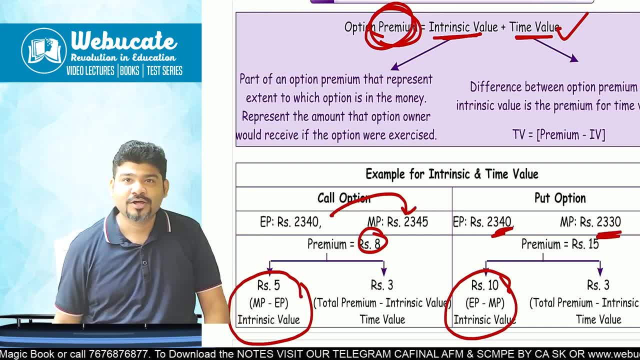 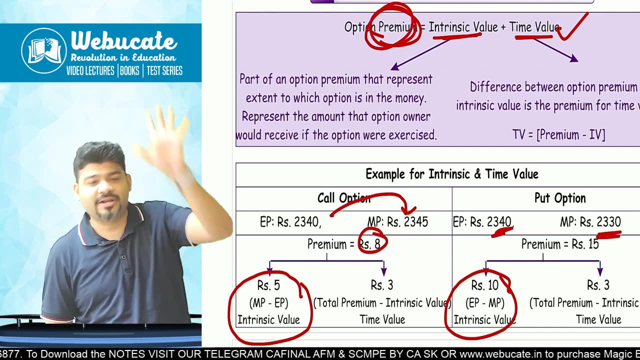 So the premium that is justified will become your intrinsic value. Any additional premium that the market is taking from you is called as the time value. What it guys? the concept of intrinsic value and the time value in premium, These are the things which will definitely be asked in your MCQ. 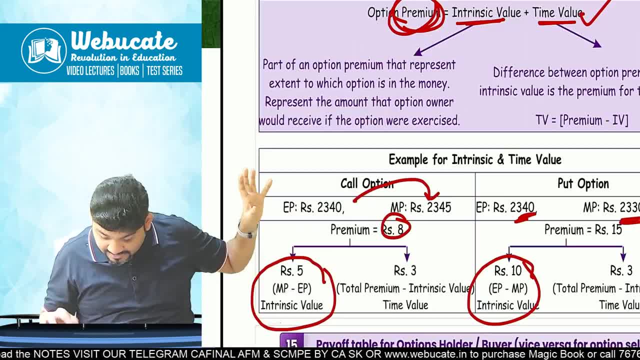 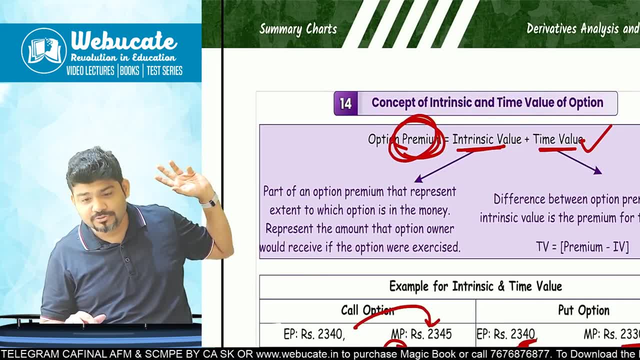 This in the money, at the money, out of the money. Oh, this in the money, out of the money, at the money thing. they will ask you in the MCQ this concept of intrinsic value and time value. They can ask you in the MCQ, suppose, if put option is there, think and answer me. 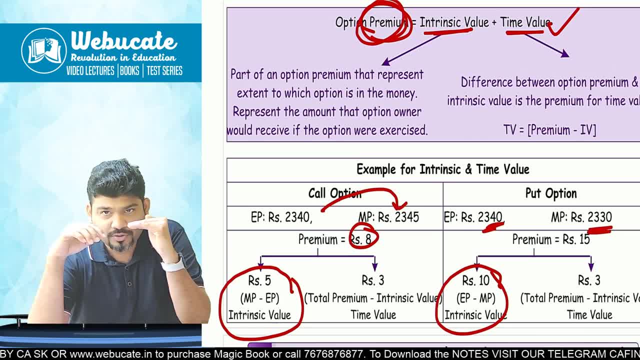 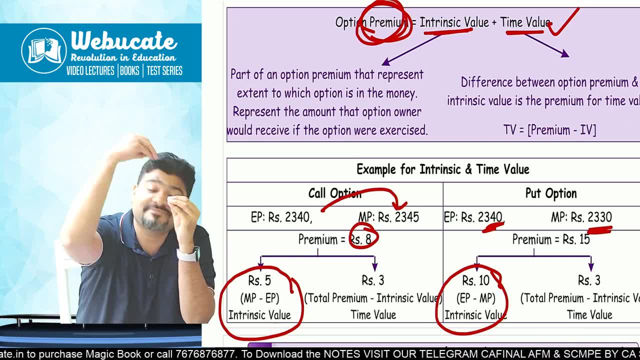 Now put option: is there two, three, five, zero? and suppose the market price is two, three, three, zero, So by default 20 rupees differences, that that will be the minimum premium intrinsic value, But suppose instead of 20.. The premium Is 27 rupees. 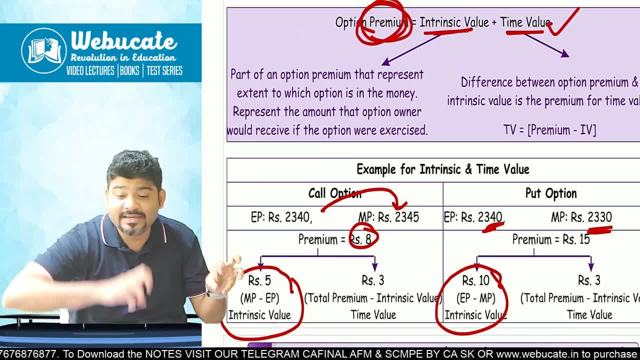 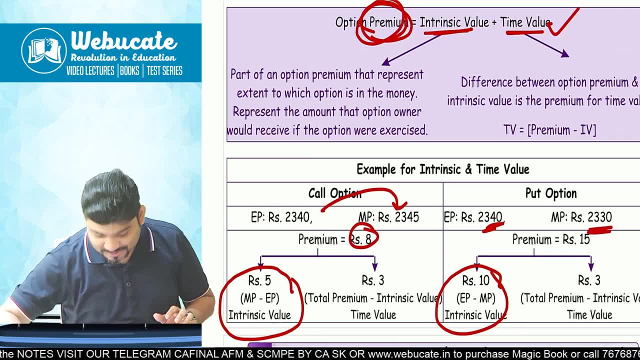 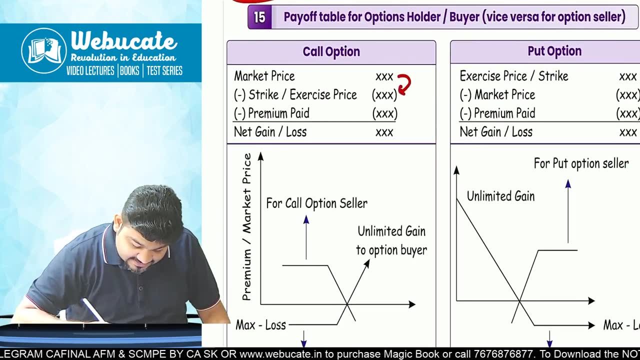 So 20 rupees intrinsic value. seven rupees is the time value. Total: 27 rupees. Everybody. Yes, sir. So that's how the premium books pay off table Very easy: market price minus the exercise price, minus the premium paid. 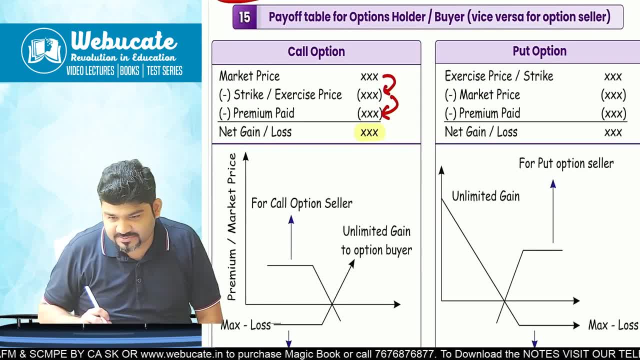 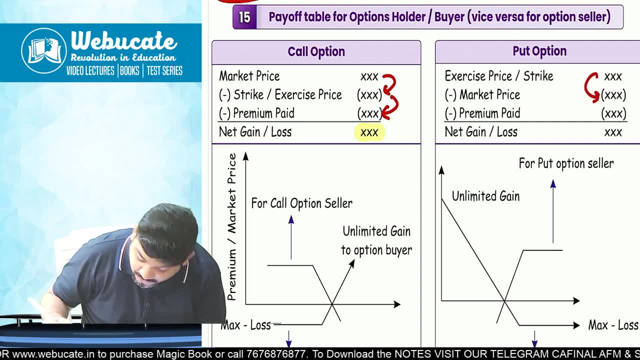 That is your gain or loss, as the case may be. but put option: exercise price. You want the market to go down. You want the market to go down. So exercise price minus strike price minus premium paid. This will be your loss or gain, as the case may. 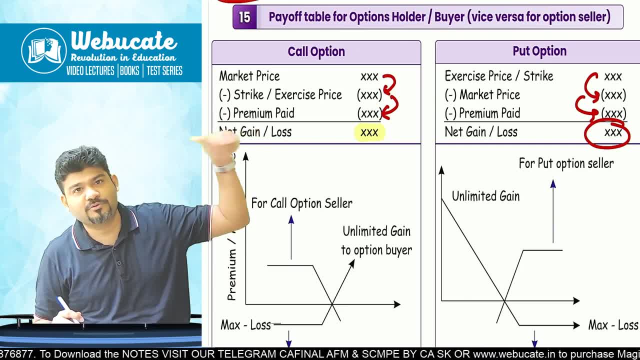 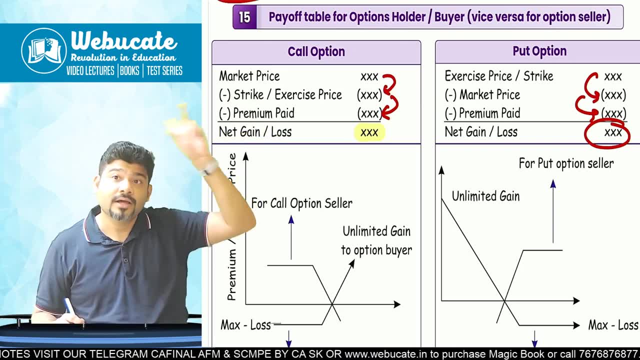 Got it. So we are very clear till here. So in case of call option, you want the market to go up, So market price minus exercise price minus premium paid will be your net pay off. Why save our support option? exercise price minus market price minus premium paid. 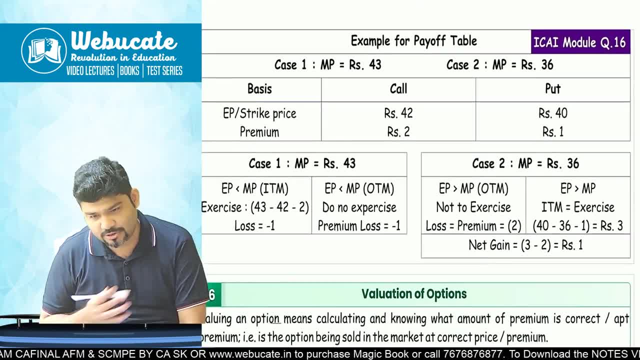 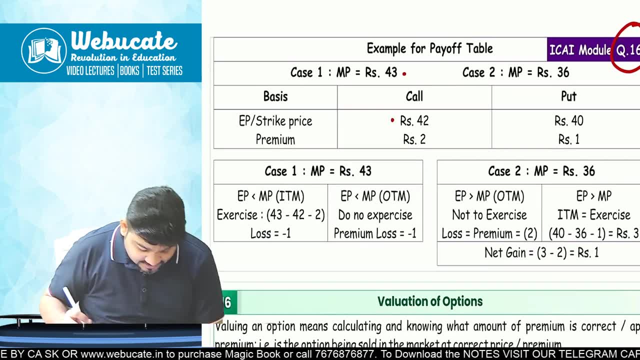 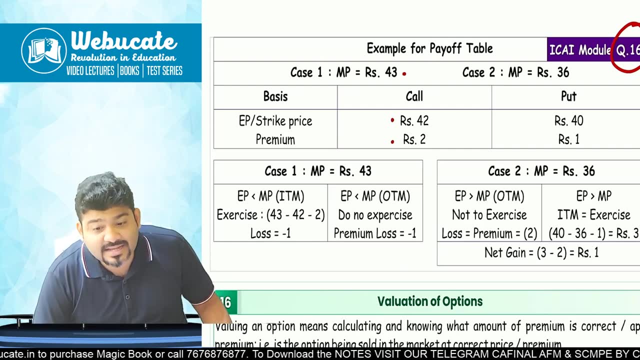 Got it, sir, Done Now. This Can also be taken as an example module question. So suppose the market price is 43. Exercise price, strike price, which we call is 42, premium is rupees two. Then what will be the scenario here? 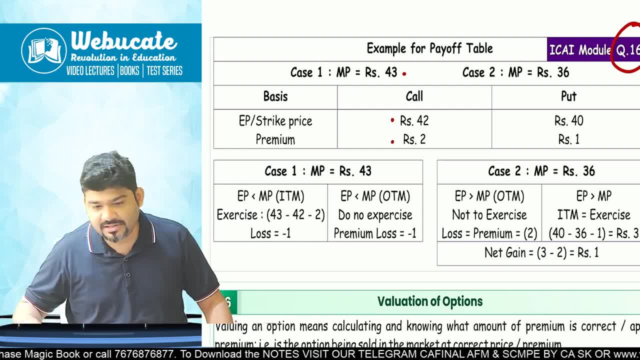 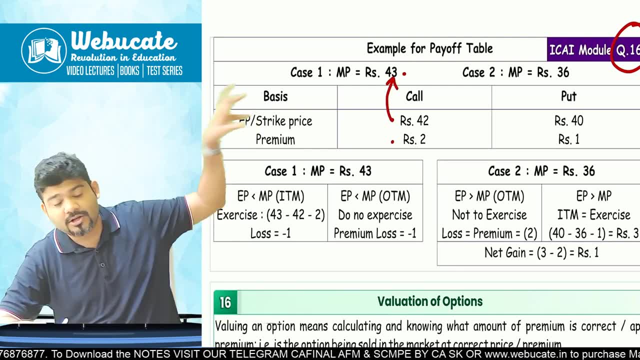 Now market price is 42, 43 and our strike price is 42. So can I say we are out of the money, right, Because we are making a loss. So in call option we want the market to go up. The market has gone up. 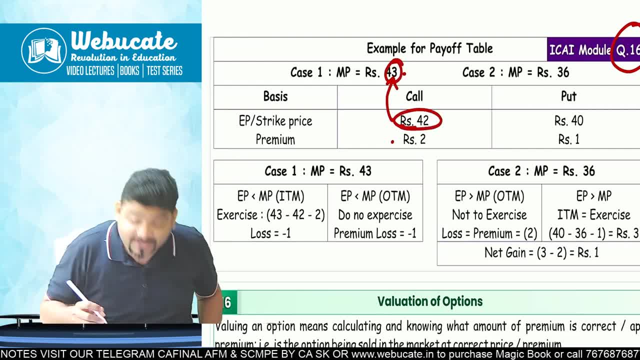 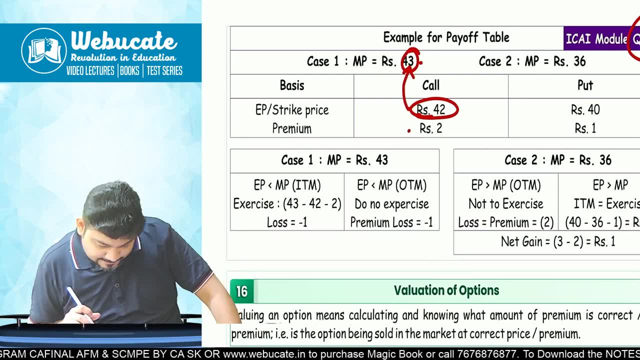 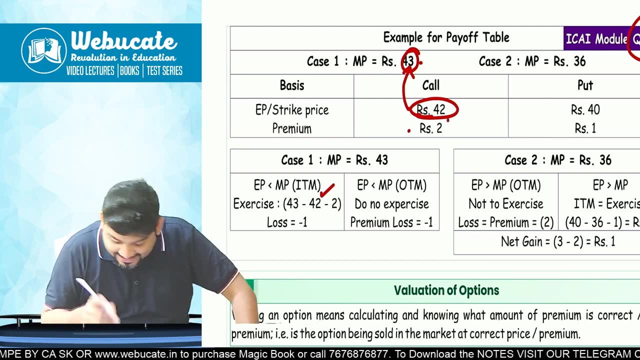 Oh yeah, So strike price 42 and market price 43.. Oh yeah, One rupees extra we are making, So that one rupees will be your gain, Got it? Yeah, So this 43 rupees minus 42, one rupees is our gain premium. 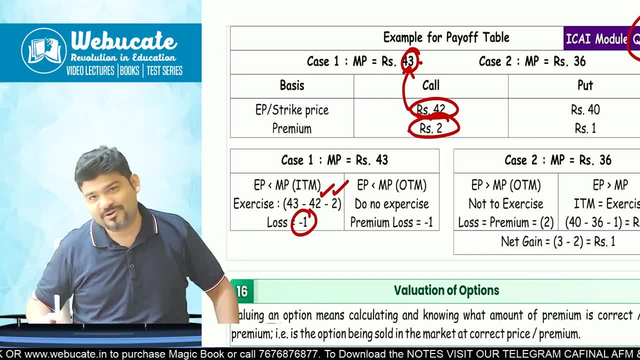 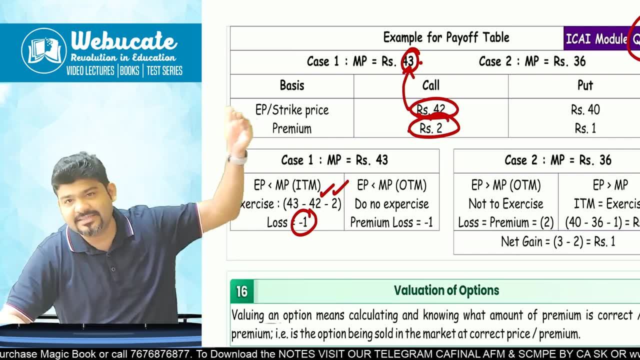 We have to pay two rupees, so that net loss is one rupees. So it is better to exercise. If you don't exercise, premium whole will be gone to rupees loss. But if you are exercising because market has gone little up also, 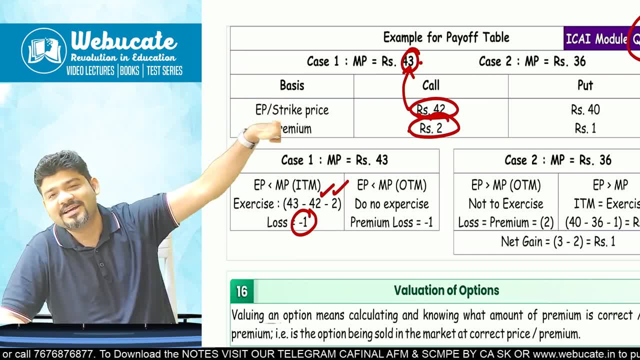 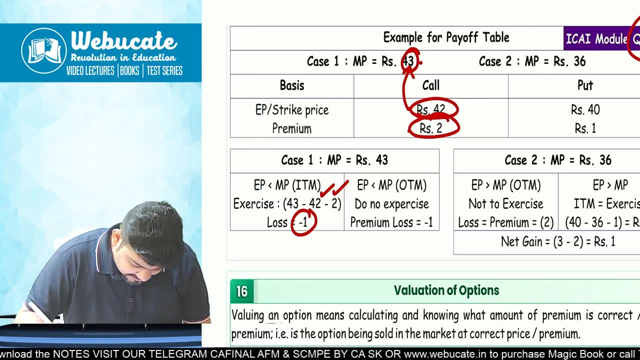 you are exercising, you are at least cutting out on your premium loss from two to one. at least Got it, guys, Done. And here, in case of put option, if you have taken and if the market goes up, you will not exercise the option. 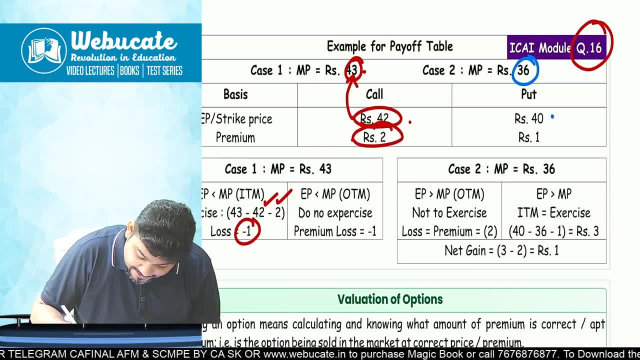 Case two: 36, strike price 40.. Oh, you will not exercise the call option. Two rupees loss there. But here you will exercise the put option. Four rupees profit, But one rupees is your premium, So three. 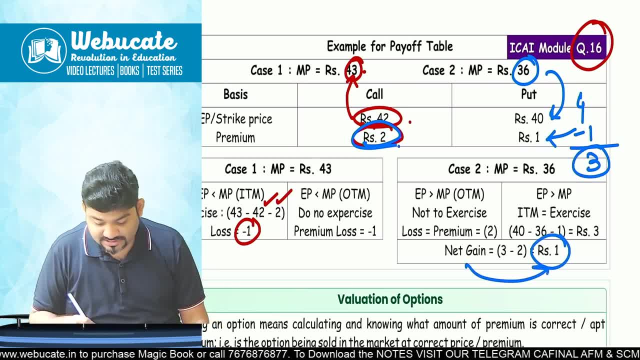 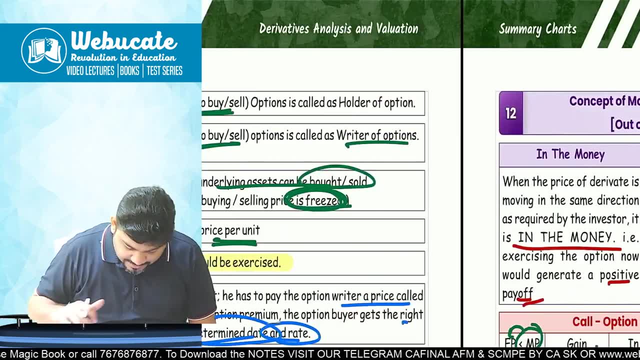 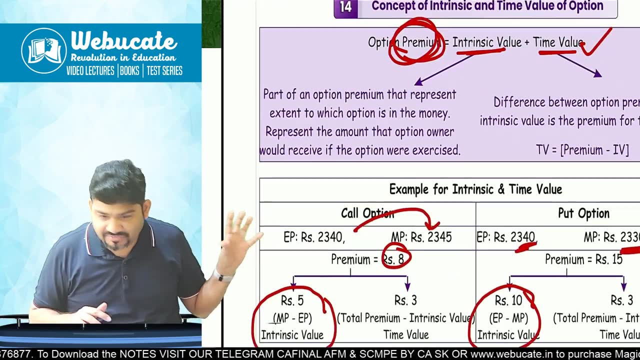 And two rupees loss. One rupees is your net gain. One rupees is your net gain Audit Done. Now with this, the main basic see. this whole chapter is divided into two major parts. One is called as the basic understanding, from which the MCQs will be asked, according to me. 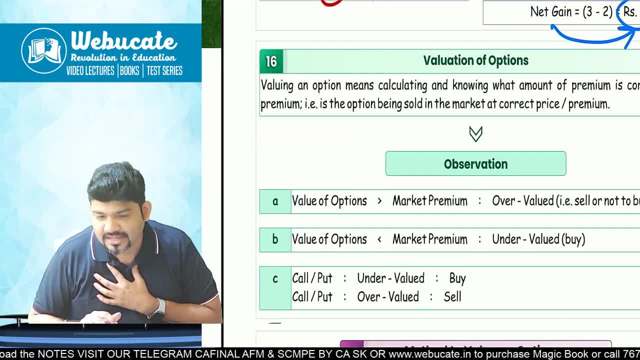 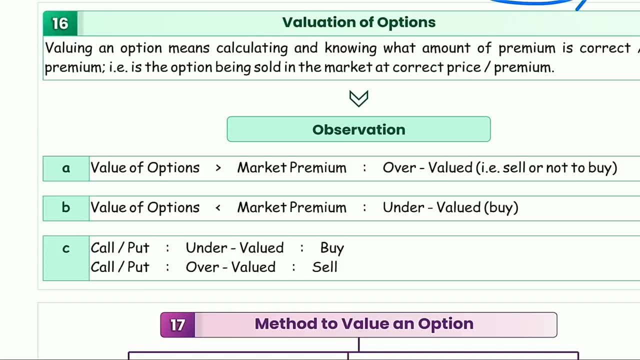 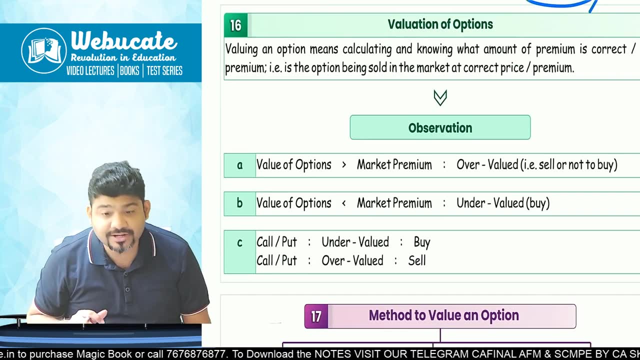 And then is called as the valuation of options. And now we are coming into the concept called as the valuation of options. Let's start, OK. next concept, as I told you, is the concept of valuation. What is valuation of options? 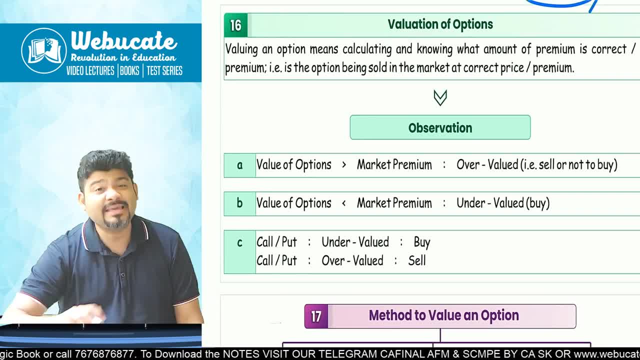 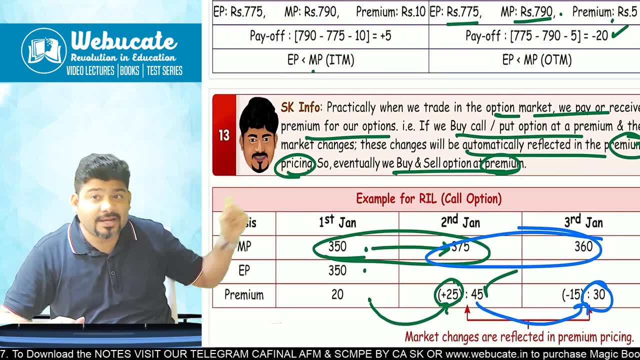 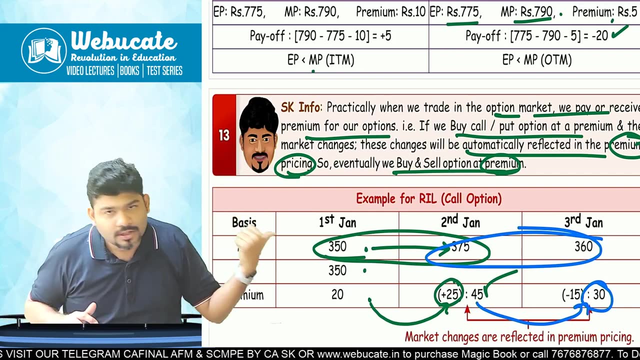 Valuation of options is deciding the premium amount, As you clearly observed here in my this example, I told you it is the premium that moves up and down And you are buying the premium, You are selling the premium. That's what gives you your profit, or could be a loss as well. 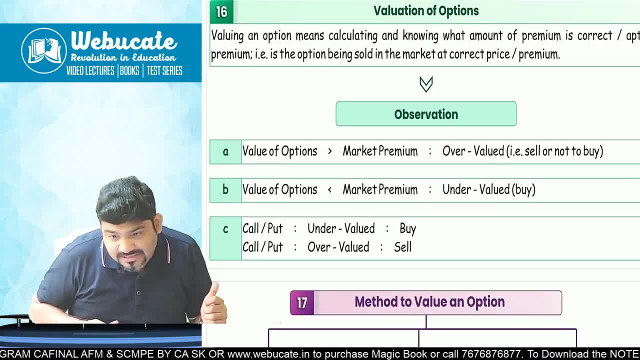 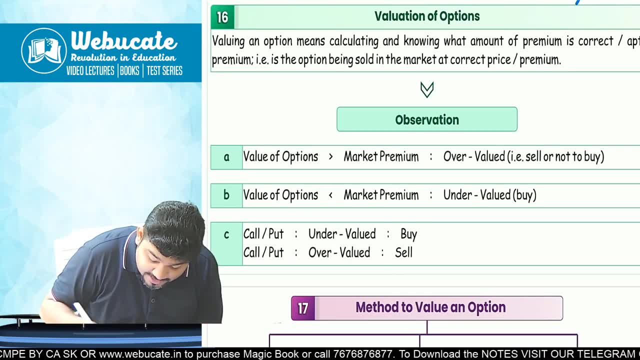 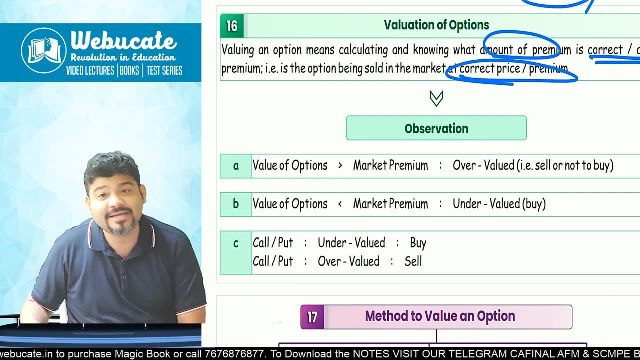 So you're, the valuation of premium is very important, and that's what valuation of options is all about. Valuing an option means calculating and knowing the amount of premium is correct or at premium, That is, the option being sold in the market is at correct price or not. 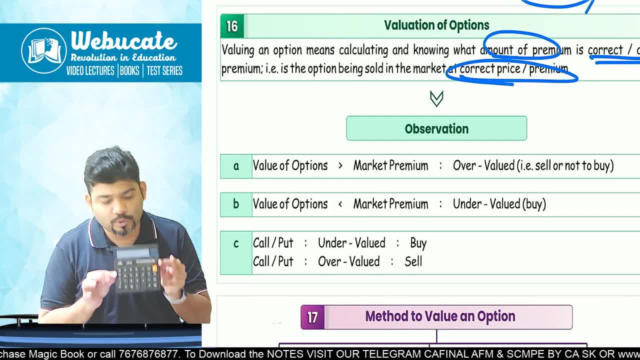 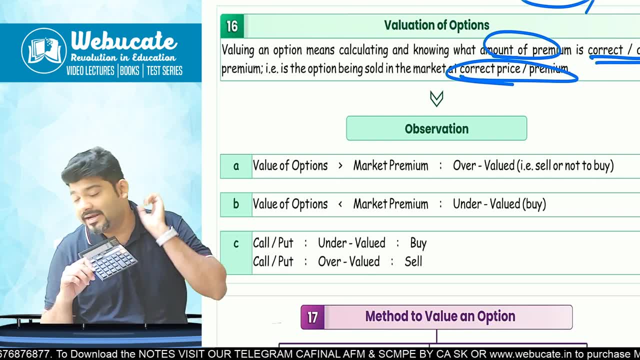 Is that the correct premium or not the way? Suppose, if I go to purchase this calculator, I will check out that this calculator is actually worth 100. But if somebody is selling it at 120, I will not buy it. I'll say: oh my God, why are you selling it at high price? 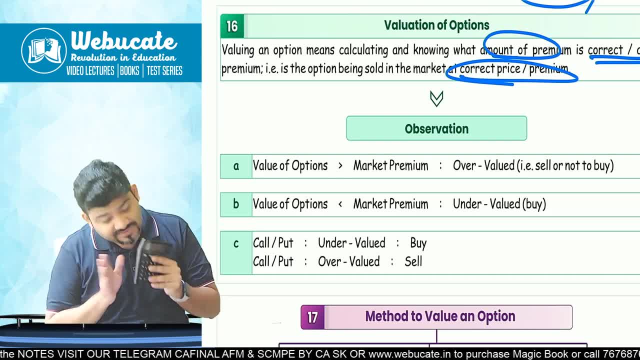 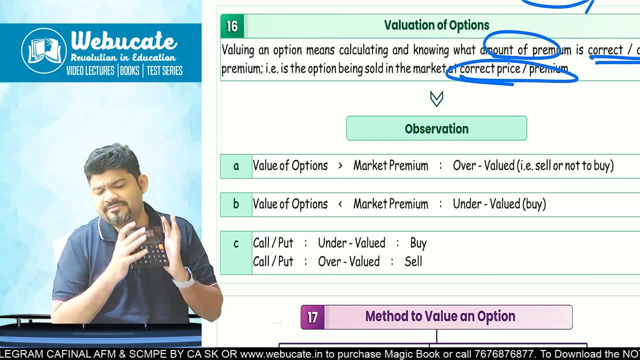 120 is a high price- 20 rupees extra. But suppose if the same calculator is being sold in the market somewhere at 80 rupees. I will buy it because it is being sold at a cheaper price. Eventually it will come at its right price. 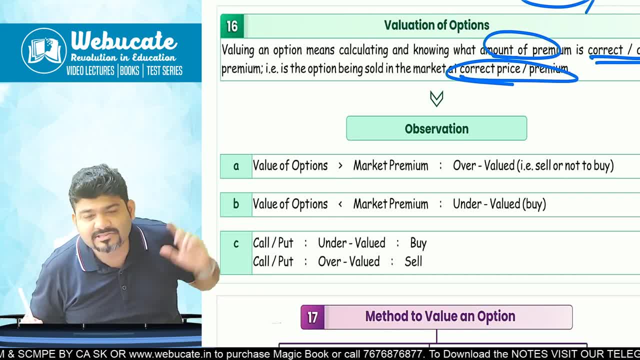 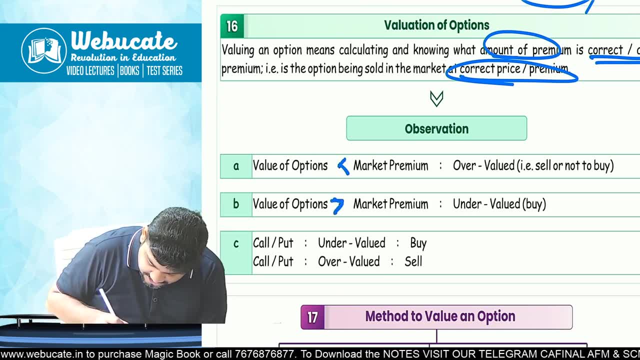 But in the same way, the same logic is to be applied here as well. Suppose: if the value of options say is: Let's change the signs, please change the signs. Suppose value of options is, say, 10 and market premium going on in the market. 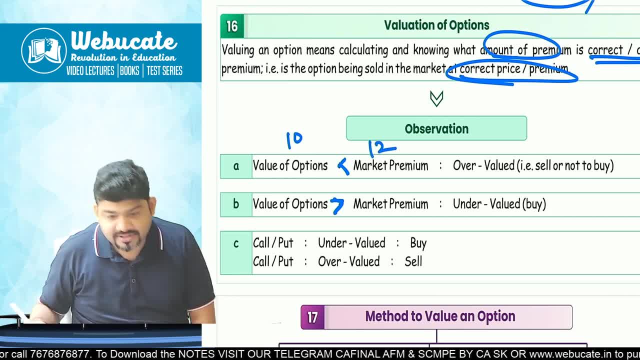 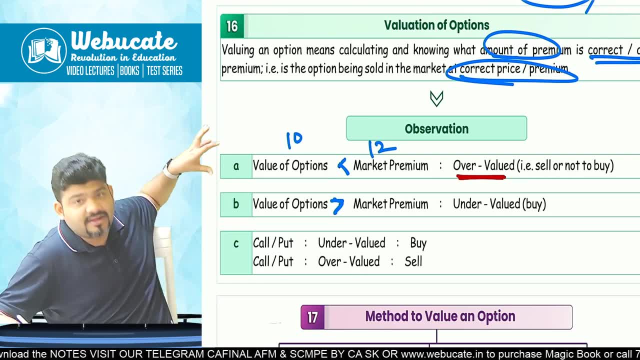 say, is 12,, then we will say that it is overvalued. Because, according to us, what is its real value? 10 rupees. Then why is it being sold in the market at 12?? It means it is overvalued. 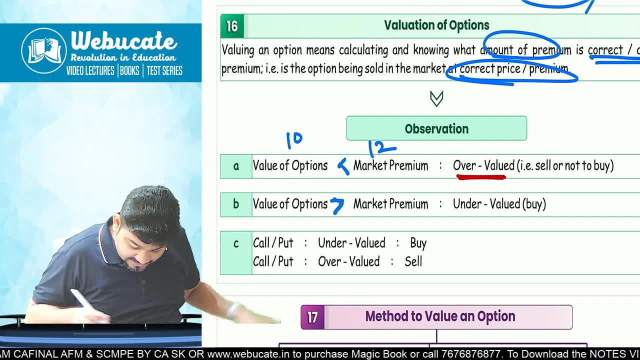 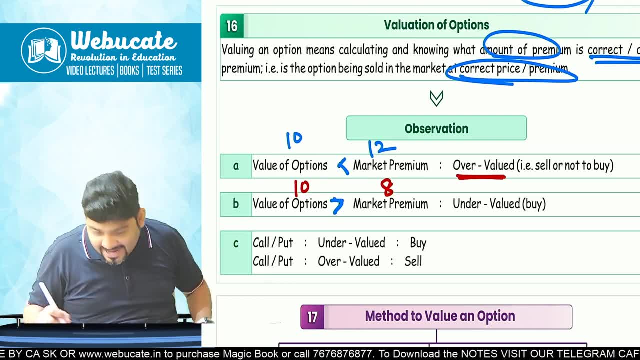 And if value of options is, say, 10 and market premium is 8. Oh, 10 rupees thing is being sold in the market at 8. It is undervalued And we will buy everybody. Yes, sir. 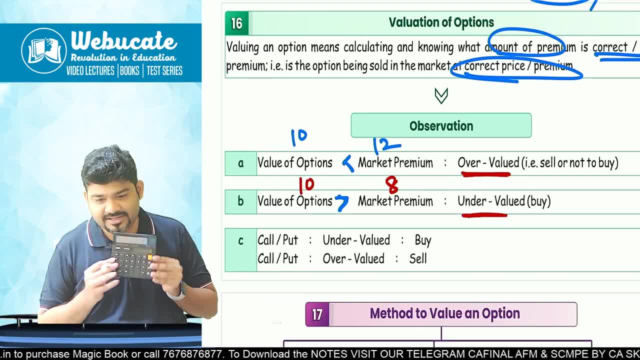 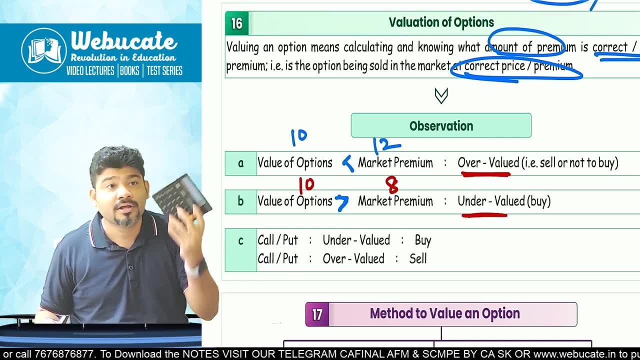 So if anything is undervalued, I told you, if anything is undervalued, 10 rupees value of option being sold at 8 rupees- Very nice, We will purchase this calculator for sure. But 10 rupees calculator being sold in the market at 12.. 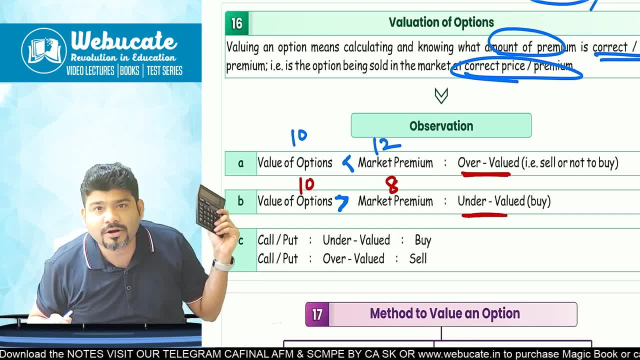 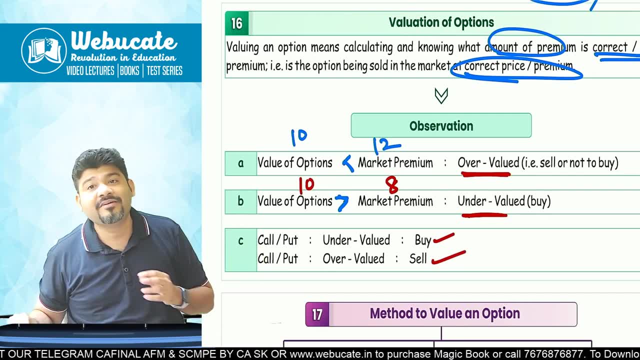 Sorry boss, not acceptable. It is overvalued. We will not buy it, as simple as this. So call option if it is undervalued by call or put option. If it is overvalued, we will sell in the market. 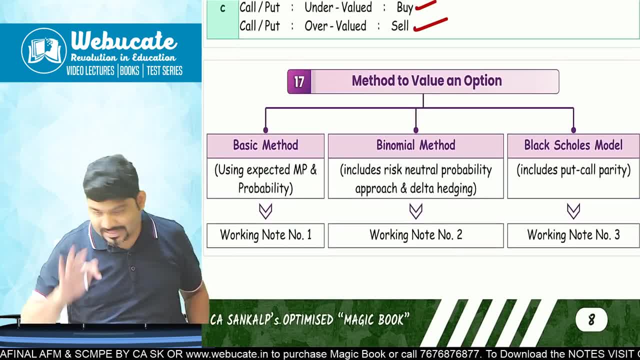 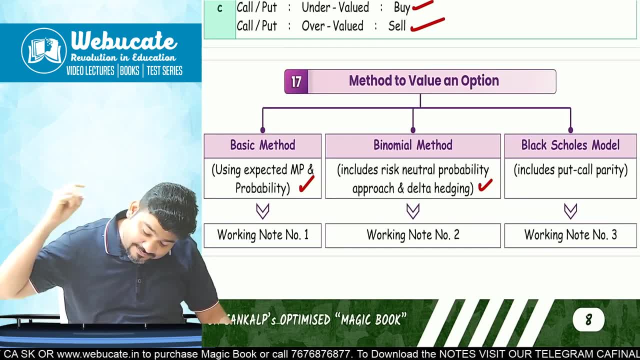 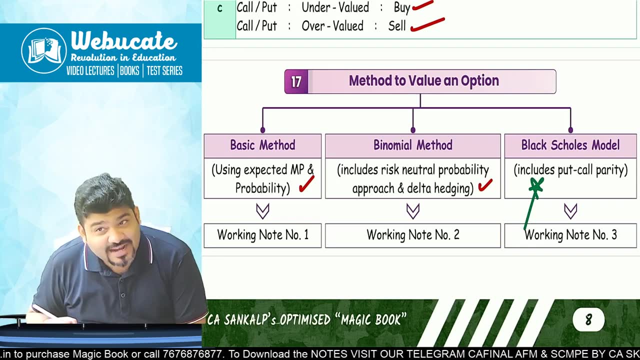 Method To value an option. method to value an option. There are three methods which are there. One is the basic method. Questions are asked in the exam for this from this binomial method Exam. questions are asked from this, But the last is the black and schools, on which questions have not been asked. 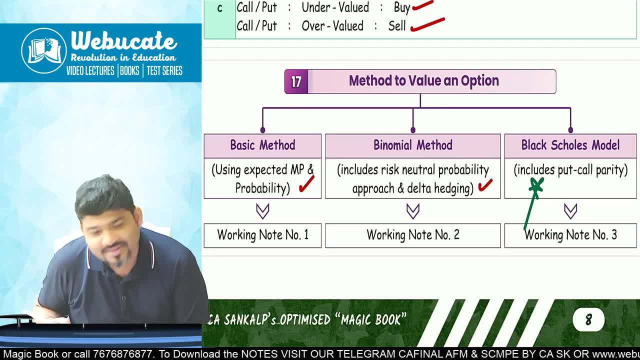 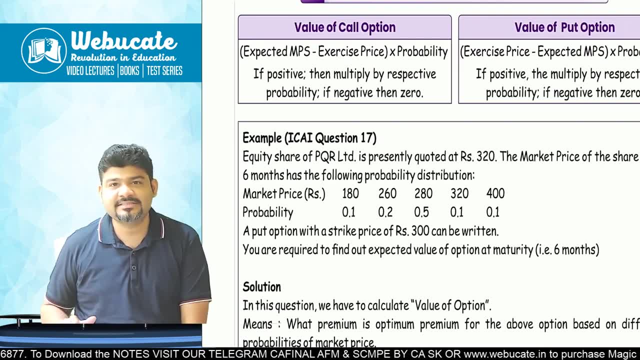 But still, I'm putting a star because you never know. Let's see what happens. So now, first we will start with a basic method. This is very, very easy. This is very, very easy. So your, they will be giving you a probability. 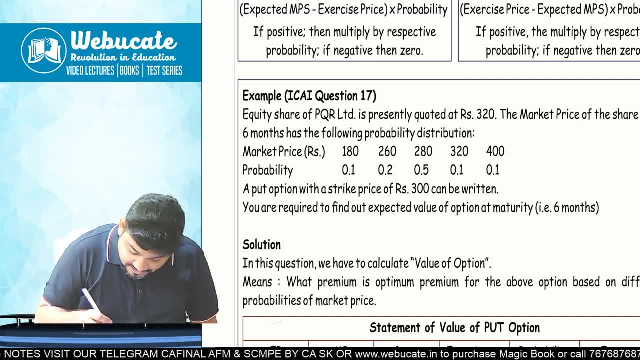 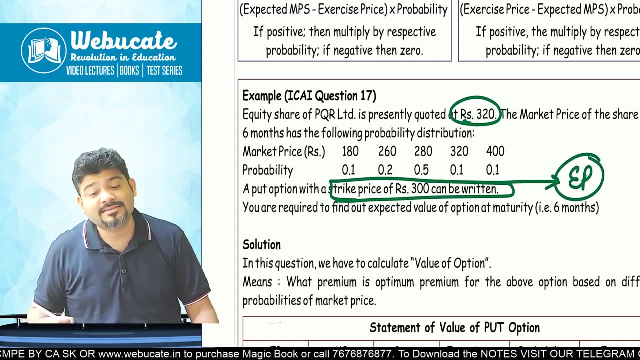 Of the change in share prices. So suppose if currently the share is posted at 320.. OK, suppose this is your put option with a strike price of rupees 300 can be written. So this is your exercise price. What is the exercise price? 300. 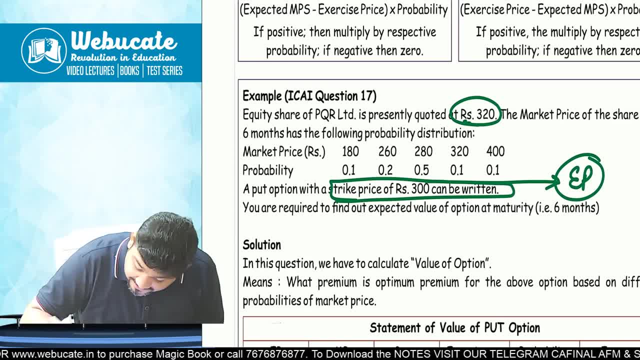 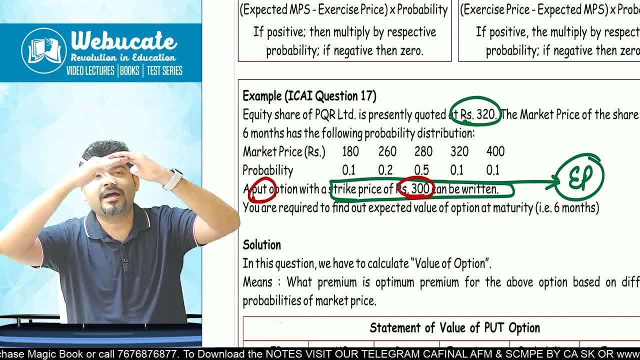 OK, now what will happen when you have taken a put option? Hello, You have taken a put option with the exercise price of 300.. So you want the market to go down And look at the probability of market going down, first case, 180.. 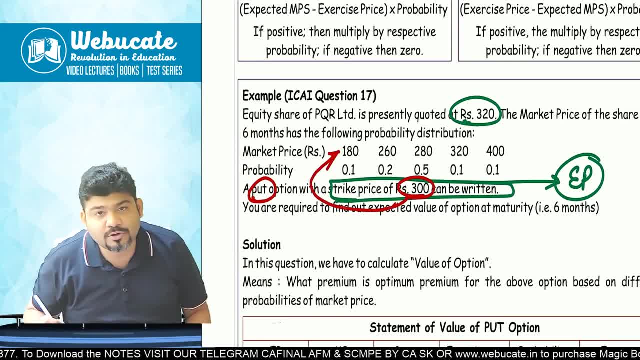 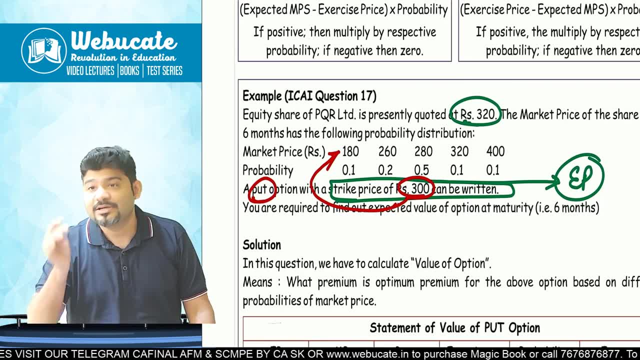 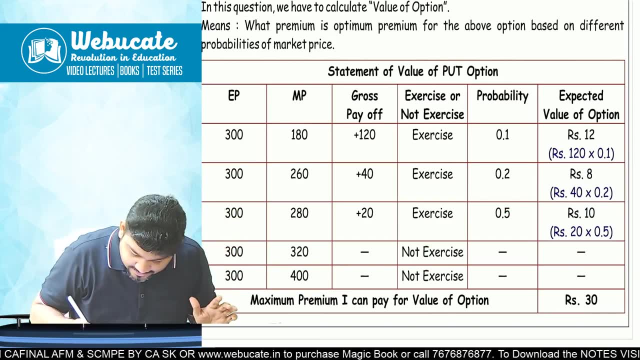 So can I say the market can go down by 120 rupees. But what is the probability? 1%, So 120, into 10%, So 12 rupees should be the premium. Likewise, we will add all the possibilities that are there and then calculate our premium. CL teacher. 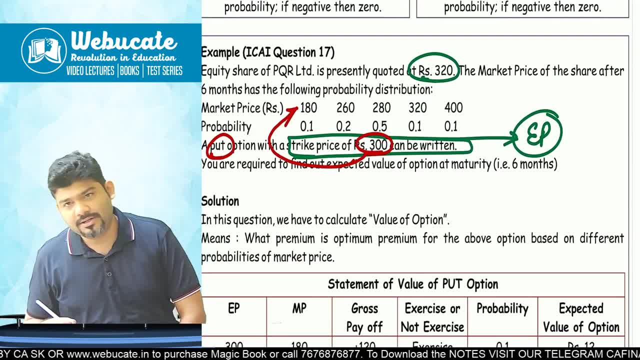 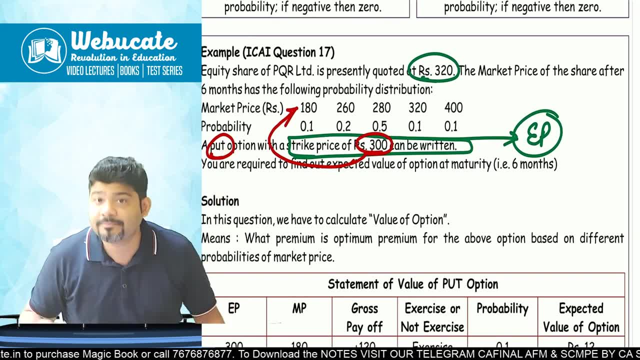 Suppose the price goes from 300. It go The exercise price of 300. But the market goes down to 180. Can I say 120 rupees is a profit But the chances of that 120 happening is 10%. So eventually 12.. 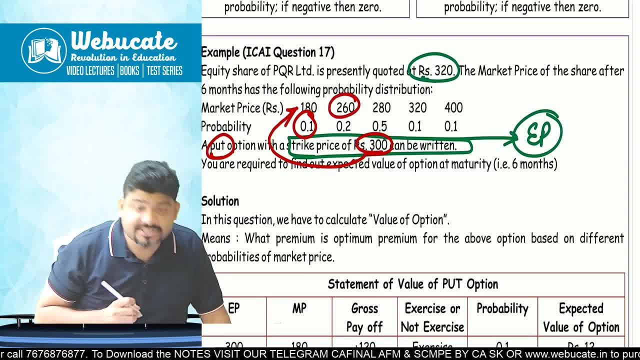 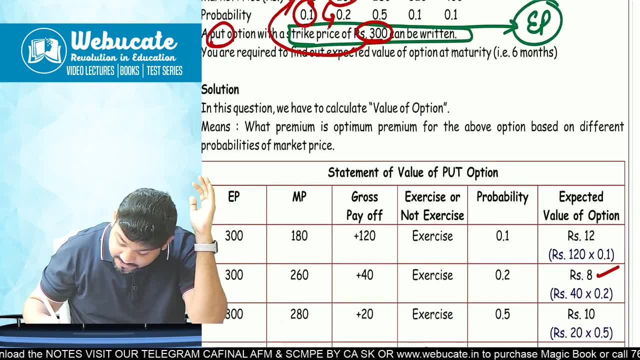 Then suppose if it goes down to 260.. Again we have a chance of making 40 rupees profit, But that possibility is also 20%. So 40 into 20%, So we will get it in the same way. Then we have the 280 and 0.5. 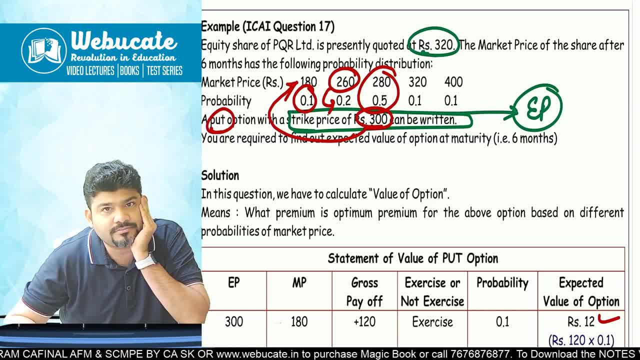 So now suppose if the market Goes down from 300 to 280.. Oh, 20 rupees down again. It is in the money because, put option, We want the market to go down, But the chances of that 20 rupees profit is 50%. 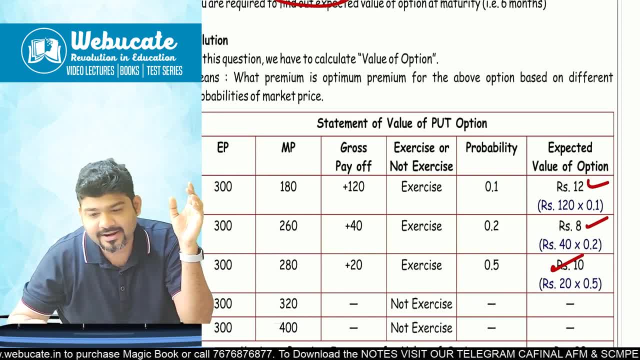 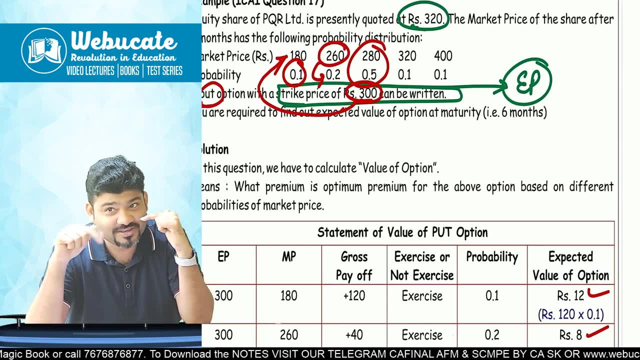 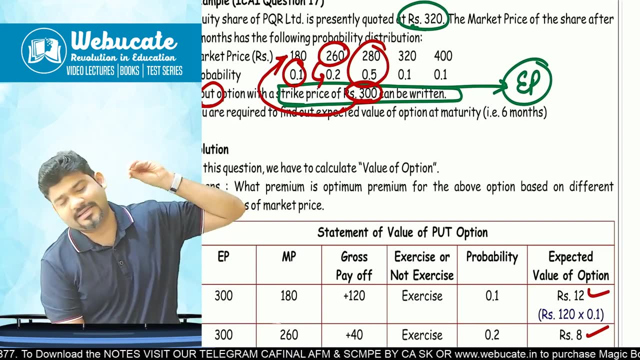 So it will become 10.. Suppose if the market goes from 300 to 320. Oh, from 300 to 320, then it is out of the money. We will not exercise the option. when we are not exercising the option, There is no point. 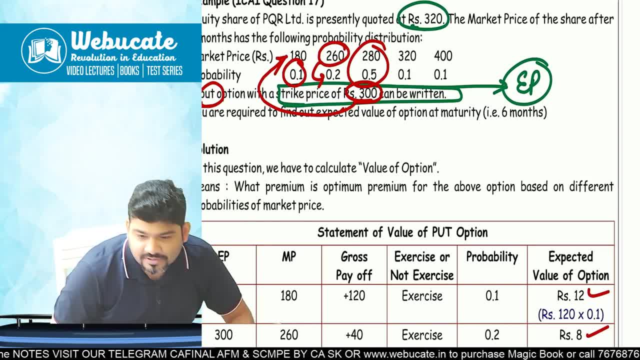 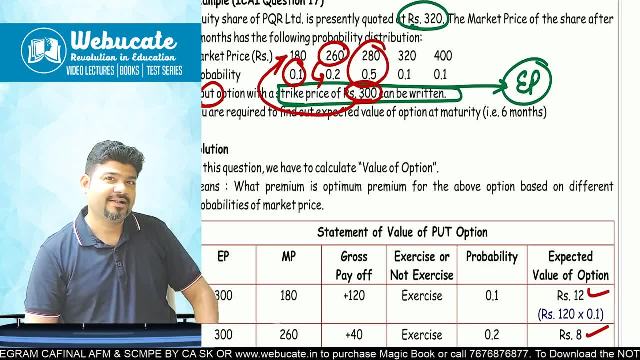 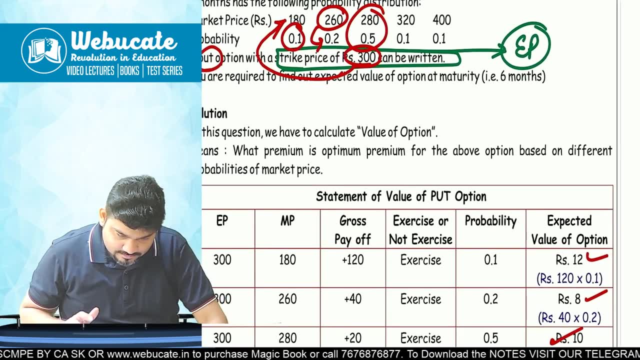 Of probability at all, Then again from 300,. if it goes to 400 again, we will not exercise the option. No point of probability at all. So that's how the whole system works. That's how the whole system works. 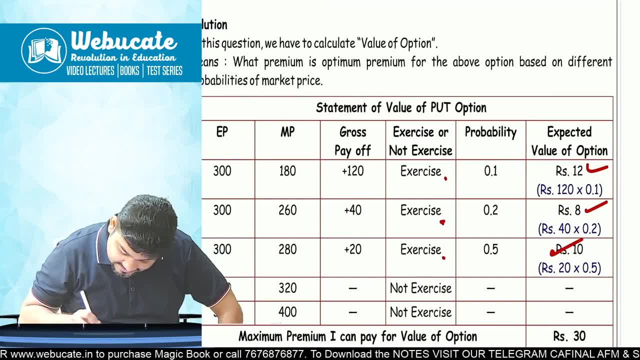 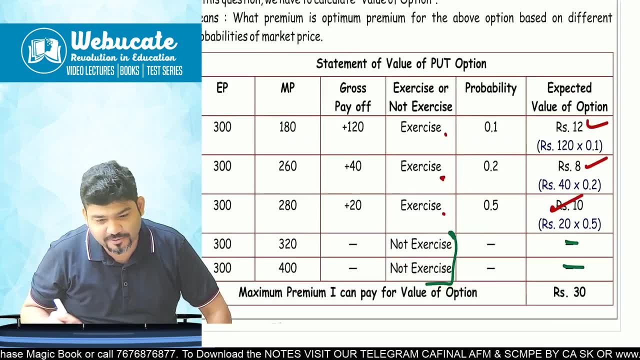 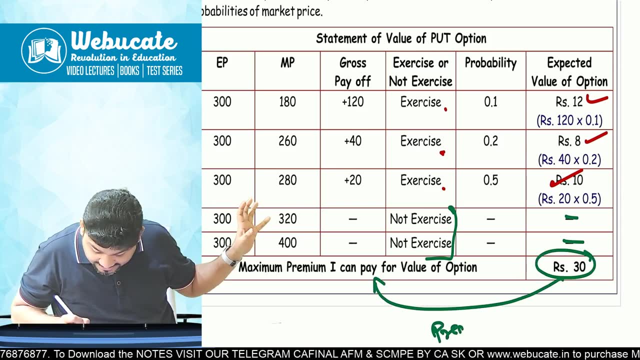 Got it guys. So exercise, exercise, exercise. Two cases: we will not exercise if you don't exercise. No expected value of option. Finally, this is the value of option that I get And this is the premium that I should be ready to pay currently for this share. 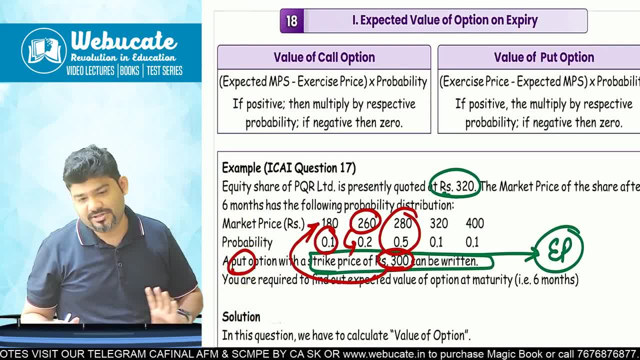 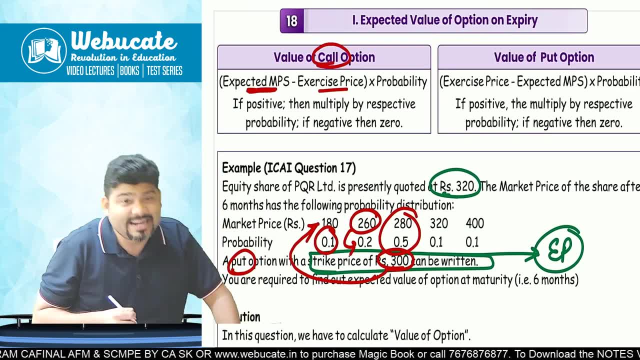 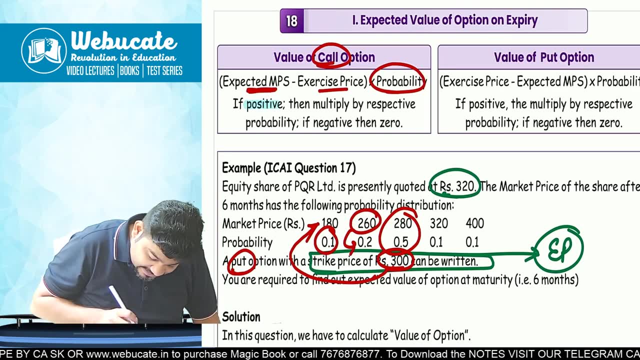 This is the premium that I should be ready to pay for this share. So in case of value of option, pay attention to call option If expected market price is greater than expected market price minus, exercise price into probability. if this is positive, then multiply by. 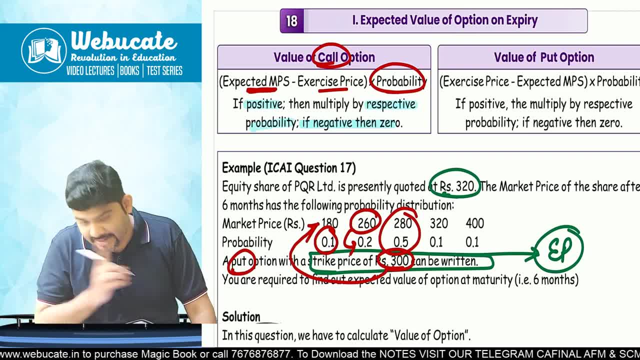 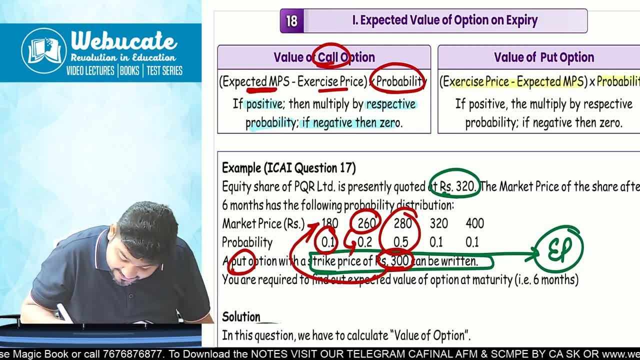 respective probability, if negative, then zero. And in case of put option market price, exercise price minus expected market price into probability. if positive, multiply by respective probability, if negative, then zero. I think we should write here: Yeah, correct. 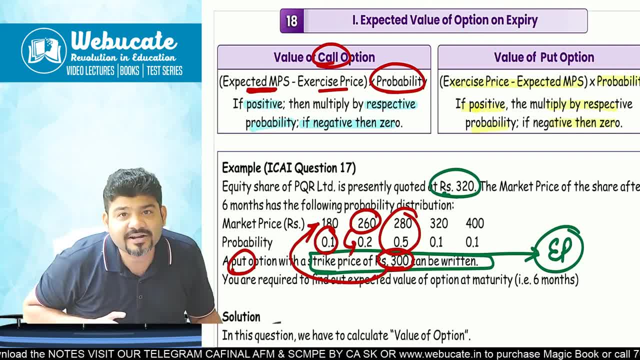 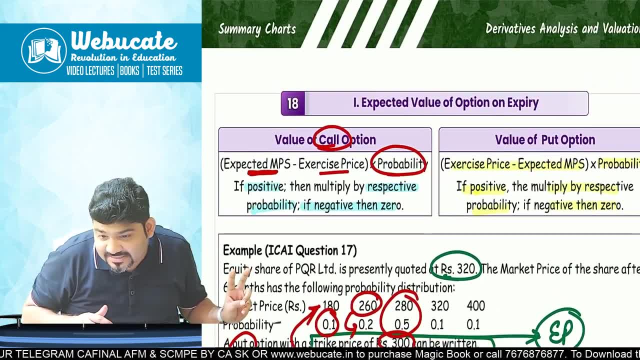 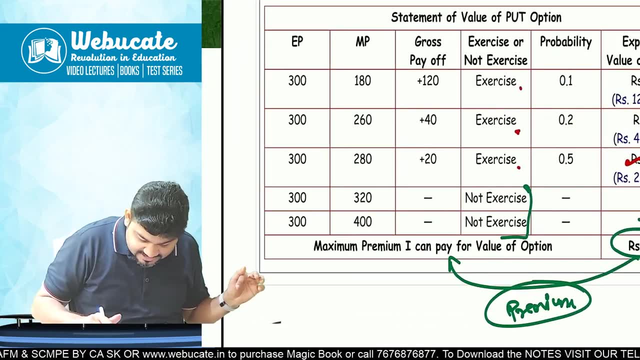 Exercise price minus expected market price: Perfect, Perfect. So if your exercise price is higher, 300, minus expected market price, 180.. We will exercise Yes Into probability. So if positive, then multiply by respective probability. Yes, If negative, which is the last two cases. 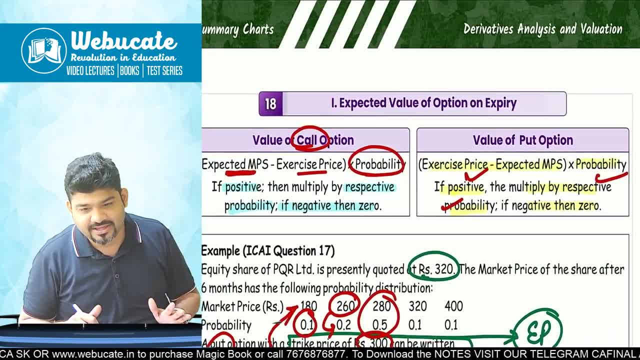 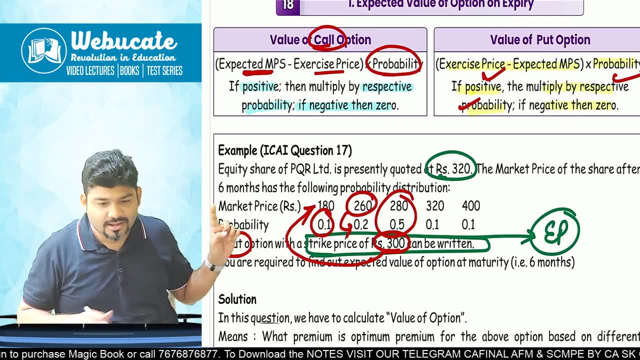 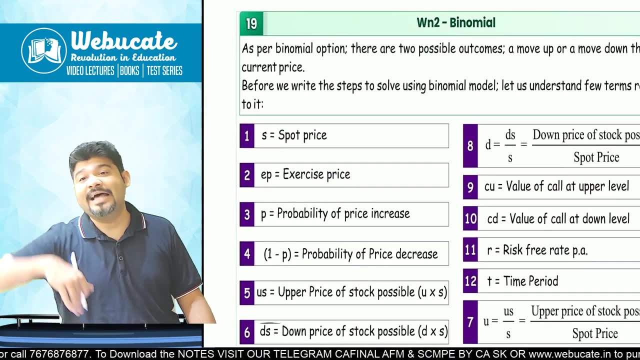 you will not exercise that, everybody here. So this is called as the expected value of option on expiry, one of the methods to do it. OK, now we move on to the second method, And the second method is called as the binomial method. 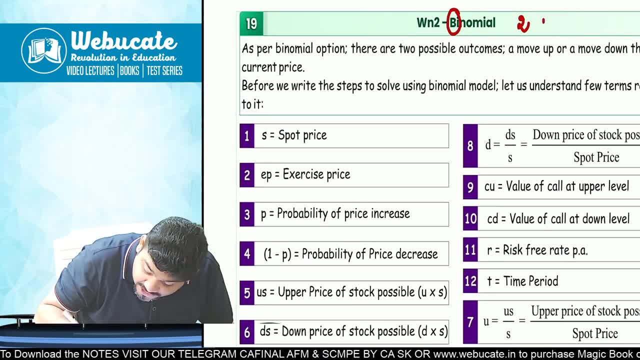 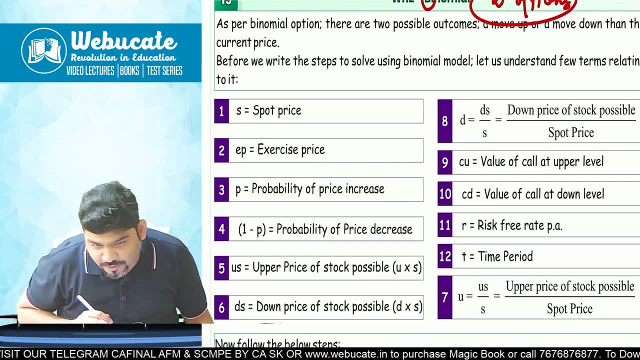 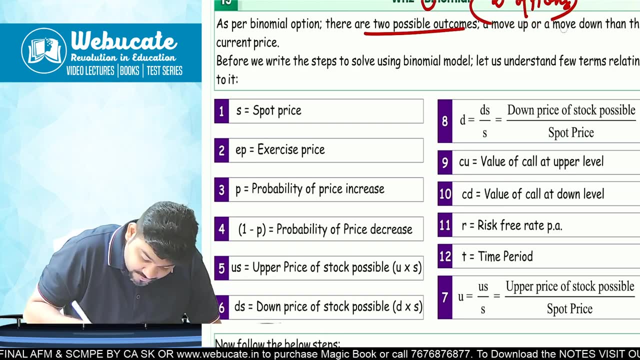 As the name suggests, binomial means two options will always be there. Two options will always be there. So, as per binomial option, there are two possible outcomes by two possible outcomes: a move up or a move down. a move up or a move down. 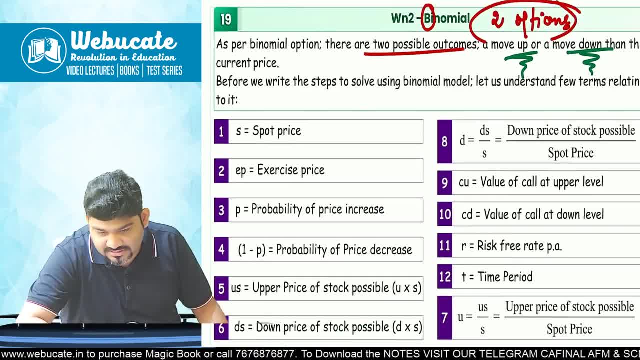 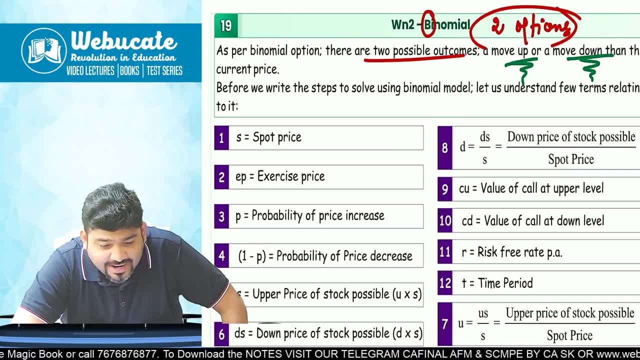 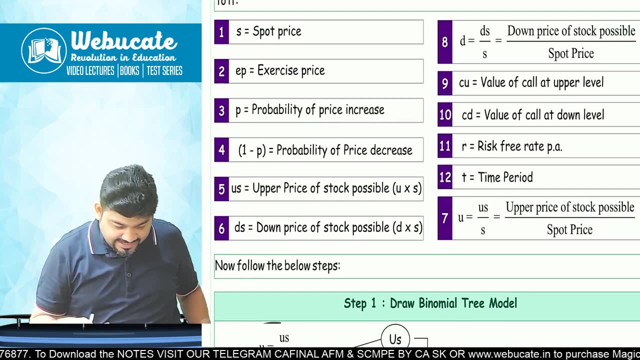 Then the current price. OK, so this is your, this is your binomial option. Now, before I teach you all the whole concept of binomial, I will want to you to understand few of the points or few of the terminology, So to say, of binomial model. let's start. 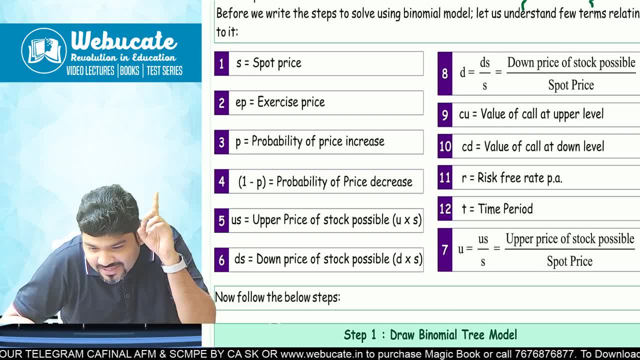 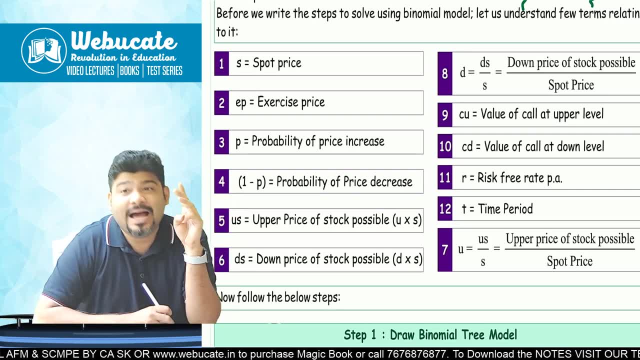 S will be called as the spot price, EP is called as the exercise price. P is the probability of price increase, Again binomial. So there will be two prices: One When we expect the price to increase. when there is a word of expectation. 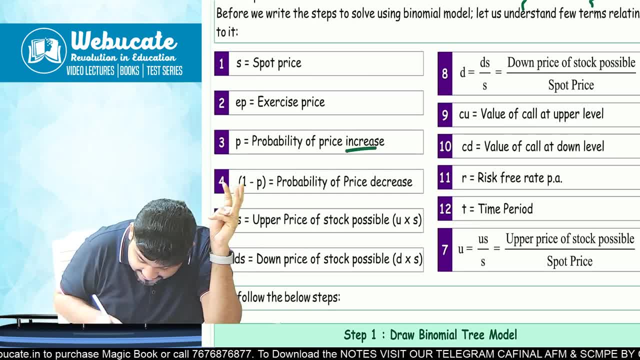 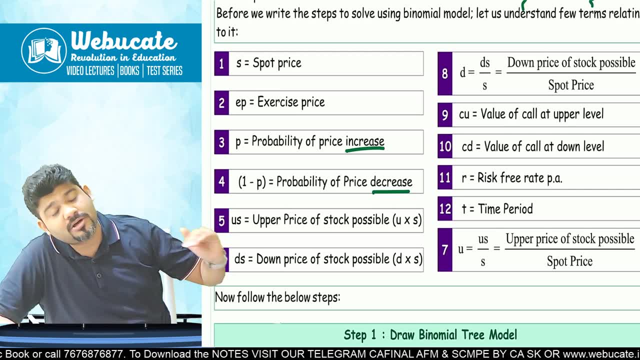 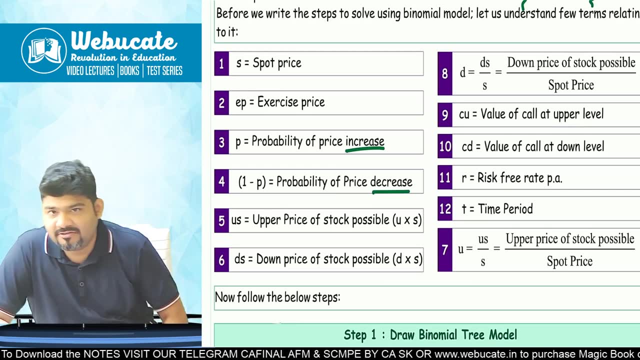 probability will always be there. so probability of price increase And obviously the other one minus P will be the probability of price decrease. How much the price can go up? Suppose the exercise price is 50. We expect that the price may go up till 60 rupees in one month's time. 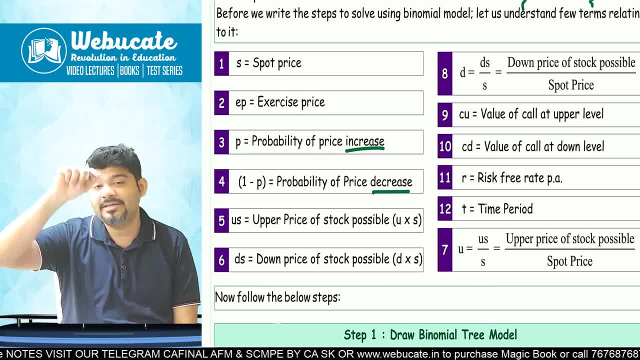 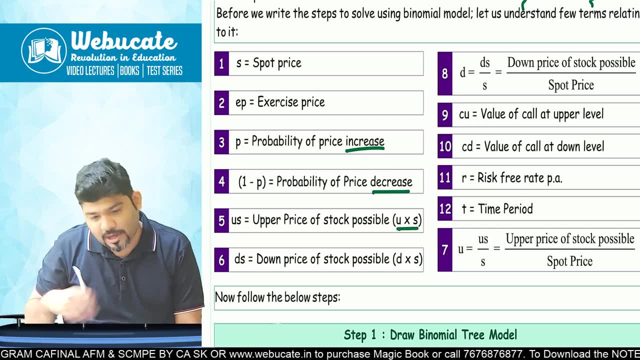 So what is that? Probability of price going up is the P? How much is called as US Proper price of stock possible and down price of stock possible? So we expect that it can go till 40 as well. So that will be called as BS. 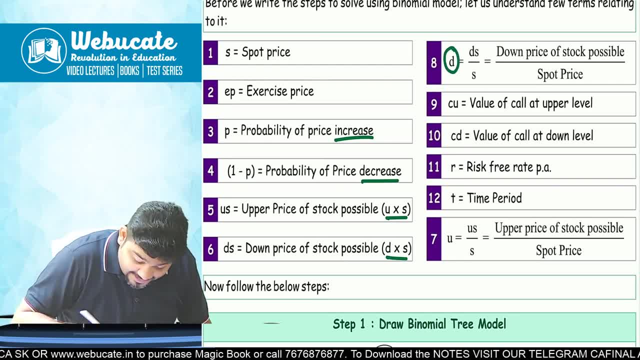 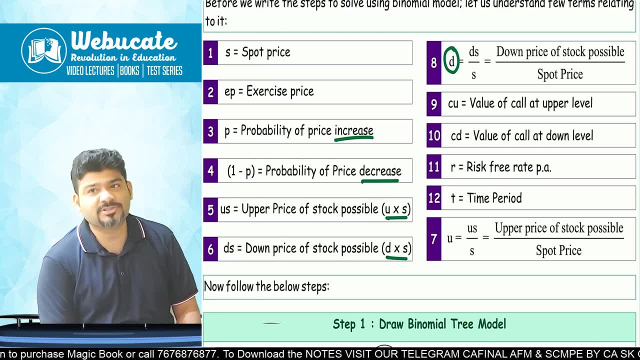 Right, OK, Now then is: then there is something called as D. What is D? D is the times that the price goes up. Suppose we are we having an exercise price of 50. We are expecting a US, which is the higher market price, upper market price. 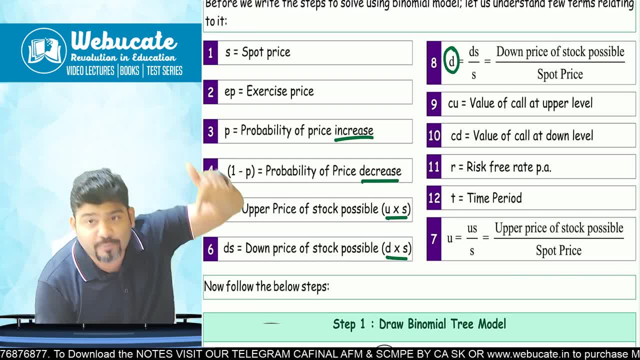 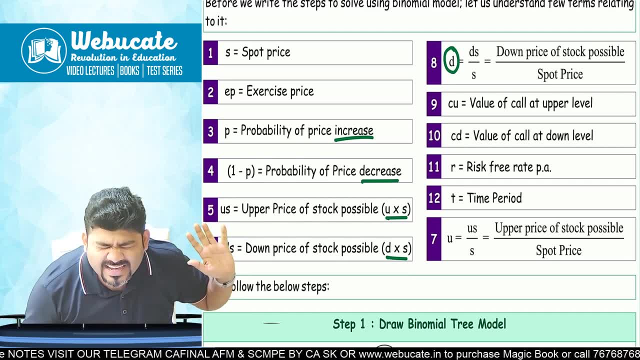 It can go till 60 there. in that case Can I say 1.2? Times chances are that the market will increase. or suppose if we expected the market will go down to say 40 rupees from 50 to 40.. 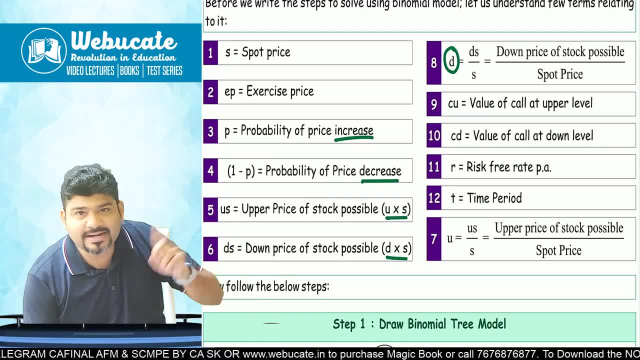 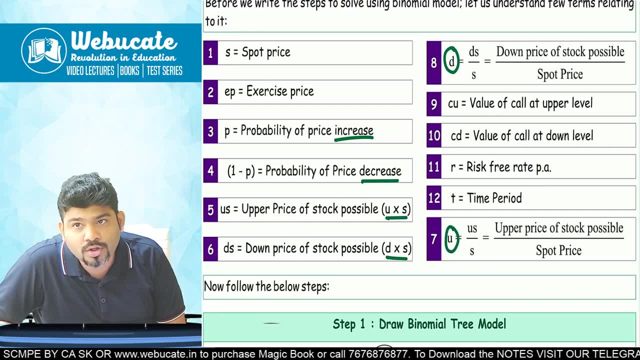 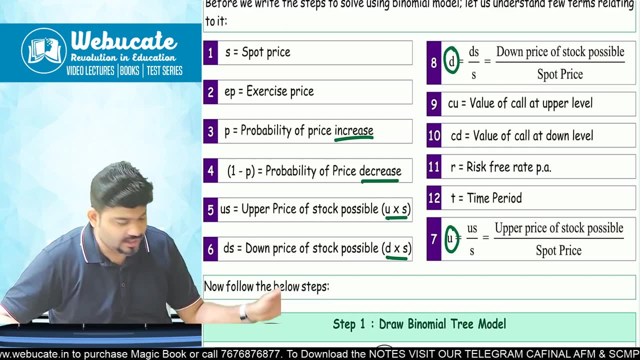 So can I say that D will be point eight, point eight times. the market will decrease. So that basically is called as the D and that basically is called as the U Right. What is the U times? that the price will increase and you is called as the. 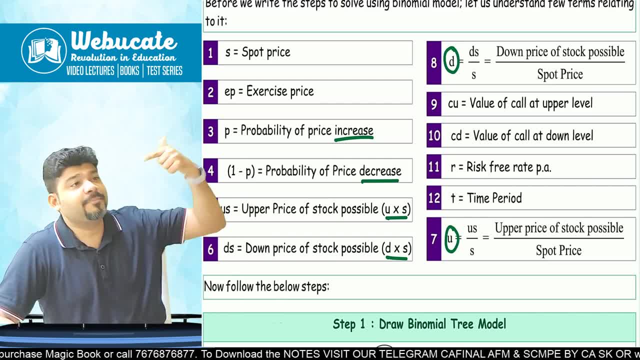 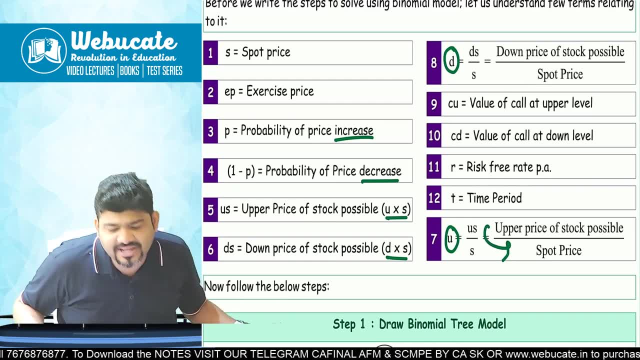 U is called as the upper price of stock possible divided by the stock price. So say, if I am expecting it to go to 60, spot price is 50. So I am expecting this to be one point two times of my exercise price spot price. 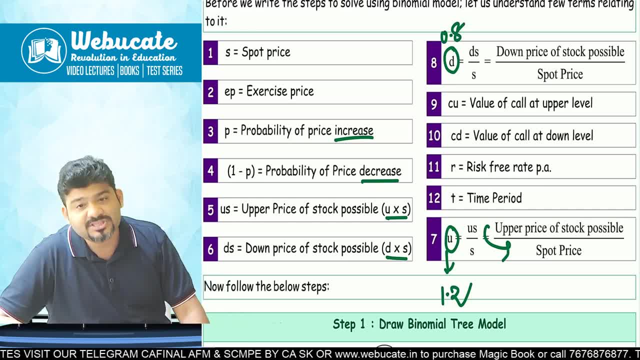 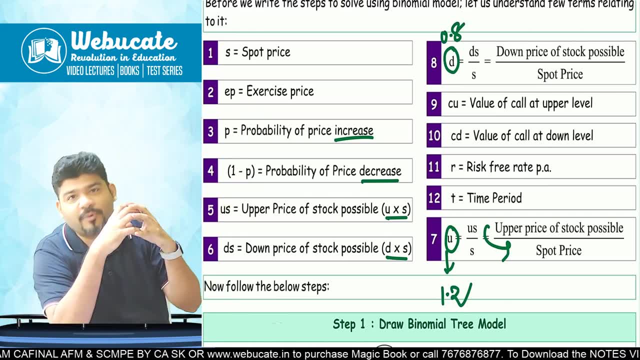 And this will be point eight times of my spot price. So that is your BS upon S. is your D as in? how did you get this 0.8?? Tell me BS 40. You are expecting the market to fall till 40 upon the spot price. 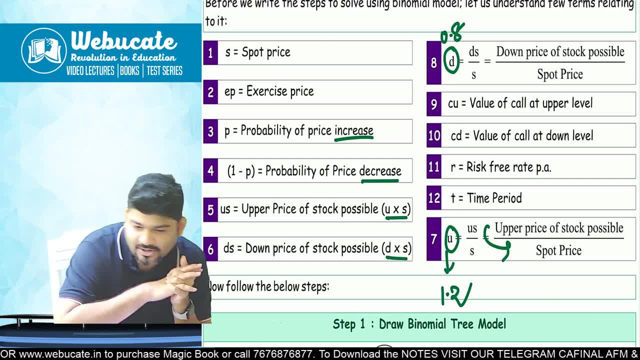 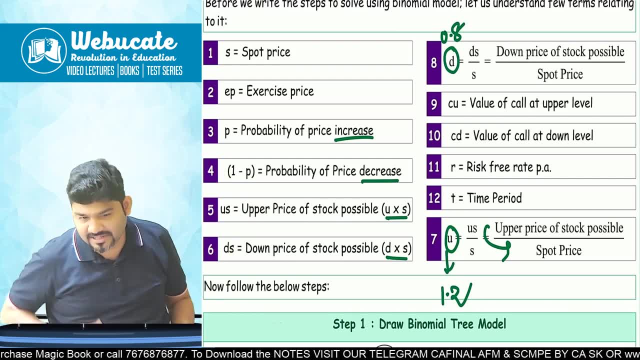 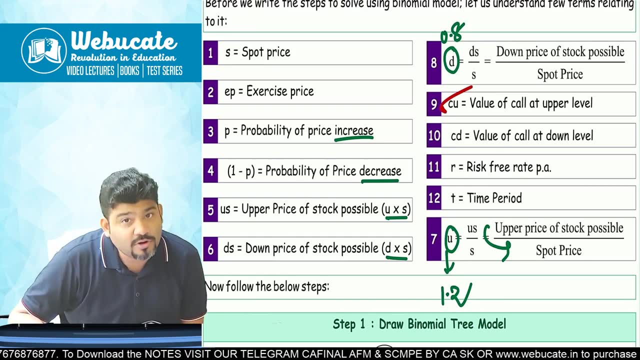 50 BS, DS upon S or US upon S. What is US DS? maximum price possible. lowest price, minimum price possible. Probability: we are class for exercise price. We are clear. And then, if the market goes up, what are the value of call? 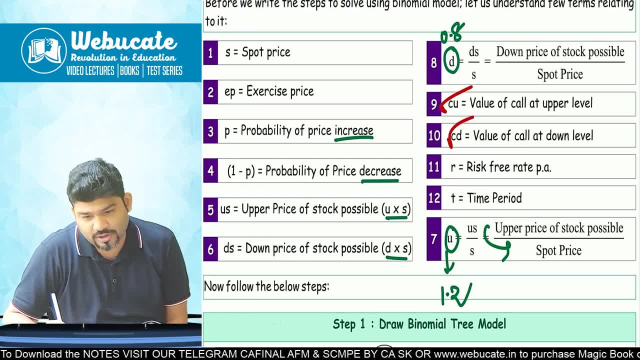 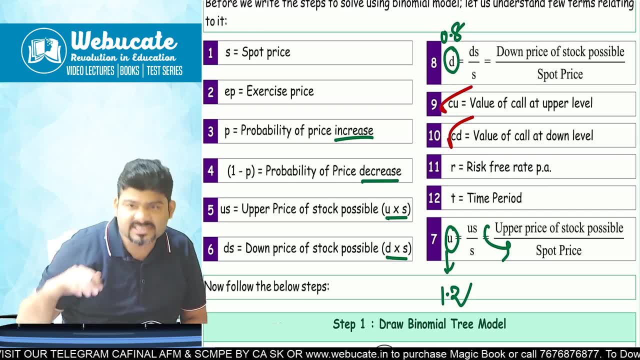 So we have a specific formula for that. If the market goes down, what will be the value of call? Now, all of this is going to happen three months later, Four months later, six months, as the expiry is there. So we will have to get it at the current present value. 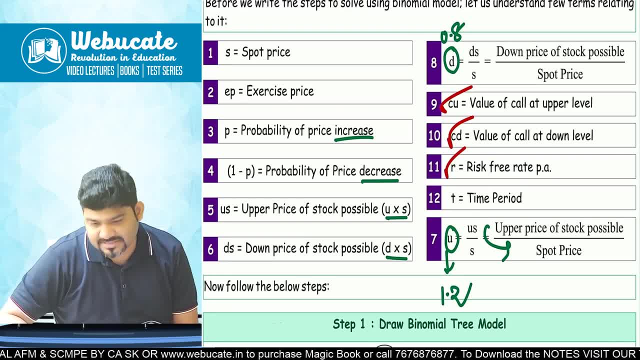 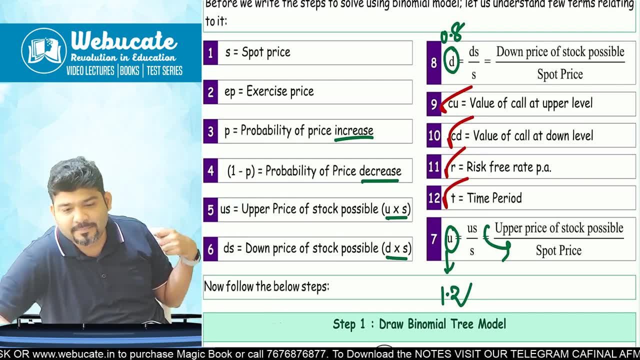 So we will use the risk free rate to bring it at the present value. How much is the? T is the time period, And that is how we will bring all of this at the present value. This overall will give us the binomial model. 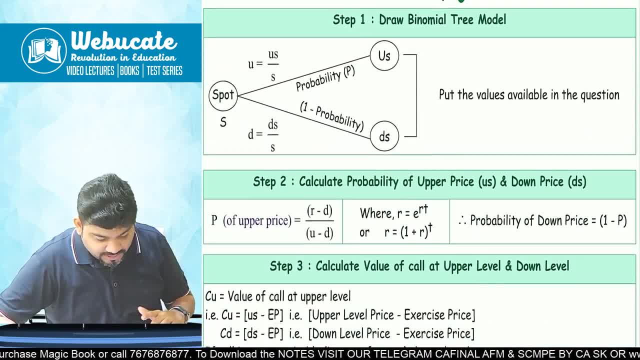 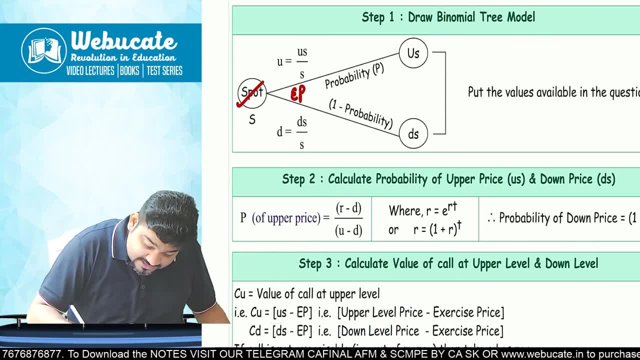 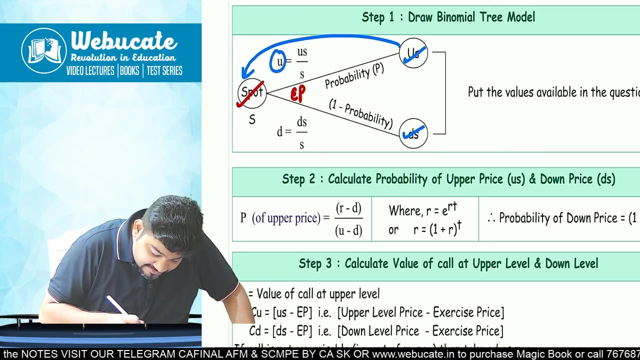 This overall will give us the binomial model. So first in the situation we have to spot the spot price. We also write down the exercise price here. Then we write the US, Then we write the DS by default. Now we have the US, We have the spot, as we will get the U. 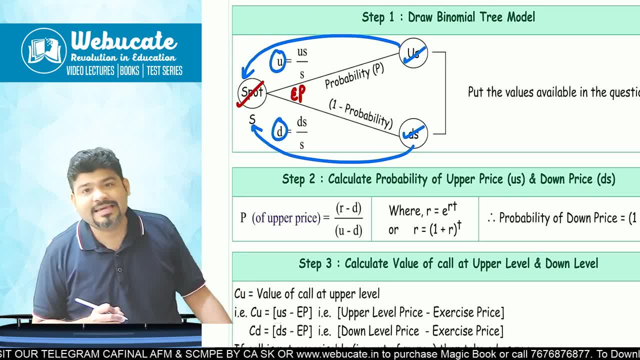 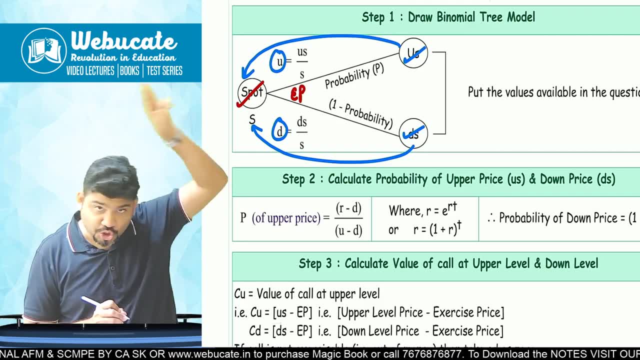 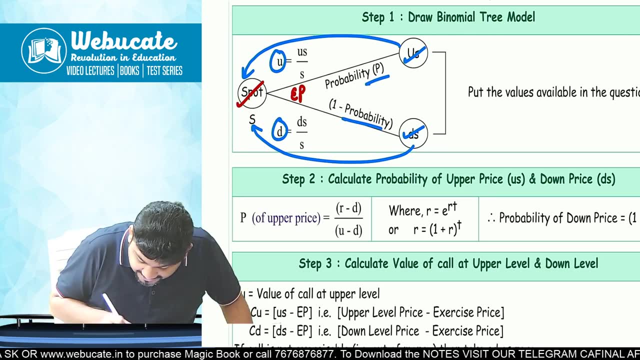 We have the DS, We have the S, We will get the D. So spot exercise price: US DS, US by S, DS by S D. That's how P probability also, if it is given P and one minus probability. 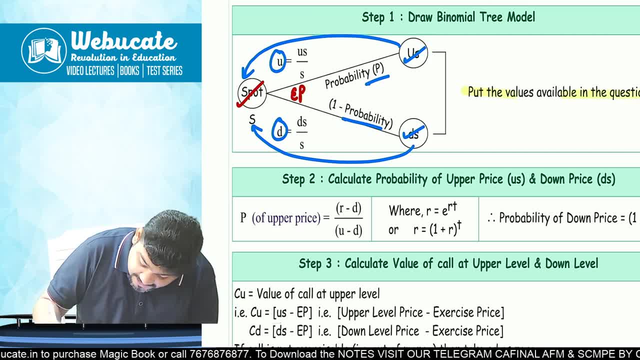 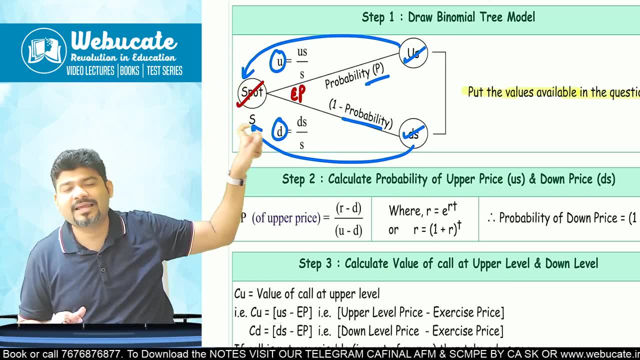 So all of this information, we have to put the values available in the question. Overall, we need all of these four values. Whatever is given in the question, pick it up from there and put it here. Whatever is not available, I will teach you with the formula, which is the next step. 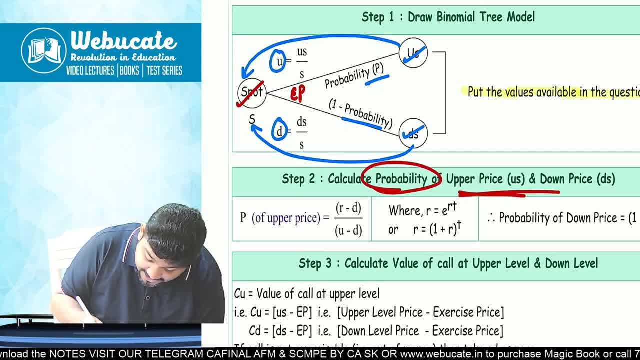 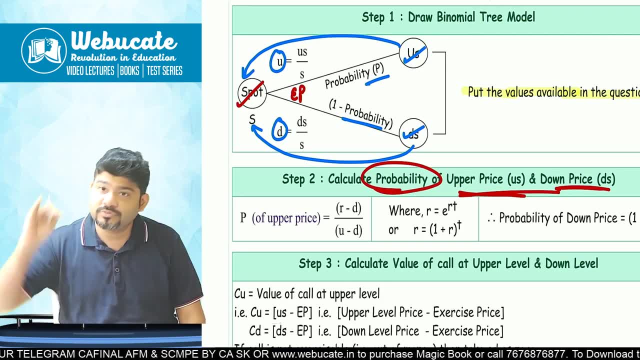 So second step is calculation of probability of upper price- US- and probability of down price. For that we have a formula. Obviously we don't have time to get into the derivation in regular math. Probably I also get into the derivation. 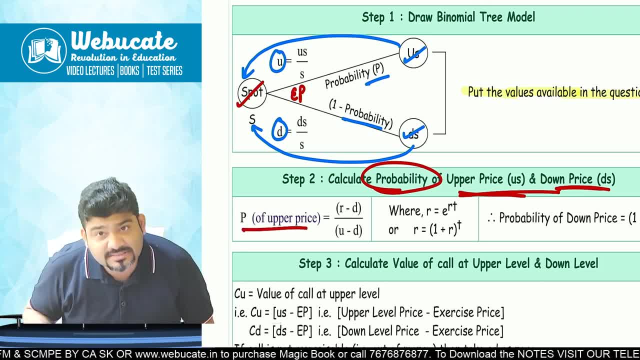 But now we will directly use the formula, which is R minus D, upon U minus D. We know what is D, We know what is U, What is R? R is the rate of interest, So R can be e raised to RT. 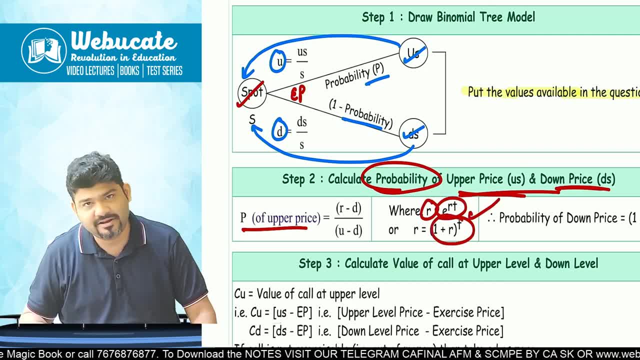 One plus R raised to T as the information that will be given. If it is continuous compounding, it will be e raised to RT. It will be. if it is a compounding, it will be one plus R raised to T, But this will give us the probability of upper price. 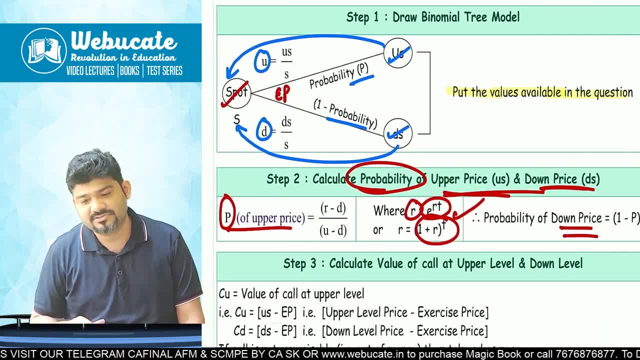 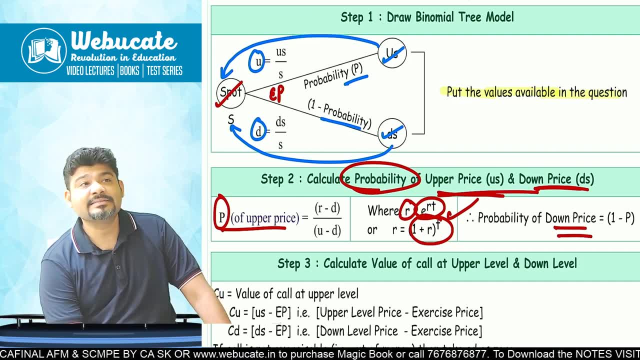 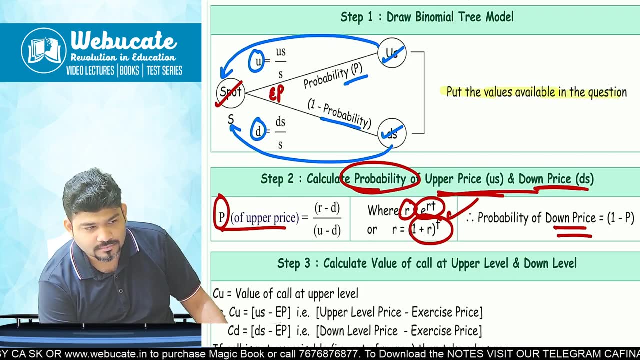 And then there is also probability of down price, which is one minus P, which is one minus P. Now, what is the probability of upper price? It is R minus D upon U minus D. It is R minus D upon. It is R minus D upon U minus D. What is R? 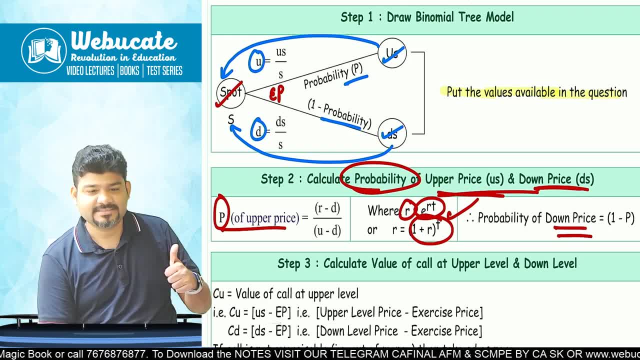 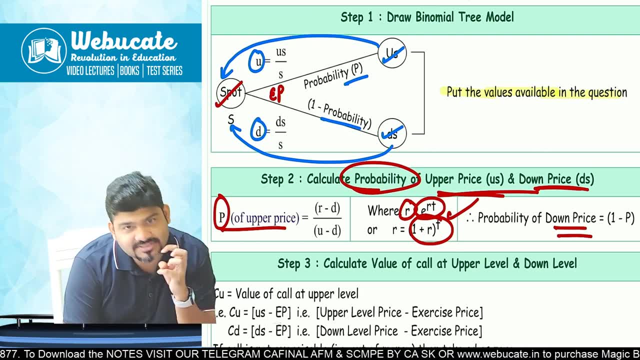 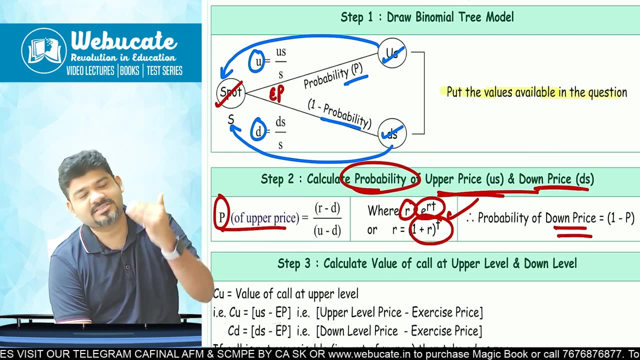 The rate of interest. That's right. Minus D D. Yes, Down Down. What is the chance? I mean, what is the you can say the times the price will come down. What is the chance that it will go up? is your U? 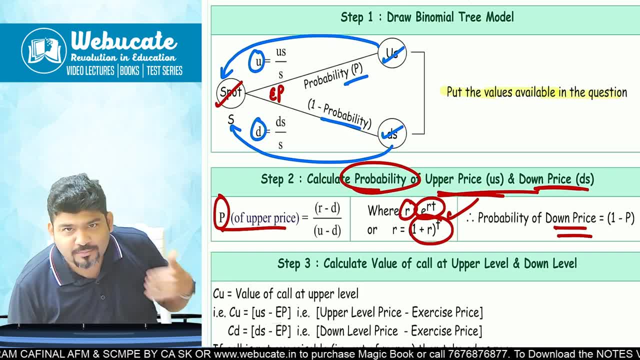 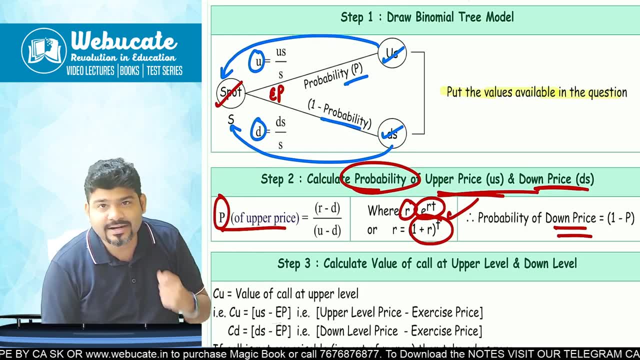 Not exactly the word chance, but times: How many times from the spot price, How many times the market will go up, How many times the market will go down. That is your U and D R. basically is your R is equal to E raised to RT. 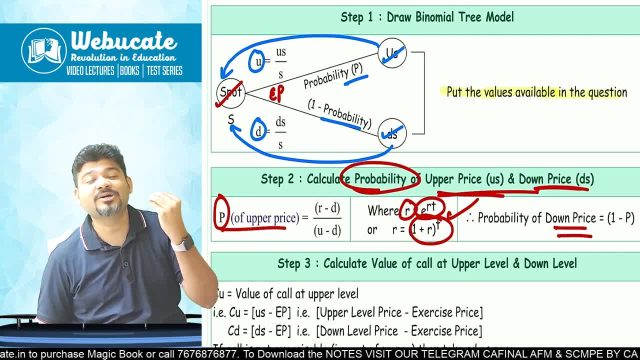 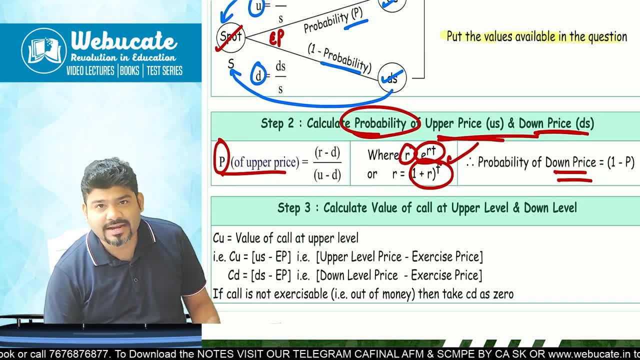 R is equal to one plus R raised to T, R basically is your rate of interest. R is equal to rate of interest. Got it Done? Then we have calculate the value of call at upper level and, obviously, value of call at the down level. So let's see this. 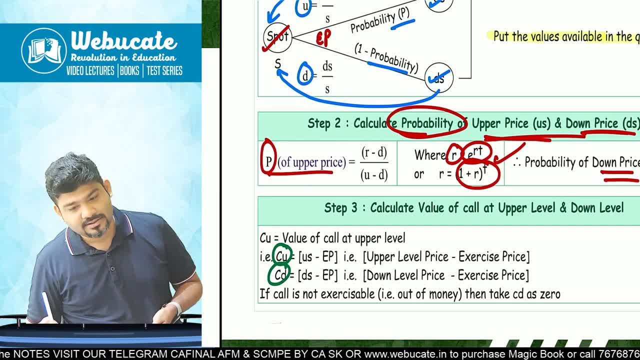 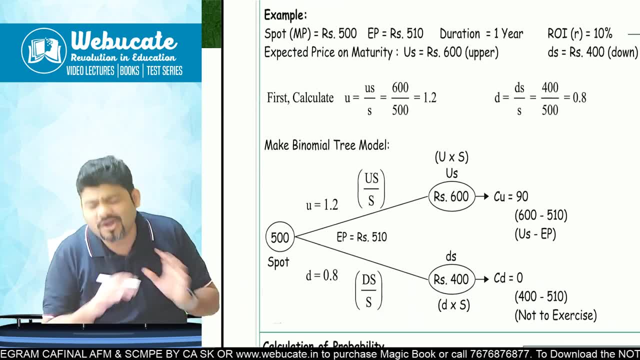 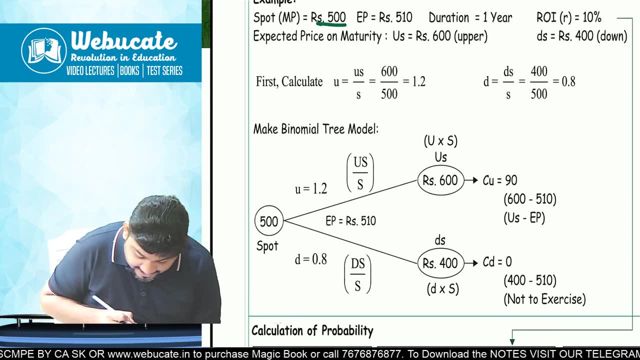 C, U and C D. So how do we do this? Let's solve an example and try and understand all of this At a very, very easy level. Suppose now the question is given: spot price market 500,. exercise price 510,. 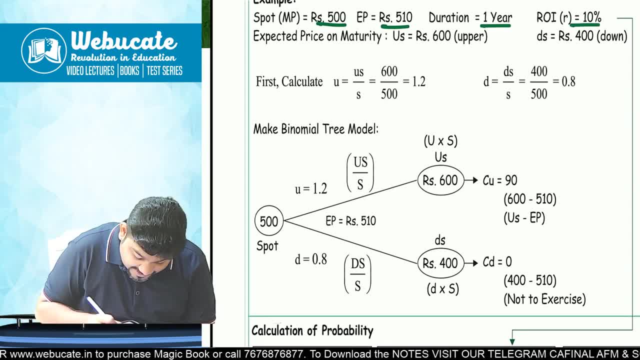 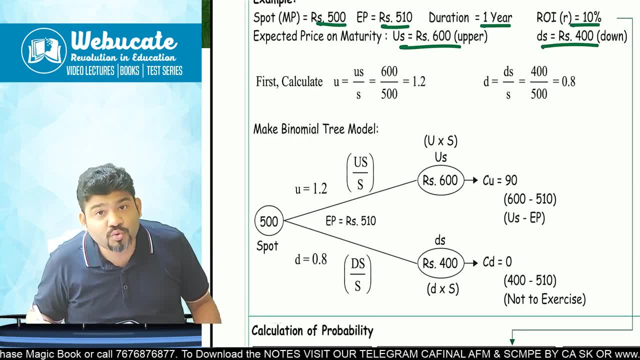 duration: one year. rate of interest: 10%. expected price on maturity: US 600, DS 400.. First thing that we have to do is calculate the U and the D based on the information available. Can I say US is given? Can I say DS is given? 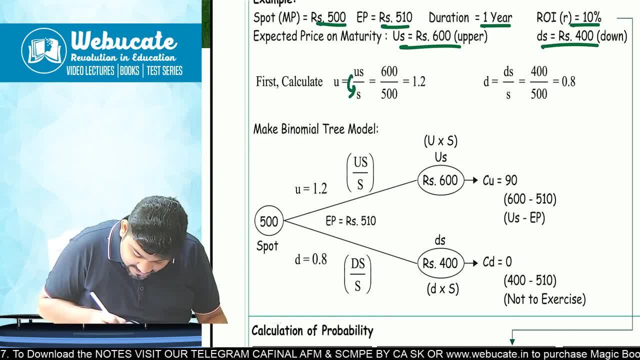 Can I say S is also given. So if US is given US upon S, DS is given DS upon S. So US upon S spot is 500, 600 upon 500, 1.2, 400 upon 500, 0.8.. 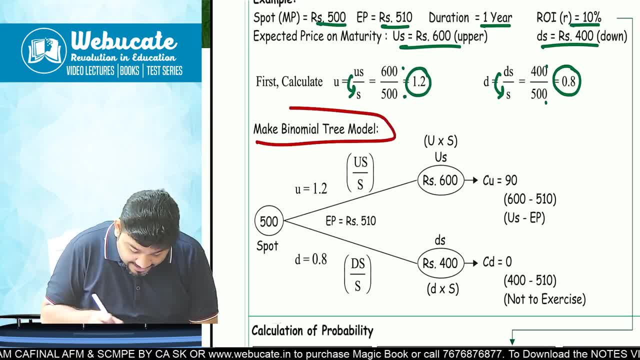 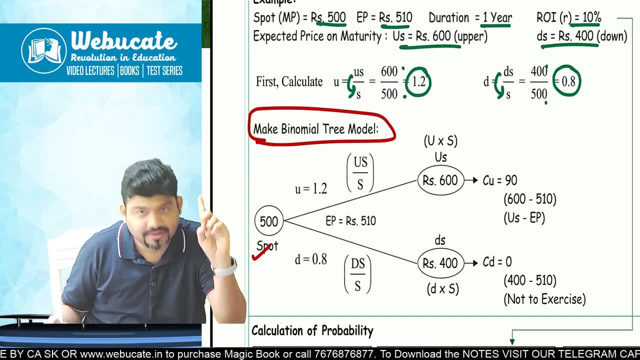 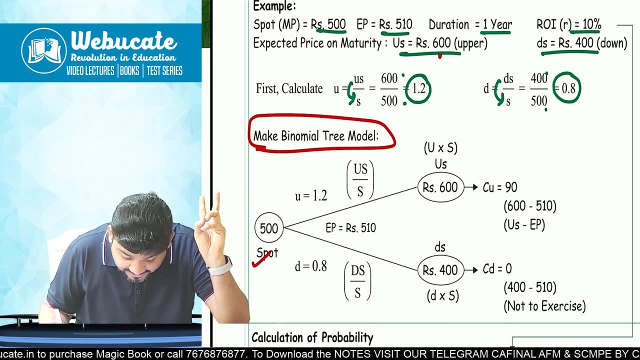 Gotcha everybody. Yes, sir, Make the binomial tree model. How do you make the binomial tree model? Spot written exercise price given in the question. Sorry, exercise price. exercise price is given in the question. Yes, EP 510, 510.. 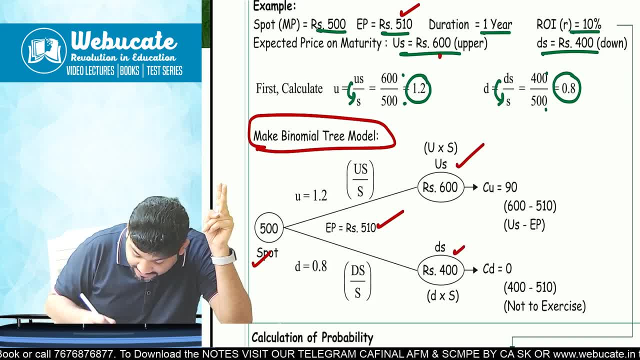 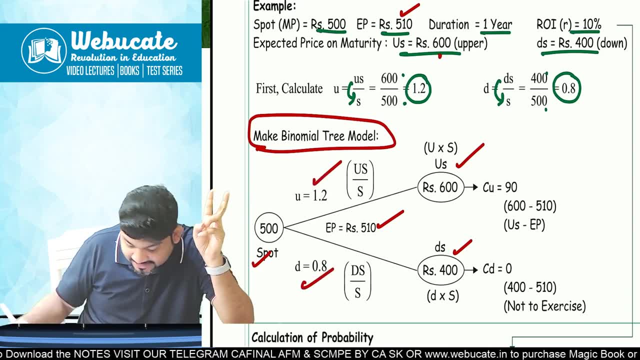 First write down the US, Then the DS US, sir written, DS, sir written, given in the question. If you have US, if you have S, you will be able to calculate the U. You will be able to calculate the D. 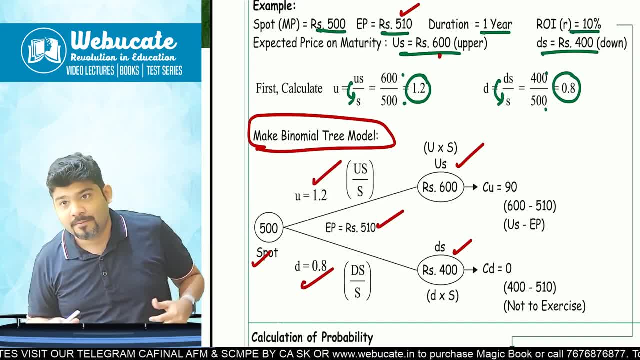 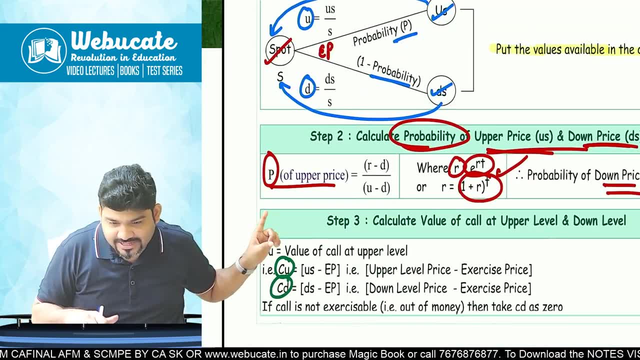 Clear till here. Now missing is P and 1 minus P, Probability and 1 minus probability. How do you calculate that R minus D upon U minus D? We have already taken the formula here: Calculation of probability: R minus D, U minus D. 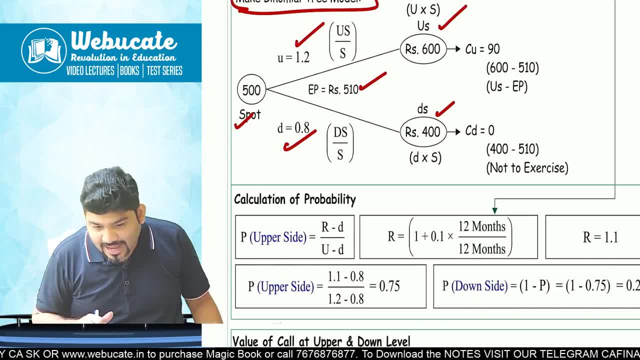 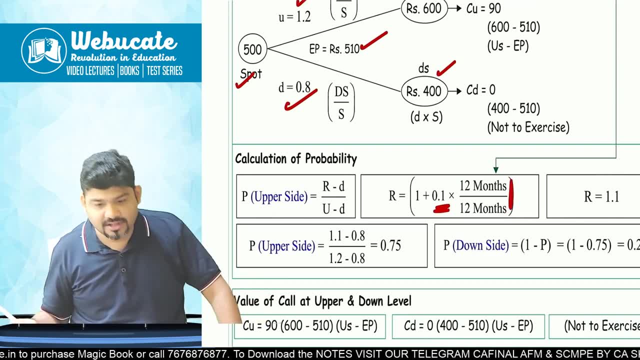 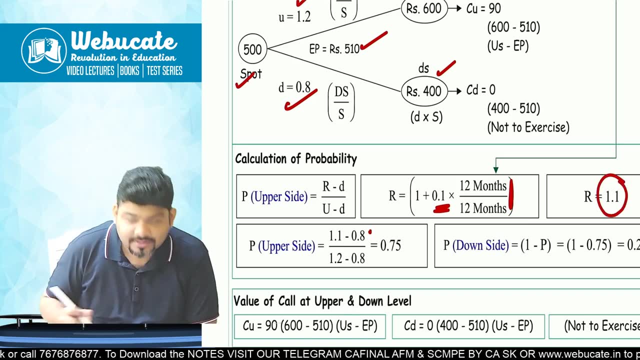 Okay, sir, No worries at all. So R is 10 percent. It is given in the question 10 percent So R into obviously the duration, which is 12 months. So R is 1.1.. So 1.1 minus 0.8, which is D upon 1.2 minus 0.8.. 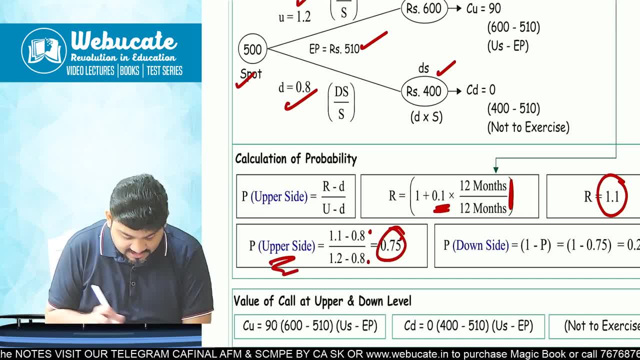 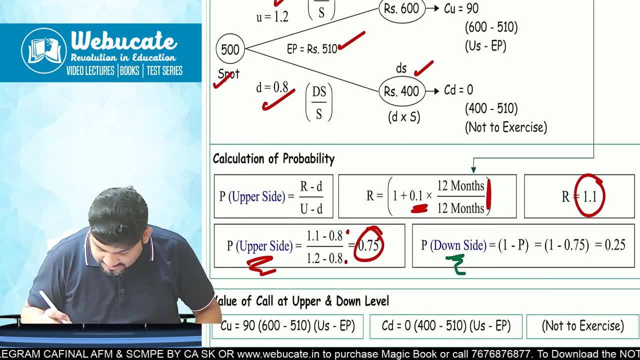 So this will become 0.75, which is the probability of upper side. And then we have the probability of downside, which will be 1 minus P. So 0.25 will remain. So 1, so 0.75,: 0.75 for upper side probability and 0.25 for the remaining one. 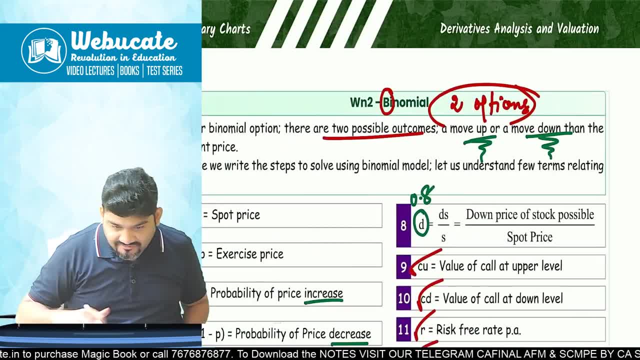 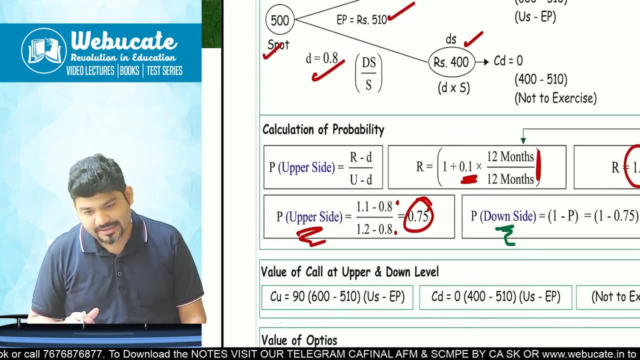 Got it everybody? Yes, sir. Now the value of call at upper level and down level, something that we were discussing here. Now tell me, in case of upper level, can I say I will exercise? The answer is 110 percent, sir. I will exercise. 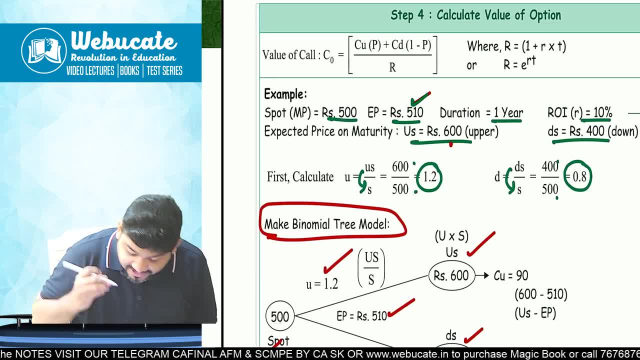 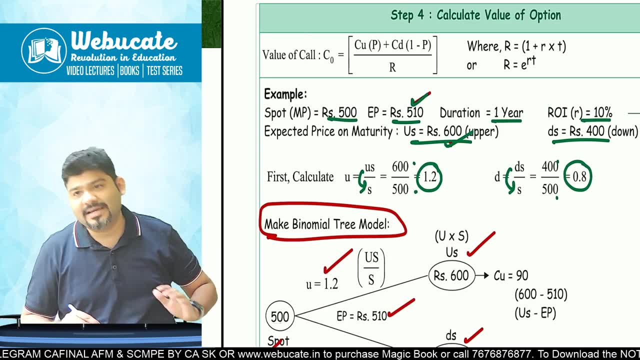 Because because my exercise price is 500, but my upper has gone to 600. And that's what I want because it's a call option. So right to exercise, call option when the market goes up. So 90 rupees Yes. 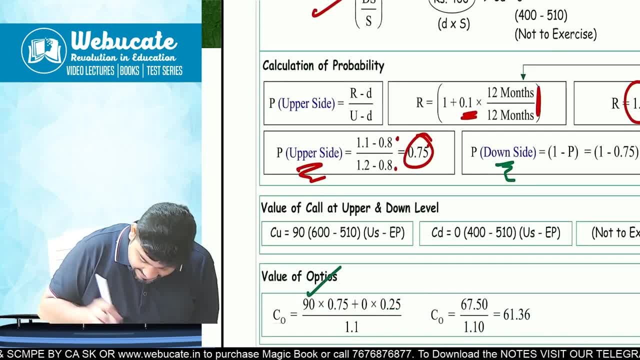 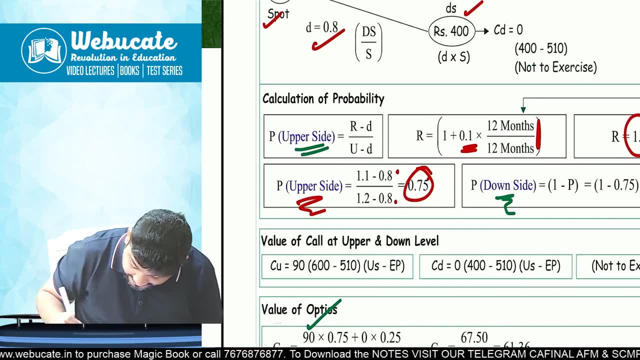 90 rupees is the profit that I'm making Exactly 90 rupees is the profit I'm making at 90 rupees profit. Can I say: at upper side profit Probability is 0.75. at downside Probability is 0.25. 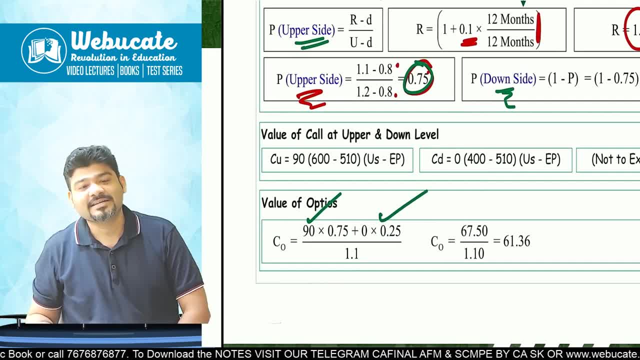 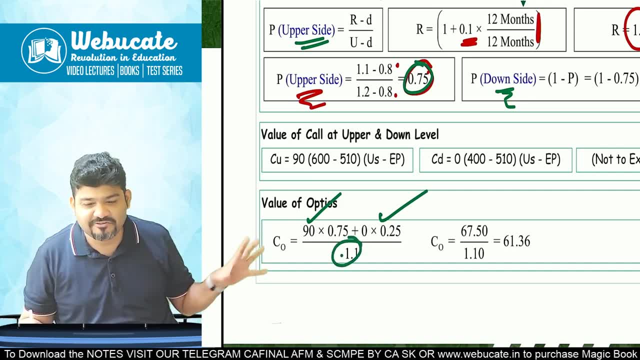 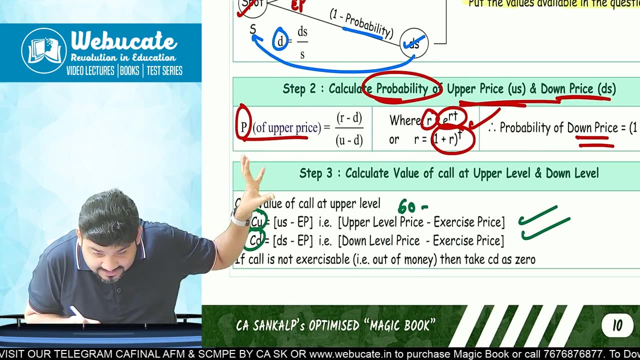 Gotcha. So plus 0 into 0.25 upon 1.1 to bring it at the present value. This is the value of call See here. this is what they were trying to explain here: Upper level price 60 minus lower level price 50.. 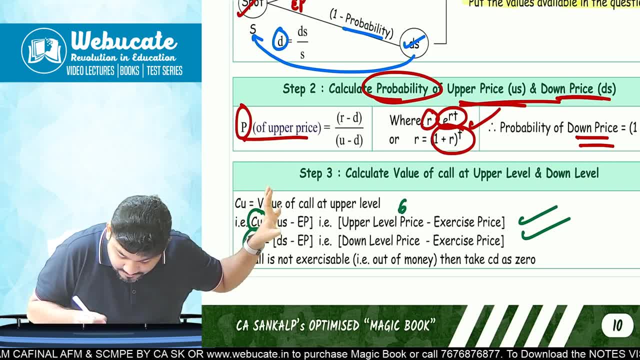 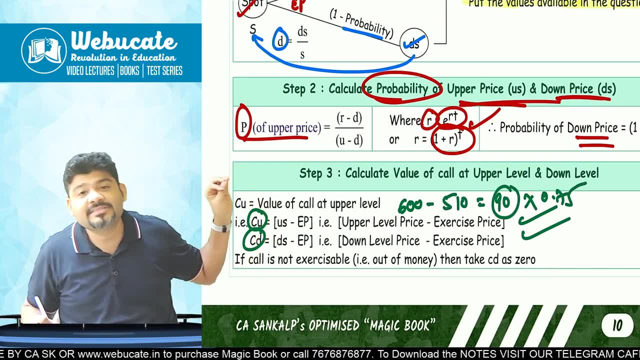 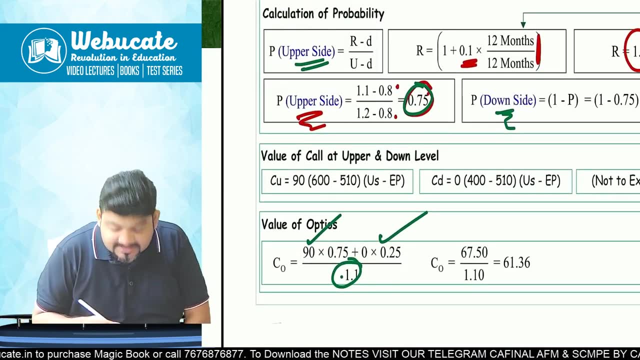 So 600 minus 510.. 600 minus 510, 90 into probability of this happening 0.75.. Then then, if it goes down, then in that case you will not exercise it. So if you don't exercise it you are making a zero rupees profit. 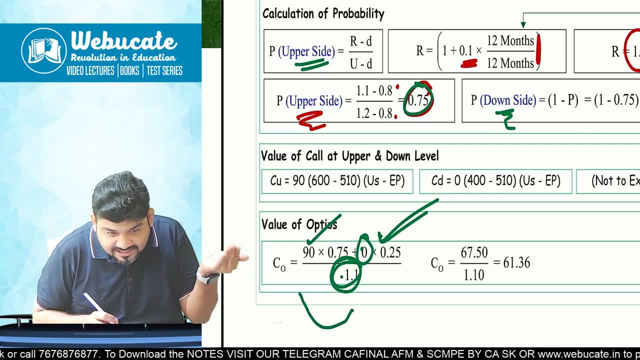 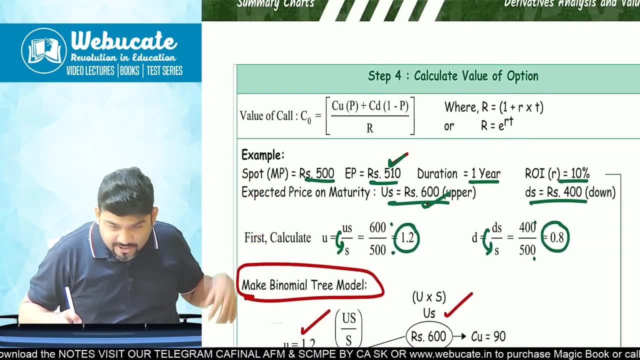 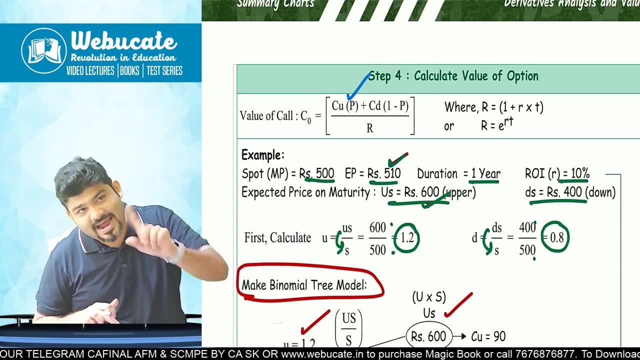 Chances 0.25. bring all of this at the present value will give you value of call option which works out to 61.36.. So value of call CU into P CU is value of call at upper level. See here: CU US minus EP, upper level price minus exercise price. 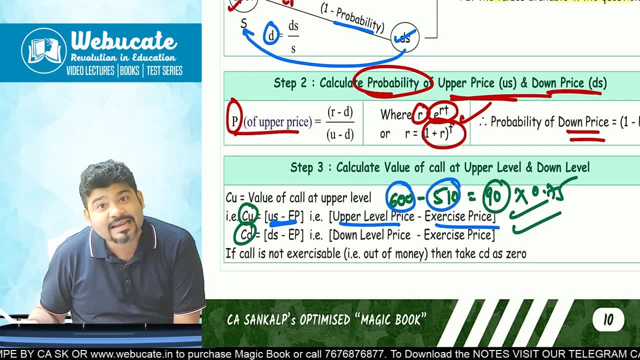 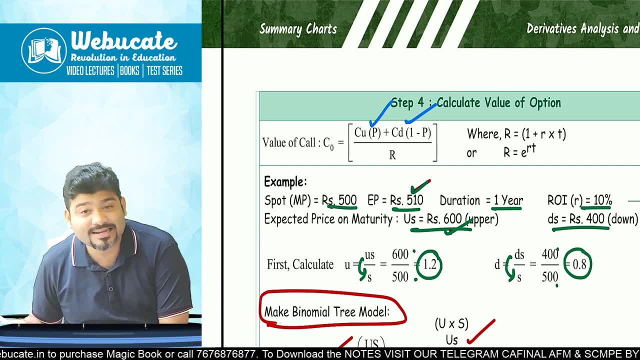 upper level price 600, exercise price 510,. 90 into probability 0.75.. And then CD into 1 minus P. Chances of it going down into 1 minus P. So chances of it going down. you will not exercise 0 into 1 minus P. 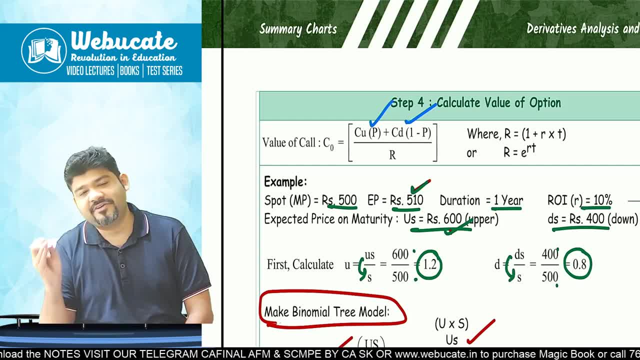 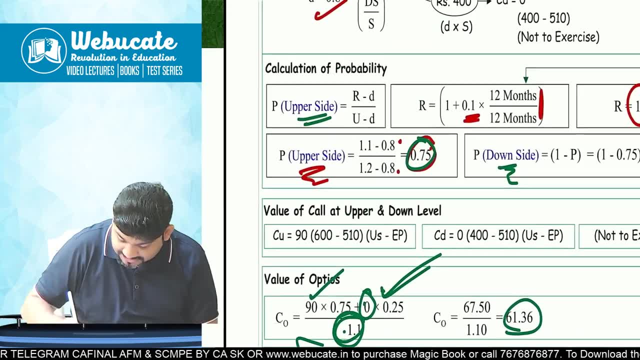 What is 1 minus P, So 0.75, and the remaining 0.25 upon R. Bring it at the present value 1.1.. So this R could suppose if this was for six months. So we would have done 6 upon 12.. 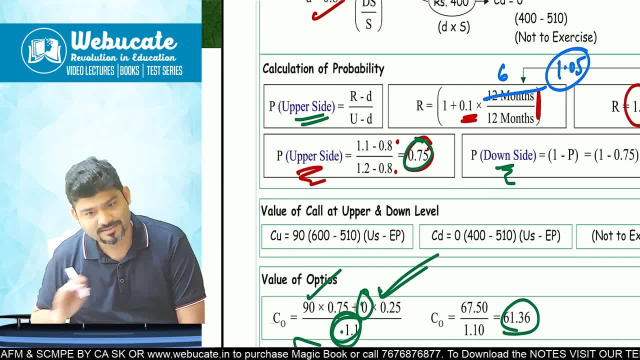 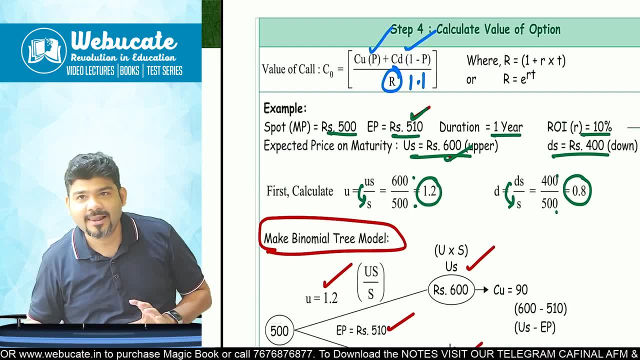 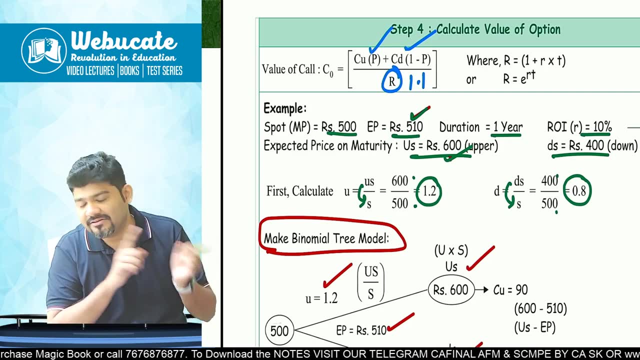 So this would have become 1.05.. Easy peasy Done. So this is how you solve a question on binomial Information will be given. Calculate the probability R minus D upon U minus D Probability, then 1 minus probability is done. 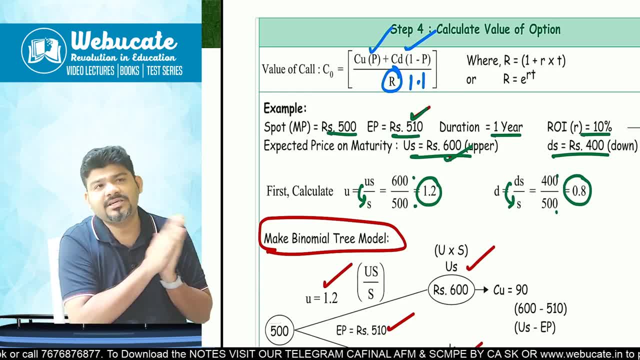 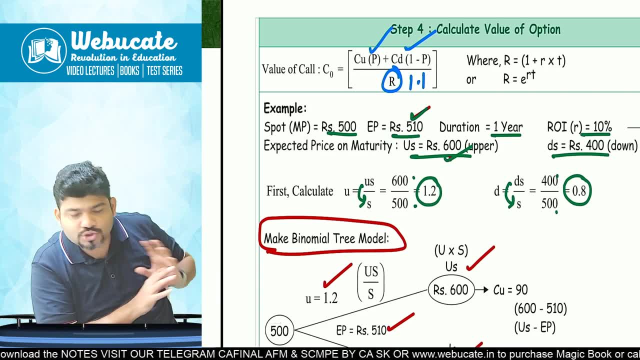 Then calculate the value of call How CU. When it goes up, how much profit you are making, It's probability. When it goes down, you are making a loss. Don't exercise 0 into probability. will remain 0.. Bring both of this at present level by R. 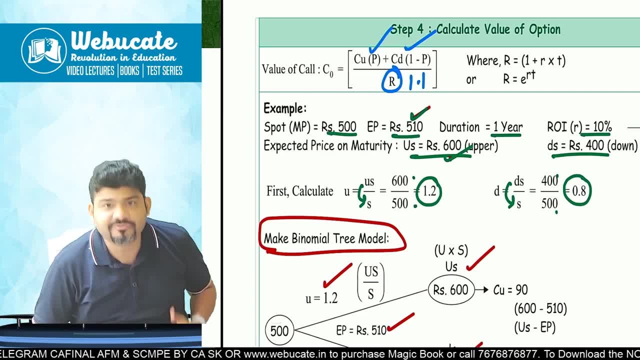 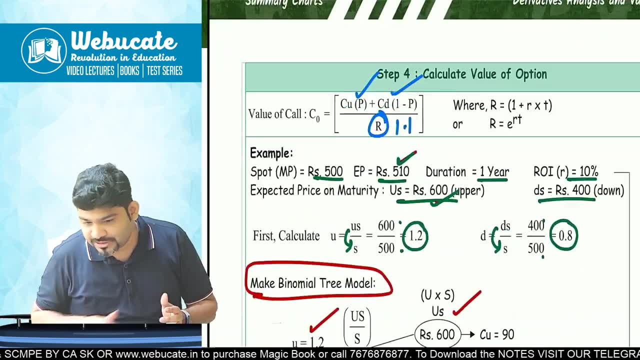 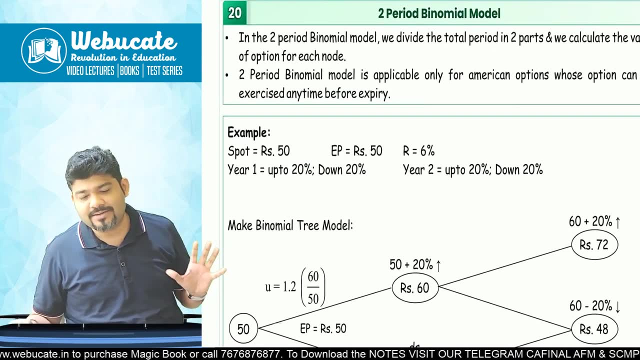 and you are through with the answer for value of call Gotcha. Yes, sir, So that is how we calculate, using the binomial option Done. Then there is something called as a two period binomial, almost on the same lines, Just that you will have to do the same process twice. 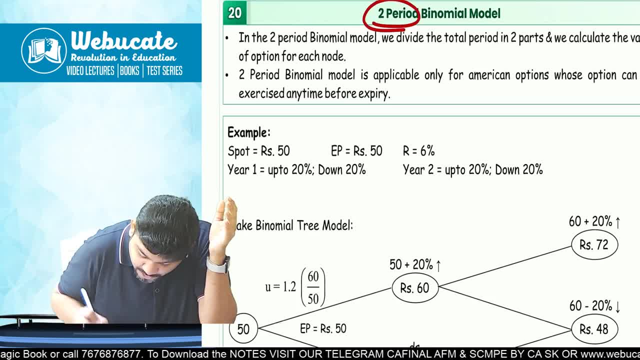 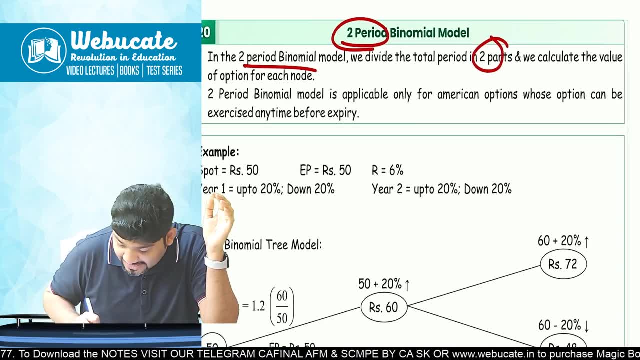 One is binomial, Then there is two period binomial, So doing the same process twice. in the two period binomial we divide the total period into two parts and we calculate the value of option for each node. Two period binomial model is applicable only for American options. 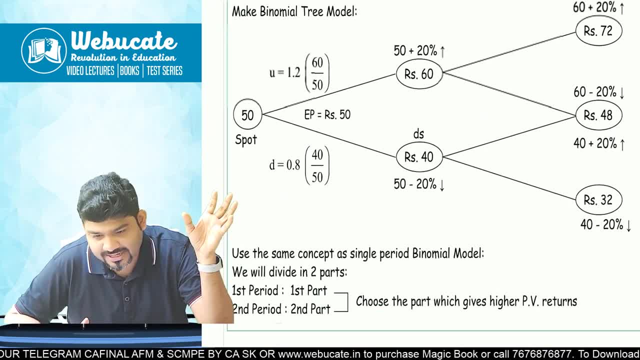 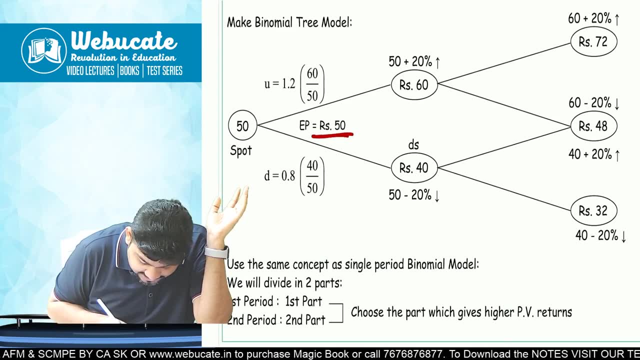 whose option can be exercised any time before expiry. Now here we have the two period binomial model, almost similar type of question. See: 50 is the exercise price, 50 is the spot chances of it going up. So this is your US for one year. 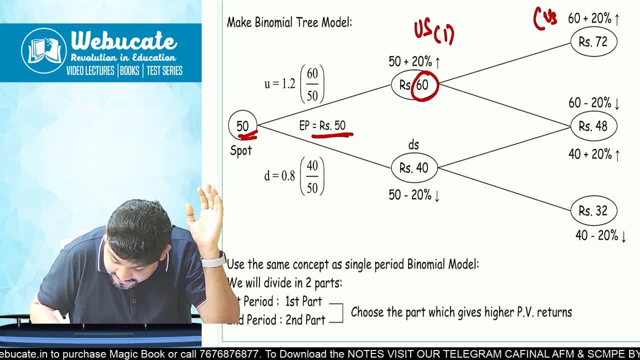 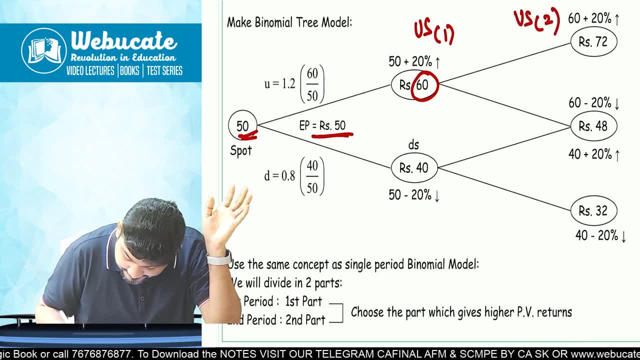 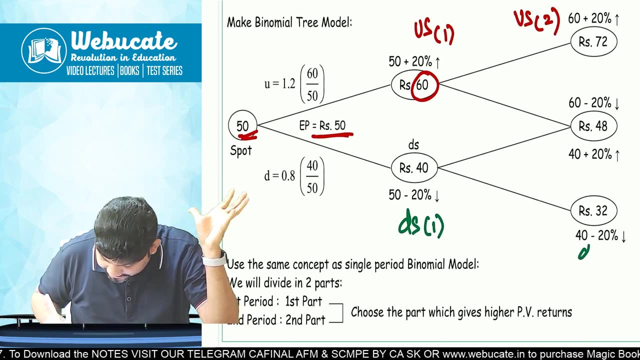 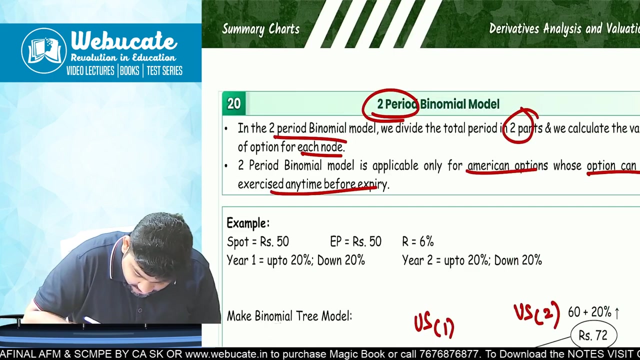 This. then again it goes up to 20 percent US for two years. Then we have DS for one year, And then we have DS for two years. Simple, This is your downside for one year. This is your upside For second year. this is your downside for second year. 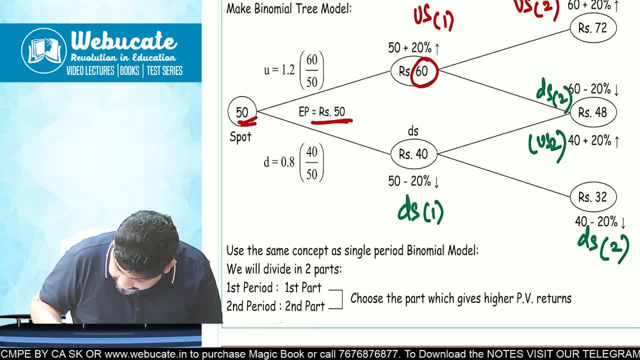 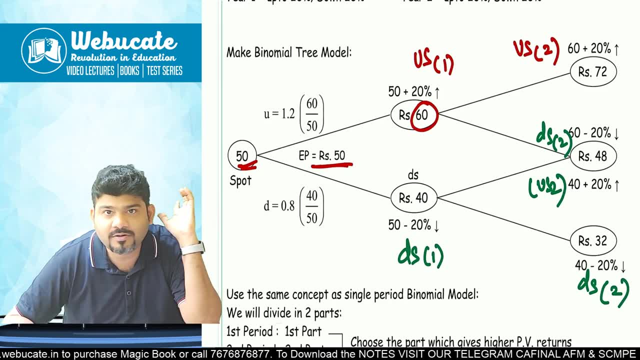 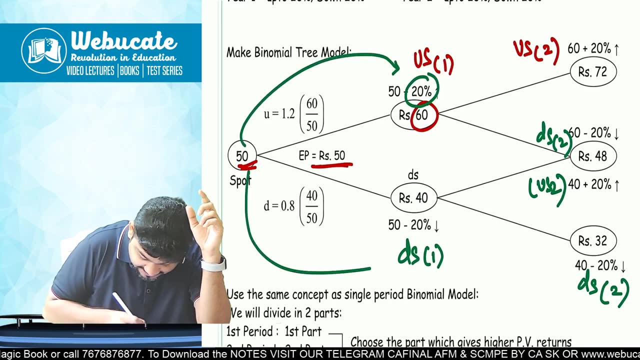 Sorry, Downside for second year. So this all information will be given to you. This all information will be given to you that the increase in price is at the rate 20 percent. So you increase from spot: 20 percent increase, 20 percent decrease. 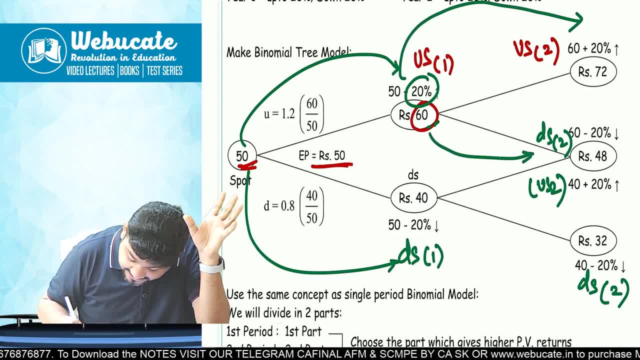 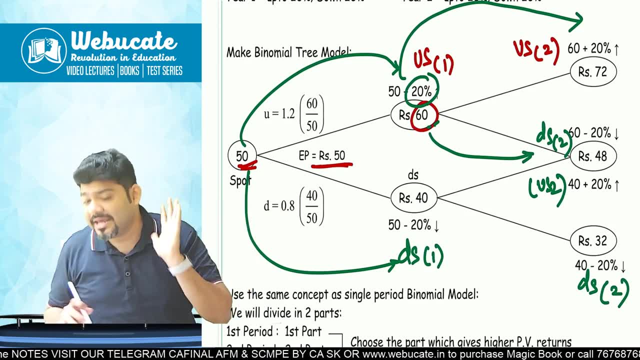 Then again 60.. OK, 20 percent increase, 20 percent decrease. Got it everybody. Now calculate the probability, like we do, and then the value of call, like we do. So let's start. So choose the part which gives higher PV rate. 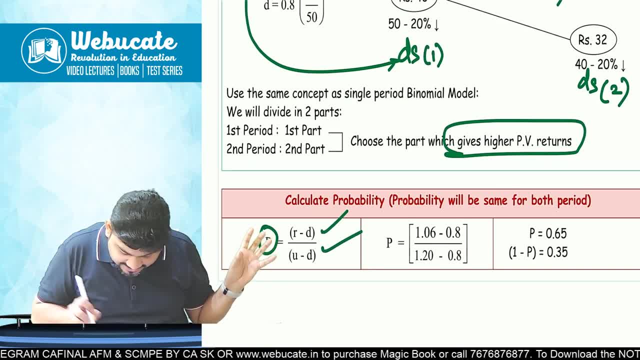 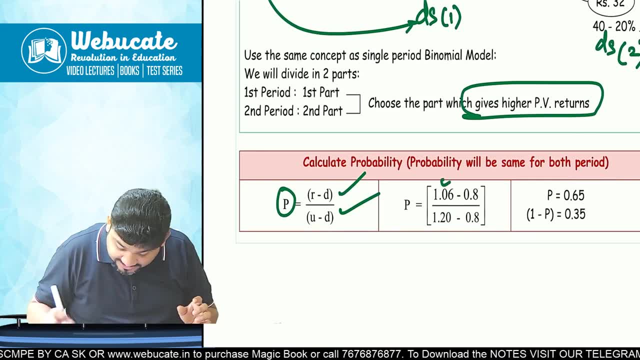 I'll tell you how. So first we will calculate the probability R minus D upon U minus D, So we know R. Now in this question, R is say 6 percent. OK, So 1.06 minus 0.8. one point upon 1.2 minus 0.8, because 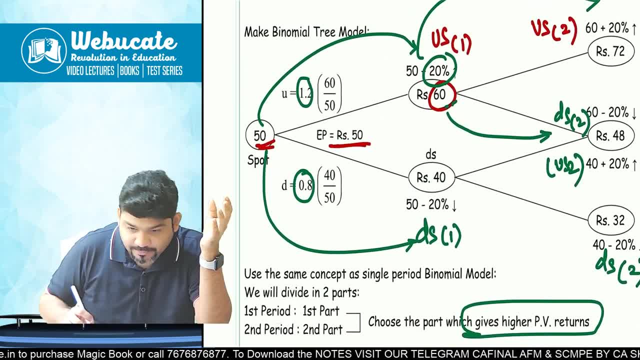 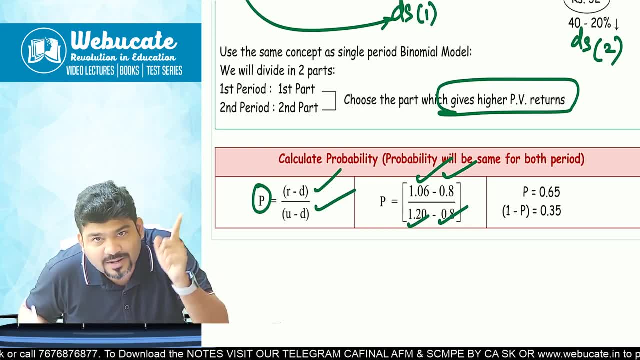 probability of coming down is 80, going up is 1.2, going up is 1.2.. Got it everybody. So P is equal to 1.06 minus 0.8 upon 1.2 minus 0.8.. 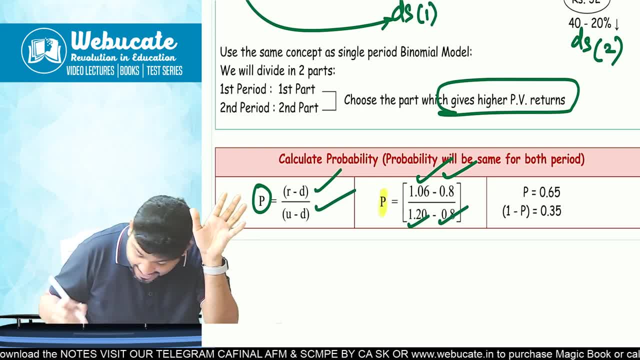 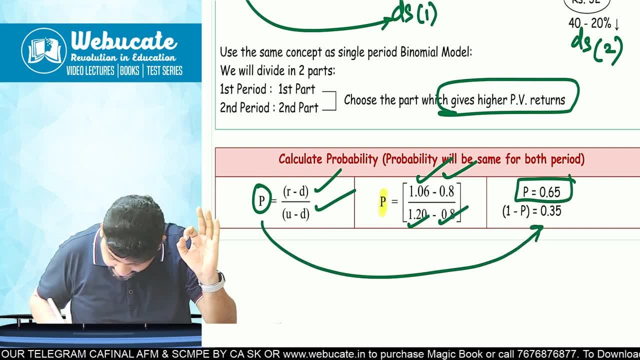 We will get the probability at 0.65.. Sorry, we will get the probability at 0.65.. And then 1 minus P will become obviously 0.35.. Done Now, the whole sums probability. we know what is it. 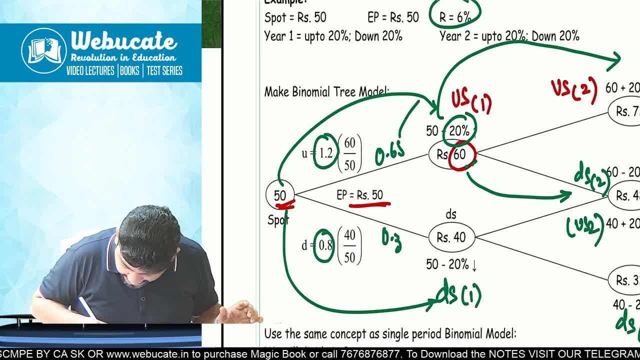 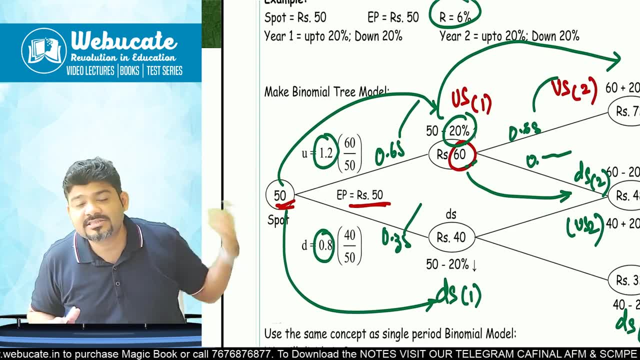 It is 0.65, 0.35,, 0.65, 0.35.. Got it, So probability of going up 0.65.. Now comes the main comparison. In period one we are going to get 10 rupees profit. 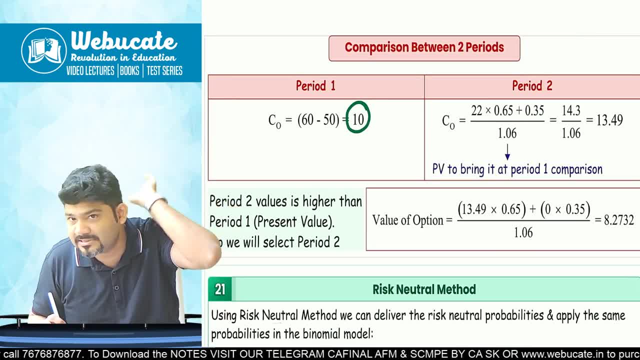 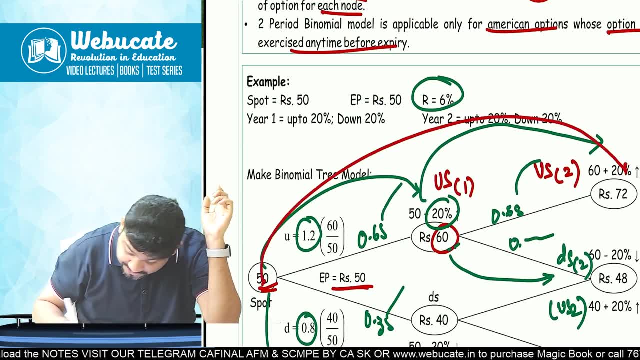 Correct Because 50 rupees has gone up to 60 rupees. Correct In the case of period two. pay attention. Can I say it has gone up from 50 to 72?. Pay attention everybody. Can I say from 50 it has gone up to 72.. 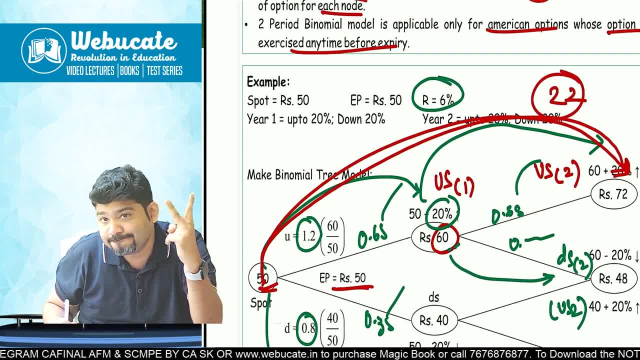 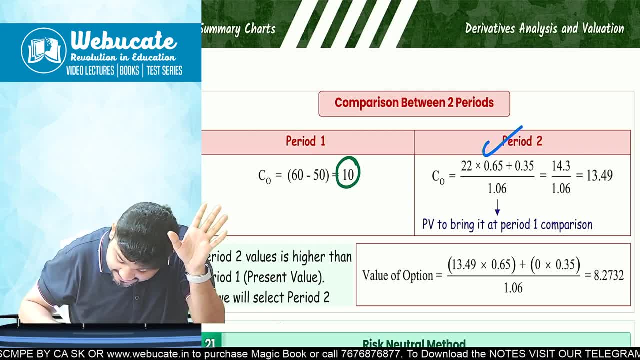 So 22 rupees profit it is making. What is the probability? 0.65?. So 22 into 0.65, 22 into 0.65. Then chances of it going down. But if it is going down, then in that case I will not exercise. 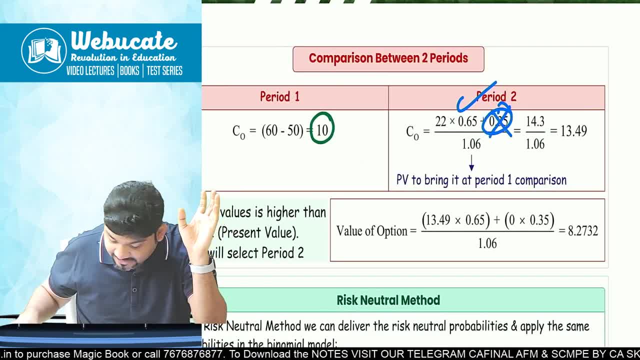 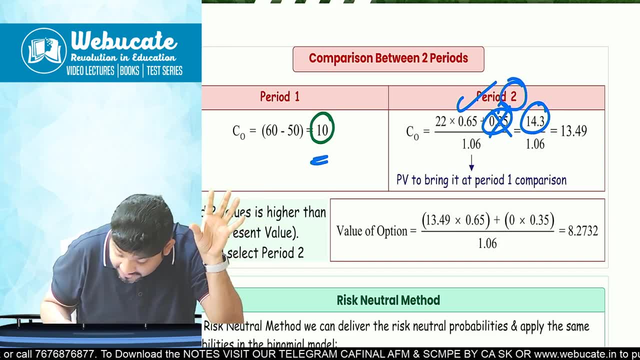 So this will remain zero. This will remain zero. So 22 into 0.65 will give me 14.3.. Bring it at first year's value. This is after two years. after two years, Ideally it should be. if I want to bring it at the present value, 1.06 raised to two. 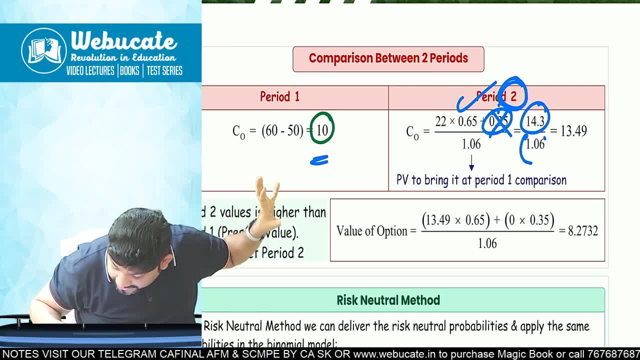 But I just want it at this period one level. So just do it till for once. So from year two it will now come to year one, So it is 13.49.. Tell me if you have taken the call option, you want the market to go. 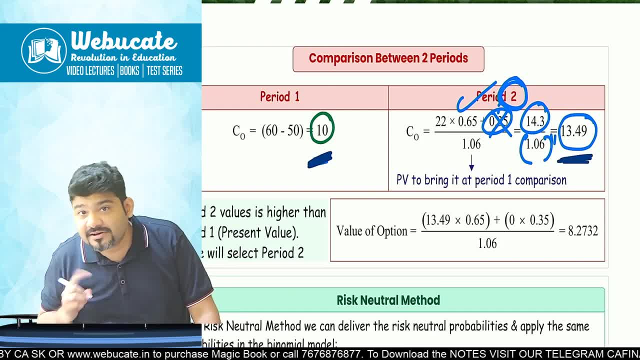 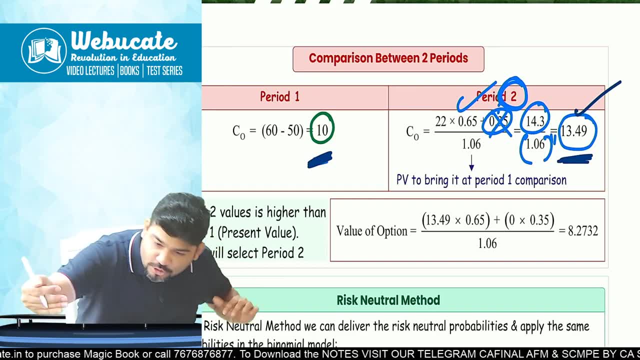 Till 10 or 13.49.. But obvious 13.49.. You will exercise period two, You will exercise at period two, And then that also you will bring at the present value. So then again, 13.49 is free. 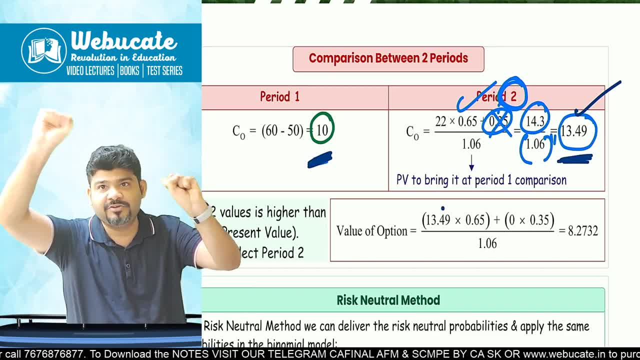 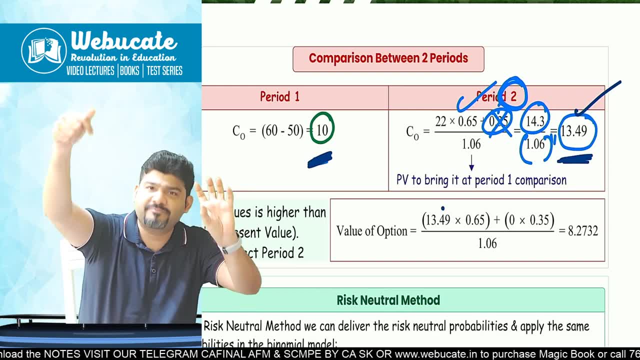 See period one or period two. We have two options. When do we want to exercise? If you are exercising at period one, 10 rupees profit. If you are exercising at period two, 22 rupees profit, But with a 65 percent probability brought at period one by 1.06.. 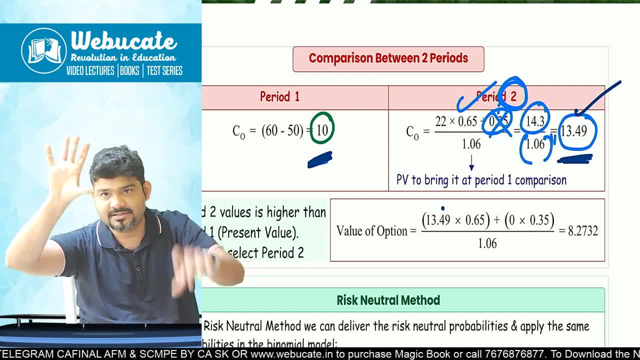 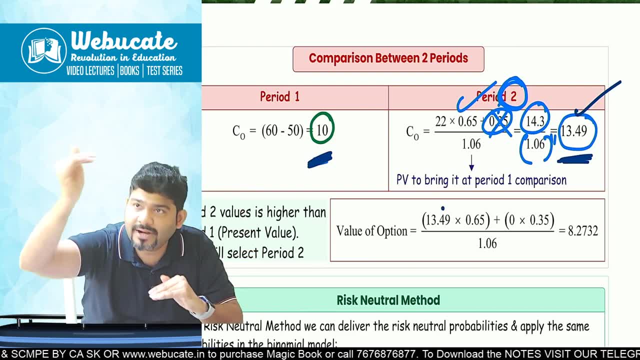 Present value, So 13.49.. Comparison: 13.49 is better By 10.. 13.49 finalized: Again, bring it at the present value. But the 13.49 chances are again 0.65.. So we bring it at the present value, 1.06.. 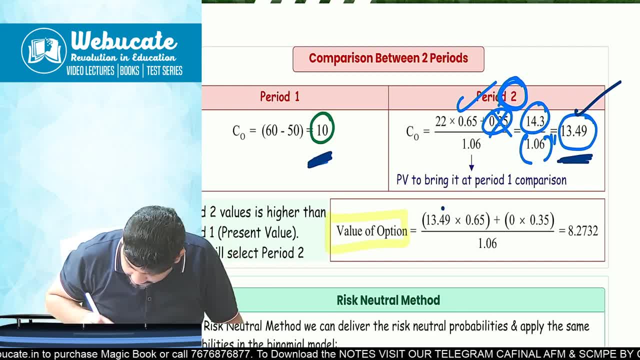 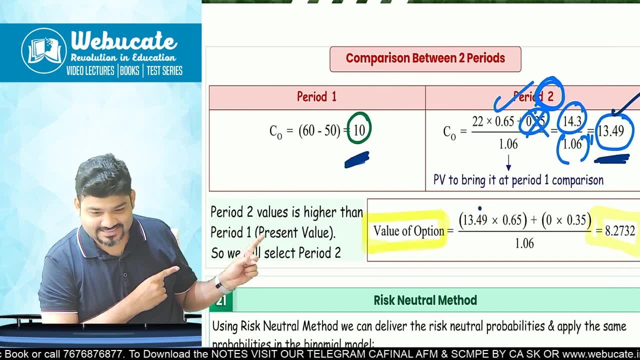 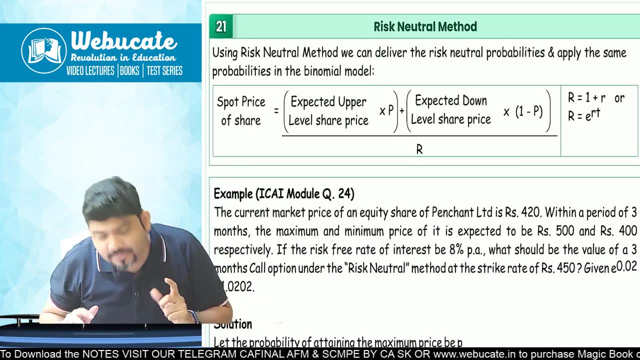 And that's how we will get the value of option. That's how we will get the value of option. Hey everybody, That's how the comparison between two periods happen. Now, in this, to calculate probability, there is another method, called as the risk neutral probability method in question, 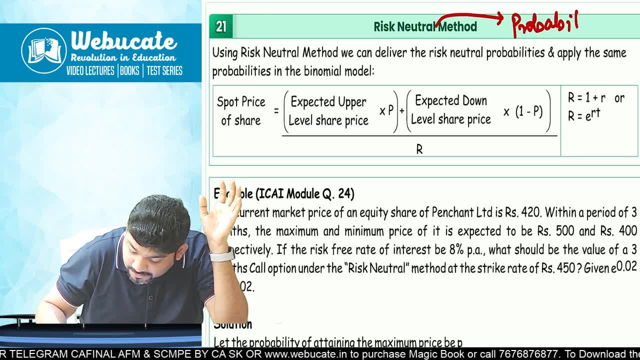 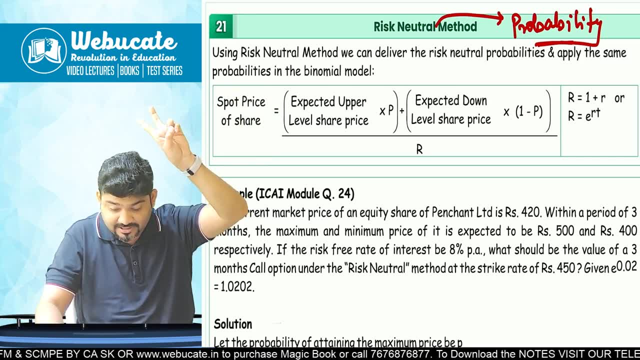 If they say: calculate using the risk neutral probability method, then you have to calculate probability using this method only. There are two methods to calculate probability. One is: probability is equal to R minus D upon U minus D. The other method is risk neutral probability. 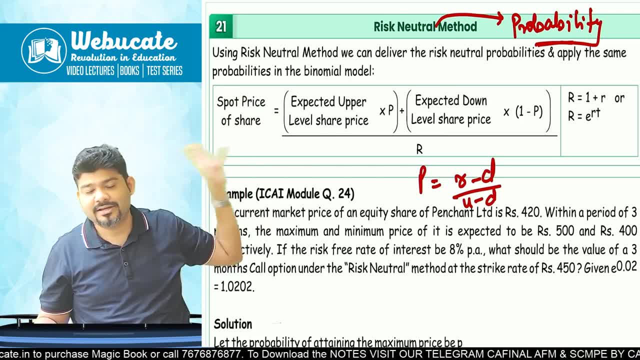 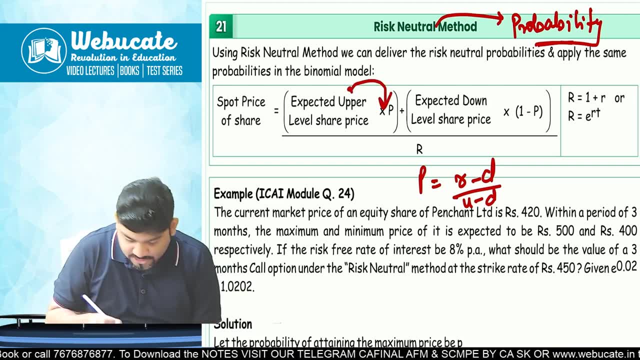 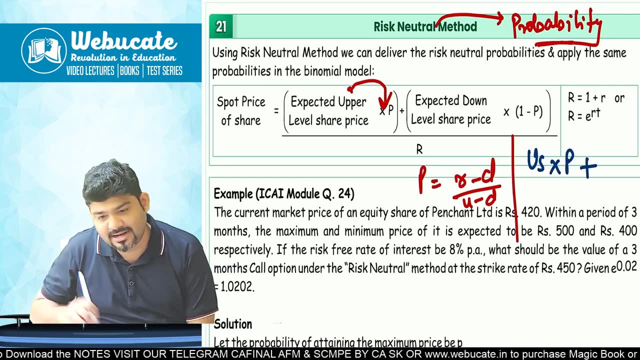 And this is what that calculation is. This is what that calculation is. What is it? Expected upper share level price into P. So US into P. So the other method is the other method: US into probability plus expected level at down price. 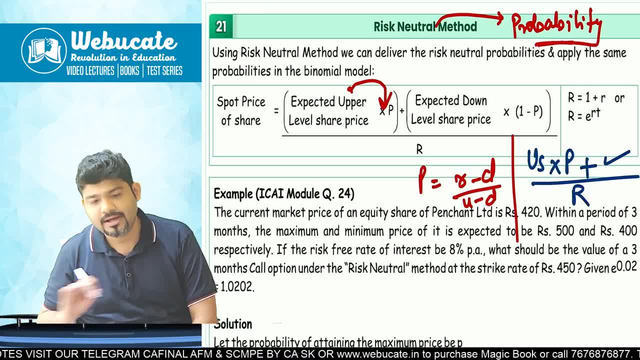 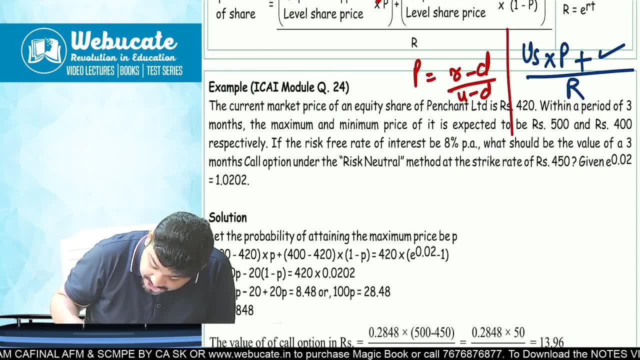 Only if we exercise upon R, upon R. So we have a calculation. We have an example down here. Let's try. The current market price of an equity share is rupees 420 within a period of three months. Maximum and minimum price. 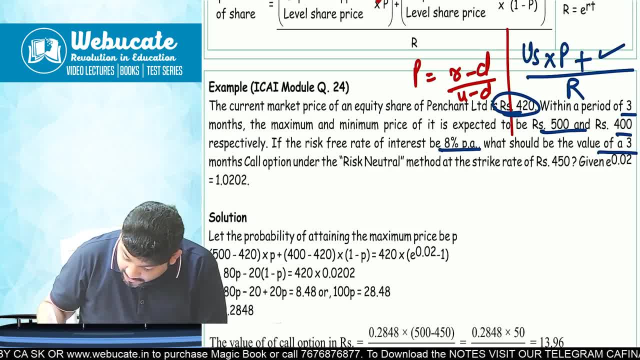 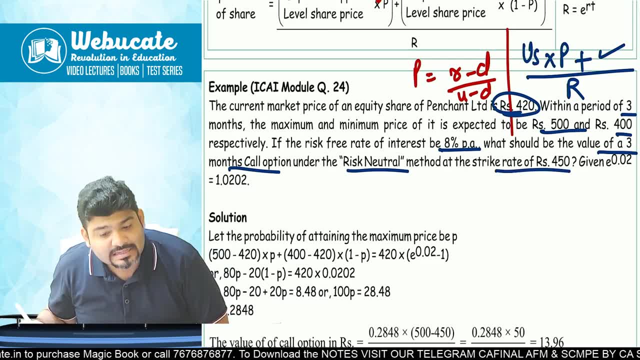 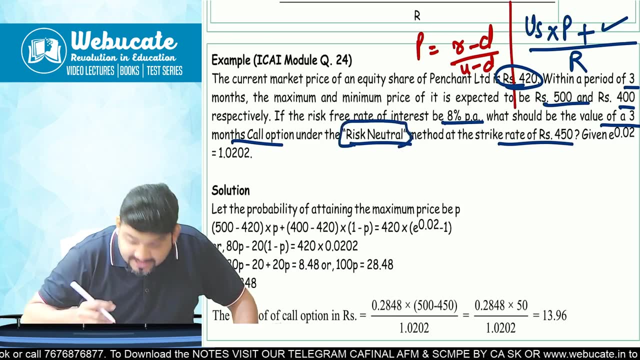 If the risk rate zero eight percent, what should be the value of three months call option under the risk neutral method at the strike price of rupees 450?. So now here you will have to try and calculate using the risk neutral method, because they have specifically told the risk neutral method. 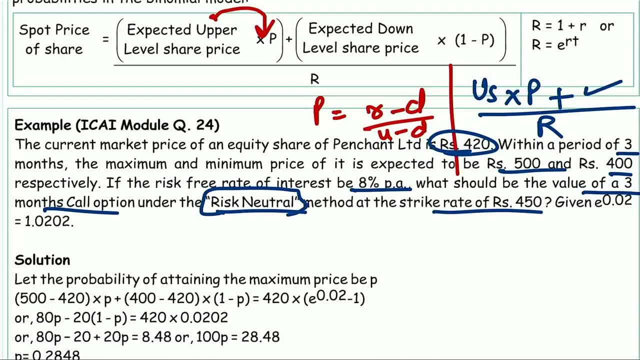 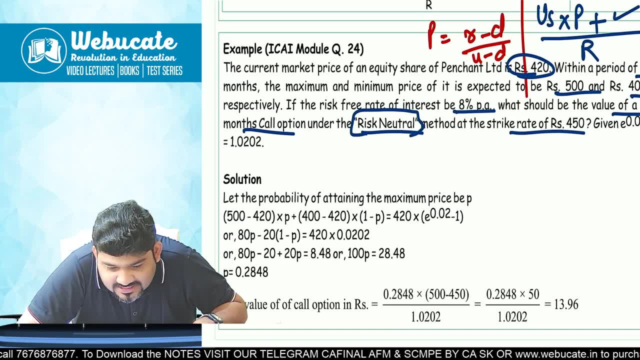 Use the formula that is given here and see how you will get the answer. Come on, give it a try. So I'm assuming you would have paused the video and solve the question Now. let me give it a try. So what's the formula? 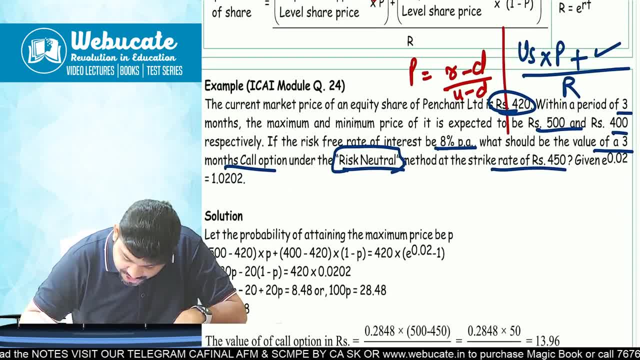 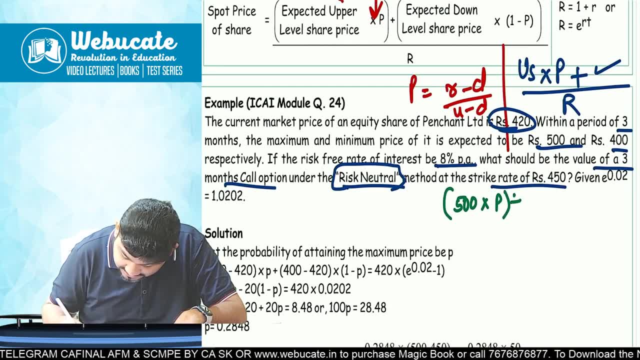 Upper expected level of price. level of share price. Can I say it? The upper level is expected to be 500.. Yes, sir, Multiply by P. Yes, sir, Plus expected share level price, that can go down. It can go down to 400 into one minus P. 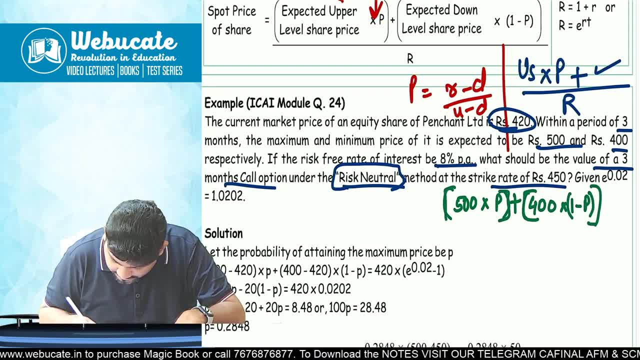 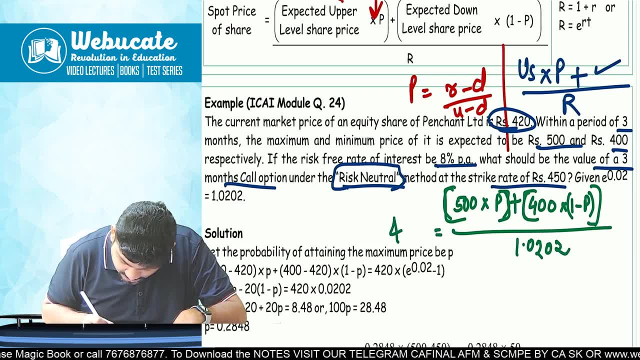 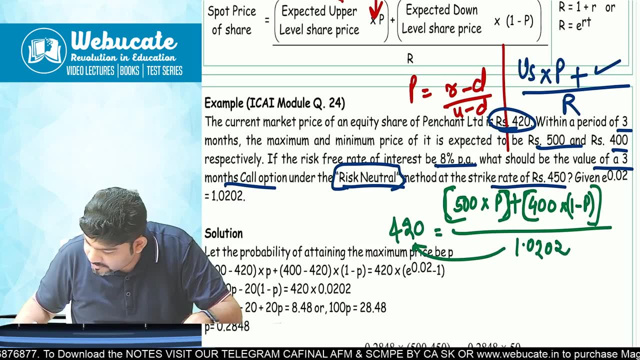 P, P, P, P P. One point zero two, zero two is equal to 420.. Now let's now take this year, So 420, into. how did you get this? So, given zero point zero two is equal to one point zero two, zero two. 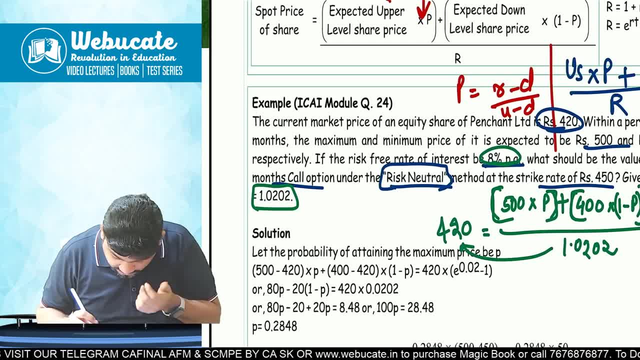 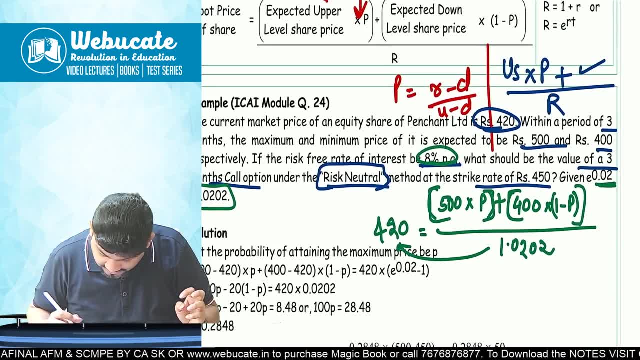 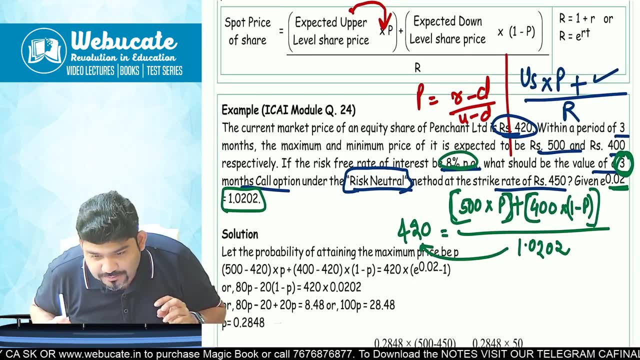 Eight percent per annum, But all of this is for three months. No guys Here of a three month Call option? Yeah, three month call option. So eight into three by twelve, two percent e raised to zero point zero, two point zero, two zero two. 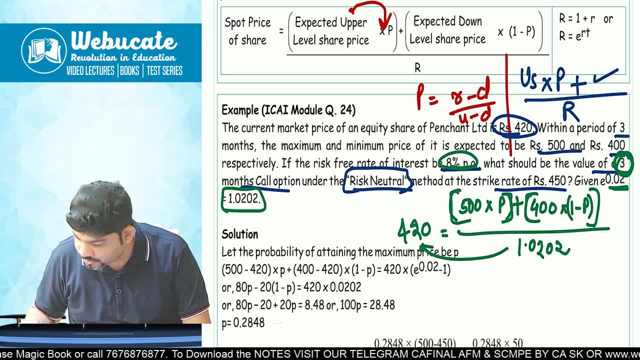 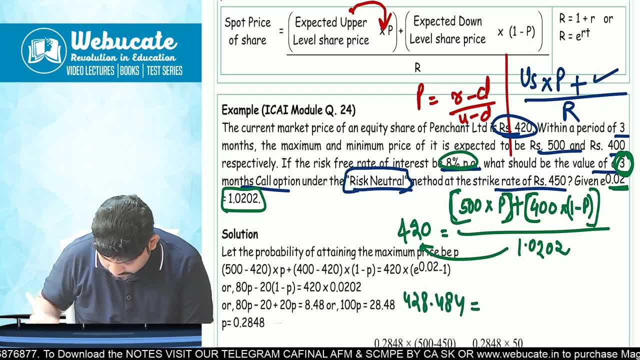 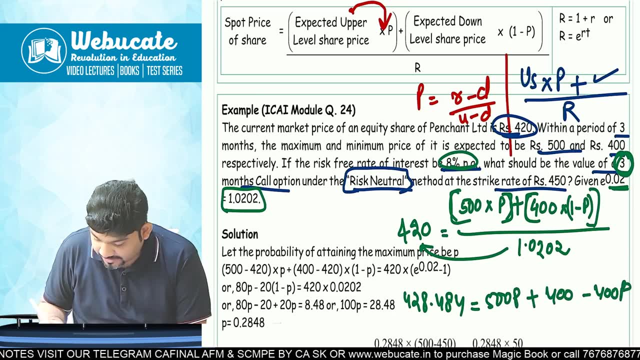 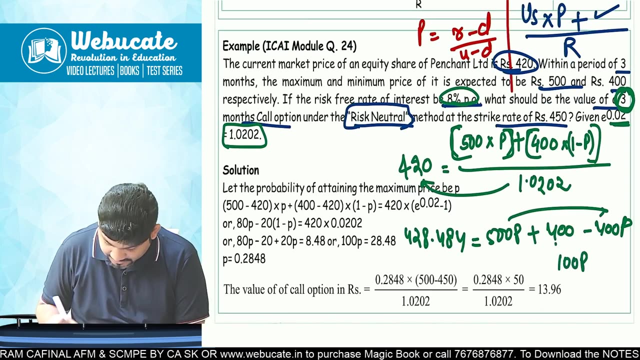 So 420 into one point zero two. zero two will become four twenty eight. point four eight four Will be 500 P plus four hundred minus four hundred P, That, So this will become 100 P. This will go here, So it will become 400 minus four twenty eight. 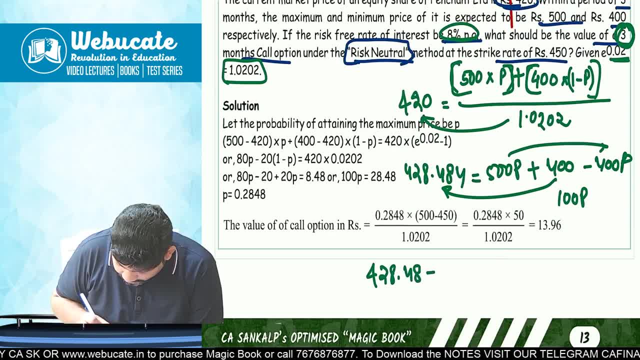 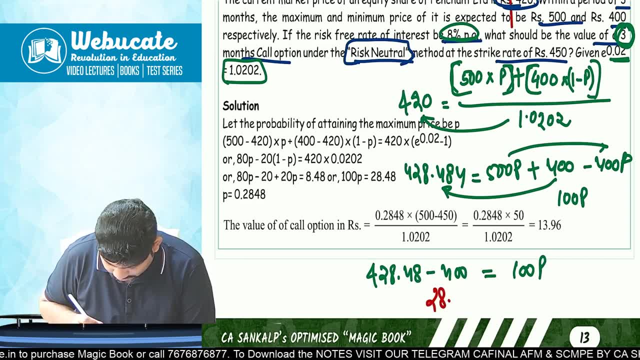 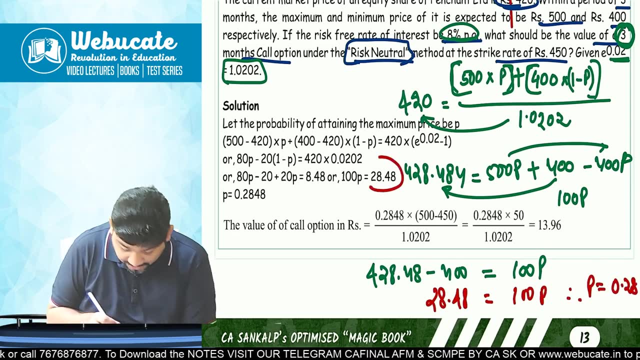 So it will become, see like this: four, twenty, eight point four, eight minus four hundred is equal to 100 P. Twenty eight point four, eight is equal to 100 P. Therefore P is equal to point two, eight, Four. P is equal to point two, eight. 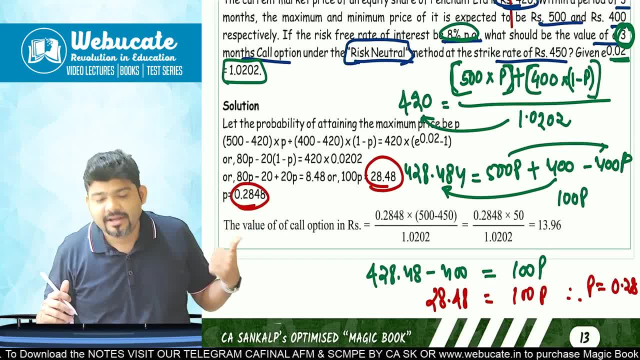 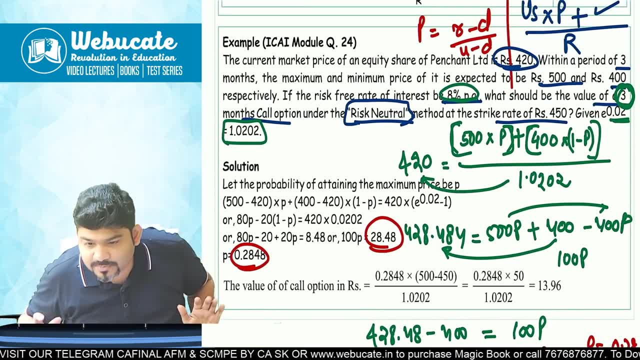 Four ten. That is a probability. Now how do you calculate the value of call? So how do you calculate the value of calls at 420? And then goes, it can go up. So the exercise price is what. Exercise price is what. 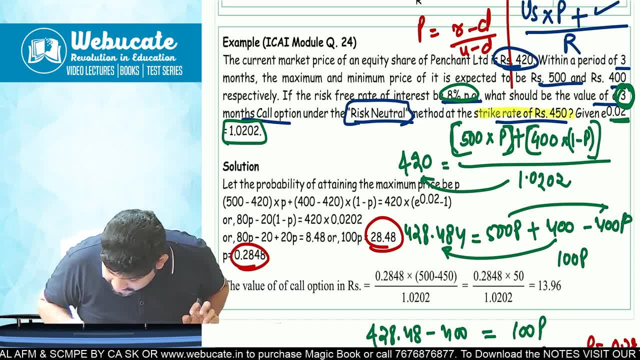 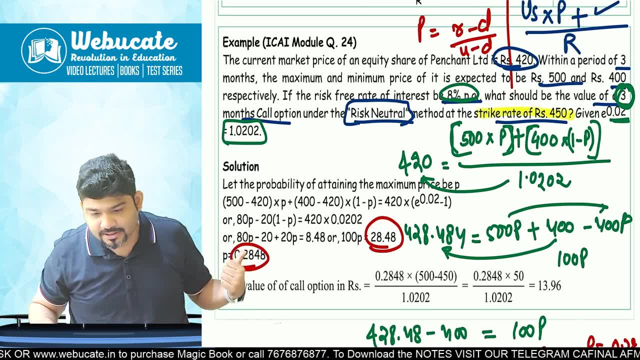 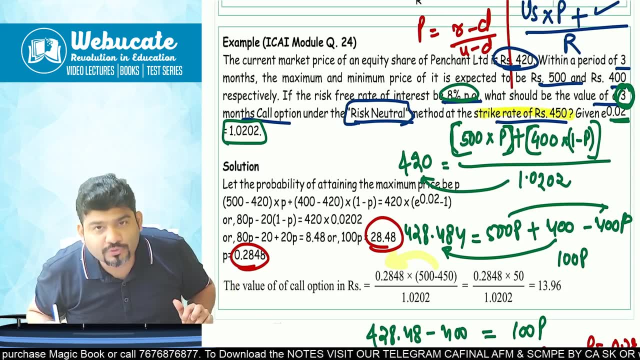 450, I guess Strike price is 450.. So if strike price is 450 and it can go up till 500.. So 50 rupees, What is the probability? Point two: eight, Four, eight, Right, And the other option is it goes down to 400.. 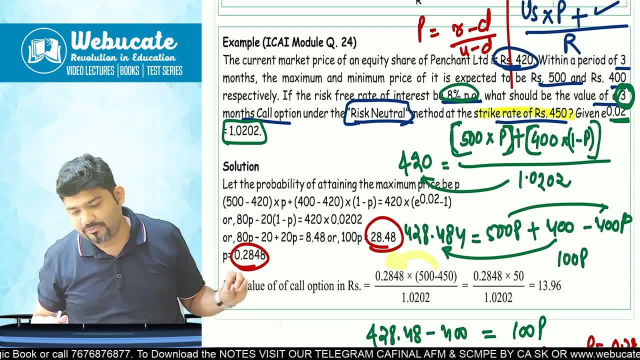 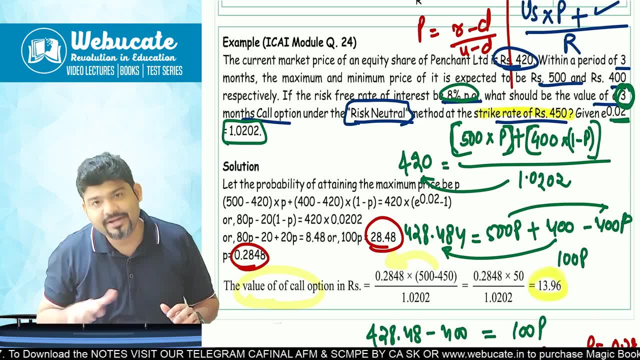 We will not exercise So point two, eight, four, eight, into 50 upon one. point zero, two, zero, to bring it at the present value, We will get the value of all option. Hello, We will get the value of all option. Thirteen point nine, six. 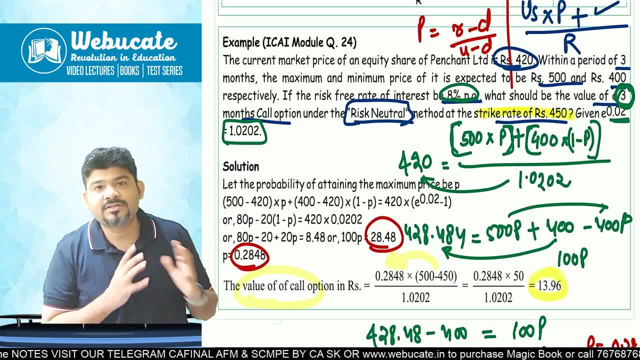 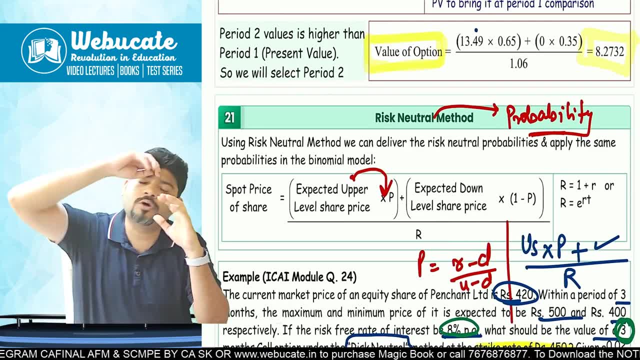 Thirteen point, nine, six, Got it everybody. So this is how the system works. as regards risk neutral probability method, One of the most important questions that can come is going to be based on binomial, So we are done with binomial. 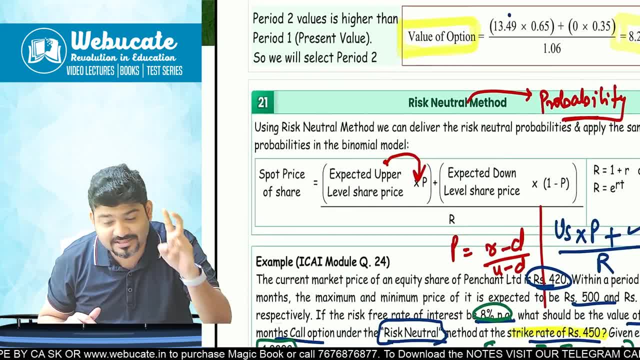 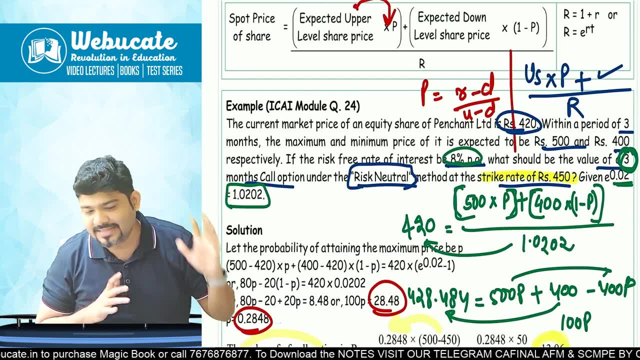 We are done with the two period binomial as well. We are done with the risk neutral method, Probability, that simple way, Probability, all of the methods we have done on it, And that's where we complete the binomial method as well. And now you come to the black and schools. 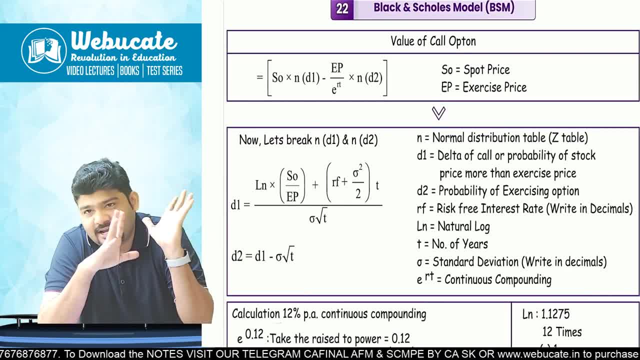 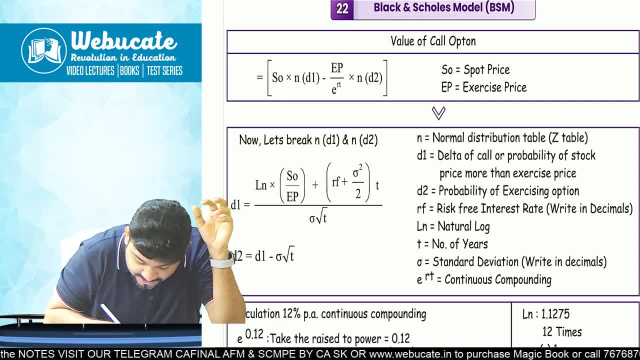 So far in the exam, either the basic level comes or the binomial method. Both of that we are done. Now comes the black and schools. the chances of black And schools coming in the exam are very low As per the previous probability, as in in previous exams. 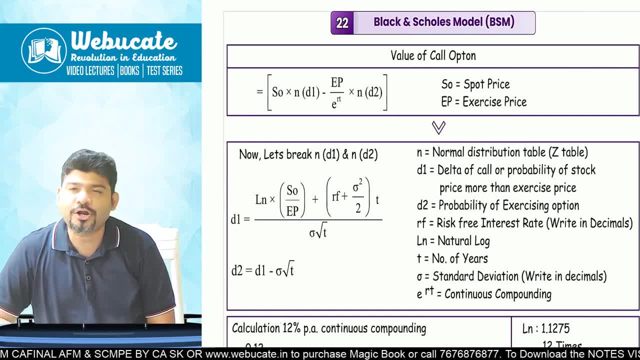 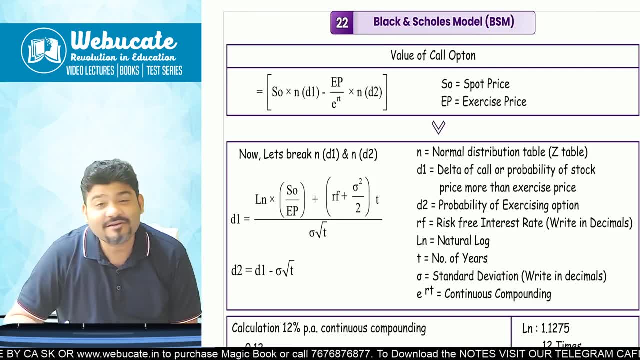 black and schools has not been asked for a lot of years, a lot of years. Even when I was studying, we were expecting this not to come. But you never know what. if your attempt is going to be the golden attempt and black and schools is going to be asked, 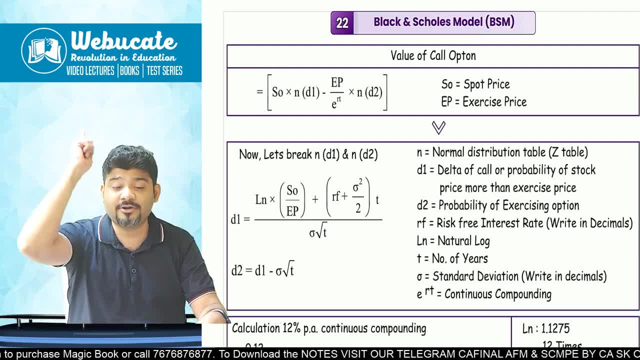 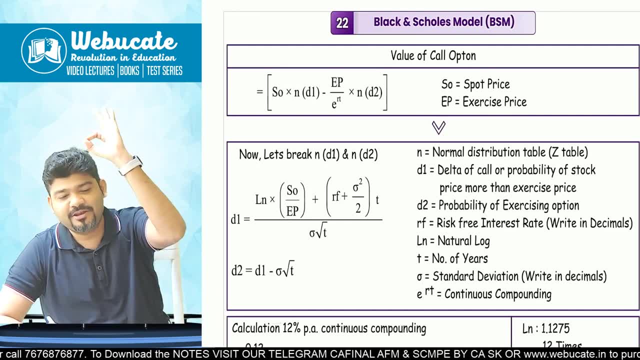 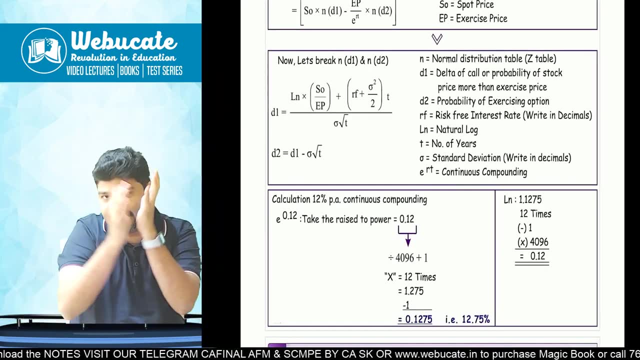 So I will be specifically solving questions on black and schools right from your module, Yes, But that right from the module I will be solving questions on black and schools method, but not at this point in time because that is a lengthy process. So what I will do is first I will complete. 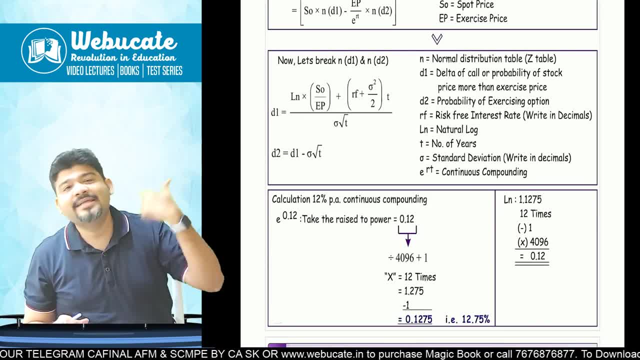 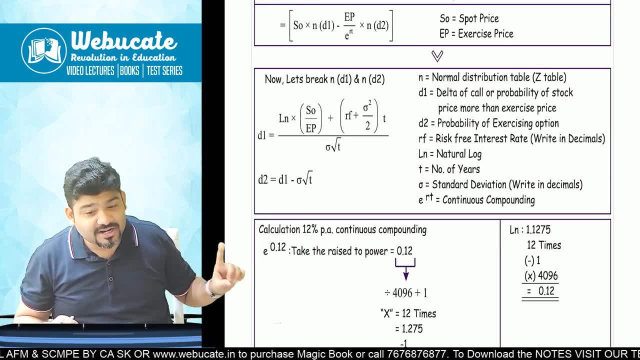 the remaining parts, as in whatever is left in our options, And then the whole futures I will complete, and then we will come back to this. Don't worry, We will come back to black and schools. I will teach you all how black and schools is to be practically applied. 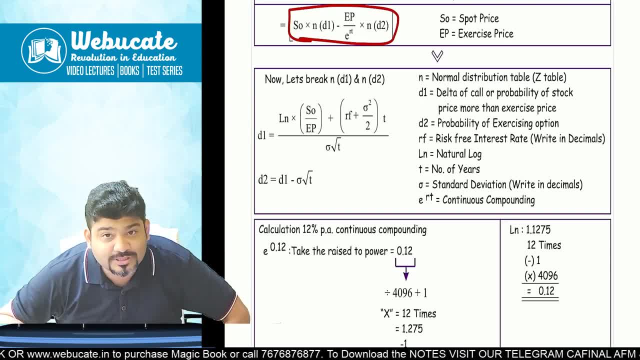 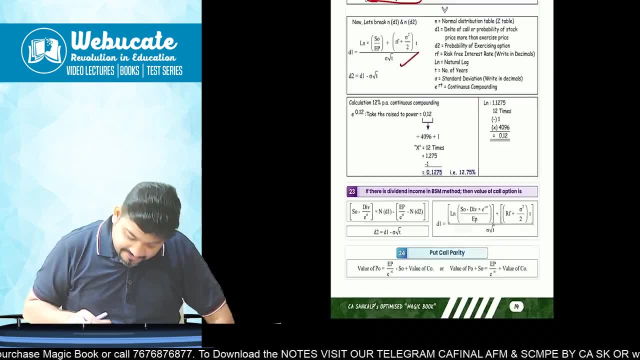 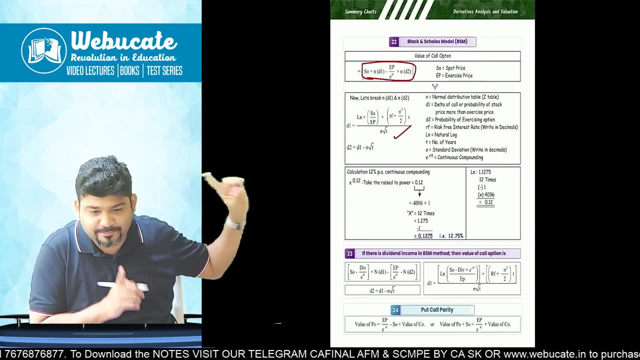 How this, as in the formula, is to be thought of and how you can actually remember the formula. It will be a very, very easy process. Once you are done with that, we will say that, OK, the thing is done. So for now, only with your permission, only with your permission, only this one page. 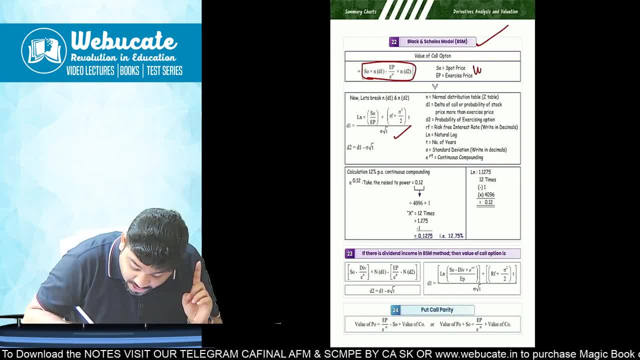 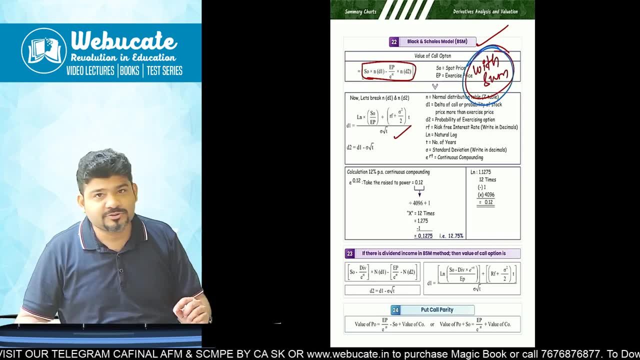 I am not touching because black and schools I will be solving with some. Why am I going to solve it with some? Because, as for the new syllabus, as for the new syllabus, there is something called as real options, which has been introduced, which has 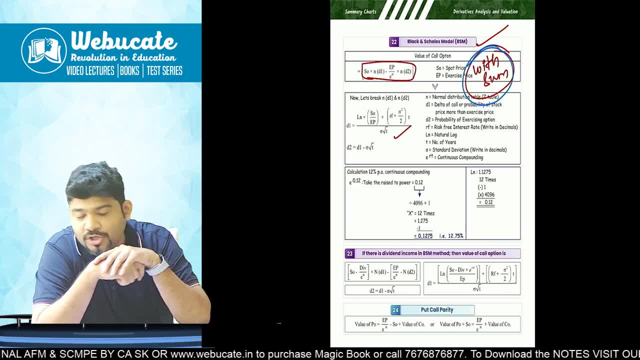 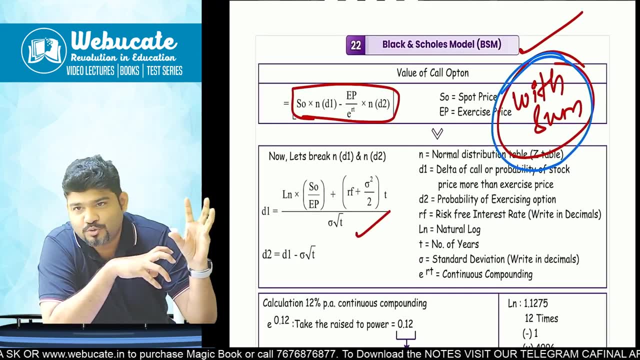 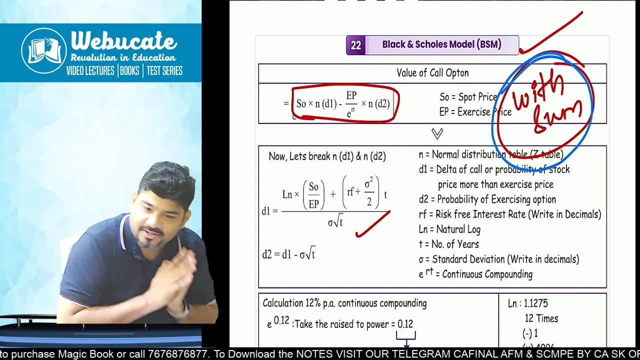 abandonment option, Timing of options and all of that. So all of that has few traces of black and schools model. So I will teach you black and schools model plus real options, with practical examples given in our module Right, So that you are totally secure. 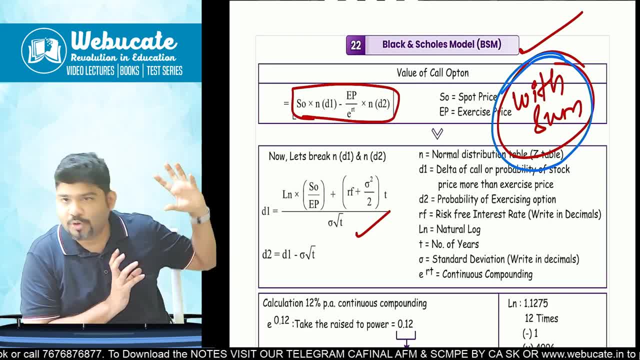 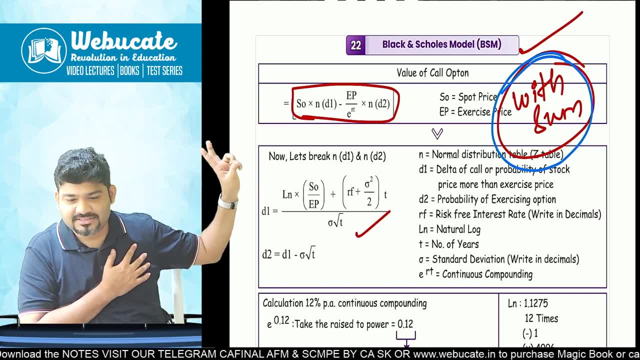 All of the questions which are there possibly in the module. I will teach you So black and schools, plus real options with sums. I will teach you all with sums. I will teach you all, But at the end. So now we will continue with our options thing. 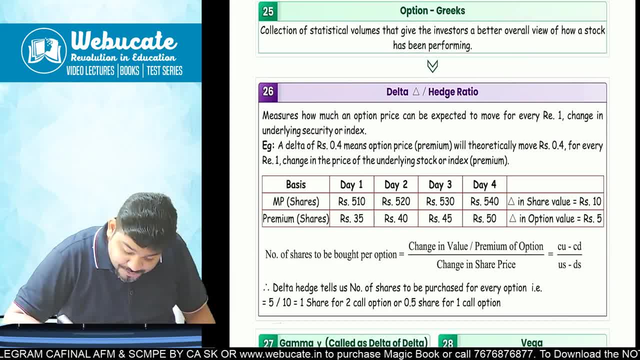 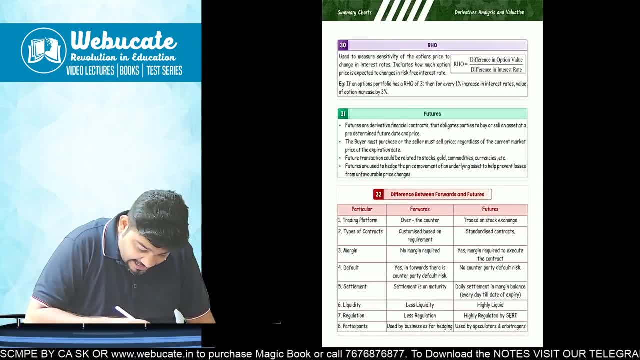 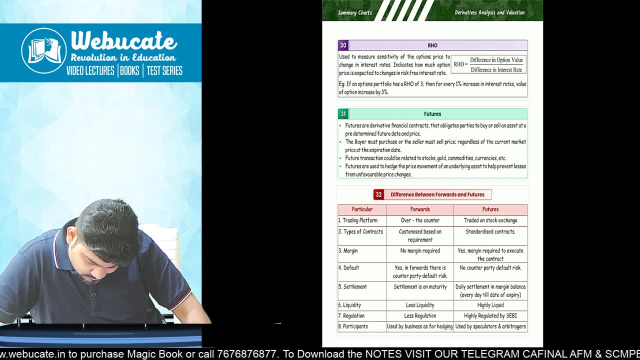 wherein we have the last part, which is called as the options Greeks. But again, even after this, if you observe, we have the real options, as I told you, that is the real options And as you will find it in your book. so, 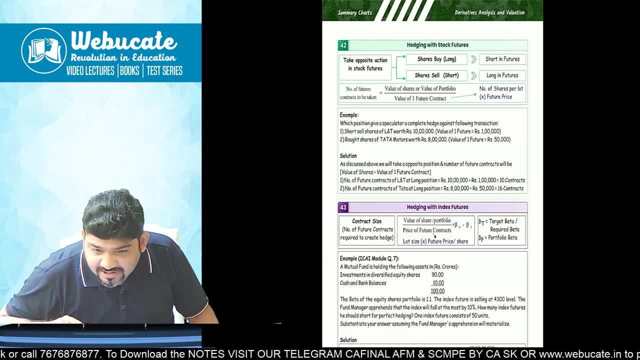 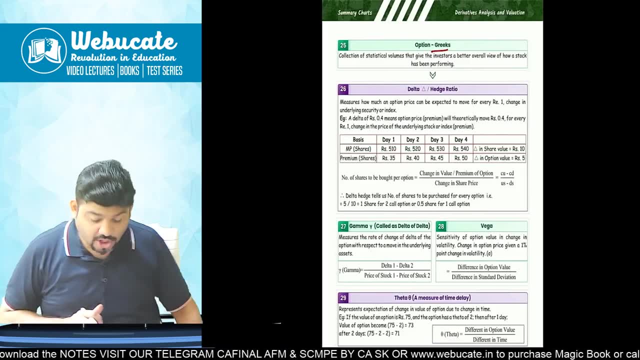 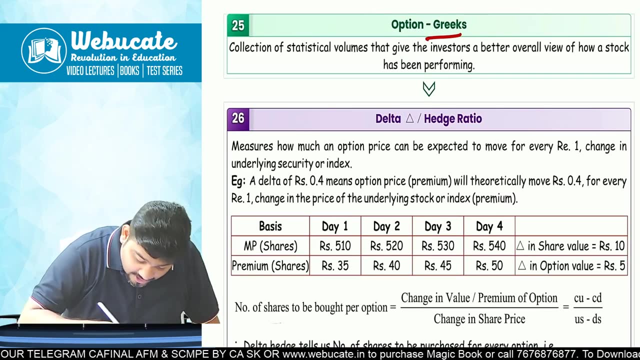 that, real options, the abandonment option, and all of that I will be doing again, as I told you all, with the practical sums of our ICI module. Till then, let's complete the next concept, And that is called as the option Greeks. 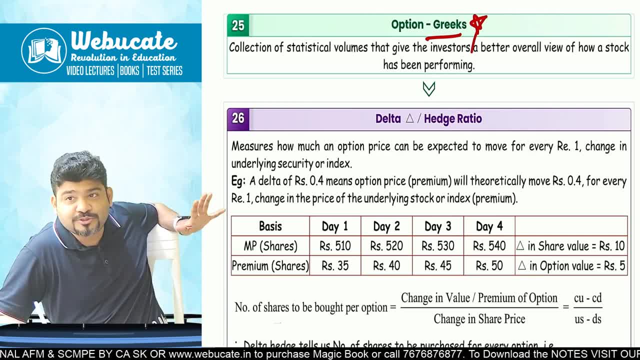 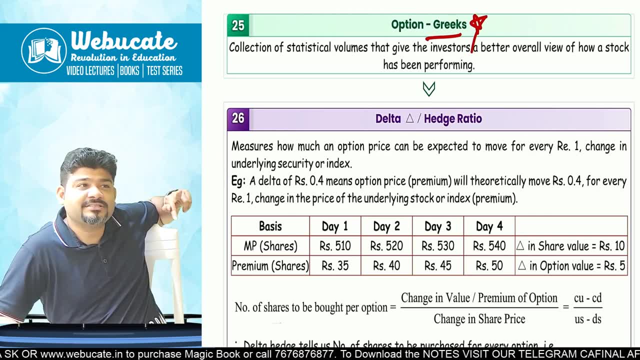 From once we are done with option Greeks, we'll be done with options, but without black and schools and real options. then we will do the whole futures, then we will come back to Options and real options and then the whole derivatives will be complete. 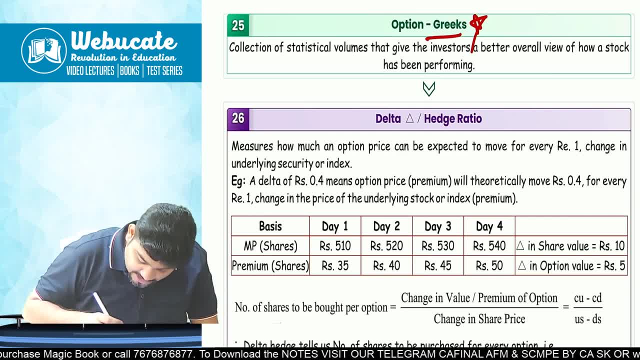 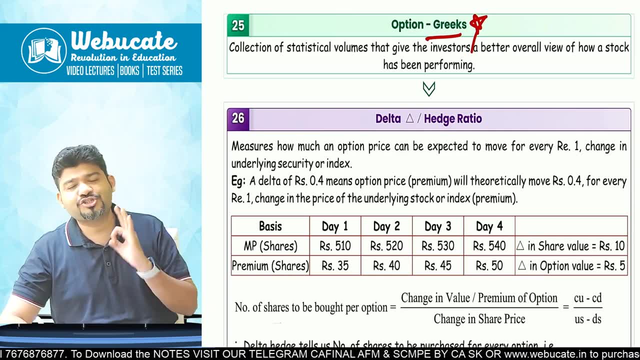 Let's continue now in option Greeks. This can also come for the MCQ, for sure, If I am your paper setter, mind you, if I am your paper setter, for sure I will have a three to five mark question on option Greeks, and that to a case study. 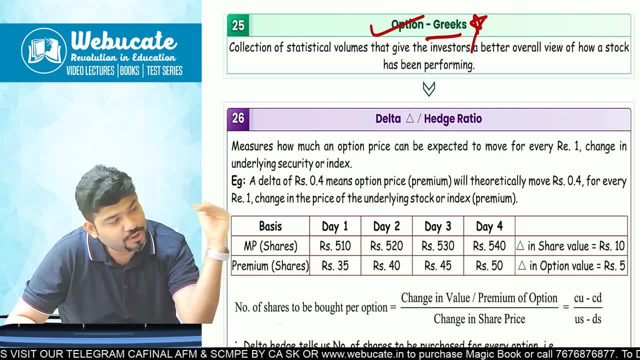 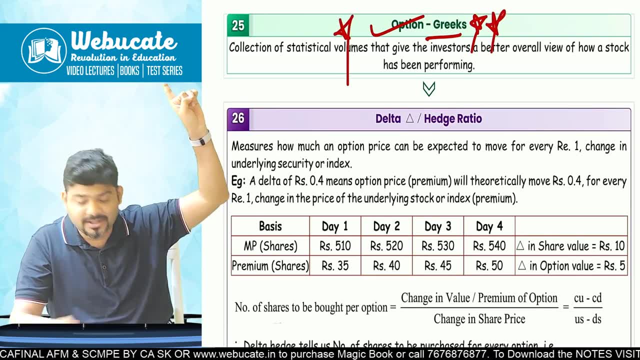 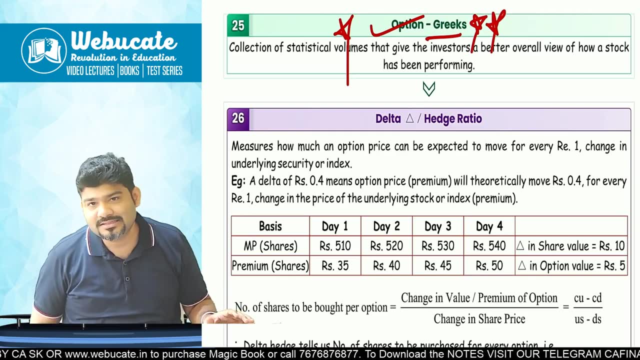 And in that case study, I will ask you questions One, two, three, four, five, all related to option Greeks. So, mind you, it is very, very, very important. if a paper setter like me comes, then you are definitely expecting a five mark option question in this case. 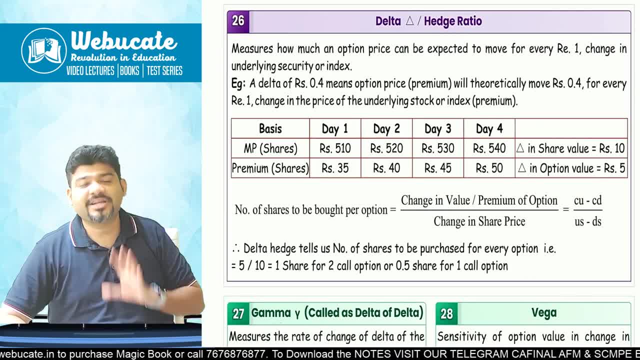 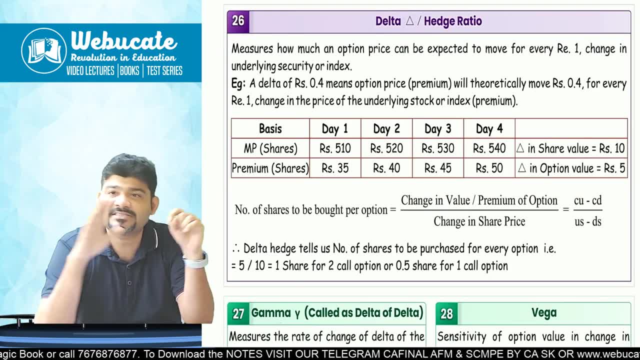 So first is called as the delta or the hedge ratio, meaning There are two things which we have: one: either we invest in shares or we invest in call options. So there is a ratio which both of them have that instead of buying the shares, 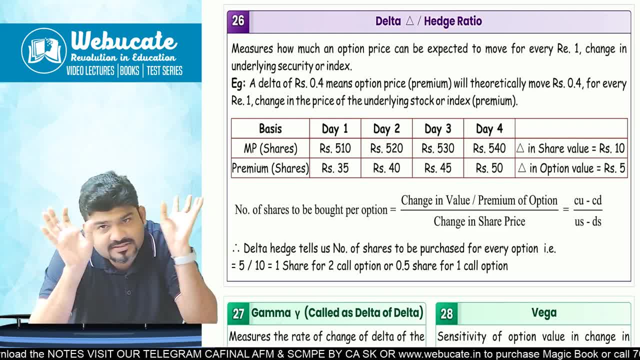 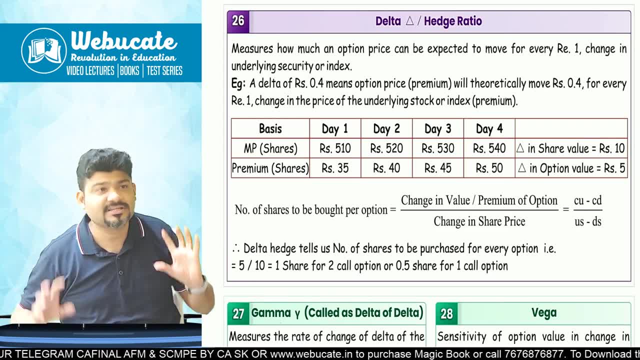 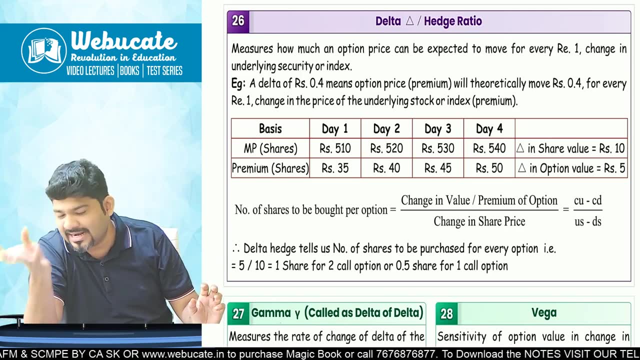 if I buy options, it will result to be the same amount of profitability. So how many options should I bear? Should I purchase instead of purchasing the real shares? Because in real shares I will make a loss if it goes down, and that loss can go unlimited. 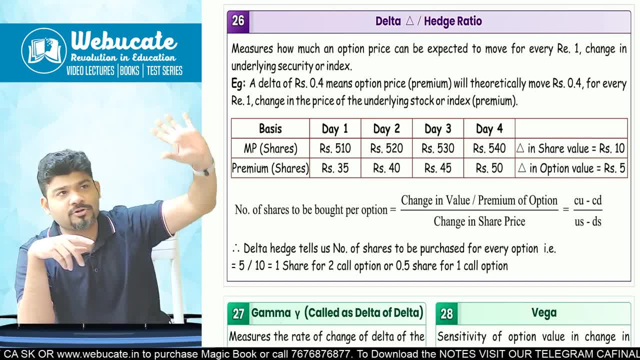 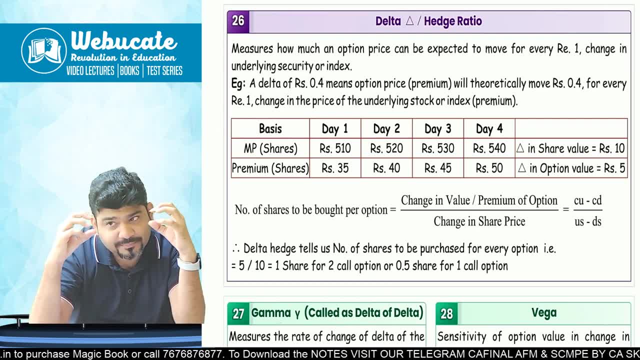 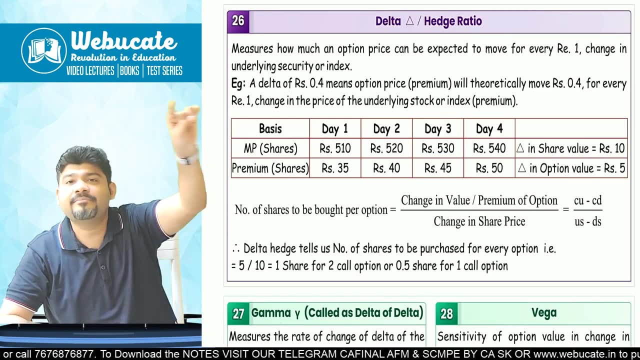 But in options I know at least that if I make profit, good, But if I make loss it is only going to be restricted to the premium amount, All is well. So what is that combination, Where instead of purchasing shares I can purchase equivalent number of options, is given by the delta or hedge ratio? 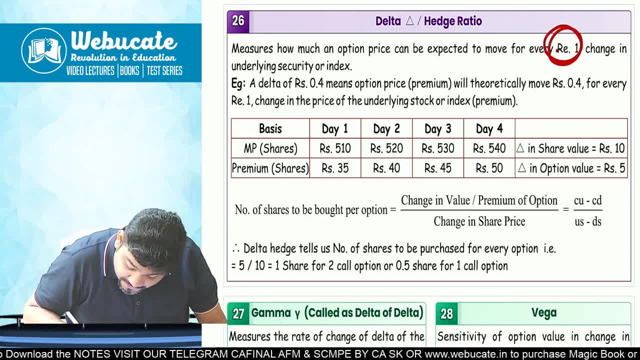 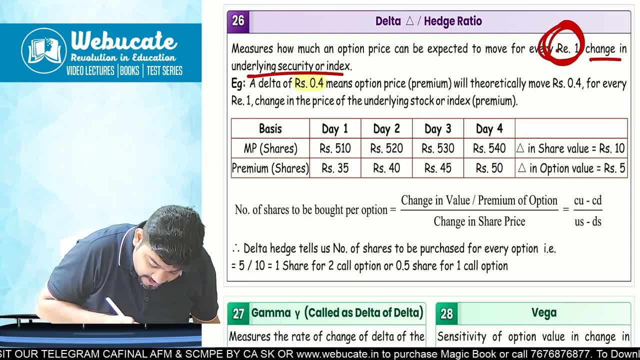 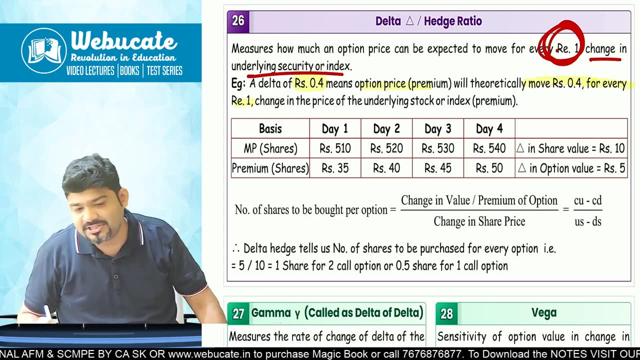 measures how much option price can be expected to move for every one rupee change in underlying security or index to a delta of zero point four means option price will theoretically move zero point four for every one rupee change change in the price of underlying stock and that will tell us how many shares can. 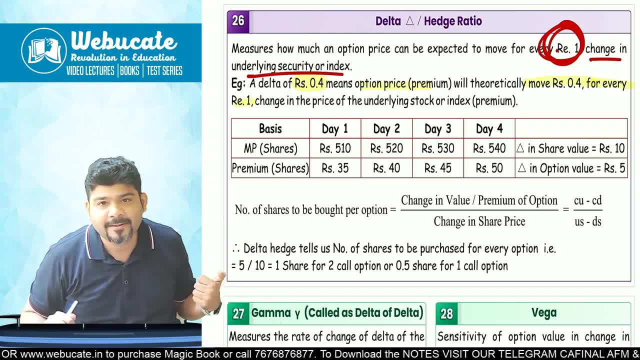 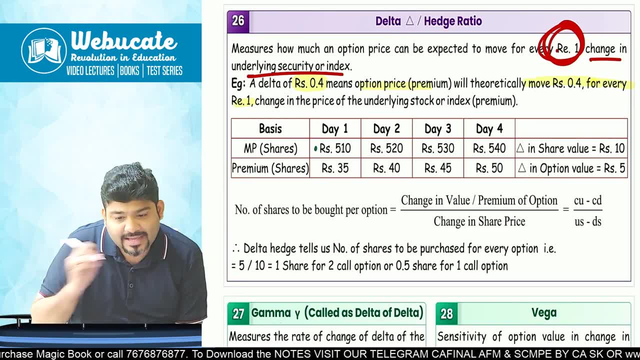 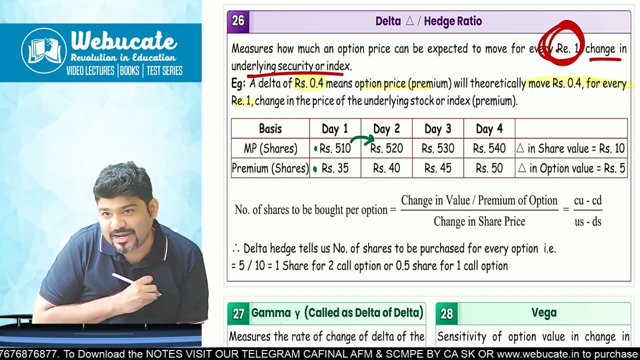 be bought instead of options, or vice versa. Let's take this example. You will be more clear Now. first, market price of shares is five hundred and ten and the premium of this is thirty five. Now pay attention When the market goes from five hundred and ten to five twenty. 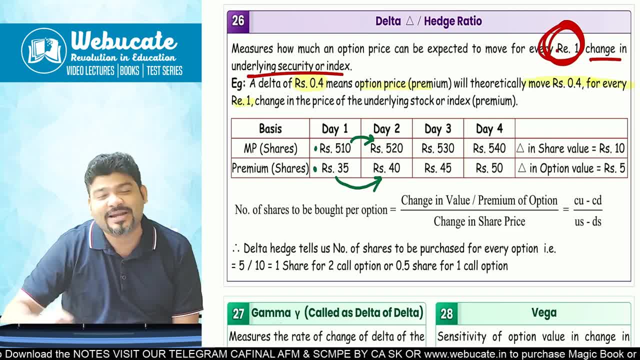 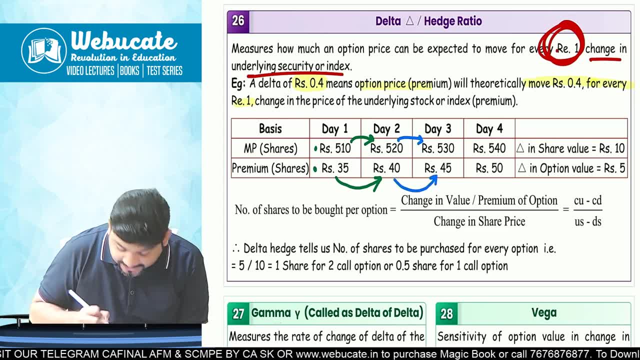 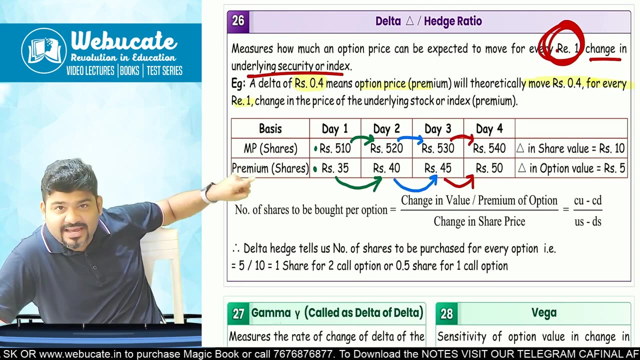 the premium goes from thirty five to forty. from five twenty to five thirty. the premium goes from forty to forty five, Gotcha, And then finally, from five thirty to five forty. it goes from forty five to fifty. So what is happening? on every ten rupee increase in shares. 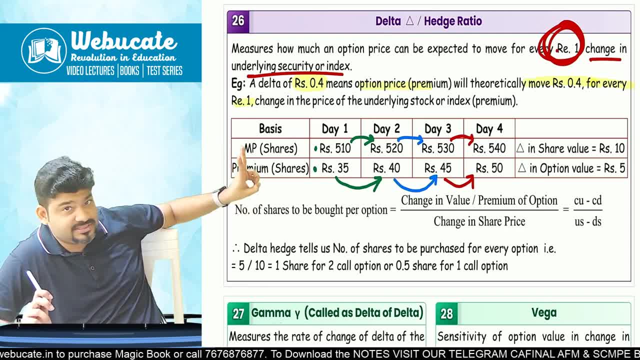 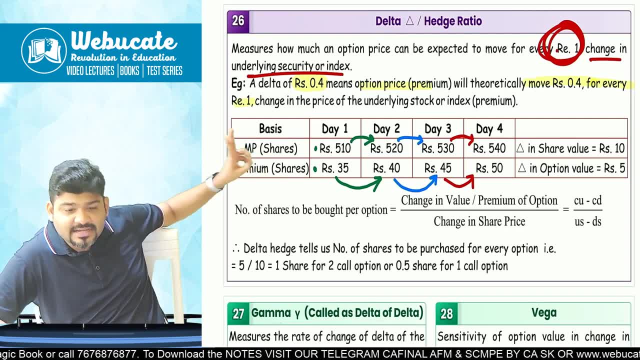 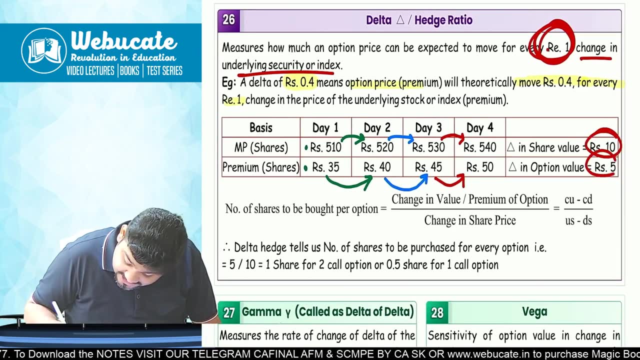 The premium is increasing by five rupees. Did you observe this? I'm sure you observed this on ten rupees increase in market price of shares. Five rupees is the increase in premium. so change in share value is then change in option value is five. 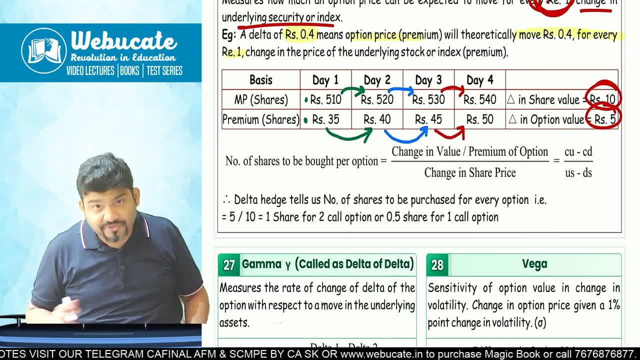 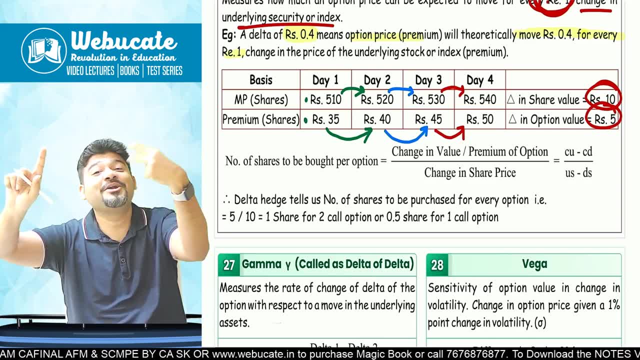 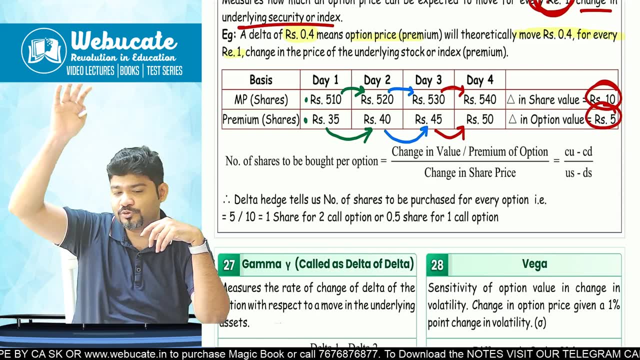 So this tells us that for every two option we can buy one share, or for every one share we can buy two call options. So now, if suppose you buy one share, the market goes from five hundred and ten share goes up to five twenty. 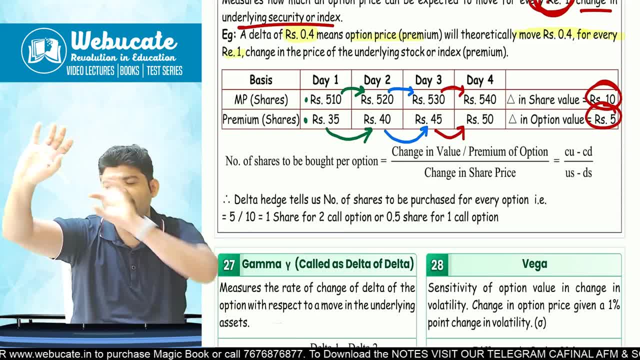 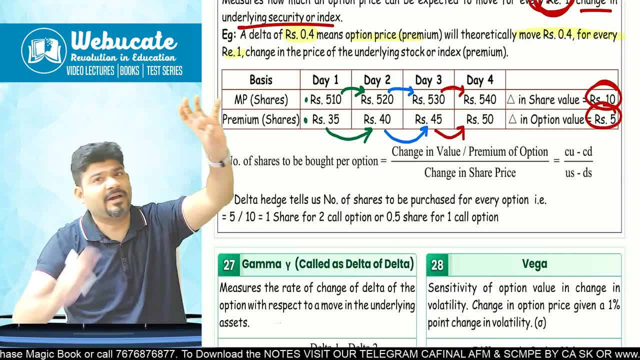 So ten rupees profit you are making. instead of buying that share. you can buy a call option when the market goes from five hundred and ten to five twenty. If premium increases by five rupees, you have two option. So automatically now premium will increase by ten rupees instead of buying the share. 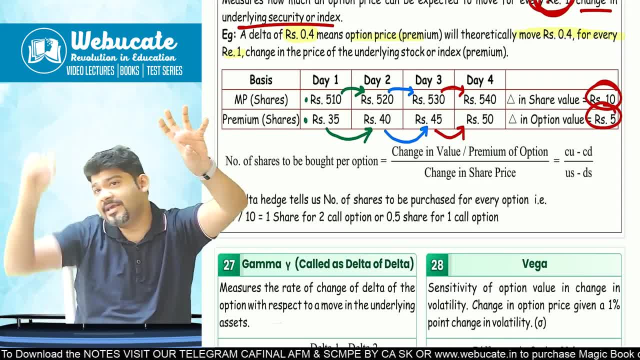 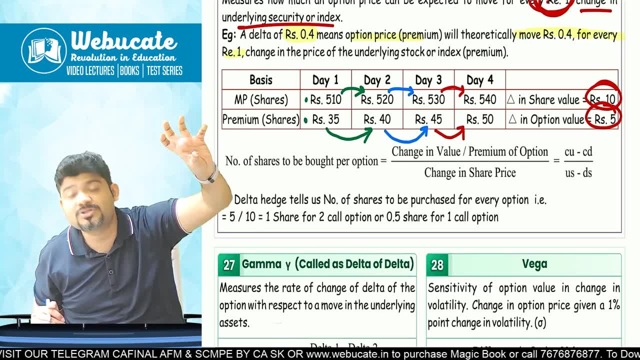 I have bought the call option because that saves me from the downfall. also because if the market goes from five hundred to four hundred there will be a hundred rupees loss in shares, But in options it is only going to be till the amount. 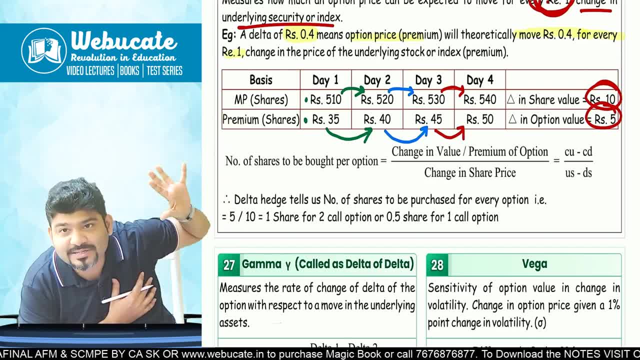 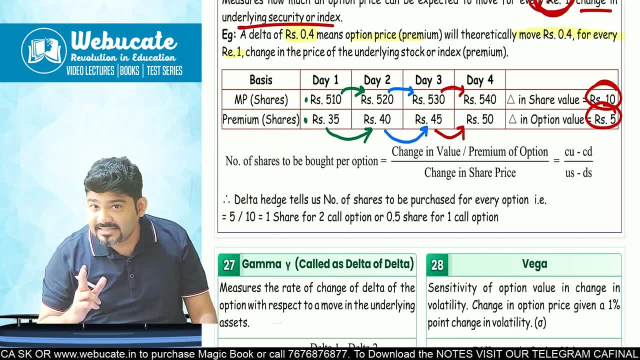 of the premium, which could be twenty to forty rupees, And that is where delta hedging is used by a lot of companies to secure them. Got it, guys? Did you get it? So that's what delta hedging means, or that's what delta hedge ratio means. 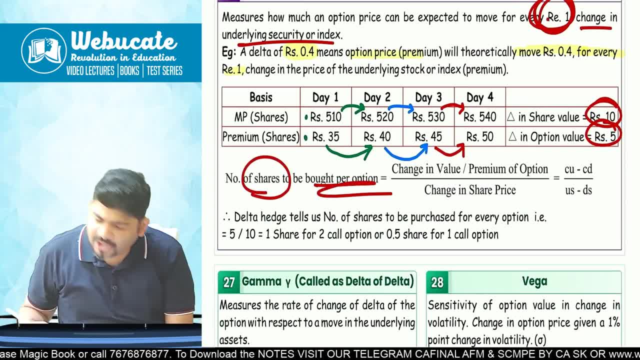 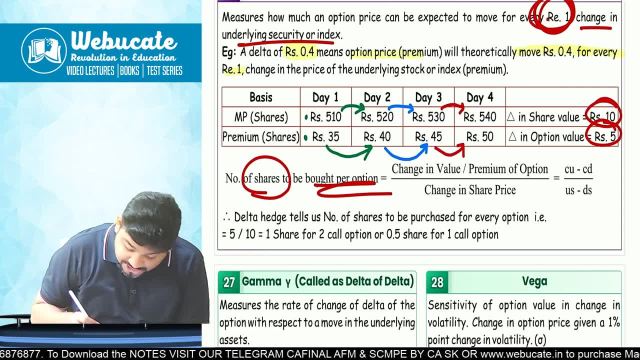 Number of shares to be bought per option or number of option to be bought per share. But here the formula is given in this way that number of shares to be bought per option, So change in value or premium of option, So which is a change in premium, is five, change in share price is ten. 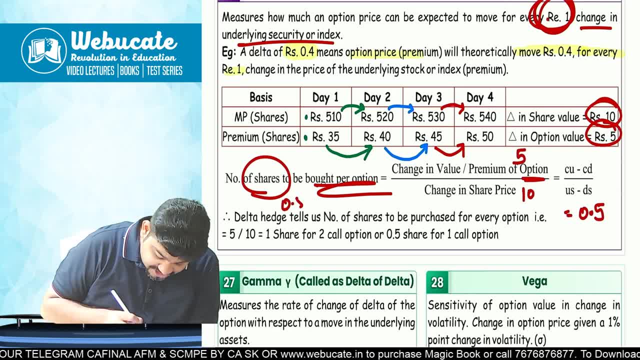 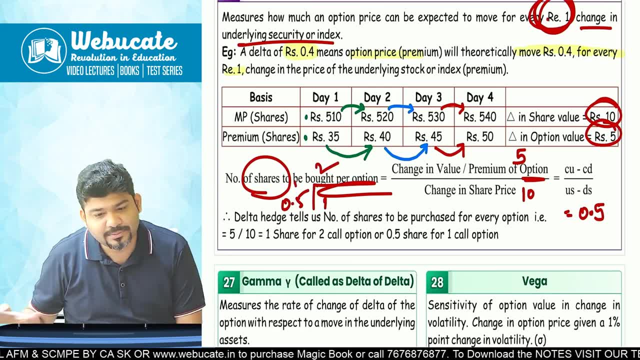 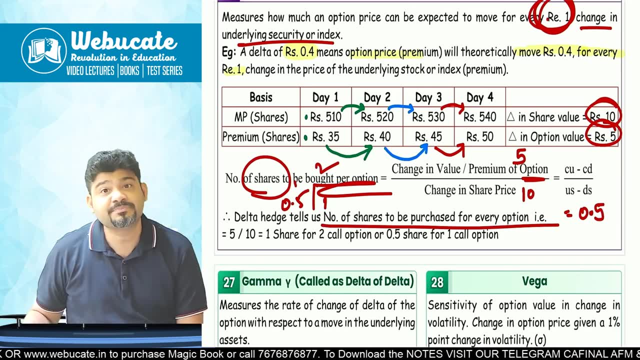 So it is zero point five. So point five shares For one option. So basically, one share for two options. Simple Delta hedge tells us the number of shares to be purchased for every option, or number of options to be purchased per share. Got it guys? What is the formula? 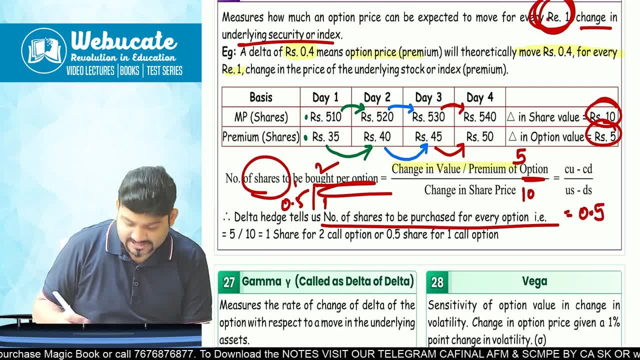 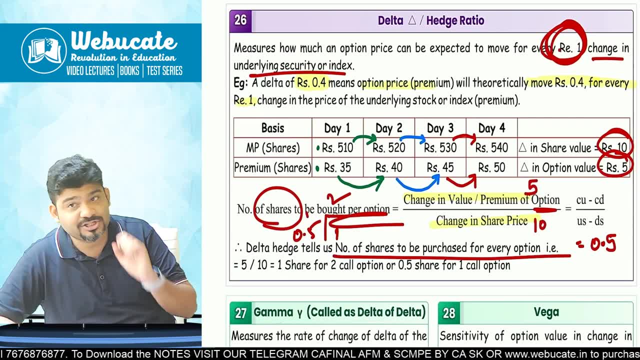 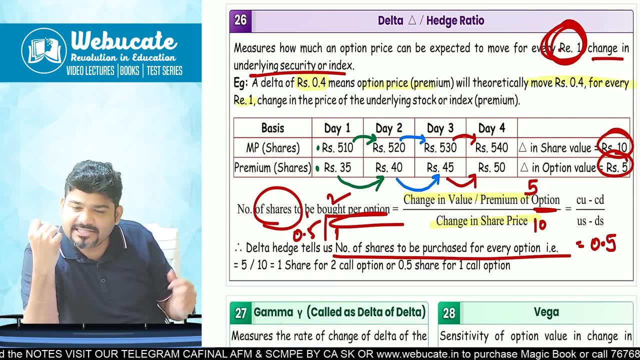 Change in value of premium of option upon change in value of share price. Gotcha, So that is what is called as delta or hedge ratio. Very important: Instead of buying shares, I can buy How much options So that the change in share price or increase in share price will be offset by an equivalent. 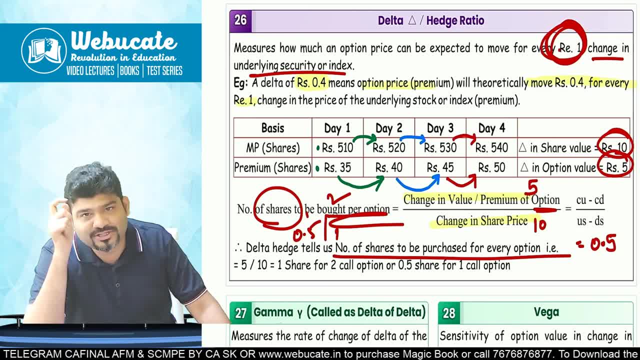 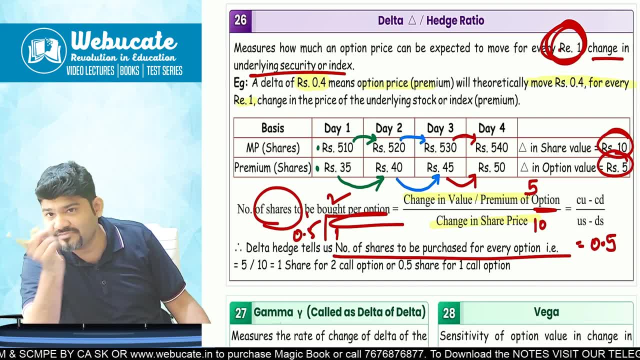 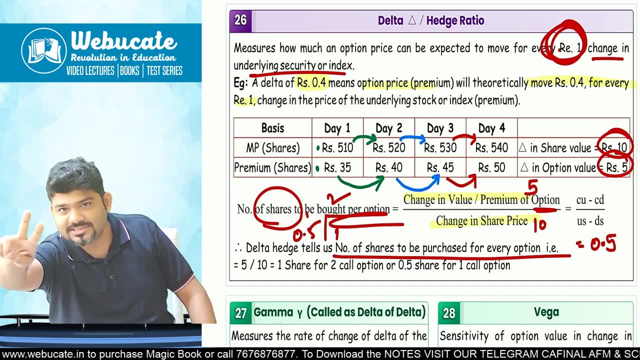 options is what is called as the delta change or hedge ratio. Delta hedge ratio. How do you get that? change in value of premium upon change in value of share? Five upon ten point five share per option or per share, Two options. Then the same thing will continue. 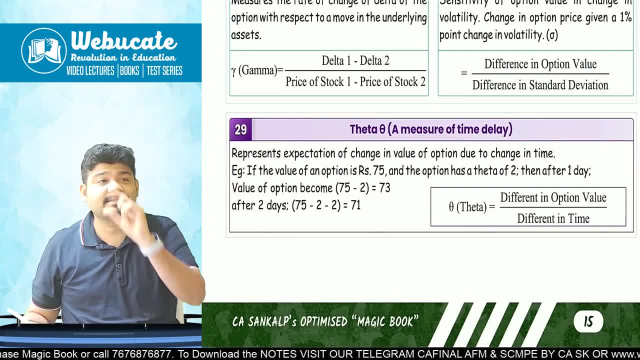 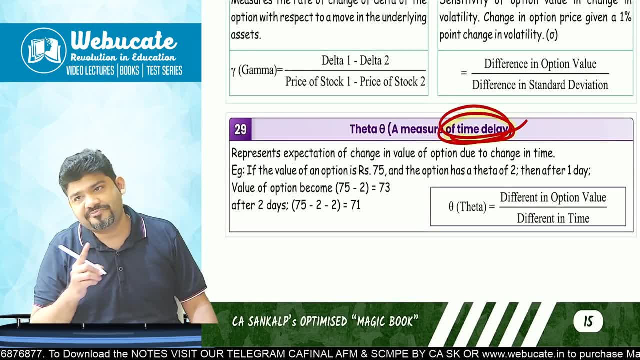 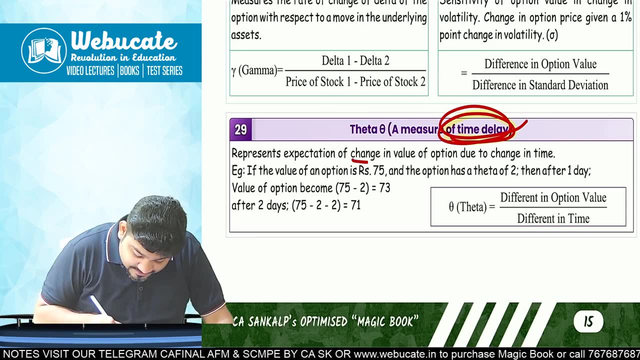 Then there is something called as theta. Theta tells us that how much the change happens on account of time delay, on account of time delay, how much value of option changes on account of time delay, What is value of option premium? So represents expectation of change in value of option. 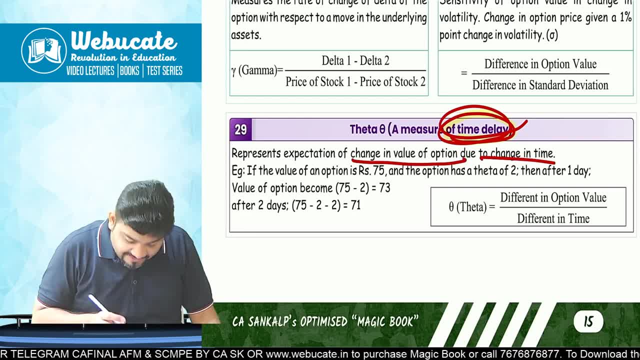 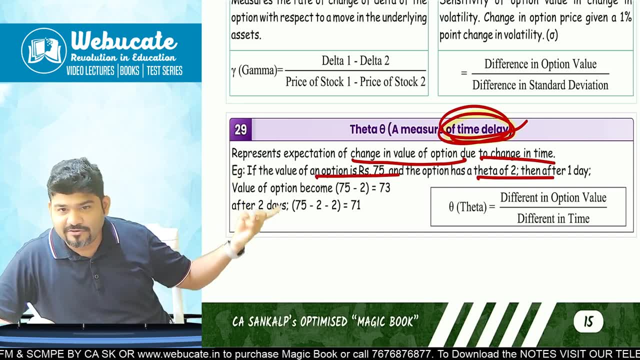 What is value of option premium due to change in time? If the value of an option is seventy five and the option is a theta of two, then after one day, after one day, the value of option will become seventy five, Seventy three, because the theta, which is the time delay. 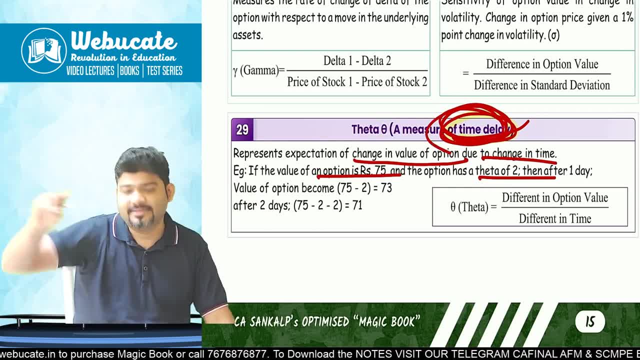 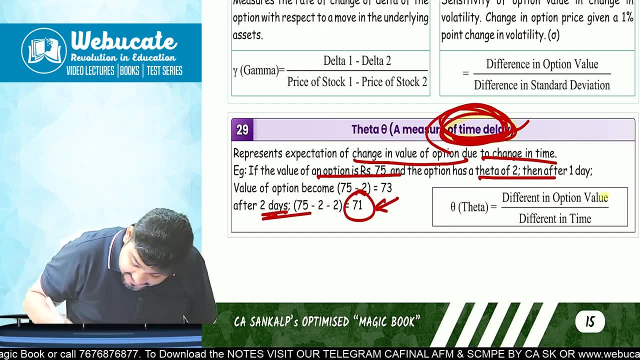 Is theta is to next day again, the price will go down by two rupees. Seventy five to seventy three. Seventy three to seventy one. Theta is difference in option value upon difference in time. Difference in option value upon difference in time. 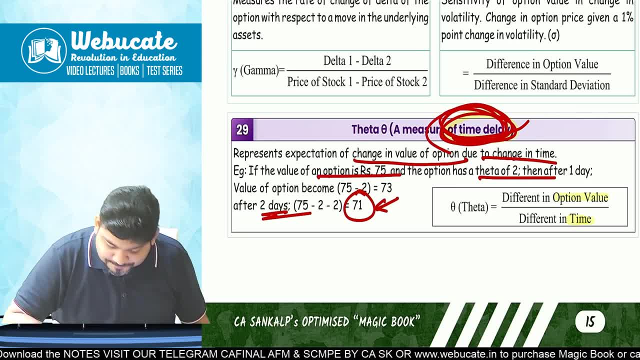 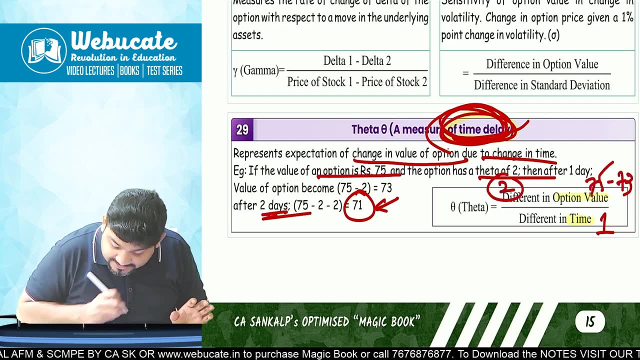 Everybody, Yes, sir. So So If my Time goes, say one day has gone and option value has decreased from seventy five to seventy three. so two rupees option value, degrees, one rupees Time decrease two by one. 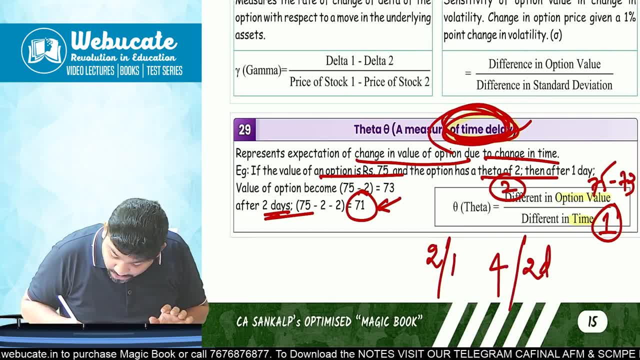 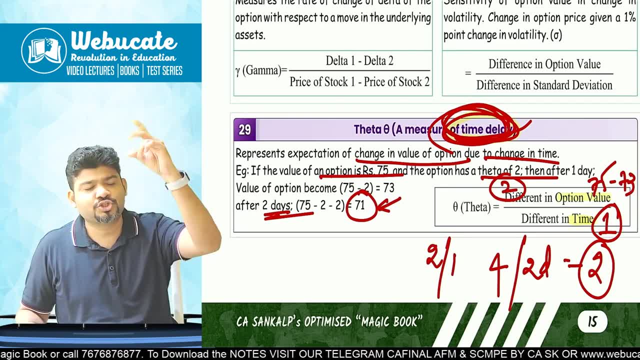 OK, for two days four rupees has decreased, So two basically becomes your theta. So now you know, for every one day increase, theta is two. So for every one day increase two rupees, the value of premium will go down. 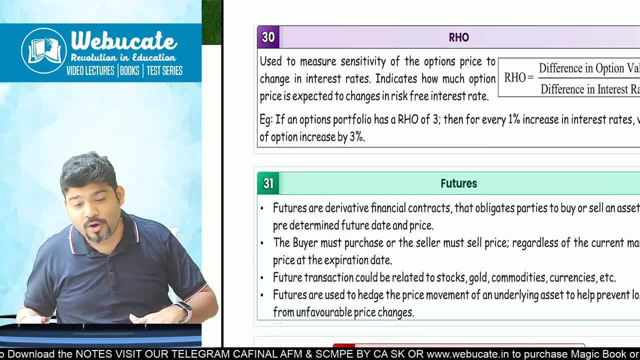 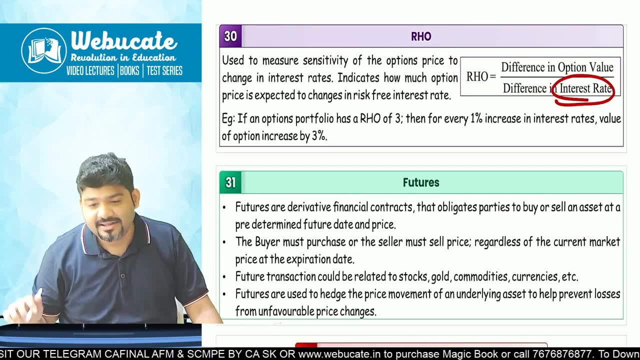 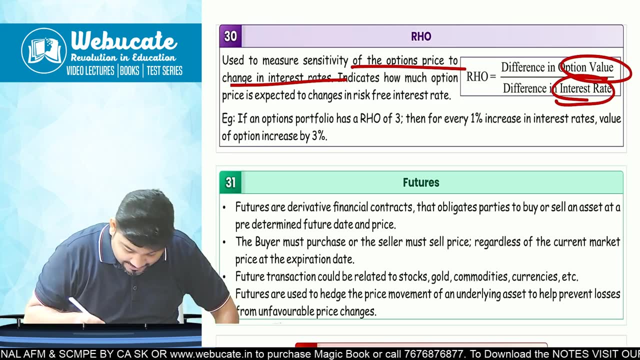 So that was theta time. Then there is row or HO that will be based on interest rates. for every change in interest rate, What is the change in option Premium measures? the sensitivity of option price to change in interest rate indicates how much price expected to change in risk free rate. 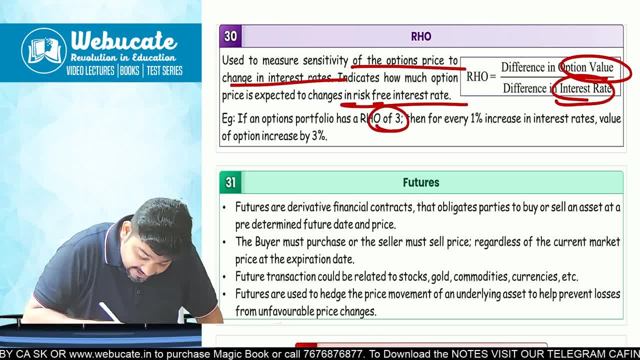 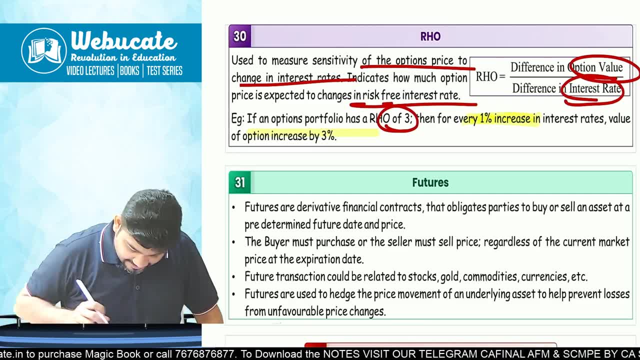 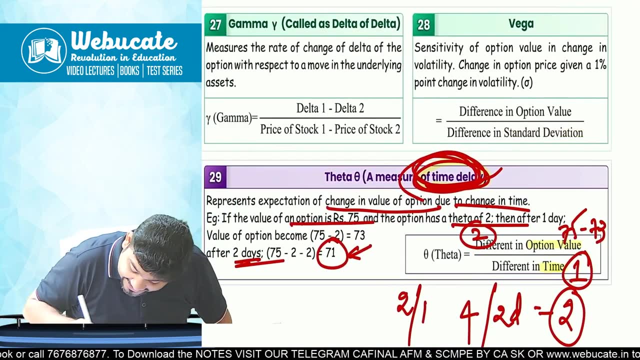 So if an options portfolio has a row of three, then for every one percent increase in interest rates, value of option will increase by three percent. Simple Then. So row is done, Theta is done, then there is Vega. Vega means change in standard deviation and the change in option value. 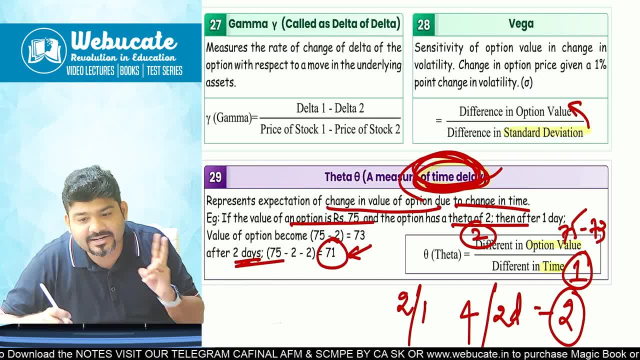 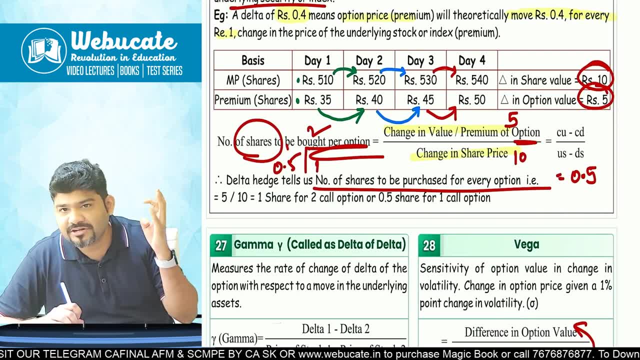 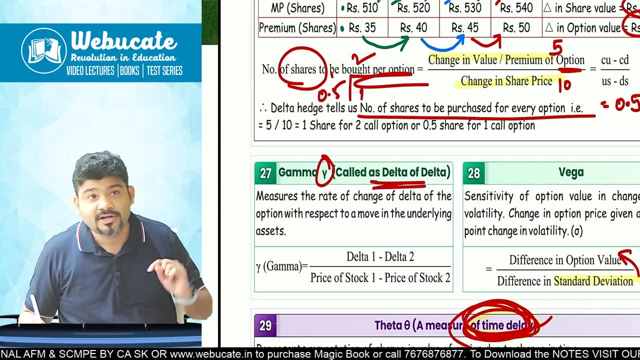 So T, theta row, interest rates, Vega, standard deviation, delta pure, pure change in option, premium upon change in share price And then last is called as the gamma delta of delta. What is the change in delta as regards the stock price of the share is called as the gamma measures. 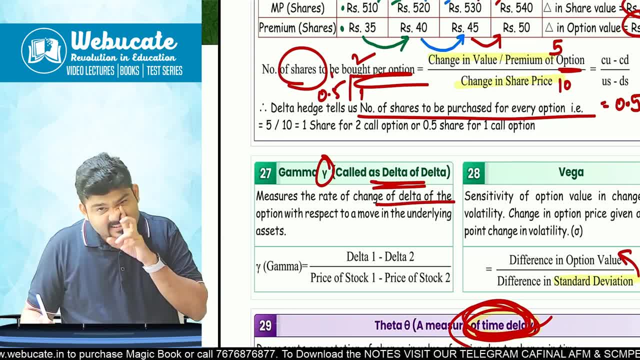 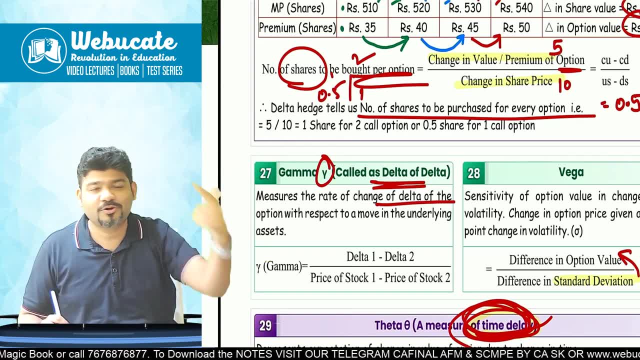 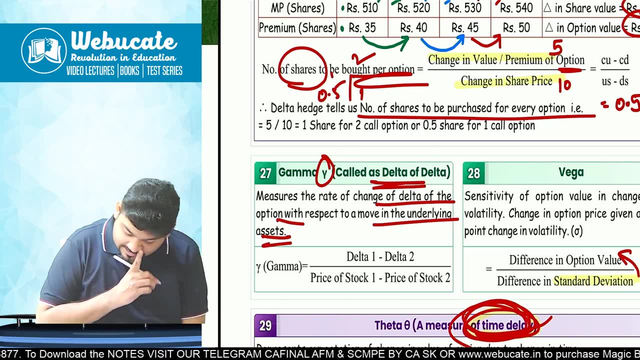 The rate of change of delta. my friend Is a delta trader. he uses only these things which are given to you and you know Marx's trades of stock, so measures the rate of change of delta of the option with respect to a move in the underlying assets. 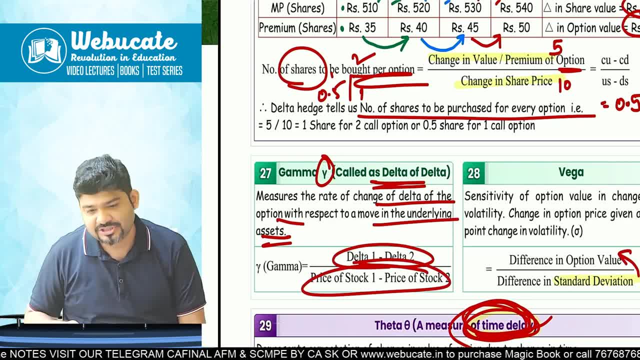 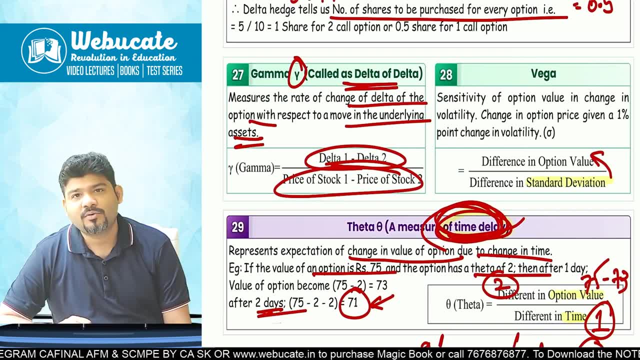 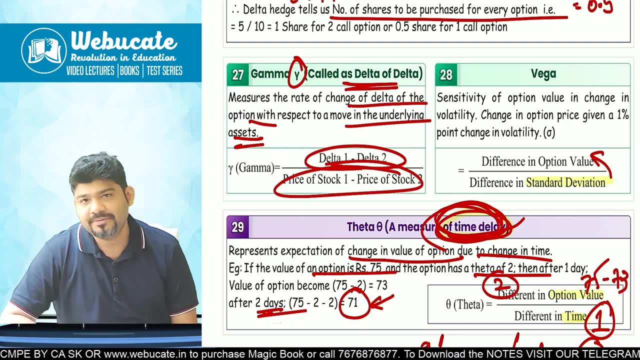 So change of delta upon change in price of shares. So that's how the whole system works. Delta ratio Gamma Vega. What is Vega? Change in standard deviation and the resulting change in options: Premium, theta time options, Premium row interest rates. change in option premium. 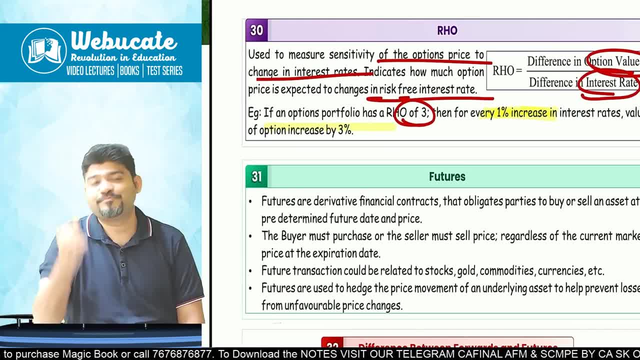 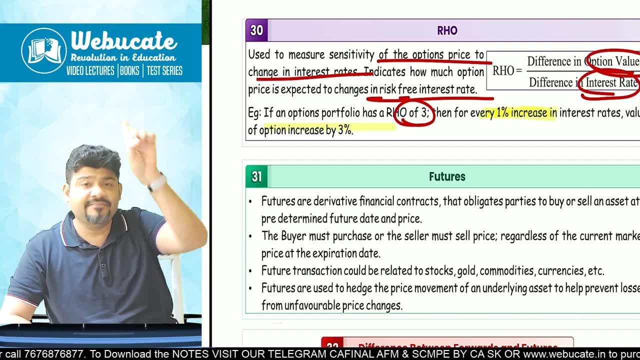 And with this we complete the whole of options theory. How was it? Did you understand everything? Yes, Now only black and shows and real options are left, which I will do after doing the future. So now we are basically going to start with the next derivative. 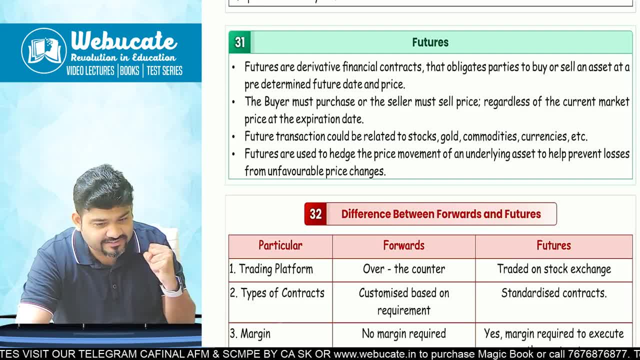 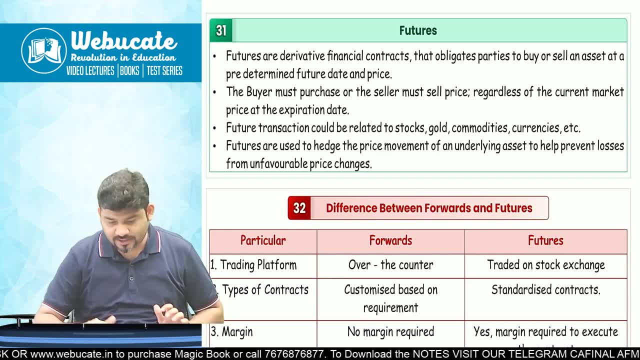 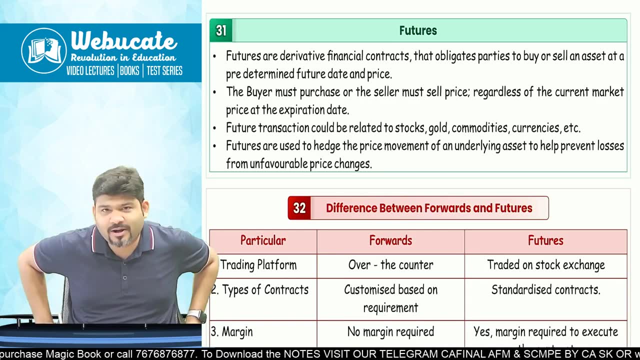 And that is we are now going to start with the next derivative, And that is the future. OK, futures is another derivative instrument which is used by the, by the speculators, everybody whoever wants it. But now, in case of options, there was a scene of right and obligation. 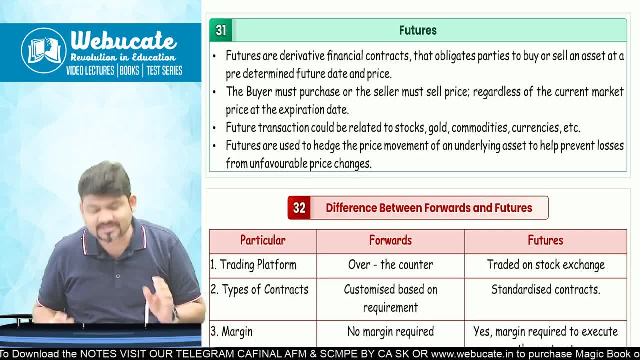 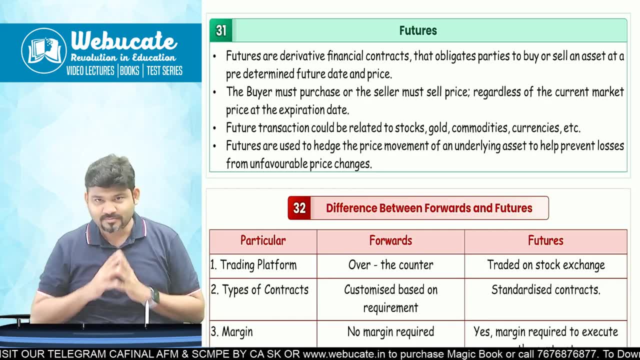 In futures. it is not going to be the case. in futures. There is a compulsion that you have to square off the trade. So what does that mean? I'll tell you. So in futures, again, you are going to do the same thing. 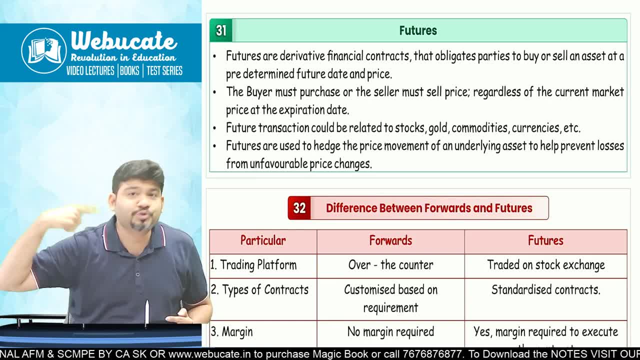 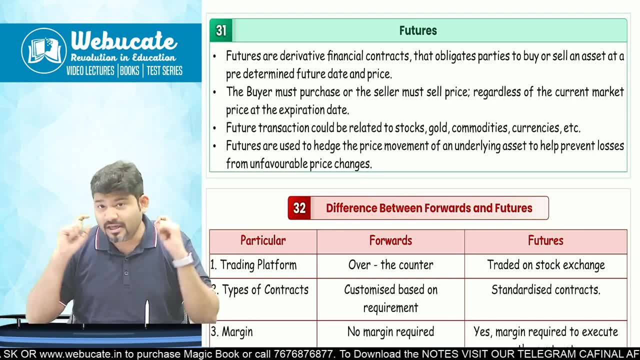 You are going to predict, according to you, according to your analysis, whether the market is going to go up or the market is going to go down here. If whatever you think actually happens, then you are going to make a huge profit. But if it goes against what you had thought, if it goes, 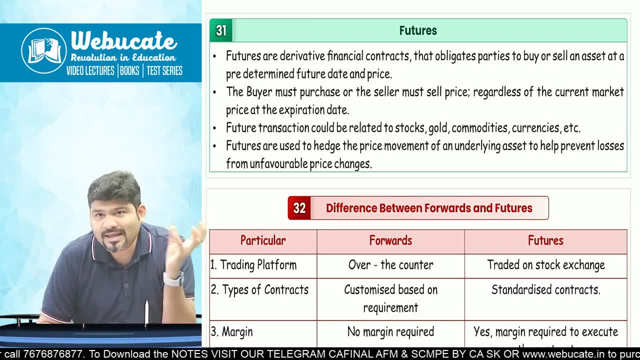 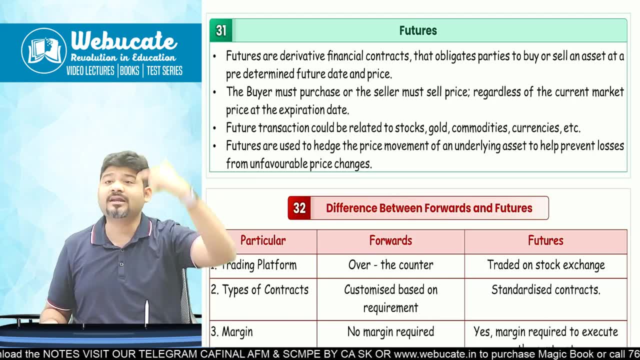 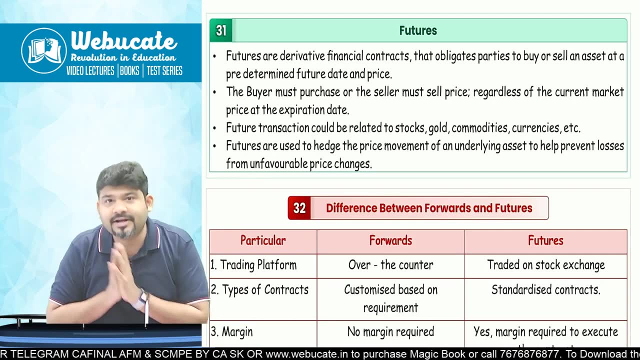 opposite of what you were planning or of what you had analyzed, then in that case you will also lose a big amount. Right? So you're, the profit is unlimited. The loss is also unlimited in case of option buying. The profit is unlimited, but the loss is limited, because if you do not exercise, 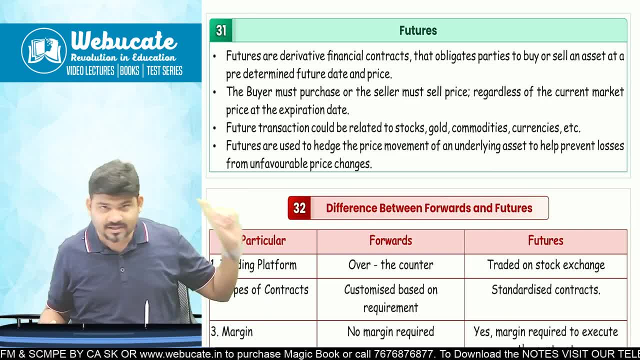 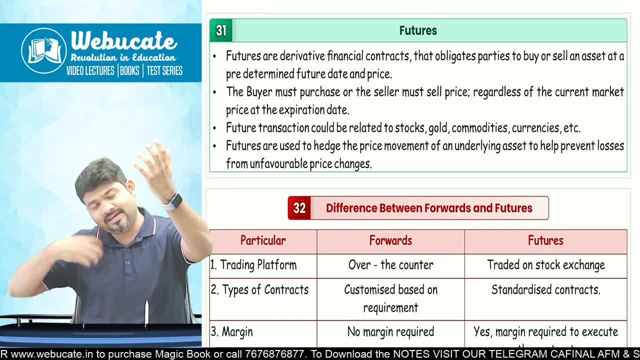 then that premium amount is your loss. So that's still OK, But you're, it is not going to be the case. Second thing: in futures, whatever gain that you are making, there is somebody who is making that much loss, or whatever loss you are making. 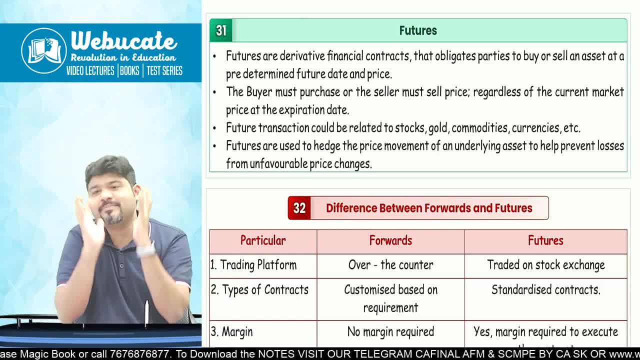 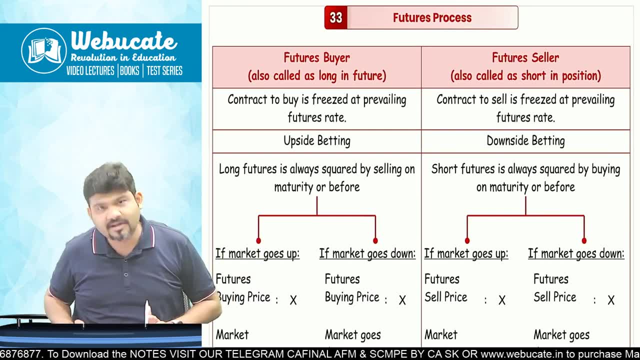 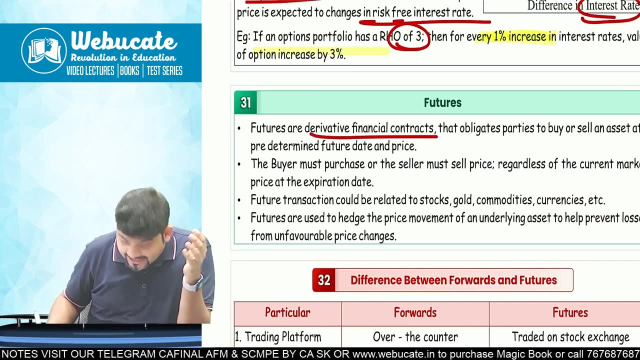 There is somebody who is making that much amount of gain. So that basically characterizes futures in detail. How does it work? The whole futures process is given here, which I will discuss with you. So first just have a quick read. Futures are derivative financial contracts that obligates parties. 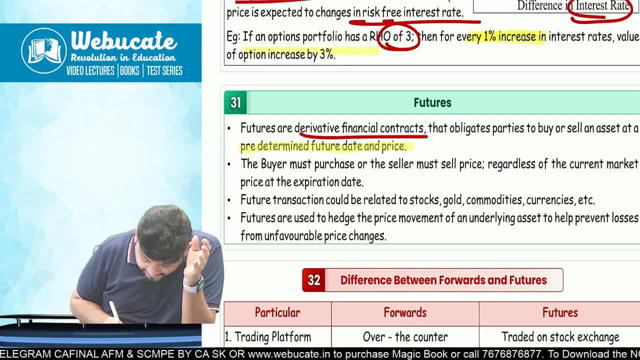 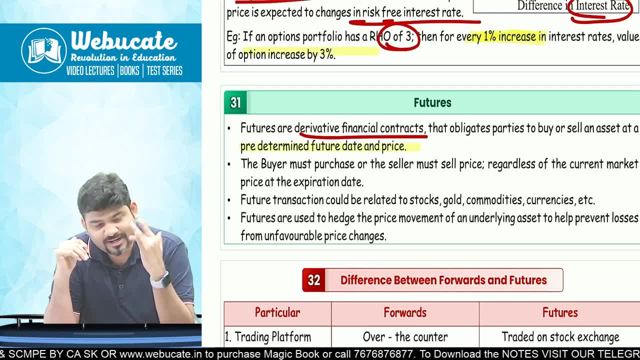 to buy or sell an asset at a predetermined future date and price. So you will priorly decide that what you are going to do One is buying futures, other is selling futures. One is buying futures and one is selling futures. How the process will work, I'll explain that. 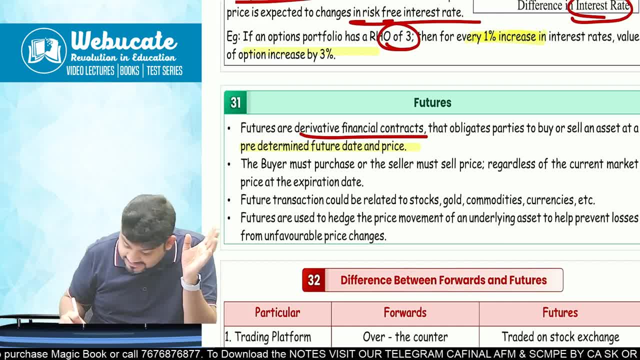 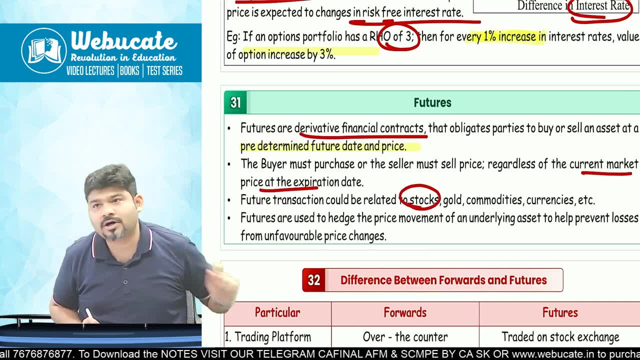 Don't worry. Then the buyer must purchase or seller must sell, regardless of the current price at the expiration date. Future transaction could be related to stocks, So you can have a future futures transaction in stocks in gold, in commodities, in currencies, etc. 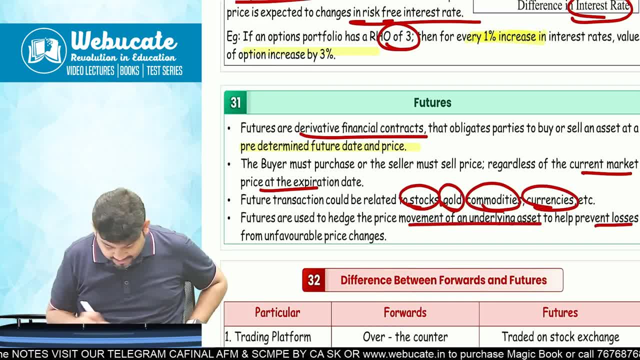 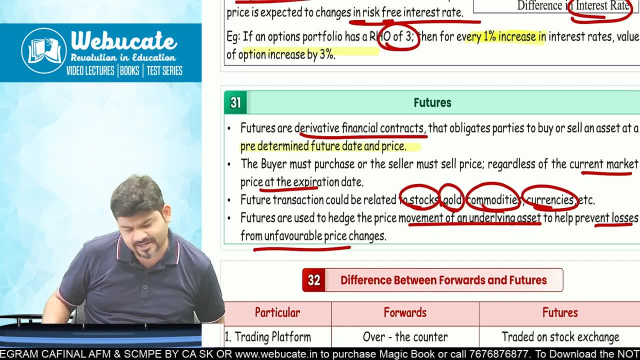 They are used to hedge the price moment of an underlying asset to help prevent losses from an unfavorable price chain. So I told you this is also used by hedgers, speculators, arbitraisers alike. Now, what is the difference between the forward and futures? 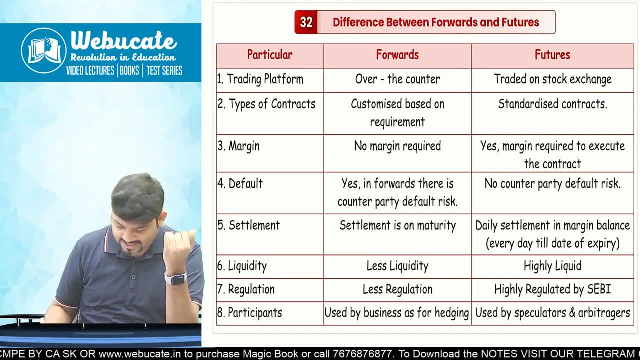 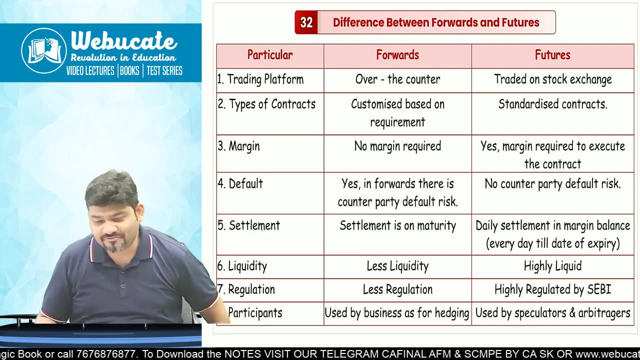 So let's have a quick discussion. Two, three points can come in the examination. Let us understand them. One forward is OTC over the counter. There is one question in ICI BOS app wherein they have given this: what forwards? what are forwards? 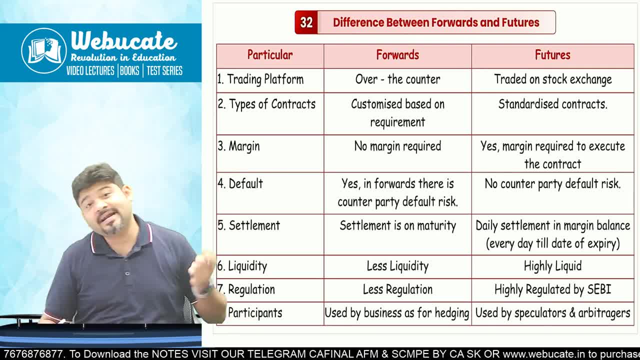 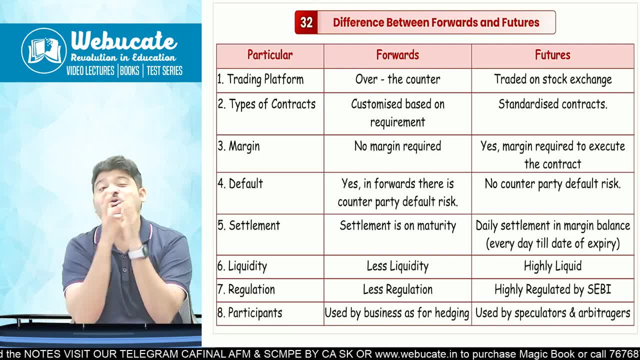 They are over the counter, whereas futures are traded on stock exchange. In case of forward transaction, there is no SEBI or a stock market, which is prevalent. You will go to the bank and you will tell the bank: bank, I want a forward or authorized dealer. 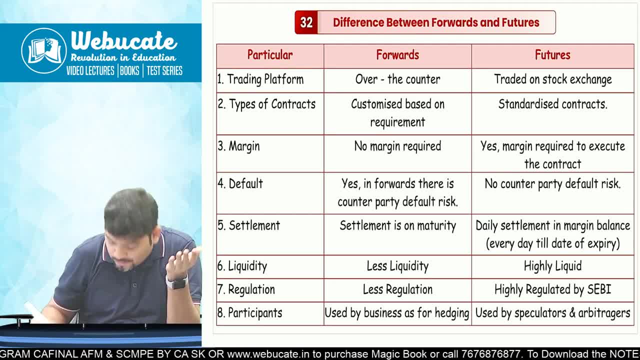 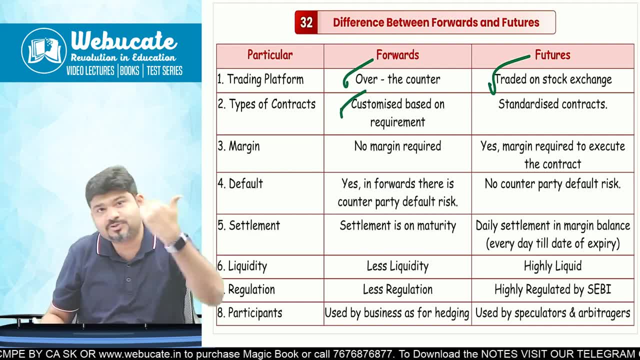 You, I want the forward, That person will give you the forwards and that's how it works. So it is over the counter. Other is traded on stock exchange type of contract. Here you can customize it because you are face to face, over the counter with the banker. 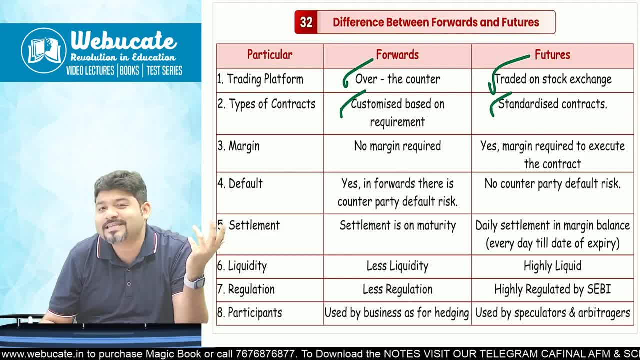 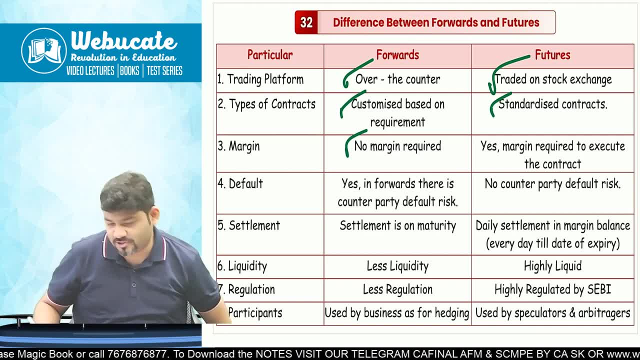 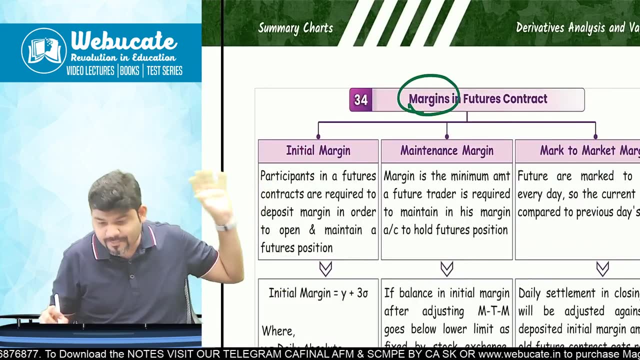 In case of futures, it is a standardized contract because SEBI is intermediately involved. Then margin: no margin is required in case of forward, But in futures the margin requirement is there. So what is this margin requirement? So we have a typical 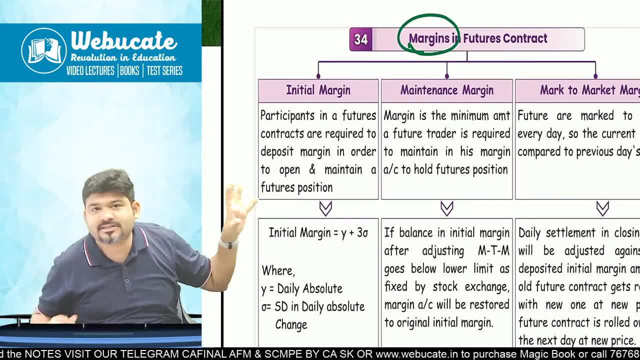 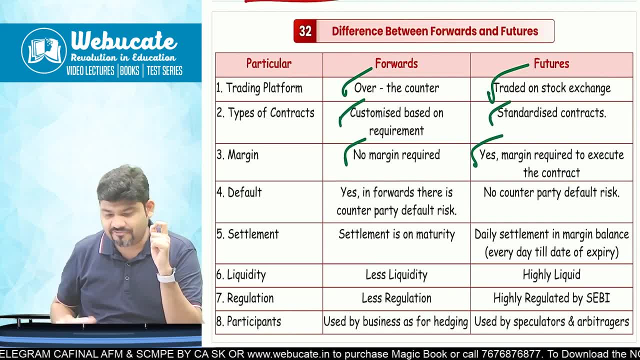 separate- you can say concept and making you understand what is going to be the margins in futures contract. Then there is a default. In case of forwards there is a high chance of a default. Yes, in forward there is a counterparty. counterparty default is because I will go to the bank and say: bank, I will come after three months, please freeze my date and rate. Suppose if I don't come up after three months, then because there is no margin requirement here and I don't come. 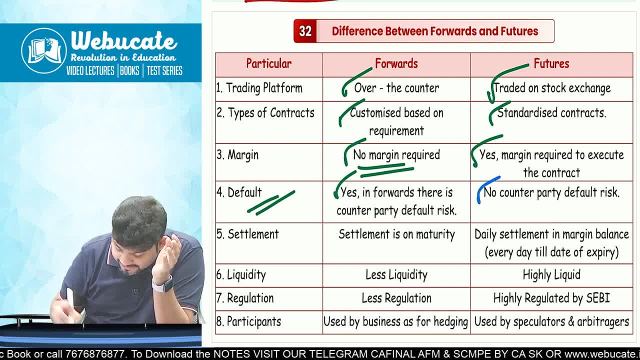 then I will default. but it is not going to be possible in case of futures because the margins requirement is there And if any default is there, then the amount will be deducted from the margin account. Next settlement is on maturity. Your daily settlement is possible. 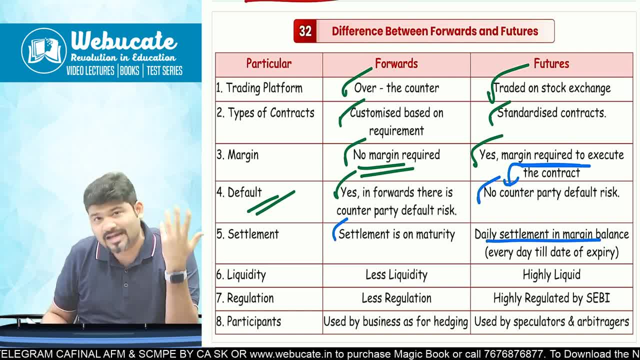 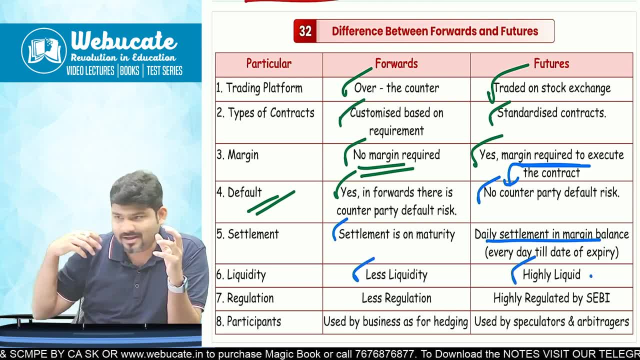 Any time, any second you want to settle, it is done through the stock exchange. That's possible. Here the liquidity is less. Here it is highly liquid. Why highly liquid? Because whenever you want to sell, you can sell at any point in time. 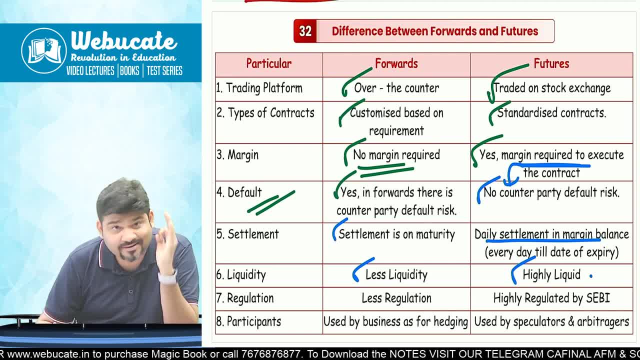 In case of forwards, a specific date and rate is fixed. You have to come on that date Only. you will get that rate. only Here it is volatile. OK, less regulation. but in case of forwards, but in case of futures. 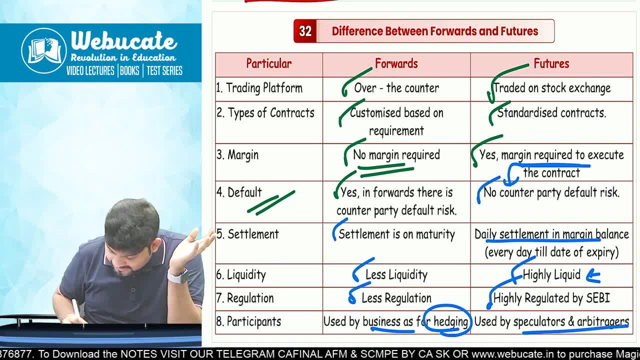 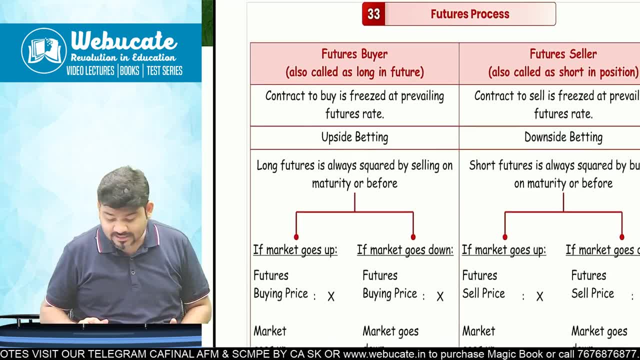 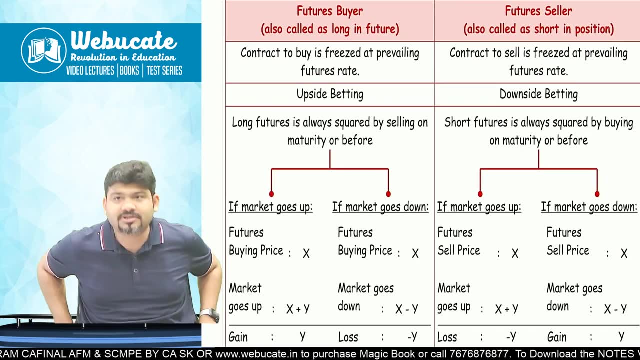 highly regulated by SEBI, used by business for hedging, used by speculators, arbitrators and even hedgers as well. So this is the difference between the forwards and futures. Now let's understand the process of your futures. So one there is a future buyer and the other there is a future seller. 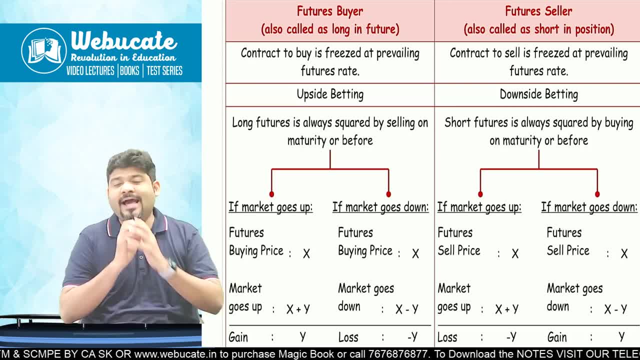 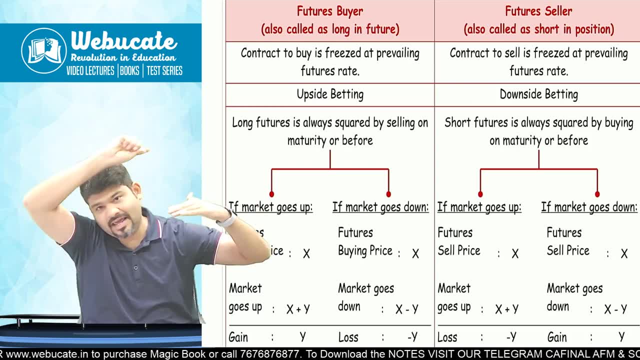 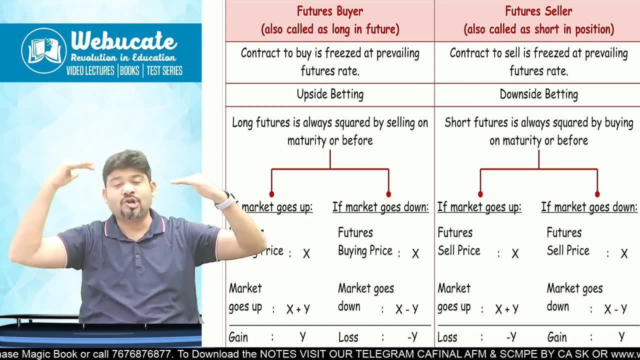 The one who buys the futures is called as longing futures. Now, if you have bought futures, you are expecting the market to go up, Like we had the right to call right, So right to buy call option. in the same way, here there is long and short. 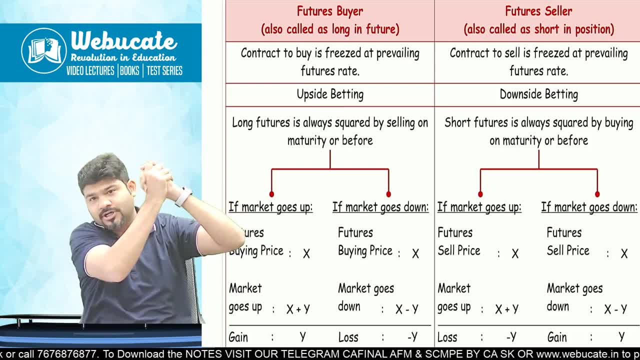 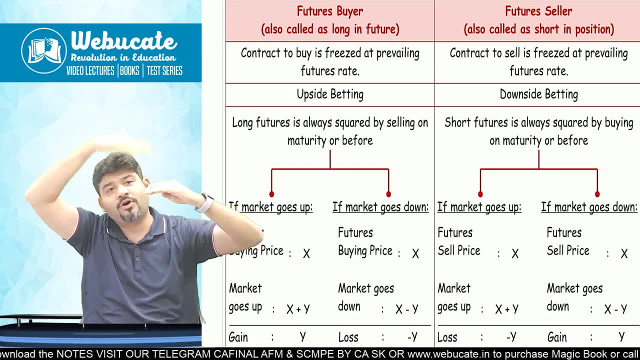 So suppose if you have done long futures means you have bought futures in future. now you will offset the transaction by selling the futures. So you want the market to go up. If you are expecting the market to go up, you will long futures. now market will go up. 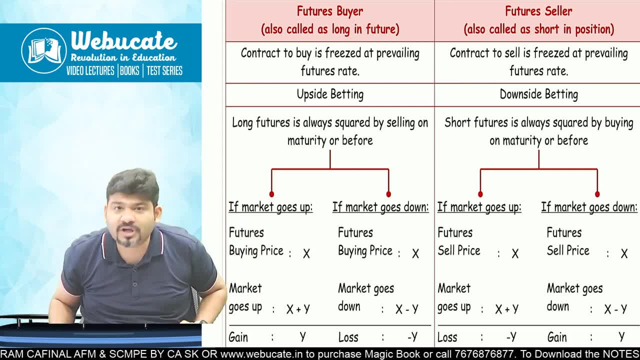 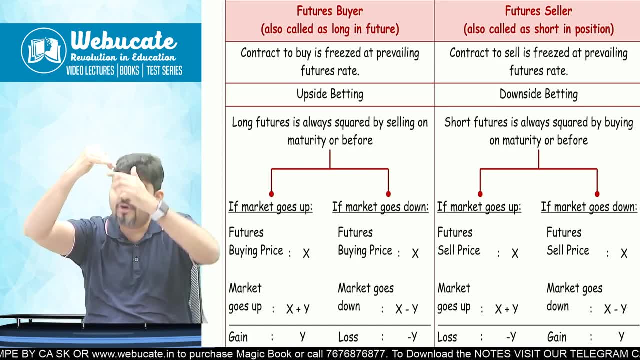 You will offset it by selling the futures. and vice versa in case of selling futures. Suppose if you sell futures at this rate now, you want the market to go down so that you can offset it by buying futures. So selling futures at high rate. let the market go down. 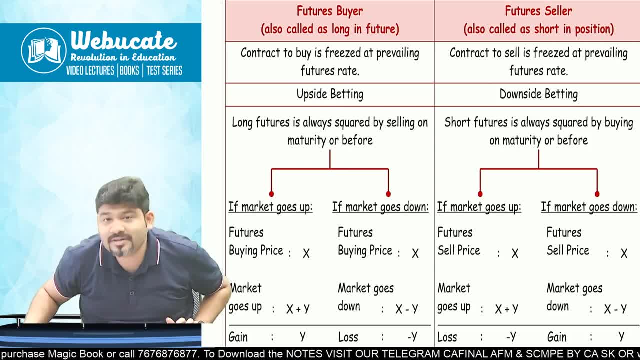 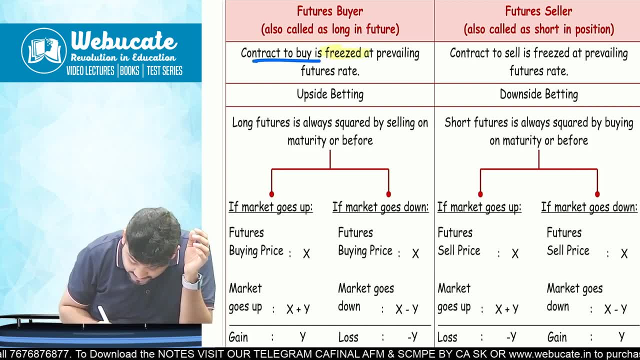 You will buy futures at a lower rate and the difference will be the profit. Are you clear? everyone Yes. So contract to buy is freeze At the prevailing future rate. This, basically, is your upside betting. You want the market to go up. 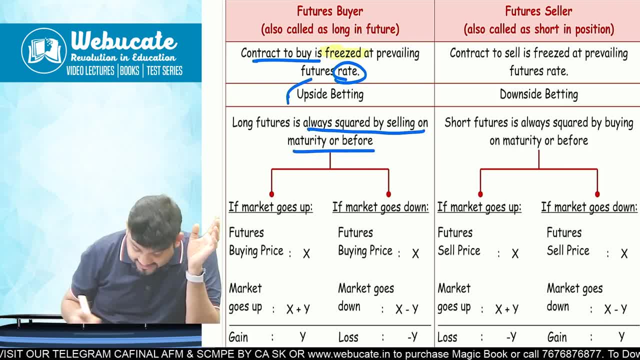 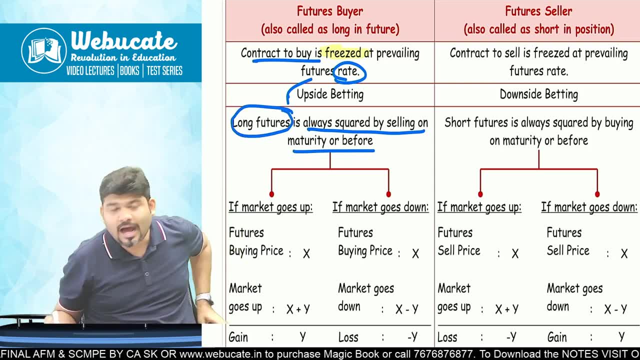 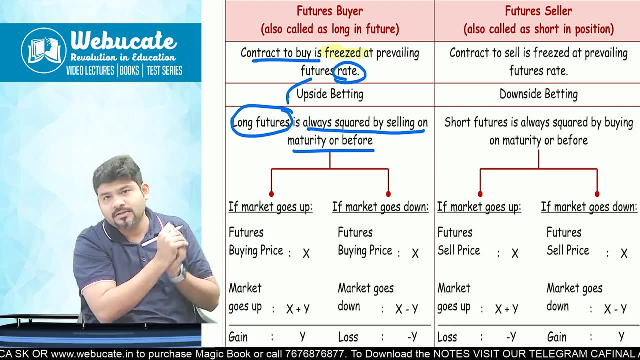 So long futures is always squared by selling on maturity or before. So what is it? It is called as long futures. How do you offset a long future? by selling it in future. So you want the market to go down. up So long futures. let the market go up, sell futures. 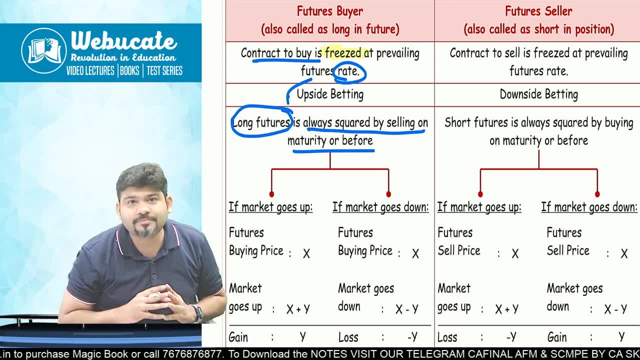 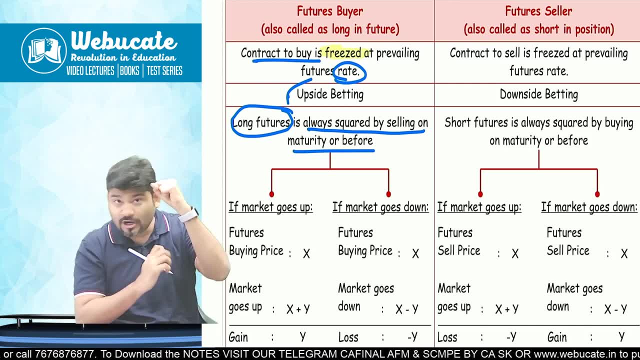 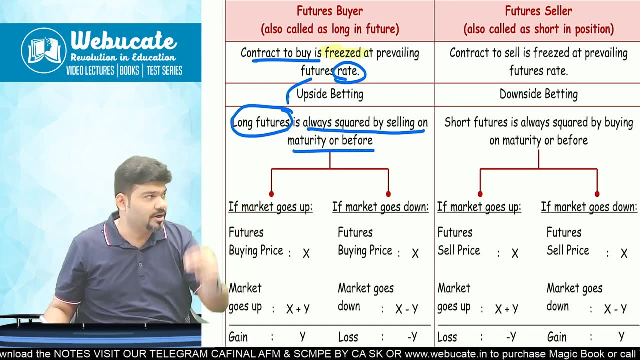 Close the deal at a profit, But you have long futures and if the market goes down you will have to sell futures for offsetting, because this is compulsory. The difference will be a loss and there is no right here. By default, there is an obligation. 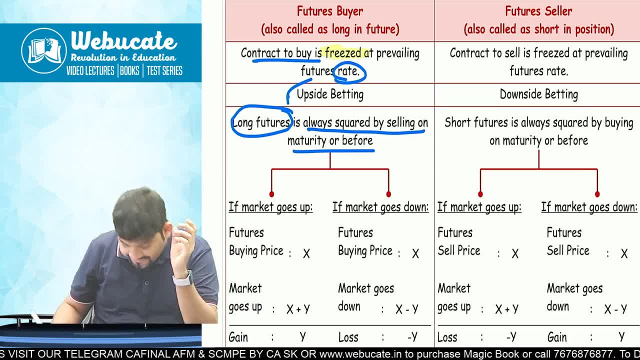 So you have to have to have to honor it. So if the market goes up, hello. if the market goes up, futures buying price. X Market goes up. So now it is X plus Y. The difference will be the gain, which is Y. 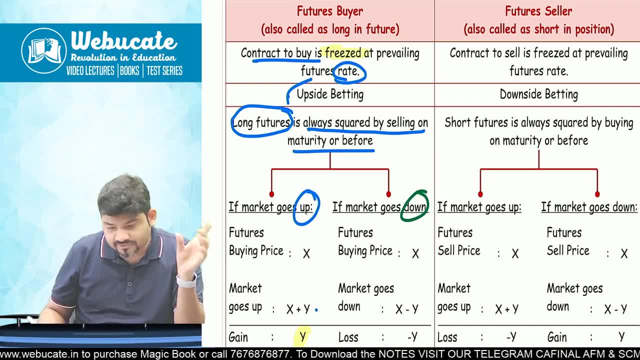 And in case of market goes down, futures buying price: X, Market goes down, X minus Y. That minus Y is your loss, Gotcha. everybody In the same way. there can also be in the same way. There can also be future seller, which is called as short, which is called as shorting. 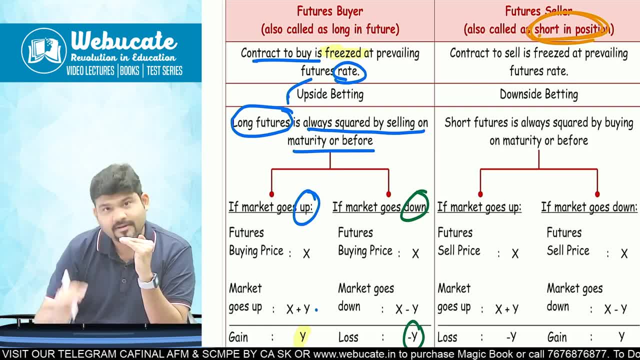 Now, if you have done Shorting? if you have done shorting now market goes down, You will have to offset the position by buying. So contract to sell is freezed at prevailing futures rate. Here you are doing a downside betting. 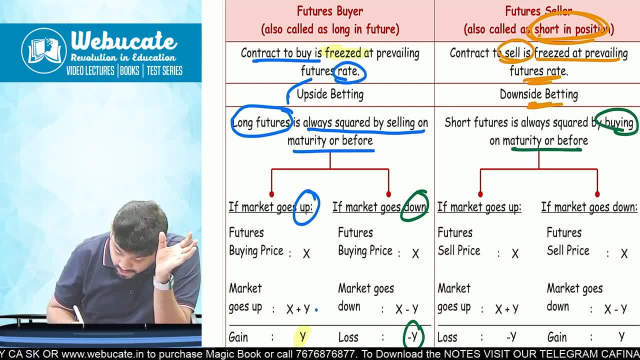 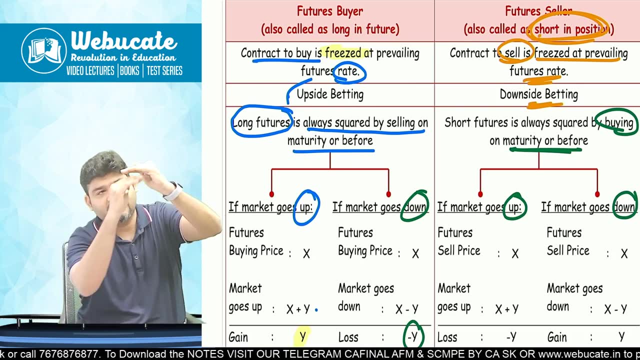 Short futures are always squared by buying on maturity or before. If the market goes up, if the market goes down, What will happen? So, future sellers? so you have shorted the futures. If the market goes down, you will buy. difference will be your profit. 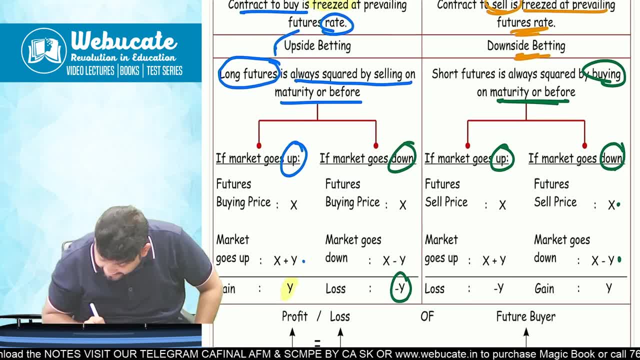 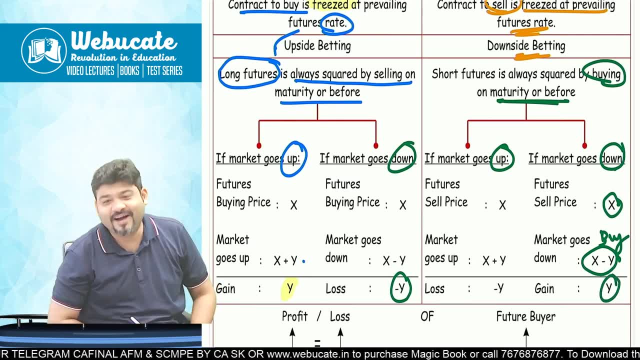 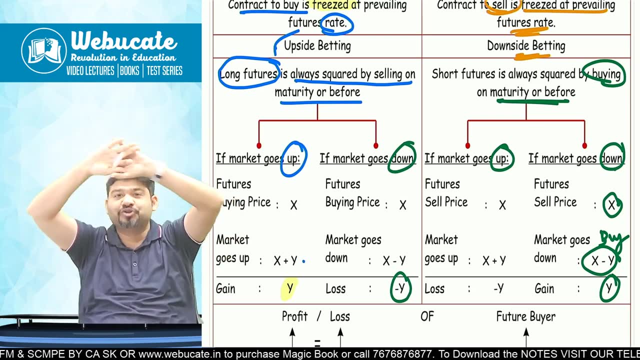 So here, if the market goes down, X, X minus Y, So this is your selling price. Market goes down, X minus Y will become your buying price. Gain will be Y, and vice versa if the market goes up. So as I told you that there will either be a huge loss or huge profit in futures, for sure. 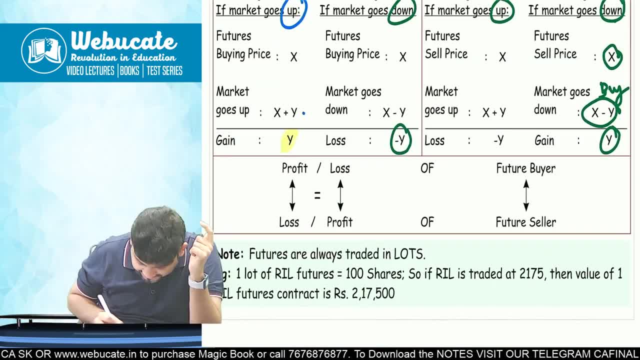 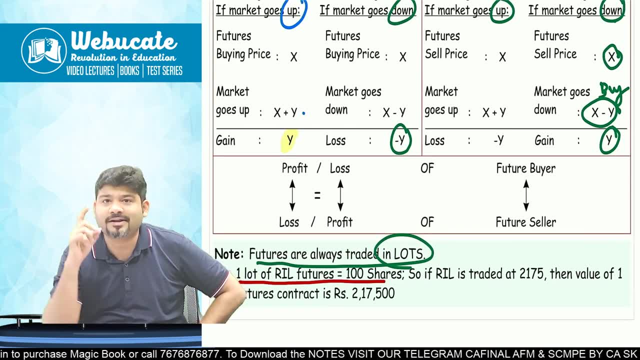 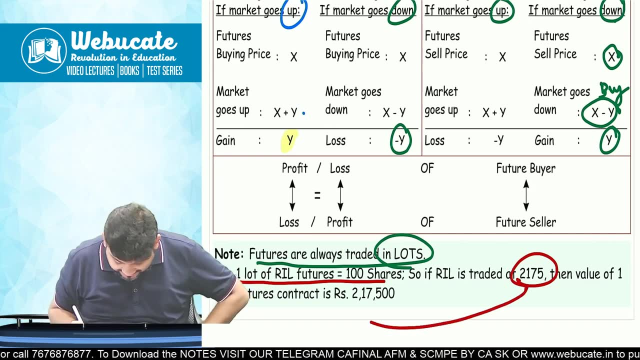 But this number is magnified because of one thing which is called, as futures are always traded in lots. One lot of RIL futures is minimum 100 shares. Yes, So if RIL is traded at 2175, then value of one lot will be 2175 into 100, which is 217,500. 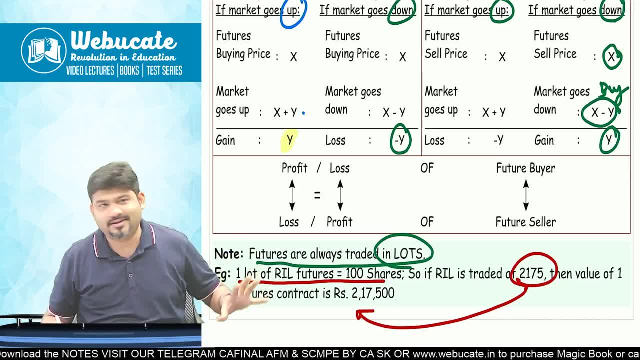 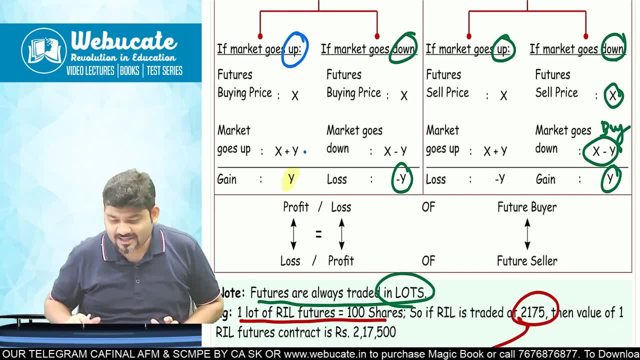 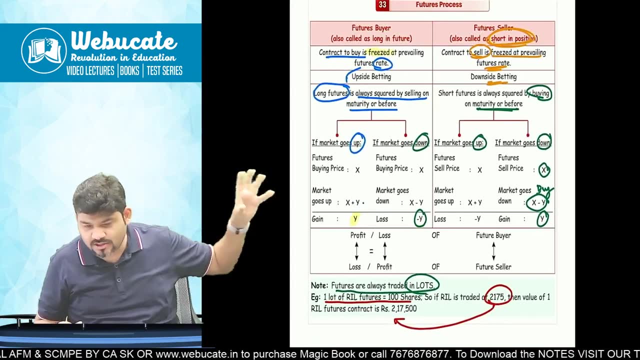 Just imagine. So this is where people have become from rags to riches and riches to rags, just by dealing in a futures market. Right, Are we clear everybody? Yes, Please confirm. Are we clear? So what is the whole process of futures? 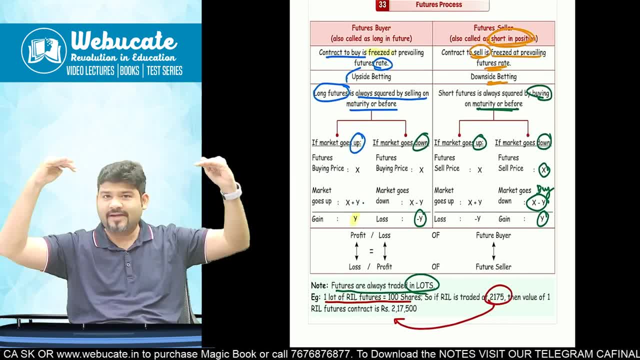 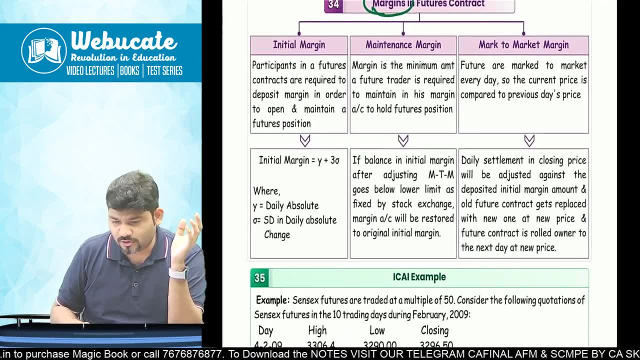 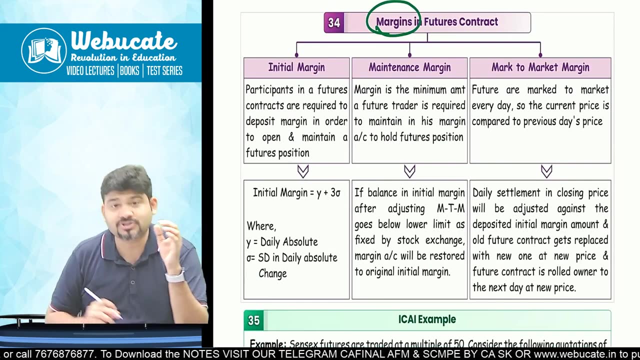 Either you sell or you buy. Right to sell, right to buy. The difference will be your gain or loss, as the case may be. OK, then we come to the whole concept of margin in futures contract, Something called as margins in futures contract. 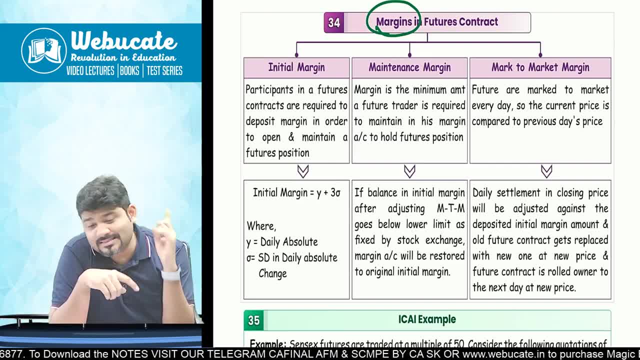 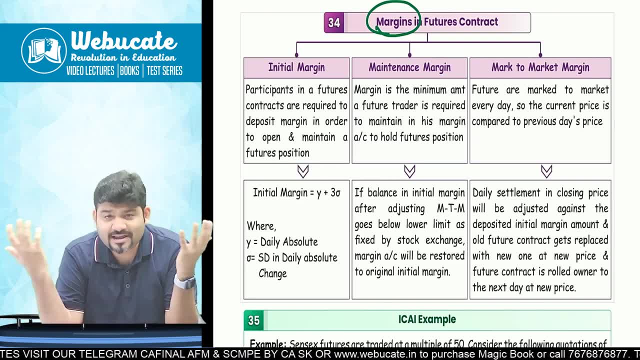 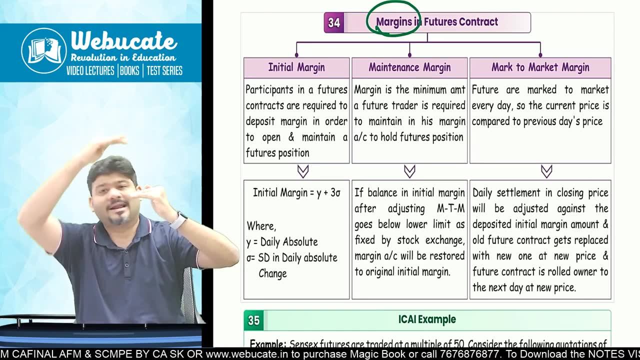 Now there are two types basically, margin. One is called as the initial margin, Another is called as the maintenance margin. Now try and understand. See, futures is a high volume game, high money value game. So stock market is afraid that. what if you are expecting the market to go up? 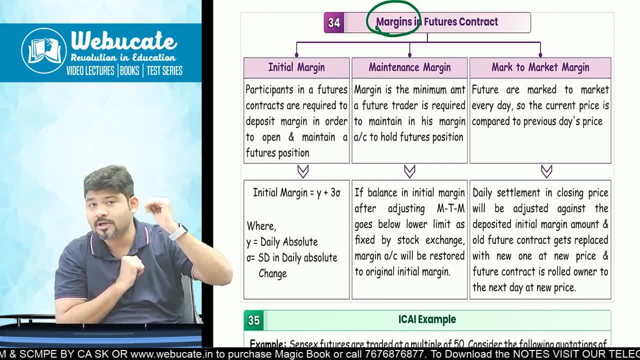 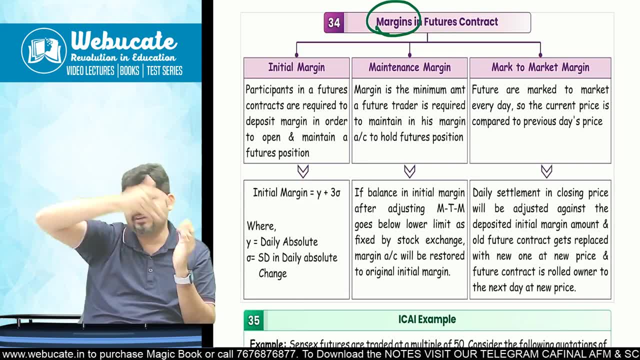 but the market goes down, then you are going to incur a huge loss. What if you don't reply and you run away with the loss? The other party, who is going to make the gain? he will want his gain. No, Now what will happen? 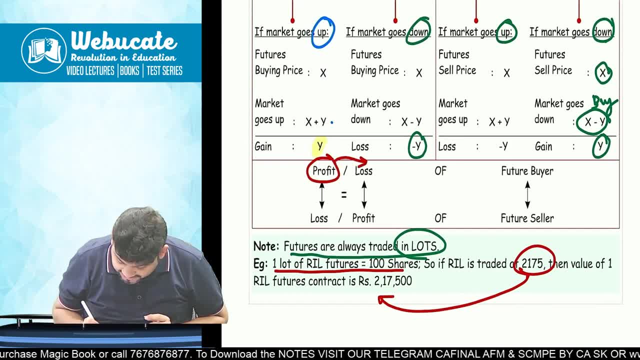 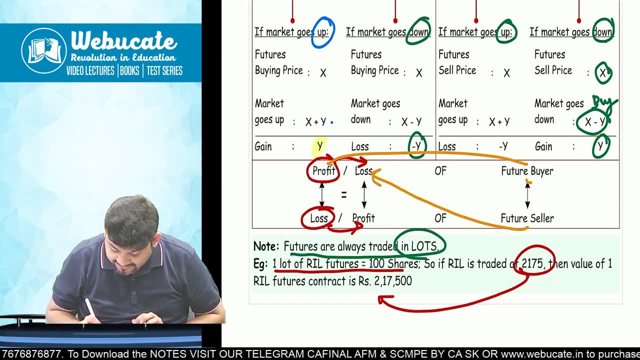 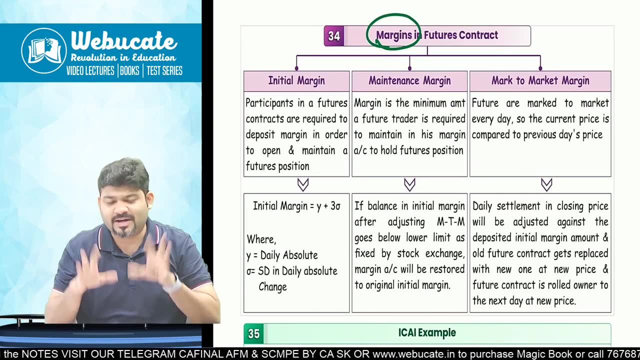 Because here I told you, somebody's profit is other person's loss, Somebody's loss is other person's profit, Right? If future buyer is making a profit, future seller will make a loss, and vice versa. So, in order that there is no default, they will take an initial margin from you. 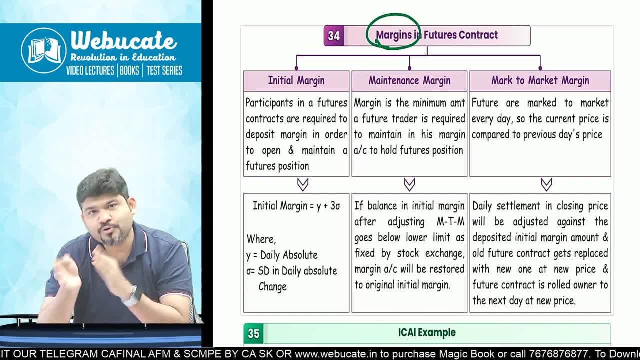 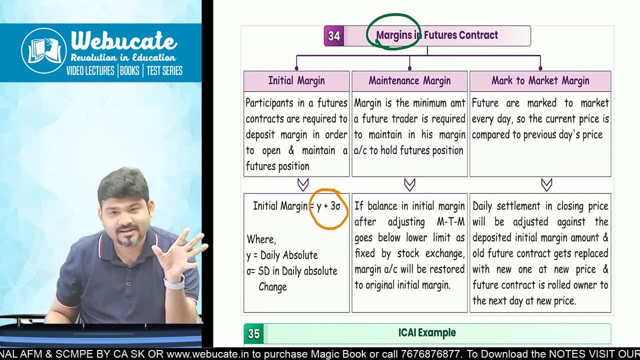 Yes, they will take an initial margin from. they will say that: OK, you have to pay ten thousand rupees as margin. So how is it decided, the amount of margin? for that? We have this formula, which is called as mu. This is not why this is actually new, but it's OK. 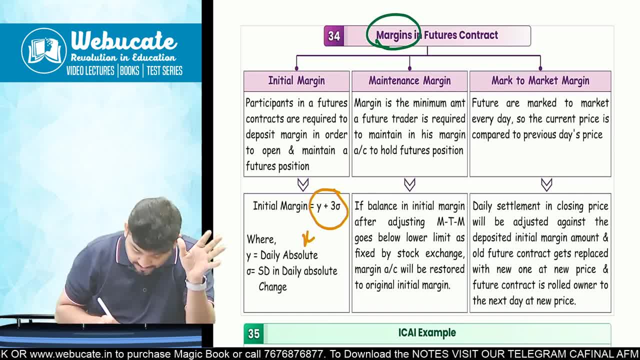 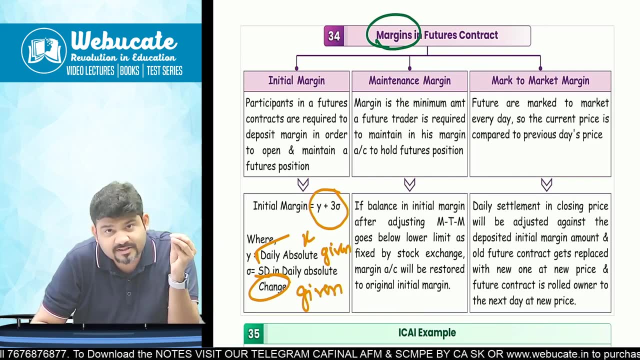 Plus three into standard deviation. Mu is your daily absolute, which will be given in the question. SD is your daily absolute change: daily absolute change. This will also given in the will be given in the question. So both of this will be given in the question. 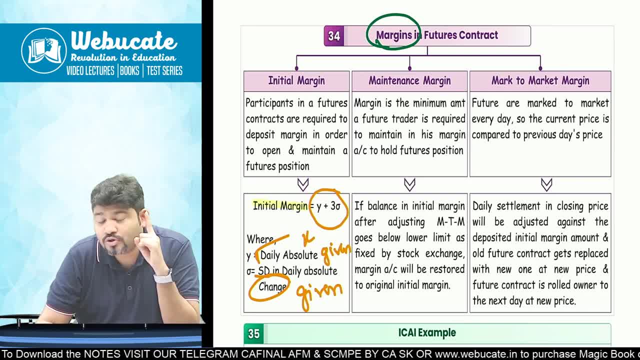 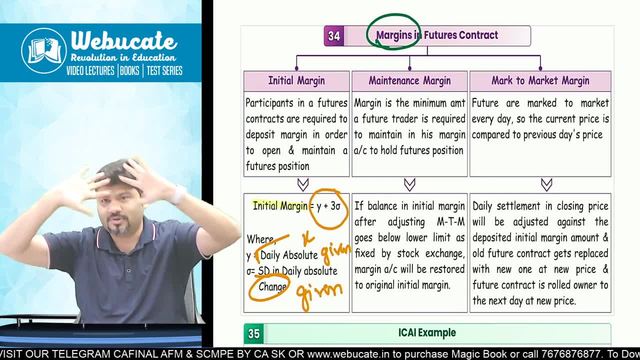 You have to calculate the initial margin. till the time you do not deposit that initial margin to the stock market, You are not allowed to trade Now this is not final. So initial margin: ten thousand rupees you have paid. now, as every day the market goes, 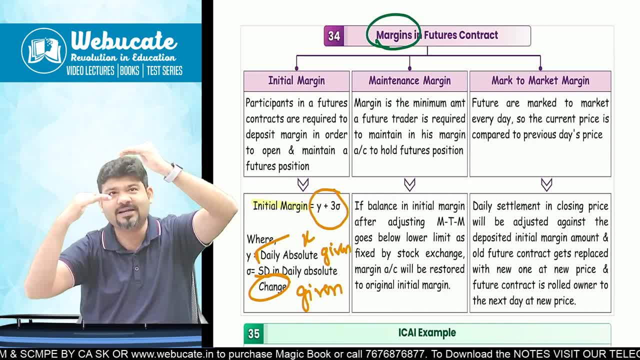 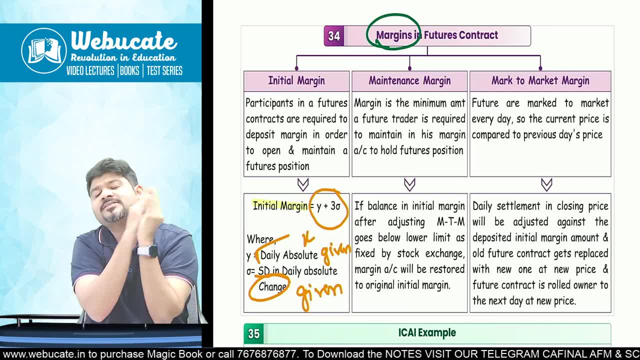 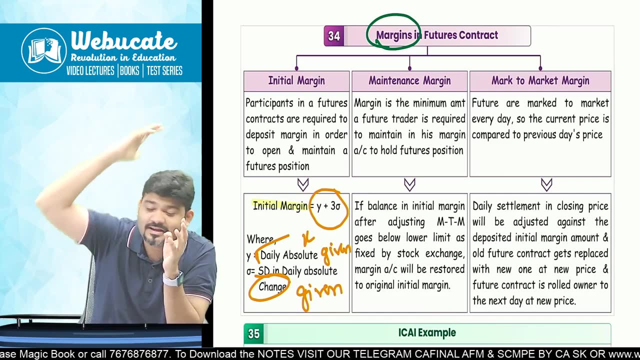 on. Suppose your balance is going down and down, We will keep a trigger which is called as the maintenance margin. So say the trigger is at four thousand. So if the market touches four thousand, by default you will have to refill till ten thousand again. that four thousand is called as the maintenance margin. 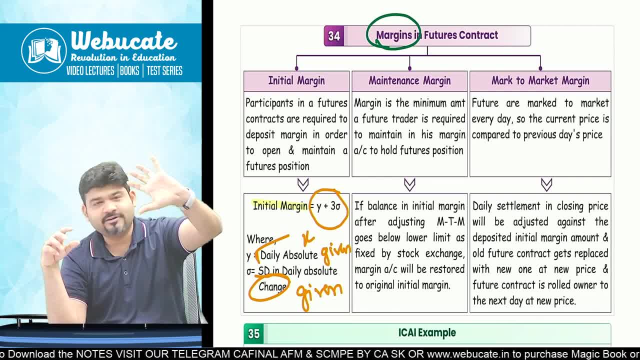 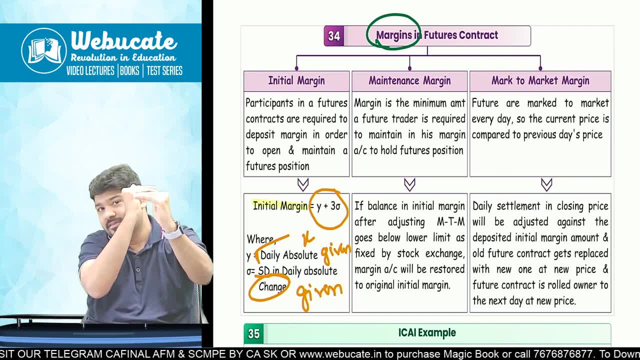 Are you clear? So initial margin initially that you have to bring. if the margin goes down, There is a trigger margin which is called as a maintenance margin. If The margin goes below the maintenance margin you will have to refill. But why will the initial margin go down, sir? 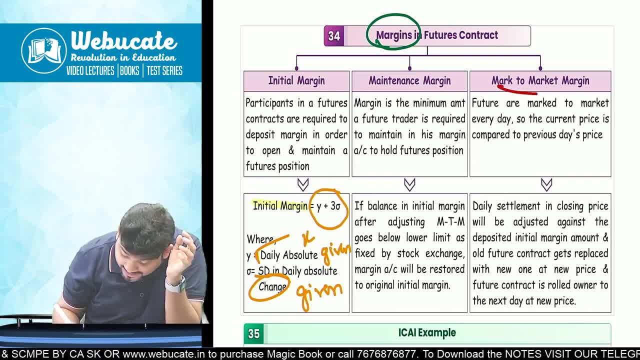 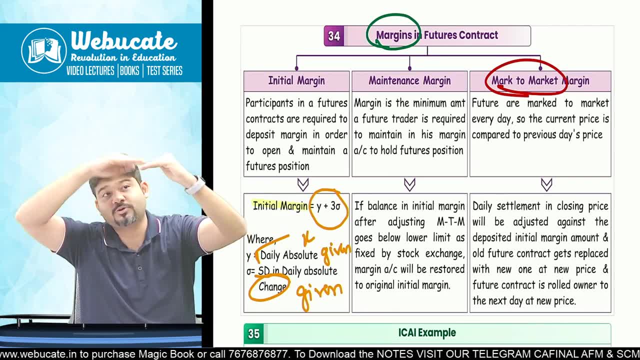 That is because of the concept of mark to market. So what is mark to market? I'll tell you. suppose you have a long position at one thousand rupees, So you are expecting the market to go up. But suppose if it goes to nine, fifty, 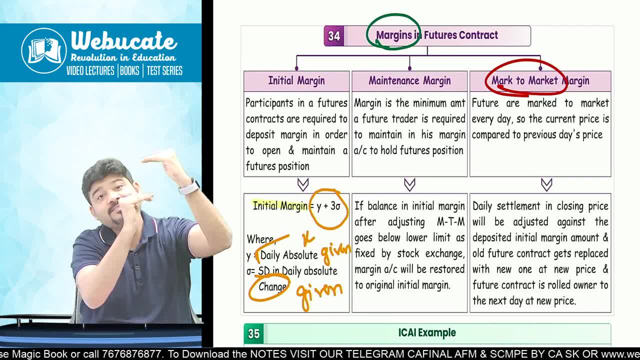 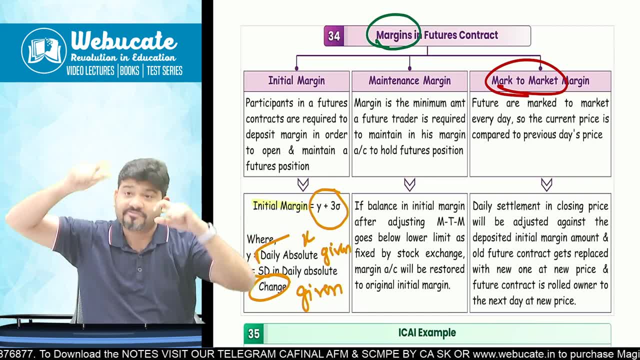 So nine one thousand is your long position. Nine fifty is your. now the opposite, If the short, the sale positions of fifty rupees is your loss, Now that rupees fifty rupees loss will be adjusted on a daily basis from the initial margin. 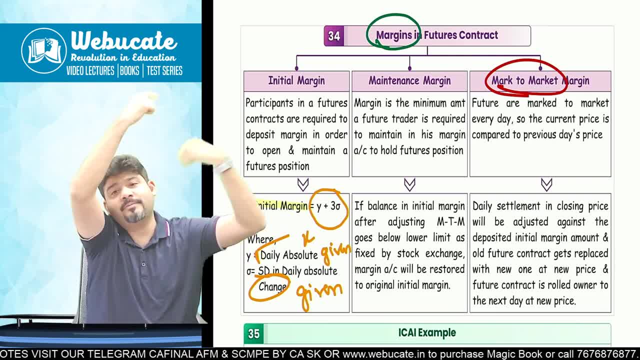 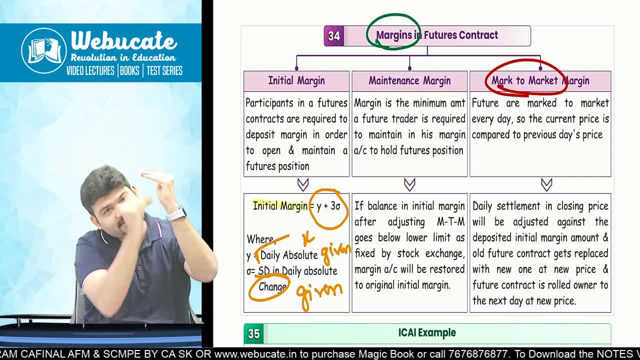 Suppose, if one thousand goes to one thousand, one hundred hundred rupees will be added to your initial margin, But if it is a loss it will be deducted from an initial margin. In this way, the margin will keep on going down. If it touches the maintenance margin, it is a trigger. 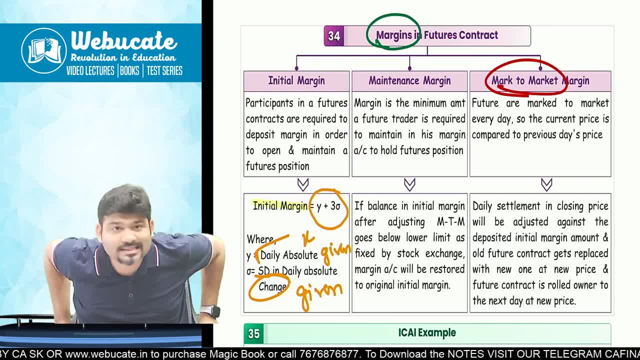 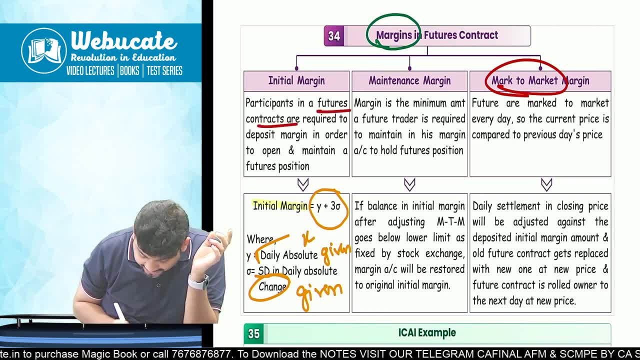 You have to refill the whole initial margin amount, which is ten thousand As the example. So in our case, everybody. So what is initial margin? Participants in a future contracts are required to deposit margin in order to open and maintain futures position are required to deposit margin. 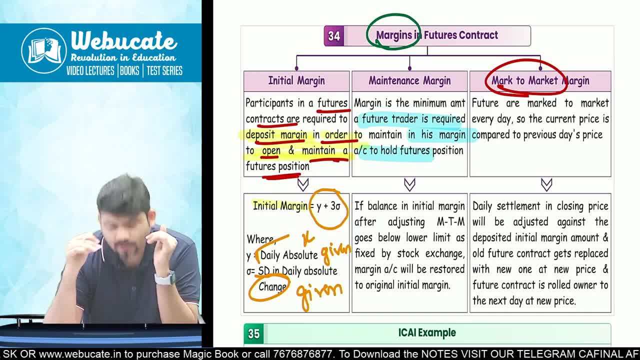 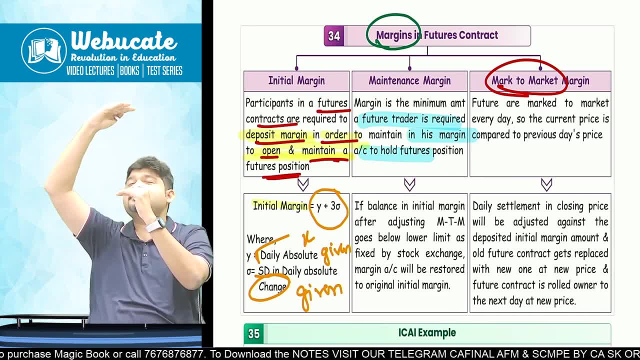 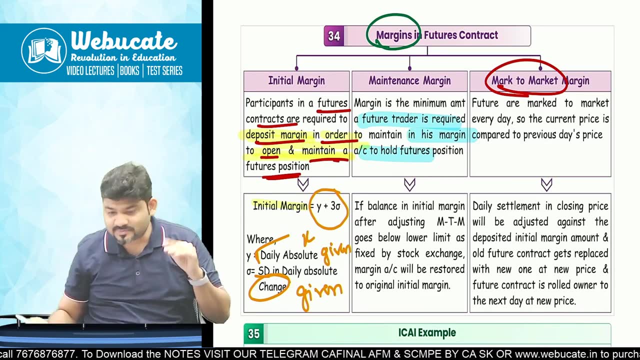 Right So. So as soon as it touches the maintenance, you have to go back to your initial margin, see initial margin Once you deposit, can fall, can fall. can fall, But minimum. it can go to maintenance margin, minimum amount. 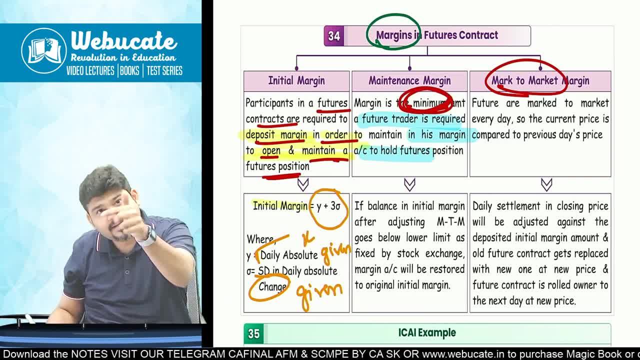 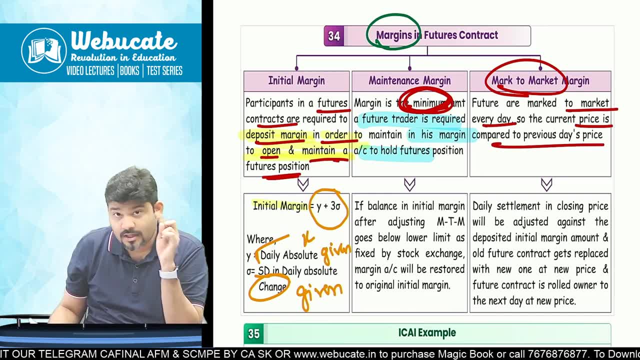 That is why it is called as a minimum mark to market settlement. Futures are marked to market every day, So the current price is compared to previous days price Now. in case of maintenance margin: if it touches maintenance margin, refill till the original initial margin. 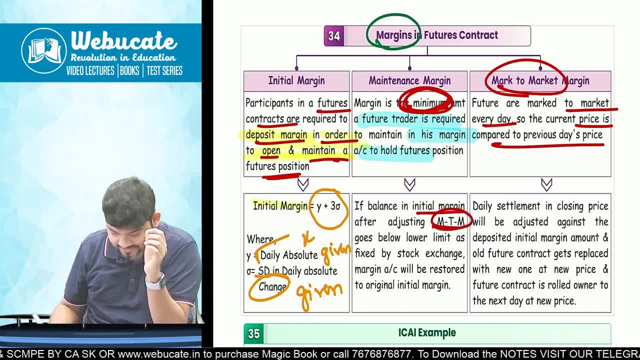 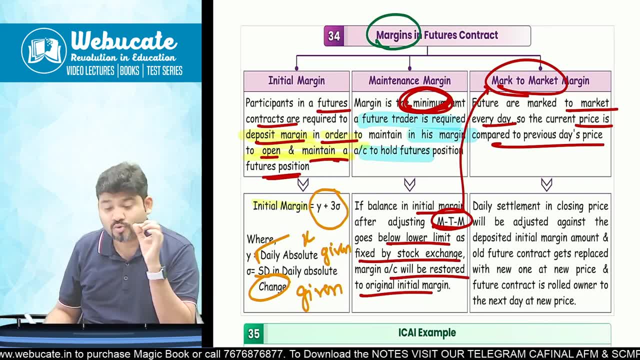 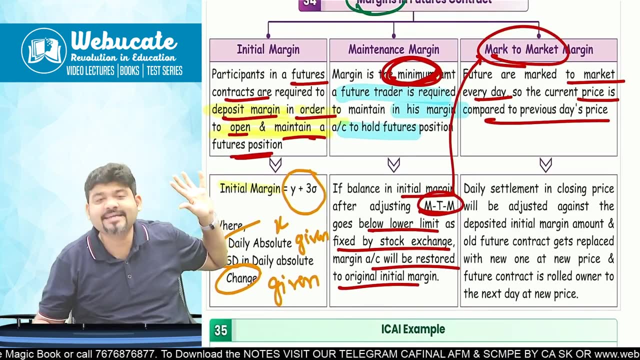 if balance in initial margin after adjusting MTM mark to market goes below the lower limit as fixed by stock exchange margin account will be restored to initial margin. margin account will be restored to the initial margin. Got it guys? Yes, sir. 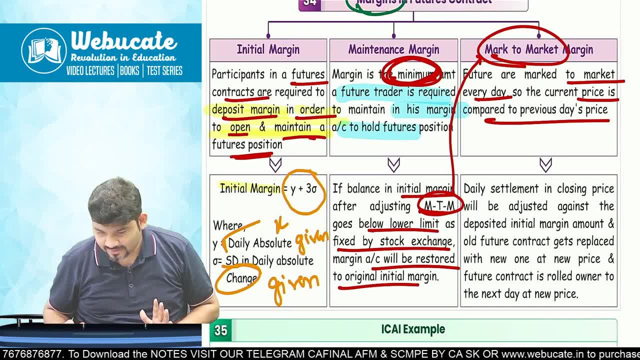 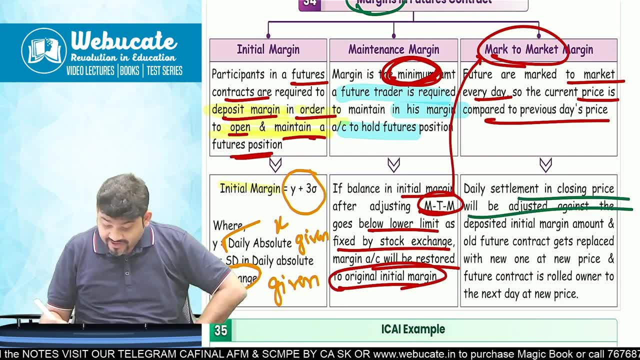 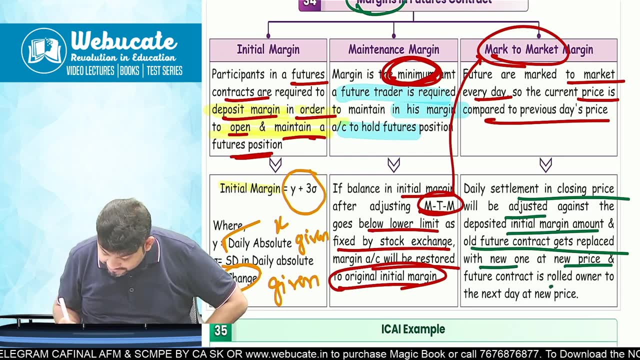 Absolutely clear- Will be restored to the original initial margin. Now what is mark to market Daily settlement in closing price will be adjusted against the deposited initial margin amount and old future contract gets replaced with new one at new price. and future contract is rolled over to the next day at new price. 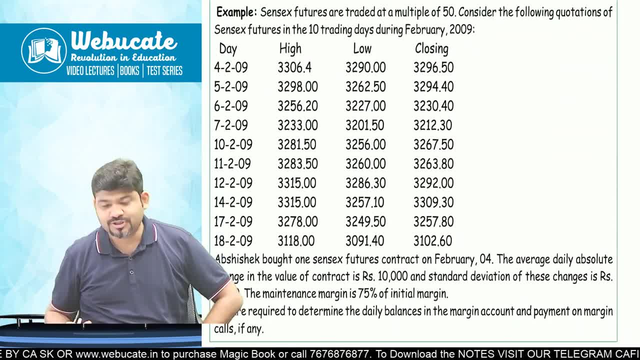 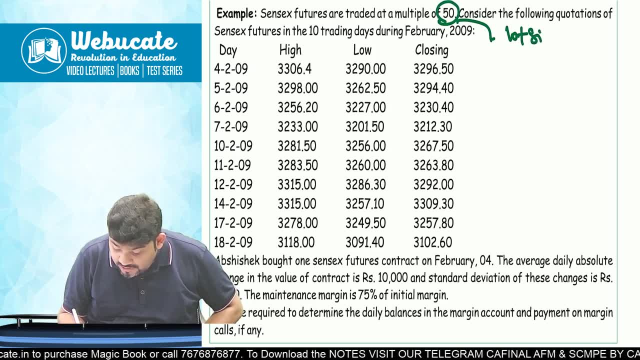 Let's have an example of ICAI module. Sensei, I traded at a multiple of 50. Consider this. So this is what. this is your lot size. Hello, This is your lot size. Following quotations are obtained for the trading days: 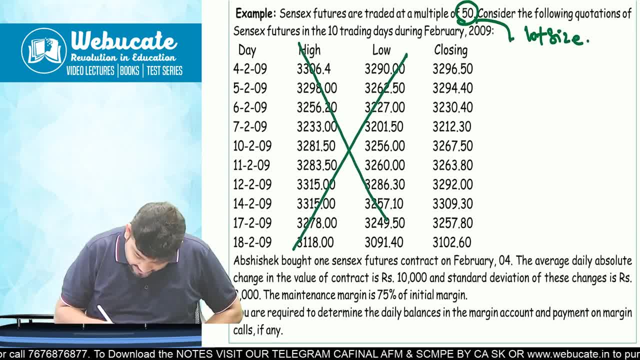 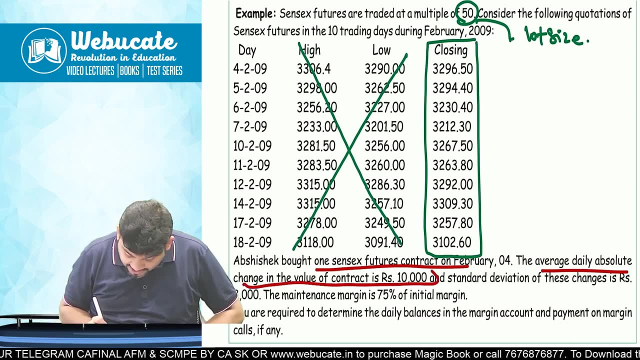 Low, high closing. We are not concerned with the low and high. Let's remove the unwanted information Now. the only wanted information is there, which is the closing balance. Abhishek bought one sensex futures contract on February. The average daily absolute change in the value of contract is ten thousand. 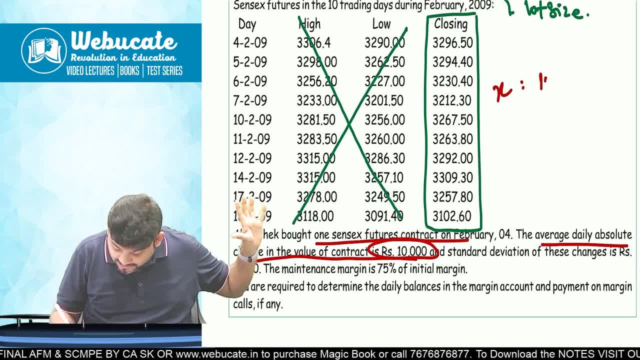 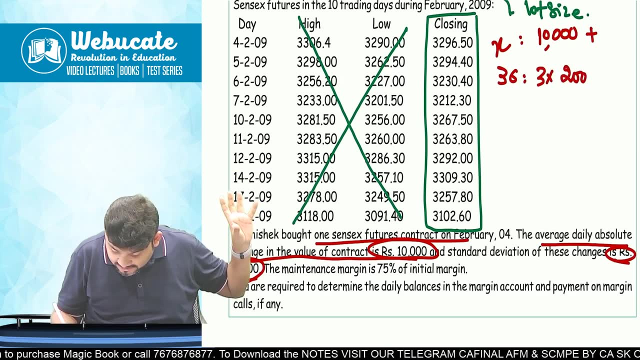 New, new, new, new, new, new. new is how much? ten thousand, new is How much. it is Correct: Ten thousand plus three, standard deviation. standard deviation is rupees two thousand, three into two thousand, three into two thousand, so total will be sixteen thousand. total will be sixteen thousand. 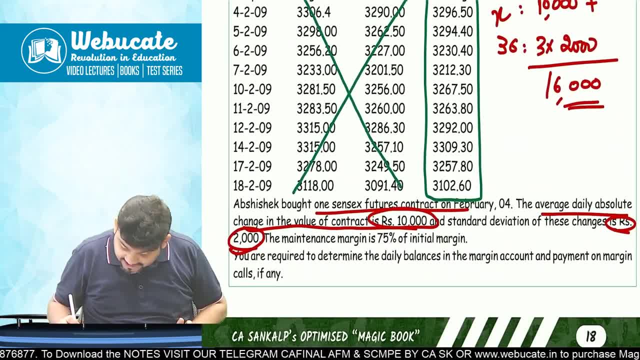 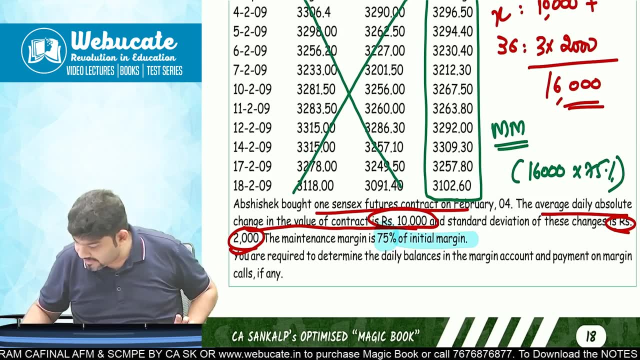 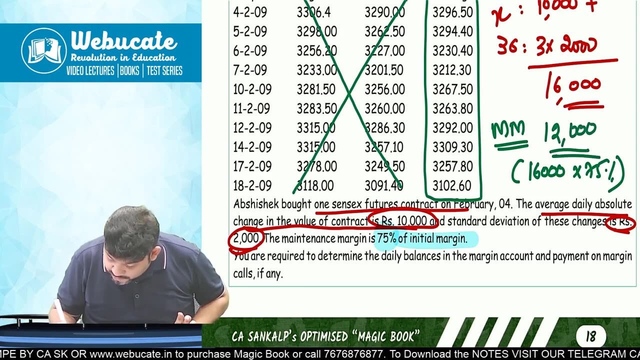 So new plus three into standard deviation Sixteen thousand. The maintenance: maintenance margin is 75% of initial margin. So what is your mm? It is 16,000 into 75%. So it will be 16,000 into 75% And this will be, and this will be, 12,000.. Got it everybody? So? 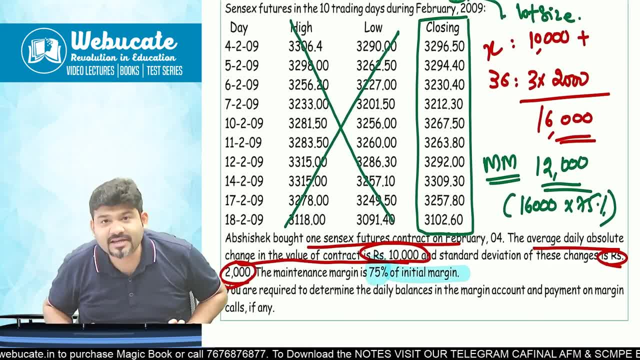 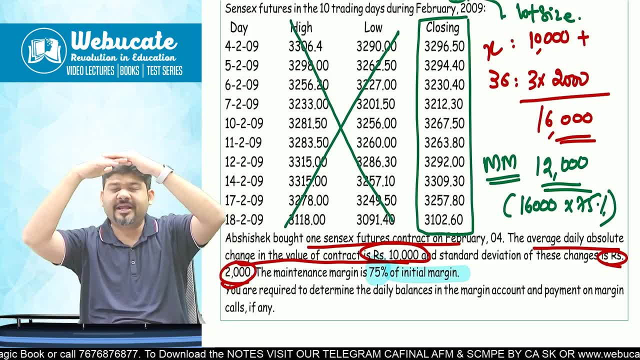 mu plus 3 into standard deviation 16,000 and maintenance margin 12,075% of this. So as soon as the MTM goes below 12, you will have to refill it till 16,, not till 12, till 16.. Remember that. 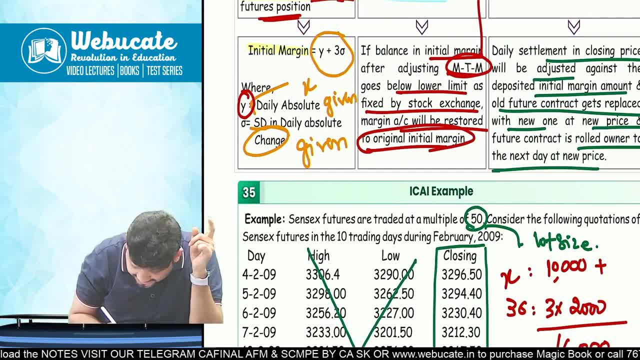 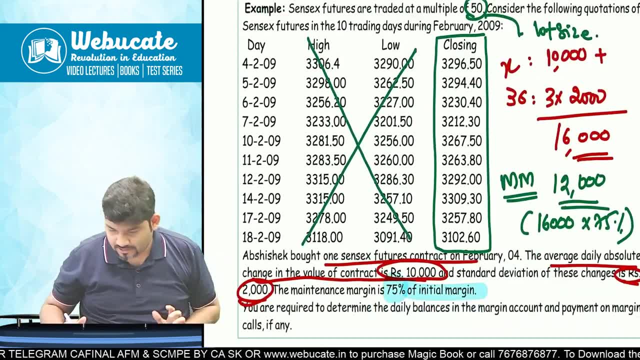 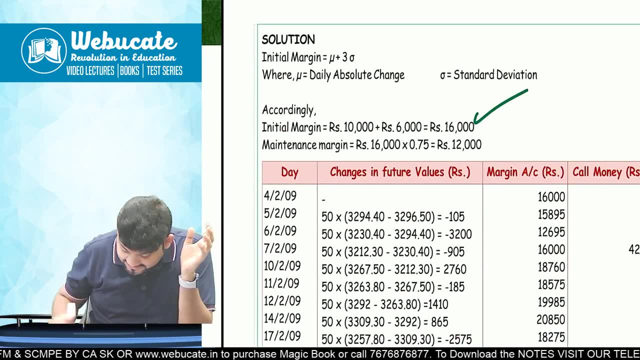 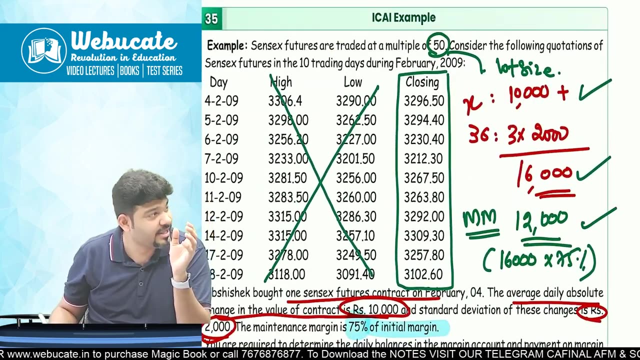 till 16.. So original initial margin. Hello, You have to restore it till the original initial margin. Got it? Now let's try to calculate it. So see here, we have already calculated the initial margin, 16,000.. We have already calculated the maintenance margin, which is 12,000.. So 16,000 and 12,000. 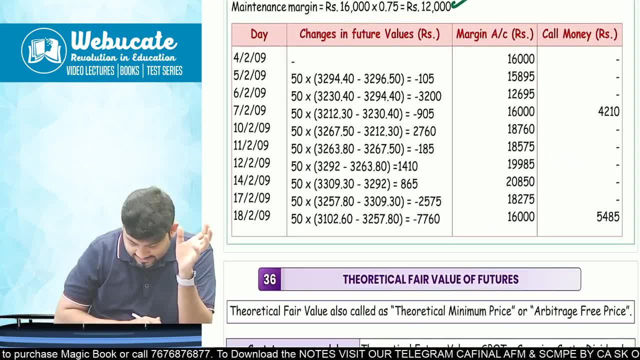 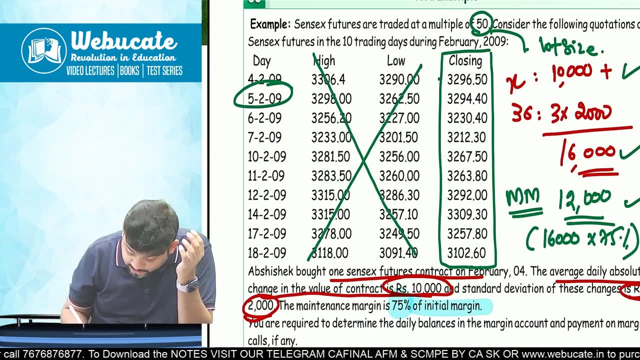 Everybody done. Now let's start fourth Feb. Obviously, it's the beginning. Now let's go to the fifth Feb: 3296.5 and then 3294.4.. What has happened? Oh, value is falling Down from 3296.5.. Now it is gone to 3294.4.. So can I say 2.1, there is a loss of 2.1.. Hello. 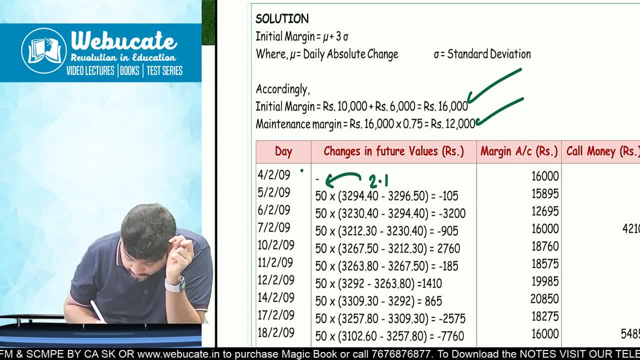 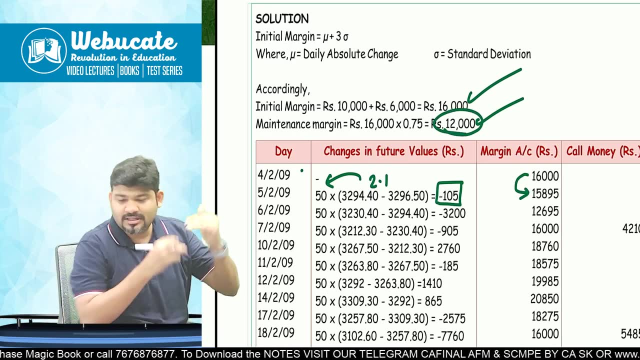 there is a loss of 2.1 into 50. So into 50. This will be 105 minus, which will be reduced from the margin, correct? so is it gone below the maintenance margin of 12 000? no, so let it continue. this is. 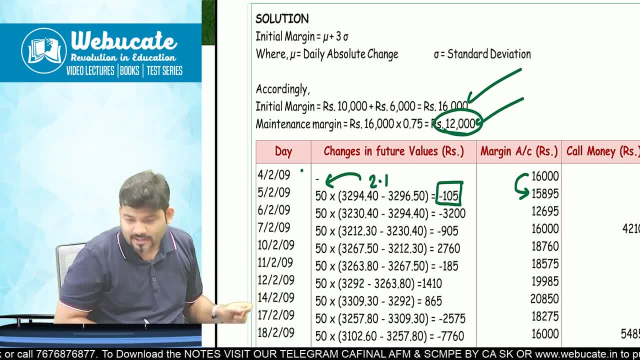 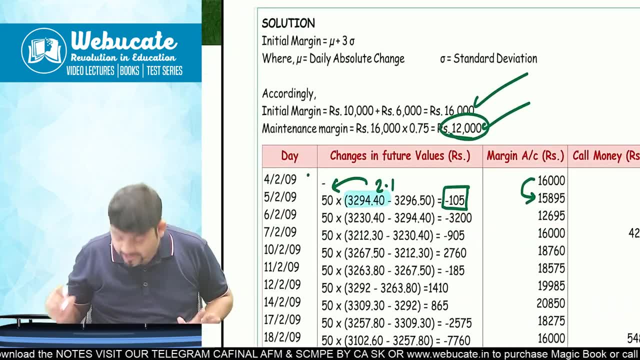 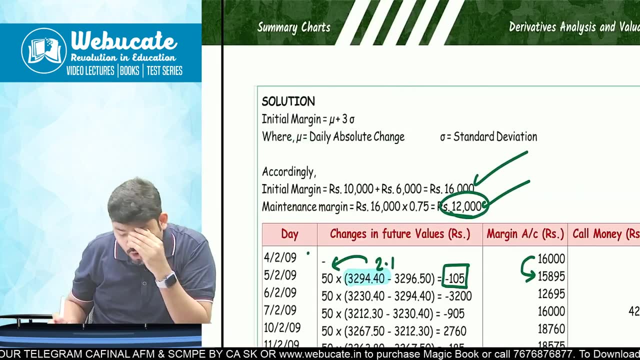 called as mtm mark to market. now again next day. for next day the price is now freezed at 3294.4, so now 329. so comparison will be from: with 3294.4, next day the price moves to 3230- again a loss. so 3230 minus 3294.4. multiply by 50 again, a loss of 3200 will be reduced from 15 895, again 12 695, and i will tell you that 12, 695 is the new margin balance account mark to margin. 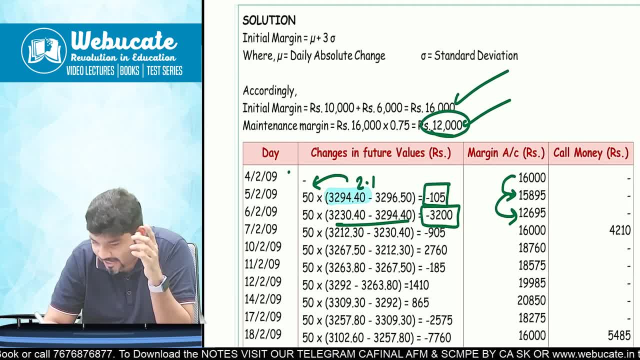 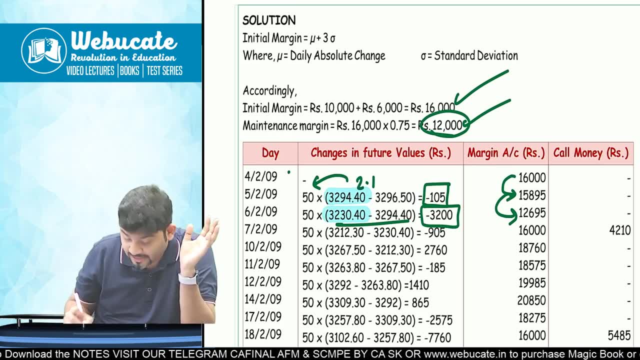 everybody. now. next day again. see now your new price is 3230. now the comparison will be with 3230, 3230, 3230, 4.4. next day again. what happens? this falls down to 3212.3. multiply by 50, so there is a loss of minus 105. 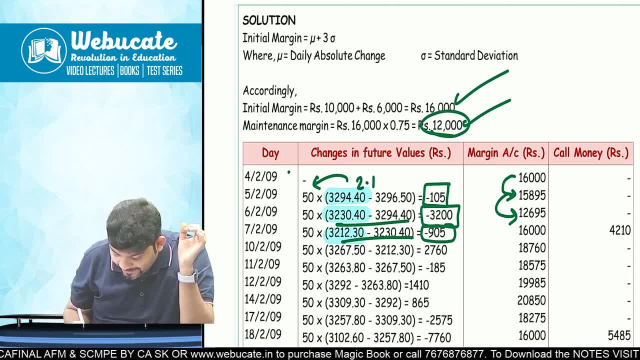 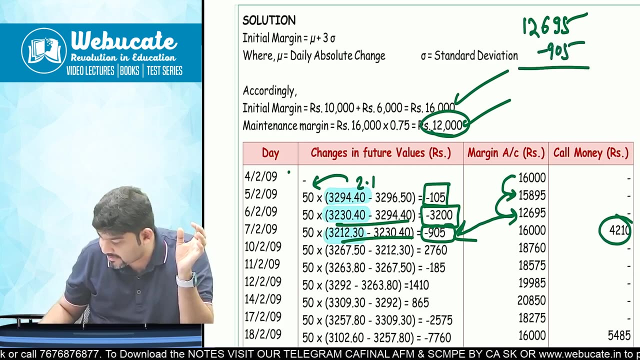 omg, now can i say it is falling below. so 12695 minus 905, so 11790. my god, we will have to refill it till 16. 4210 is what we will bring. are you clear? 12695 was there, right of which now, because of mtm905, will become minus. so 12695 minus 905, oh, my god, you will. 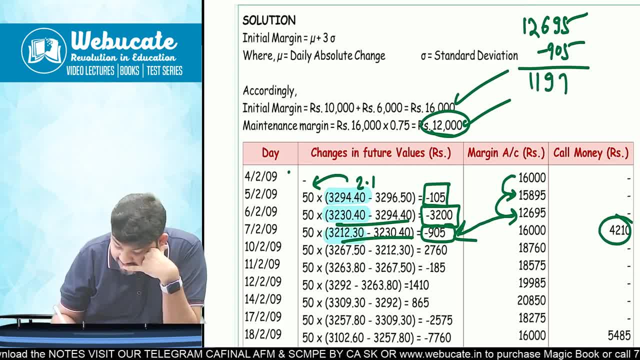 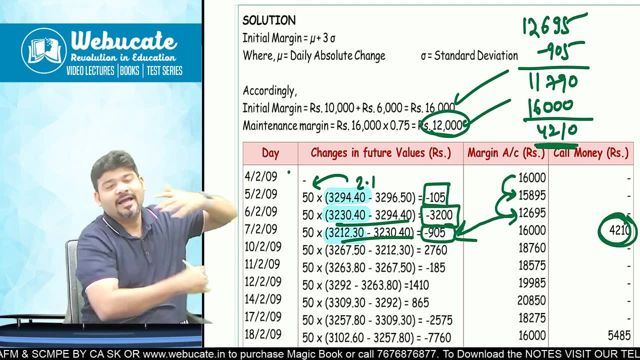 immediately get a call from stock market. sir, please refill, sir, please refill. how much i have to refill, how much i have to refill till 16 000. so how much i will have to bring. so 11790 minus 16 000 and it will be 4210, and you can see here 4210 and this is how the system will work. this is called. 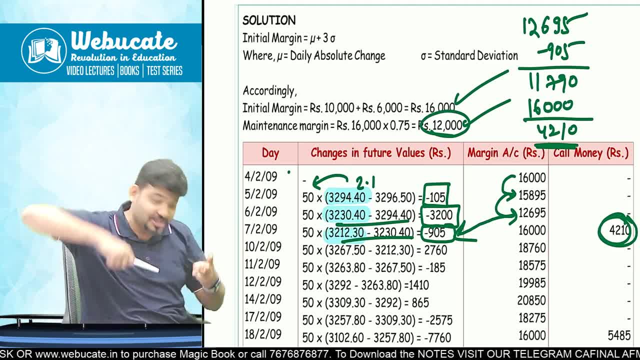 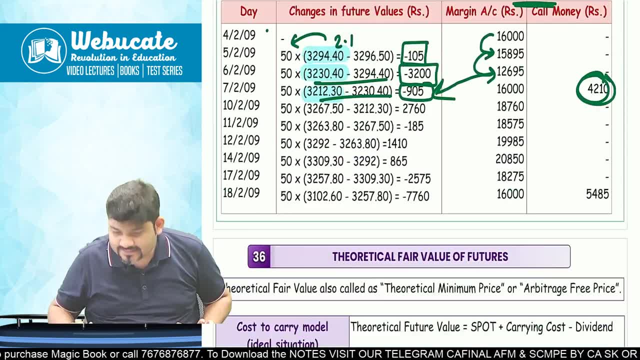 as the concept of initialization of the stock market and we will see how the system will work. margin maintenance, margin mark to market gotcha everybody, yes, any questions, any doubts? no sir, done next. so with this we are complete with first the understanding of futures, then the futures. 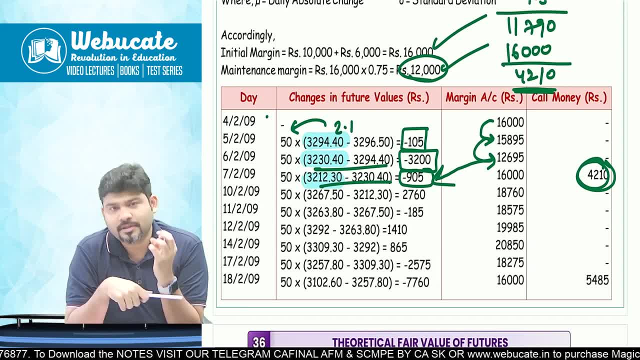 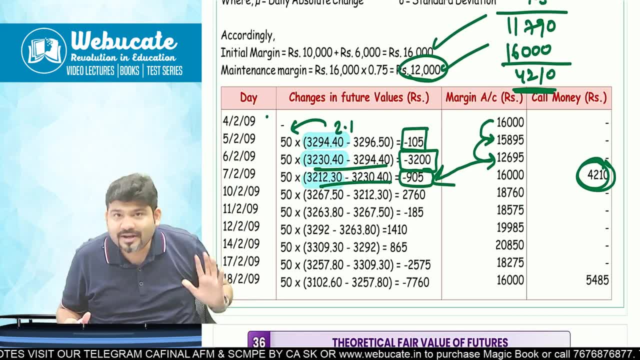 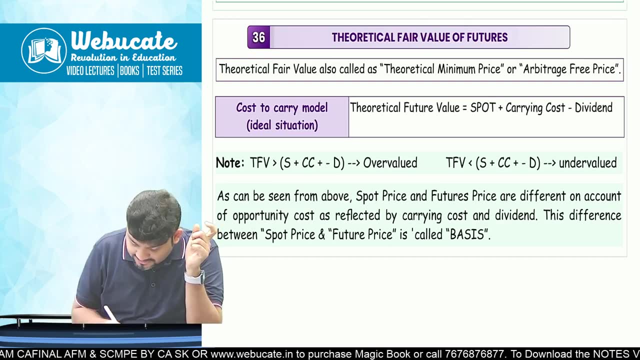 process. then we did the initial margin maintenance margin mark to market and along with that we also did one sum related to it. got it done. now we come to the concept of theoretical value of futures. now we come to the concept of theoretical value of futures. so what exactly is your theoretical? 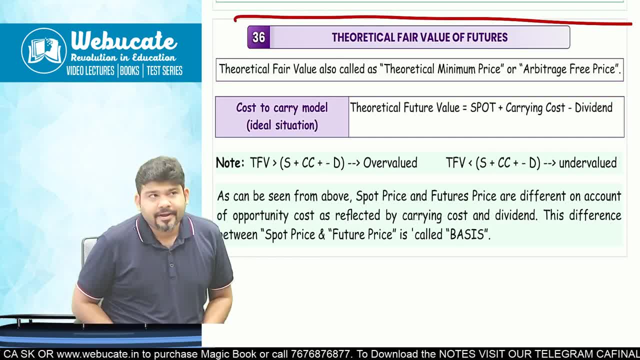 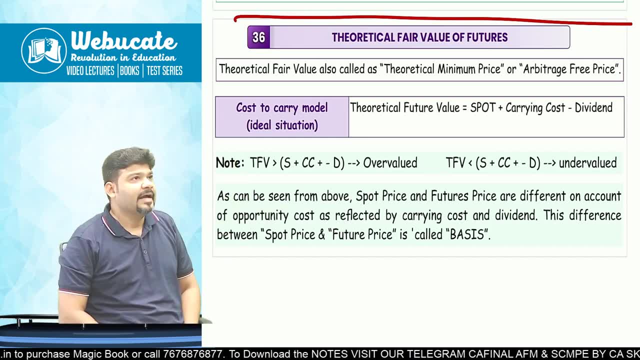 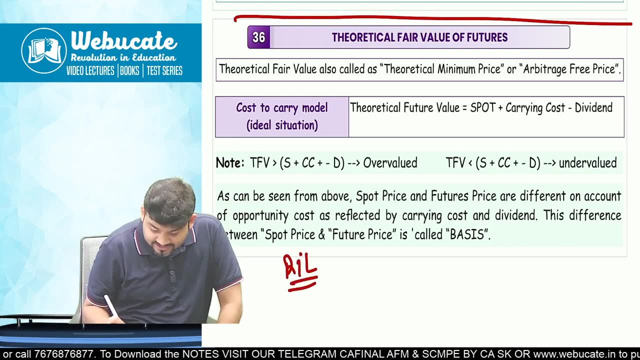 value of future. see, i'll tell you when you are planning for a buy position or long position or a short position. okay, after three months. so one: there is a spot price say. i'll just give you a practice example. say one there is a spot price, say of reliance: spot is rupees 1000, spot is rupees 1000. 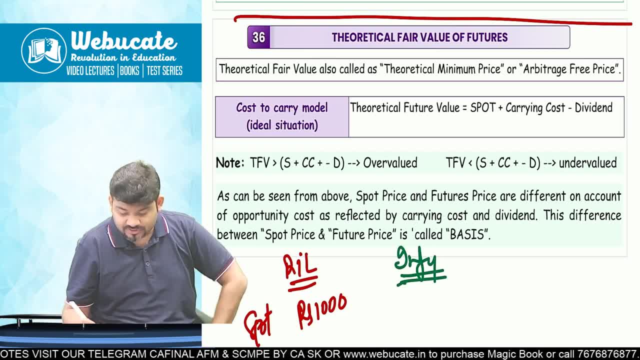 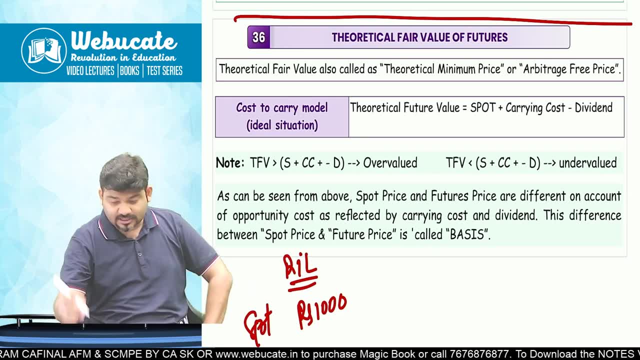 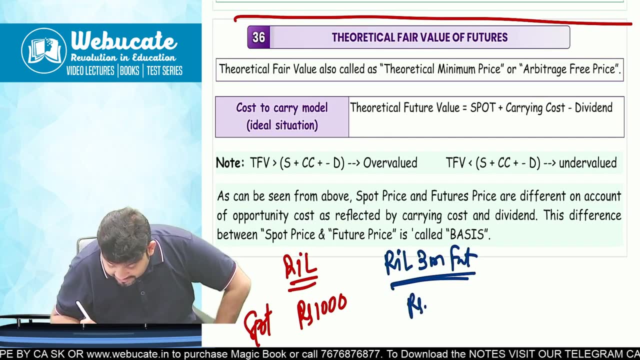 and the other is: say infosys, say infos. sorry, let's go with the reliance only. okay, suppose reliance spot is 1000, you will always find that reliance three months futures will be a different amount. say it will be 1090. what? you will always find that reliance three months futures will be a different amount, say it will be 1090. what? 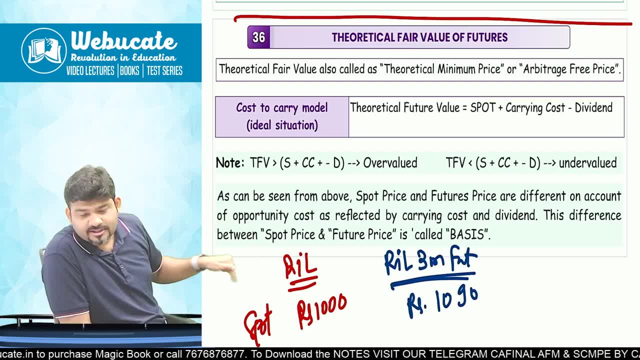 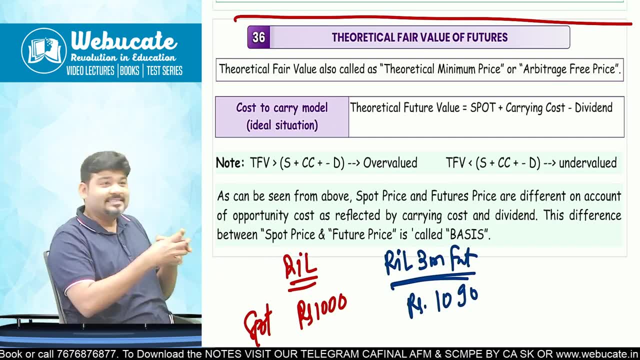 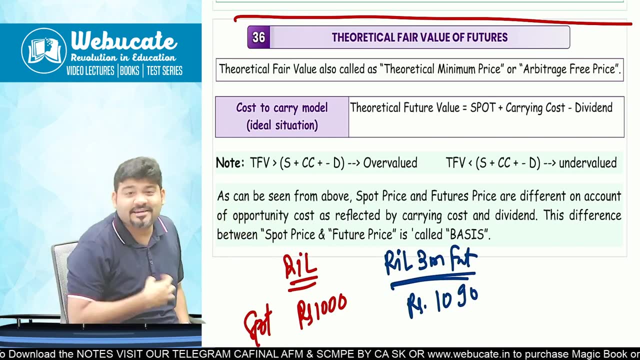 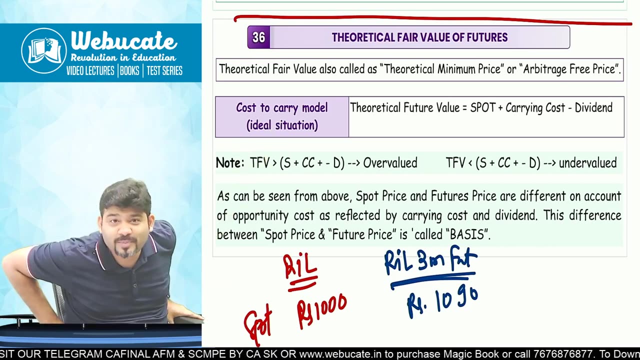 so the same reliance today is 1000. why is it that reliance three months futures will be 1090? because this 1000 is now going to be executed after three months. i, the stock market, is giving me a price of 1090, which is currently 1000 for three months later. so who is going to bear that? 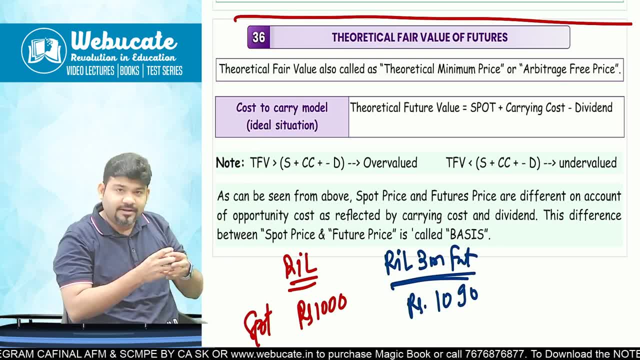 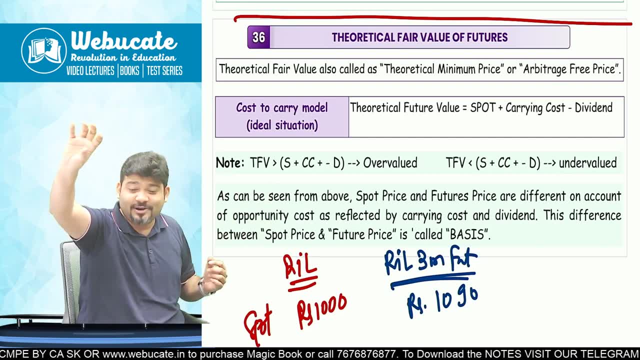 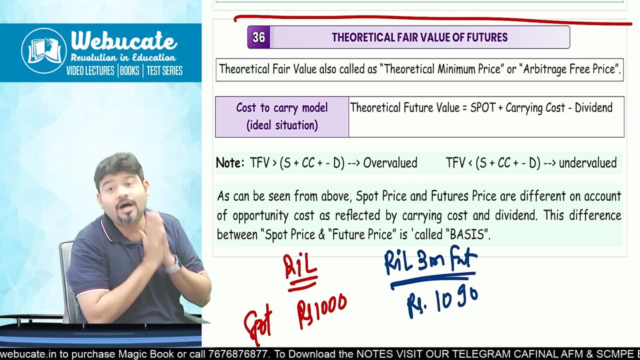 opportunity cost. this 1000 might as well. i would have invested in it for three months later, so i would have invested as well. but now, instead of investing, i am freely getting 1090 price, so that 90 rupees kind of is like the opportunity cost of managing the futures is like the opportunity cost. 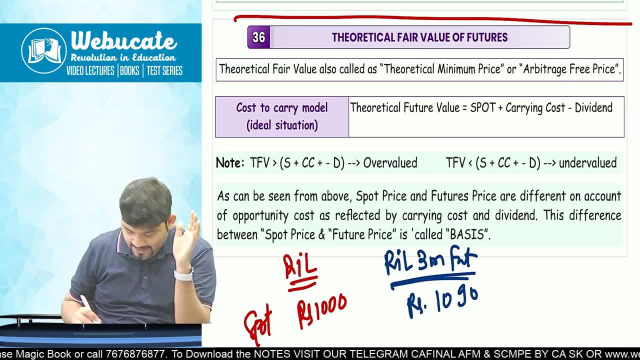 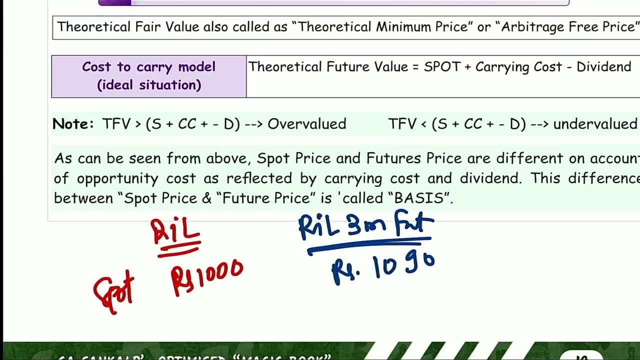 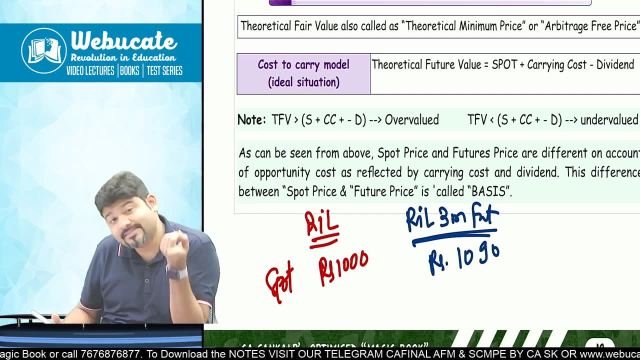 of managing the futures. so now, how do you calculate? this is now i am going to teach you for sure, for sure, wait, okay, now let's continue with this example. so suppose reliance today is 1000, reliance today for a three month future is at 1090. so why this 1090? i'll explain that to you. 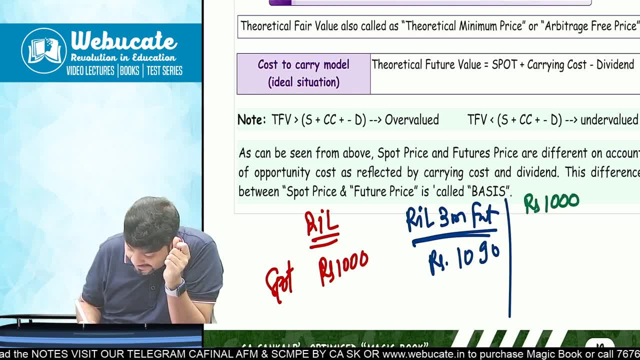 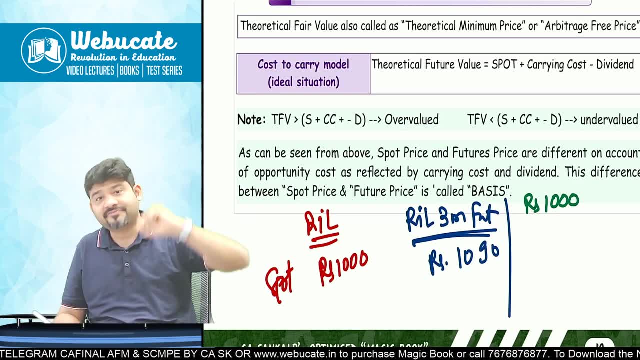 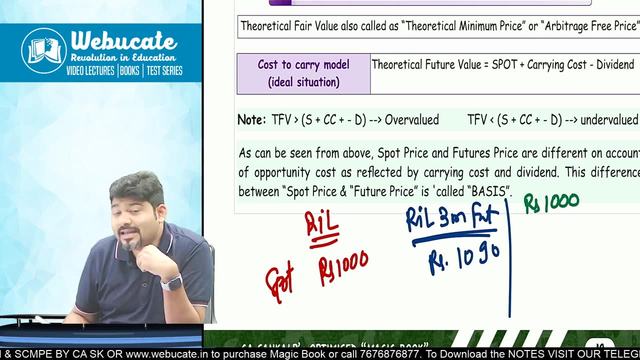 suppose if 1000 rupees is the price today, correct, i am getting the price for a three month future without paying anything. see, margin is a different thing. but other than that, for freezing this 1090 i don't have to pay anything. so basically i am getting a benefit of how much of the current 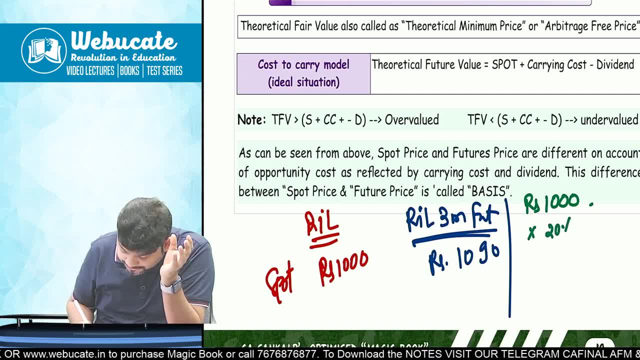 interest rate now. this is the price of the future. so i am getting the price of the future, so i am getting a benefit of how much of the current interest rate now, this 1000 rupees, i am able to save. suppose it is for 20 months, and this say reliance future is for, say, six months. 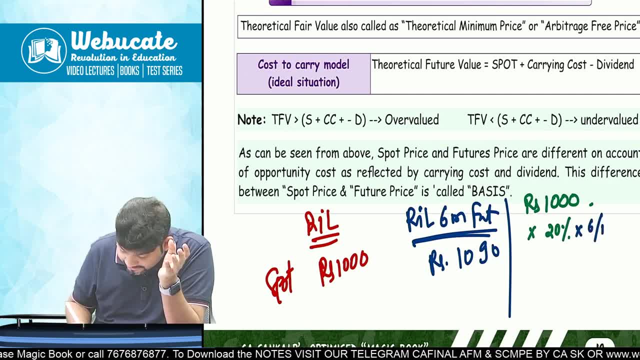 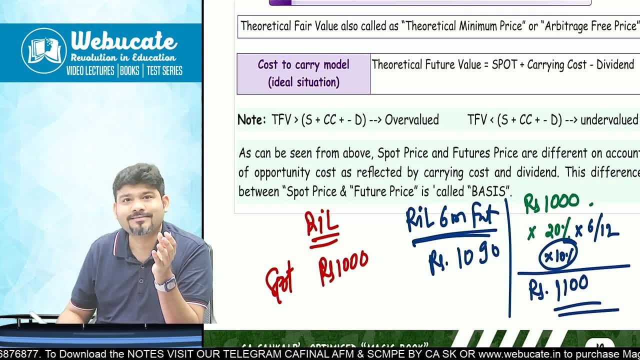 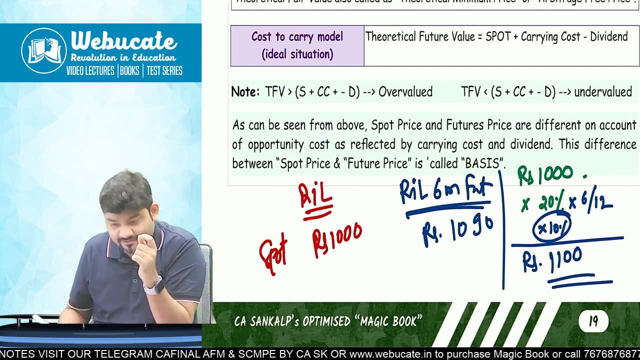 they reliance. this is for six months, so twenty percent into six by twelve, so it will be ten percent, so it will become one thousand one hundred. this will become, say, one thousand one hundred now, now, now, now. so ideally i should be paying one thousand one hundred for a spot, one thousand. 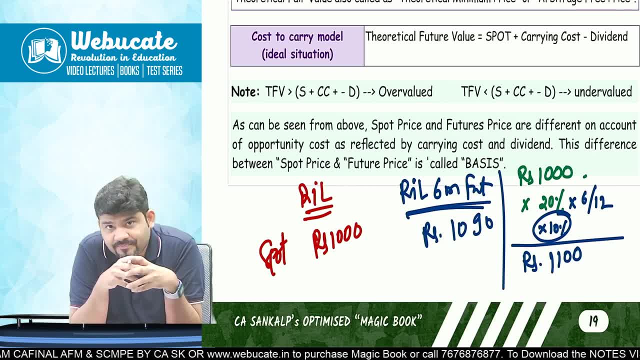 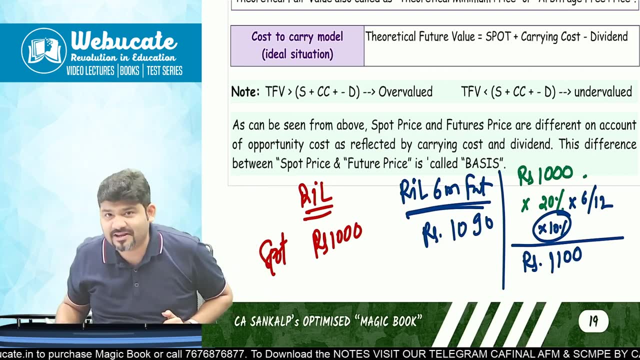 reliance future. so spot is one thousand. if i purchase it, my money will get blocked. if my money is blocked, i would have earned hundred rupees, which now i am not able to earn, if i would have purchased the spot now. stock market is giving me this benefit. 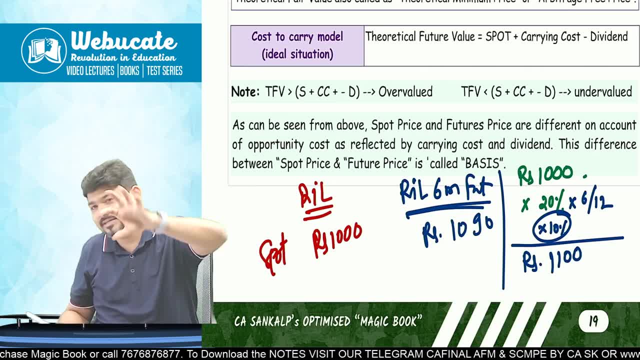 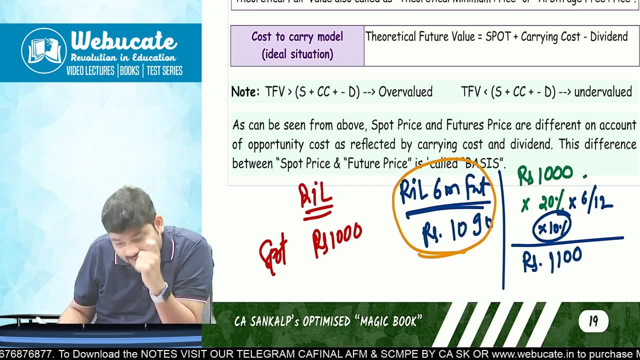 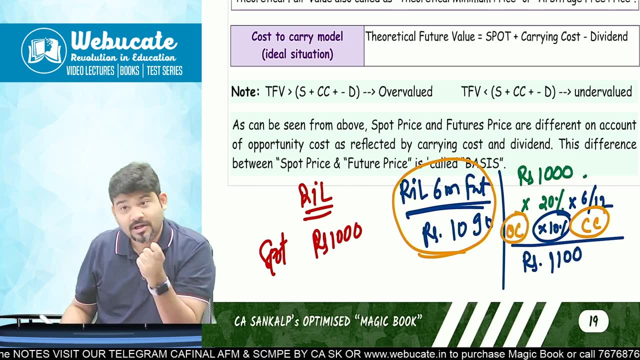 hundred rupees benefit, that even without taking hundred rupees, they are giving me- that you know- opportunity to sell or buy after six months. so that is where we will adjust this, something called carrying cost or something called as a opportunity cost. but, but, but this person will say: what if there? 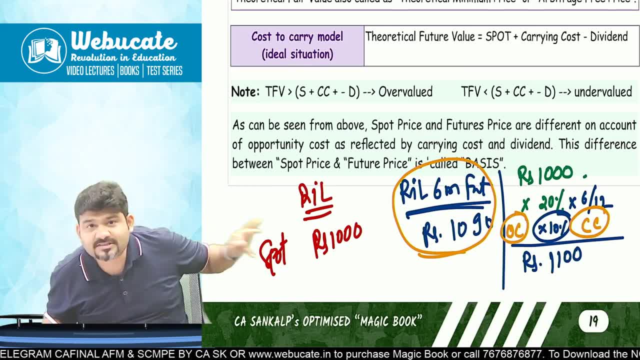 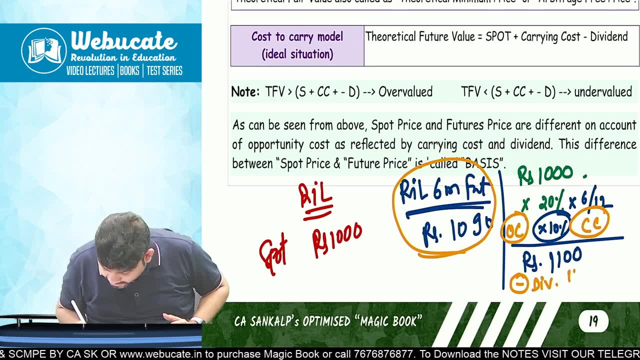 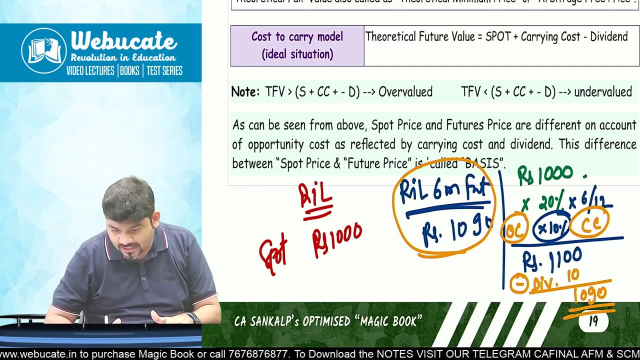 is a dividend. declare this dividend. if i would have purchased the spot, i would have got the dividend. now i am not going to get the dividend, so okay, okay, so we will reduce. suppose the dividend of 10 rupees would have been received and the net amount will be 1090. so the net amount will. be rupees 1090. so it is like this that i go to the market when i get the pairs, but when i get the driven figure and the judge orders them so they do not sell at presentations. and this is exactly what you do. the jurors do something, they do not sell a lot, but if aurer can do one, that is it. would be beneficial. so for now, if, of course, you give something to me, just to do it. so if it is not generous, so it will be there for this. if i amți the fact that if i buy not think this you will be either s tag that goes to where i will determine. 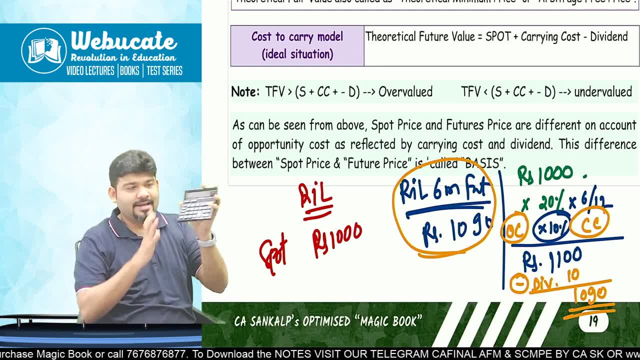 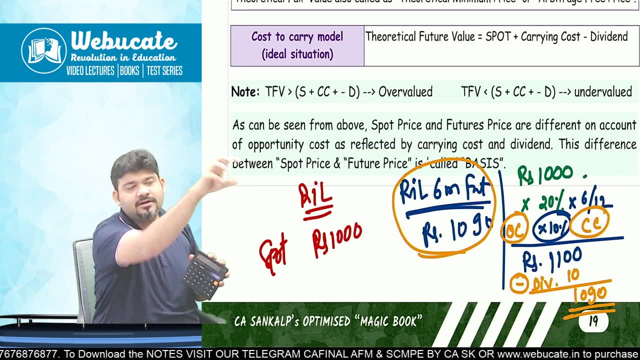 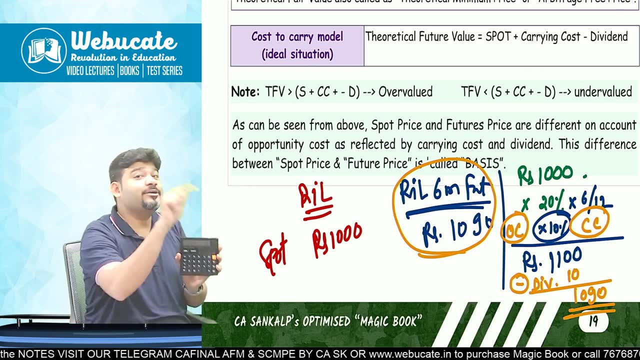 zero. so it is like this that i go to the market and purchase this at one thousand rupees. instead of this, the customer shopkeeper tells me: come after three months, i will give you at the same rate of one thousand rupees. but is he going to charge me one thousand only? the answer is no, he. 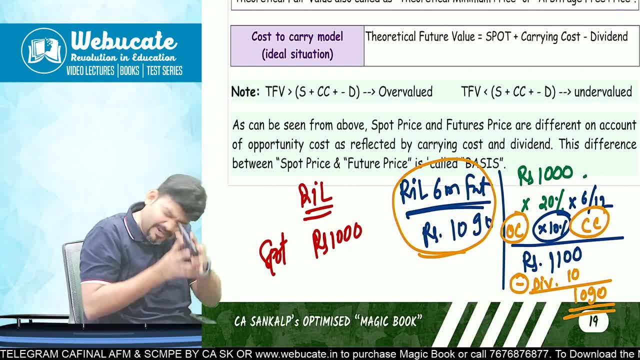 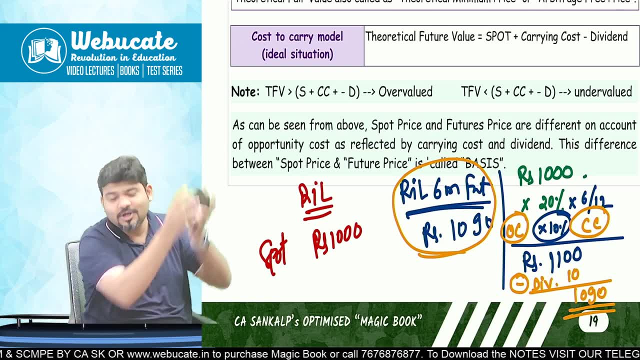 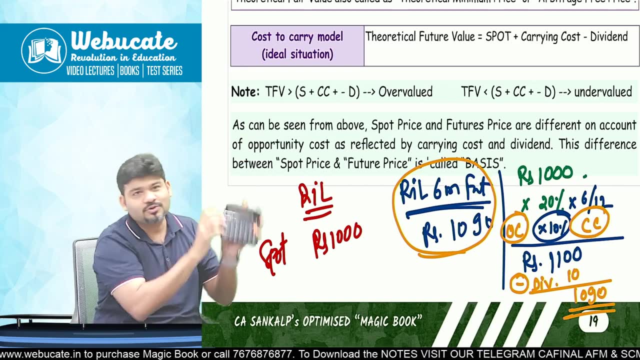 is going to say, even though i am going to give you the same price, only one thousand, but i am saving your opportunity cost that also you have to give me after three months. so in all, after three months the price will be one zero, nine zero for you, or one thousand one hundred dividend reduced so one. 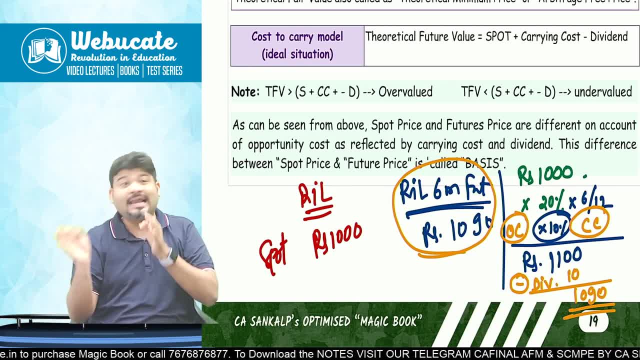 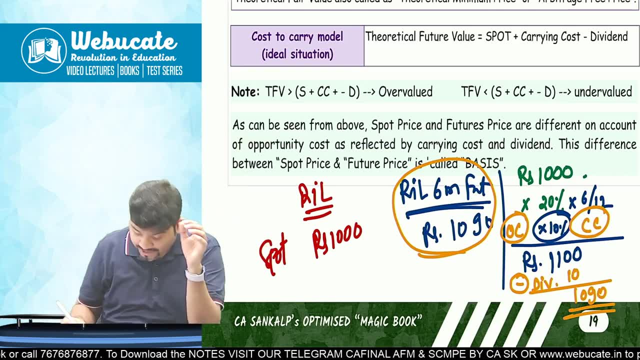 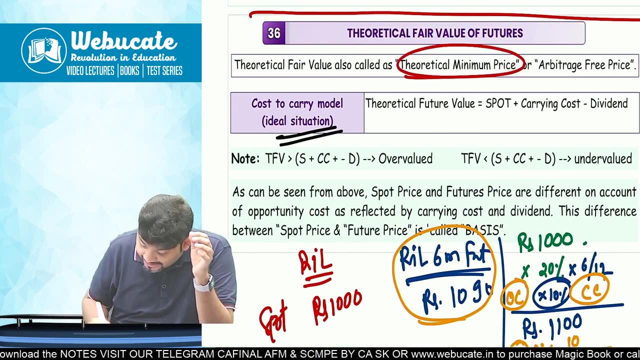 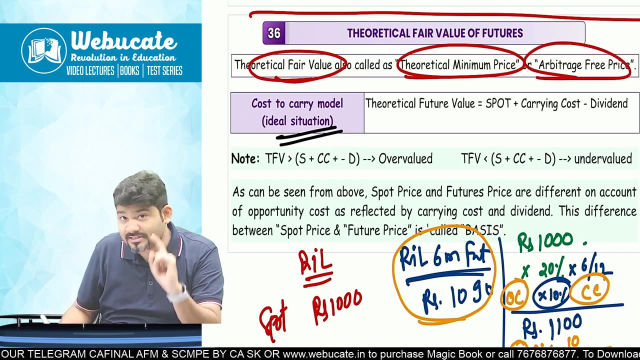 zero, nine zero is what you have to give me for this calculator at a three month later stage. this is called as the carrying cost or cost to carry model of the futures price- theoretical future theoretical theoretical. theoretical minimum theoretical fair value price, or called as the arbitrage free price. what is it? it is going. 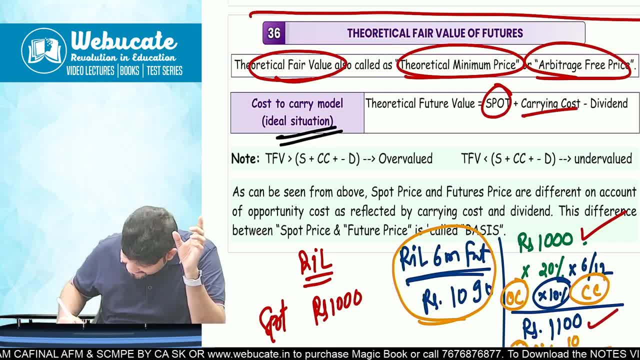 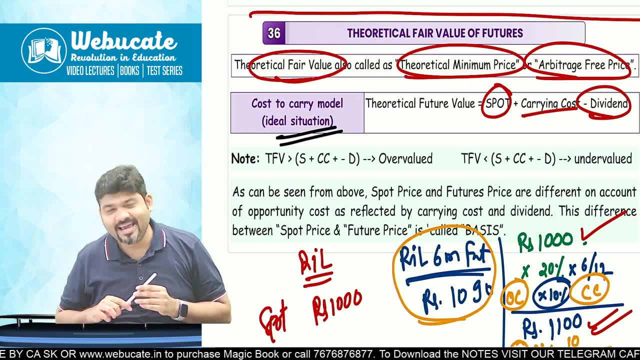 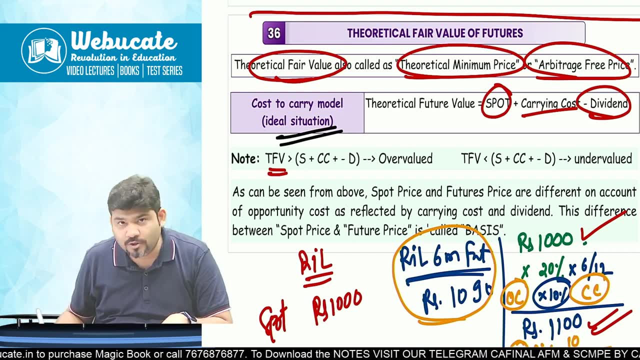 to be the spot price. yes, plus the carrying cost: hundred rupees. yes, minus the dividend, minus ten. yes, hey, are we clear, everybody. now, when we do this calculation of theoretical future value, suppose. so now, ideally it should be one zero, nine, zero, correct, suppose if, IF YOU ARE DIVIDED, 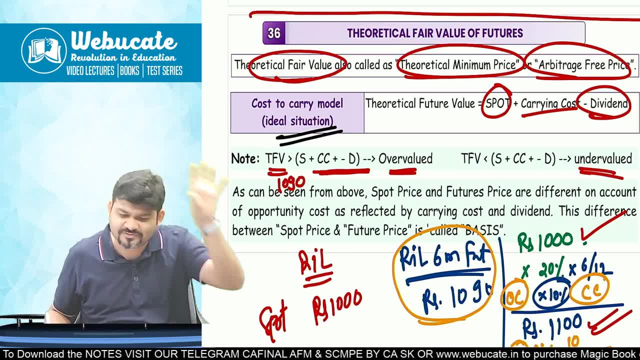 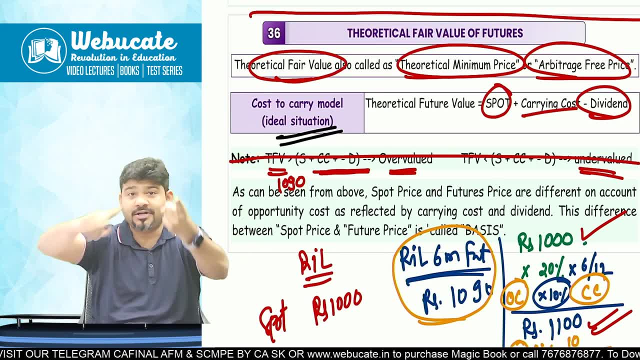 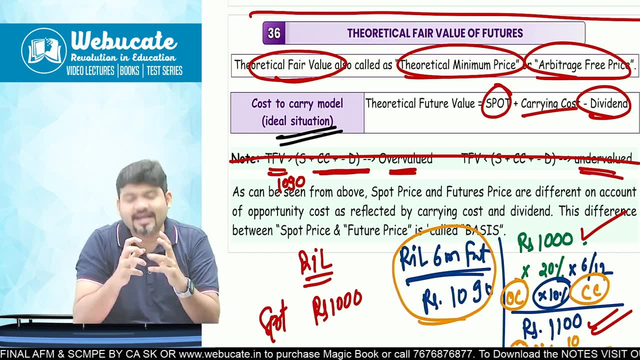 IF YOU WOULD LIKE TO GIVE THE Dividendy LOOK AT THIS, ok. so in this case, let me give an example. if this theoretical future value is overvalued or it is undervalued, then it will give rise to arbitrage, which we will see later on. for now, just try and understand the calculation. how do you calculate the? 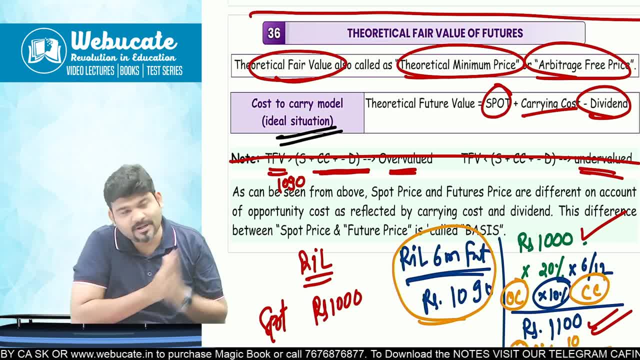 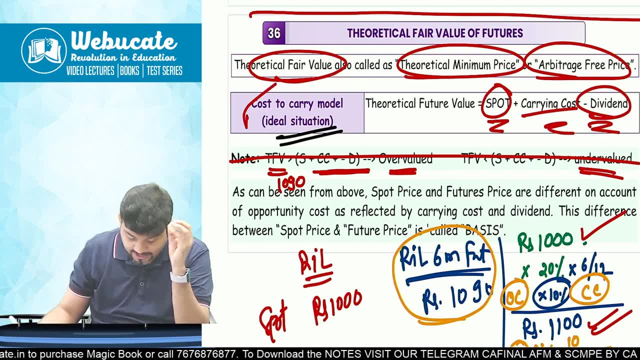 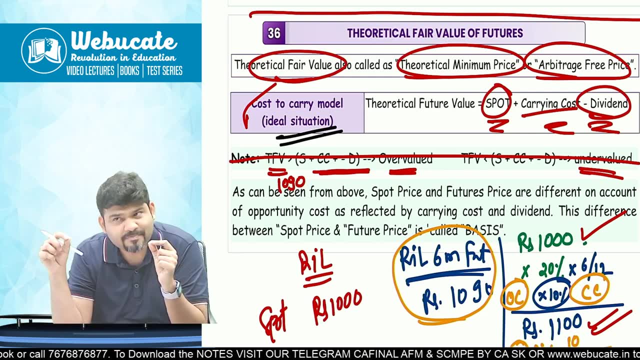 theoretical future value, spot plus carrying cause. but if any dividend was to be received by the spot point two interval between two level return and Canad Grammar EPP dividend, are you clear: spot plus carrying cost, less dividend. is your cost to carry model? got a done so, will your spot price and futures price be same? ideally no, the three month difference. 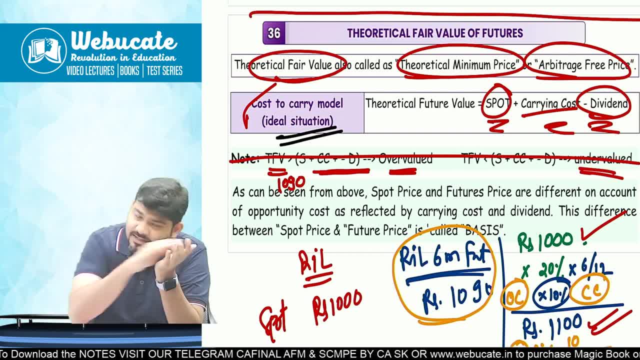 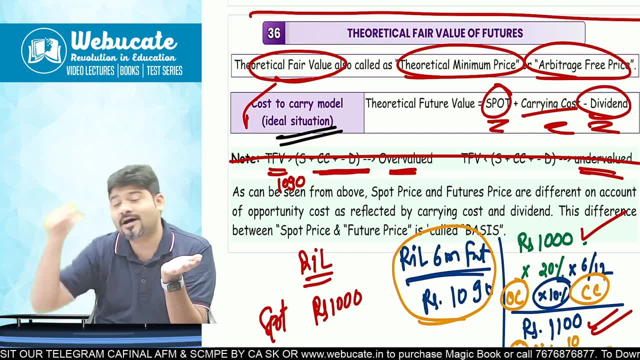 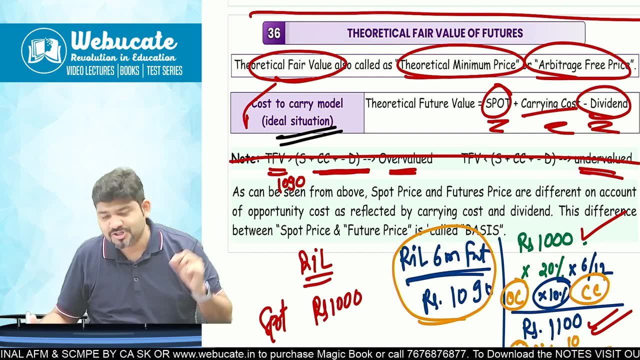 will give rise to a different pricing, at this price only, but the difference will only be of the opportunity cost or the carrying cost. i has also adjusted with the dividend because there is a difference in the spot price and futures price for the same share. it is called as something. 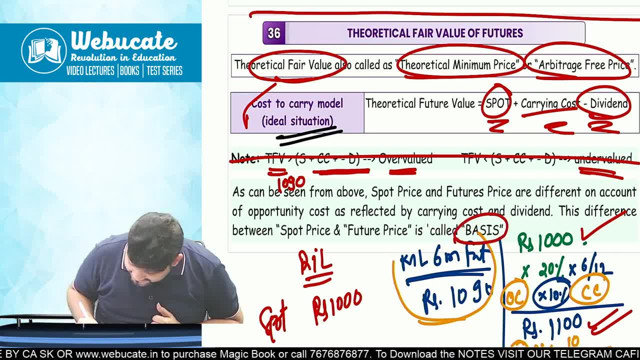 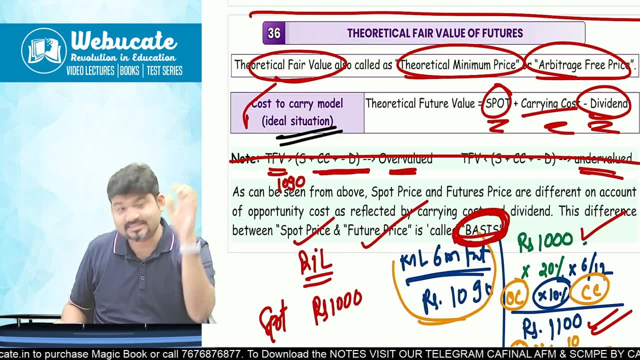 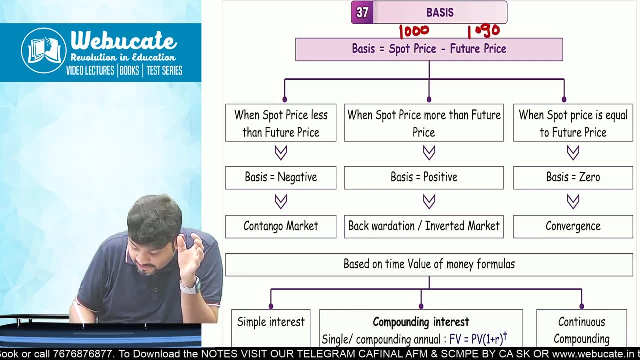 basis. we call this as the basis. we call this as the basis. the difference between the spot price and futures price is called as the basis, gotcha everybody? yes, sir, so spot price was 1000, future price was 1090, as we did in this example, which was: price was 1090. 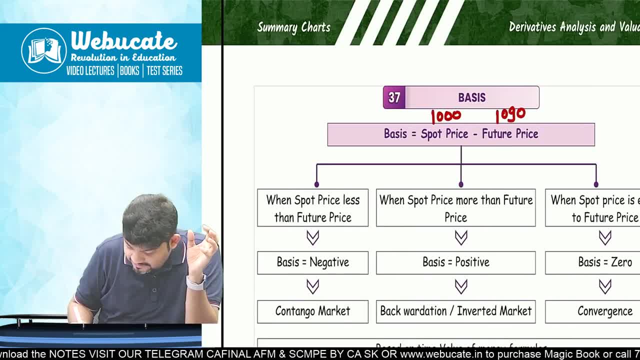 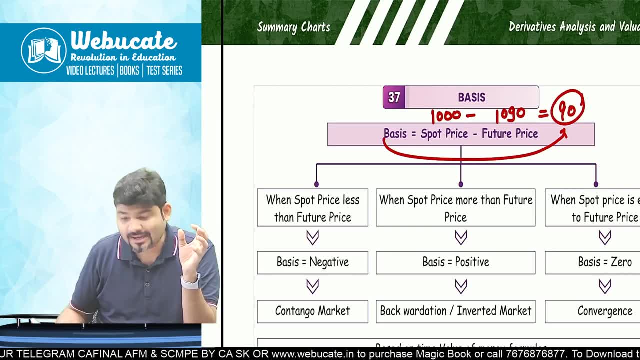 you, you, that's it. this is your futures price. basis will be 90. basis will be 90. now there can be three situations. in some cases spot is 1000 but the future price is 950. maybe on account of high dividend, maybe on account of a reverse rate of interest, like in japan there. 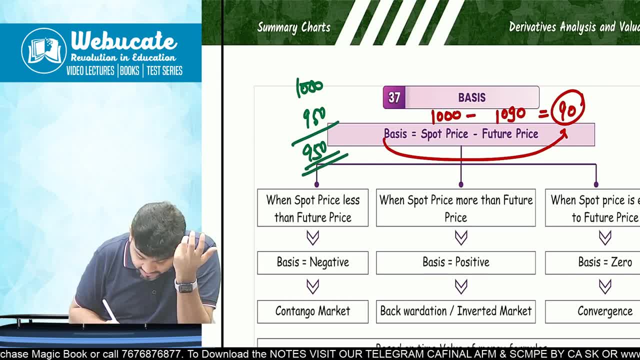 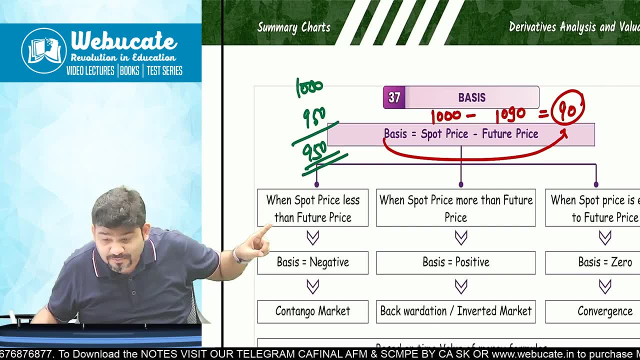 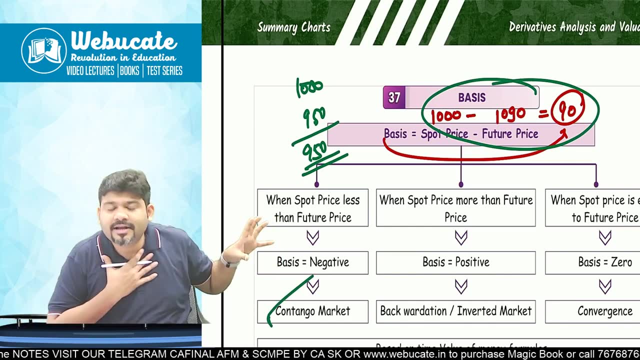 is negative rate of interest, so it could be any reason- will become 950, are you understanding guys? so if spot price is less than the future price, which is our scenario, we will say it is a contango. market basis is negative. it is india. in india there is a. 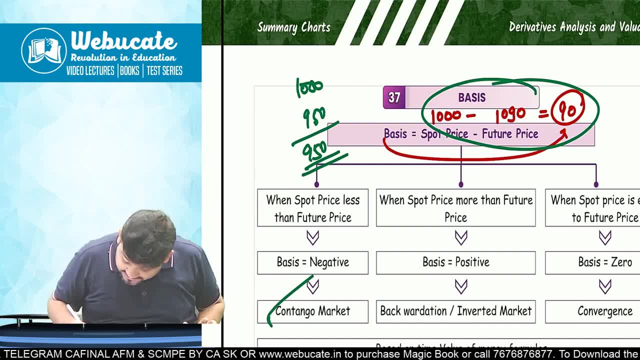 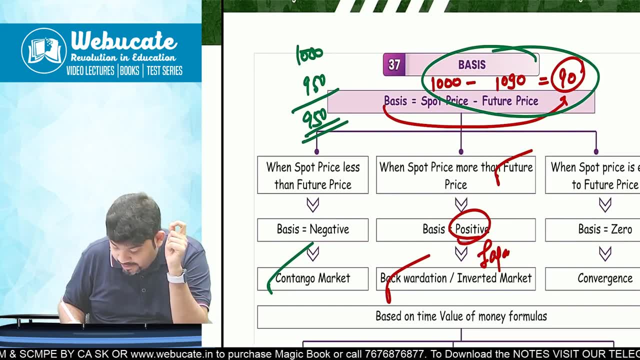 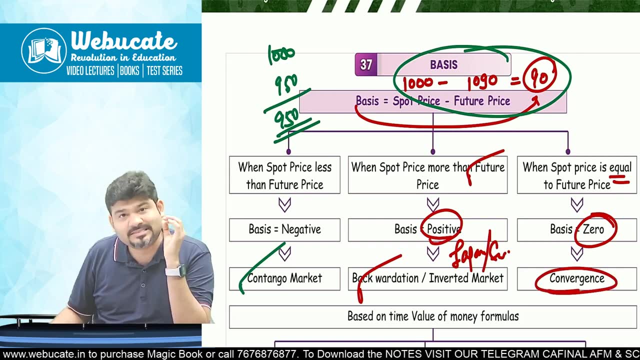 contango market. when the spot price is more than the future price basis is positive, it is called as a backwardation or inverted market. you can say japan or switzerland are the examples of this. but when it is equal, then in that case the basis is going to be zero. it is going to be a convergence. 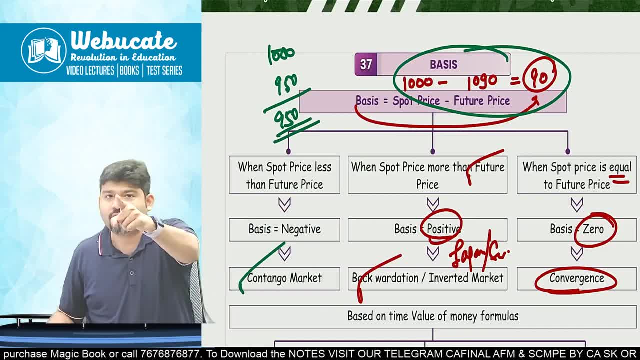 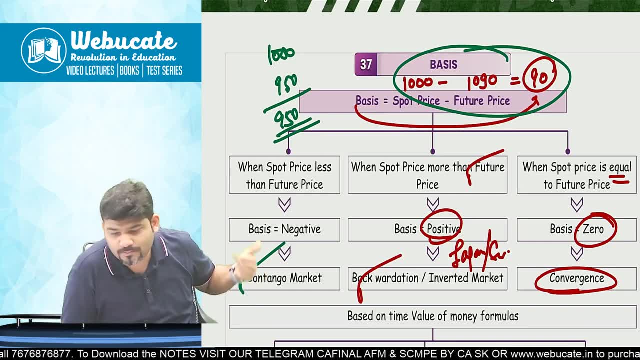 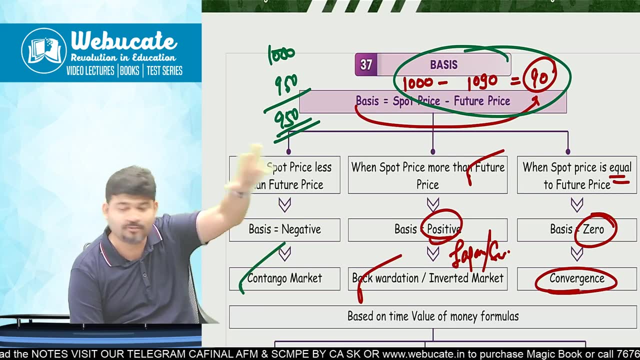 market. this is a sure shot question for your mcqs multiple choice question. sure shot question: expect contango backwardation convergence. india is a contango market. futures price will always be higher than the spot price. you can watch it out in money control in any of the uh zero, the any of. 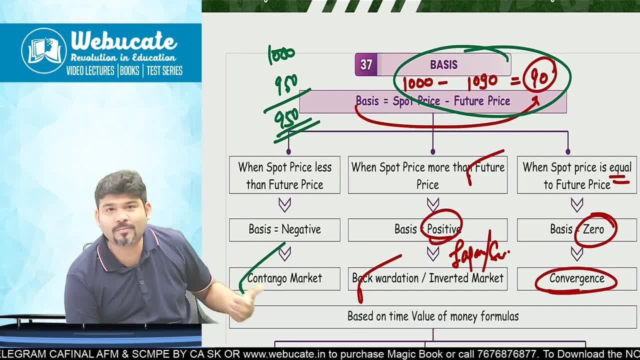 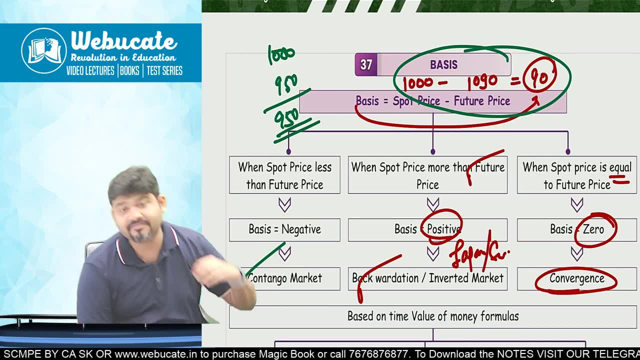 the apps that you know. try it out, watch it out. india is going to be a convergence market. this is a contango market. basis is always negative. when futures price is less than the spot price, basis is positive backwardation market, which can be a case of a japan or a switzerland. and then we have 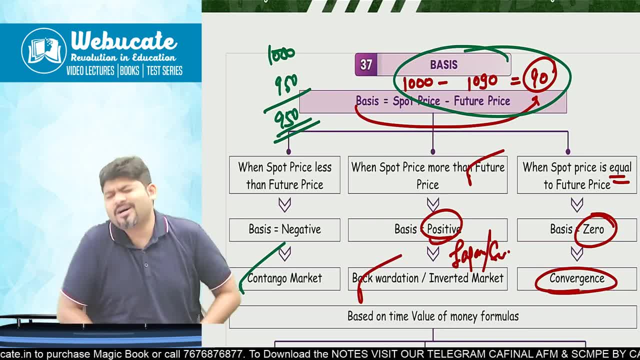 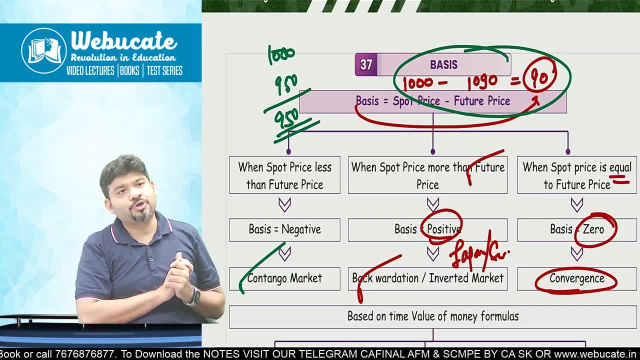 when spot price equal to future price basis is zero, when the almost the interest prices are very low and there is also a dividend which is there, which could be a case of a usa or a uk developed market that is called as a convergence market. got it everyone? yes, sir. 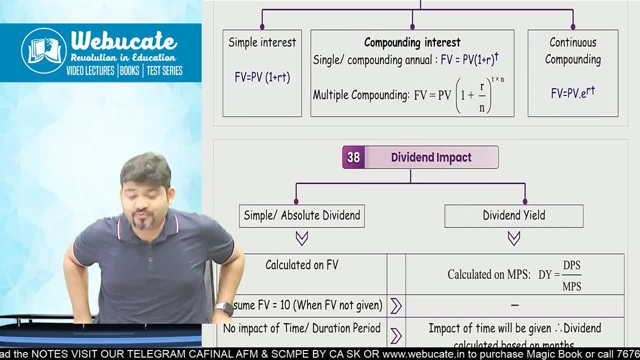 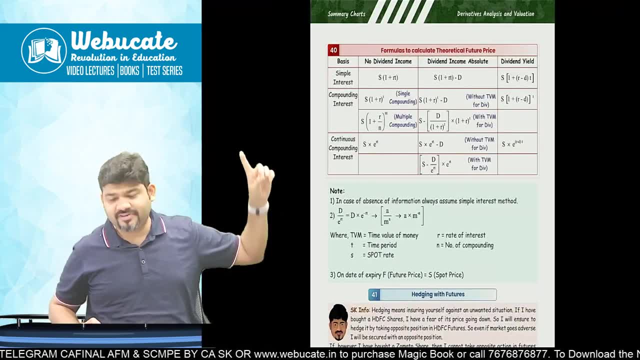 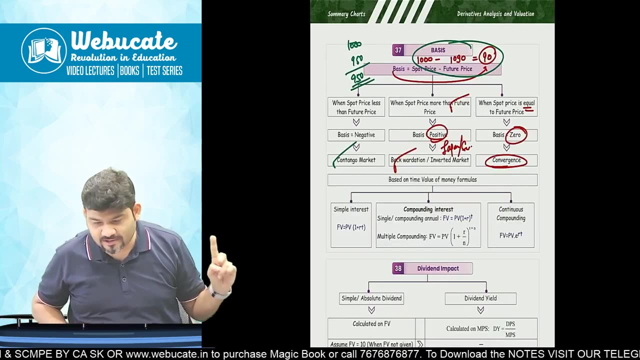 now calculation of theoretical future price. but you don't have to worry, because i have made it all easy in this with a whole box level formula sheet. yes, whole box level formula sheet is available with us and, trust me, it will make things very, very easy for you. let's start now. the first. 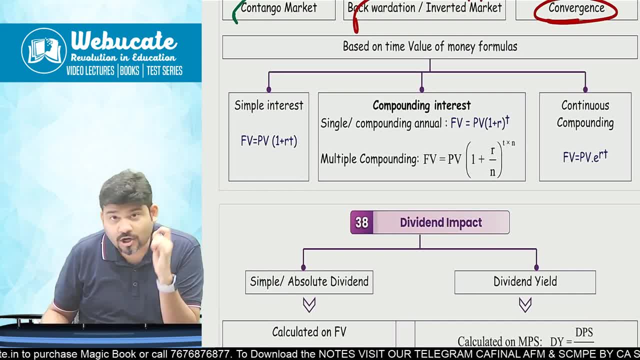 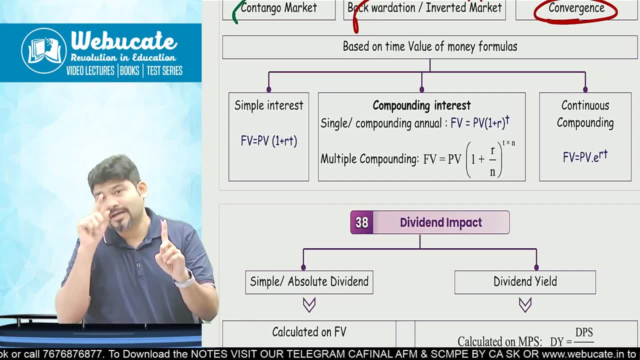 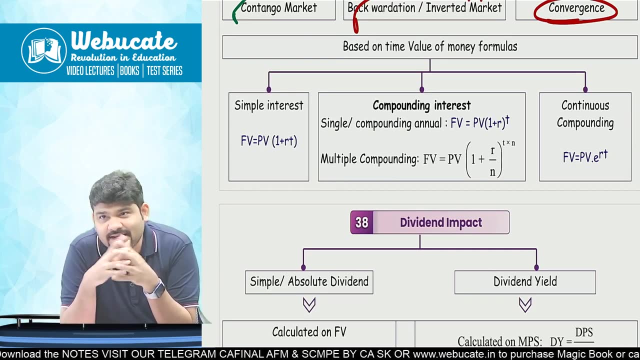 is the calculation of theoretical future price. now, how do you calculate theoretical future price, spot plus carrying cost, less dividend plus carrying cost? carrying cost is based on the interest. interest could be a simple interest, compounding interest, continuous compounding interest, so so so all of these three scenarios will have to be taken care of. simple interest: 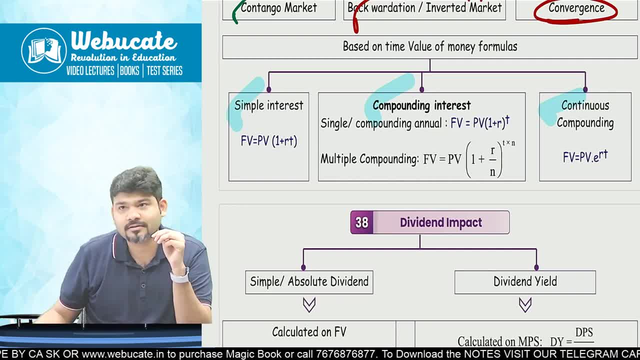 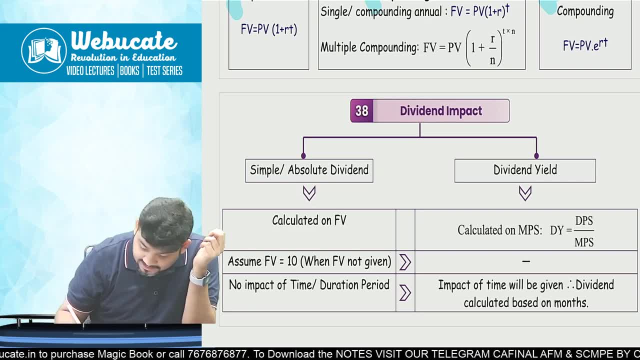 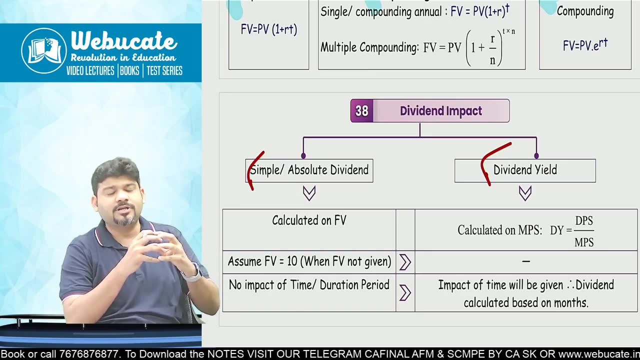 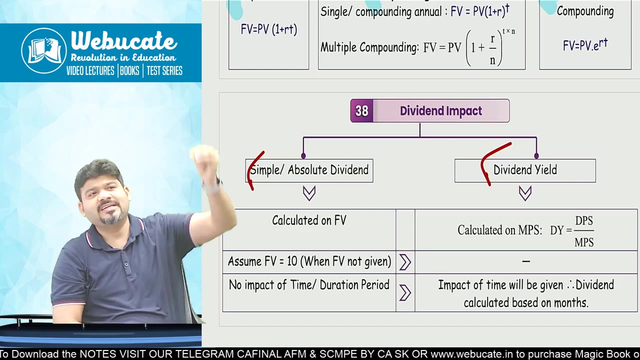 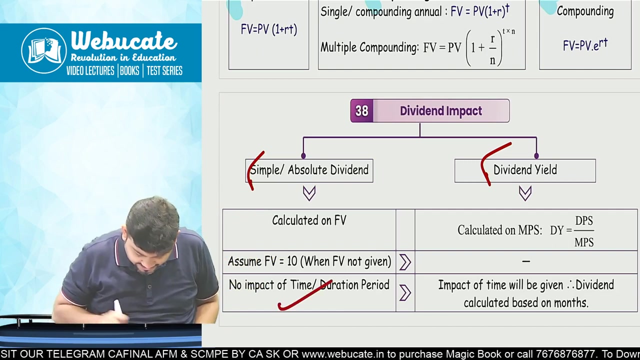 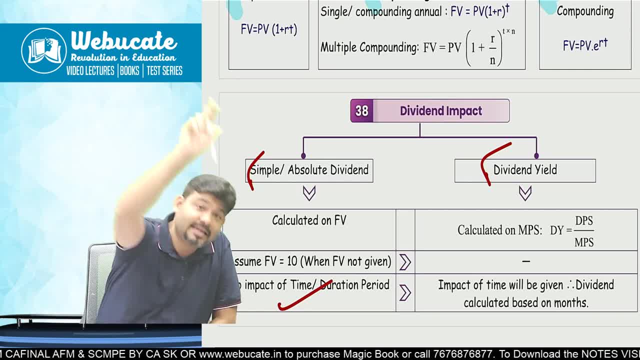 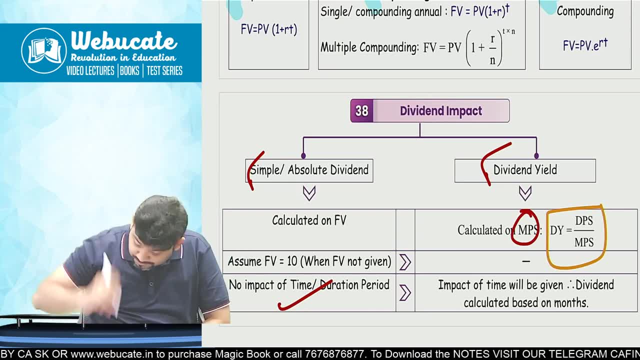 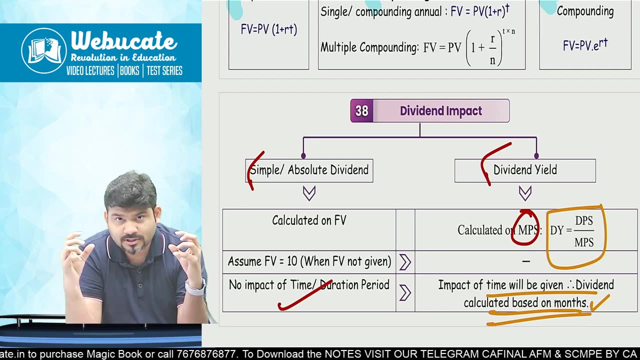 duration or anything, but in case of dividend yield, it is based on market price per share. so dividend yield is dps upon mps. impact of time will be given and dividend will be calculated based on once. this is what you will have to remember. so dividend will be of two types: one: 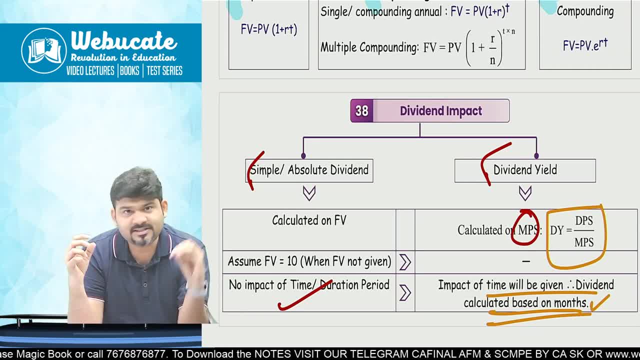 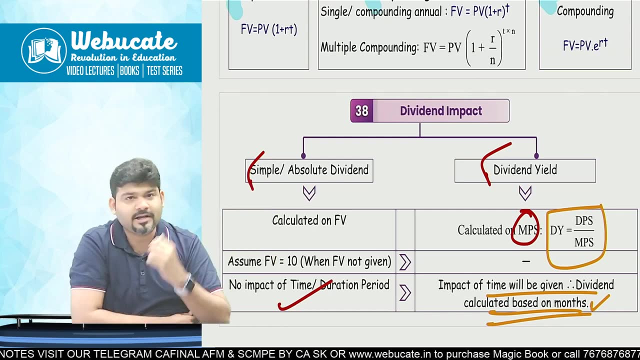 absolute dividend, pure numbers. 10 rupees dividend is paid or 20 dividend is paid on face value. even if face value word is not used by default, it will be assumed that if nothing is given it will always be on face value. so if it is on face value it is always simple: or absolute dividend. so say 20 of 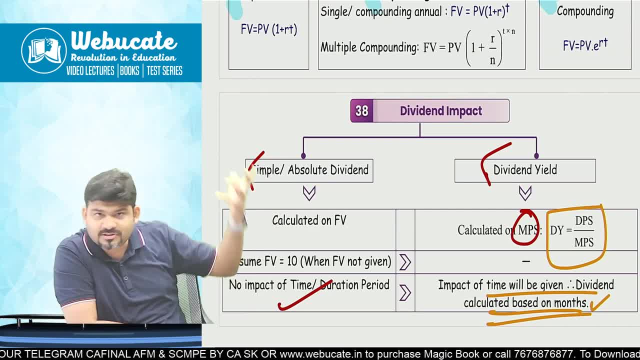 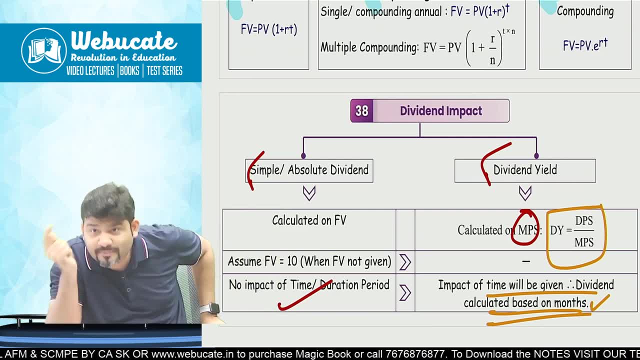 10, 2 rupees is your dividend. so simple, absolute dividend will be reduced that amount, no impact to be given of months or anything. but if it is a dividend yield, it will be based on market price, dps, upon market price per share and in that, the impact of months or years or, as the case may be, 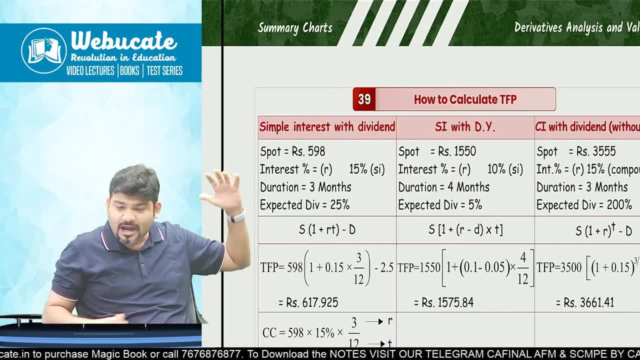 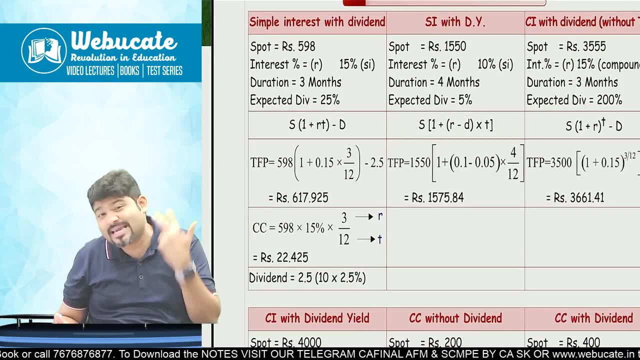 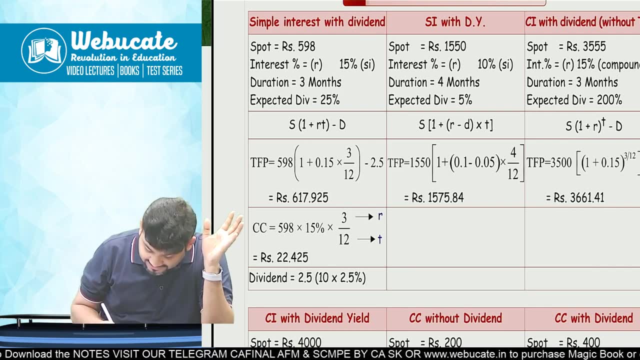 should also be given. so this is your dividend impact. now we will try to understand the yes, yes, yes, the interest, or the opportunity cost, or the carrying cost impact of all of the situations which are here. suppose, if it is a simple interest with dividend, so spot price is 598, interest is say: 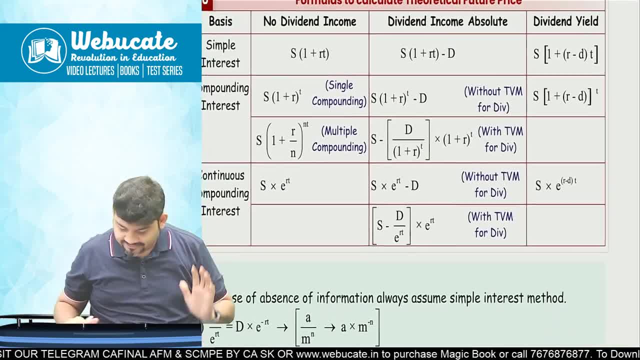 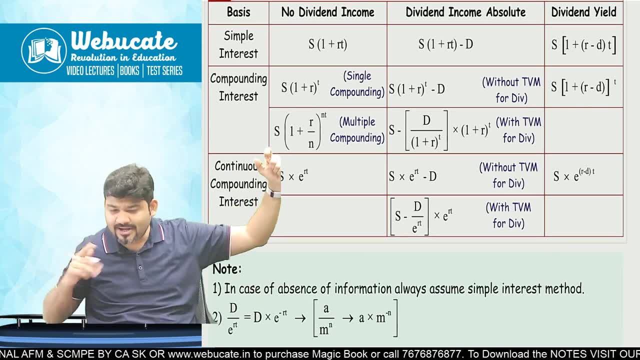 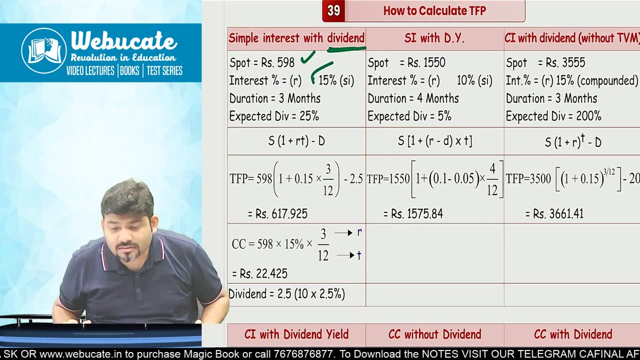 15, all of the cases i have taken here and then for your examination. i made this. all you have to do is just pick, as the question says. pick it up from this box, apply it gone full marks in your pocket. yes. so here we are. how to calculate the theoretical future price: simple interest with dividend. 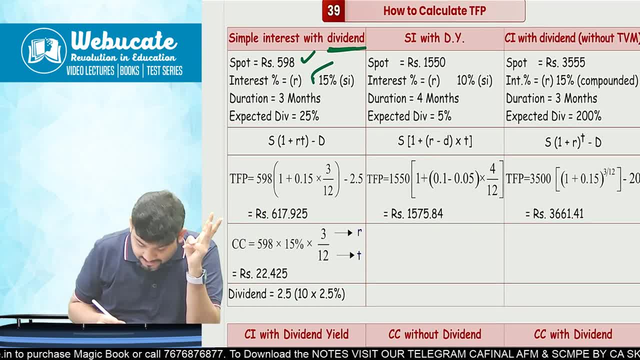 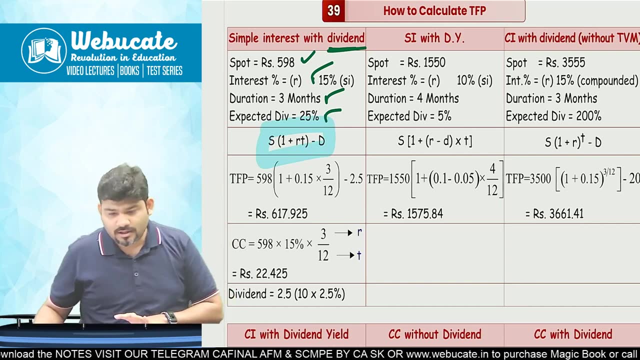 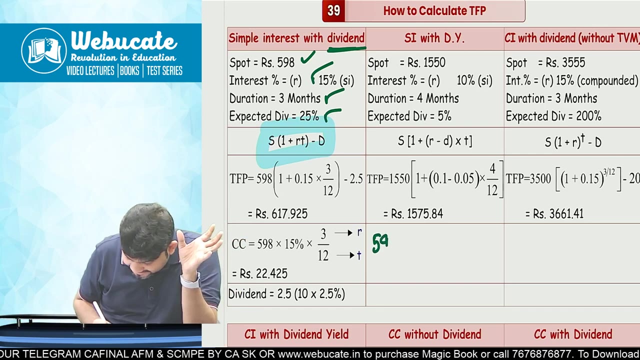 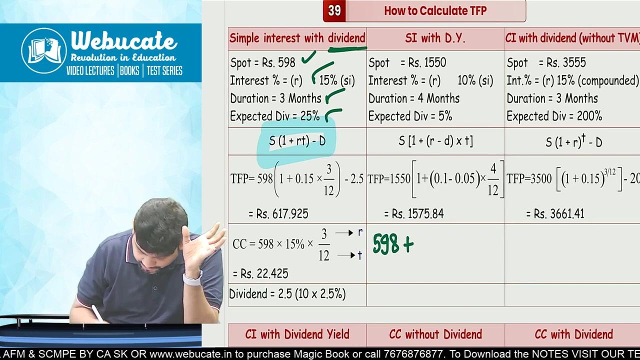 spot is 598. interest is 15. duration is three months. expected dividend is 25 percent. expected dividend is 25 percent. in this case, how will you calculate the? in this case, how will you calculate the theoretical futures price- let's try it logically- plus carrying cost. so what's the formula? it is spot. what's the formula? it is spot plus carrying. 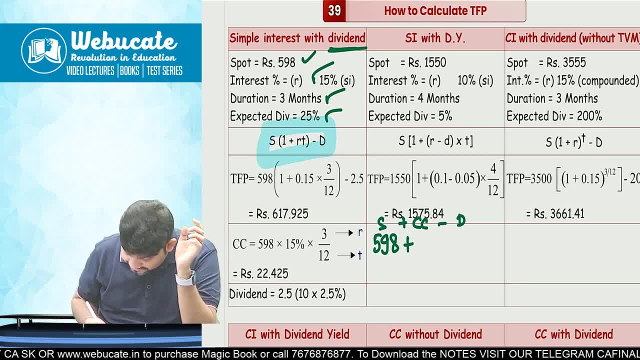 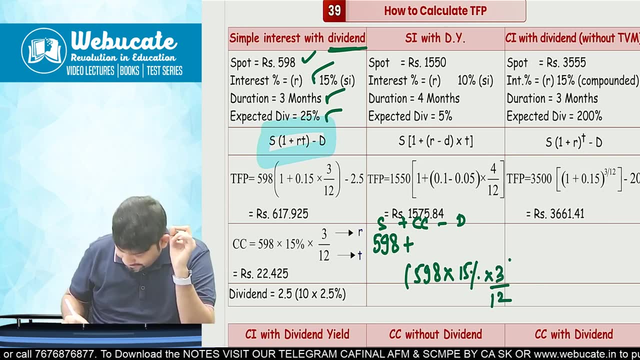 cost less dividend. what is the carrying cost? carrying cost is going to be 598 into interest, which is 15 percent into three months, so into 3 by 12, right? all right, this is your interest amount. yes, so plus carrying cost, what? how much does it work out to 598 into 15? 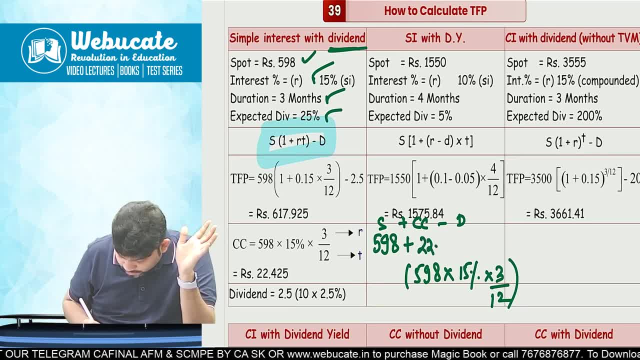 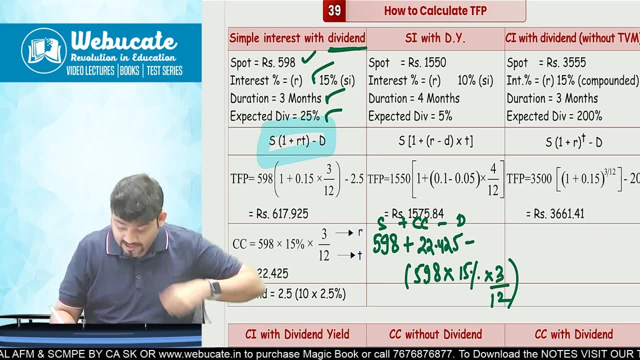 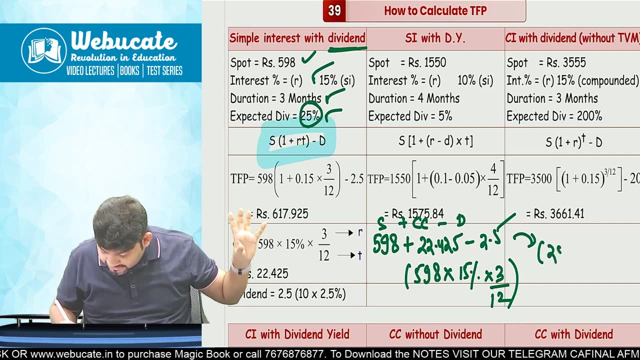 into 3 by 12, so it is 22.425 less, say, dividend. in this case, any dividend is given expected dividend: 25 on face value, if nothing is given by default face value. so say 2.5. how did this come? 25 percent of 10 rupees will be your face value by default, so 2.5. so what's the? 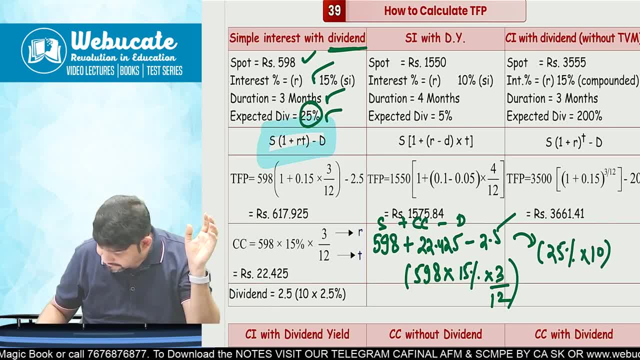 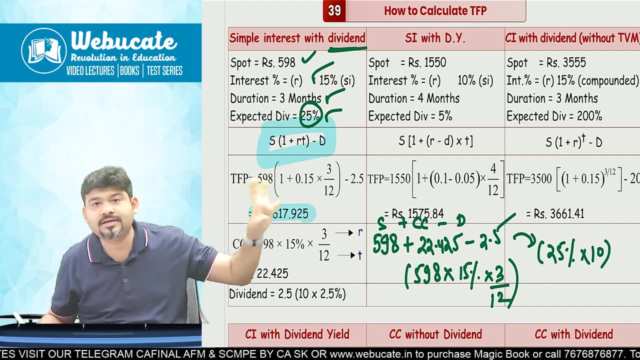 the answer: 598 minus 22.425, sorry, plus. so 598 plus 22.425 minus 2, 2.5, so this will be 617925. and here we can see. but now, instead of solving it, this whole big method, instead of doing it like 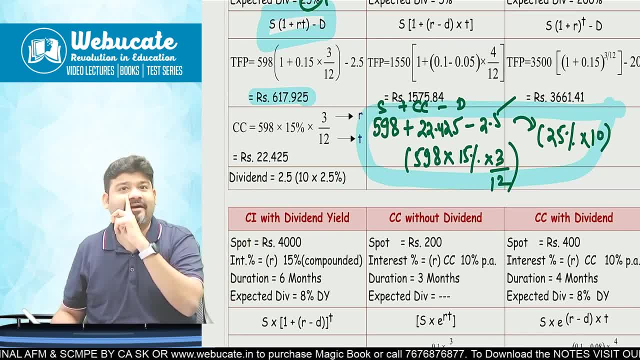 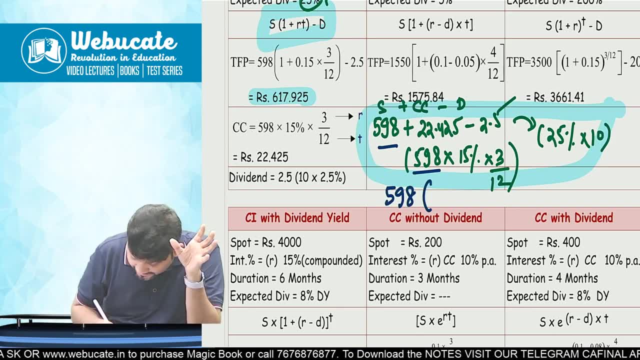 this. there is a shortcut that we have. there is a shortcut that we have. what will we do? so 598 let's take in common. okay, sir, this will become 1 plus 598 is common, only so common into what is 15 percent rate of interest, into time is 3 by 12, into t the whole minus d. what is 598? can i say it? 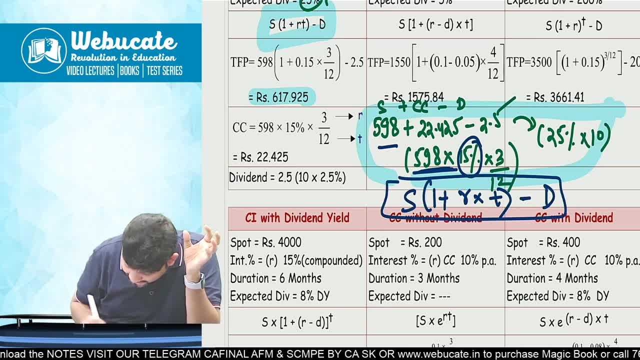 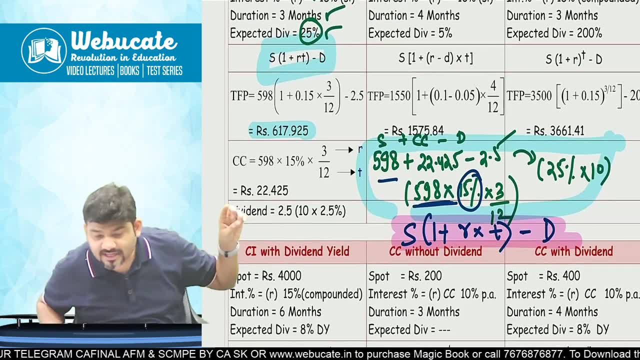 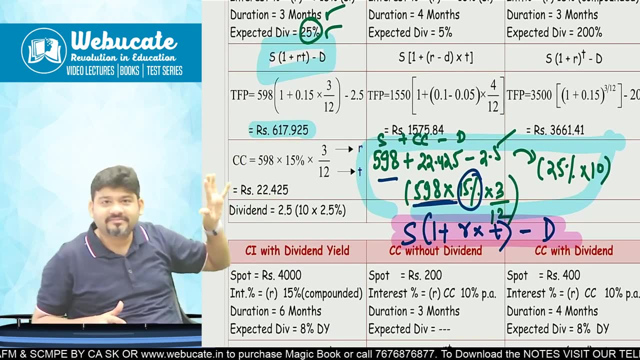 is nothing but spot. so here we get the first formula logically. here we get the first formula logically, and that is: s into 1 plus r t minus d, s into 1 plus r, t minus d. are we clear, everybody? are we clear everybody? so this is your. 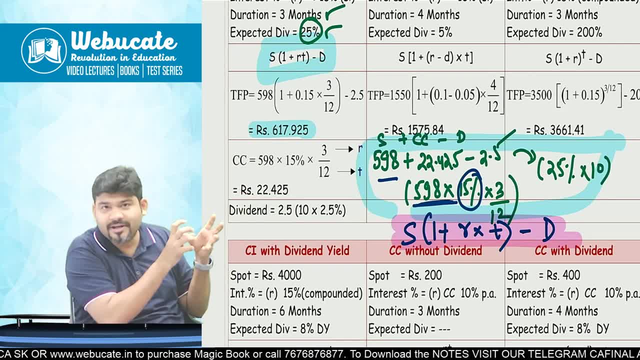 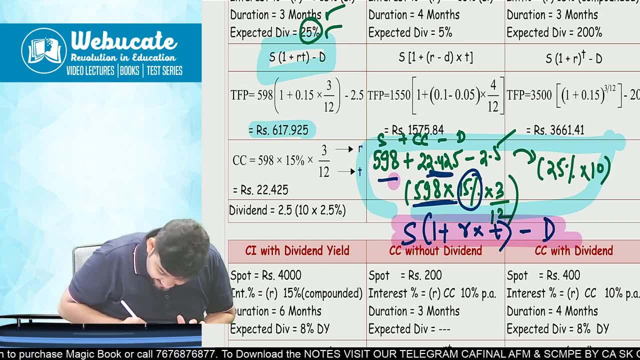 first formula again. did you get it 598 in common? then again, here we have to write 598, so this will become that 1 plus 598 is there by default, into r, which is 15 percent, into t, which is 3 by 12 s. 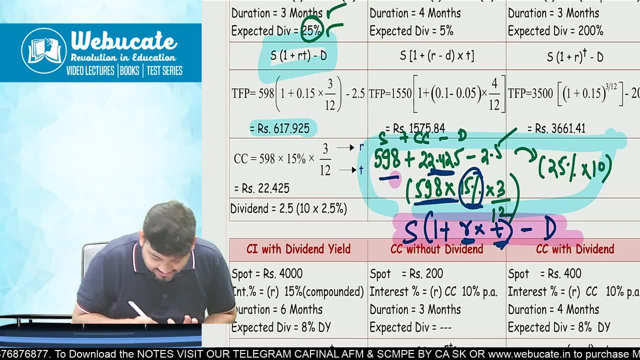 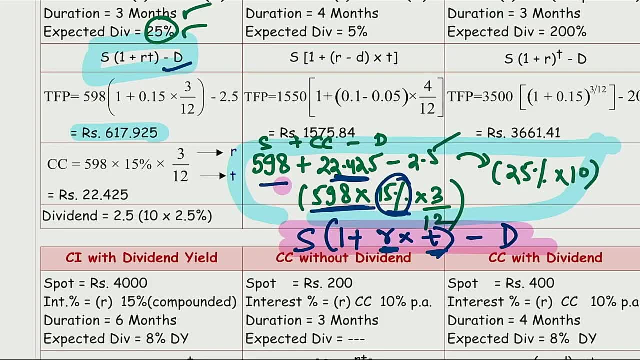 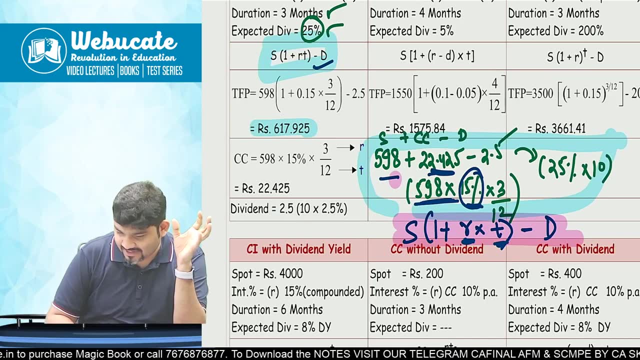 into 1 plus r, t minus d, and here comes my first formula. in the same way, can i say now we will keep on applying this to all the other things? wait, i'll take you through now. this was a plain situation. a plain situation like a- a. 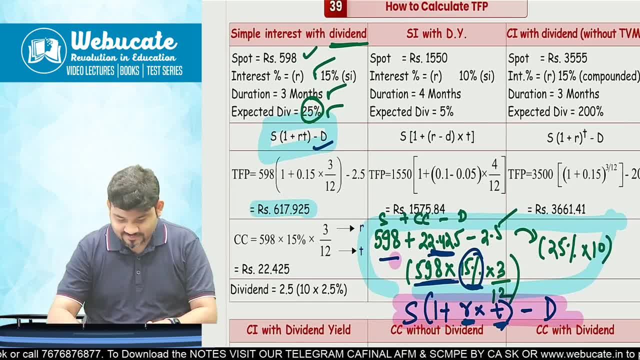 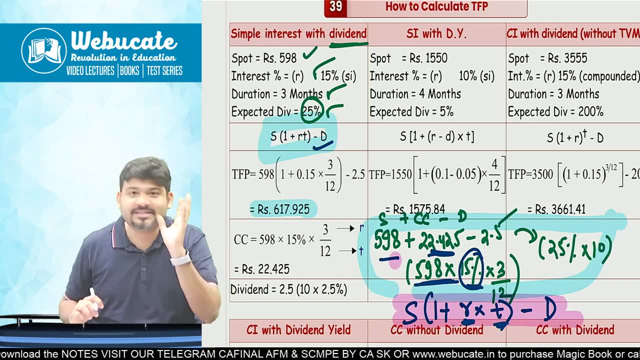 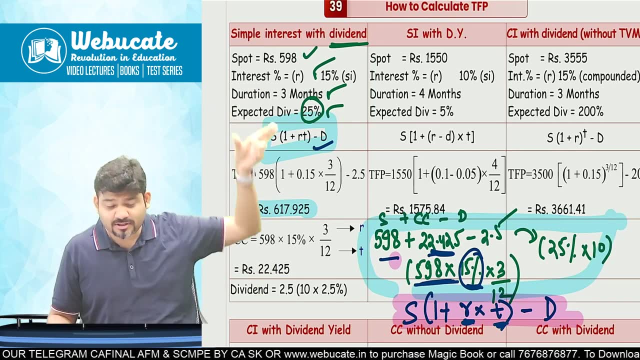 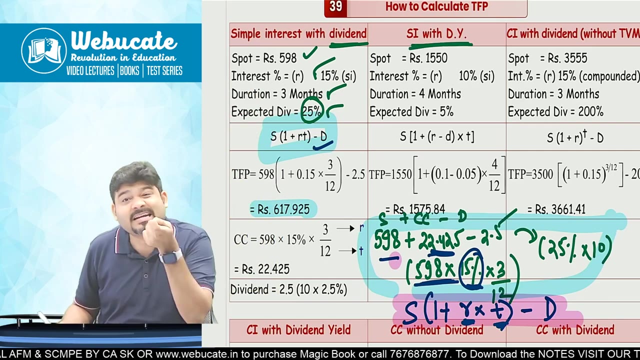 simple interest, a spot interest at simple rate, with dividend. you'll be happy to know that 8 out of 10 sums are based on this format: simple interest with dividend. now, second concept that i'm going to take is simple interest with dividend yield. the formula changes only with one aspect, and that is: 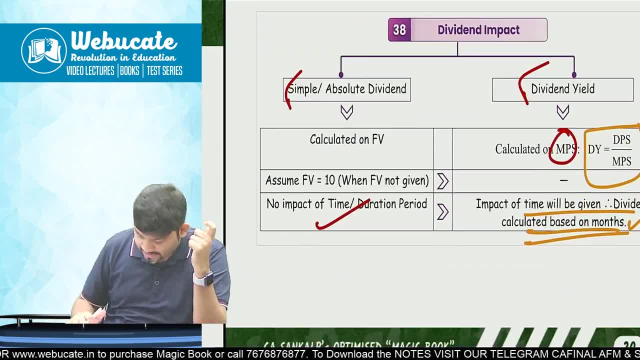 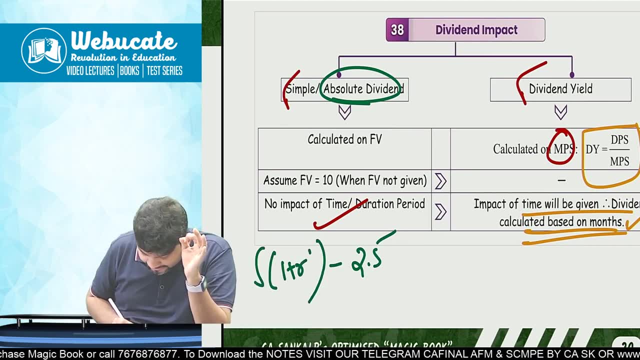 the dividend aspect. see, i told you all here, in this case the dividend is absolute. so whatever dividend that you have calculated, you will reduce it from that s into 1 plus r, t minus d. but in case of dividend yield it is dependent on market price. it is dependent on, so market price. basically, it is dependent on. 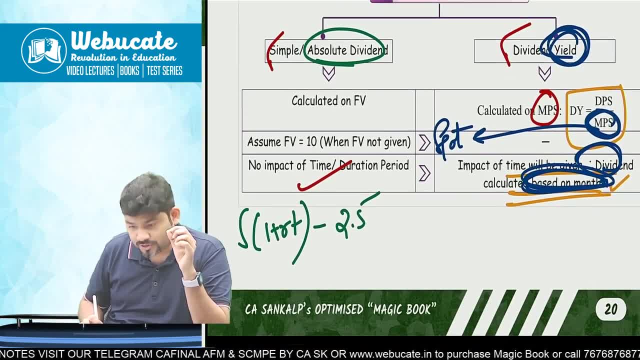 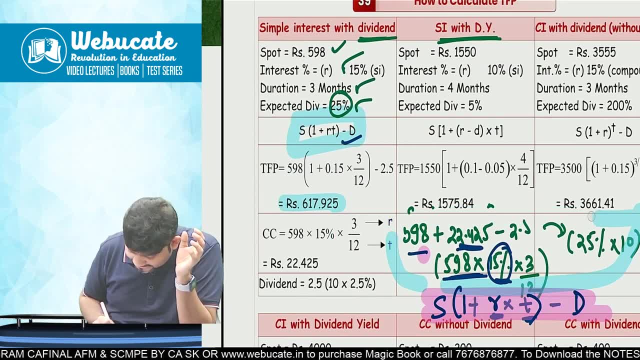 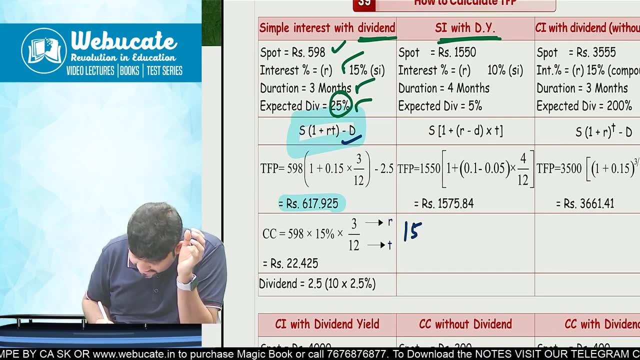 the spot rate, it is dependent on the number of months. so here, when we calculate the spot, uh, when we calculate the interest, suppose if i remove all of this, suppose if i remove all of this, then what is going to happen is spot, which is going to be, say, 1550, plus there is a carrying cost. what is the carrying cost? it is: 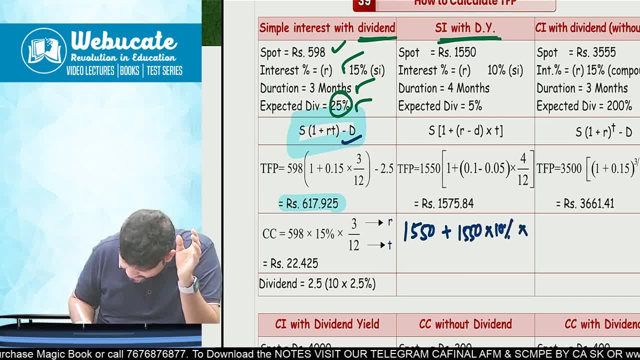 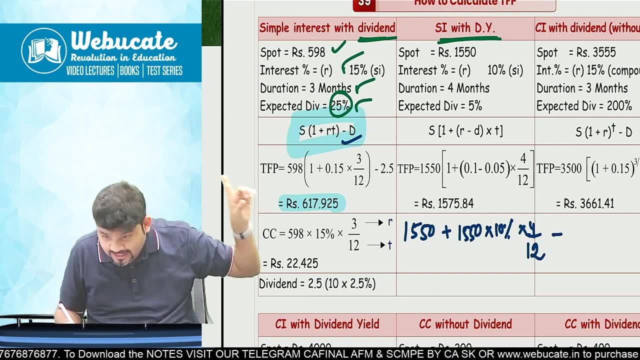 1550 into 10 percent, into 4, by 12, right minus, listen now minus dividend, say expected dividend 5 percent. they will have to deduct 5 and 0. so in the end they are not going to be able to give you the interest. so if i remove all of this, suppose if i remove all of this, then what is going to happen? 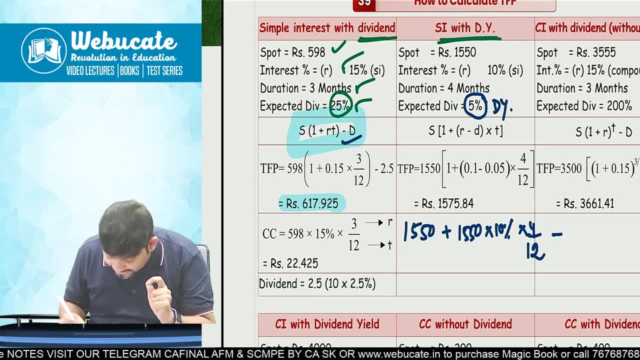 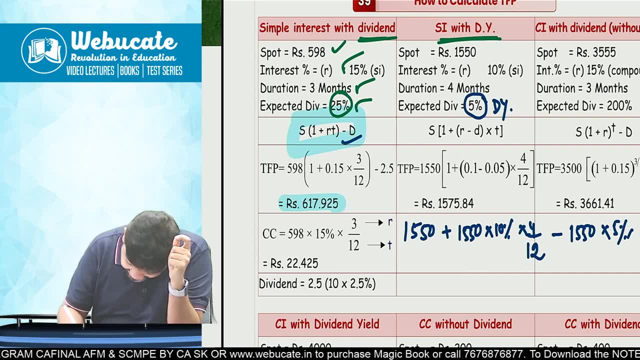 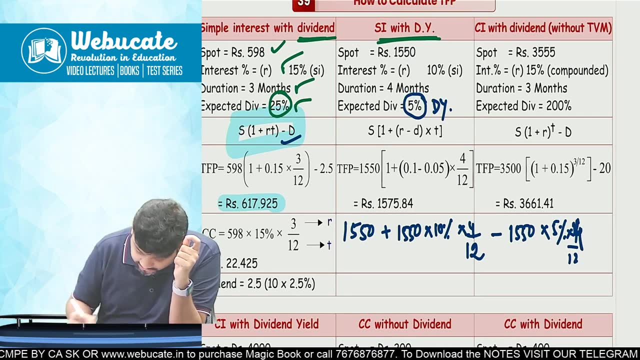 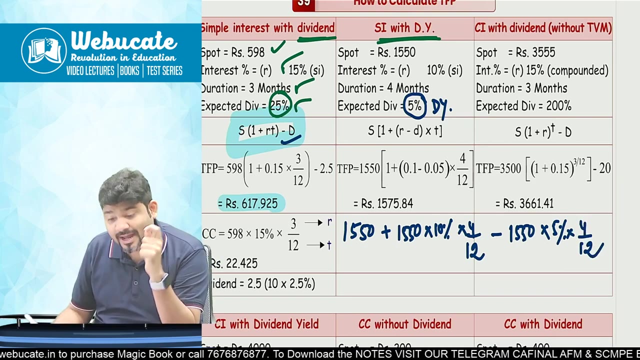 to write here dividend yield. so now, how do you calculate this? it will be 1550, market price, multiply by 5 percent. multiply by 4 by 12. hello, multiply by 4 by 12. so here, yes, this 4 by 12 is to be reduced. so multiply by 4 by 12. now, what do you see here, correct? so see, 1550 is still in. 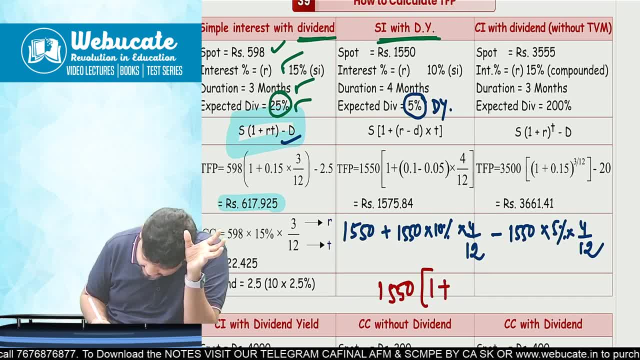 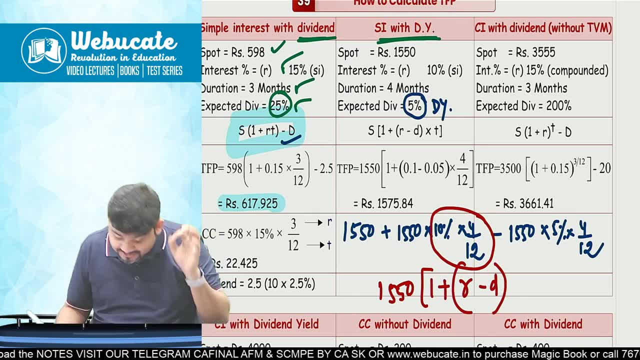 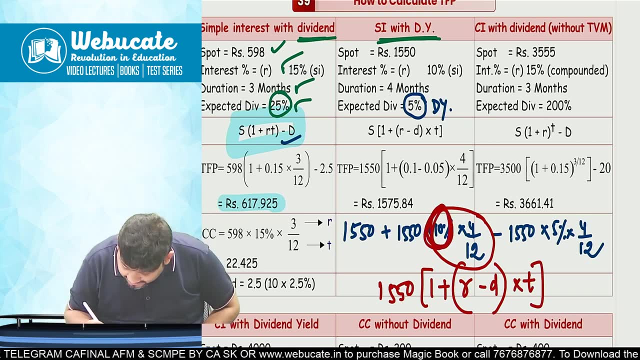 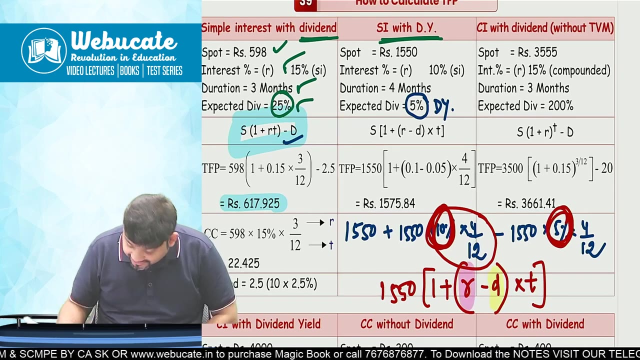 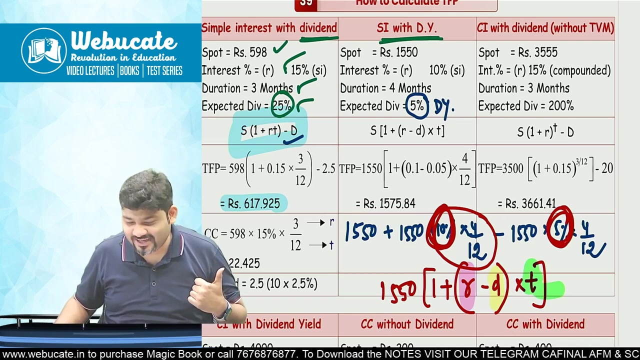 common: 1 plus r minus d, absolutely correct. multiply by 4, by 12, which is t, so r minus d, r, which is your 10 percent d, which is your 5 percent, into t, into t. hey, are you clear everybody? so it will become spot into 1 plus r minus d into t, and that's what your theoretical. 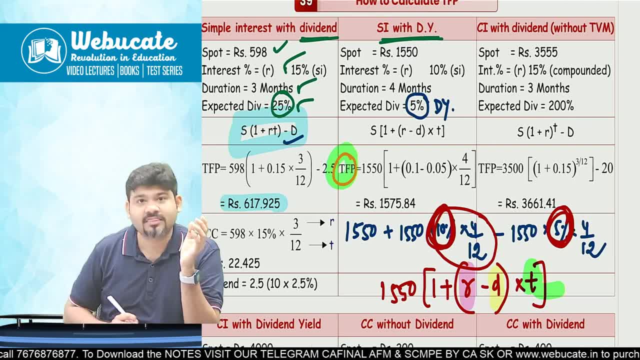 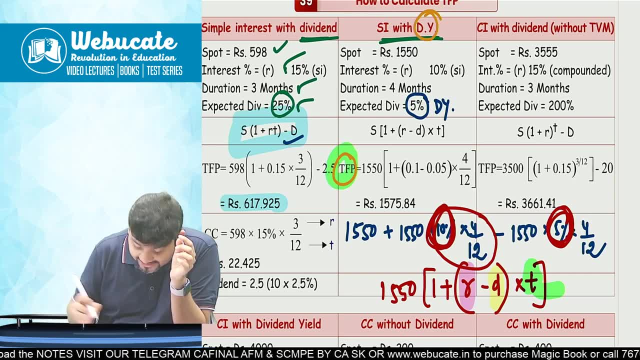 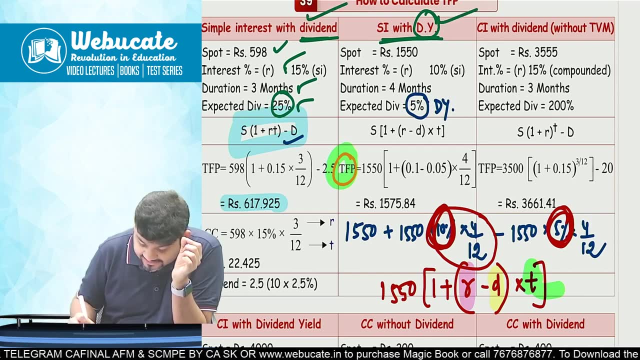 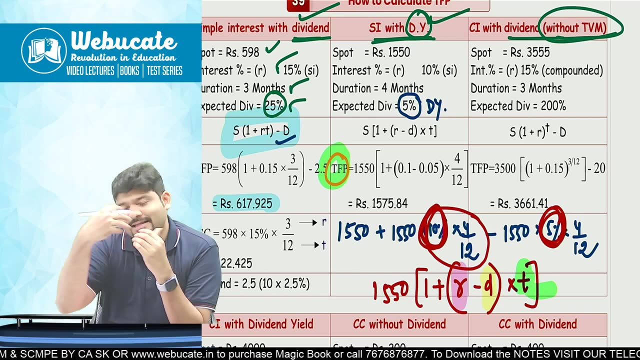 future price calculation says theoretical future price calculation says simple interest, but with dividend yield. simple interest, but with dividend yield. so this is with absolute dividend, this is with dividend yield. now compounding interest with dividend, but without time value of money. so now let's come to compounding interest. now compounding interest. 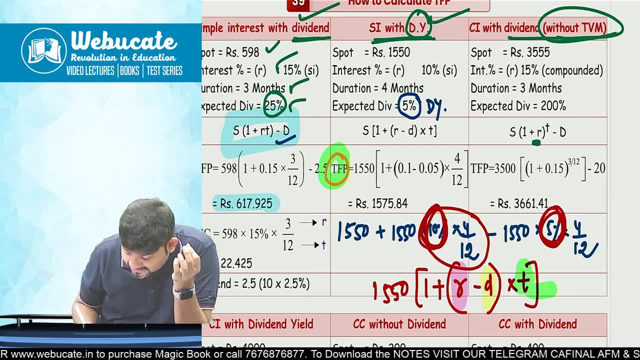 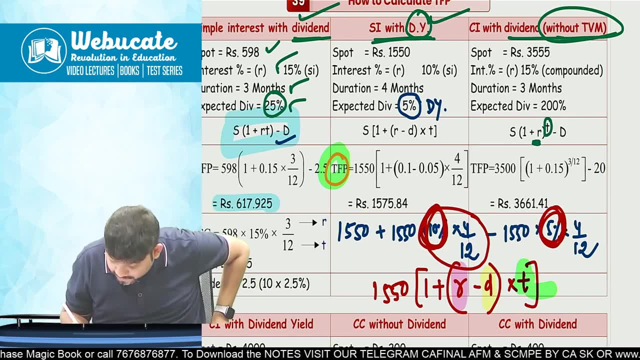 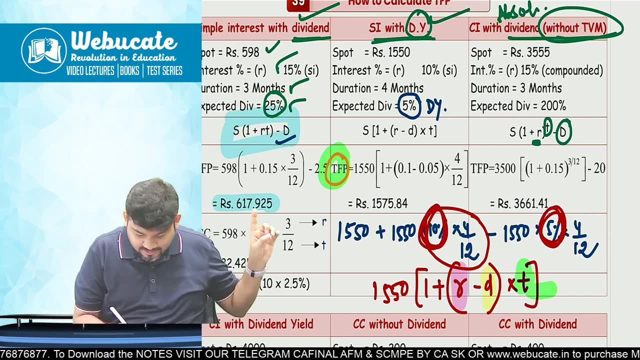 with dividend. same thing. the only difference here is 1 plus r raised to t, because it is compounding minus d and instead of suppose, if this is not absolute dividend, this is compounding interest with absolute dividend. what is the formula now? i please confirm, are you clear with this explanation? one spot into 1 plus r minus. 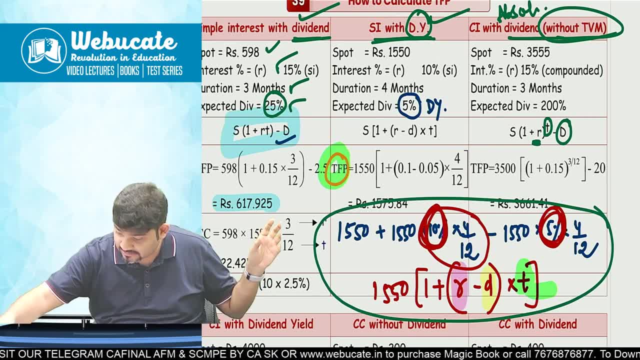 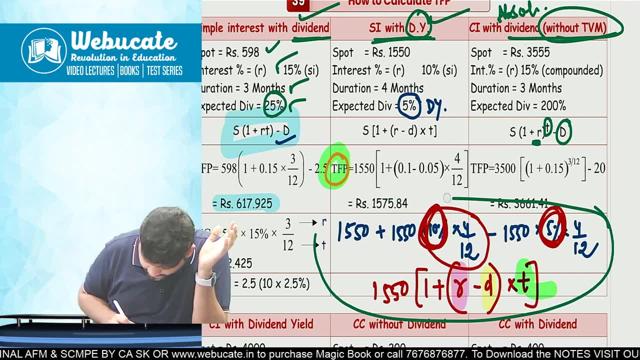 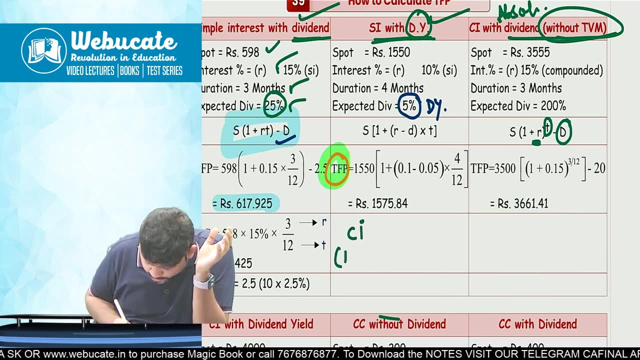 d into t. are you clear with that explanation, guys? tell me, tell me, tell me, everybody. yes, yes, sir. okay, now comes compounding interest with absolute dividend. so what is it going to be now we are able to do it on our own absolute dividend. what will it be? logically, spot plus. 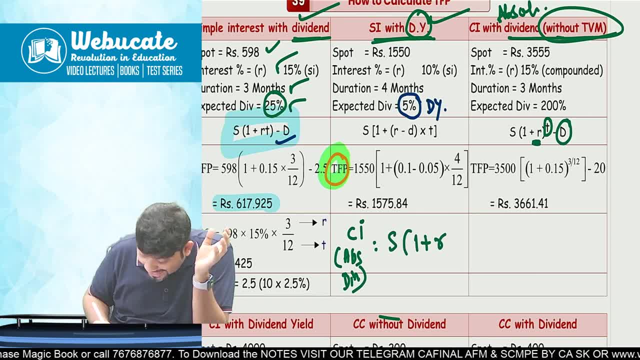 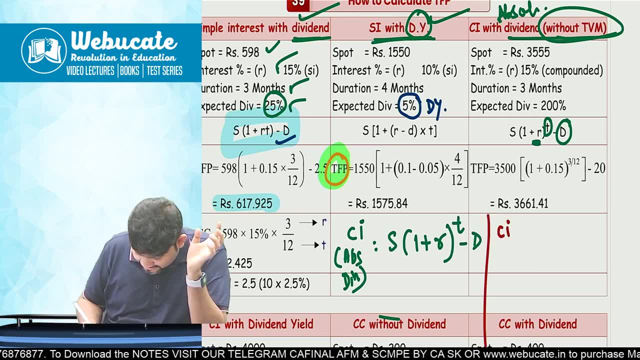 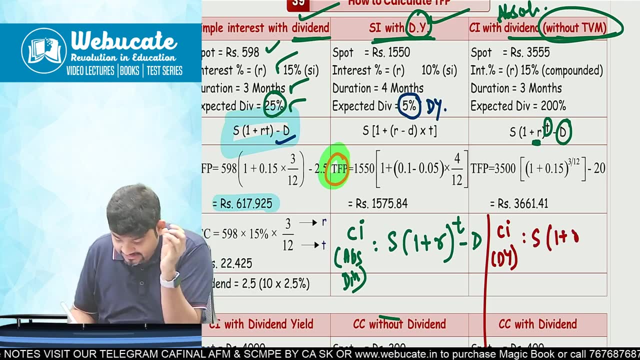 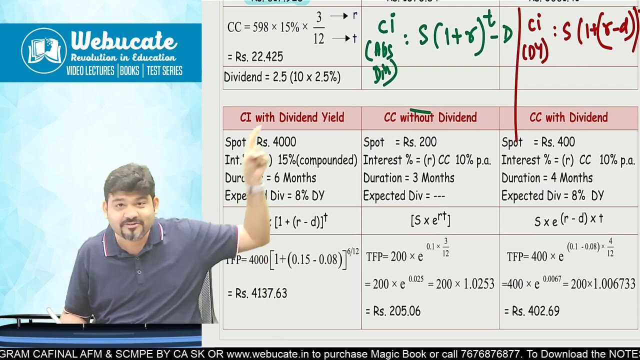 sorry spot spot into 1 plus r raised to t, minus d gotcha. and then there is compounding interest with the dividend yield, which will become s into 1 plus r minus d raised to t. that's it, and see here: compounding interest with dividend yield r minus d raised to t. now we are able to. 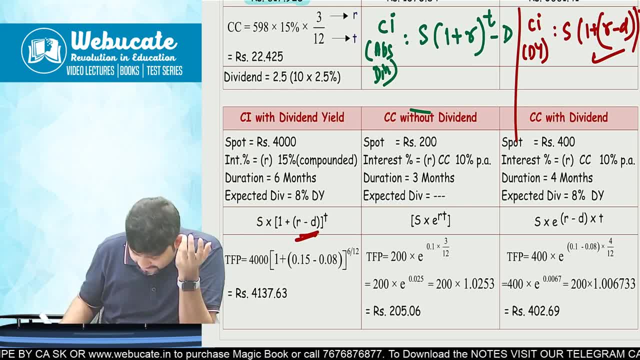 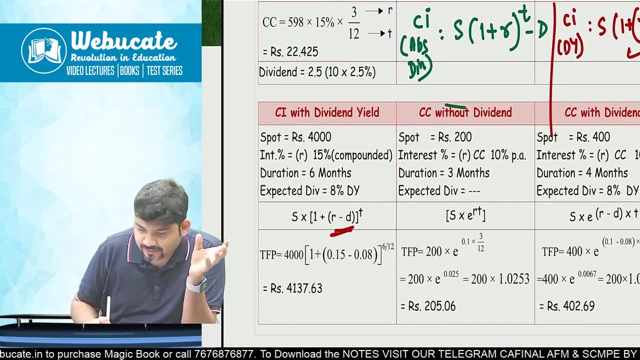 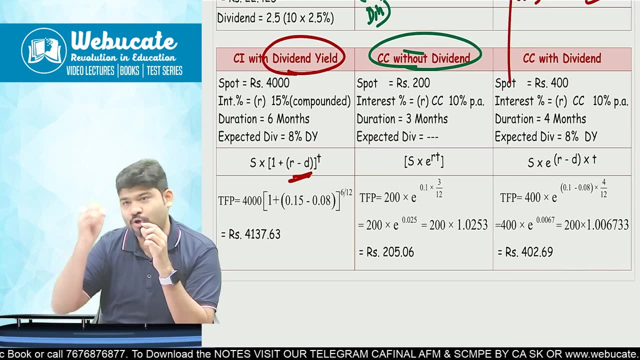 calculate it on our own compound. then there is continuous compounding. so this is compounding interest with dividend, compounding interest with dividend yield, and now we have continuous compounding without dividend and with dividend. so here it is. we all know compounding. continuous compounding is e raised to r t, so your first will be e raised to r minus d raised to t. so 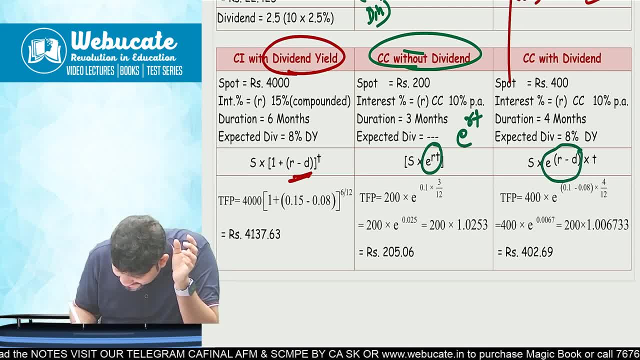 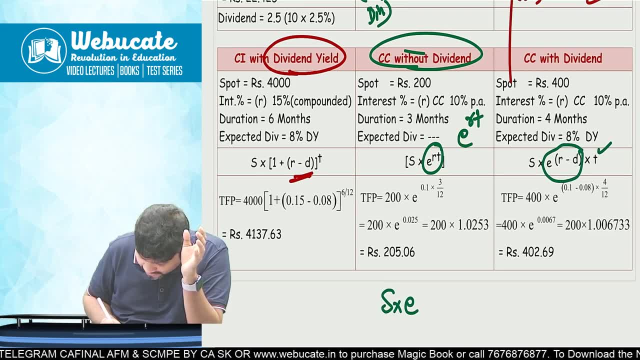 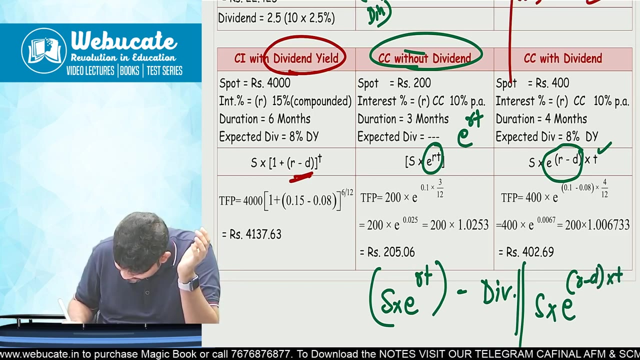 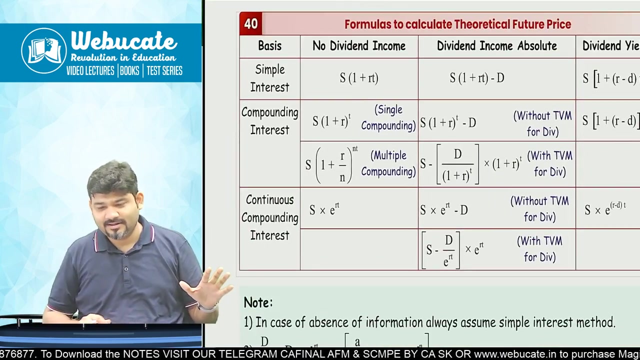 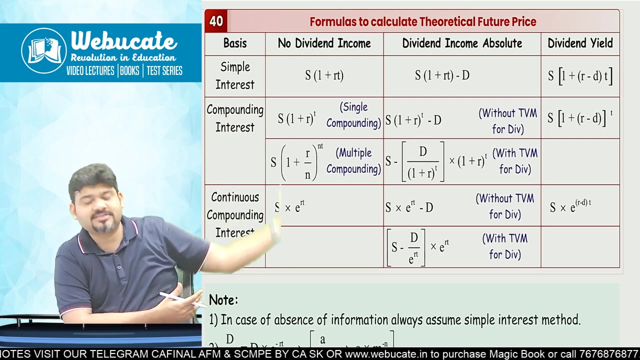 r t and the other will be e raised to r minus d into t simple. suppose if there is dividend, simple, dividend, so s into e raised to r t minus dividend, and if it is dividend yield, s into e raised to r minus d into t everybody done. now all of this, what i have explained, is easily available in the form of this table. 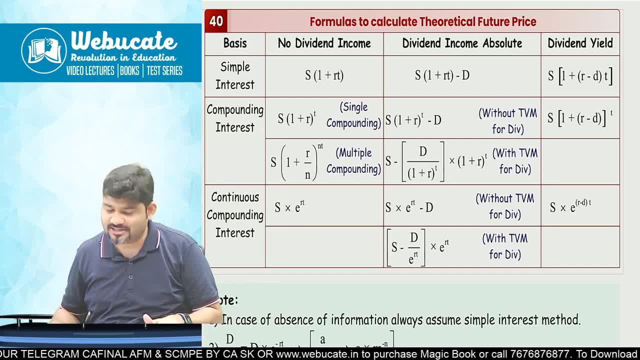 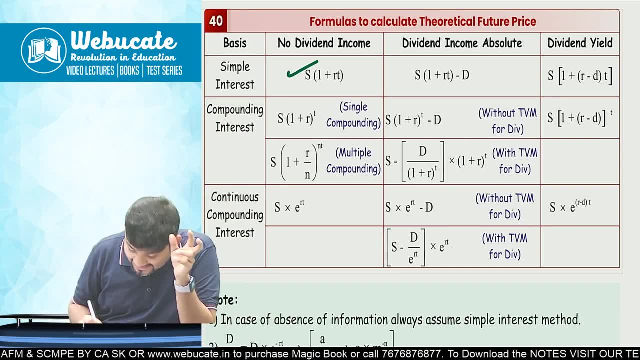 during the examination. all you have to do is just follow this table and you will be through. simple interest: no dividend income. one plus r t. one plus r t minus d. okay, 1 plus r minus d into t Compounding interest. Single compounding. 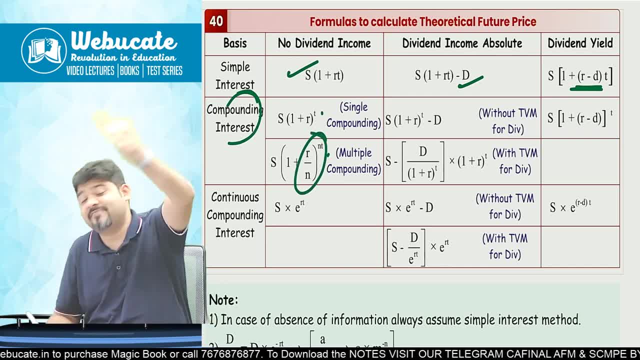 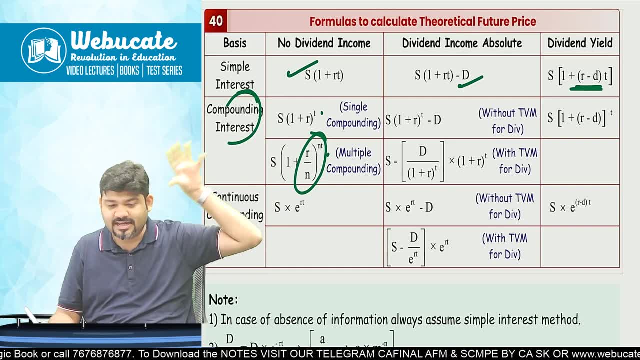 There is something called as multiple compounding. Please listen to my time value of money lecture. I have made a lecture on time value of money. Please listen to that lecture. You will get to know what is multiple compounding. So if that is the scenario, this is what you will use. 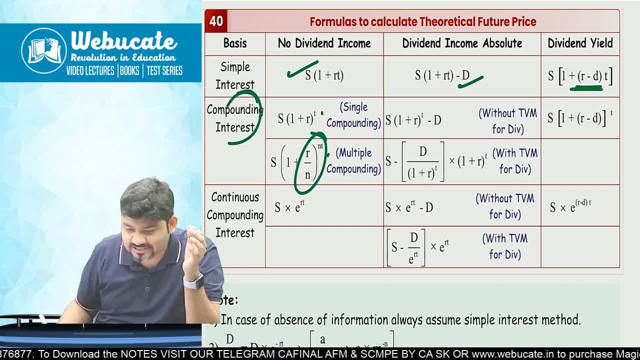 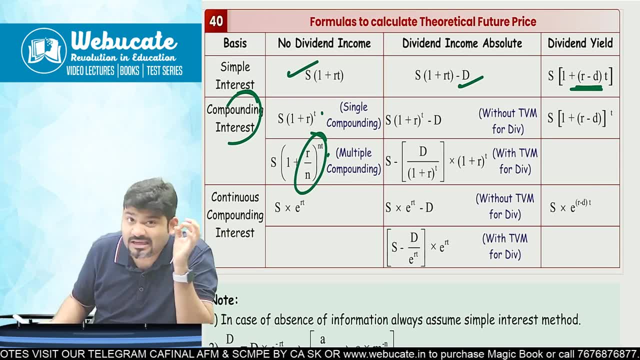 Obviously it is a revision lecture. I cannot get into the depth of each and everything, But yes, definitely you will get this table, this magic book summary table, And will really be helpful if there is a question on theoretical future price, Which can be asked in MCQ as well. 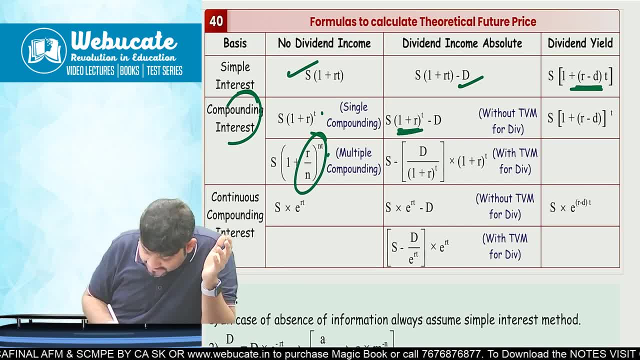 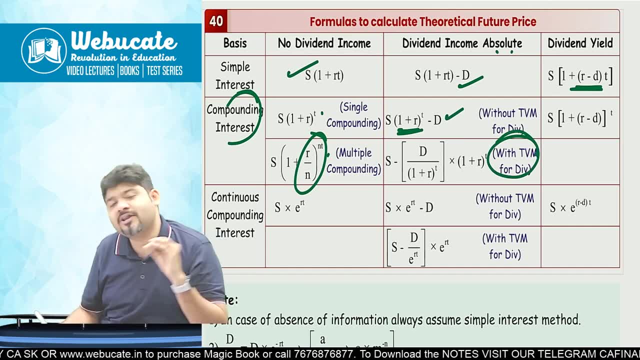 Beware, Yes, Cool, 1 plus r raised to t minus d, Then if dividend is absolute, If suppose with time value of money for dividend is there, Then in that case first reduce dividend. Bring it at the present value. 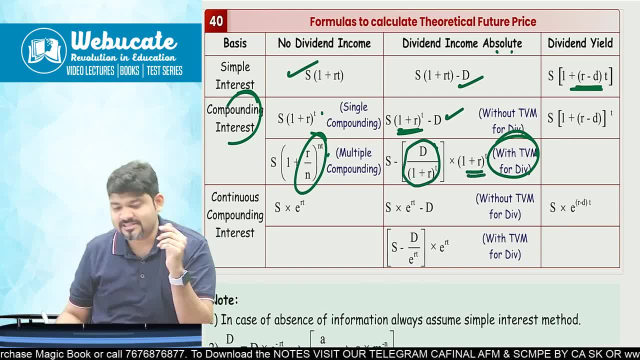 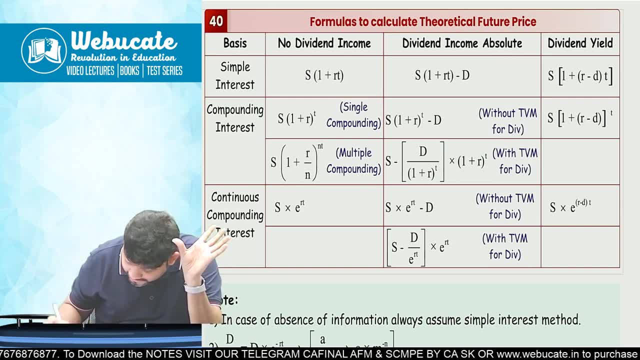 And then multiply it with the interest rate which is there. It is a rare case which is going to come. So in the exam, what are the chances of exam questions? I will tell you They can ask you a question on this, this. 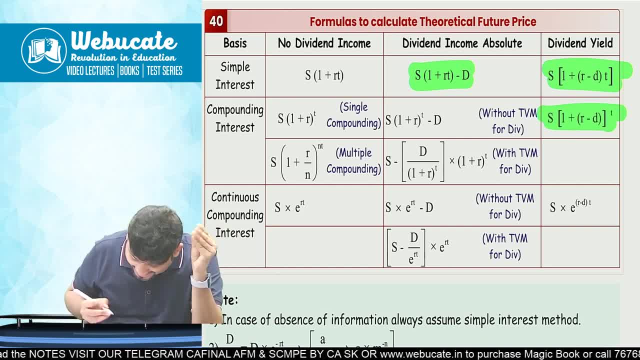 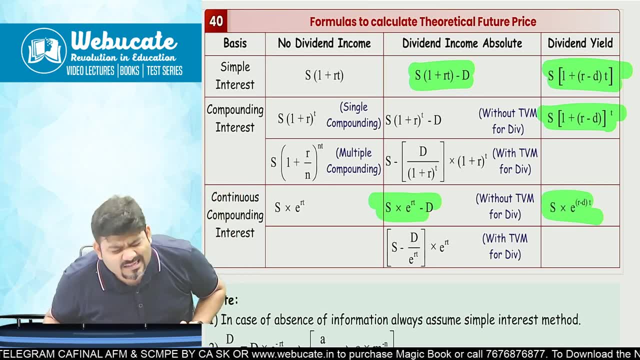 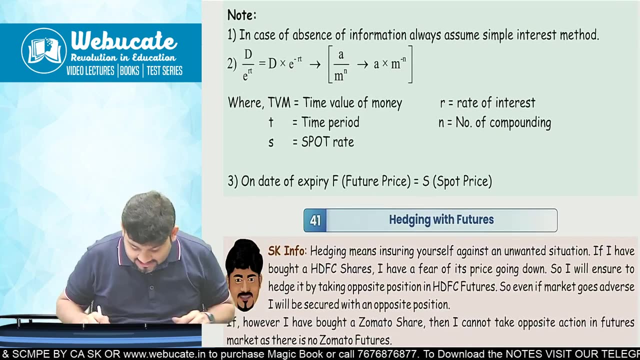 They can ask you a question on this And at max, they can ask you a question on this and this. The ones which I have highlighted in green- are the 99.99% chances that the questions will be asked on Done. So with this we complete theoretical future pricing. 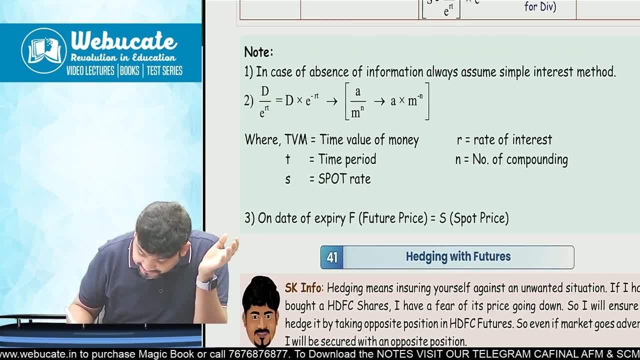 Some notes. Let's go through those notes. In the absence of information, always assume simple interest method. I told you That's what they are going to ask. This d upon e raised to r t can also be written as d into e raised to minus r t. 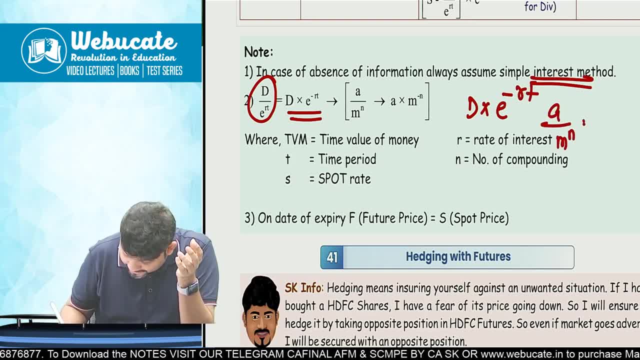 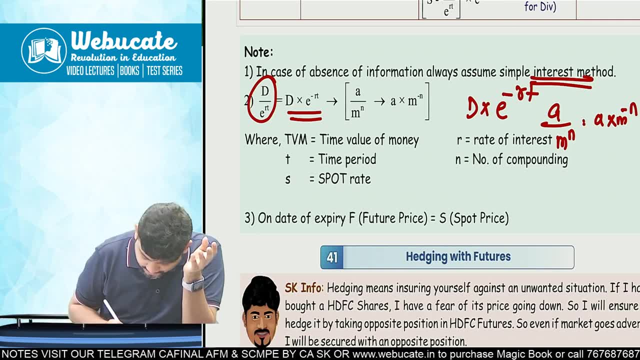 So that's absolutely okay. Like a raised to m- n can also be written as a into m raised to minus n, That's okay. So t, time period, spot rate of interest, number of compounding- All of this is there. On date of expiry: future price is equal to spot price. 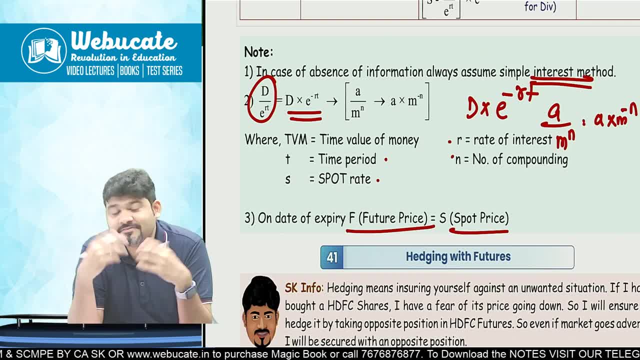 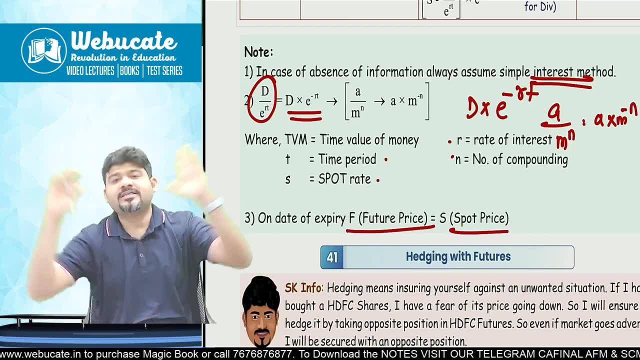 Because now there is no interest component, No Dividend component or no opportunity cost component. So on the date of expiry future price will be equal to spot price. With this we complete another concept called as theoretical future price, TFP. 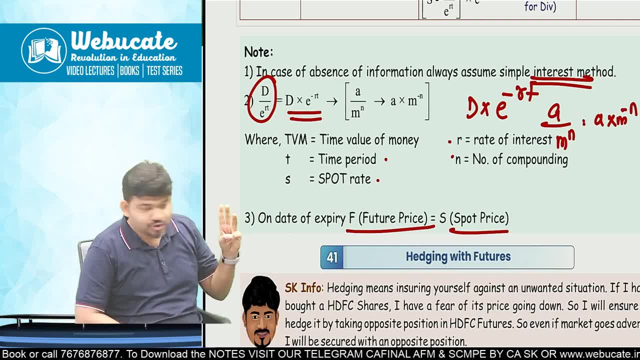 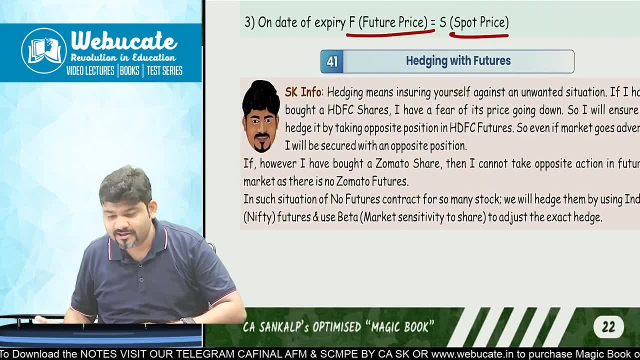 Maintenance margin: Initial margin Done. Futures process Done. Basic of futures Done. Now we come to the next concept, guys, And that is called as hedging with futures. That is called as hedging with futures. What is hedging? 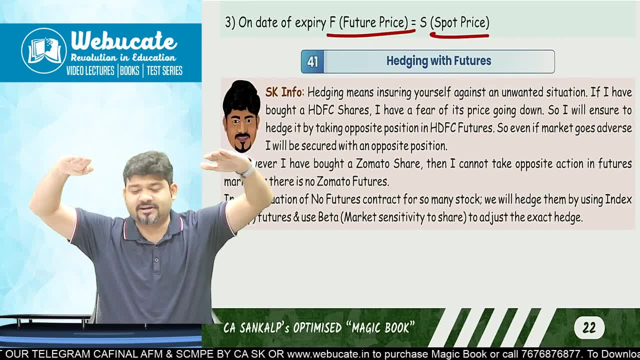 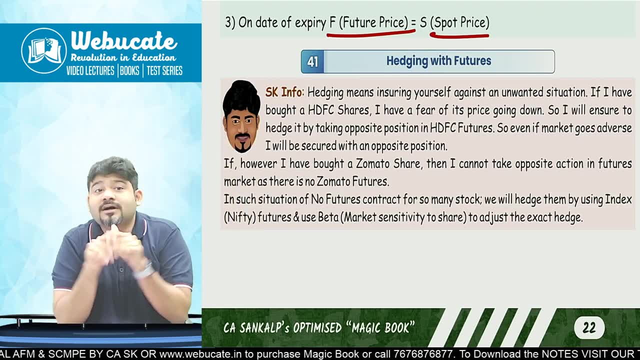 What is hedging? Hedging means insurance cover. Simple word Insurance cover. What is insurance cover? Managing the risk, What is the risk that you have, That, whatever price that you have raised and say whatever is the price going in the market? 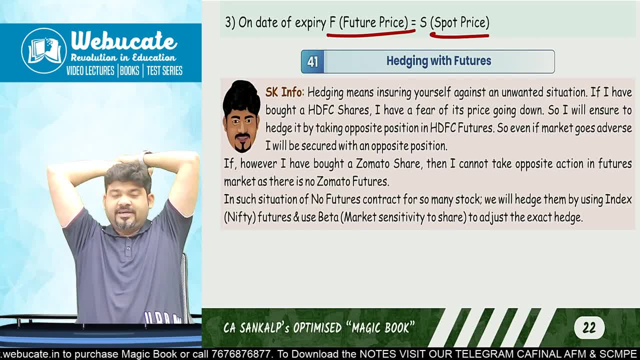 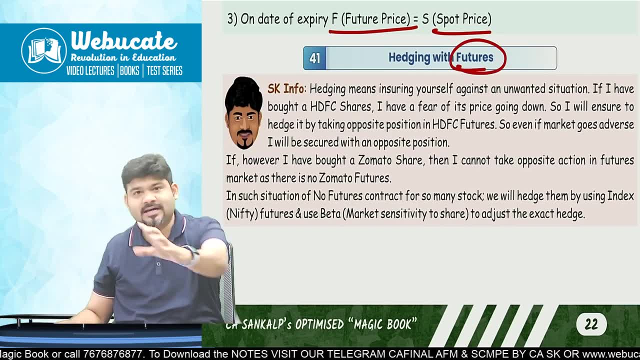 If it goes up down then I may lose a lot of money. So I want to insure, hedge myself against that risk. I will use futures for that, For example. I'll give you a small example. Suppose I have taken a. 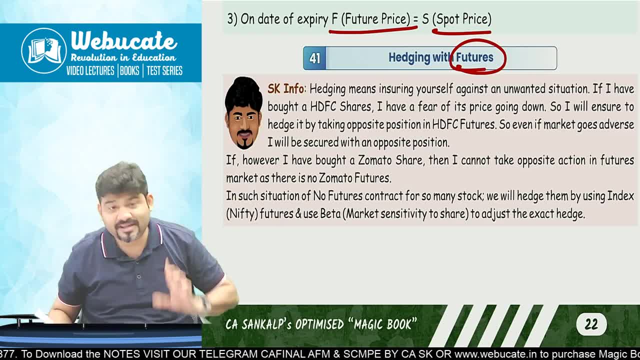 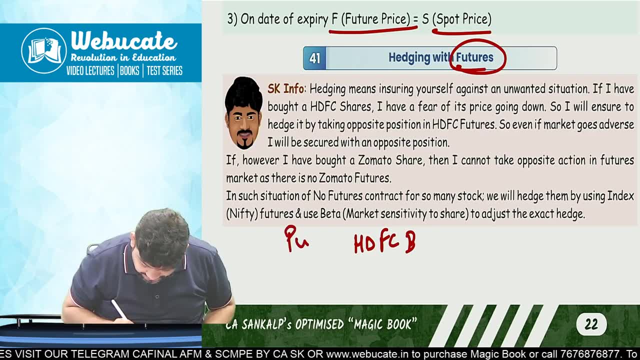 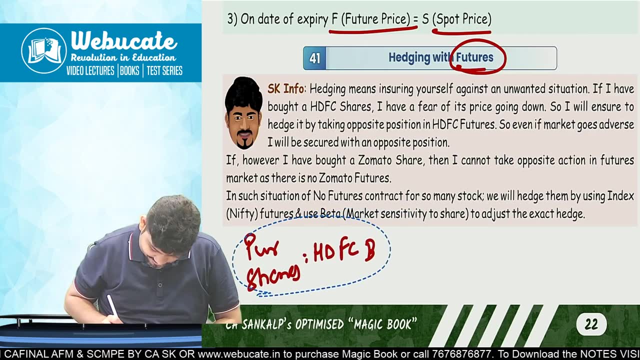 Shares of HDFC bank. Listen to my example very, very carefully. Suppose I have purchased a share of HDFC bank, Purchased a share, Purchased a share. Purchased shares of HDFC bank. Purchased shares of HDFC bank. 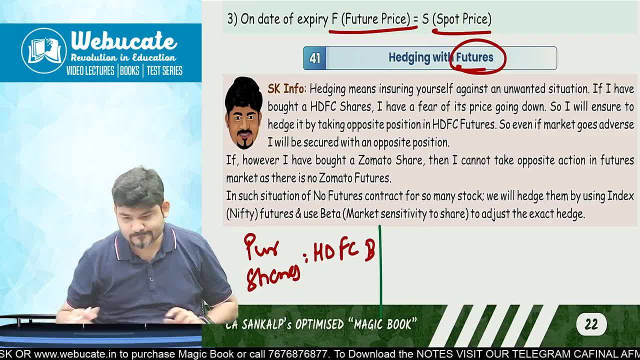 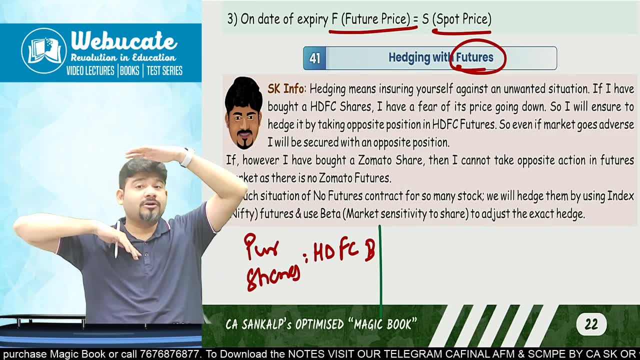 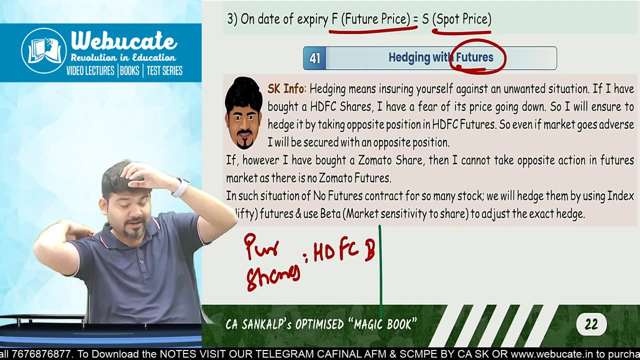 Okay, sir, Purchased. Now What is my fear? My fear is that If, what? if it goes down, I will lose a lot of money. So if anything happens as regards going down, then what will happen? I will lose the money, right. 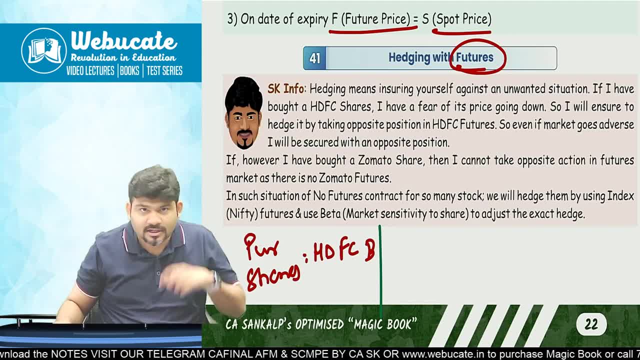 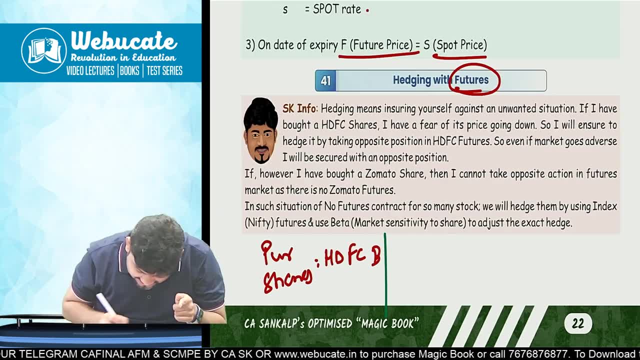 So what I can do is I can enter into a futures. I will enter into such a future that, even if the market goes down, I will gain, And what I will do is, if I have purchased the shares, I will short futures. So see, using futures. 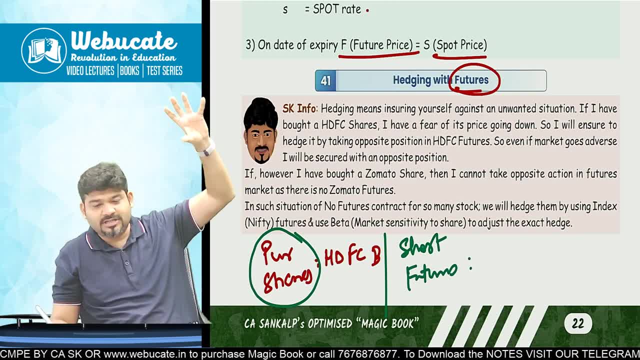 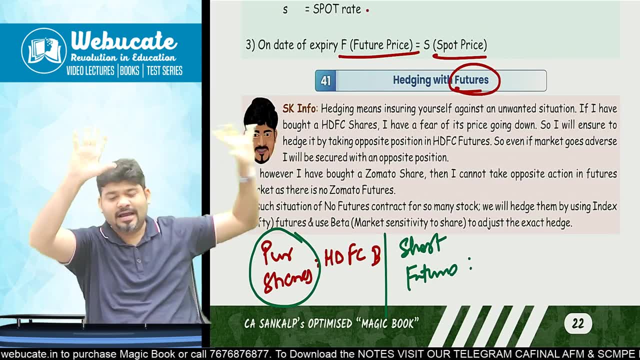 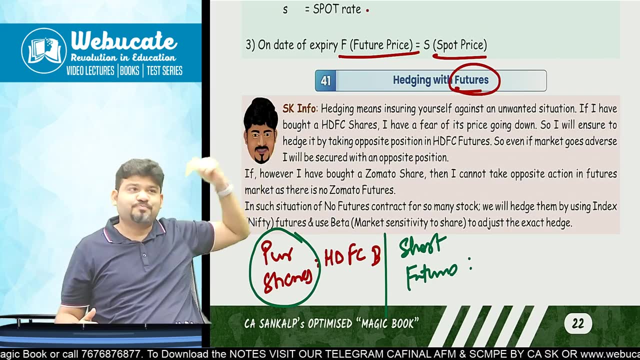 I am hedging the risk Now. if the market goes up, the share price will go up, No worries, I will gain here. I will lose in futures market. In short, I am not losing anything. Net net Suppose. if the share market goes down, I will lose in the share market. 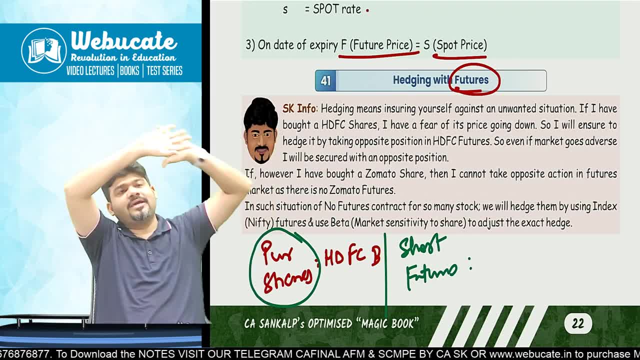 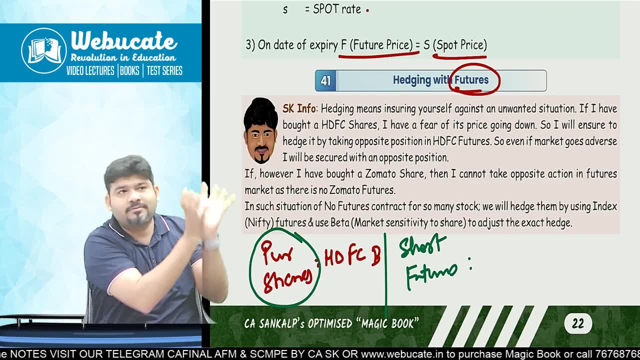 But in futures market I will gain Eventually. I am not losing anything. I have secured myself. I have protected myself from the risk. My intention is not to earn My intention, My intention is to secure myself from the risk. I don't want to incur a loss. 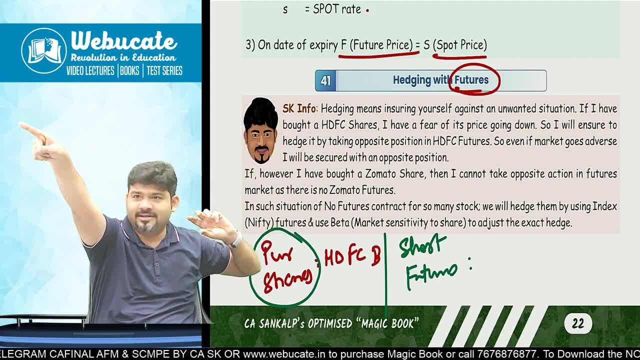 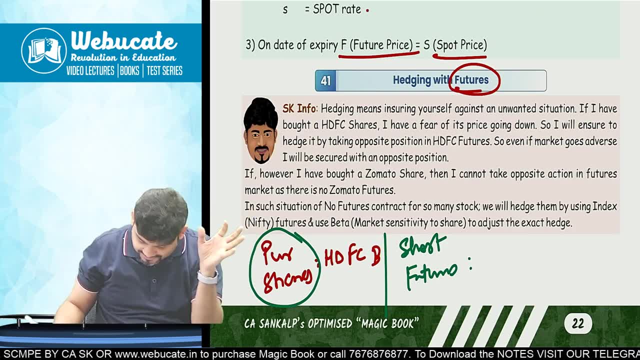 It's okay if I don't earn. For earning, you are a speculator, But for hedging, you are a businessman. You want to secure yourself. That's it, Got it, guys. So here, hedging means insuring yourself against an unwanted situation. 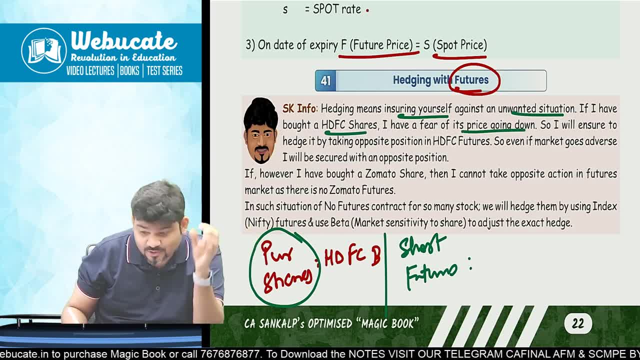 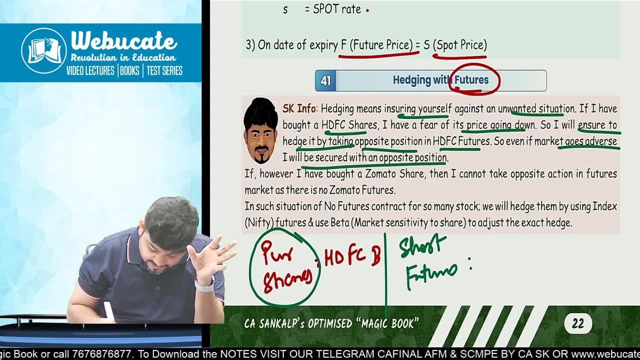 So if I have bought a HDFC share, I have a fear of its price going down. So I will ensure to hedge it by taking opposite position in HDFC futures. So even if market goes adverse, I will be secured with an opposite position. 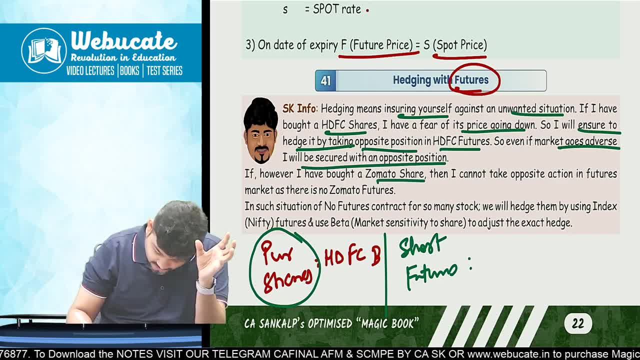 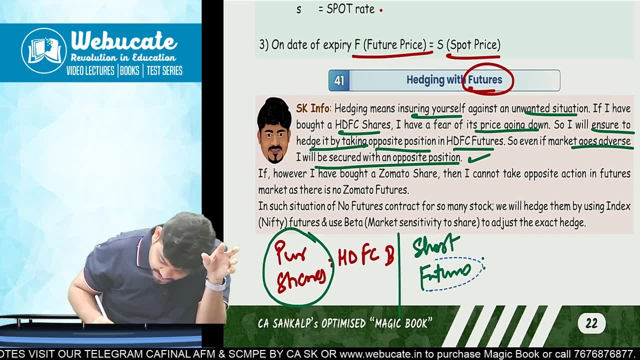 However, if I have a Zomato share, So see what I can do is I can take an opposite position in HDFC futures. So purchase shares but short HDFC futures. But obvious, I will short HDFC futures. So this I can do with HDFC futures. 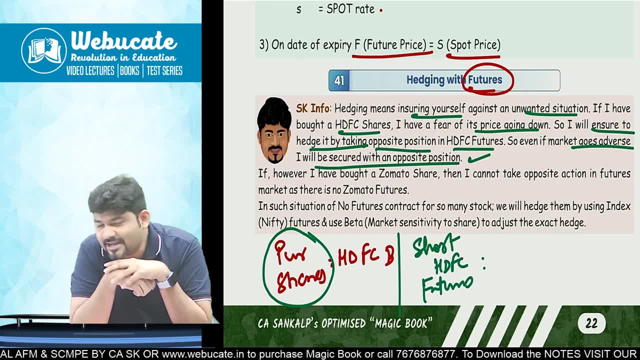 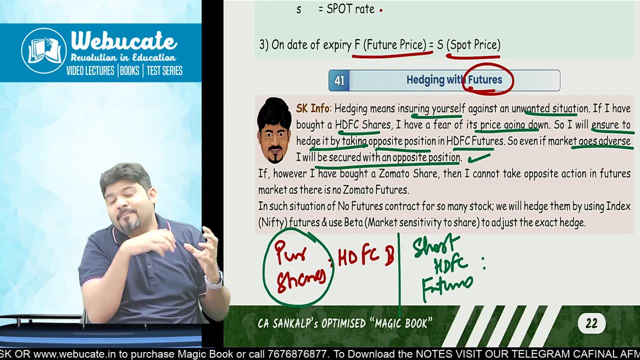 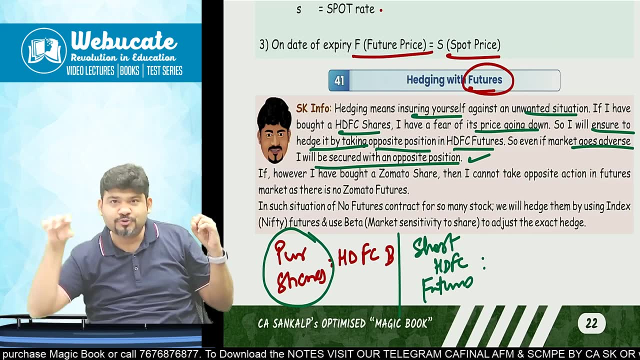 But what if I have purchased a Zomato share and I want to hedge the position? I purchased a Zomato share, But listen, I purchased a Zomato share but I want to hedge the position. I cannot take a Zomato futures because there is no futures market of Zomato. 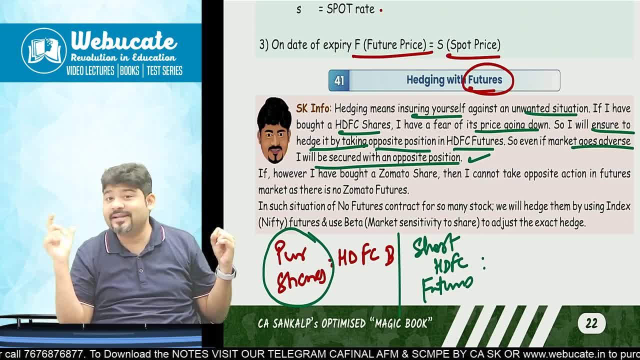 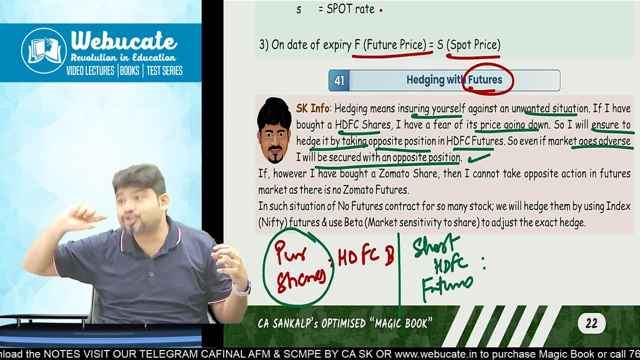 There are only good companies which are there in the futures market, because this is very risky. So what will I do? So I will hedge it with a stock index, which is Nifty. But sir, Zomato is a share. I will purchase the share. 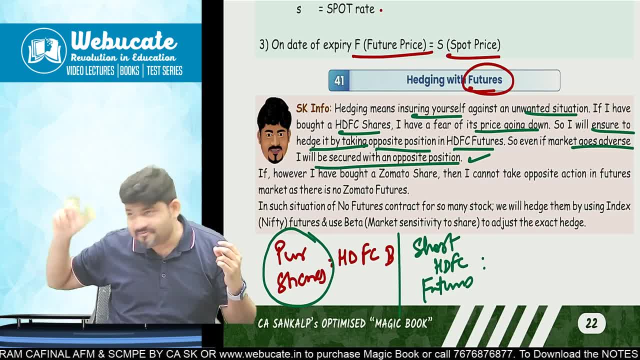 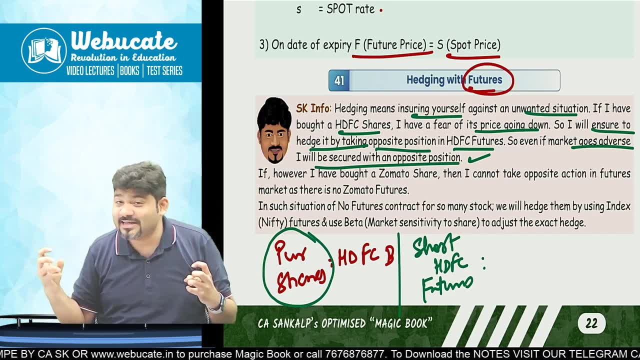 I will purchase the share. I will short Nifty, So Zomato share will go up. Nifty may go up, may go down. They are not related. So what I will do is, with this Nifty I will take a beta of Zomato. 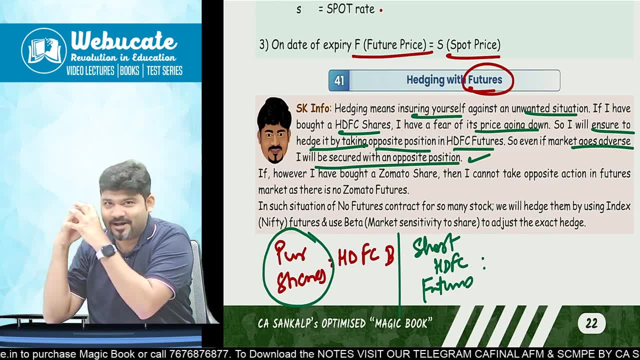 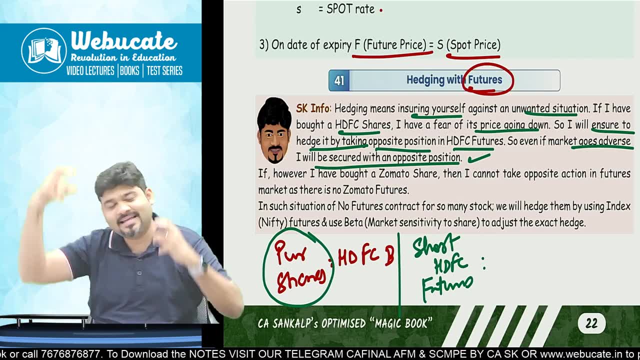 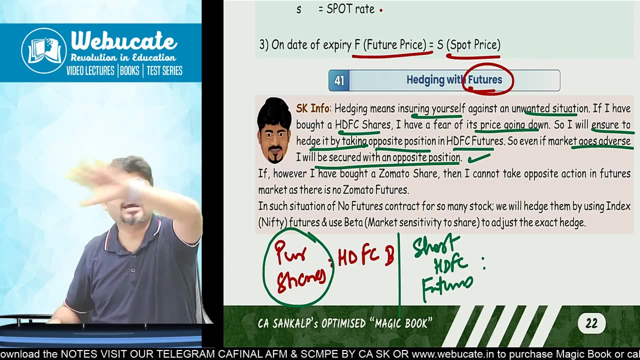 Once I multiply Nifty's price with beta of Zomato, then can I say I can make them equivalent And that is how I will hedge the position, using Nifty futures as well for shares which are not listed on or futures which are not listed. So if I have bought a Zomato share then I cannot take opposite action in futures market. as there is no Zomato futures In such situation, no futures contract for so many stocks, we will hedge them by using index Nifty futures and use beta to adjust the exact hedge. 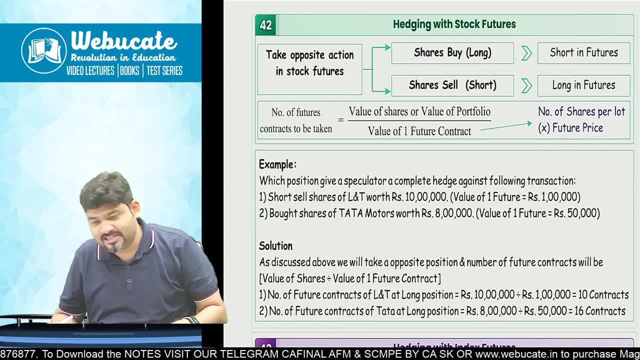 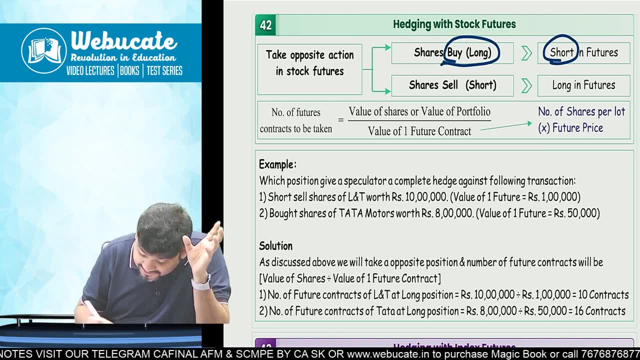 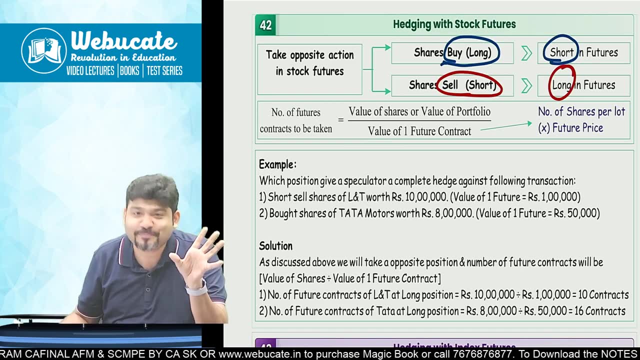 got it everybody. yes, sir, hedging with stock futures. so if you have shares bought, you will hedge it with short in futures. but if there is a short sell, you have done on shares and you are worried what will happen long the futures. it will all be okay. how many futures will have to be taken? 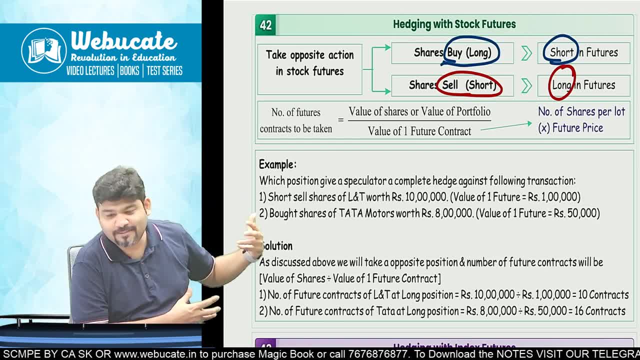 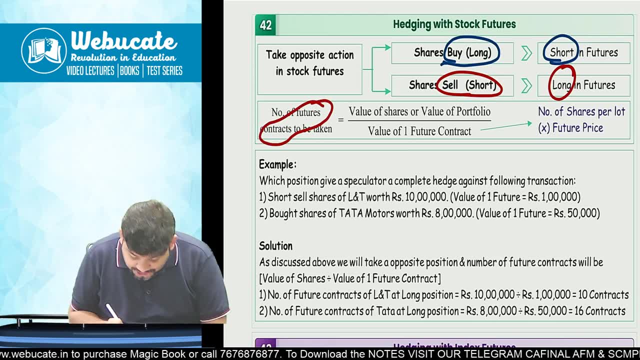 i will take i'll. i'll explain you with this example and then we'll be able to connect it, because number of futures contracts will have to be taken right. so which position gave us will give a speculator a complete hedge. so pay attention. suppose there is a short sell of lnt. 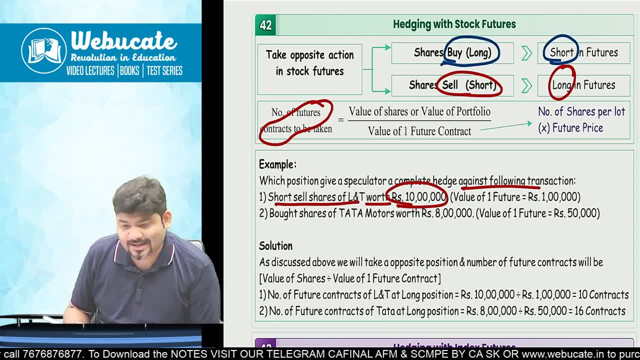 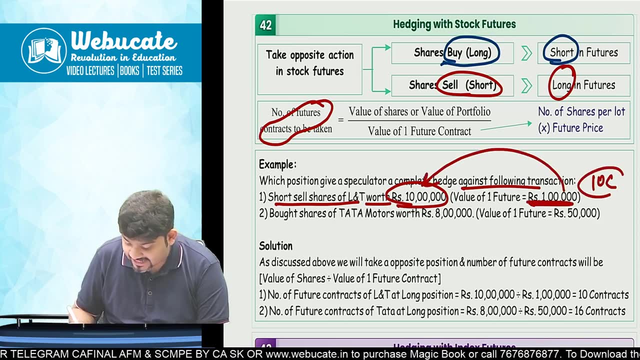 shares worth rupees 10 lakh. now, if you have short sold, you will have to. you will have to long the future. so value of one future is equal to rupees one lakh. total you have short sold 10 lakhs. can i say there will be. 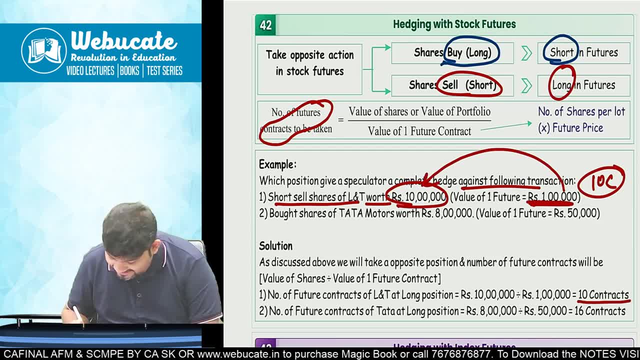 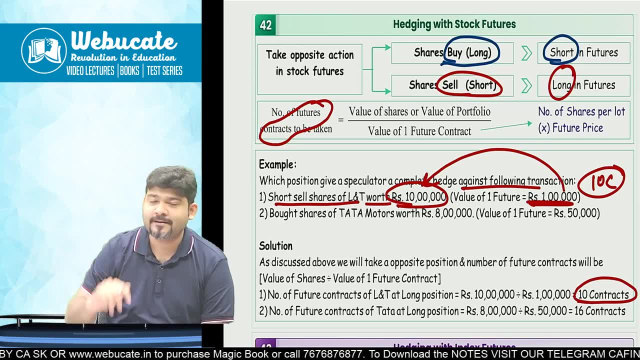 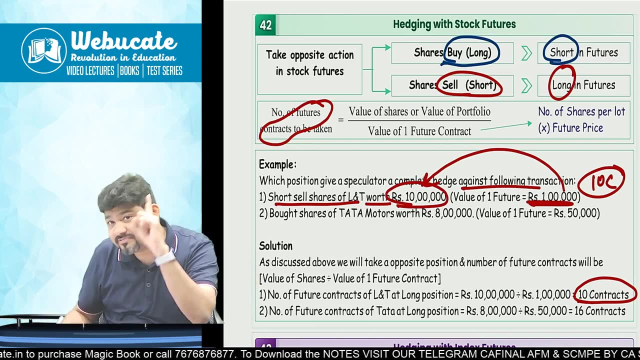 10 contracts. are you understanding correct? so 10 contracts? how did you calculate that? logically, that total value of short sell was 10 lakh. you want to hedge all of them. if, if, if there is a future, value of one future is one lakh. value of one future is one lakh. you need 10 lakhs to be. 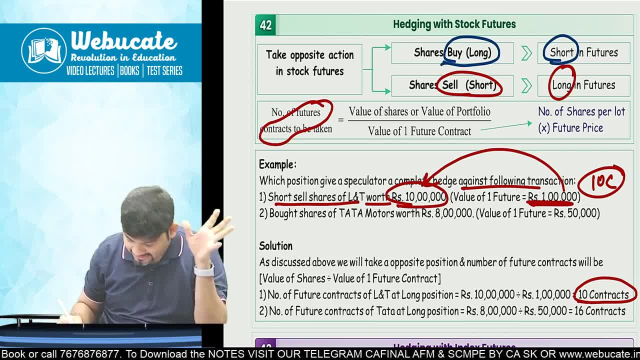 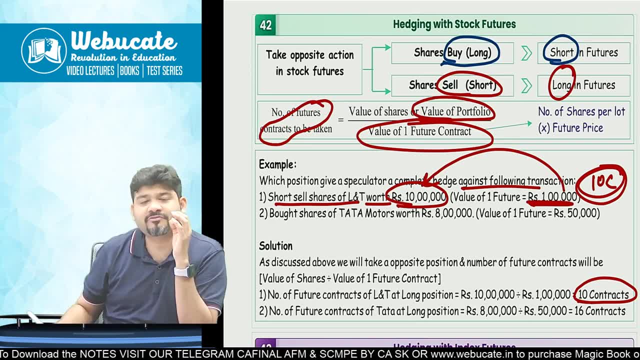 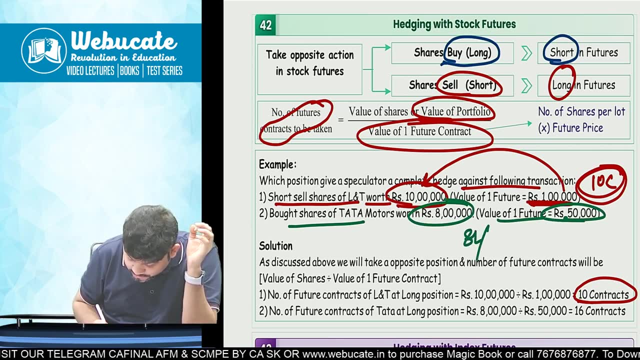 hedged. what will you take 10 contracts? you will take 10 contracts. so value of shares or value of portfolio upon value of one future contract, value of one future contract bought shares of tata motors worth rupees eight lakh. value of one future is 50 000. so eight lakh divided by 50 000, how much will it be so eight lakh? 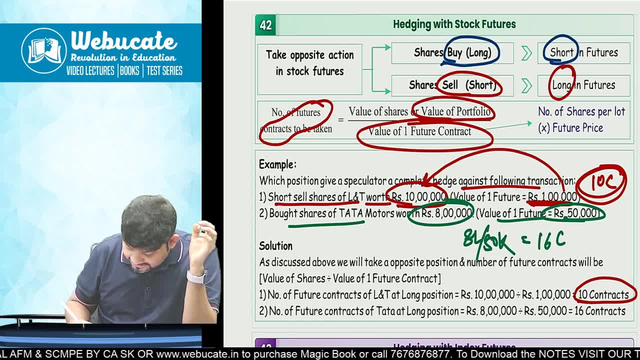 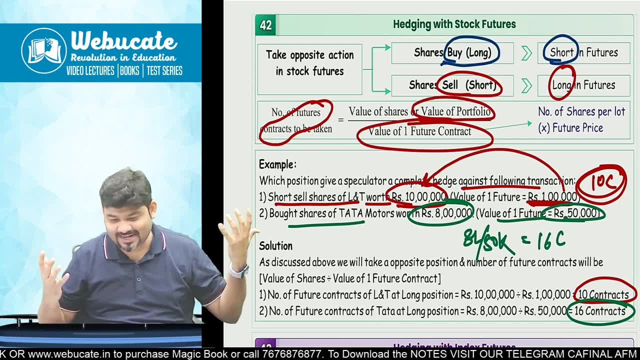 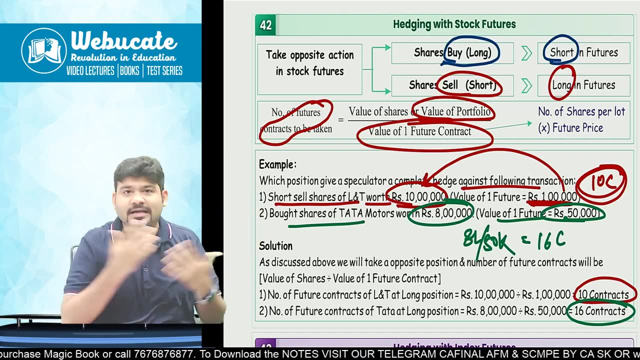 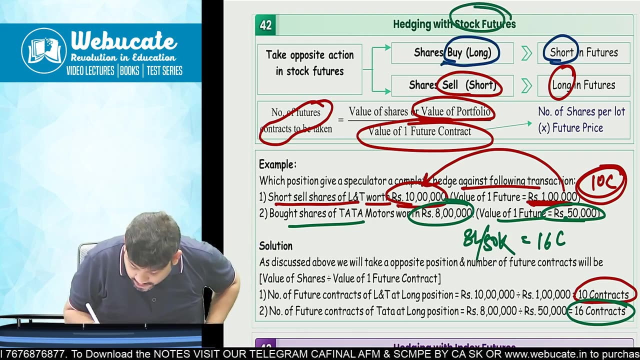 divide by 50 000, correct, it will be 16 contracts. it will be 16 contracts, rb, clear, everybody, done, done, done, done, exactly. so this is how the whole concept of hedging with stock futures can work with. yeah, stock futures can work. so hedging of hdfc share with hdfc futures is called a stock. 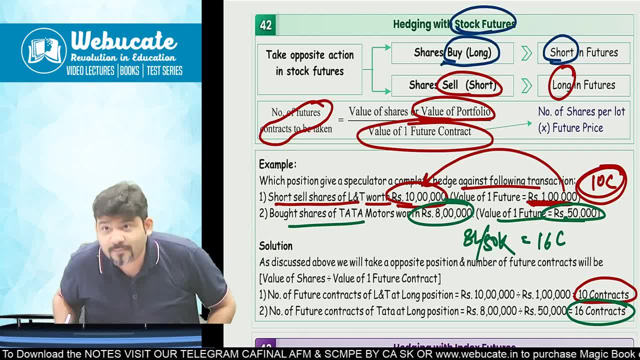 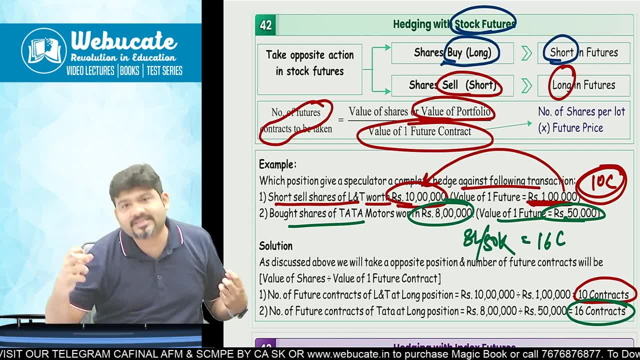 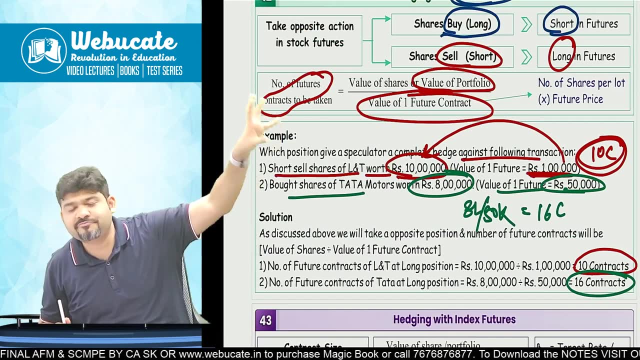 futures. it's called a stock futures, but now what if it is a zomato share? it will be hedged with a nifty, with the index future, which will also have beta. let's start with that. so are you clear with how much? how many contracts are to be required? value of portfolio divided by poor. you know value. 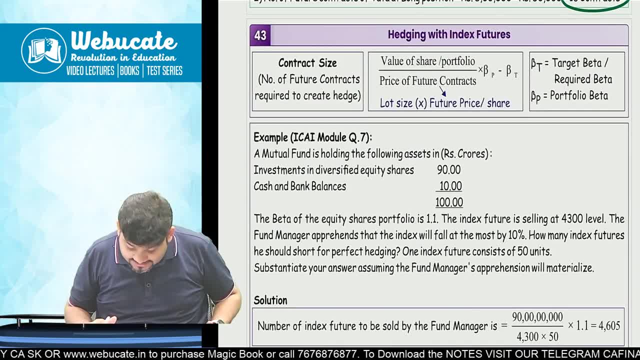 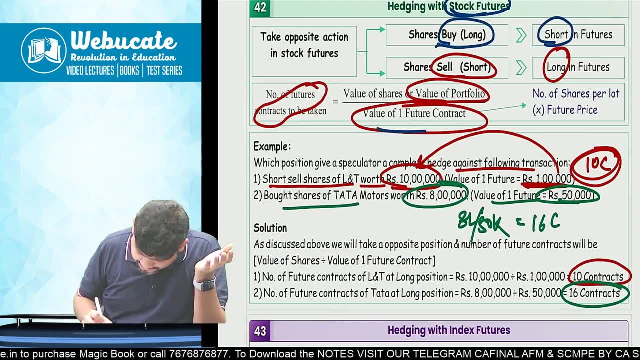 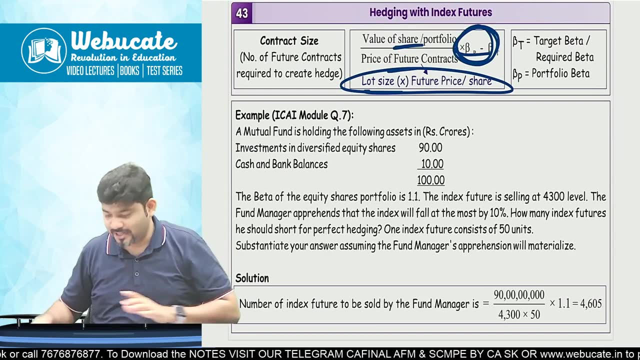 of one future contract done next is hedging with index futures. so value of share or portfolio upon price of future contracts, as we have done, it's nothing but value of one future contract, but multiply by the beta factor of that company, because what is beta movement of nifty with that? 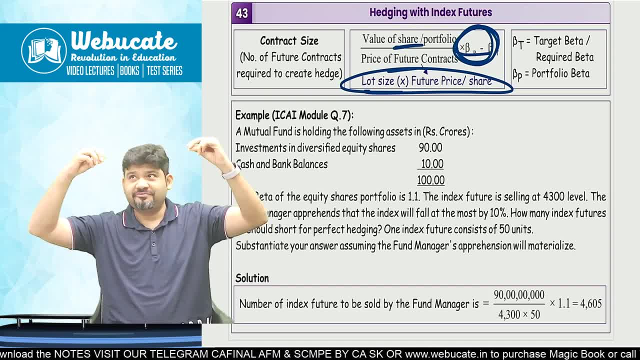 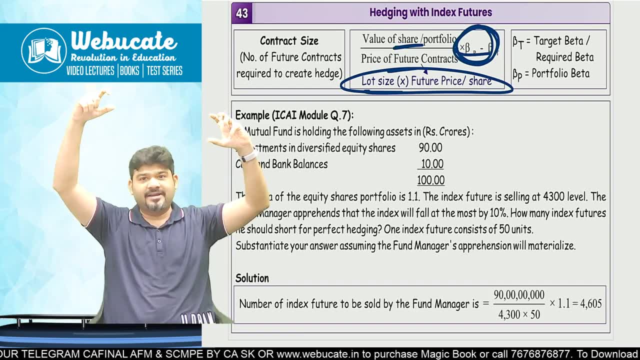 market with that of this share. so if nifty goes up by 100, this share will go up by 200. so there is a beta of 2. so what i will do is, if, say, market goes up by 100, i will multiply it by this beta, which is multiplied by 2, by 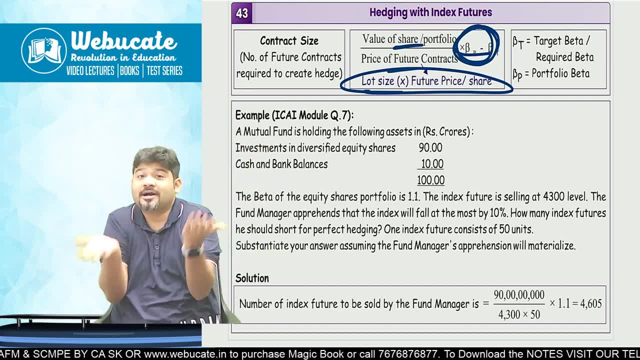 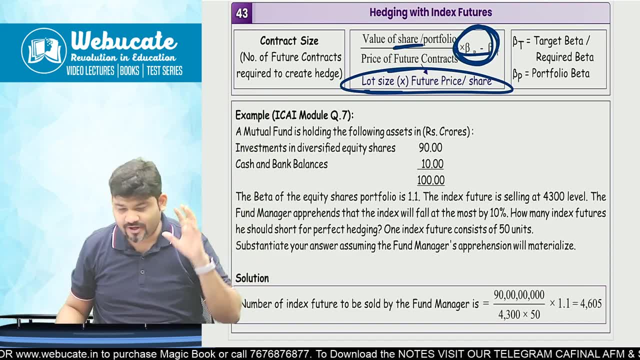 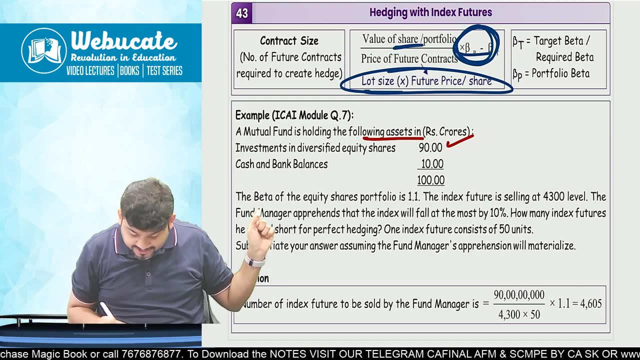 default 200 will be hedged and i have a complete, perfect hedge. are we clear everyone? so this is a classic example for here. so hedging with index futures. a mutual fund is holding the following assets: investment in diversified equity shares. cash and bank balance. cash and bank balance cannot. 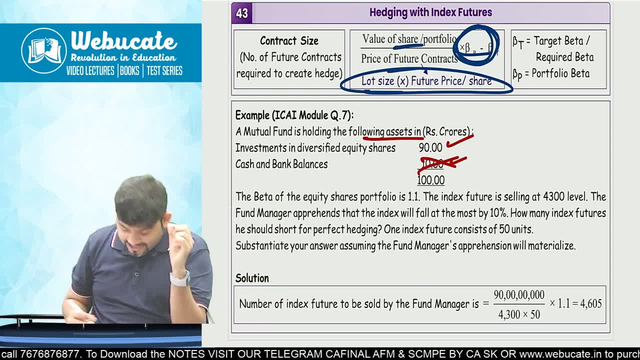 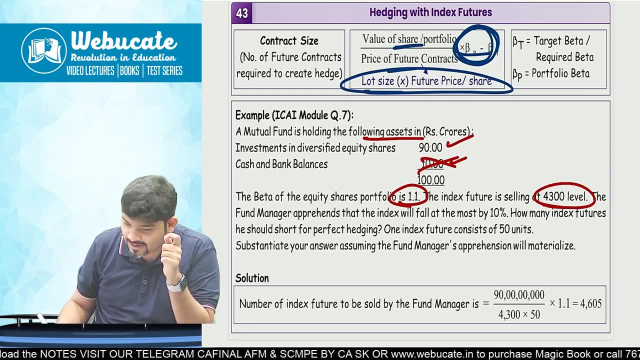 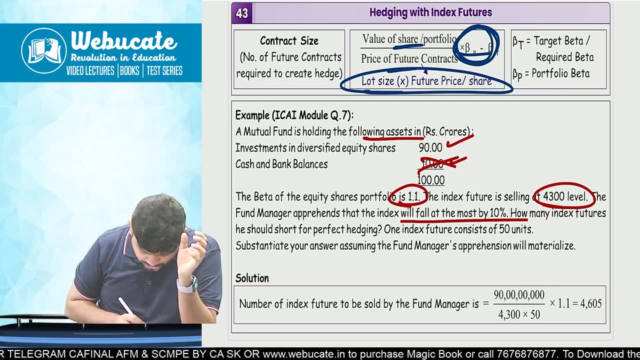 be hedged. okay, remove it. so now the beta of the equity shares portfolio is 1.1 index future selling at. index future is selling at 4300 level. fund manager apprehends that the index will fall by, at the most, 10 percent. how many index futures should you shot for perfect hedging? 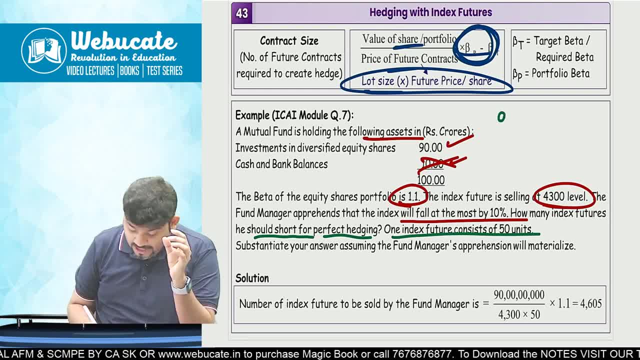 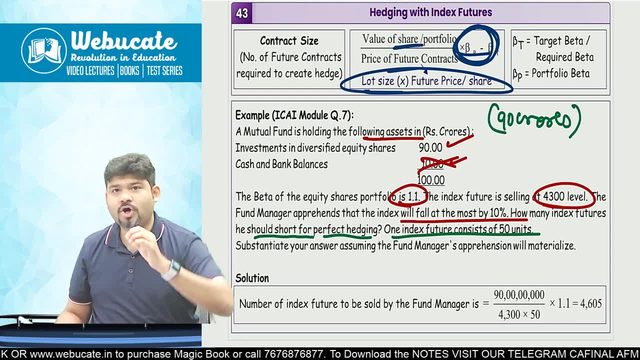 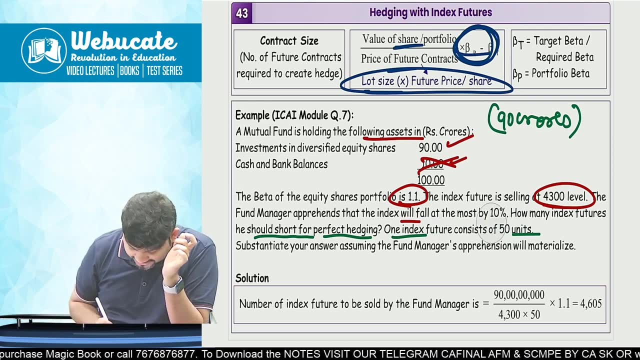 one index future consists of 50 units. so now you have 90 crores. hello, you have 90 crores worth of of equity shares, but there is a hedging that you require because you feel that the market will fall by 10. you feel that the market will fall by 10, so now, in this case, what are we going to do? 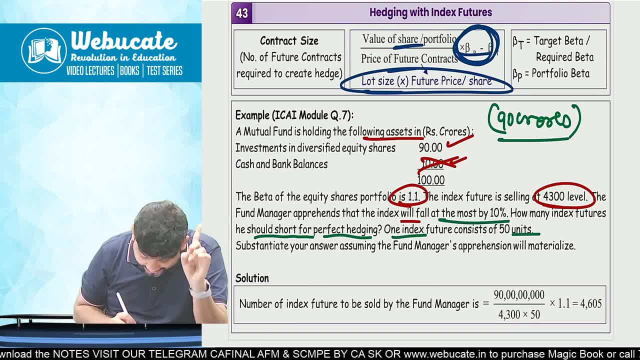 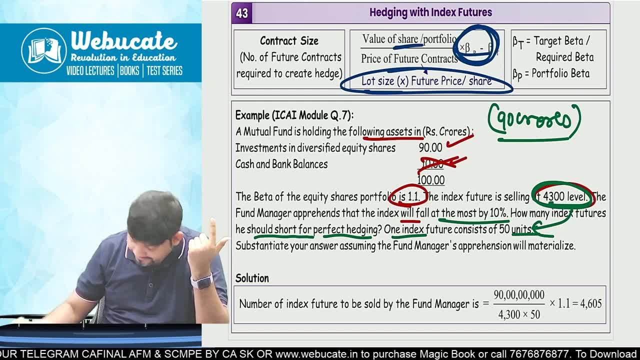 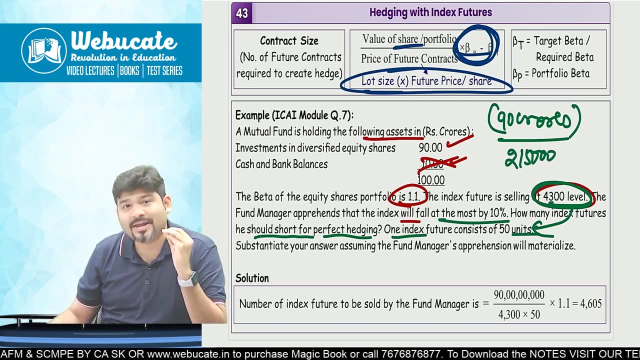 so 90 crores divide by one. what is the one value of one future contract? can i say 4300 into 50, so 4300 into 50, so 2,15,000, so total, how many contracts will require? uh, 90, uh, 90 divide by 2,15,000. so ideally 4186 contracts is what you will require. but 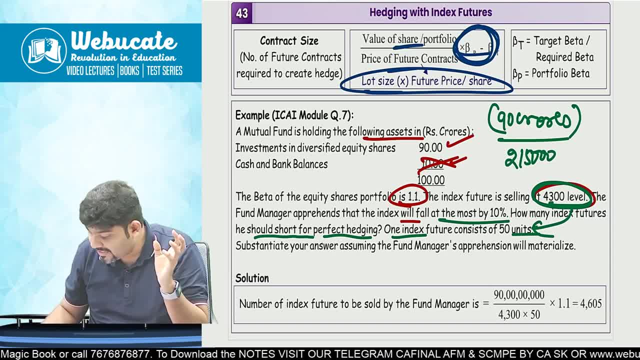 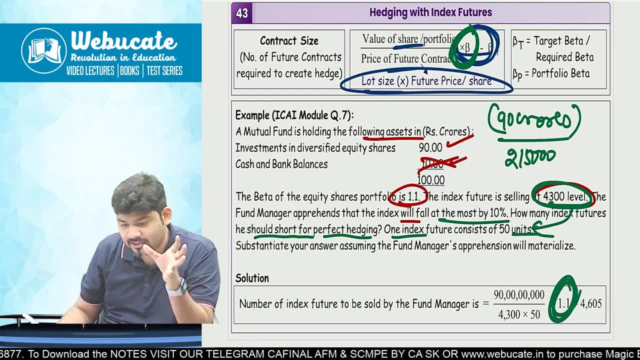 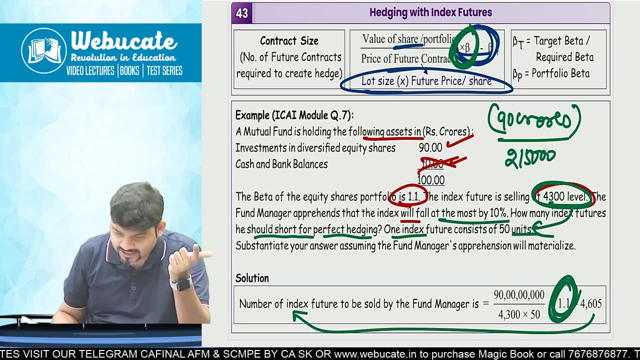 there is a beta of 1.1. so we will multiply this by 1.1. so multiply it by the target beta. simple multiply it by the target beta. so this will be 4605 index futures. 4, 6, 0, 5 index futures. 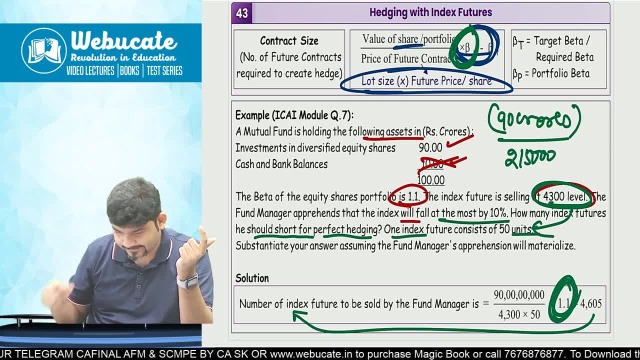 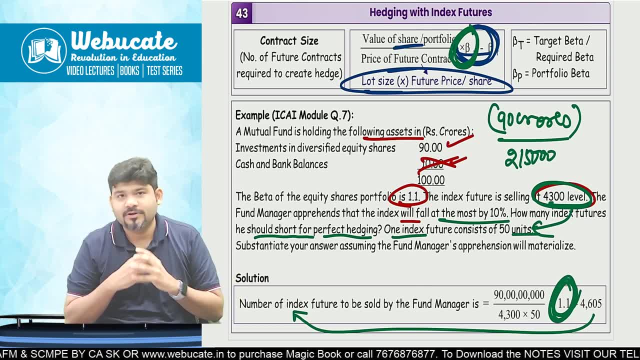 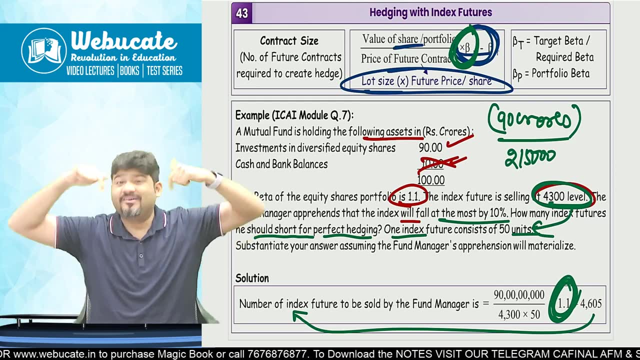 done, done, done, done, done. now you have hedged yourself by 4 6 0, 5 futures. how did you do it? value of the portfolio divided by value of one future contract, 4 6 0 0, 4 3 0 0 into 50. but if 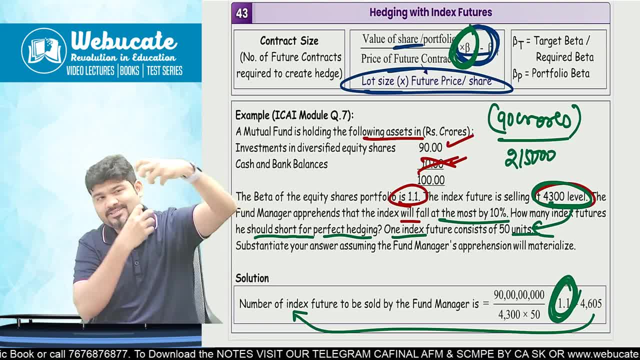 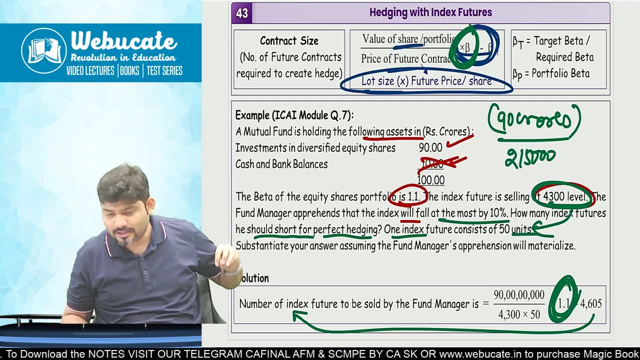 it was a stock future and stock buy. that is okay, but here there is a 1.1 beta, so multiply that by 1.1, you will get the number of index futures to be sold. this is the number of contracts: 4, 6, 0, 5. 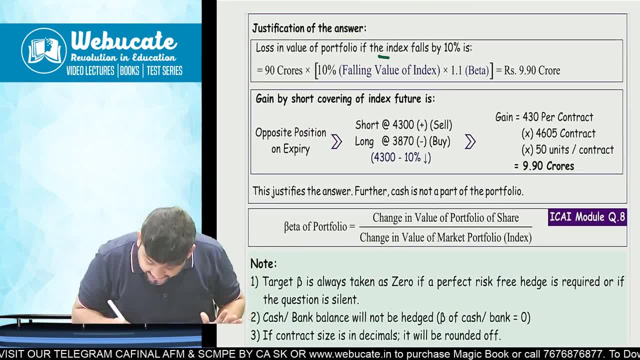 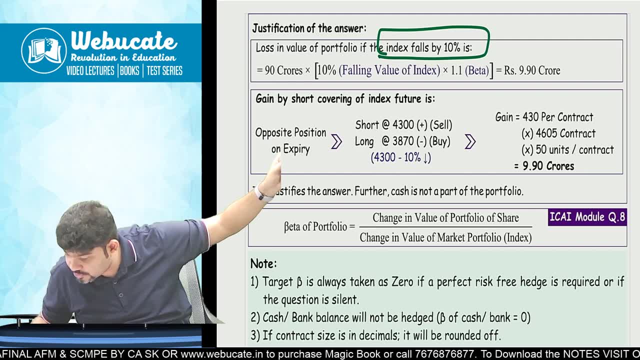 is the number of contracts. now, suppose their index falls by 10 percent, can i say that 90 will fall, 90 crores will fall by 10 percent, so it will become 81, right, so you will lose a good amount of money. so you will lose a good amount of money. so you will lose a good amount of money. 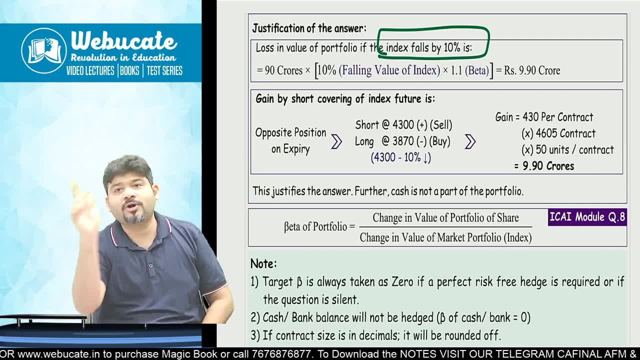 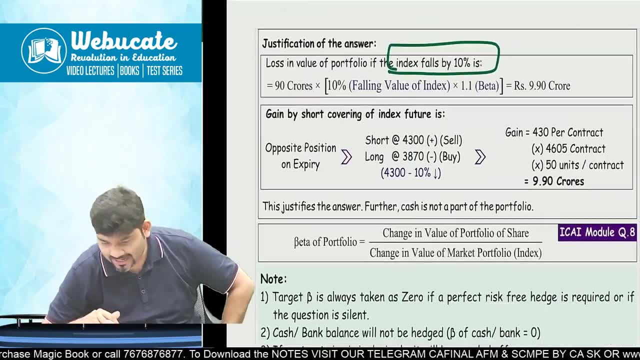 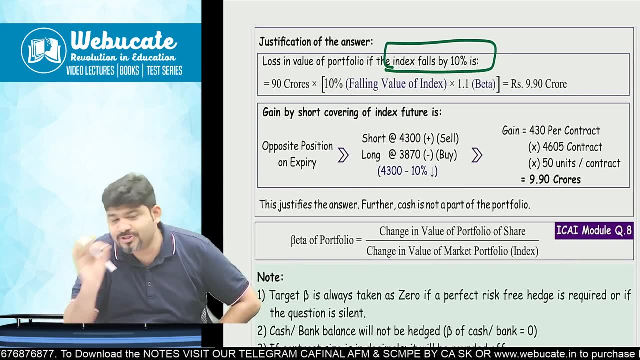 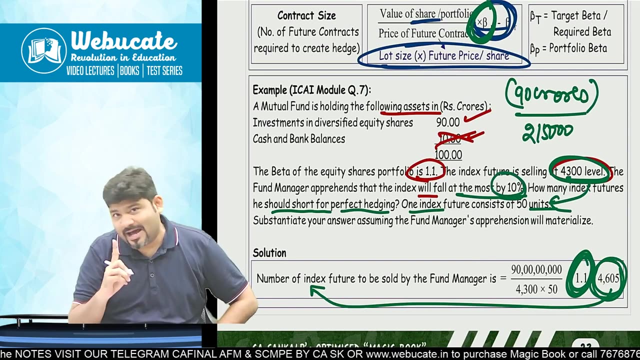 but all of this will be offset by your correct futures position. do you want to see how i'll take you through the whole concept now? you are going to lose. how much you are going to lose? market falls down by 10 percent. if market falls down by 10 percent, your beta is 1.1. so can i say: 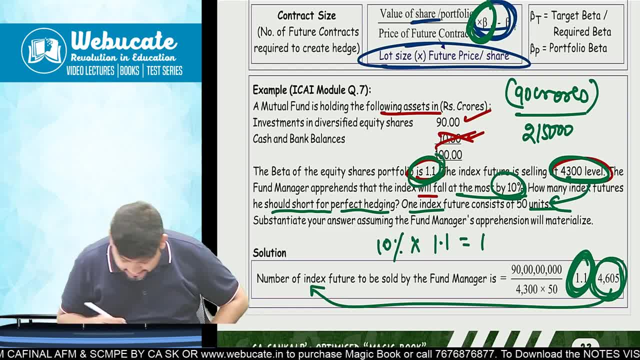 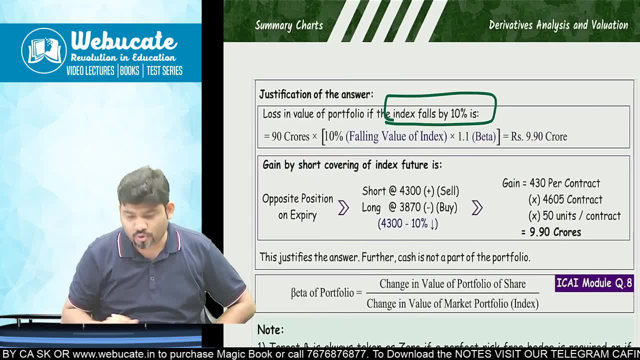 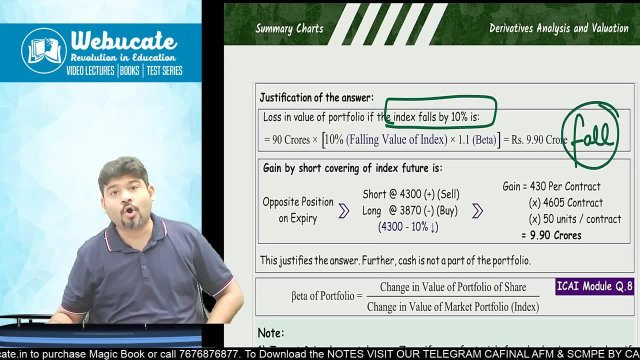 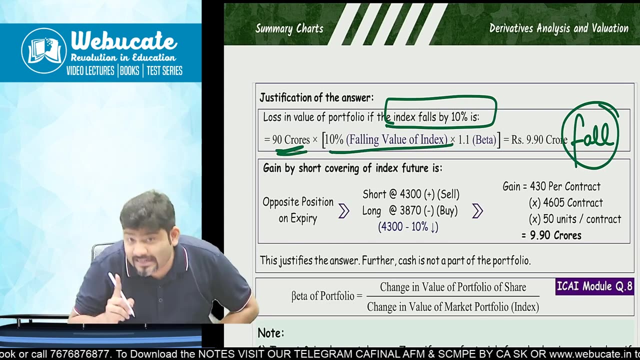 by 1.1, so 10 into 1.1 is 11, so 90 into 90, into 11 percent. 9.9 crores is the fall, 9.9 crores is the fall. 9.9 crore is the fall done. so 90 crores, 10 percent value of the index. fall 1.1 is the beta. 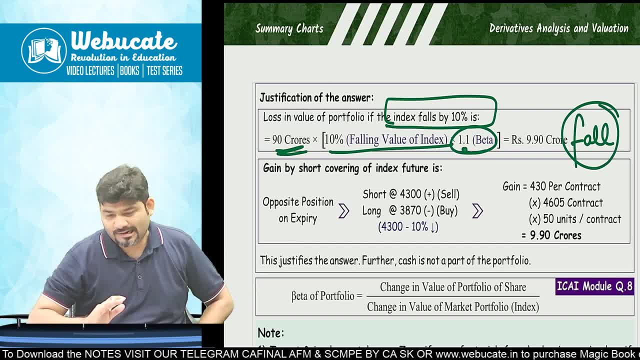 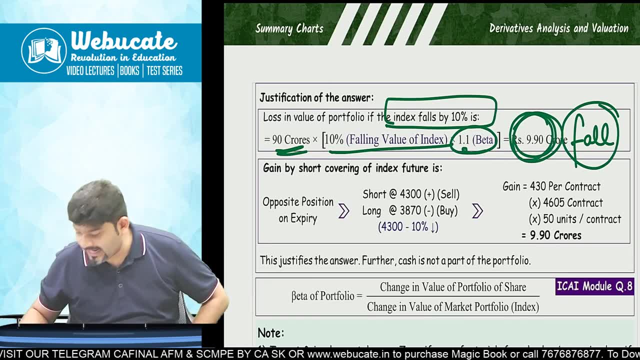 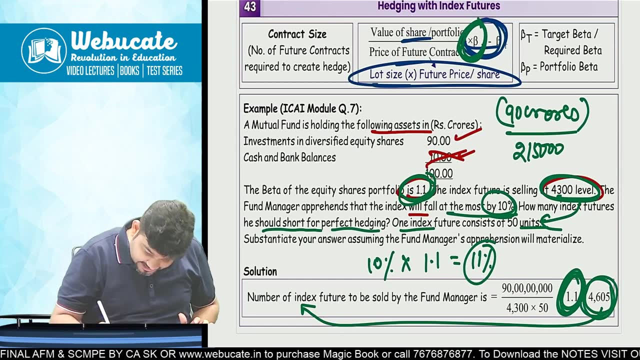 1.1 is the beta, so 11 percent is the fall. so 9.9 crores, 90 into 11 percent 9.9. now see how you are going to gain in the futures market. what you have done? you have taken a- yeah, you have taken a short position. 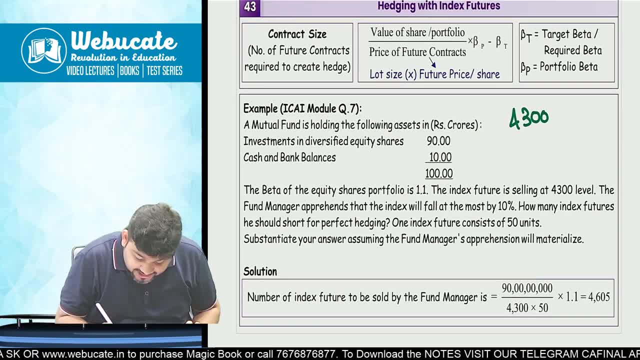 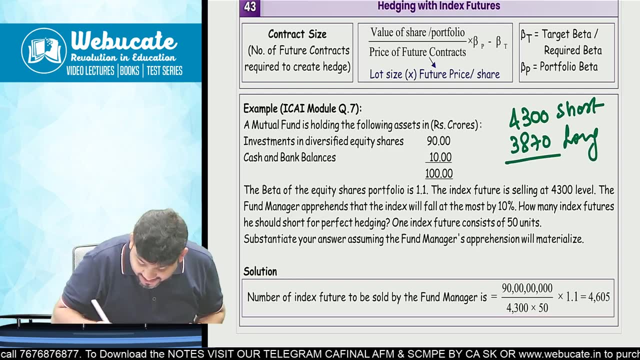 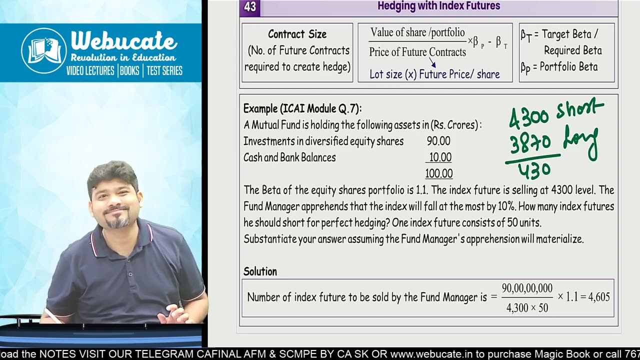 at 4300, market falls by 10 percent. so 4300 minus 10 percent. now the market is 387: 0. so you have taken a short position. now you will close it, offset it by a long position. so 4300 minus 3870, this will become 430. this will become 430. are we clear? everybody now in this 430. 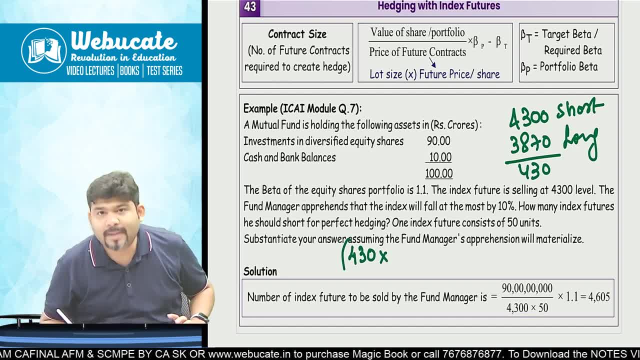 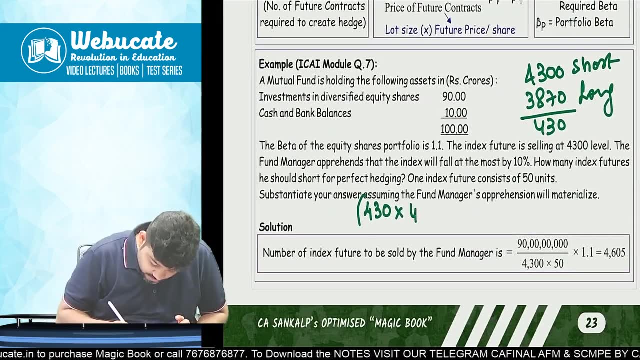 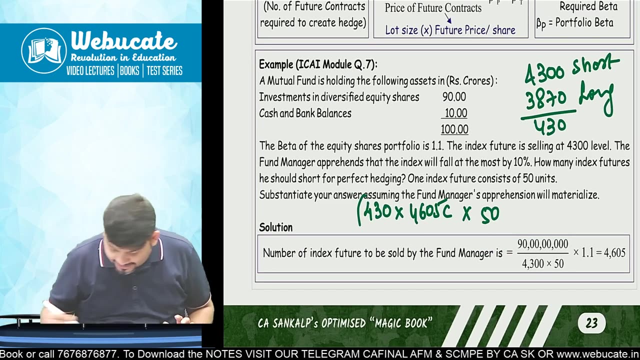 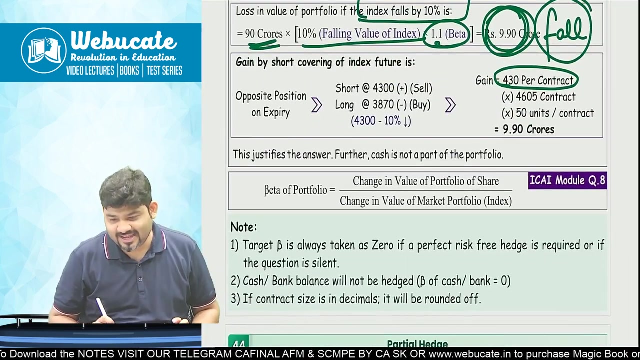 multiply this 430 by how many contracts have you taken? so 4605 into 430. so see here: 430 per contract is your gain, into 4605 contracts, into 50 per contract, into 50 per contract and this will give you 9.9 crores gain and that is offset here. done, we have justified. 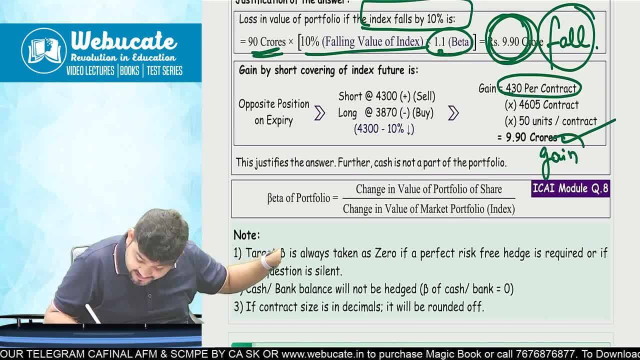 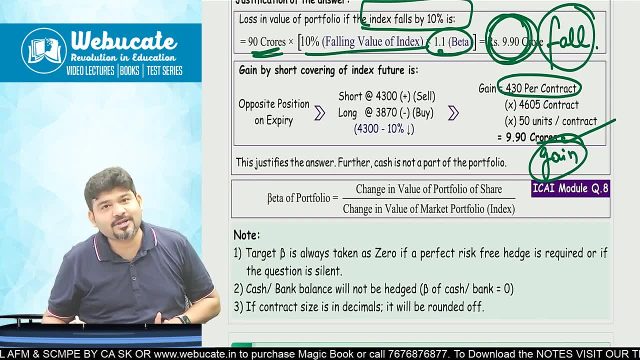 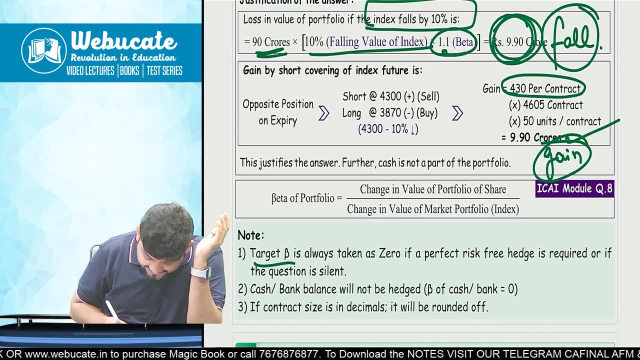 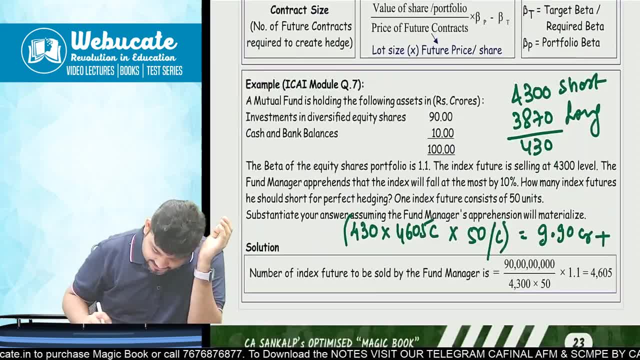 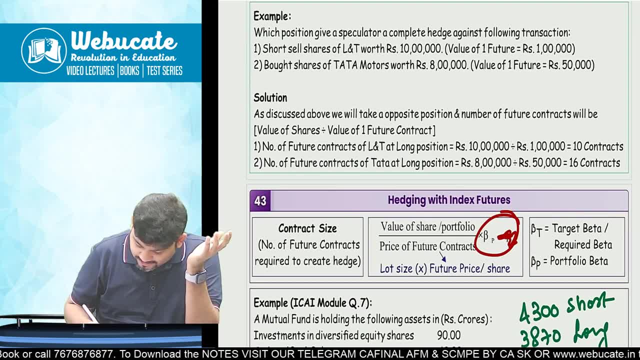 perfect, risk-free hedge is required. see, what i have done is i have given you the formula here: beta of portfolio minus beta of target. but it is not required. you can just directly multiply this by the beta. so that's absolutely okay if you need a partial hedge. 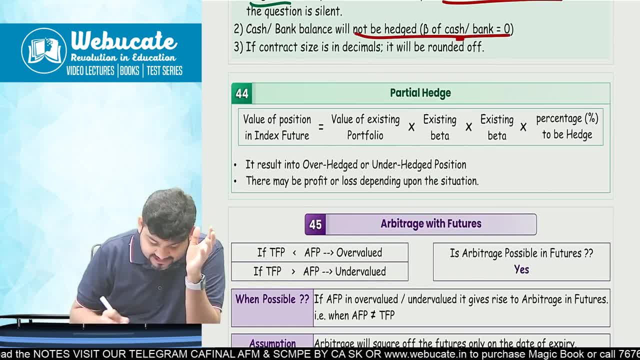 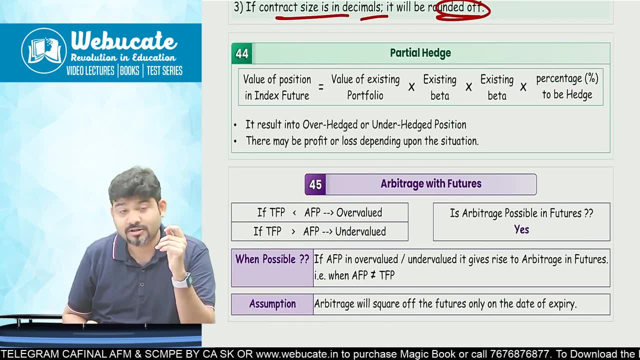 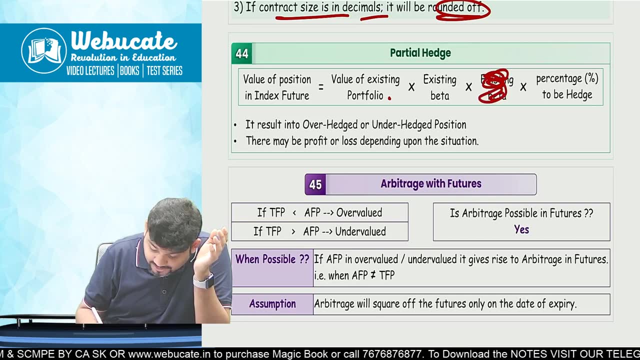 yeah, cash and bank will not be hedged because beta of cash and bank is zero. if contract size in decimals, it will be rounded off to the lower number. okay, partial hedge. what if it is a partial hedge to be done, then value of existing portfolio into existing beta, into 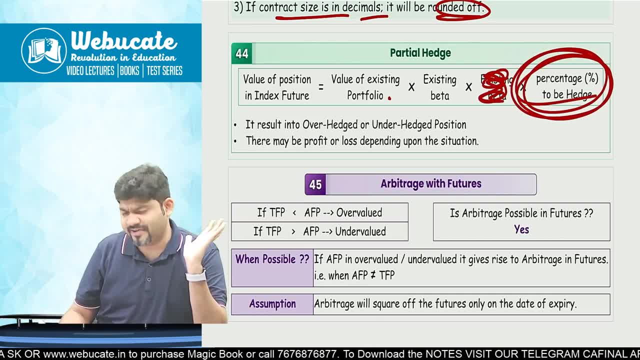 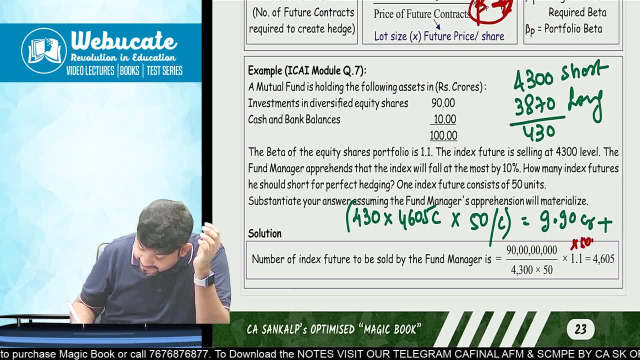 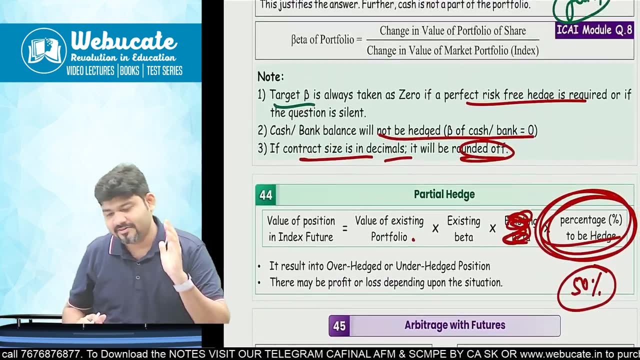 percentage to be hedged. suppose i just want 50 percent of hedge to my of my portfolio. so you will multiply this by 50 percent. so instead- so this year you can multiply this by 50 percent- only 50 percent of your portfolio will be hedged. are you clear? everybody done with this, we complete. 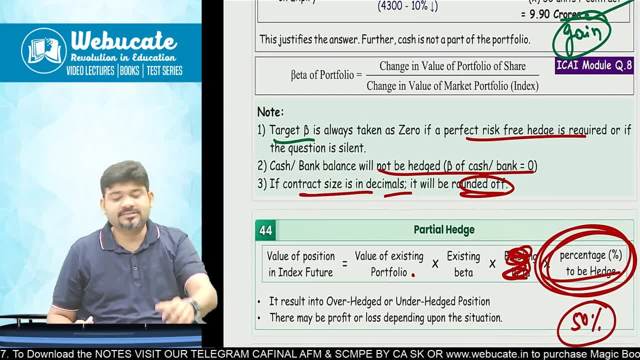 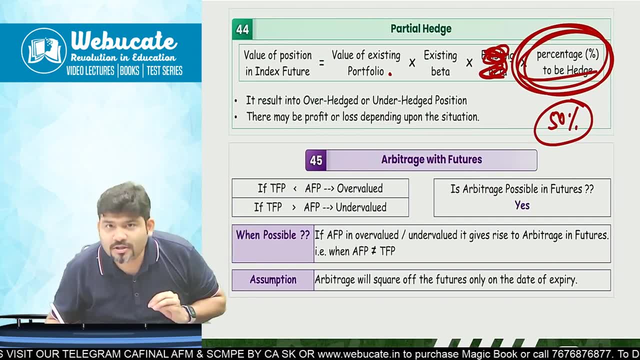 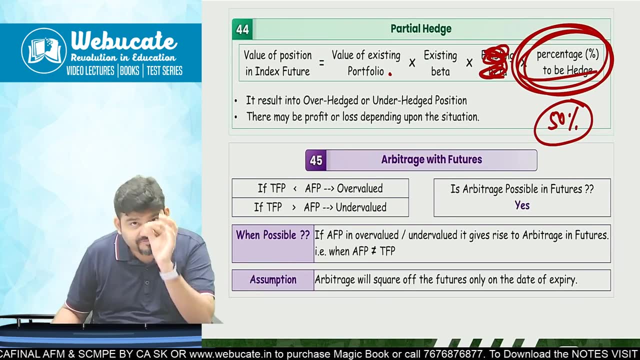 hedging with futures. and now the last concept is last, and that is arbitrage with futures. let's start with arbitrage with futures. are you ready? now, what is arbitrage? can i say? it is a game of risk-free profit. okay, now, when will the arbitrage arise? please confirm. are we clear with the hedging with? 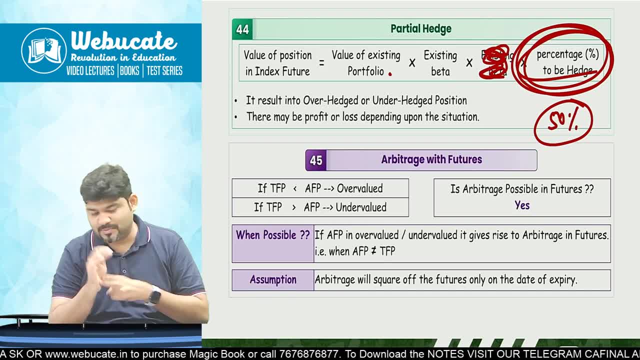 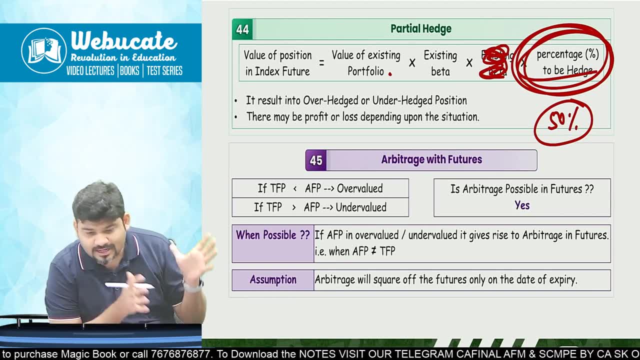 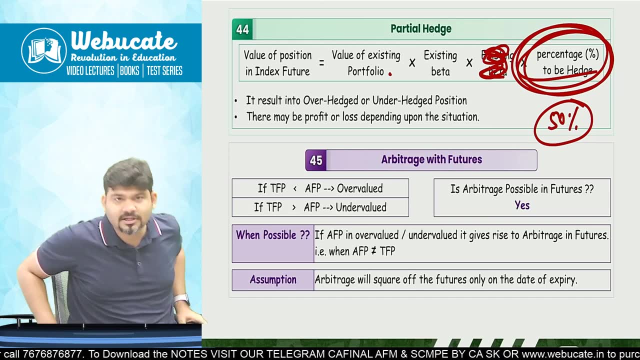 futures part right. so hedging with futures margins and you know theoretical future price and basics and future process. everything done. now the last thing, arbitrage with futures. what is arbitrage with futures? so we know how to calculate the theoretical future price. so ideally, when i go to, you know long. 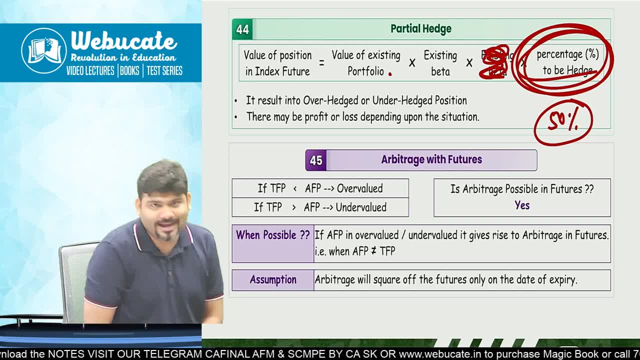 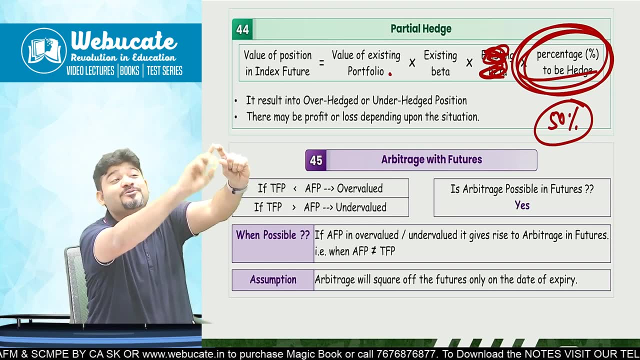 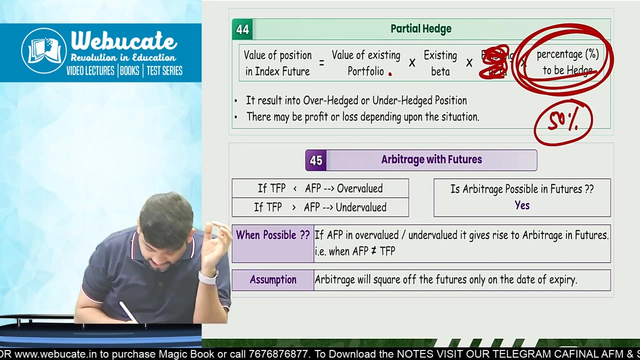 or short a future in the stock market. hello, if i go to the market and go to long or short the future, it should ideally be at the theoretical future price, right. But if it is not equal to theoretical future price it gives rise to arbitrage opportunity. So suppose theoretical future price is, say, 1090,. 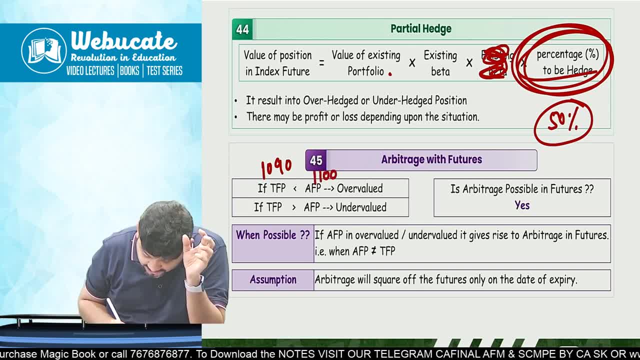 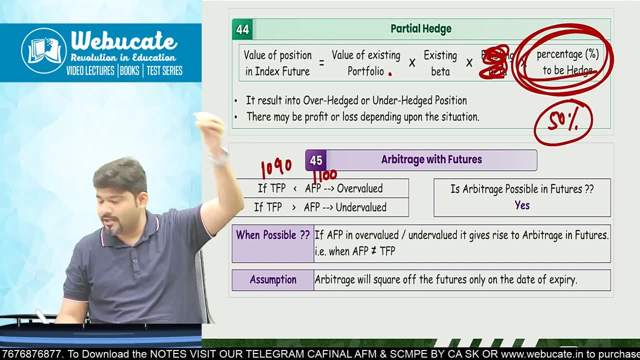 but actual future price is 1100.. So can I say, hey, ideally the future price should be 1090, but it is being sold at 1100, it is overvalued, For sure it is overvalued. And suppose, if this? 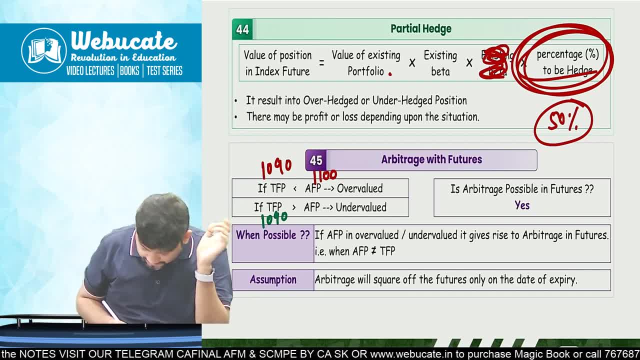 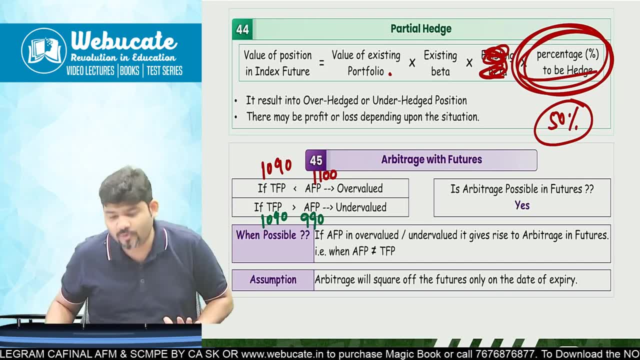 is 1090, but actual future price is 990,. can I say it is undervalued. It is undervalued right. So ideally the price should be 1090,, but we are getting it in the market as 990.. We will say: 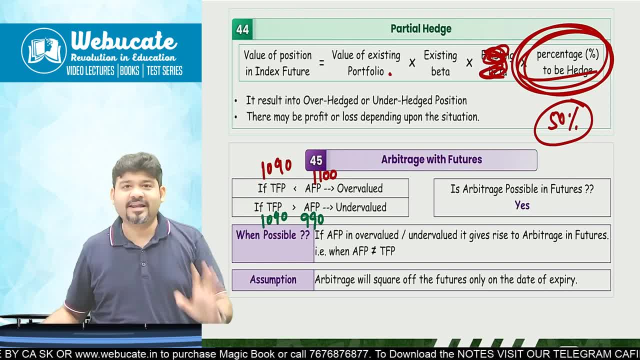 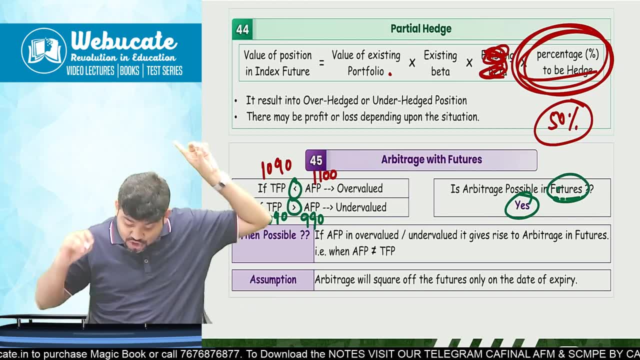 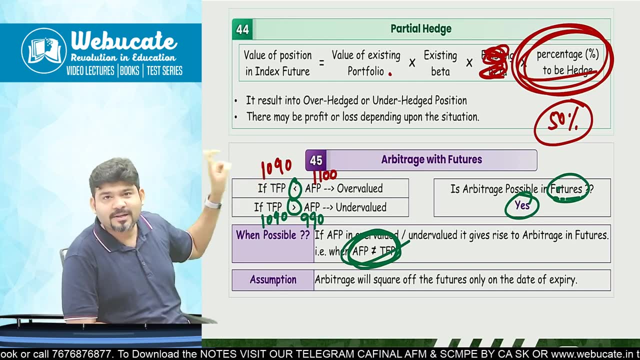 it is undervalued, We will say it is undervalued. Is arbitrage possible in futures? Yes, When when theoretical future price is not equal to actual future price, Theoretical future price, I will calculate spot plus carrying cost, less dividend. Carrying cost can be based on simple. 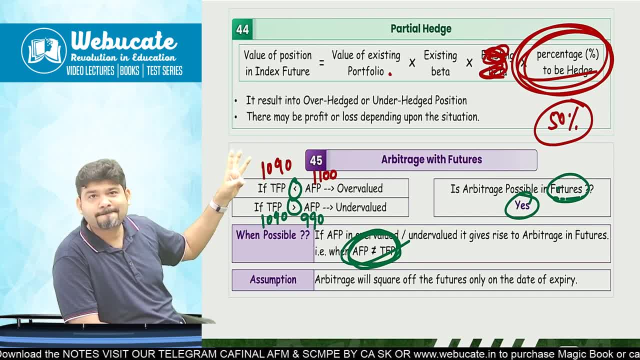 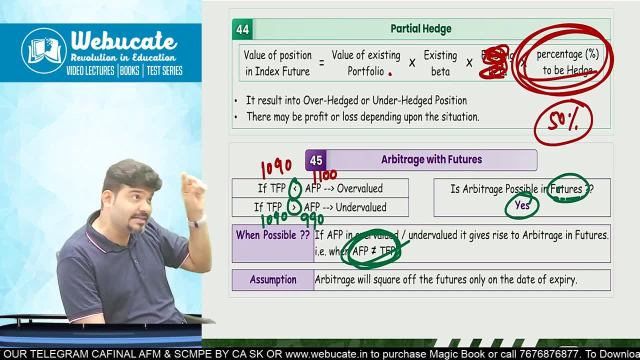 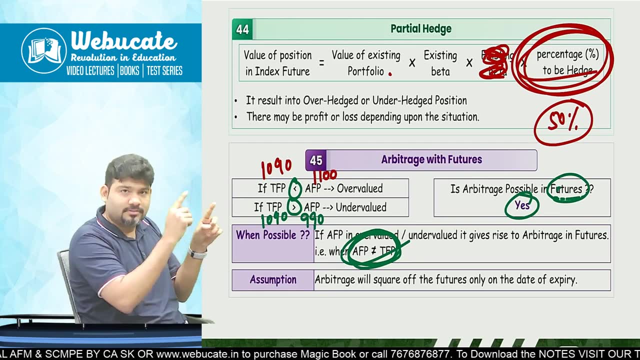 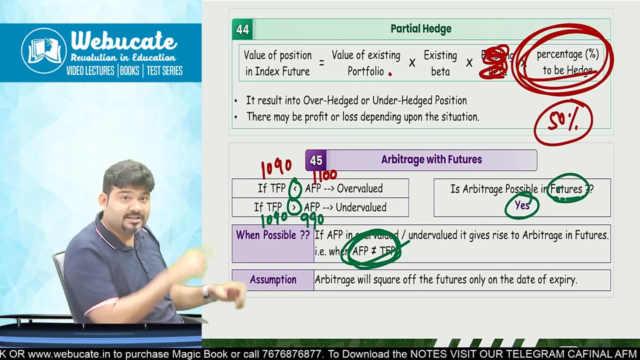 interest. compounding interest. continuous compounding. Simple interest. RT Compounding are: 1 plus S into 1 plus R, raised to T minus D. Continuous compounding with dividend yield 1 plus R minus D raised to T. Continuous compounding S into E raised to RT or S into E. 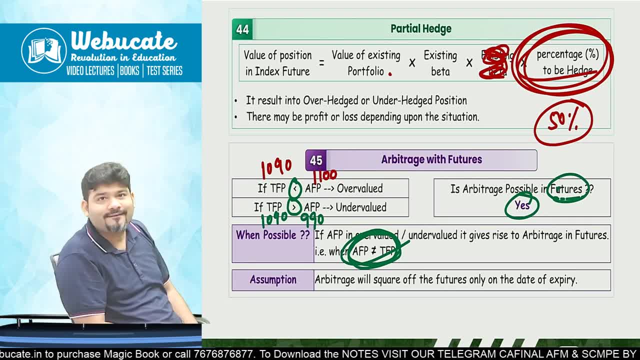 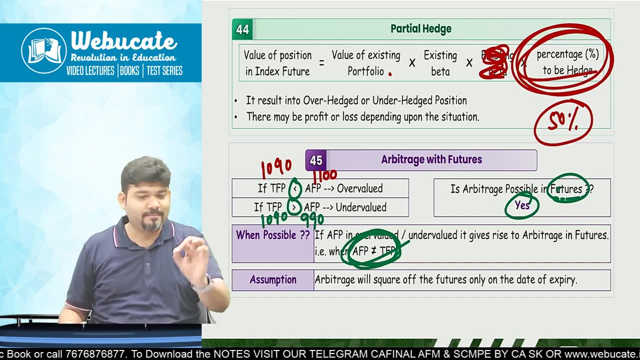 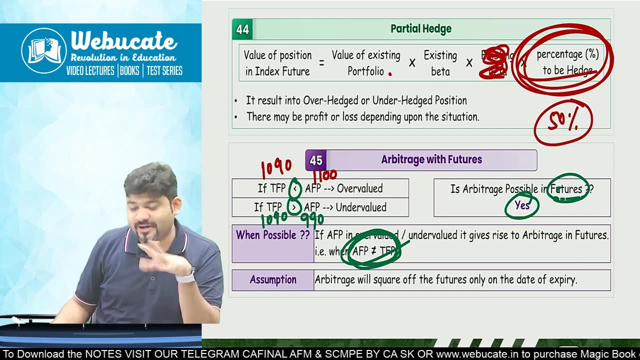 raised to R minus D into T. That is how the whole thing is. That is how clear you should be with your concepts. So profit from market imperfection, correct? So when your actual future price is not equal to theoretical future price, we will say that yes, there is. 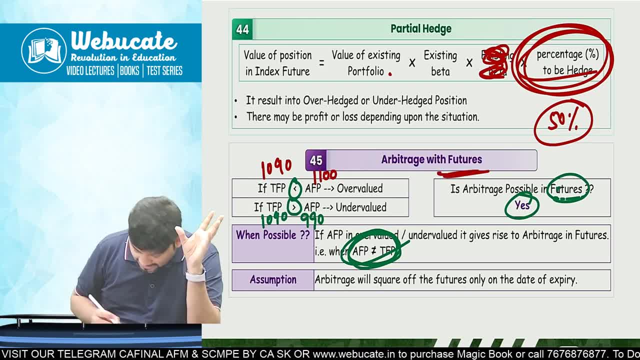 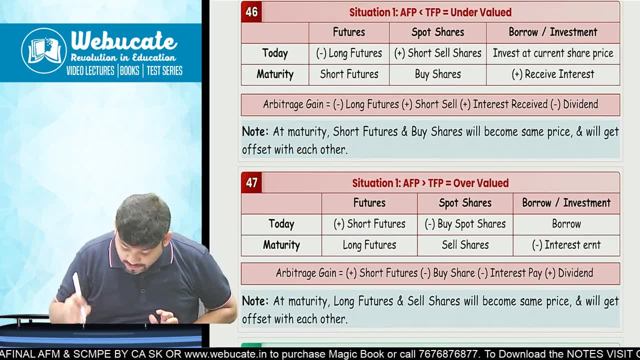 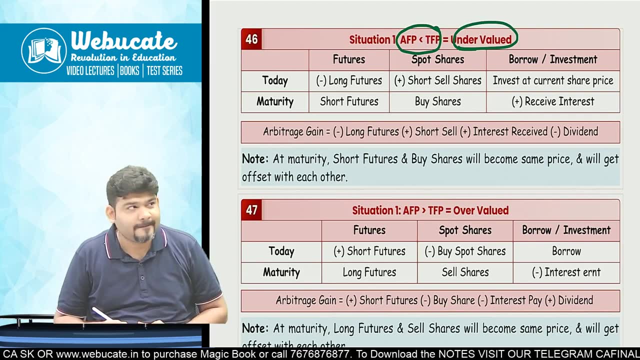 a huge scope for arbitrage. Arbitrage will square of the futures only on the date of expiry. So now we will see. there are two situations which are possible in arbitrage. One, if AFP is less than TFP and it is undervalued situation, And if AFP is greater than TFP. 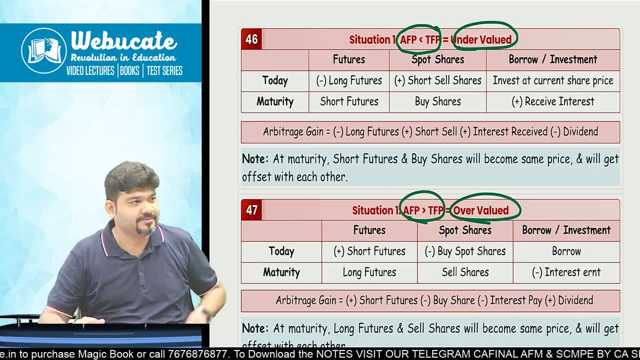 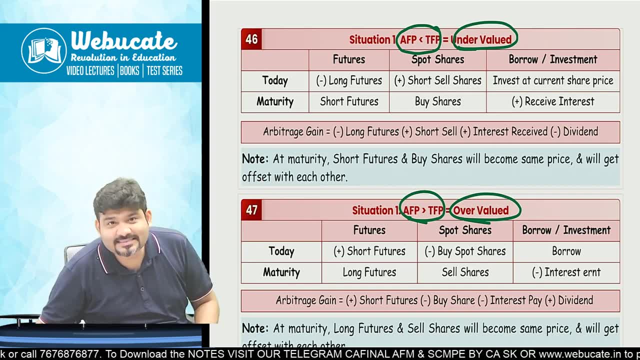 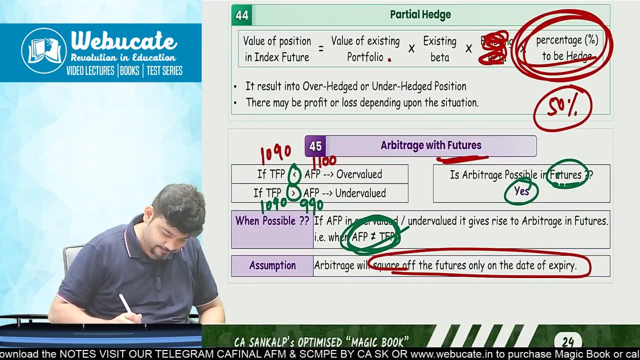 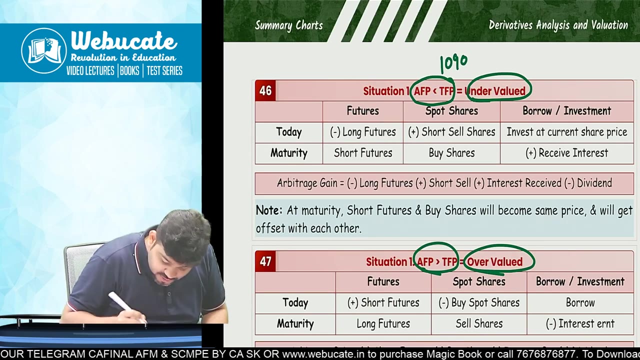 it is a overvalued situation. Yes, So if AFP is less than TFP, what will happen? Suppose if AFP is, say, 1100 or 1090.. Actual future price is, say, 1050.. Hurrah, 50 rupees. there is a full scope, 50 rupees. 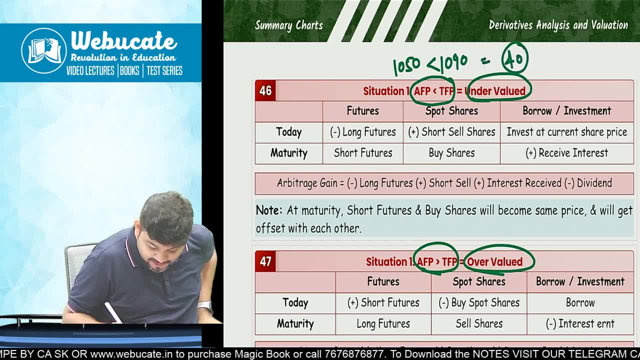 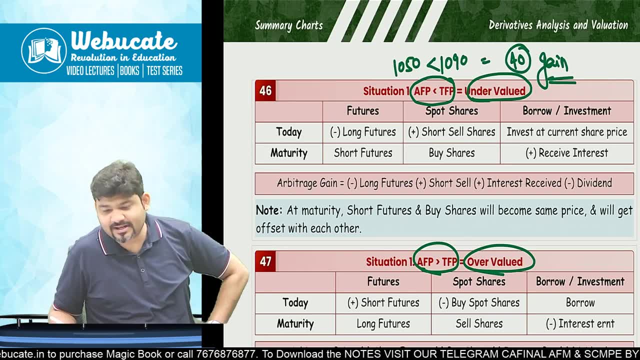 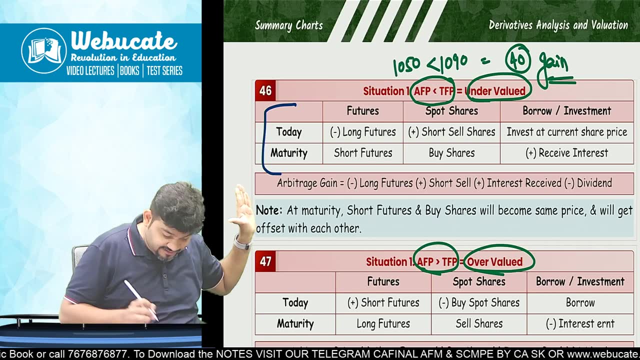 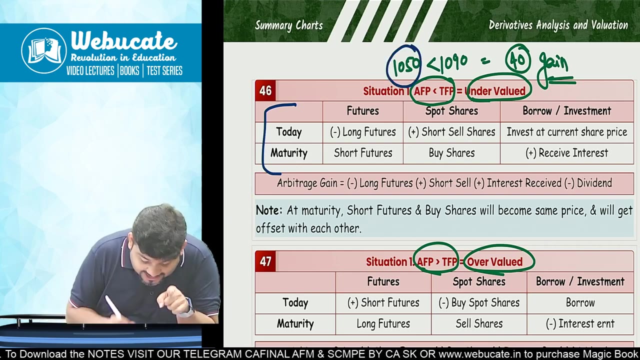 there is a full scope that we will get a profit, or what we call as the gain again. yes, sir, yes, sir. so what is going to happen? pay attention very, very carefully, pay attention very, very carefully. okay, so today you know that you are getting the futures at a less price. 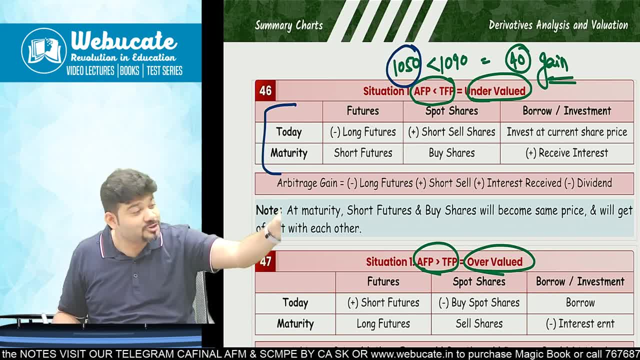 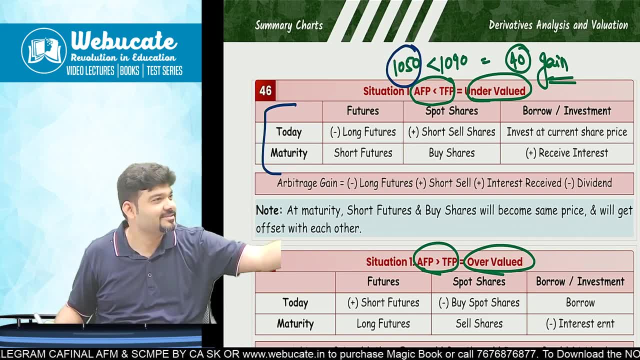 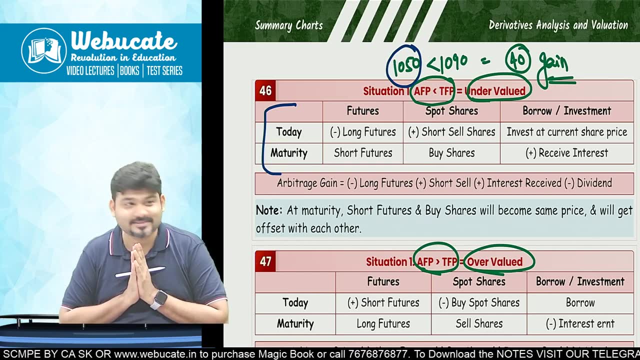 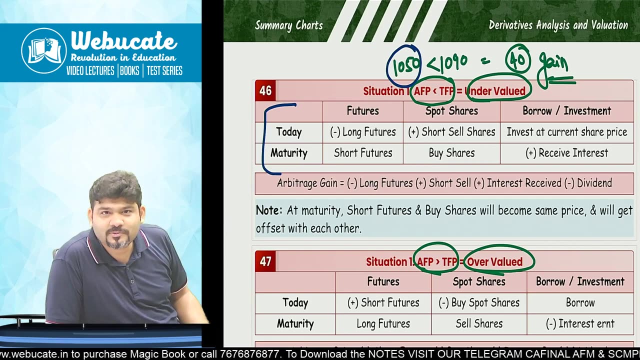 hello, you are getting a futures at a less price. are you understanding my point? my brother, this is tea or coffee, brother, tea or coffee tea. very good, you know english. okay, so some tea on the table. okay, pay attention. now you send me, you know, i'll give you my address, phone number. send it to me. so much tired taking this lecture. 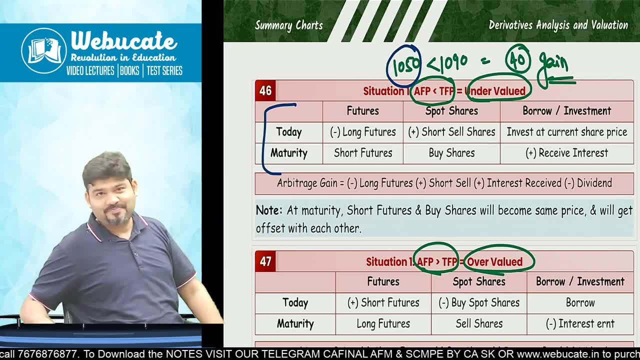 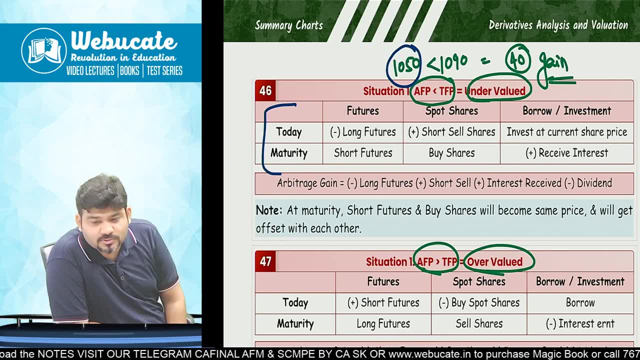 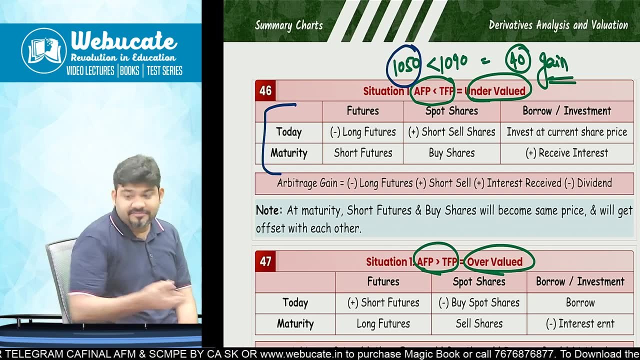 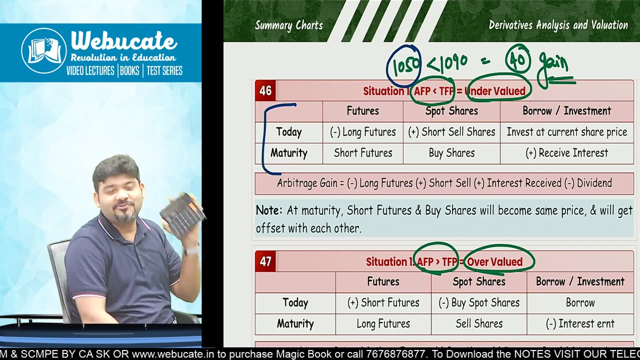 yeah, you'll send it now. afp actual futures price is less than theoretical future price. what is the theoretical future price, sir? it is 1090. actual future price is 1050. so something which is worth 1090 zero, something which is worth 1090 is available at 1050, is available at 1050. 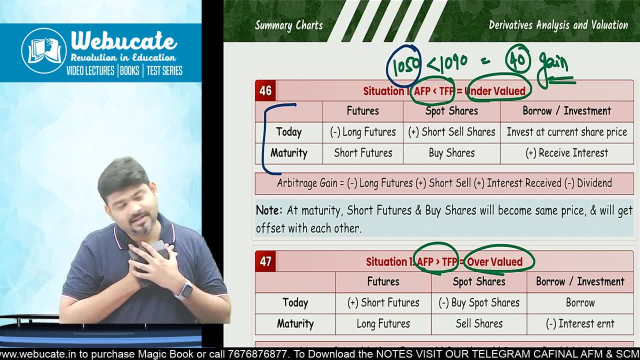 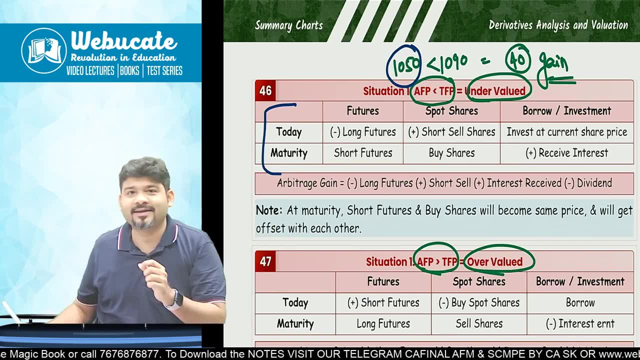 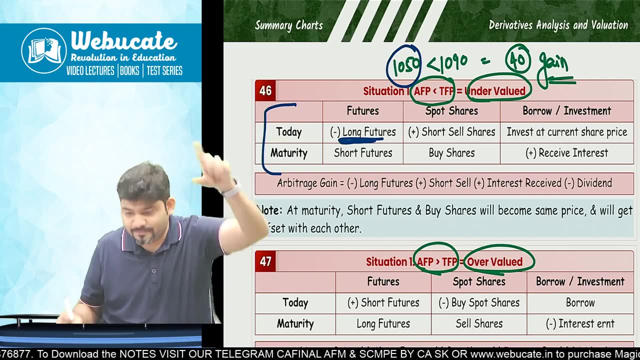 are you clear with this? yes, sir, i am clear with this. so if it is available, actually less price, buy it. meaning: long futures today. when will you long, when will you short? you should know that. if you know this, then done you are through. so you are going to long futures today. but if 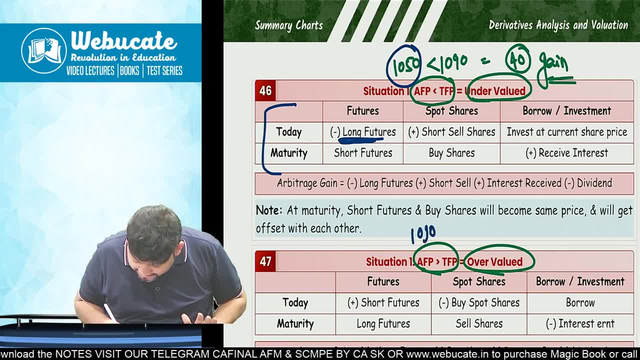 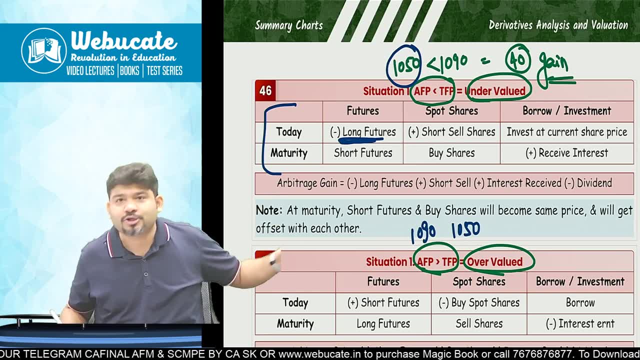 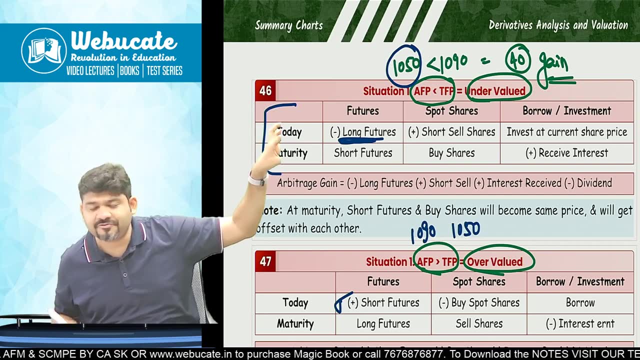 suppose it is opposite. suppose this is 1090 and this is 1050. so what is their actual future? prices are shorted. shorted because you are going to get a better price shorted. are you understanding now the process? today, if you are doing long futures opposite in shares, you will short sell. 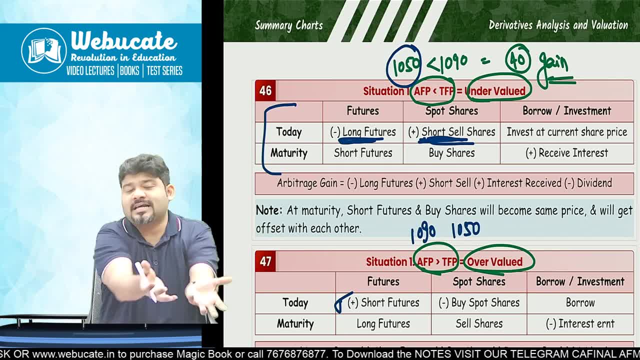 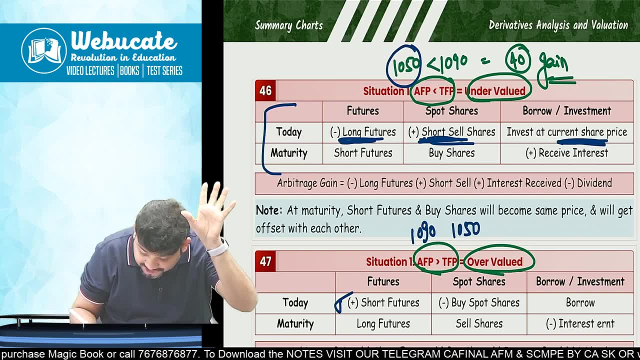 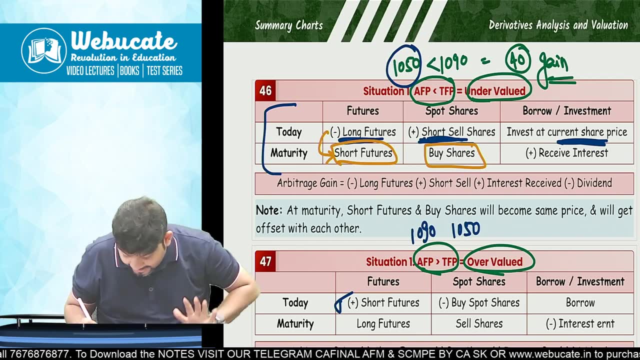 shares okay. as soon as you. short sell says you will get money invested at the current share price. after my on my on the date of maturity, you will have to close the position. short futures: you will have to close the position by shares: okay, and at the same time you will receive interest. so now, 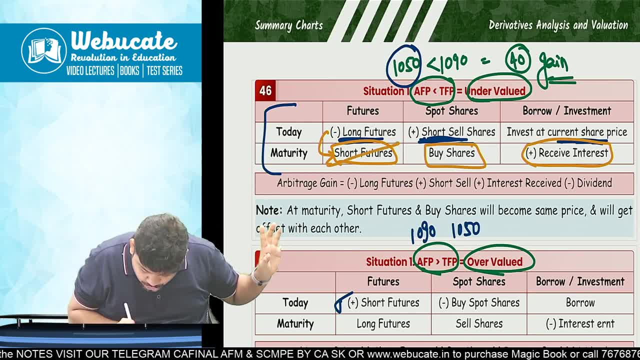 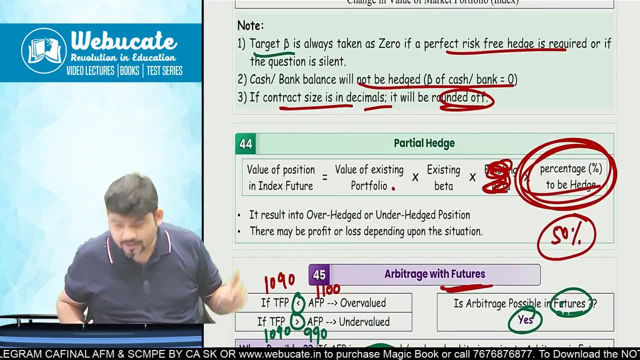 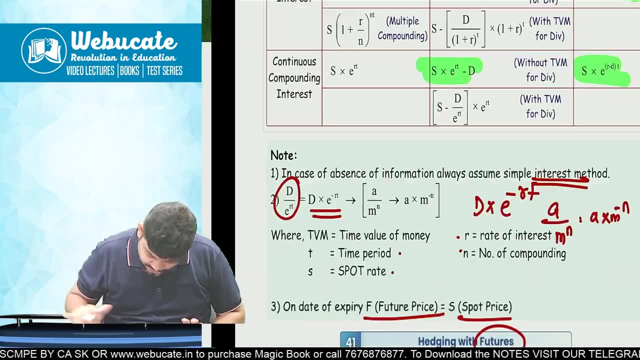 what is going to happen long see this: short futures and buy shares will get cancelled, right, because on the day of expiry, on the day of maturity, on the day of expiry, on the day of maturity, uh, it was written, no, that wait, wait, i'll shoot. on the date of expiry, futures price is equal to spot price, right? so on. 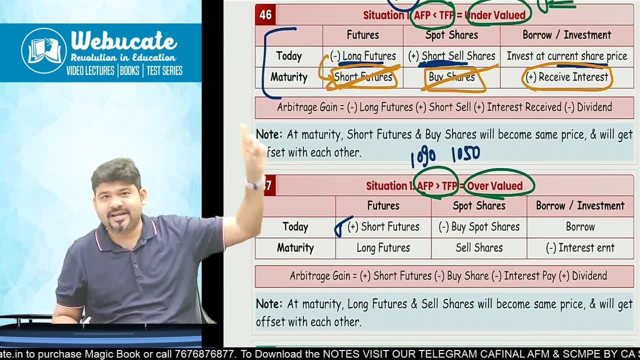 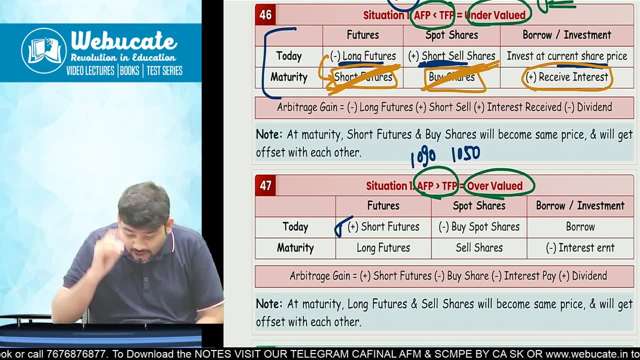 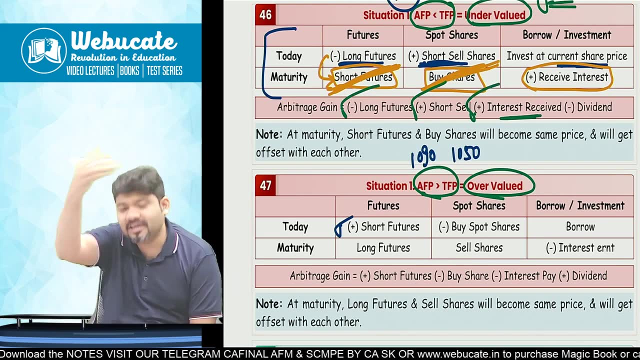 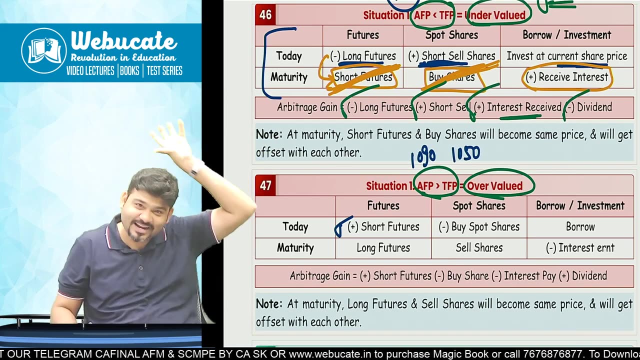 the day of maturity. short futures: buy shares. both price is going to be same. so short futures: money in, buy shares out, cancel. so in all what is left, in all what is left, long futures, short sell, add interest received. if there was any dividend, it will be reduced and finally you will get arbitrage gain. you will get. arbitrage gain and opposite situation here. if you have short futures, you will buy shares. how will you buy shares? by borrowing. if you have borrowed interest, you will have to pay then at the maturity. long futures sell shares will get offset because it's going to be the same price. arbitrage gain will. 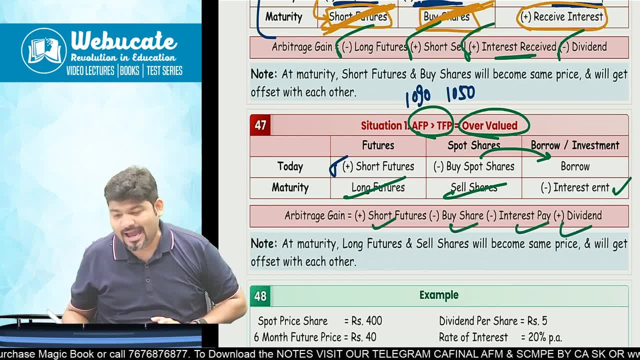 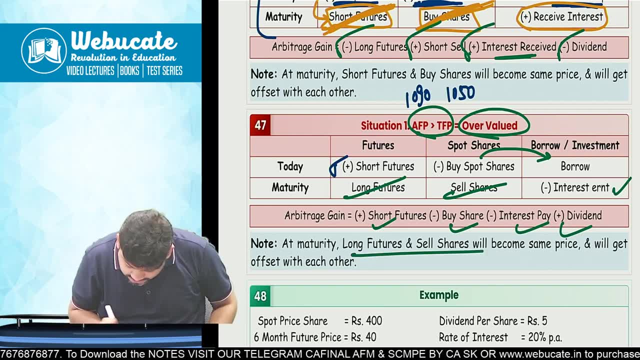 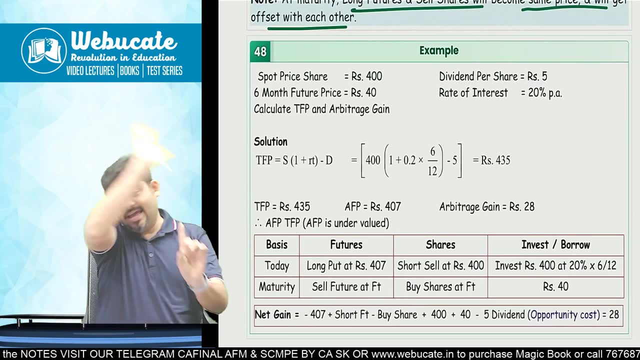 be. short futures, buy spot shares. interest pay and dividend is what you are going to receive at maturity. long futures and shell shares will become same price and will be offset with each other. i will close it with the example, and then we will come to the black and shoals method and the 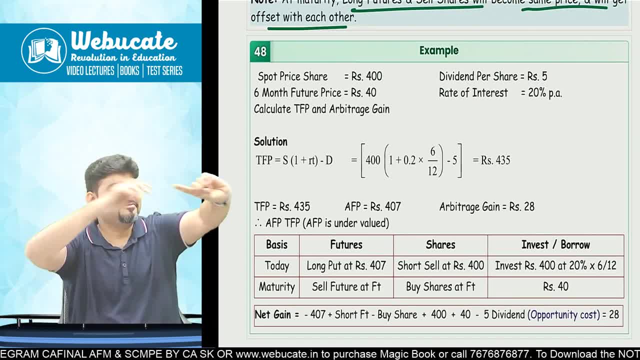 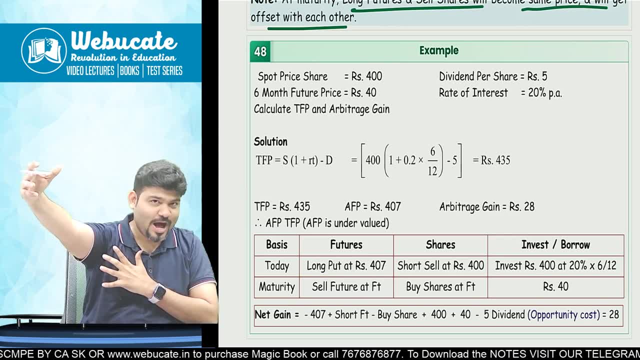 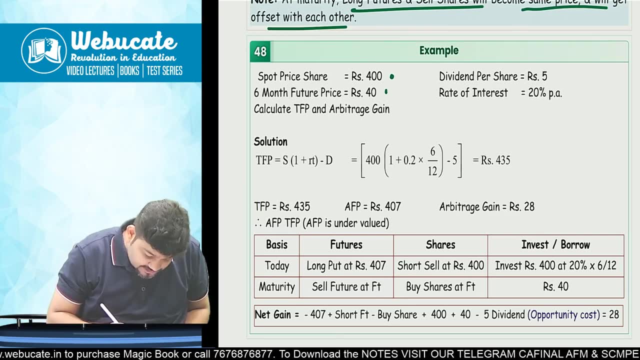 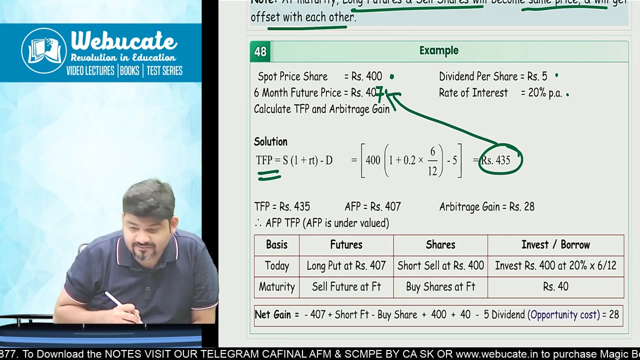 sums of real option. after the real option we will have the abatement option, timing option. so wait and watch now. example: spot price: 400. futures price: uh. six month future price: 407. dividend per share: five. rate of interest: 20. so ideally, what should be the theoretical future price? it should be 435, but it is 407 means. 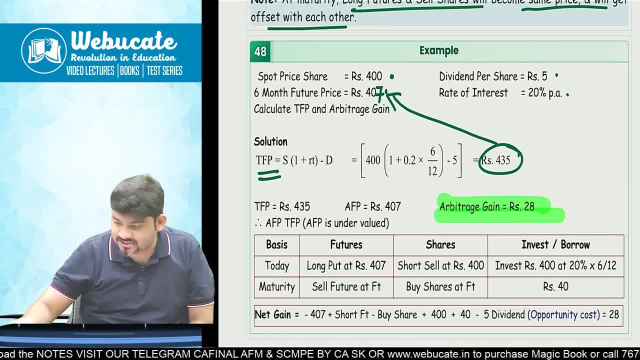 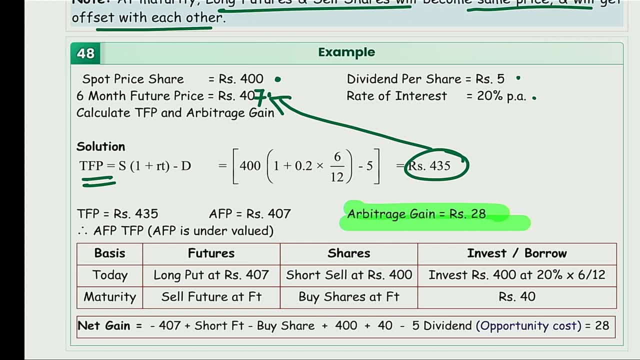 for sure. there is a arbitrage gain of 20% and then we will come to the real option. we will have the real option of 438. let's try and calculate that arbitrage gain. let's try and calculate that arbitrage gain. so first we have to find out that. what is this scenario all about? see, first thing, that you. 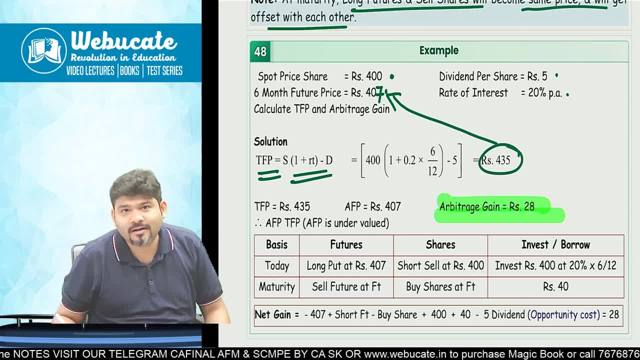 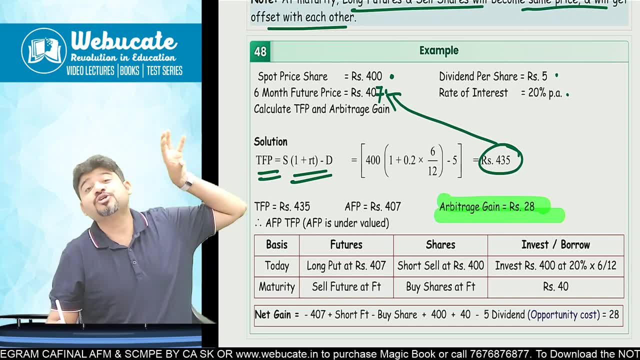 have to see is what is the theoretical future price spot into 1 plus rt, minus dividend will give you 435. 28 is your arbitrage gain. how do you come to know? because futures actual future price is 407, but in market it is that sorry. 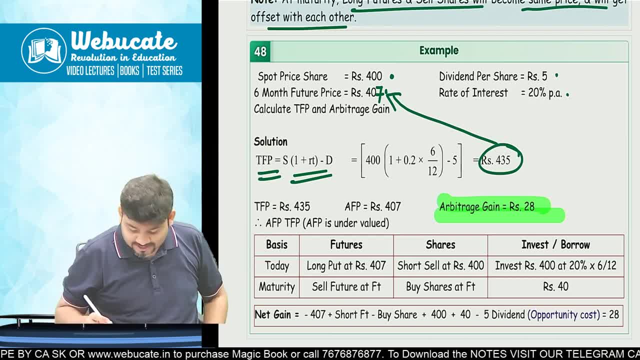 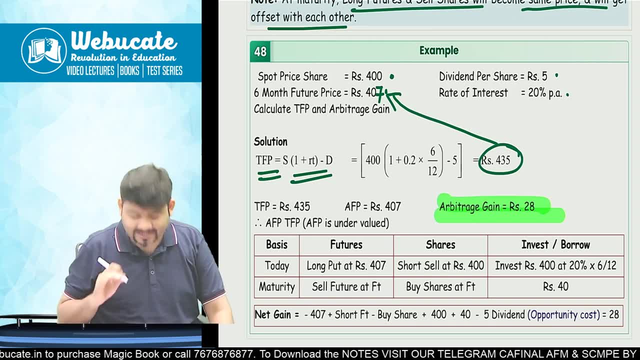 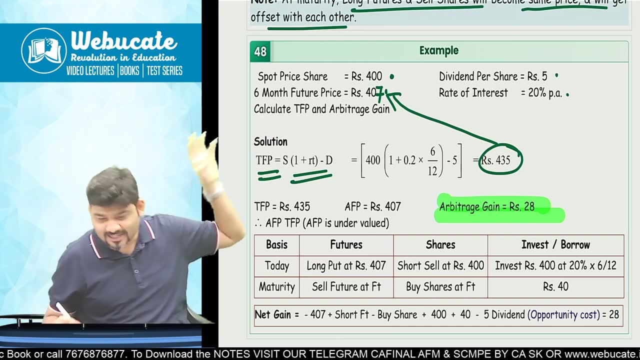 it should be 435, but it is only showing 407. so 28 rupees is your gain. now pay attention. logically, i'm explaining you about the whole formula. is there something that should be 435 is available to you at 407? okay, so arbitrage exists. so what are you going to do? you are going to purchase it right now. 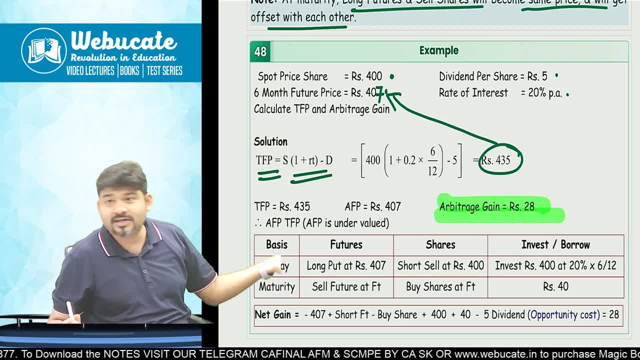 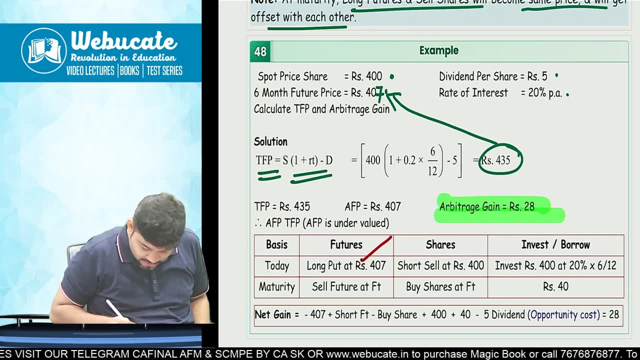 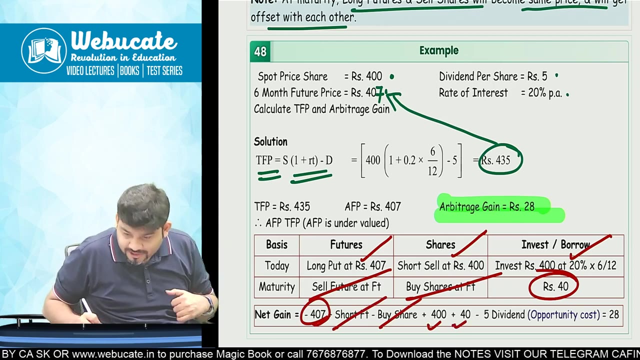 purchase the futures means long futures. long futures means short sell the shares. short sell the shares means invest. invest means you will get the interest. got it long. short sell. invest you will get the interest. buy, sell, share sell offset. so, uh, four minus 407, this will offset 400. is your selling of shares getting money which you invested on 40 rupees?